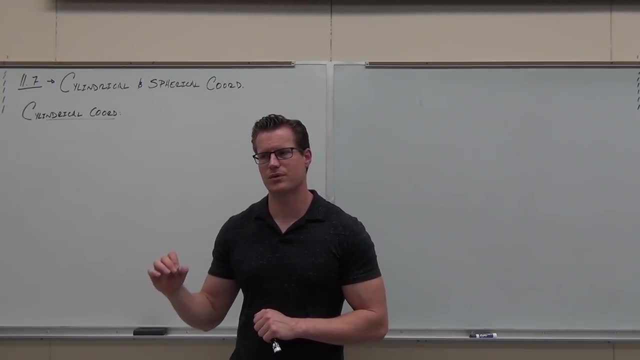 It's going to make really hard integrals easier, at least easier. I'm not going to say easy, but at least easier. You guys understand the idea behind doing it. That's the idea. Now, how it works. we're going to start with cylindrical coordinates and we're going to take off and do spherical. 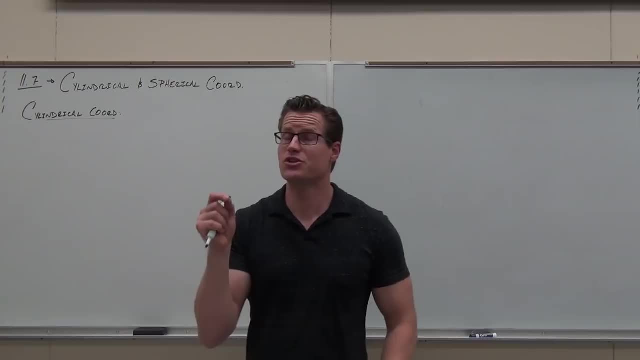 Cylindrical coordinates. they literally are just like polar coordinates. Do you remember? Do you remember polar coordinates, Section 10.3, I think, from Calculus 2, polar coordinates, maybe 10.4,, no 10.4,, one of those two ones. 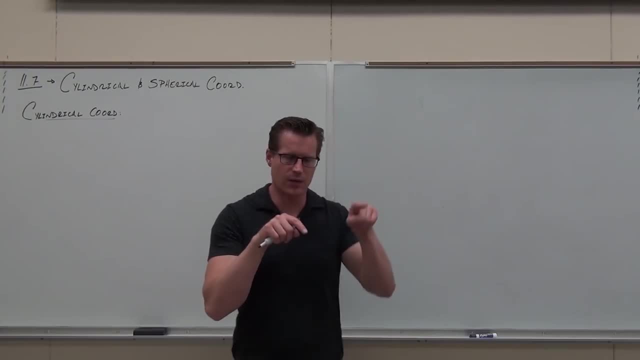 Polar coordinates. they're not the same thing as rectangular x, y. What they did was they said: I want to give you an angle to the x-axis or the polar axis and then shoot you off just like that, a radius. 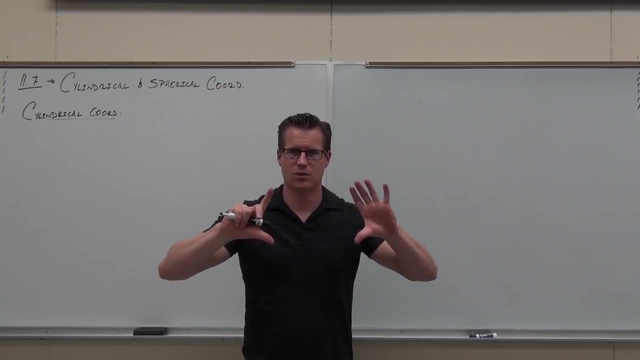 That's what they did. It was on the x y plane, though. Do you remember that It was on the x y plane? This is just like polar on the. please listen carefully. I don't want to lose you. 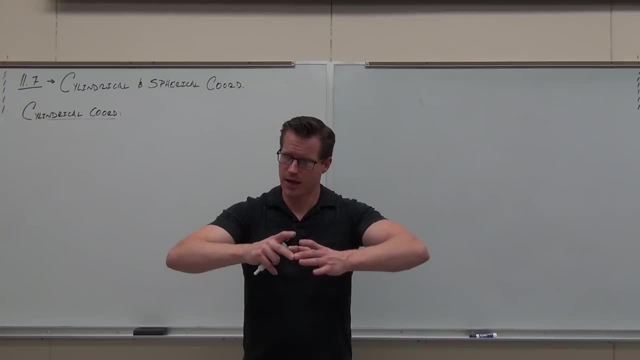 Cylindrical deals with r and theta and it's still on the x- y plane. That's this one. It's just that we have to add a z component. So what's going to happen is we're going to have this polar representation on the x- y plane and say, hey, right where that is on the polar coordinate system, right where that is. we're just going to take that and raise it up along the z-axis. 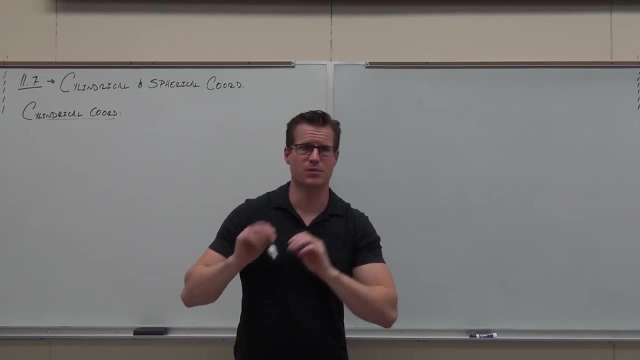 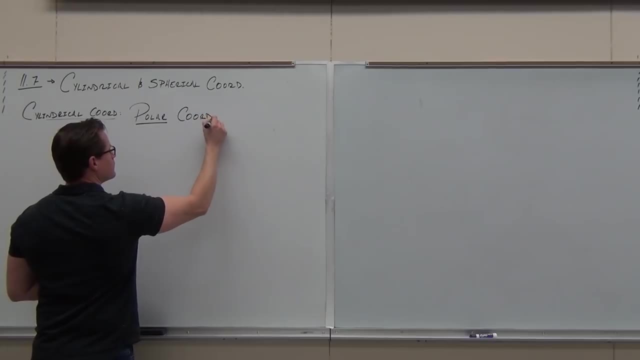 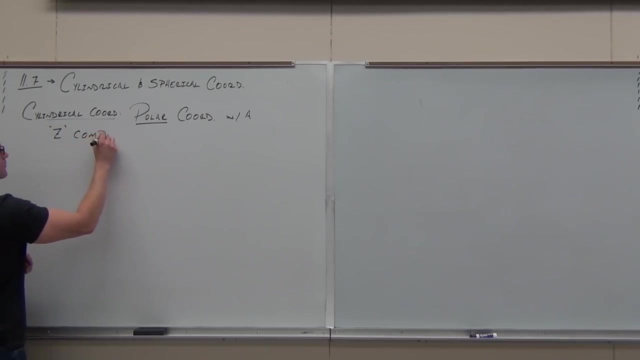 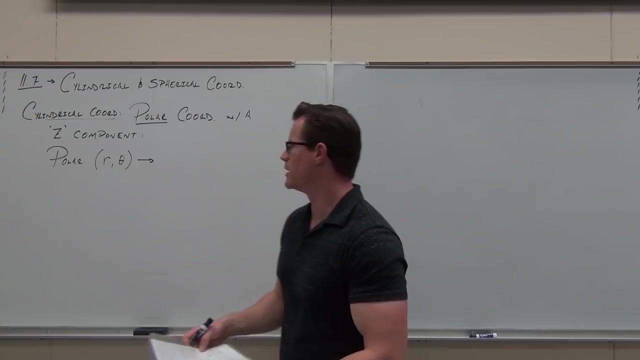 That's how cylindrical works. It is polar with a z component. Let me show you. So here's polar Polar. Polar is on a plane. Polar is on. typically we think of the x? y plane. It was just a projection onto that x? y plane. 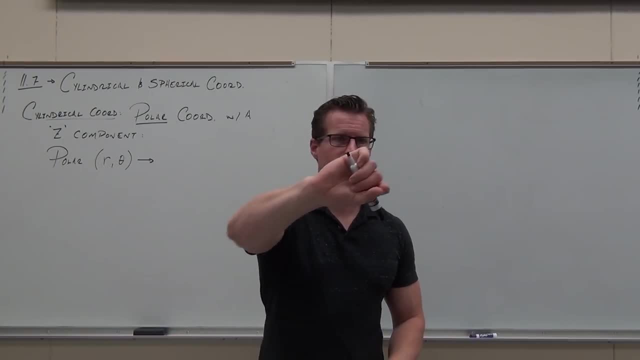 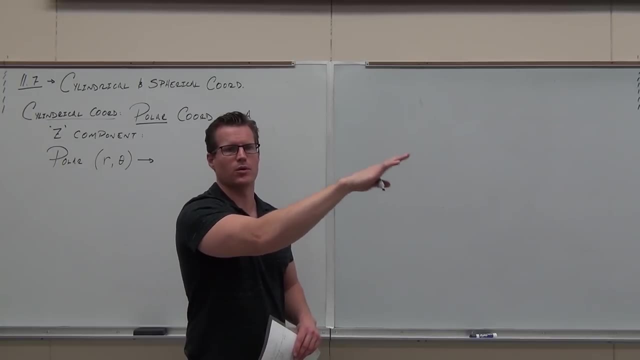 Polar had r representing the radius to whatever away from the origin that we have, and theta is the positive angle from or negative angle, but it's the angle from the polar axis. We think of the x-axis, It's still the x-axis. 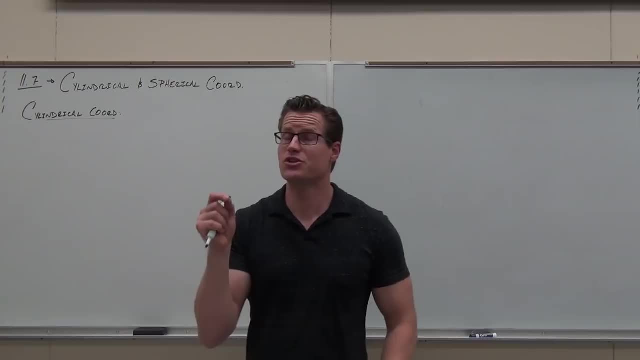 Cylindrical coordinates. they literally are just like polar coordinates. Do you remember? Do you remember polar coordinates, Section 10.3, I think, from Calculus 2, polar coordinates, maybe 10.4,, no 10.4,, one of those two ones. 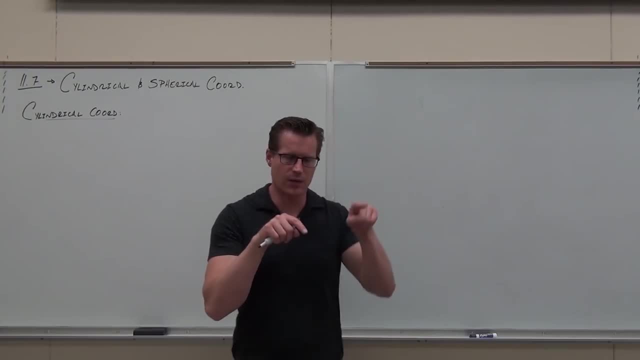 Polar coordinates. they're not the same thing as rectangular x, y. What they did was they said: I want to give you an angle to the x-axis or the polar axis and then shoot you off just like that, a radius. 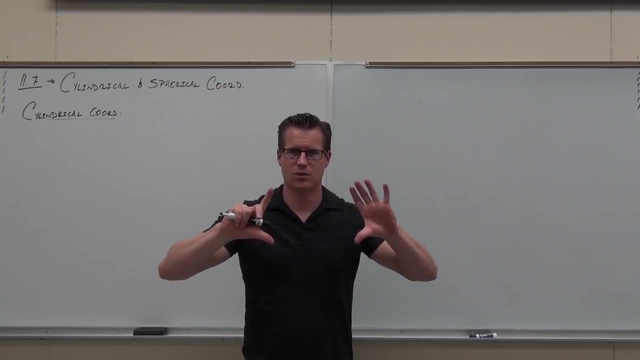 That's what they did. It was on the x y plane, though. Do you remember that It was on the x y plane? This is just like polar on the. please listen carefully. I don't want to lose you. 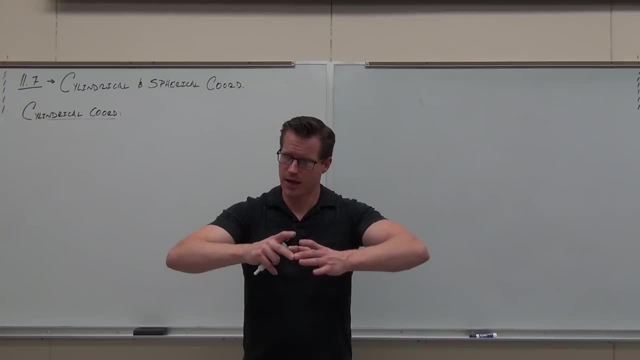 Cylindrical deals with r and theta and it's still on the x- y plane. That's this one. It's just that we have to add a z component. So what's going to happen is we're going to have this polar representation on the x- y plane and say, hey, right where that is on the polar coordinate system, right where that is. we're just going to take that and raise it up along the z-axis. 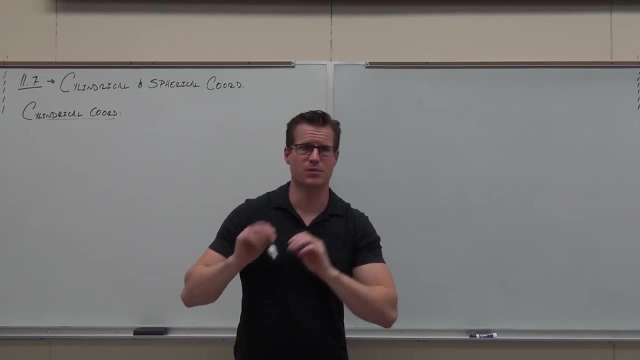 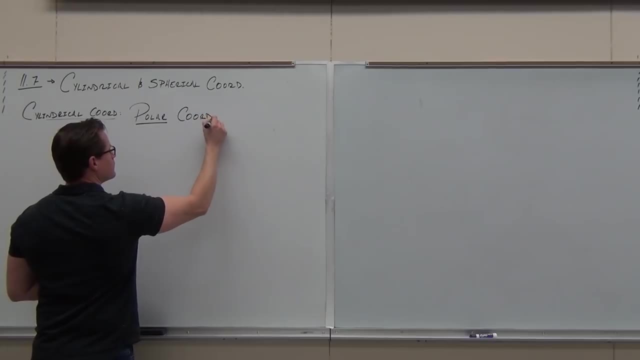 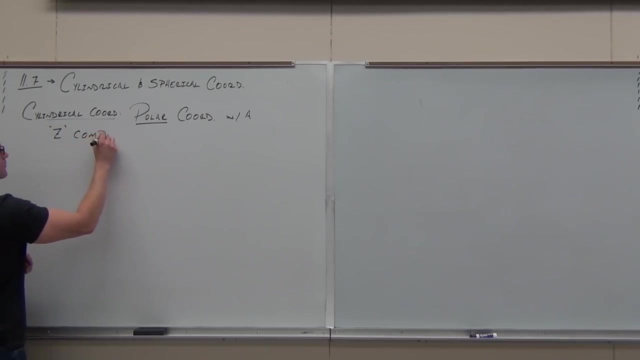 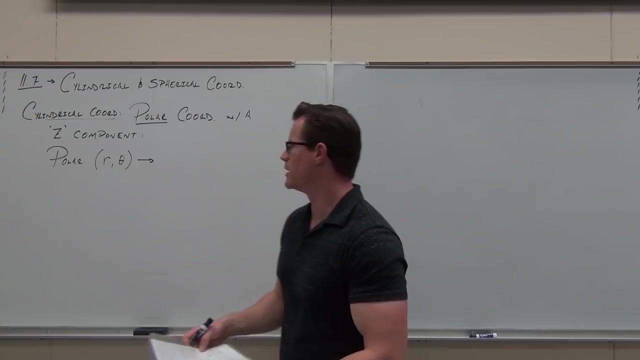 That's how cylindrical works. It is polar with a z component. Let me show you. So here's polar Polar. Polar is on a plane. Polar is on. typically we think of the x? y plane. It was just a projection onto that x? y plane. 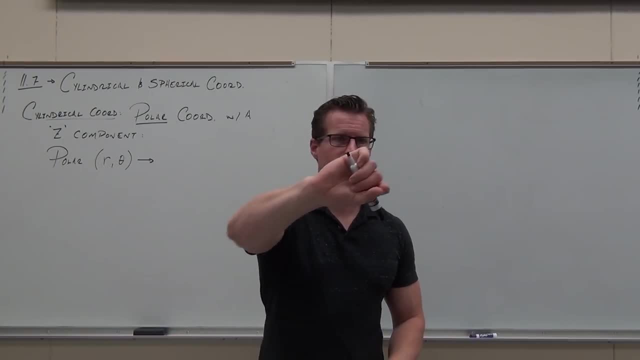 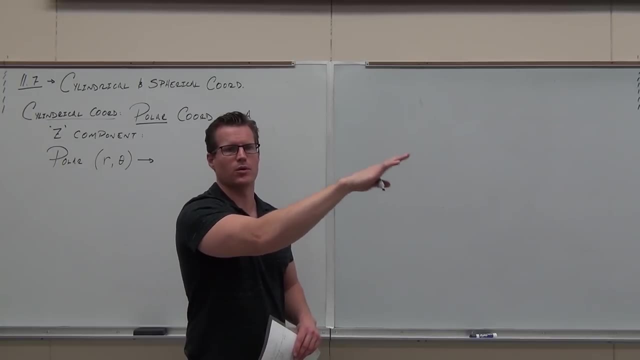 Polar had r representing the radius to whatever away from the origin that we have, and theta is the positive angle from or negative angle, but it's the angle from the polar axis. We think of the x-axis, It's still the x-axis. 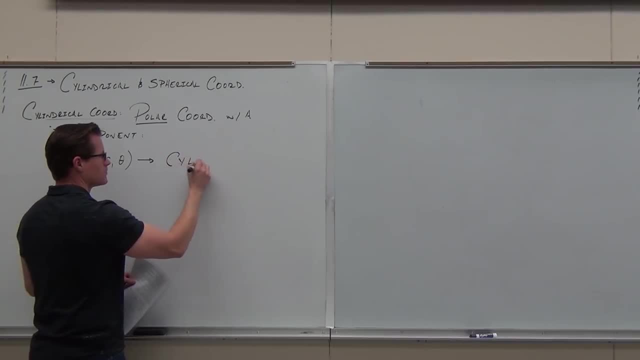 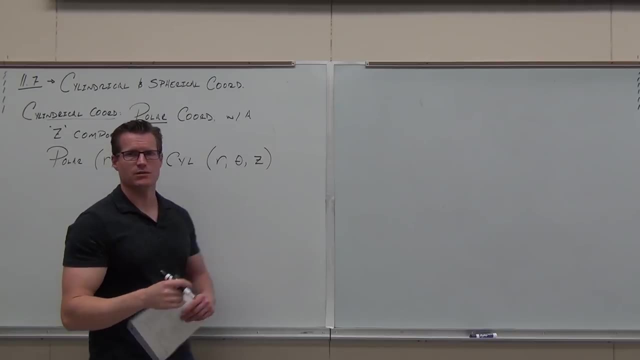 If we want to change the cylindrical. it's even the same order. We still have an r, We still got a theta, But now we have something that gives us this 3D coordinate system. that's not the x, y, z coordinate system. 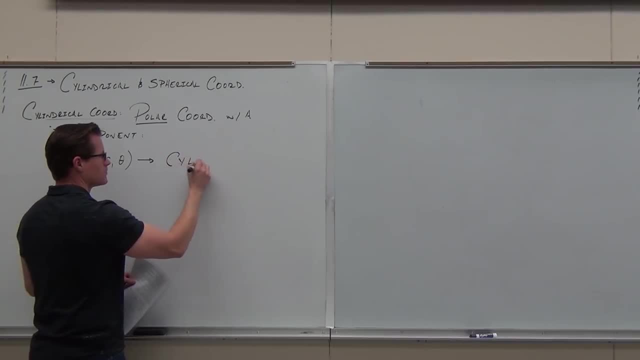 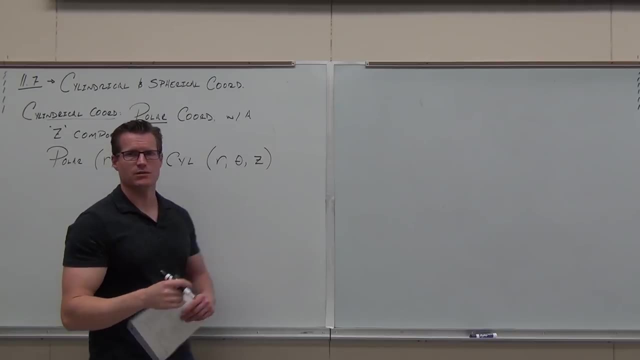 If we want to change the cylindrical. it's even the same order. We still have an r, We still got a theta, But now we have something that gives us this 3D coordinate system. that's not the x, y, z coordinate system. 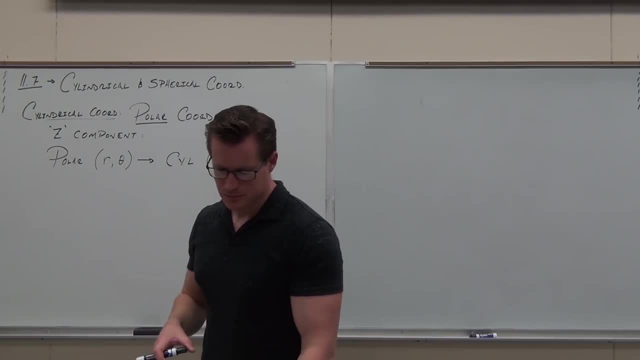 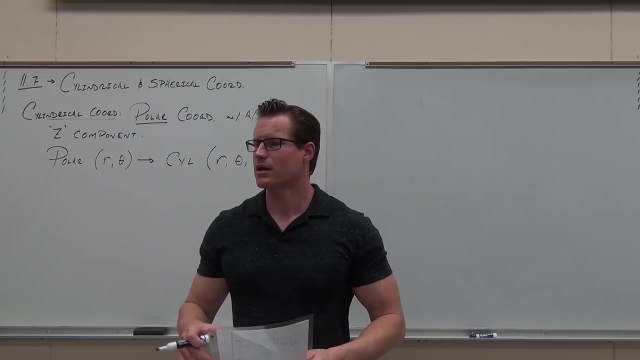 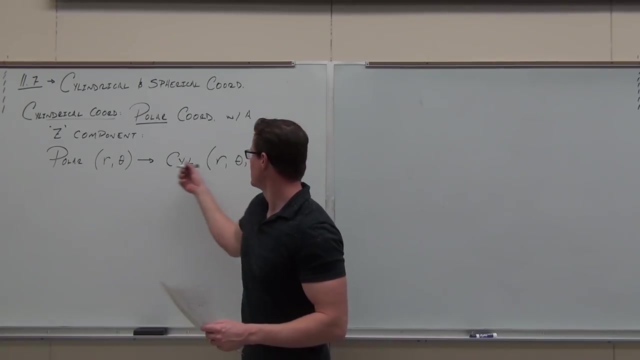 It's r, theta and z. What's even better, even nice, even more better. what's even more better about this is that all the stuff that allows you to translate from rectangular to polar, since the z is the only new thing, it all still works. 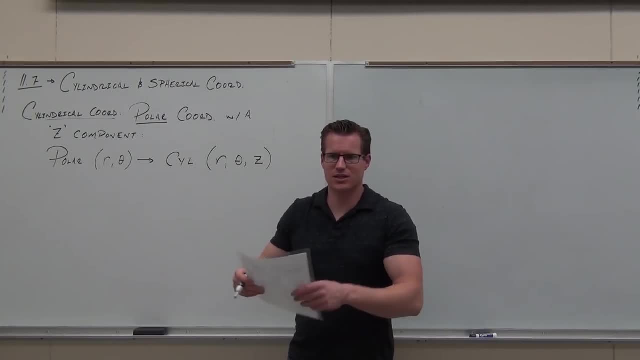 Exactly the same. The z just says: hey, you're on the polar, Now you're lifted up on the z or you're pushed down on the z. So all the stuff we use to translate between rectangular and polar is exactly the stuff we use to translate between rectangular and cylindrical. 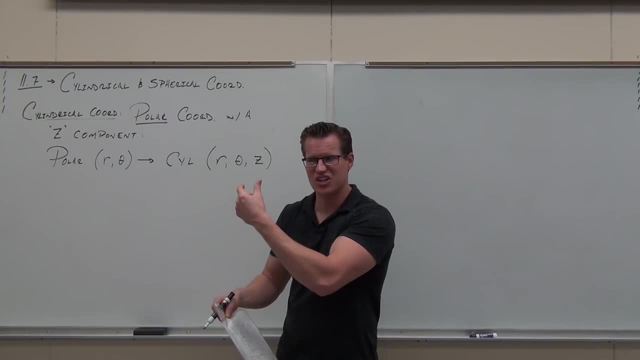 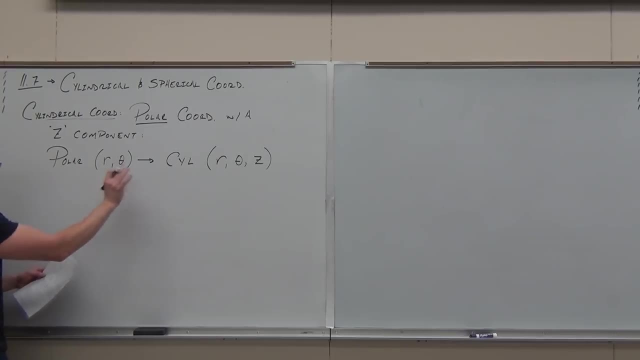 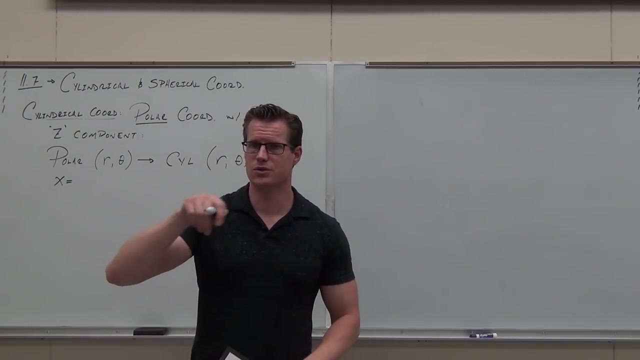 And you're going to like it, because the z coordinate just doesn't change. Z is z, You'll see it. So the same identities hold true, Same stuff for both of these. Now, if you don't remember them, Now, if you don't remember them, you can always think back to some trigonometry and do some right triangle trigonometry to get these. 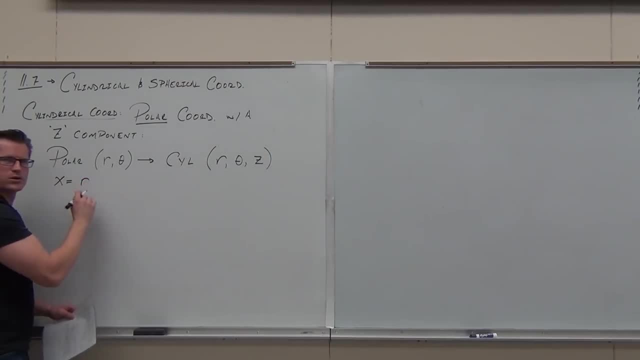 But x was always represented as r Cosine. Oh, do you remember x Cosine, Cosine, that's right. Y come on, R sine, R sine, Beautiful. So check it out. Here's what I'm talking about. 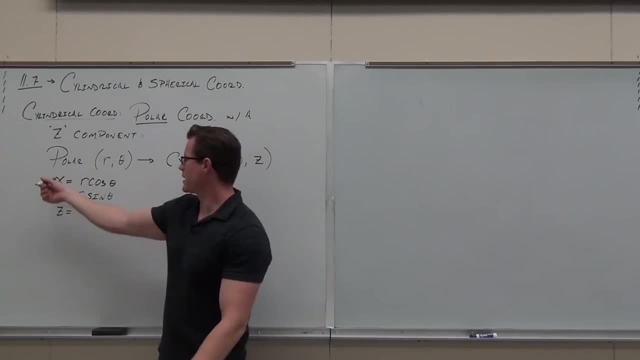 In 3D, the R3 coordinate system. we have x's, we've got y's, we've got z's. We've got a way to translate x's: it's r cosine theta. We've got a way to translate y's: it's r sine theta. 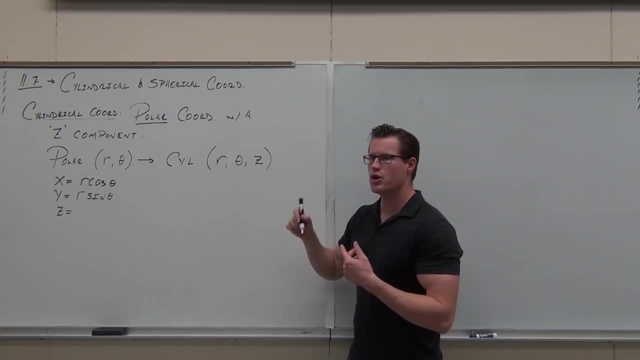 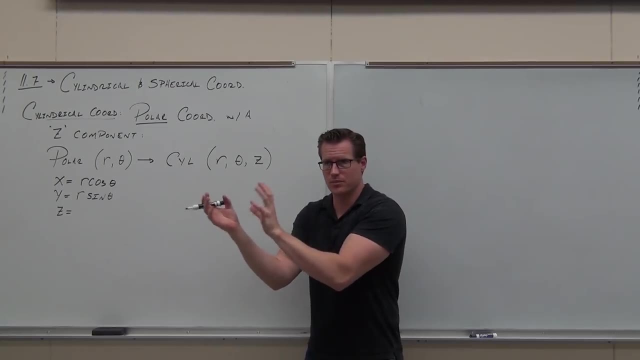 Do we need to translate z's? No, No, The z is the z, The height is still the height. That's really nice. That's what I'm talking about. The polar changiness is the cylindrical changiness, Z. just let z equal z. 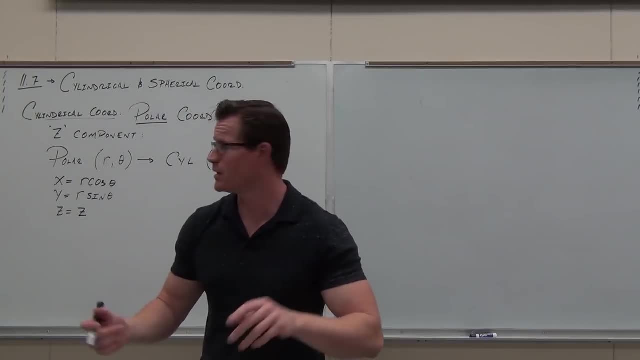 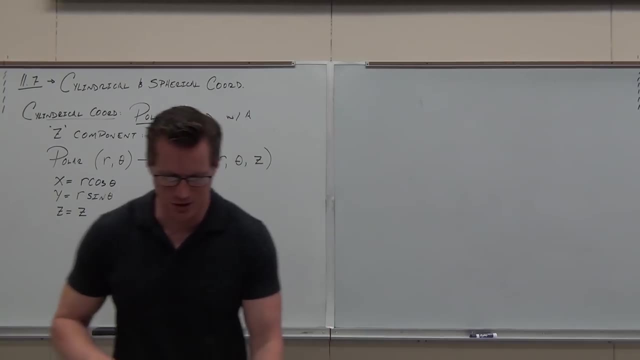 It's still giving you the height above the xy plane. This z is giving you the height above the xy plane- Same z And not, if you're with me, on the same z. That's pretty cool. It's pretty easy to do. 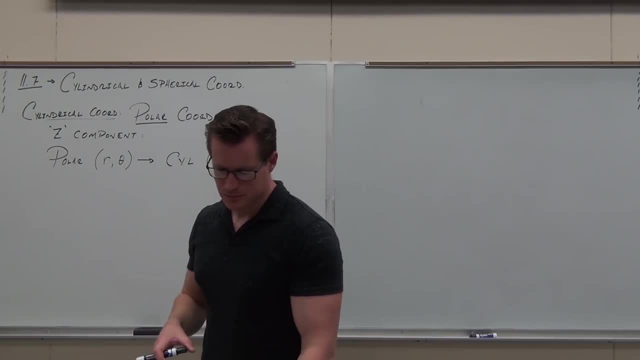 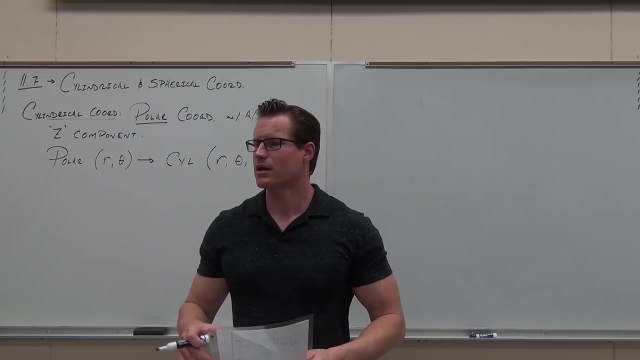 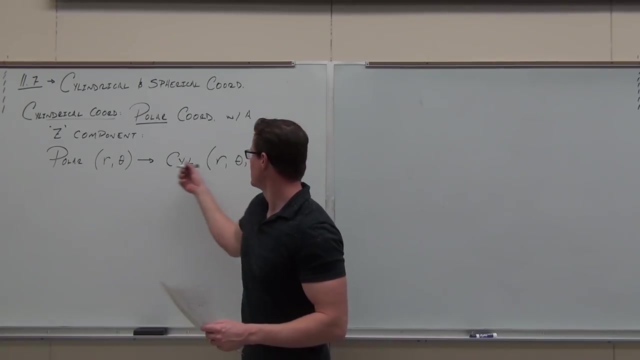 It's r, theta and z. What's even better, even nice, even more better. what's even more better about this is that all the stuff that allows you to translate from rectangular to polar, since the z is the only new thing, it all still works. 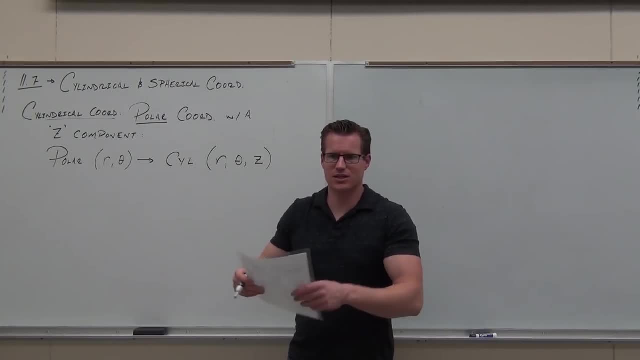 Exactly the same. The z just says: hey, you're on the polar, Now you're lifted up on the z or you're pushed down on the z. So all the stuff we use to translate between rectangular and polar is exactly the stuff we use to translate between rectangular and cylindrical. 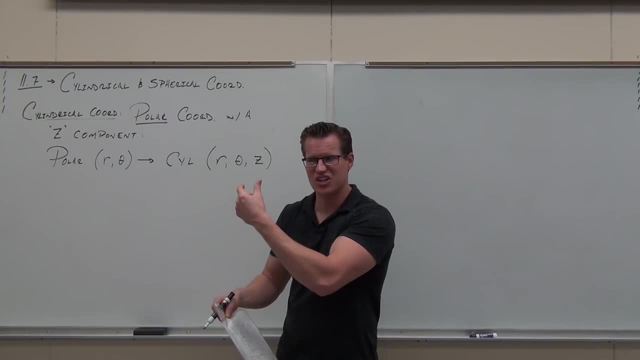 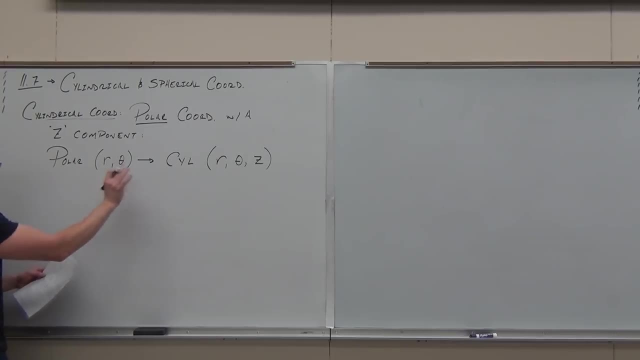 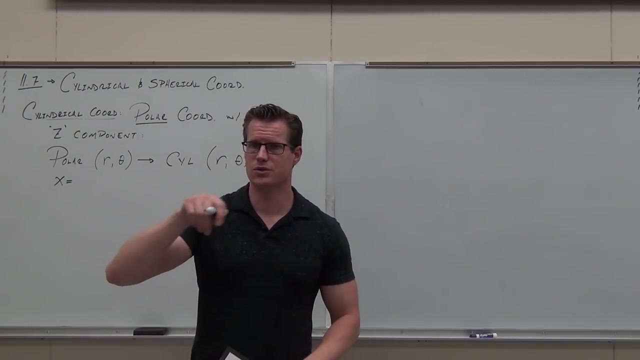 And you're going to like it, because the z coordinate just doesn't change. Z is z, You'll see it. So the same identities hold true, Same stuff for both of these. Now, if you don't remember them, Now, if you don't remember them, you can always think back to some trigonometry and do some right triangle trigonometry to get these. 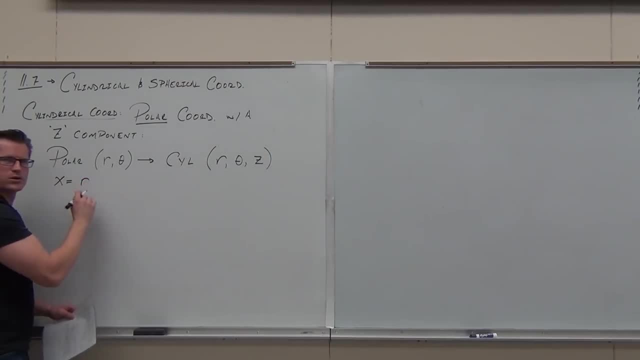 But x was always represented as r Cosine. Oh, do you remember x Cosine, Cosine, that's right. Y come on, R sine, R sine, Beautiful. So check it out. Here's what I'm talking about. 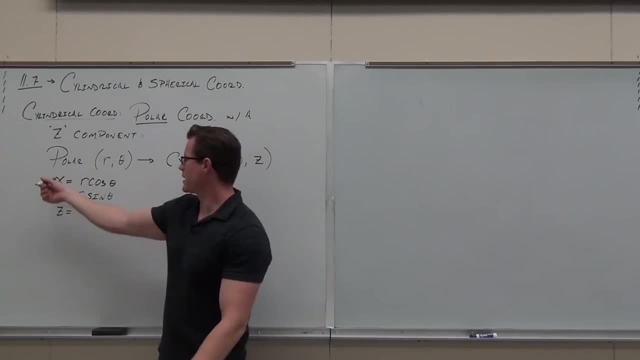 In 3D, the R3 coordinate system. we have x's, we've got y's, we've got z's. We've got a way to translate x's: it's r cosine theta. We've got a way to translate y's: it's r sine theta. 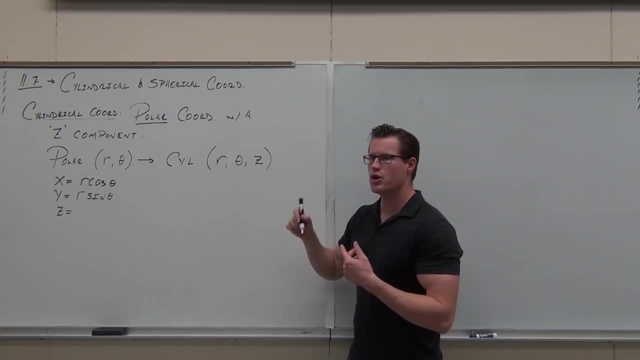 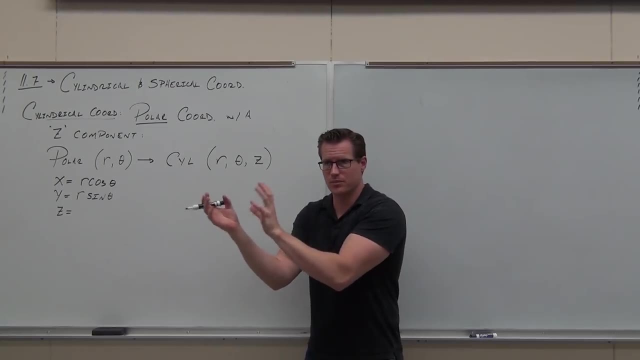 Do we need to translate z's? No, No, The z is the z, The height is still the height. That's really nice. That's what I'm talking about. The polar changiness is the cylindrical changiness, Z. just let z equal z. 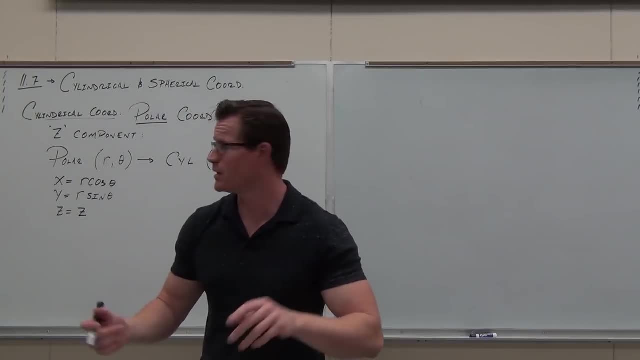 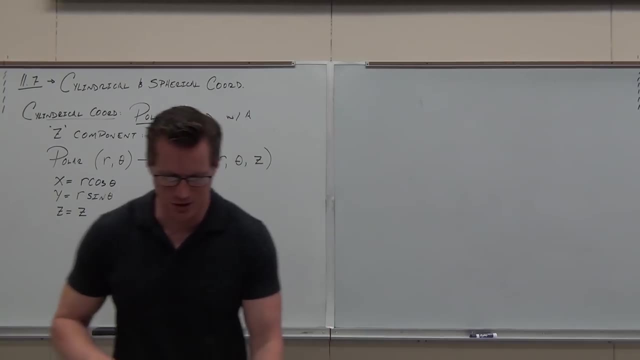 It's still giving you the height above the xy plane. This z is giving you the height above the xy plane- Same z And not, if you're with me, on the same z. That's pretty cool. It's pretty easy to do. 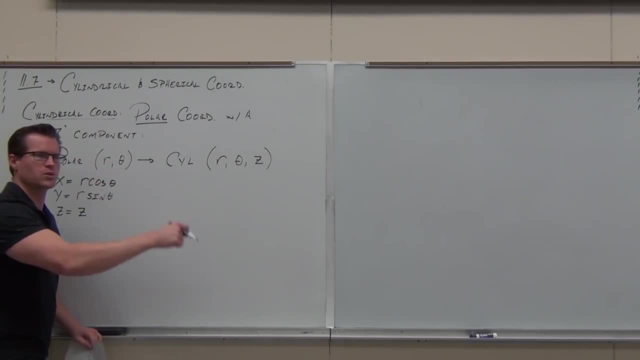 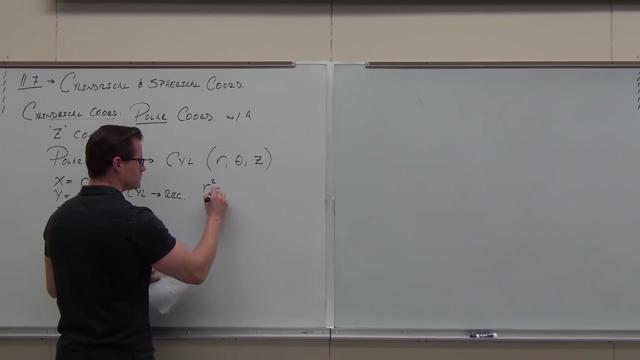 We use these identities to go from cylindrical to rectangular. You plug in cylindrical, you get rectangular. So this is used for cylindrical to rectangular. If we need to go back from rectangular to cylindrical, we use this second set. This is just Pythagorean identity. right triangle trigonometry. 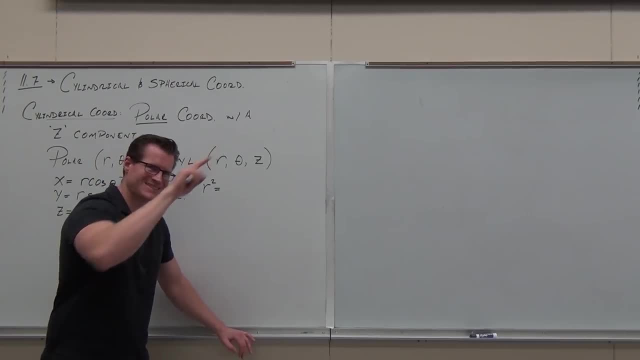 Do you remember how much r squared is? If r is the little radius, the hypotenuse if you will, how much would it be? r would be the square root, But r squared would be x squared plus y squared. We also know a couple other things. 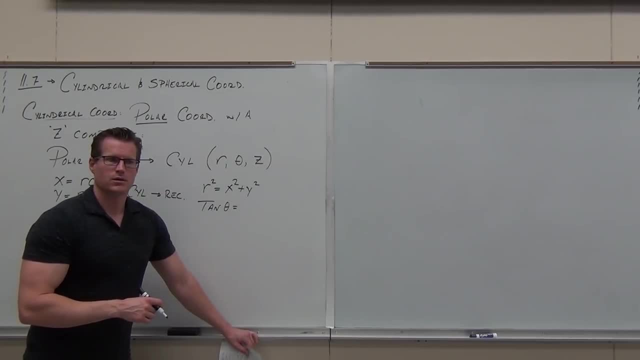 Tangent theta. we always define this as Y over x. Well, sine over cosine. But if sine is the y and the x is Y over x, Y over x, And then hey, how much is z? Z is z. 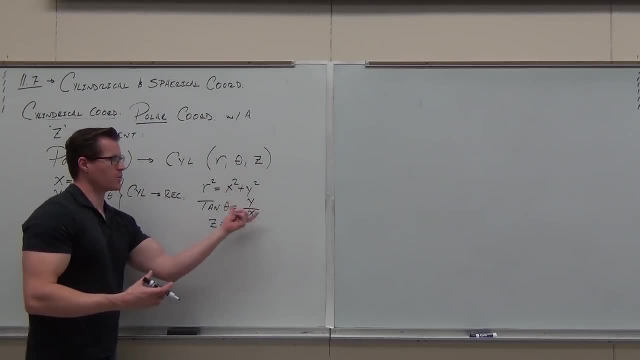 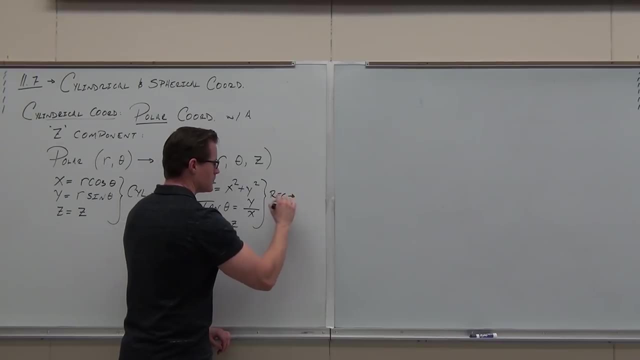 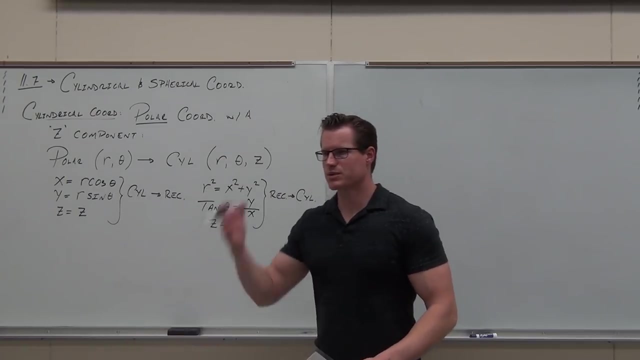 Because there's no change there. This is how you would go from rectangular to polar- Sorry, cylindrical, Same thing. A couple notes. We got a couple examples. Literally, the only like few things I want you to do is this: 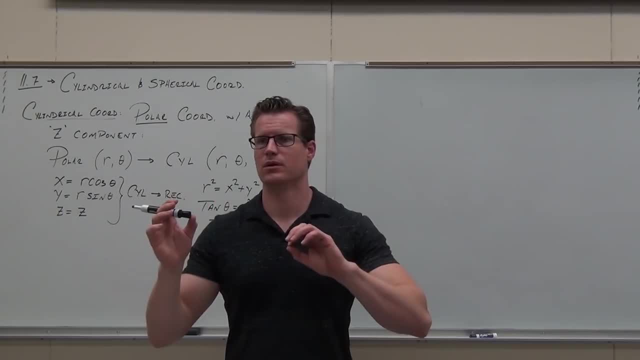 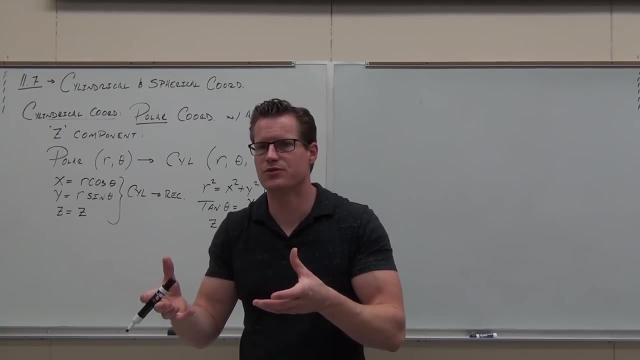 Be able to translate back and forth from rectangular to cylindrical, from rectangular to spherical- We haven't got there yet- From cylindrical to spherical, from spherical to cylindrical, And then be able to change some equations from rectangular equations into like cylindrical or spherical. 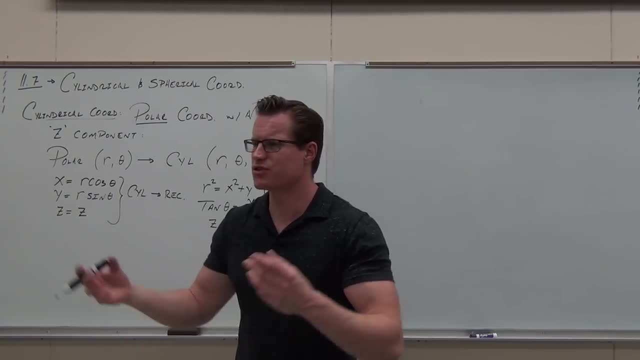 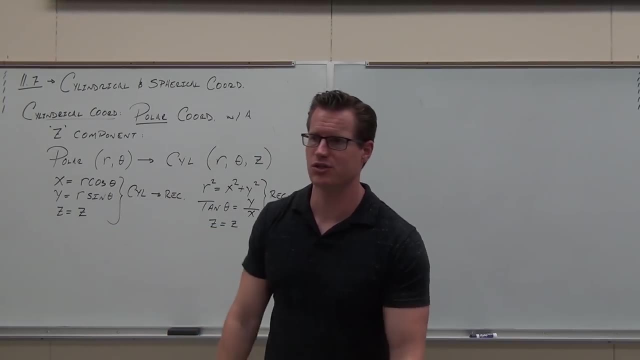 or spherical into rectangular or cylindrical into rectangular, Be able to do that stuff. Just translate it And you know what It's going to use this stuff. That's it. We've got a couple more for spherical, but it's literally just translation. 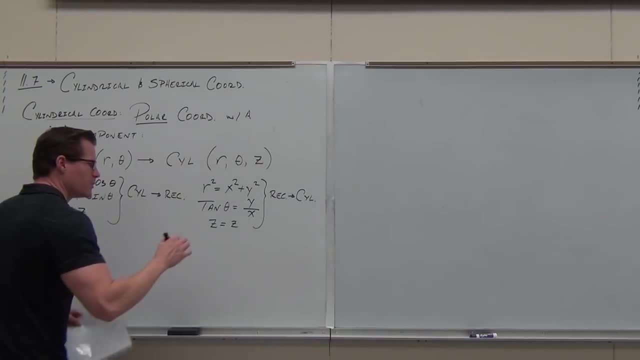 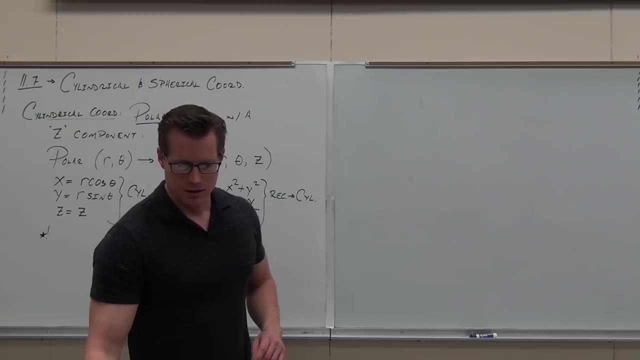 I'm being a little clever at times, but literally just translation. There are a couple notes, though. Please note Important Please R. I'm going to write all of it down, but I'm going to say it first, okay. 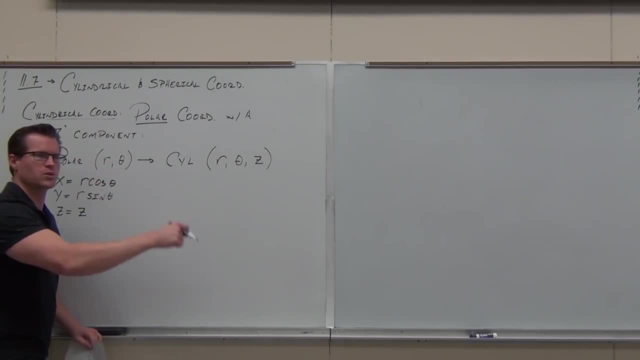 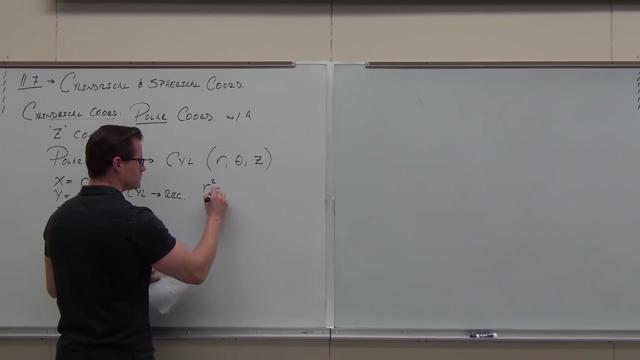 We use these identities to go from cylindrical to rectangular. You plug in cylindrical, you get rectangular. So this is used for cylindrical to rectangular. If we need to go back from rectangular to cylindrical, we use this second set. This is just Pythagorean identity. right triangle trigonometry. 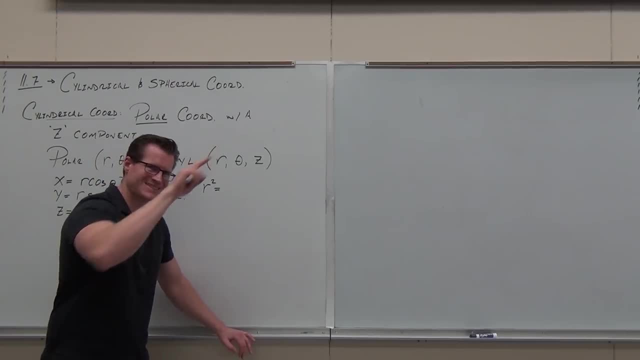 Do you remember how much r squared is? If r is the little radius, the hypotenuse if you will, how much would it be Square Square? R would be the square root, But r squared would be x squared plus y squared. 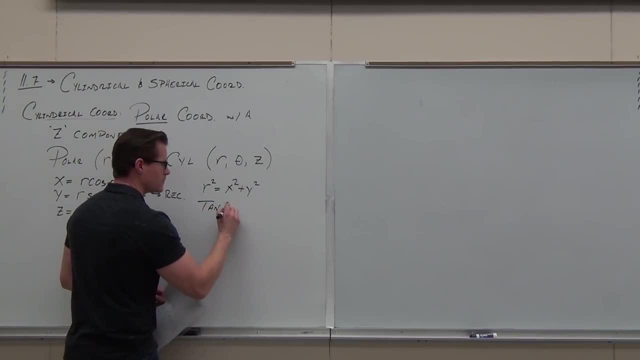 We also know a couple other things. Tangent theta: we always define this as Y over x. Well, sine over cosine. but if sine is the y and the x is y over x, and then hey, how much is z? 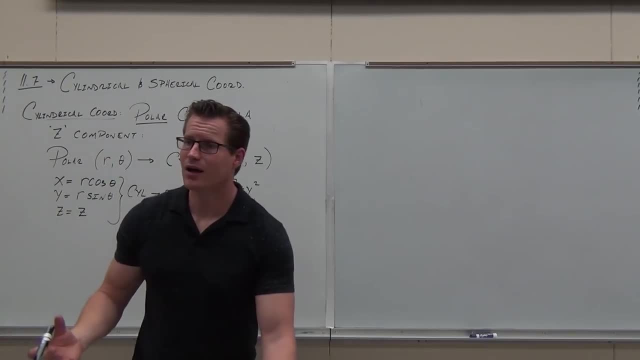 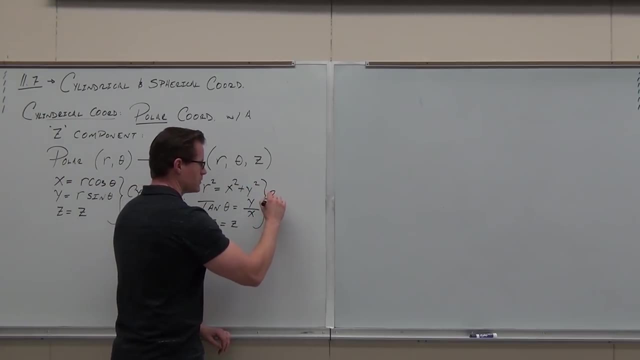 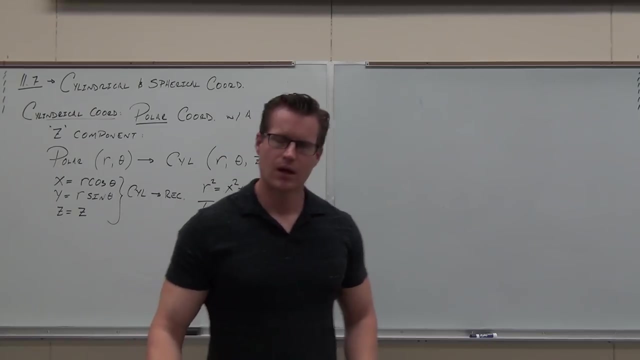 Z is z, Because there's no change there. This is how you would go from rectangular to cylindrical. Same thing. A couple notes. We got a couple examples. Literally, the only few things I want you to do is this: Be able to translate back and forth. 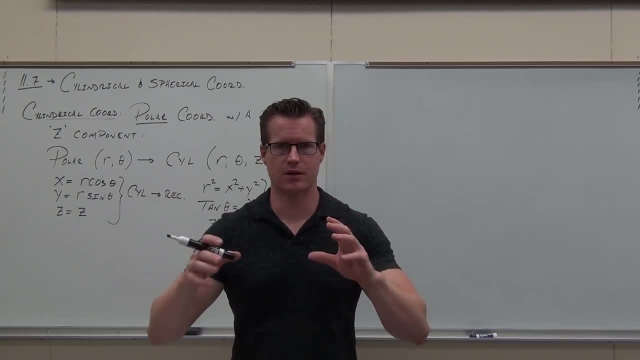 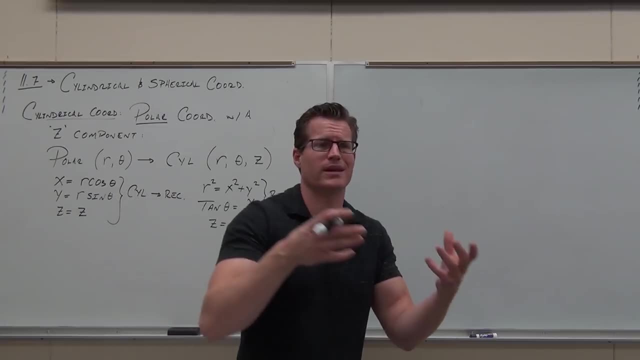 from rectangular to cylindrical, from rectangular to spherical- we haven't got there yet- from cylindrical to spherical, from spherical to cylindrical, and then be able to change some equations from rectangular equations into, like cylindrical or spherical, or spherical into rectangular, or cylindrical into rectangular. 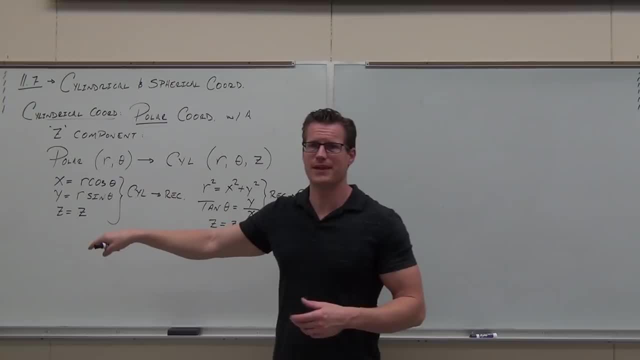 Be able to do that stuff. Just translate it And you know what It's going to use. this stuff, That's it. We got a couple more for spherical, but it's literally just translation. I'm being a little clever at times. 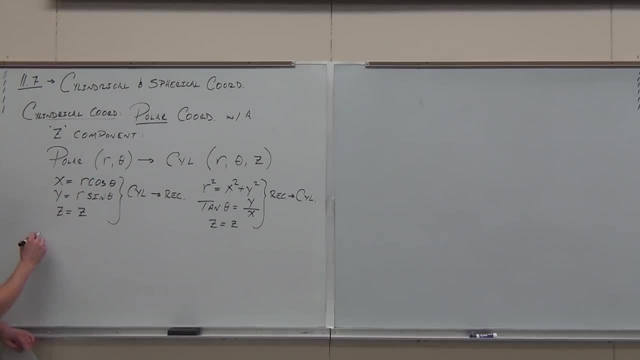 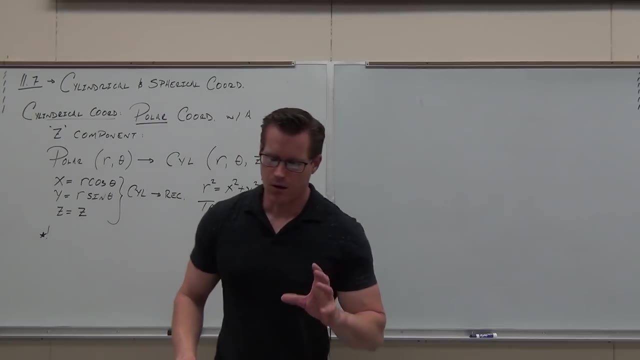 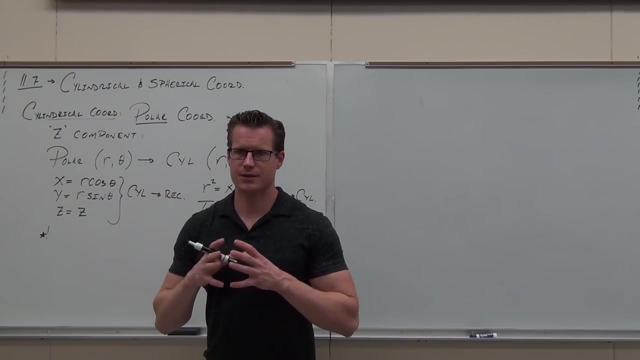 but literally just translation. There are a couple notes, though. Please note Important Please, R. I'm going to write all of it down, but I'm going to say it first. okay, R is not the distance from the origin to the point. 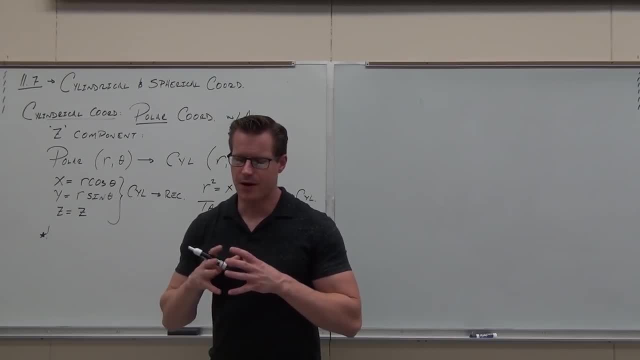 R is not the distance from the origin to the point. R is the distance from the origin to the projection of the point on the xy plane. That's what R is. I'm going to draw it for you in just a second, But I want you to write it down first. 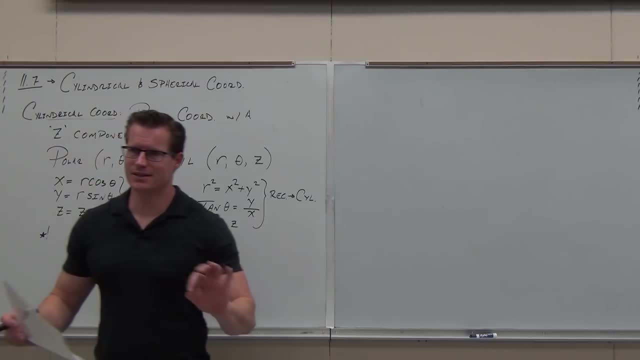 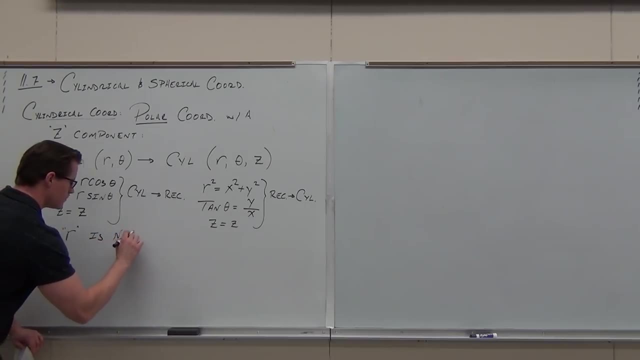 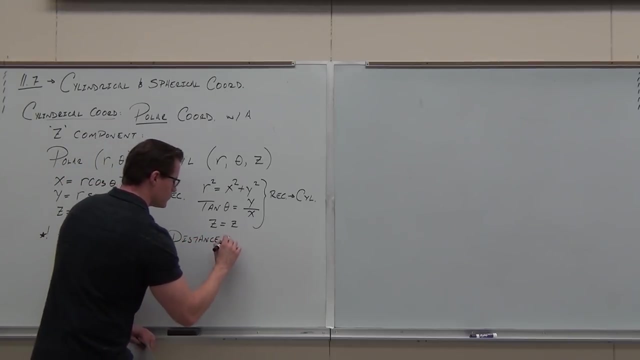 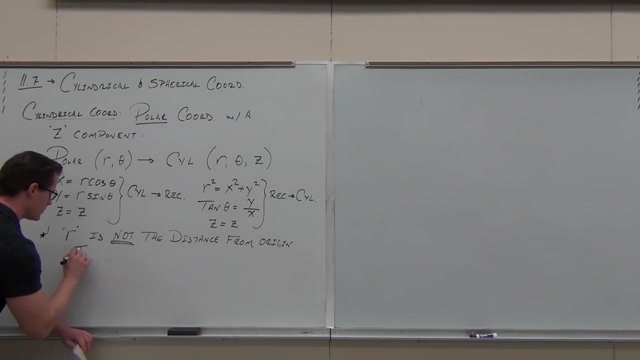 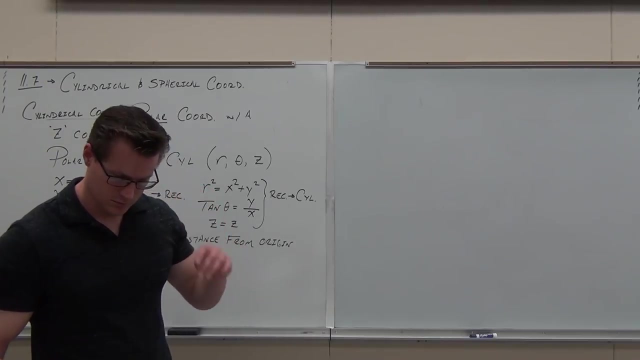 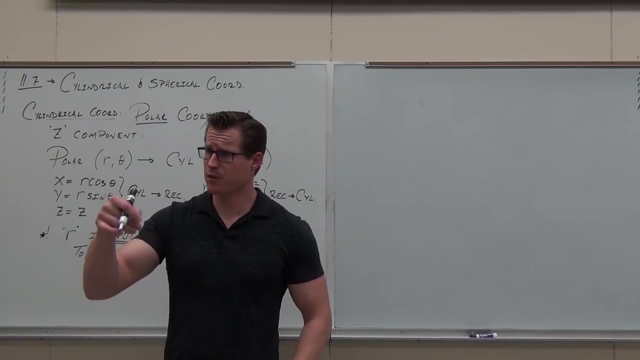 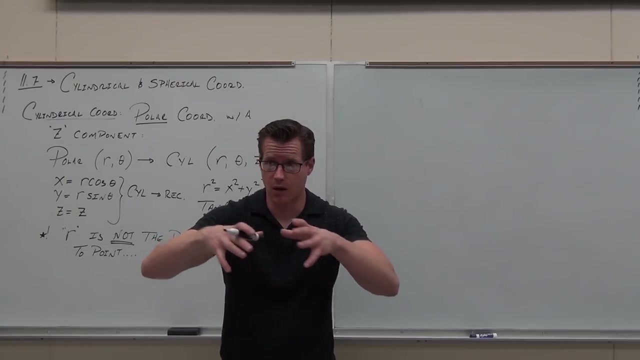 so we get this in our heads. R is not the distance from the origin to the point. R is the distance from the origin to the projection of the point on the xy plane. R is polar, which means R can't travel outside of the xy plane. 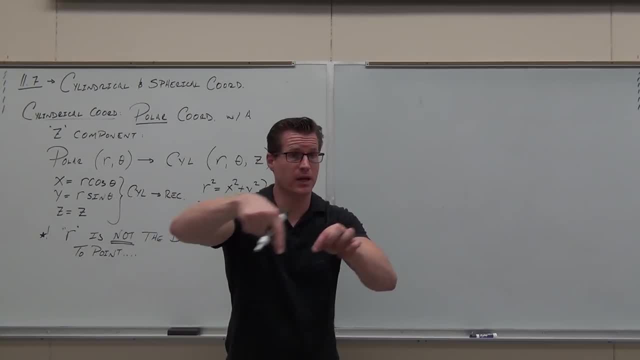 R is in that plane, which means that R can only go from origin to somewhere on the plane. One thing we can do on the plane is project the point on that plane. That's what R gives us. So R is not the distance from the origin to the point. 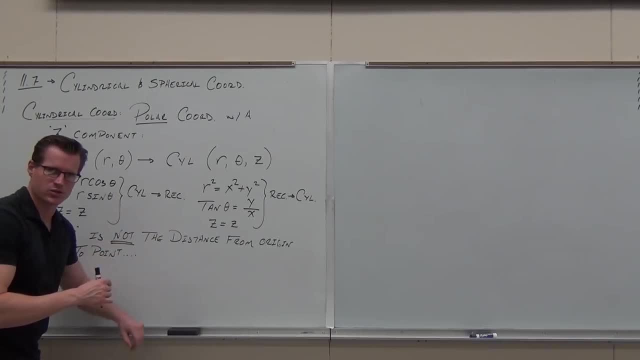 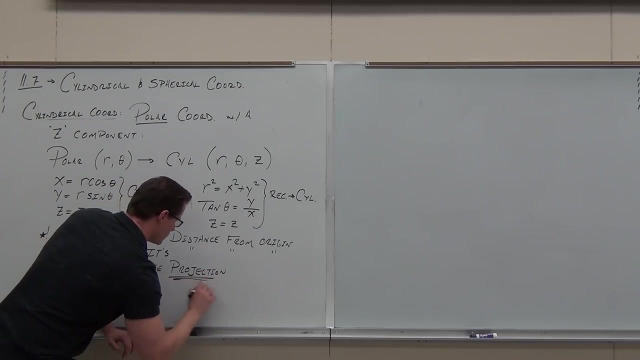 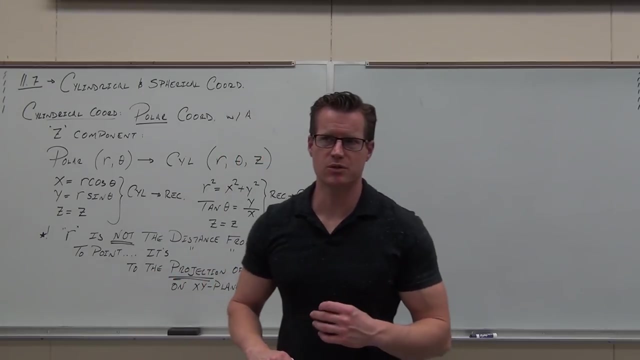 It's the distance from the origin to the projection of the point on the xy plane. it's kind of a big deal, and the reason why it's a big deal is because when we get too spherical we have something that is the distance from the origin directly to the point. 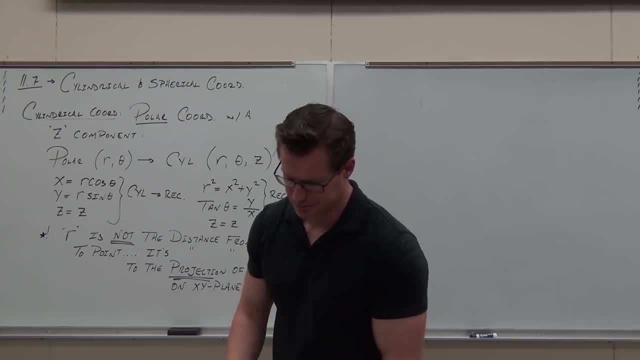 that's a different type of coordinate system. it's called spherical. one more thing- this is a big deal- we're about ready to translate between rectangular and cylindrical, cylindrical and rectangular. you've got to make sure that your quadrants and your octants match up, because a lot of times we can get these two. 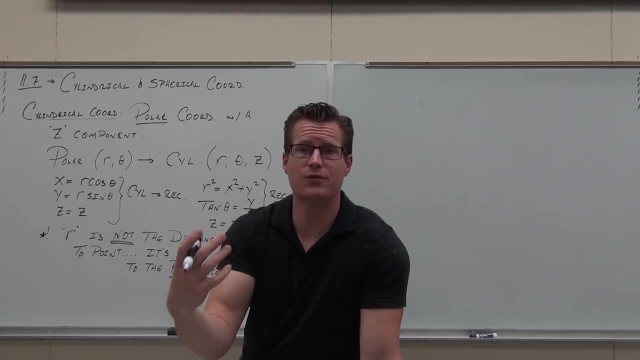 different, especially if we're going from rectangular to cylindrical. we can get two different thetas say: hey, you're rectangular, you get this tangent of 2 pi over 3, what is that? well, you got that one. but if I say tangent inverse of negative 1, 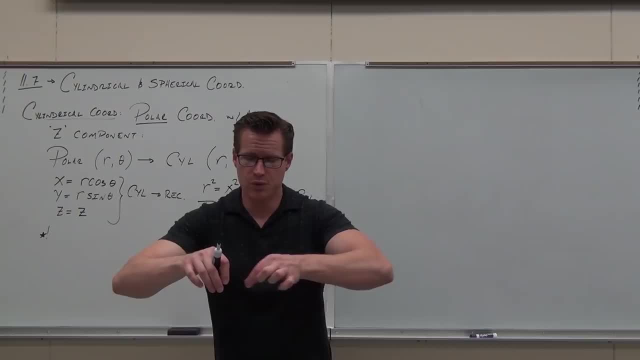 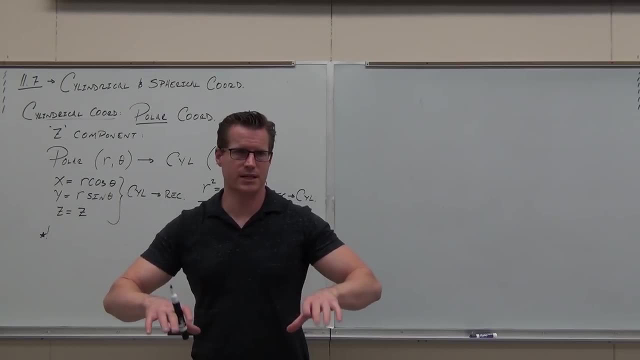 R is the distance from the origin to the projection of the point on the xy plane. That's what R is. I'm going to draw it for you in just a second, but I want you to write it down first so we get this in our heads. 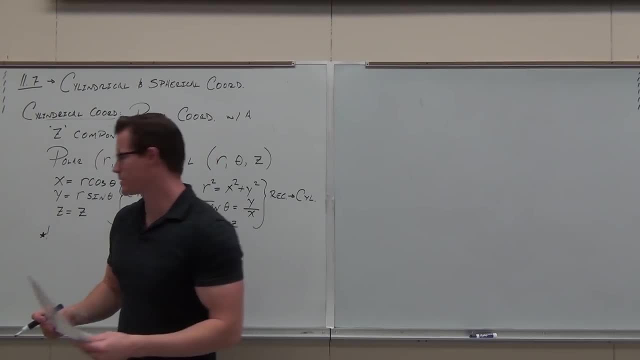 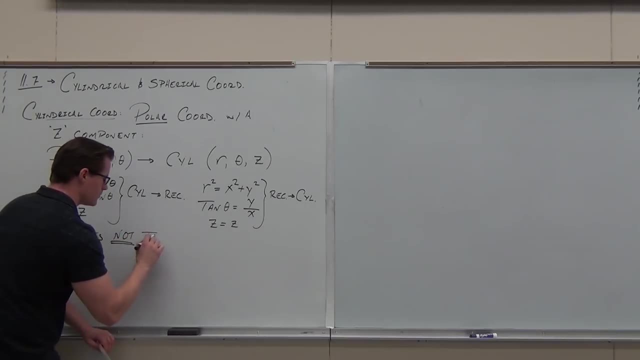 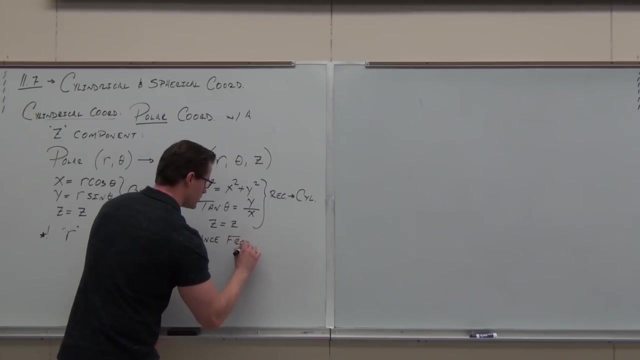 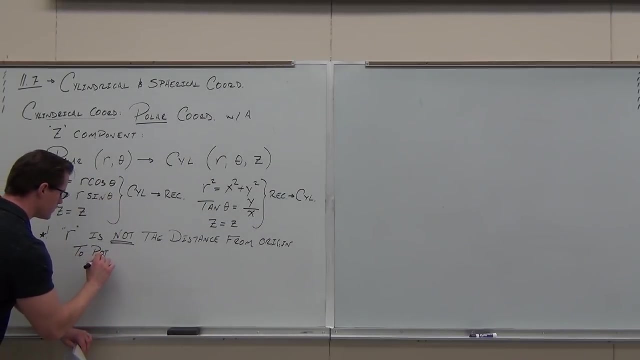 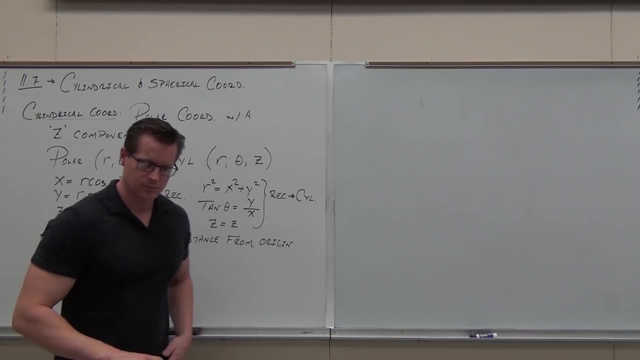 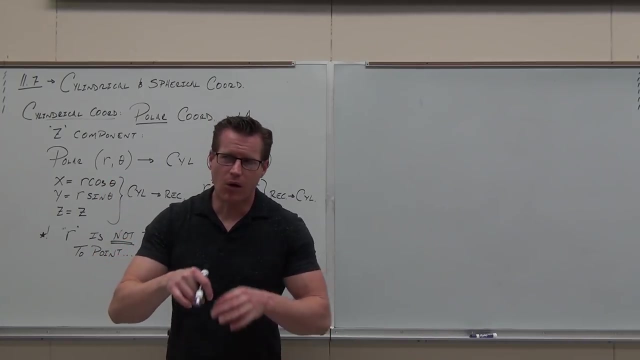 R is not the distance from the origin to the point. R is the distance from the origin to the projection of the point on the xy plane. R is polar, which means R can't travel outside of the xy plane. R is in that plane. 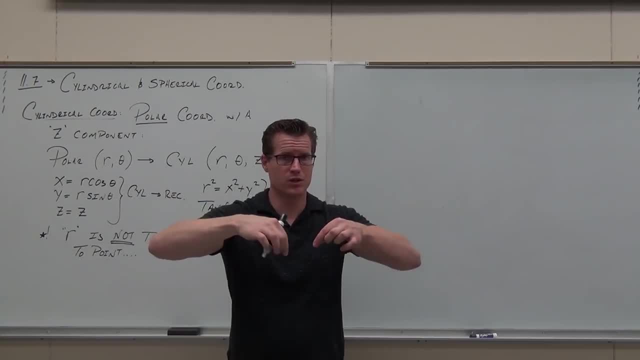 which means that R can only go from origin to somewhere on the plane. The only thing we can do on that plane is project the point on that plane. That's what R gives us. So R is not the distance from the origin to the point. 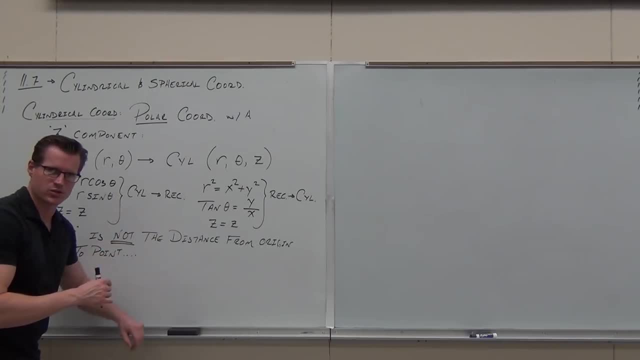 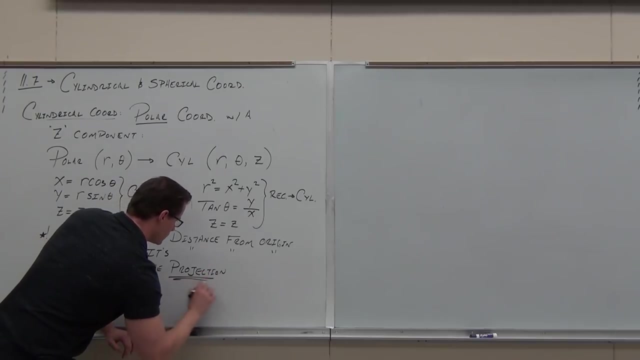 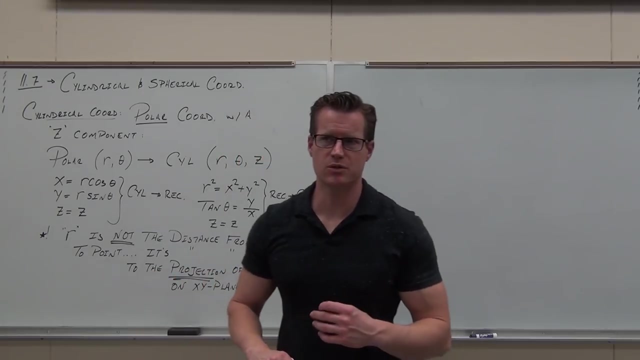 It's the distance from the origin to the projection of the point on the xy plane. That's what R gives us. It's kind of a big deal, And the reason why it's a big deal is because when we get too spherical, we have something that is the distance. 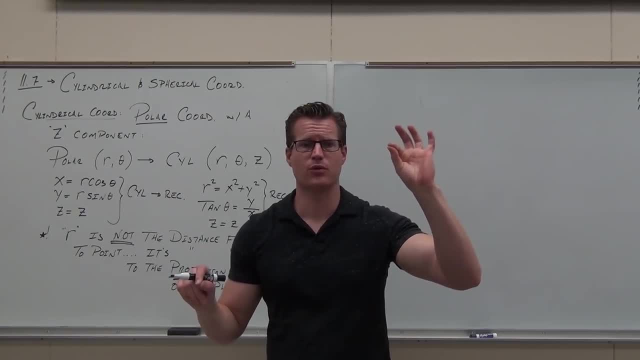 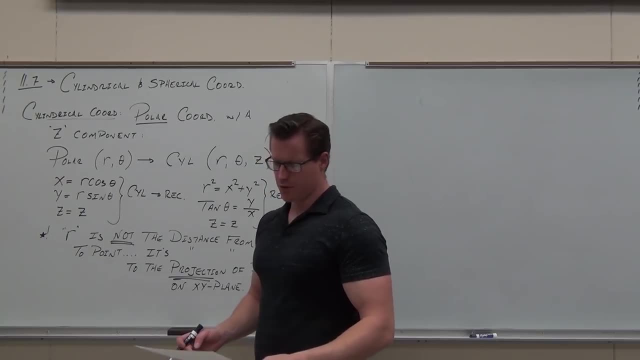 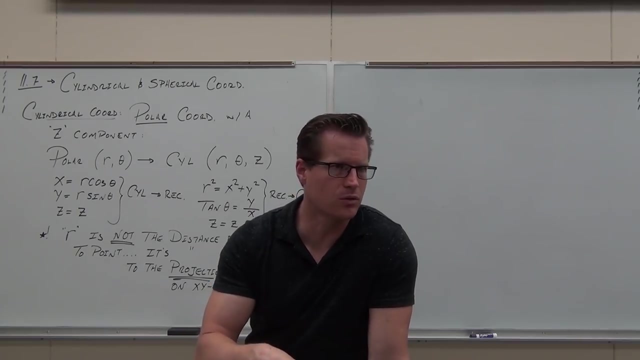 from the origin directly to the point. That's a different type of coordinate system. there It's called spherical. One more thing- This is a big deal We're about ready to translate between, like rectangular and cylindrical. Oh and, cylindrical and rectangular. 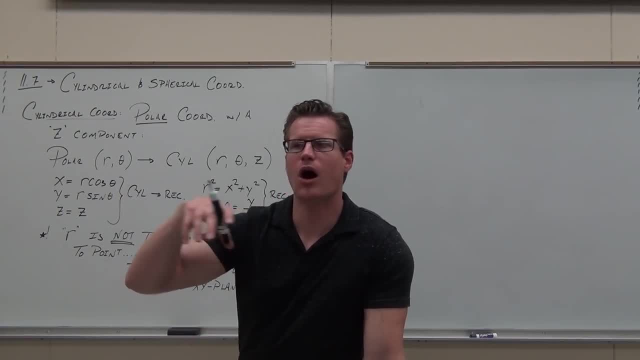 You've got to make sure that your quadrants and your octants match up, Because a lot of times we can get these two different. especially if we're going from rectangular to cylindrical, We can get two different thetas. Let's say, hey, you're rectangular. 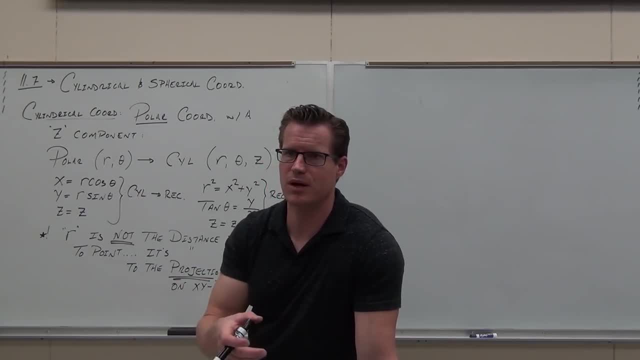 You get this tangent of 2 pi over 3.. What is that? Well, you got that one. But if I say tangent inverse of negative 1, there's a few values that you can get out of that. Does that make sense? 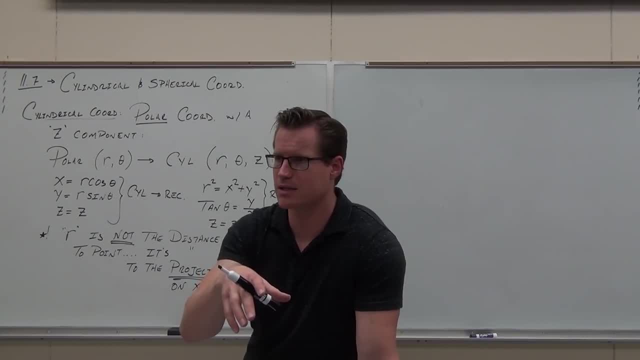 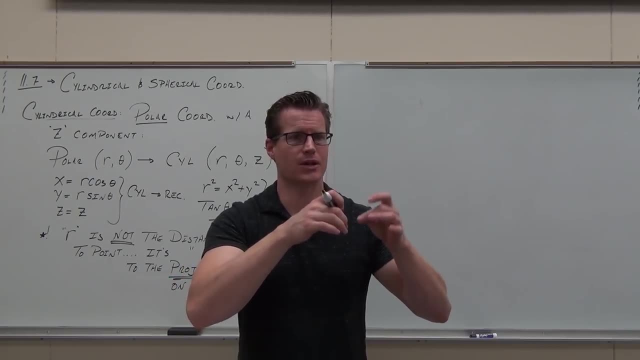 there's a few values that you can get out of that. does that make sense? for that reason, you've got to make sure that when you're changing your coordinate systems, that you're matching up your quadrants and your octants. so I'm going to put that down here. 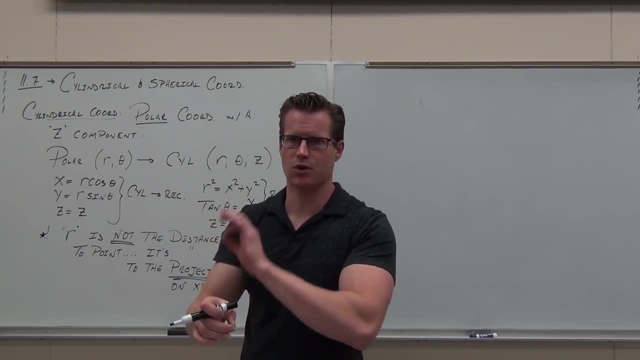 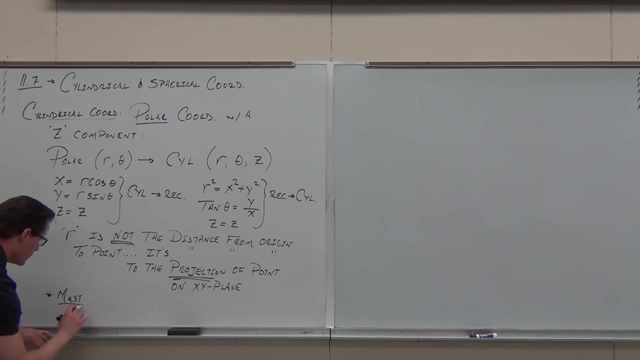 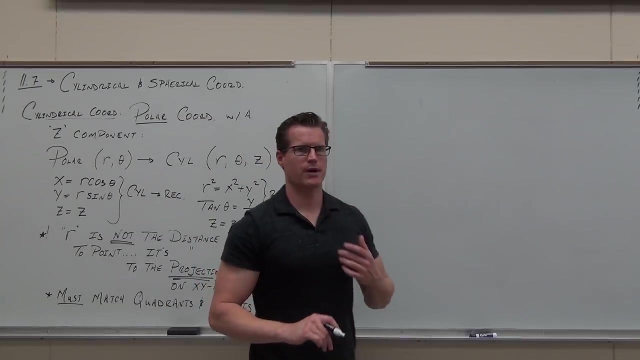 you'll see exactly what I mean in a couple of examples, but match your quadrants and octants when you're converting points. I'd like to show you a picture of how cylindrical actually works. then we're going to start doing some examples. so here's how this stuff works. 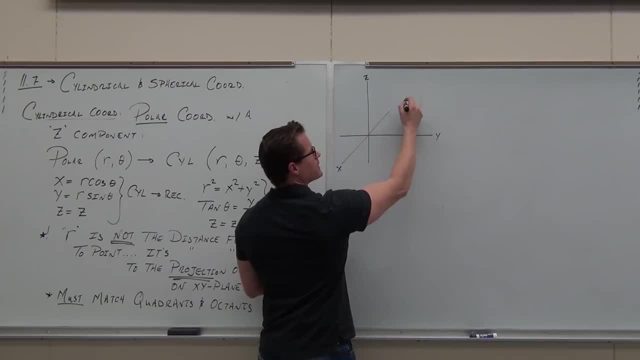 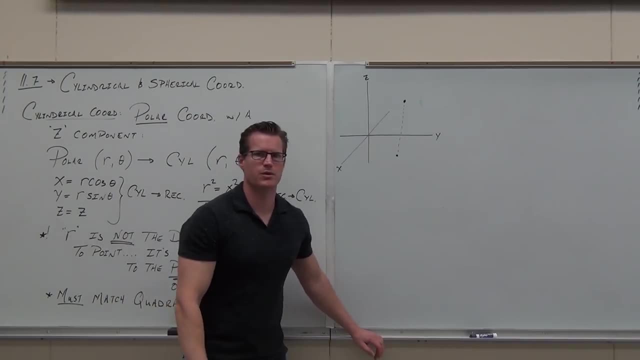 if we have this point floating out here in space. you have this point floating out here somewhere in space. do you guys see where I'm trying to represent that point? it's like it's floating out here: what quad. okay, I'm going to ask you two questions. 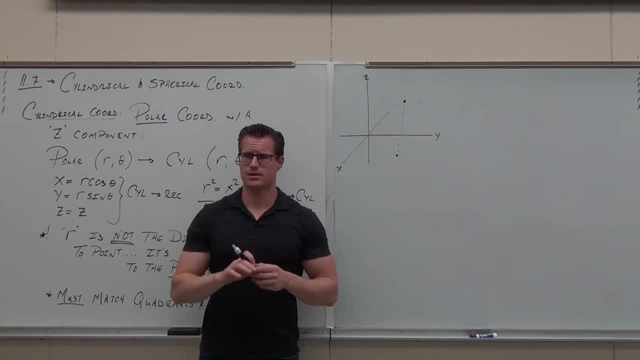 firstly, what octant is the point that's floating out here in space? what octant is the point that's floating out here in space? what octant, what octant is that point in? can you visualize that it's an octant 1? the projection is in quadrant 1. 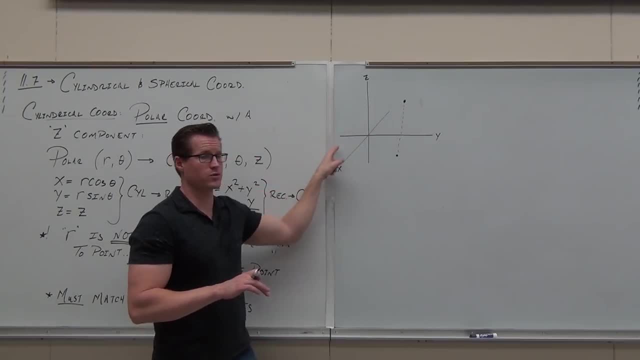 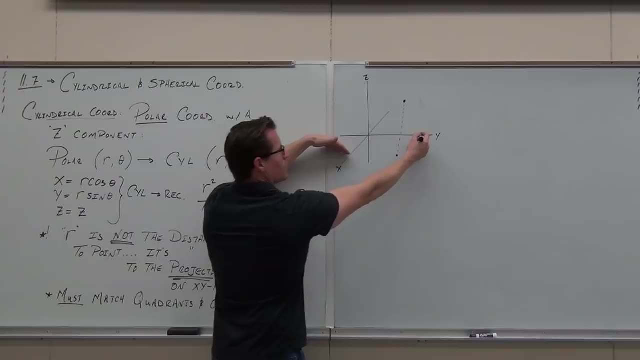 do you guys see the quadrant 1, quadrant 1,, quadrant 2, quadrant 3, quadrant 4 of the xy plane? do you guys see what I'm talking about? here's what cylindrical does instead of going. oh, here's x and here's y. 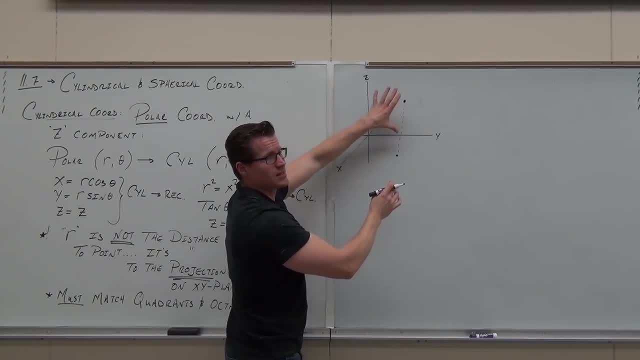 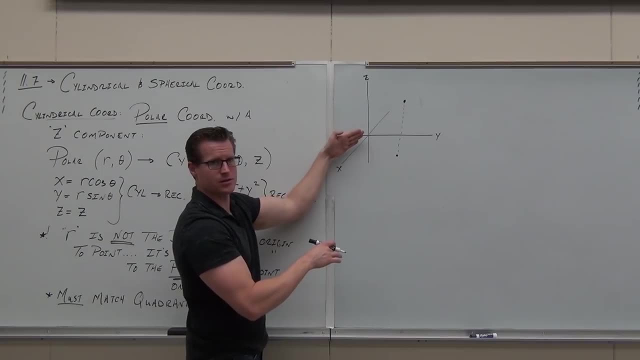 and where they meet, that's xy and here's z. this is still the z, but polar takes over. polar takes over for that plane. so polar says from the positive x axis. you get me. there's an angle from the positive x axis, from the origin to the projection of that point. 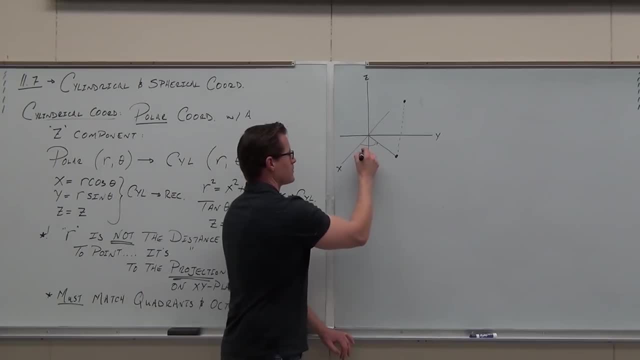 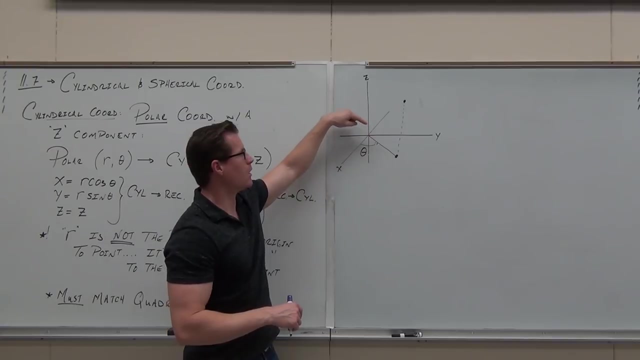 that angle is theta. that is what that is. here's the big one that people get kind of messed up on: the r, the r does not. please look at the board real quick. I need your full attention, okay. r does not go from here to here. that is not what r does. 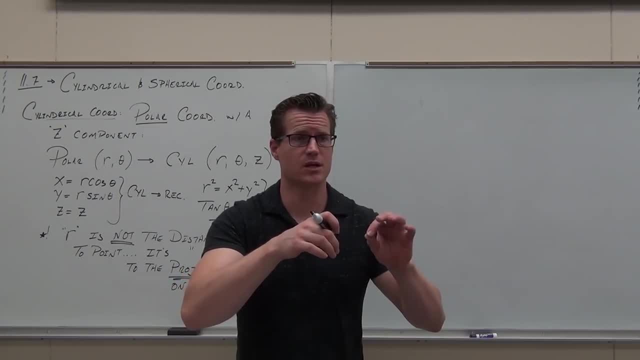 For that reason you've got to make sure that when you're changing your coordinate systems, that you're matching up your quadrants and your octants. So I'm going to put that down here. You'll see exactly what I mean in a couple of examples. 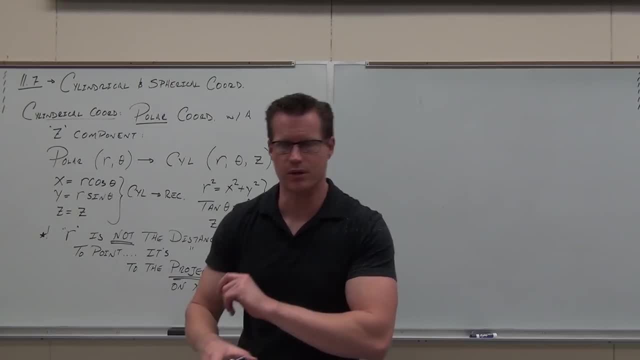 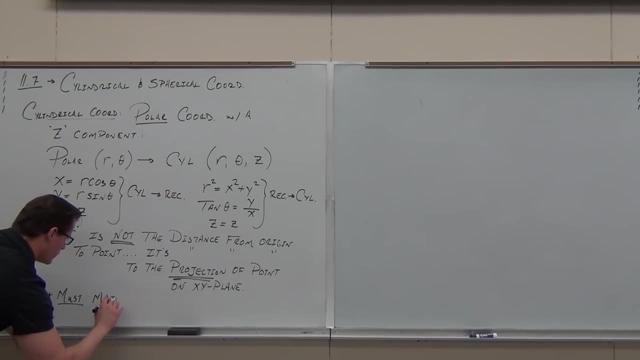 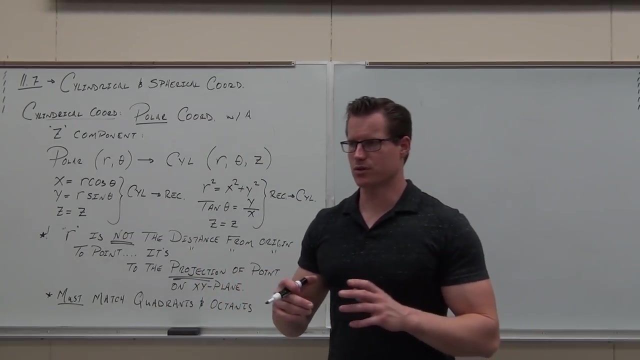 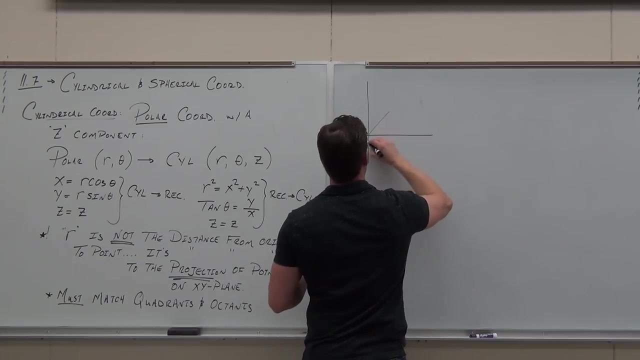 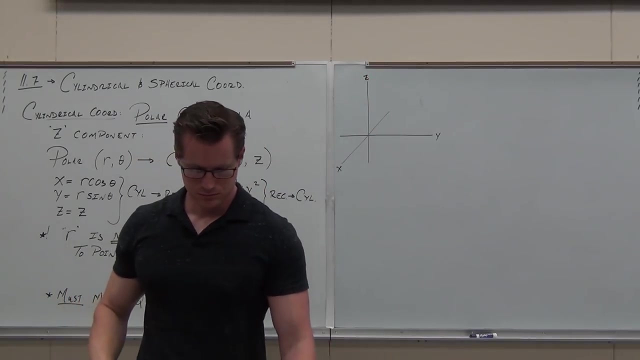 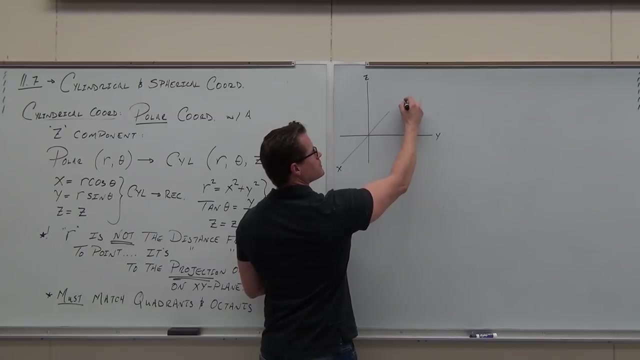 But match your quadrants and octants to your converting points. I'd like to show you a picture of how cylindrical actually works. Then we're going to start doing some examples. So here's how this stuff works. If we have this point floating out here in space, 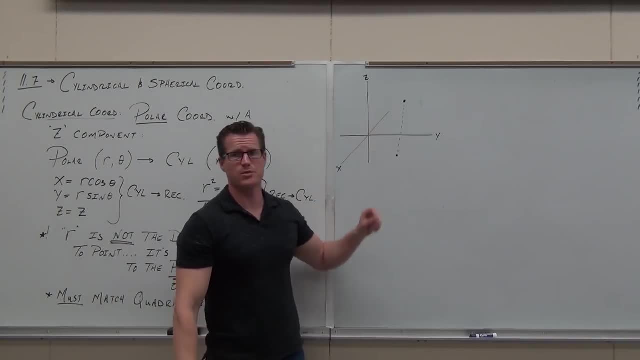 we have this point floating out here somewhere in space. Do you guys see where I'm trying to represent that point? It's like it's floating out here. Okay, I'm going to ask you two questions. Firstly, what octant? What octant is that point? 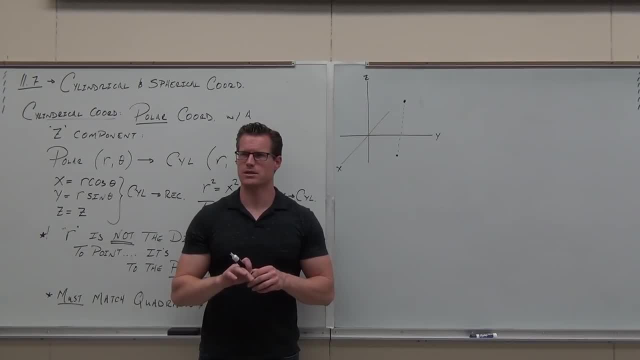 Can you visualize that It's an octant one? The projection is in quadrant one. Do you guys see the quadrant one? Quadrant one, quadrant two, quadrant three, quadrant four of the xy plane? Do you guys see what I'm talking about? 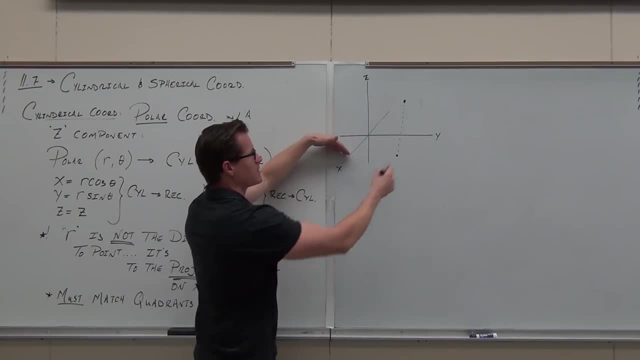 Here's what cylindrical does Instead of going: oh, here's x and here's y, and where they meet, that's xy, and then here's z. This is still the z, But polar takes over for that plane. So polar says: 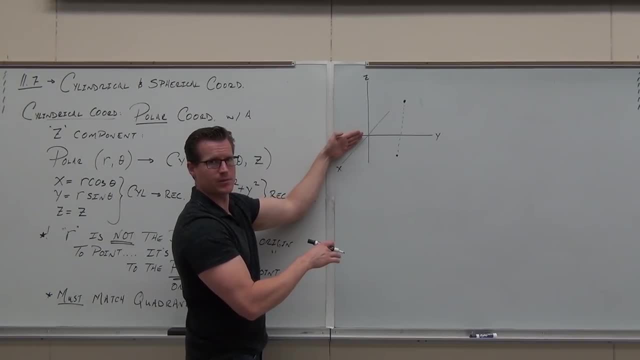 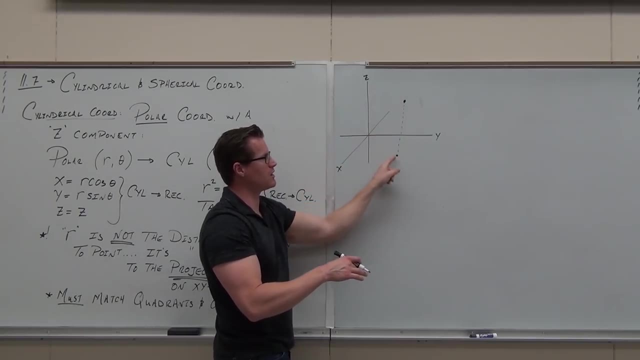 from the positive x-axis, you get me. There's an angle from the positive x-axis, from the origin to the projection of that point. That angle is theta. That is what that is. Here's the big one that people get kind of messed up on. 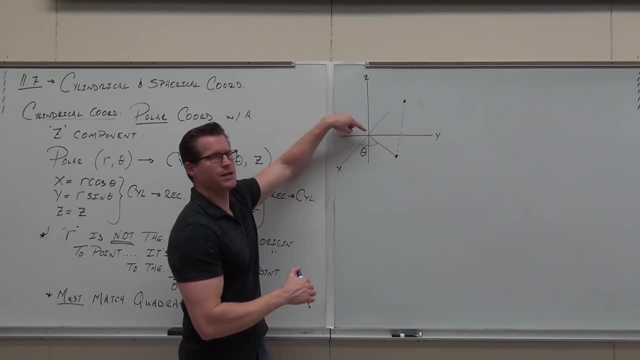 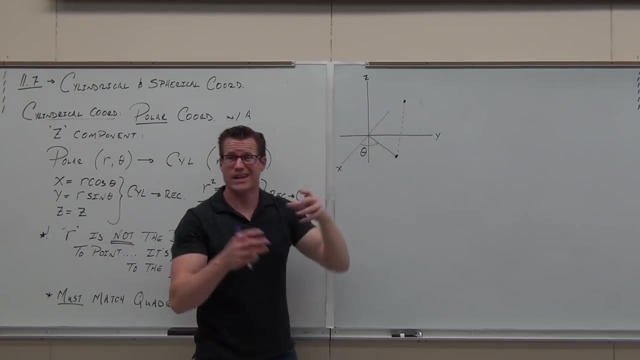 The r, The r does not. Please look at the board real quick. I need your full attention, okay? r does not go from here to here. That is not what r does. r is polar, That's all r does. So on the xy plane. 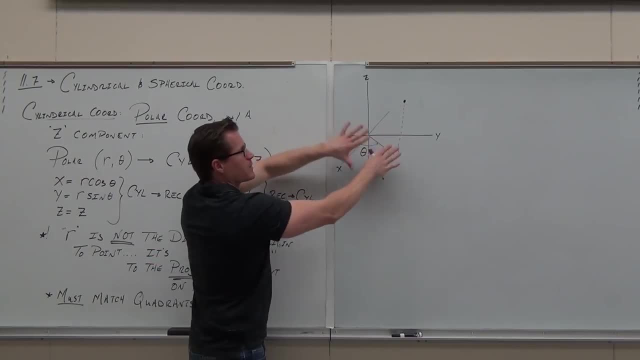 r is polar, that's all r does. so on the xy plane, like flat on the xy plane, what theta does? it sweeps out the angle, man, from the positive x to where the projection of the point is. so you're looking at it from like the top and you go hey. 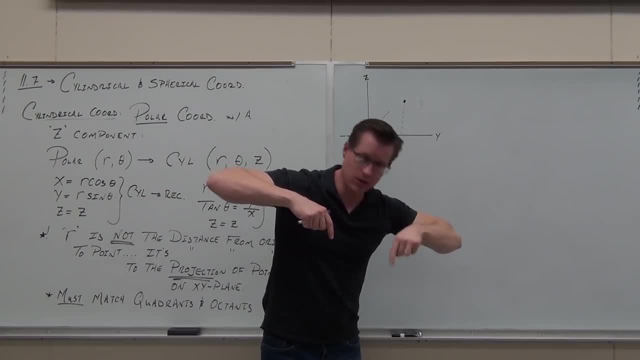 take that point. it's going to look like it's flat make sense. it's going to look like it's flat make sense. it's going to look like it's flat where it looks like it's flat, whatever angle from the positive x, whatever that is. that's theta. 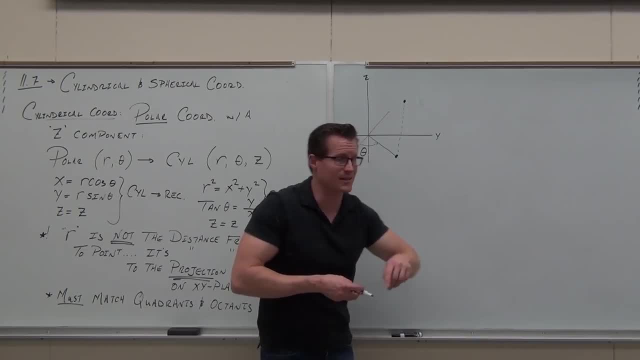 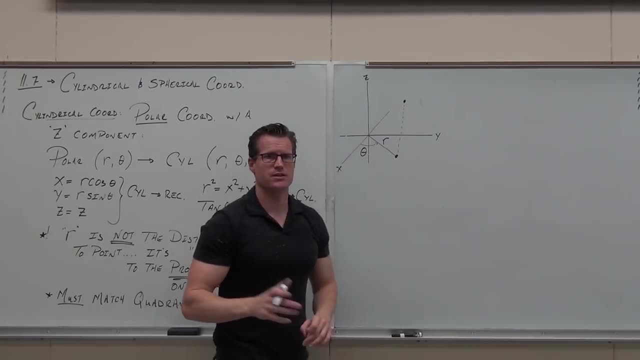 however far the origin is flat distance on the plane from the origin to the projection of the point on the xy plane. that is what r is. show of hands. if you understand what r is, that's r when we get to spherical. this distance is going to be called rho. 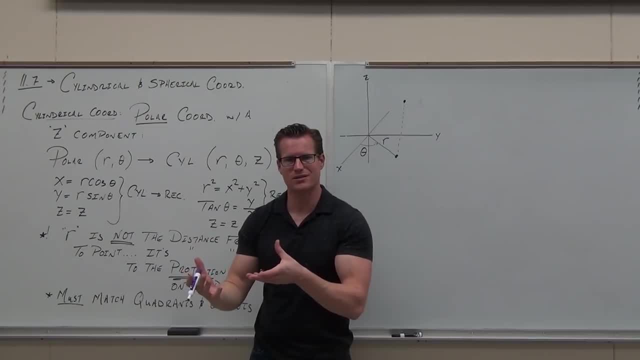 the greek letter for r standing for radius. that's what that's going to be, so we can't get r and rho confused. I need you to know which one is which. you guys okay with what I'm talking about? the z? it's still the height. 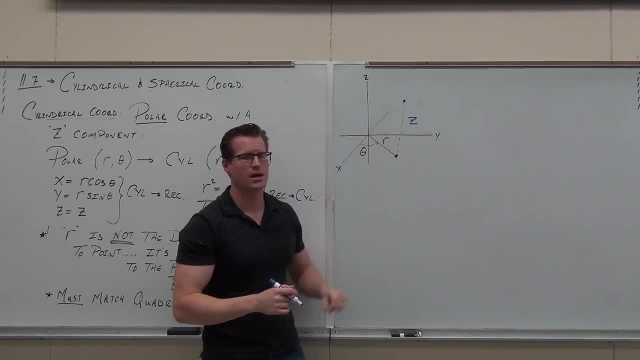 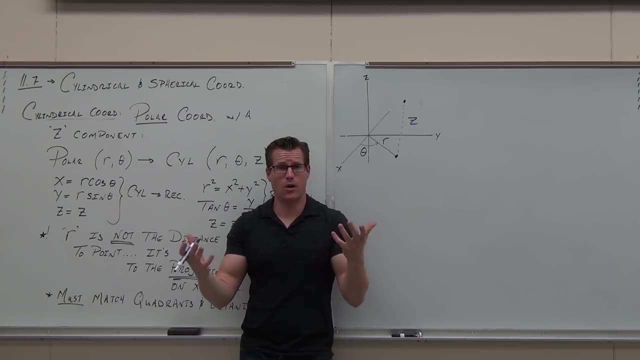 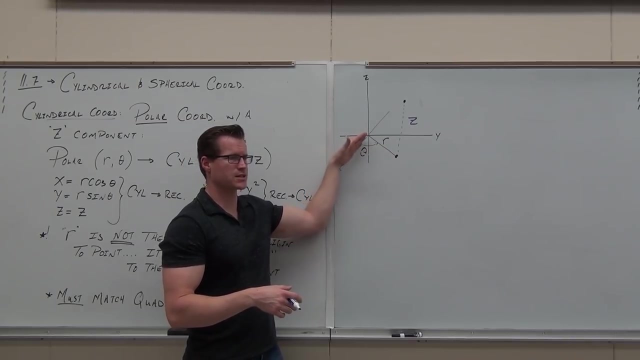 just like any other height. it's just the height that that actual point is above the xy plane. do you guys understand the idea of of this cylindrical coordinate system? so we have r. r is the distance between the origin and the projection of the point, theta, theta is the angle from the positive x axis. 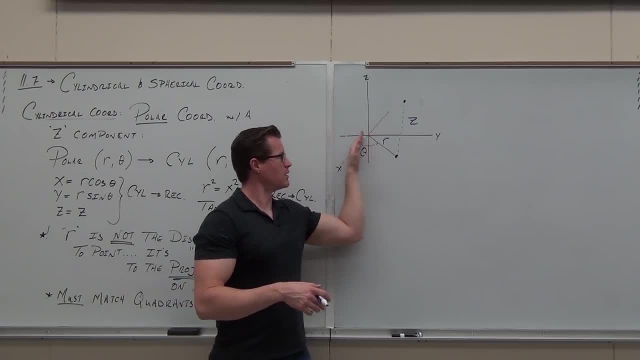 until we reach the projection of the point onto the xy plane, the z is still just the height. did I mess up my theta? let's go ahead. let's try to translate here real quick. so I'm going to give you some and I have to basically tell you what they are. 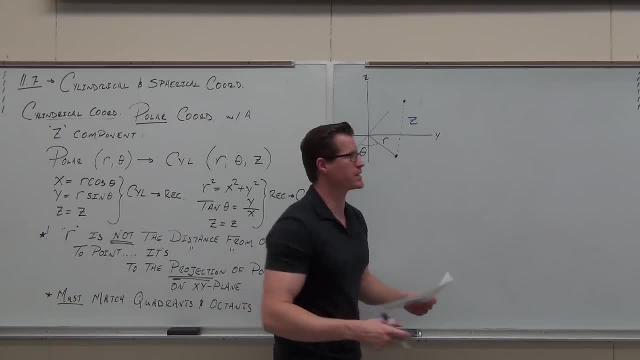 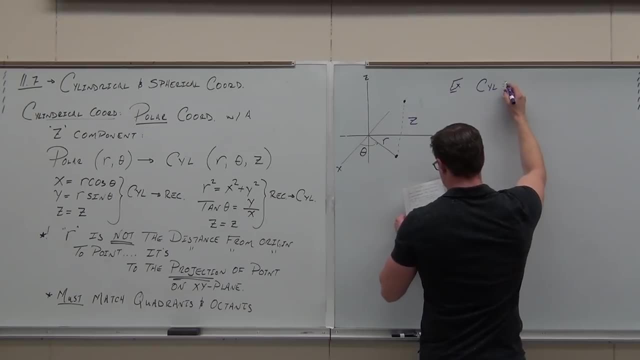 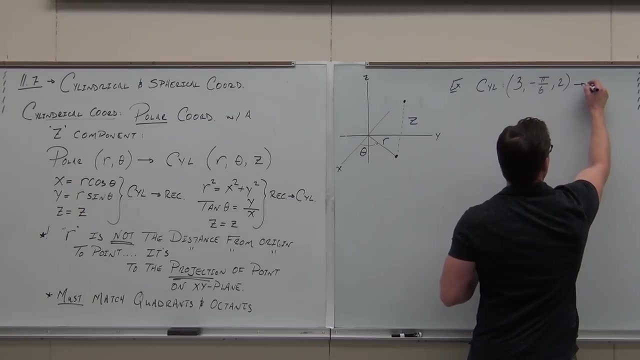 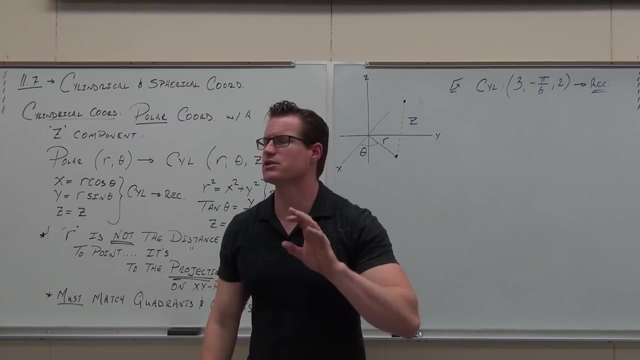 I'm going to give you cylindrical coordinates right now. we're going to translate that to rectangular. we're going to change this to rectangular. man, if I can't get you to do anything else, I want to get you to at least visualize where this is like on a graph. 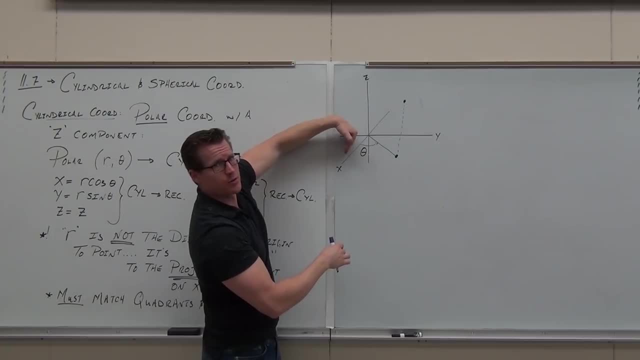 like flat on the xy plane. what theta does? it sweeps out the angle man from the positive x to where the projection of the point is. So you're looking at it from the top and you go: hey, take that point. 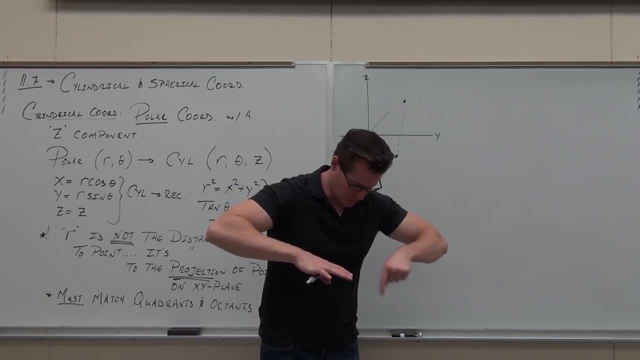 It's going to look like it's flat. Make sense Where it looks like it's flat, whatever angle from the positive x-axis, whatever that is. that's theta. However far, the origin is flat. distance on the plane from the origin to the projection of the point. 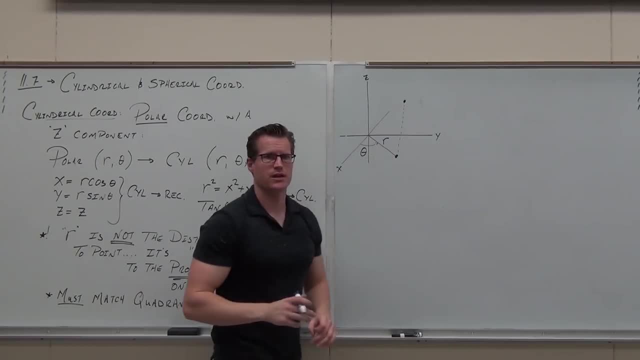 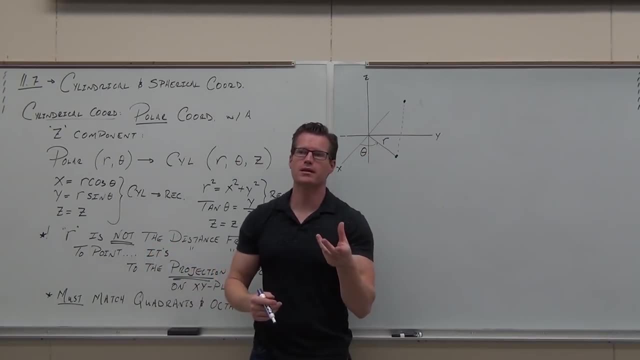 on the xy plane. that is what r is. Show of hands. if you understand what r is, That's r. When we get to spherical, this distance is going to be called rho, the Greek letter for r: staying for radius. That's what that's going to be. 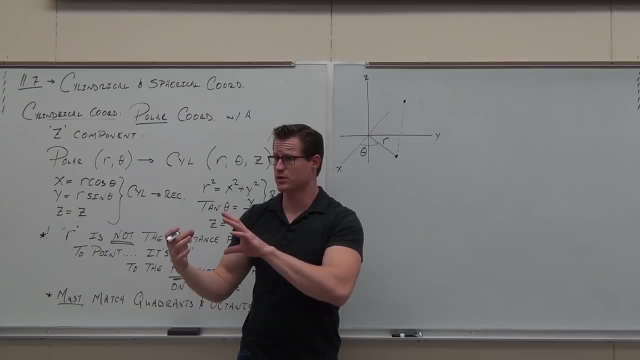 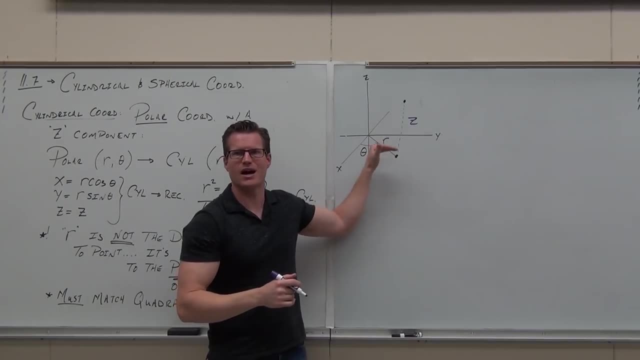 So we can't get r and rho confused. I need you to know which one is which. You guys okay with what I'm talking about? The z, it's still the height, just like any other height. It's just the height that that actual point is. 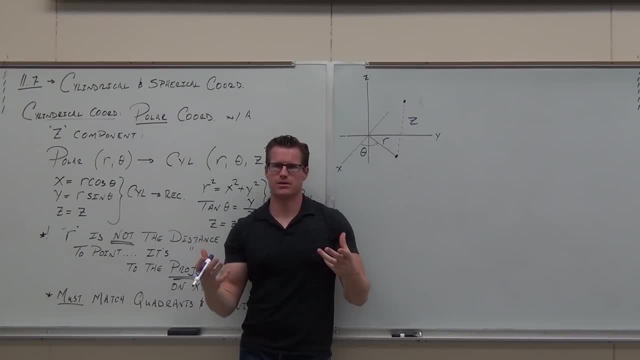 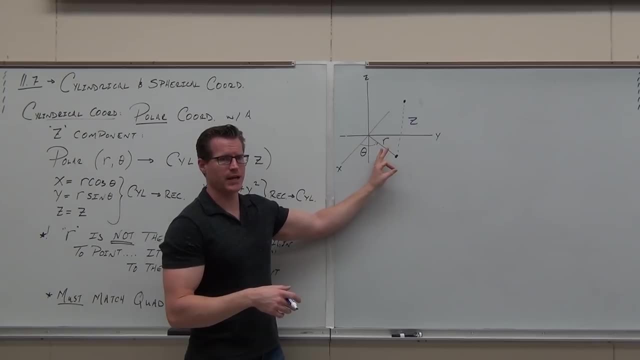 above the xy plane. Do you guys understand the idea of this cylindrical coordinate system? So we have r. r is the distance between the origin and the projection of the point. Theta. theta is that angle from the positive x-axis until we reach the projection of the point. 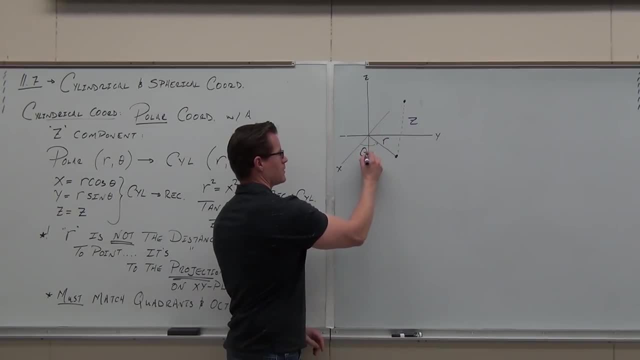 onto the xy plane. Z is still just the height. I messed up my theta. Let's go ahead. Let's try to translate here real quick. So I'm going to give you some and I have to basically tell you what they are. 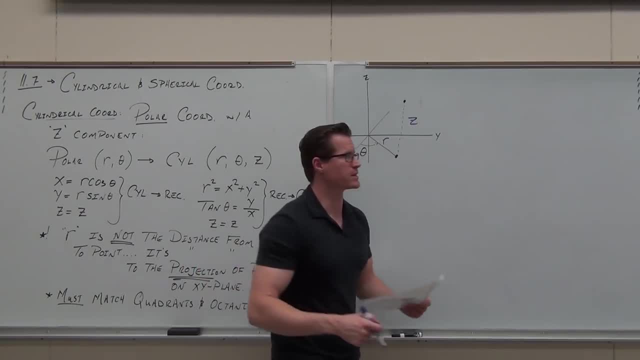 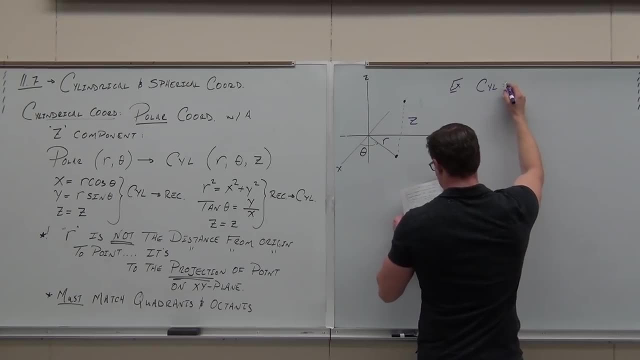 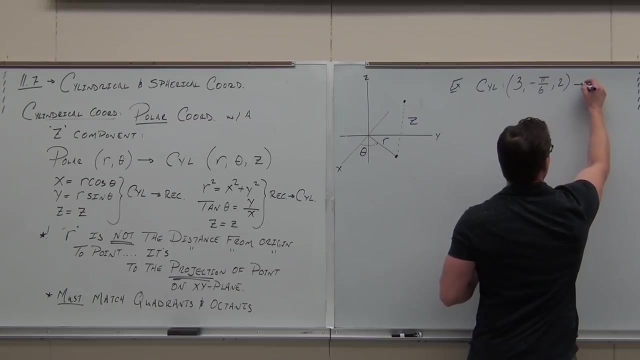 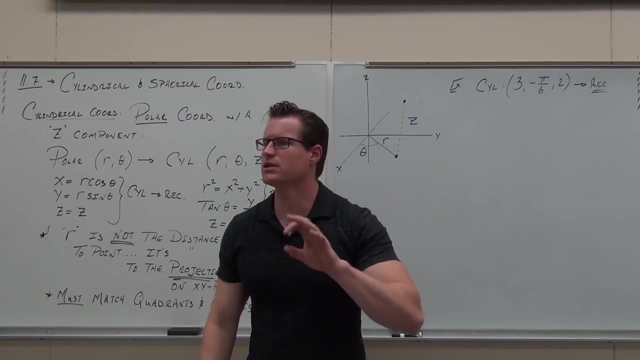 I'm going to give you cylindrical coordinates right now. We're going to translate that to rectangular. We're going to change this to rectangular. What do they do, Man? if I can't get you to do anything else, I want to get you to at least visualize where this is. 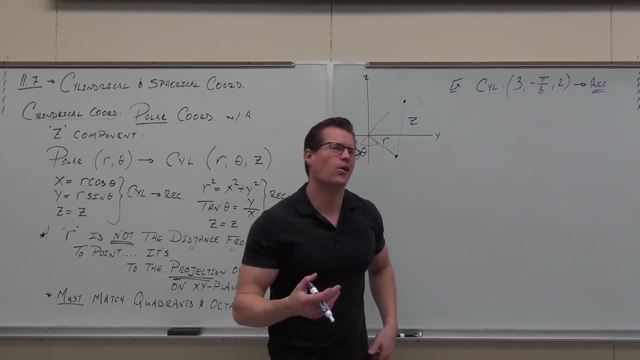 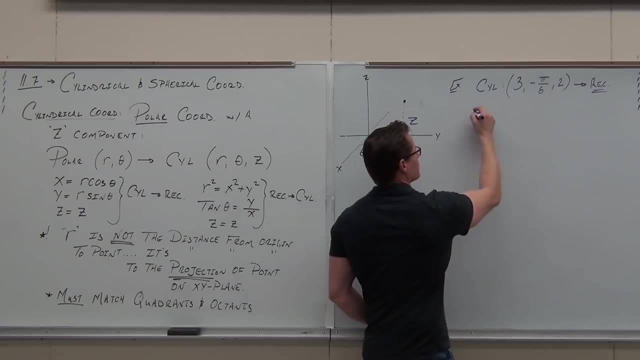 like on a graph. So number one: what's the r? Can you tell me what the r is? here It goes in order of r theta z: What's the r? Write down all the stuff you know. Let's do that. 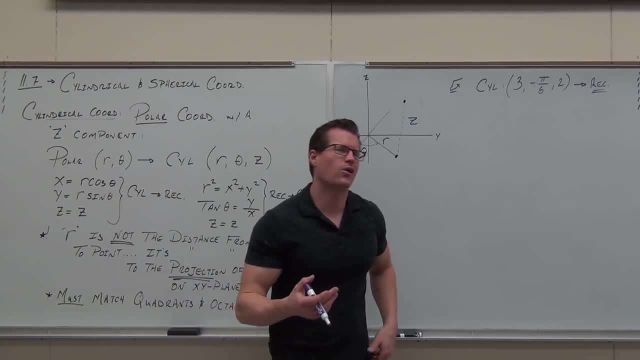 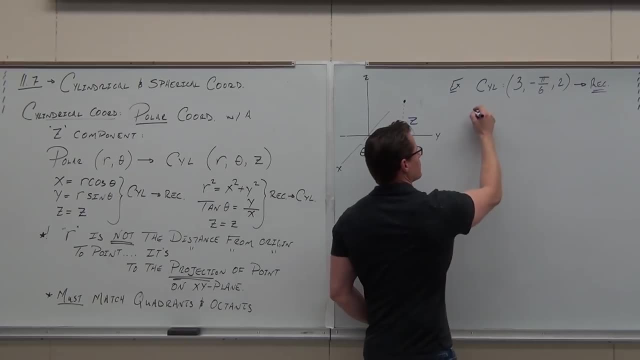 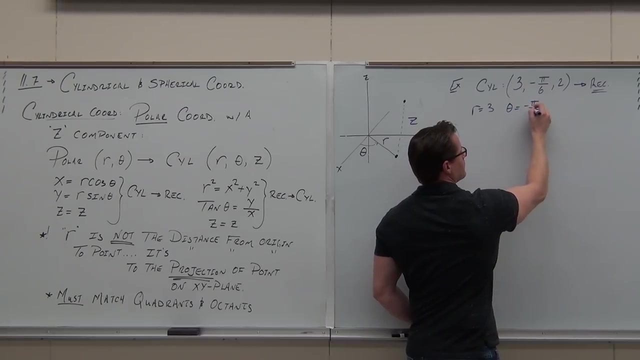 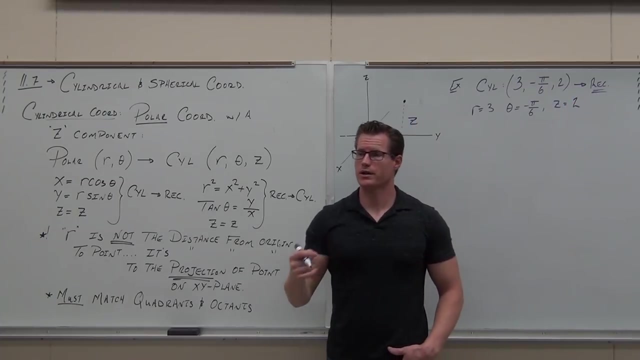 so number one: what's the r? can you tell me what the r is? here it goes in order of r, theta, z. what's the r? write down all the stuff you know. let's do that. what's the theta, theta and the z? now visualize where it is. 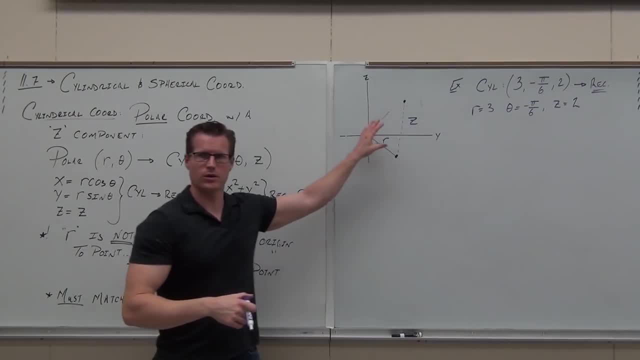 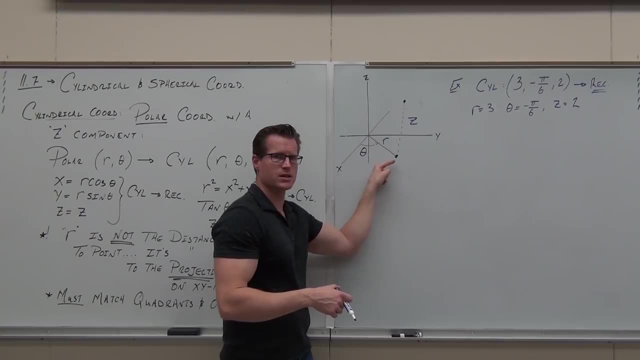 and write that down too. so visualize where that is. look at the board here real quick. this has an r of three, which means I'm coming out here three units from the origin, flat on the plane. three units, and then my angle. where's my angle? negative, negative. 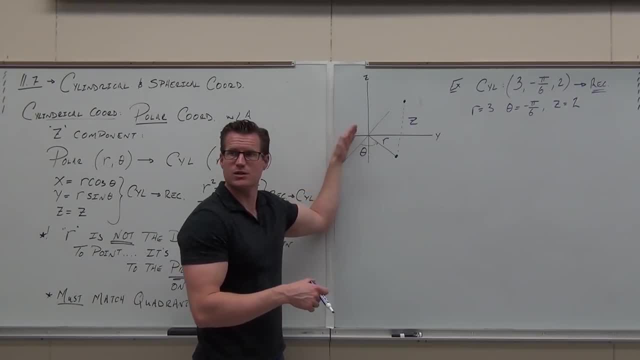 so from here I'd be going this way. do you guys see what I'm talking about? you've got to. if you're looking down at it, I'm going down negative angle, I'm going this way. so this is going three negative angle. it's over here somewhere. 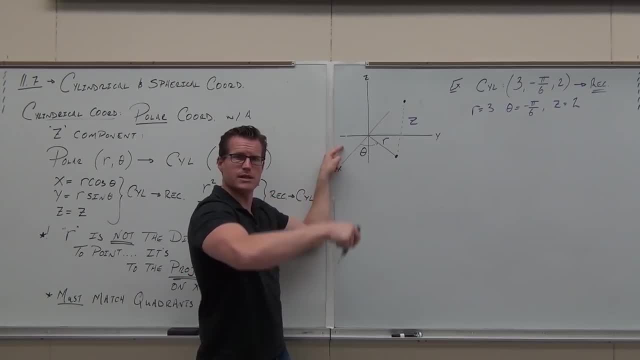 and then is it going up or is it going down. where's it going up? it's going to shoot up here a little bit. what quadrant would the projection be on? four, perfect, what octant are we in? four, four, and then we drop down five, six, seven. 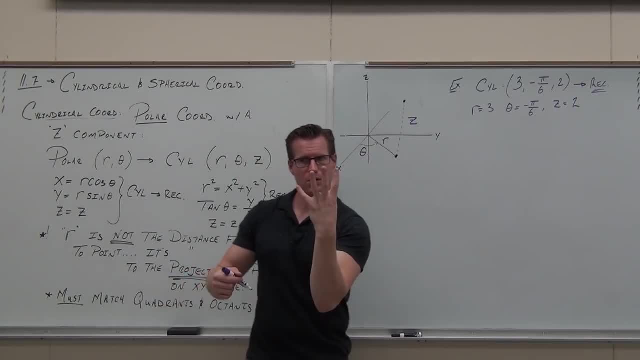 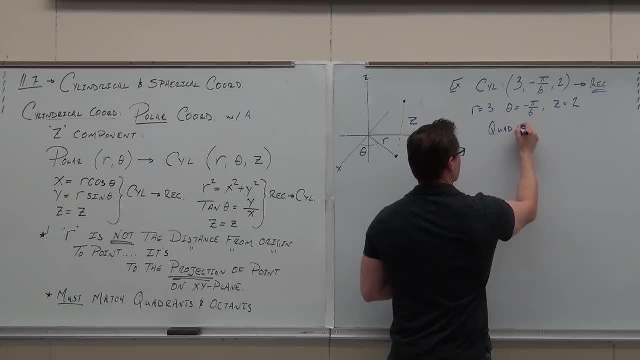 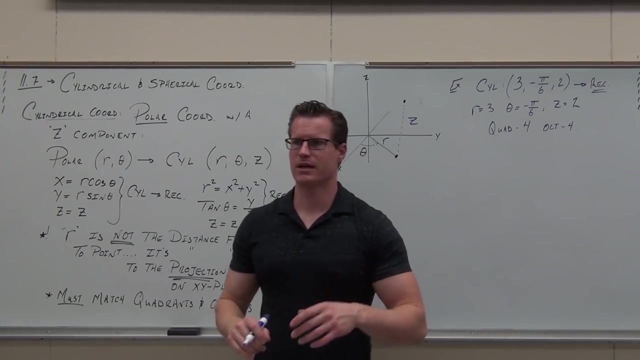 eight. okay, so we are in quadrant four. we're also in octant four. does that make sense? write that down. the reason is- and not necessarily going from cylindrical to rectangular, because you don't have any option there. it's going to be one thing, but going from rectangular cylindrical. 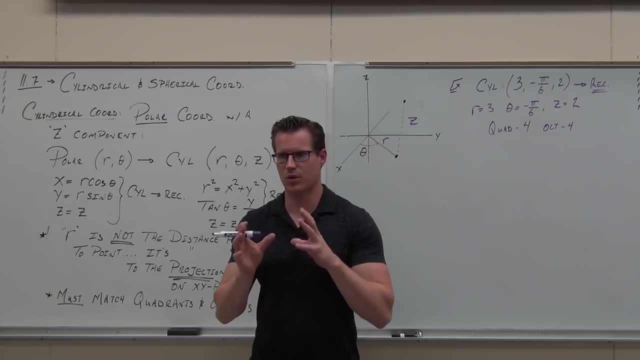 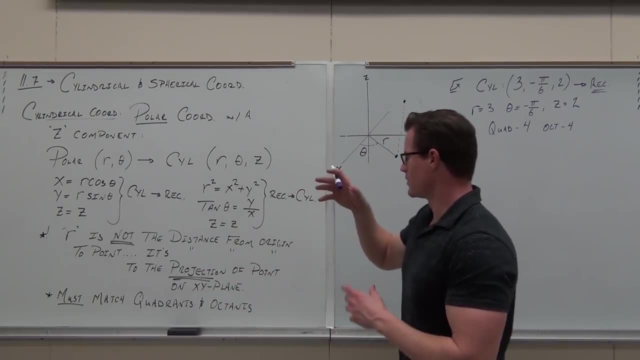 you get options for the theta. you absolutely have to match up the quadrants because you can make some mistakes here. so anyway, let's give it a try. let's go over here and see if we're going from cylindrical to rectangular. this is the only step I have to use. 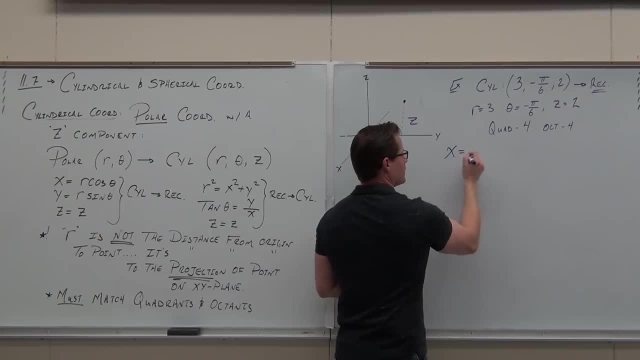 so let's see if we can fill it out. if I want to get x, x is always no matter what- r, cosine, theta. hey, do you get an r? that's why I write this stuff down. do you have a theta? yes, that's all you need. so we're going to have. 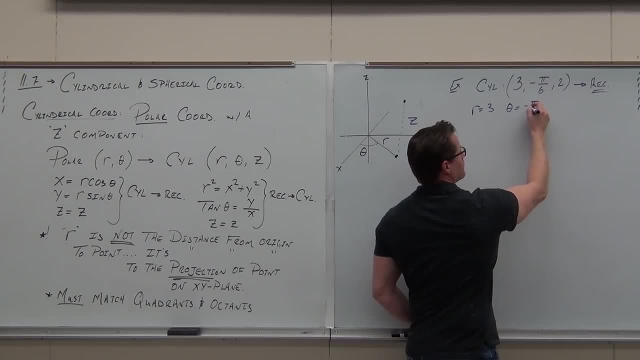 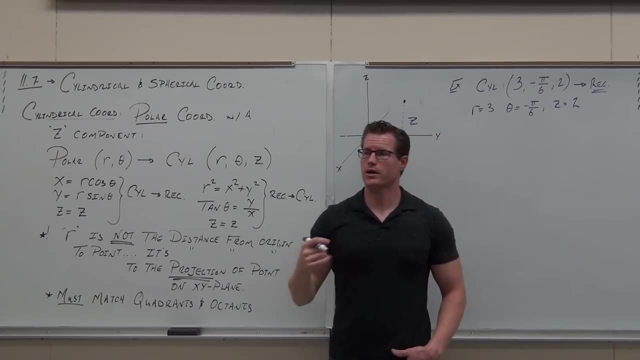 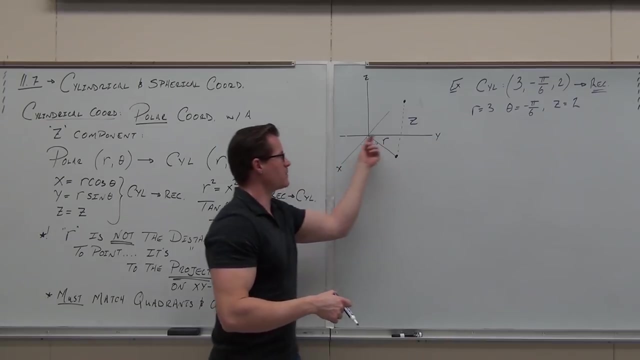 What's the theta, Theta And the z? Now visualize where it is and write that down too. So visualize where that is. Look at the board here real quick. This has an r of 3,, which means I'm coming out here. 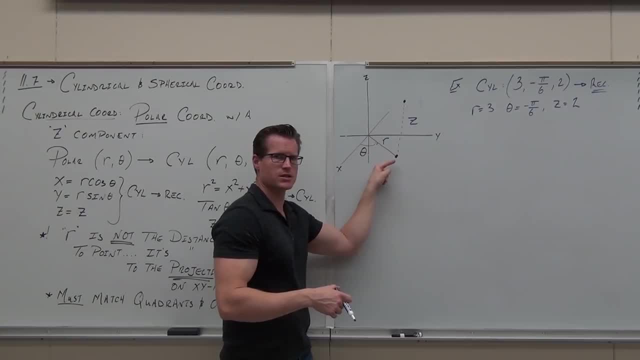 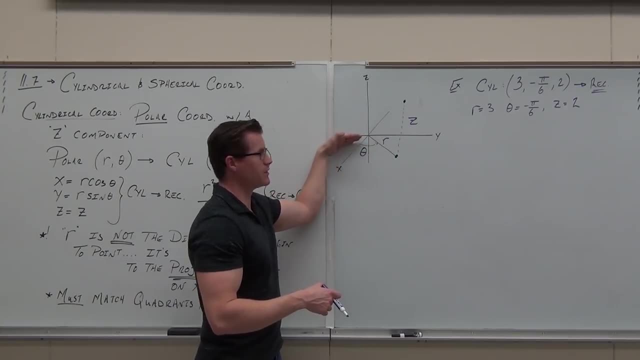 three units from the origin, flat on the plane. three units, and then my angle. where's my angle? Negative, So from here I'd be going this way. Do you guys see what I'm talking about? You've got to pretend like you're looking down at it. 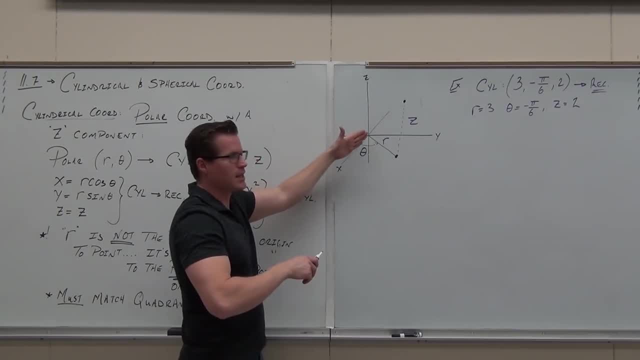 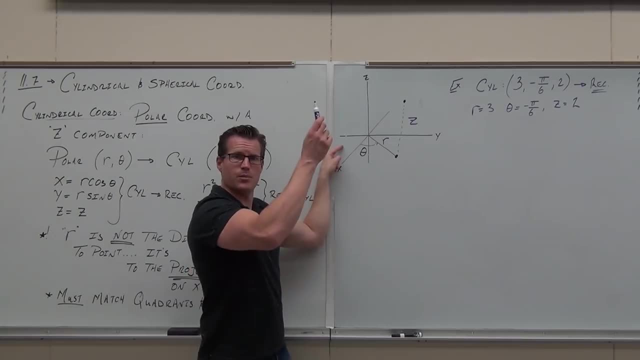 I'm going down Negative angle. I'm going this way, So this is going. 3, negative angle: It's over here somewhere And then is it going up or is it going down. Where's it going Up, Then it's going to shoot up here a little bit. 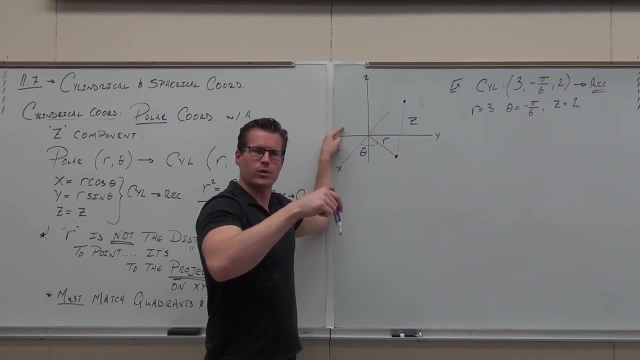 What quadrant would the projection be on? 4. Perfect, What octant are we in? 4. 4. And then we drop down 5,, 6,, 7,, 8. So we are in quadrant 4.. 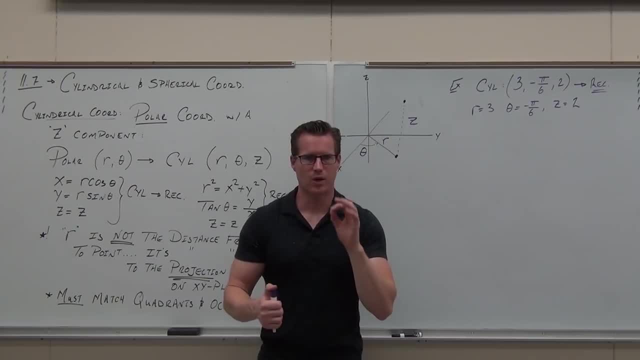 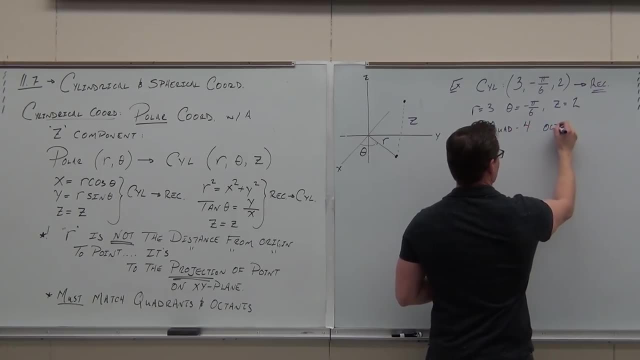 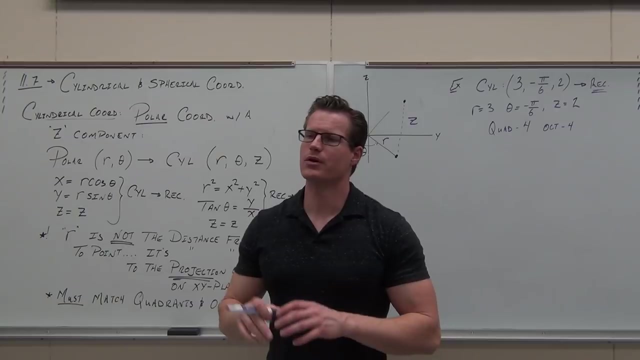 We're also in octant 4.. Does that make sense? Write that down. The reason is- and not necessarily going from cylindrical to rectangular because you don't have any option there, It's going to be one thing, But going from rectangular to cylindrical you get options for the theta. 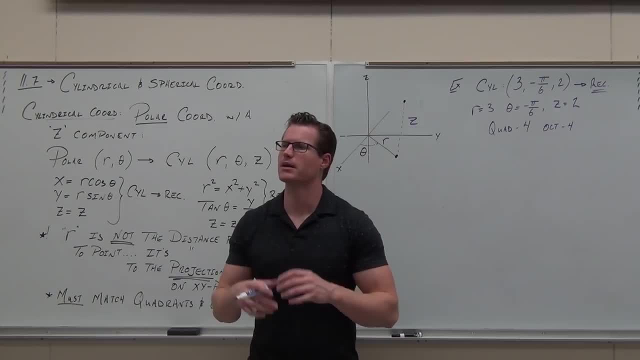 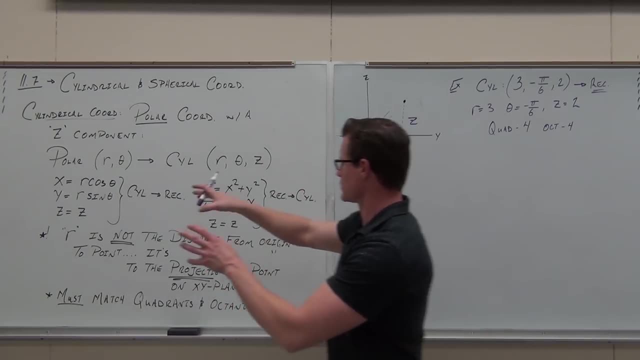 You absolutely have to match up the quadrants because you can make some mistakes here. So anyway, let's give it a try. Let's go over here and see If we're going from cylindrical to rectangular. this is the only step I have to use. 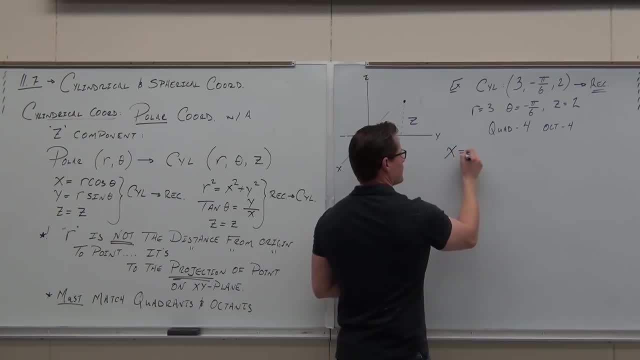 So let's see if we can fill it out. If I want to get x, x is always no matter what- r, cosine, theta. Hey, do you get an r? That's why I write this stuff down. Do you have a theta? 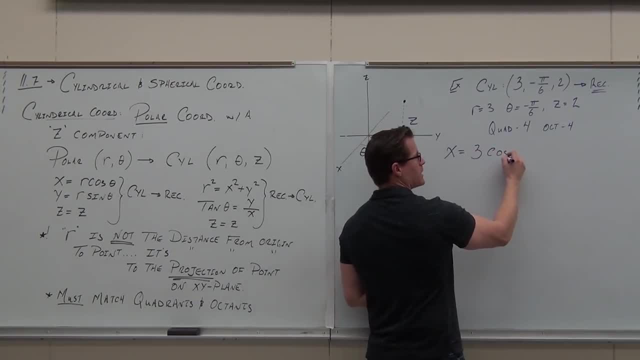 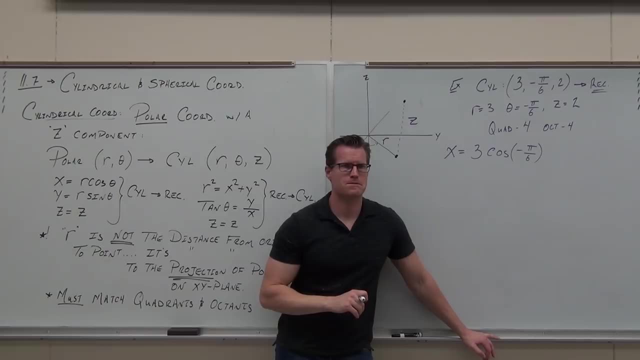 Yes, That's all you need. So we're going to have 3 times cosine of negative pi over 6.. For goodness sakes, please do not, freaking, give me decimals Ever. Square roots and fractions: All right. Unit circle people. 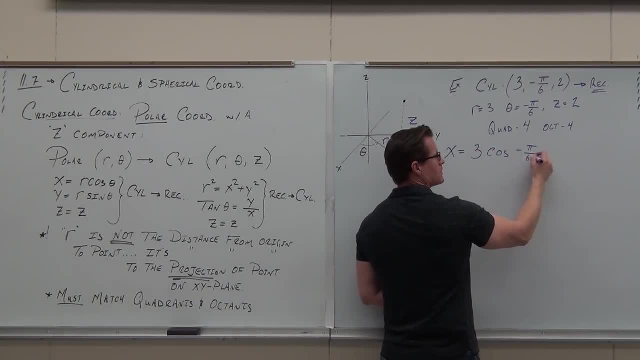 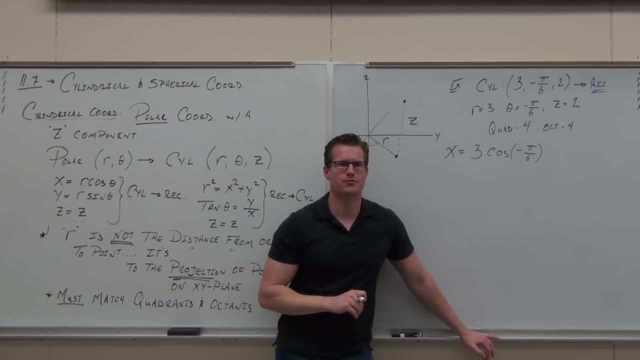 three times cosine of negative pi over six. for goodness sakes, please do not freaking. give me decimals ever. square roots and fractions, all right. unit circle- people tattooed right there. that's what I want to see someday. I really do want to see that. even Hannah, I know. 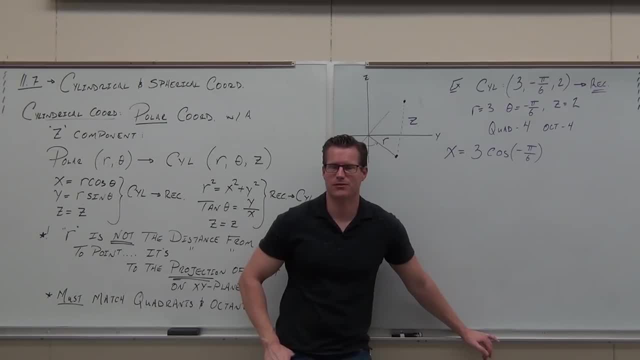 I want like a legit, but whatever I'll take. Hannah, if it's under skin you can't cheat, it's there, right? so okay, can you figure out what three times cosine of negative pi over six is? because if you can, that will give you the x coordinate. 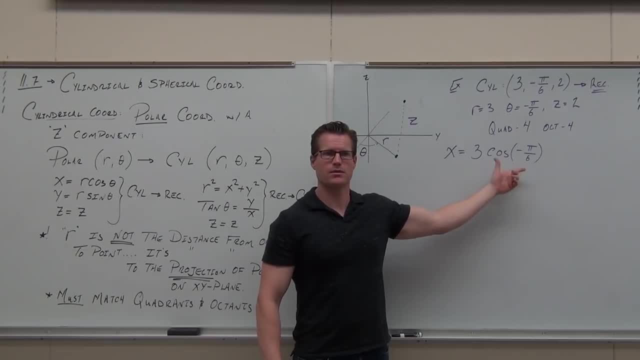 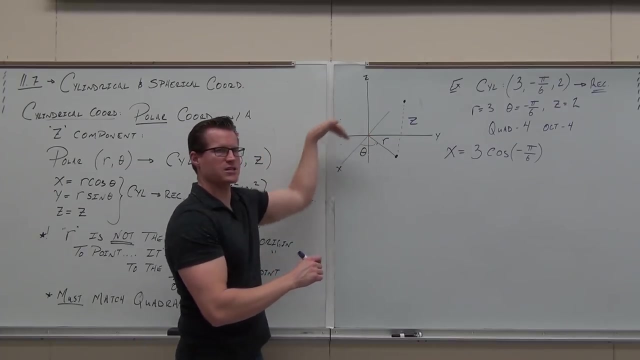 what is what's cosine of negative pi over six? do you know? I don't know. it's, it's, it's, it's, it's, it's, oh, it's, it's, oh, it's positive. hey, would you look what the point is? do you see the? it's going to be. 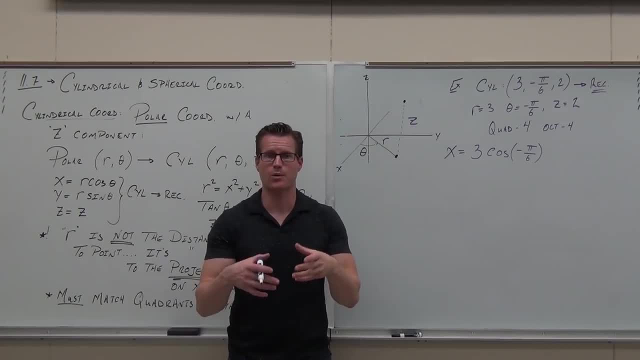 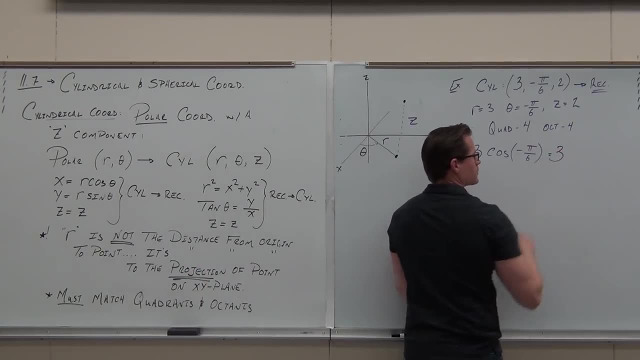 here right, and that's the projection. x has to be positive. it has to be: cos is positive in quadrant four, oh, pardon, in quadrant four. that's why we can think about these things more, writing them down, so we don't make negative, positive mistakes. that's why we think. 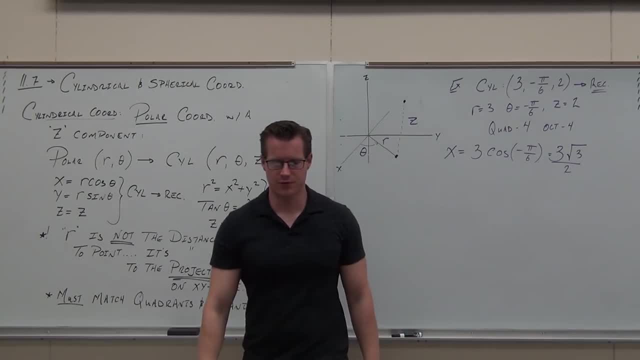 where it is. so this is going to be 3 times root, 3 over 2.. Let's try the y. The y says we're going to do 3, still the r sine theta. So we have the same exact numbers, except we have a different trig function. 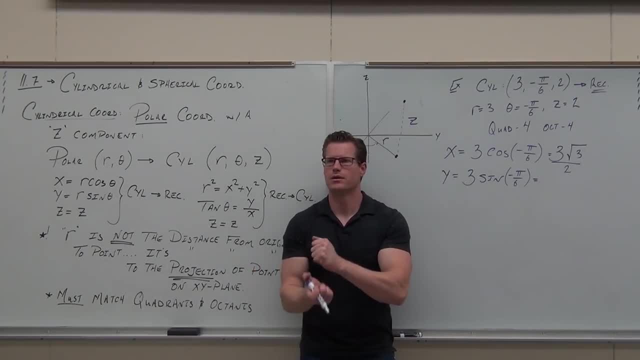 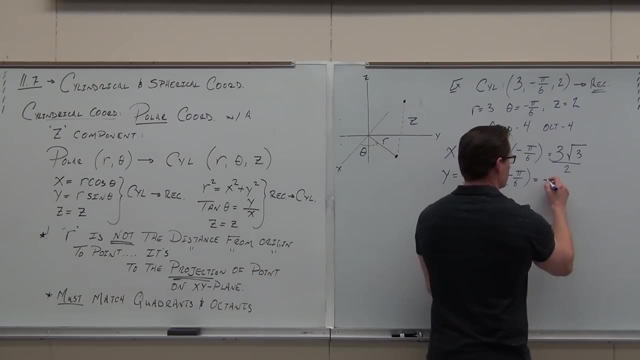 How about 3 times sine? What's sine of negative? Negative 1 half. Negative 1 half because in quadrant 4, sine is negative. We're in quadrant 4, negative. So negative 3 times 1 half. negative 3 halves. 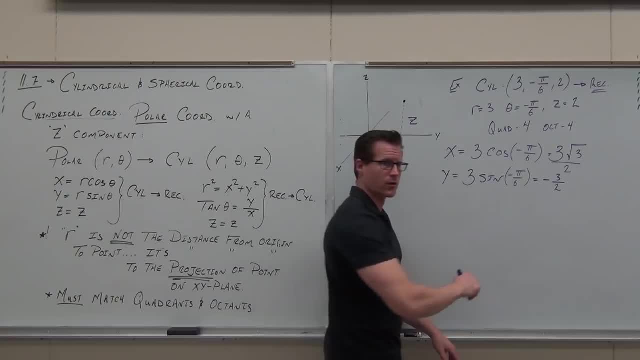 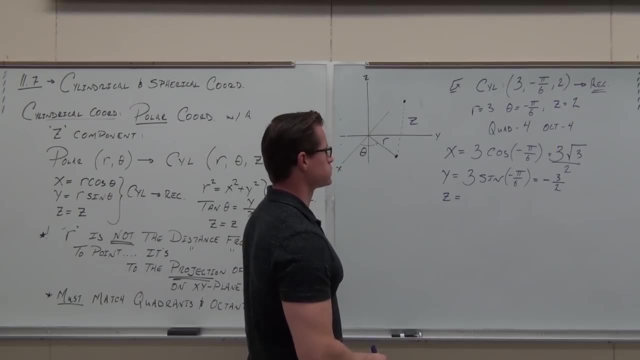 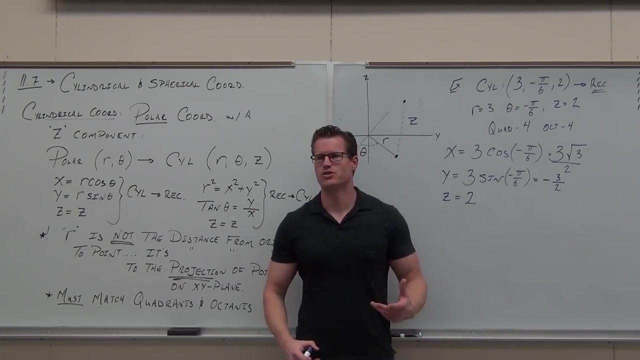 With me Tell you what. there's a hard one coming up, but I'll handle it for you all right, Z? I know it's ridiculous, I'm going to take a wild guess. Pretty sure, Pretty sure. Hey, yeah, I know I'm just joking, but do you have an x-coordinate? 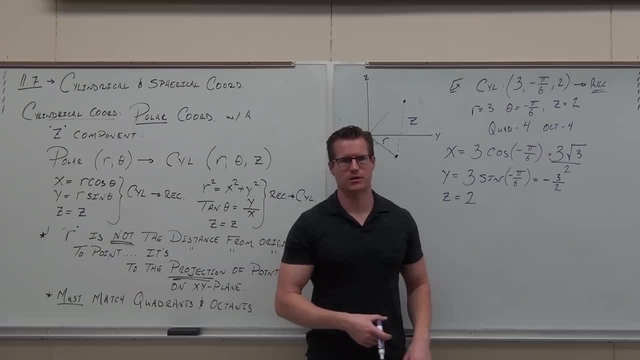 Do you have a y-coordinate? Do you have a z-coordinate? You now have a rectangular. That's how we change from cylindrical to rectangular. It's literally the plug and numbers here. It's literally just polar to rectangular. the same thing. 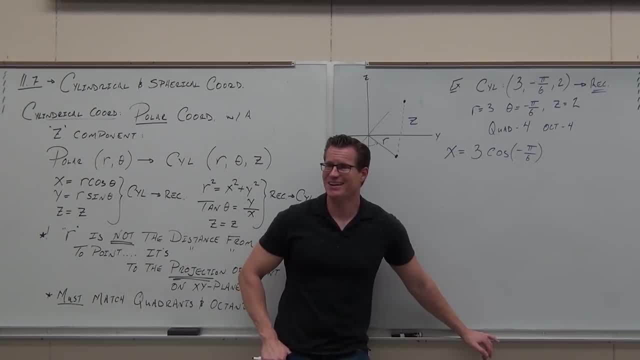 Tattooed Right there. That's what I want to see Someday. I really do want to see that, Even Hannah. I know I want like a legit, but whatever I'll take, Hannah, If it's under skin, you can't cheat. 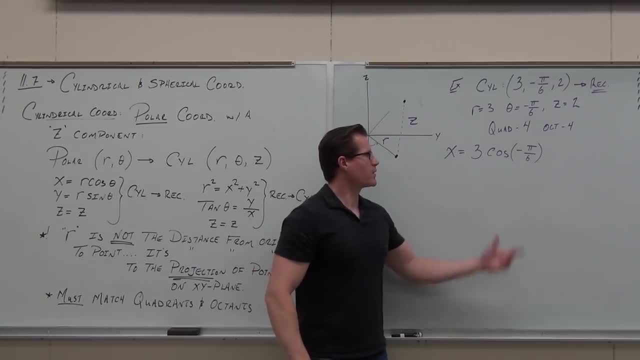 It's there, right. So okay, Can you figure out what 3 times cosine of negative pi over 6 is? Because if you can, that will give you the x coordinate. What is cosine of negative pi over 6?? Do you know? 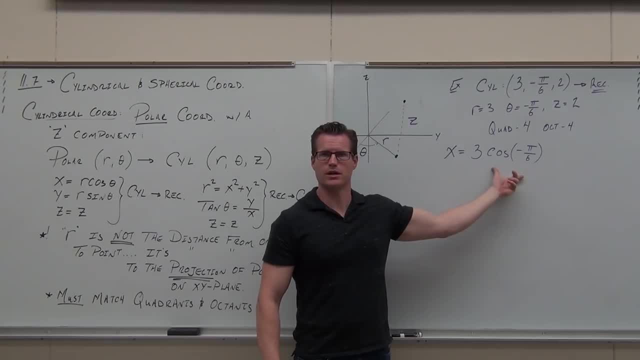 Is it positive or negative, Positive, Positive. Hey, would you look at this? It's negative, Negative, Negative, Positive, Negative, Negative, Negative, Negative, Negative. Look where the point is. Do you see that? It's going to be here, right? 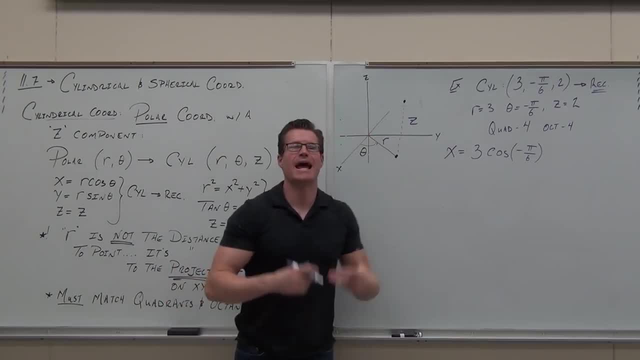 That's projection X has to be positive, It has to be Cosine is positive in quadrant four. Oh, quadrant four. That's why we think about these things. We want to write them down so we don't make negative, positive mistakes. so why we think? 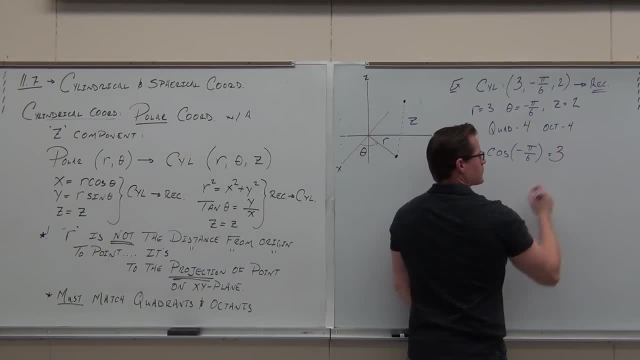 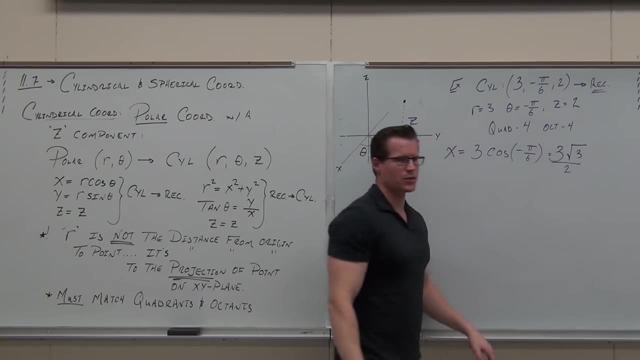 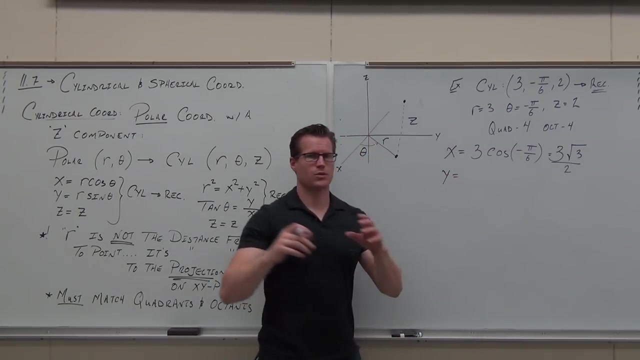 about where it is. So this is going to be 3 times which it was 3 over 2.. 3 times root 3 over 2.. Let's try the y. The y says we're going to do 3, still the r sine theta. 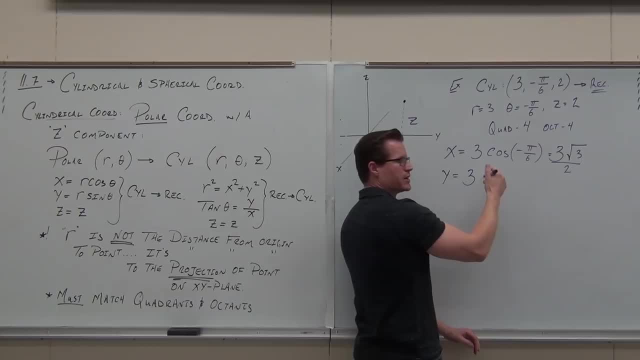 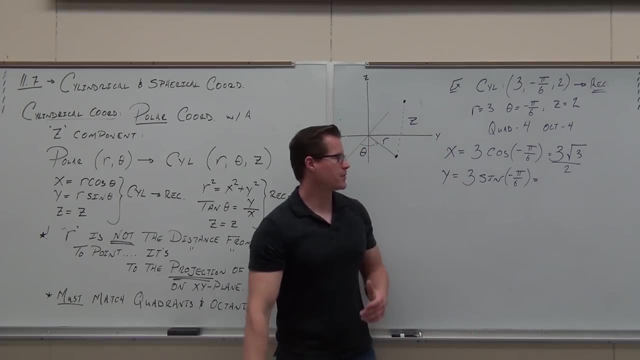 So we have the same exact numbers, except we have a different trig function. How about 3 times sine? What's sine of negative? How many strokes Negative? 1 half. Negative 1 half because in quadrant 4, sine is negative. 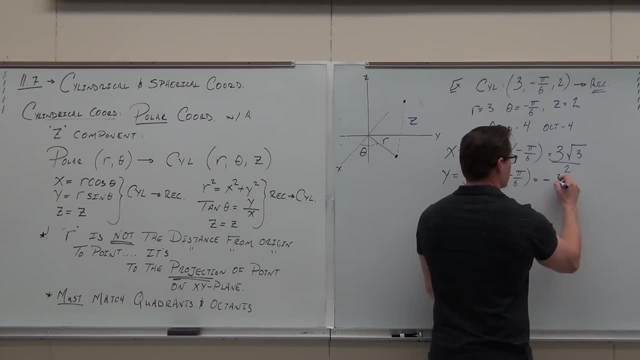 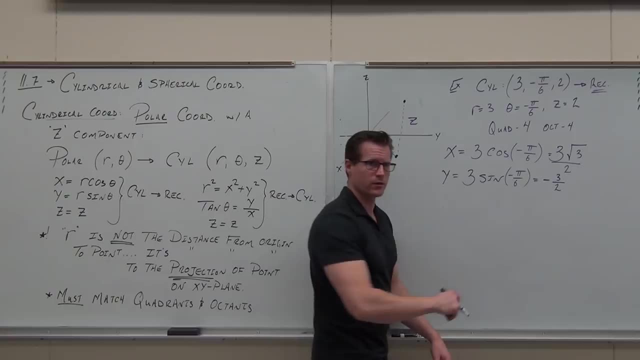 We're in quadrant 4, negative Sure. So negative 3 times 1 half. negative 3 halves. With me Tell you what. there's a hard one coming up, but I'll handle it for you all right. 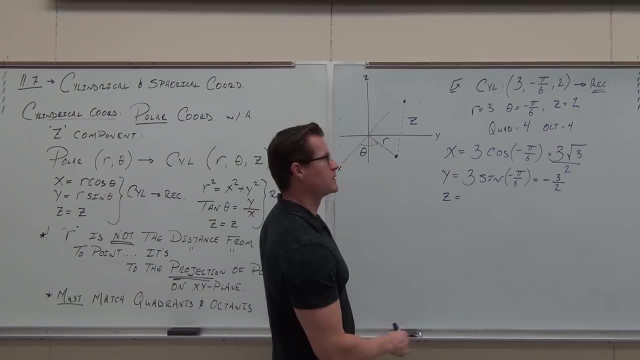 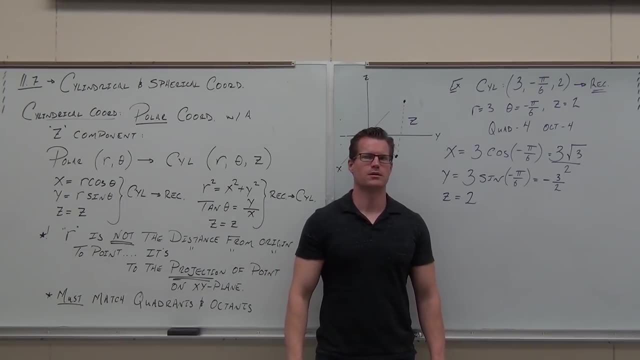 Z. I know it's ridiculous. I'm going to take a wild guess. Pretty sure, Pretty sure. Hey, yeah, I know I'm just joking, but do you have an x coordinate? Do you have a y coordinate? 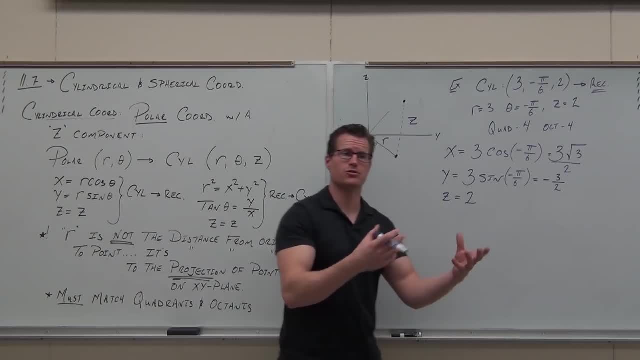 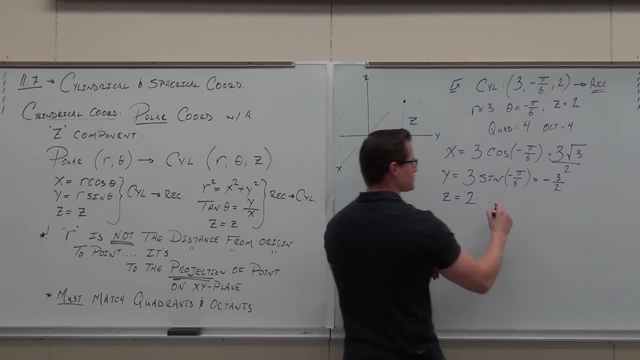 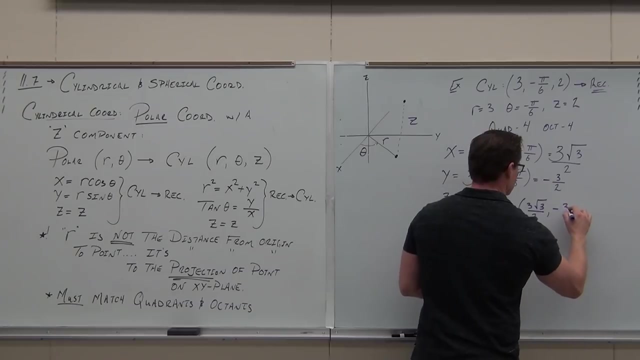 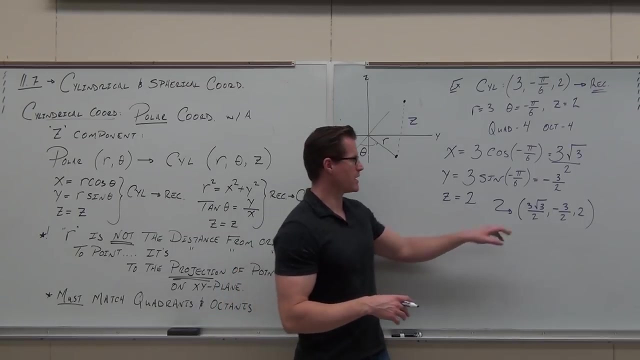 Do you have a z coordinate? You now have a rectangular point. That's how you do it. It's literally just polar to rectangular, the same thing. So our point now is that Just make sure we're in the same exact quadrant, same exact octant. so we're going to check it out. 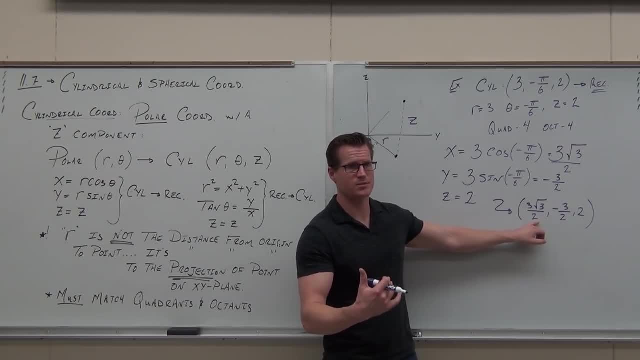 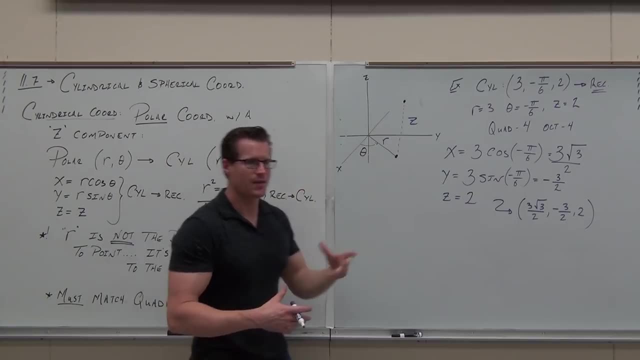 I don't care exactly where it's at, just make sure our quadrants match up and octants match up. This is our x, that's our y, Our x says positive, Our y says negative And our z says positive. That puts us in the same quadrant on the plane and it puts us in the same octant when we have. 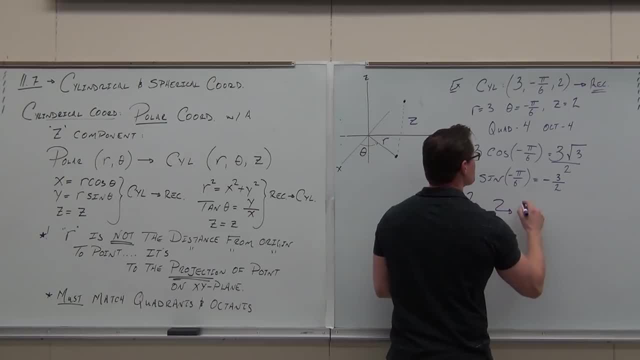 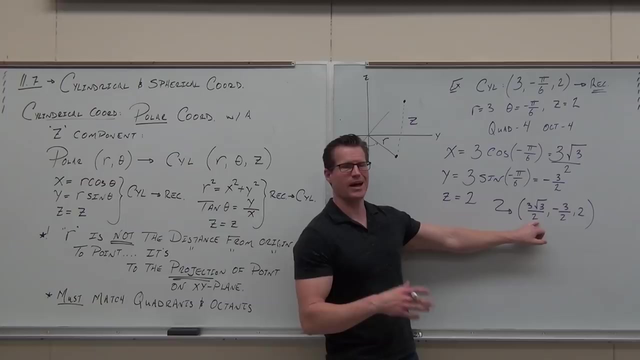 So our point now is that Just make sure we're in the same exact quadrant, same exact opt-in. So we're going to check it out. I don't care exactly where it's at, Just make sure our quadrants match up and opt-ins match up. 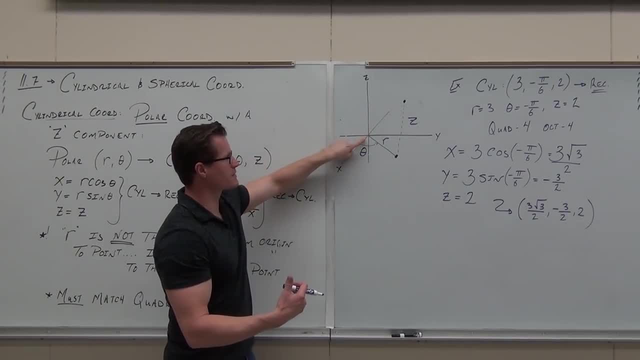 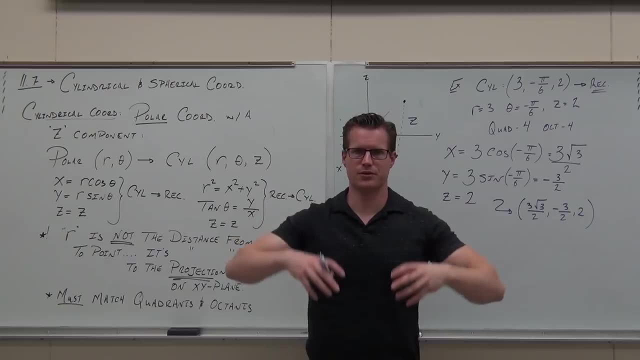 This is our x, that's our y, Our x. Our y says positive, our y says negative and our z says positive. That puts us in the same quadrant on the plane and it puts us in the same opt-in when we have a 3D coordinate system. 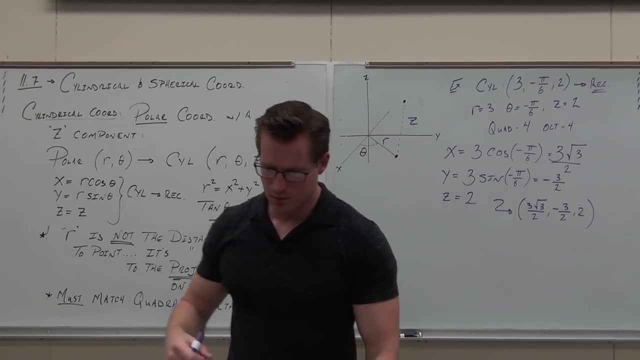 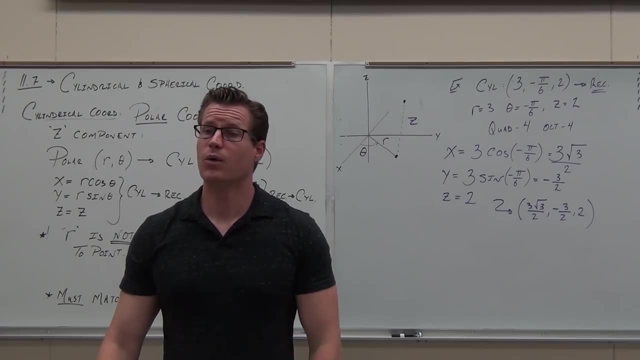 So you guys feel okay with that one. That's the idea. Tell you what. we're going to move a little quickly here, because that idea it's exactly the same every single time, every time. What I do want to do is go from rectangular to cylindrical. 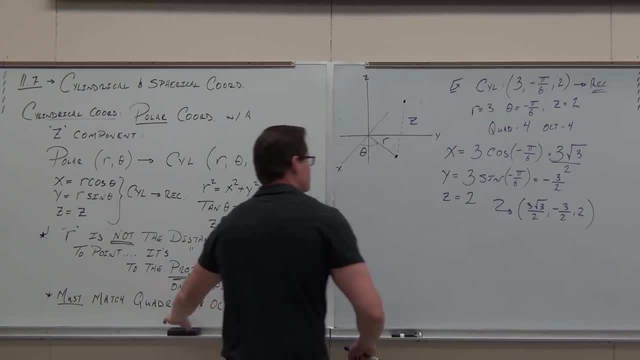 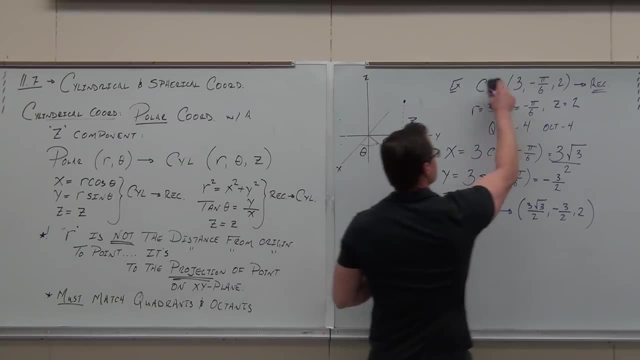 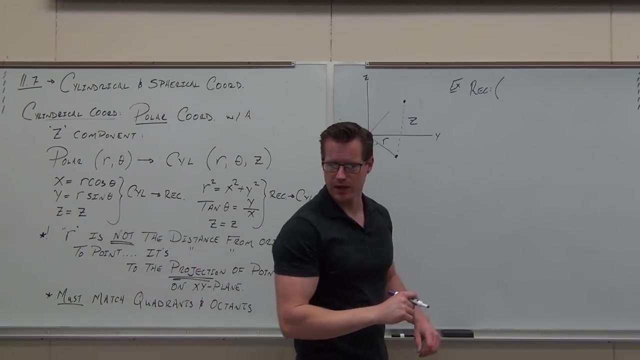 You guys ready to do that? Let's try that. Any questions at all, Because I'm going to work over here for real. anything at all? Okay? So, rectangular, I'm going to give you square root of 2, negative square root of 2, and 4.. 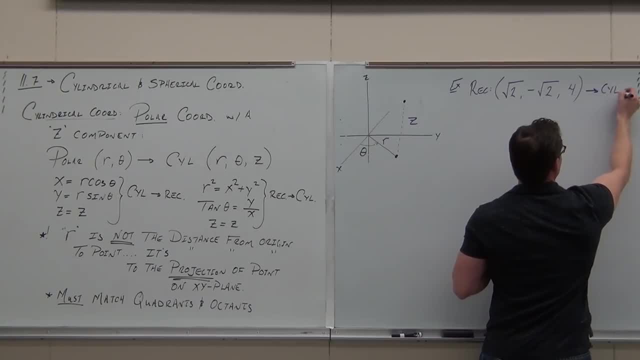 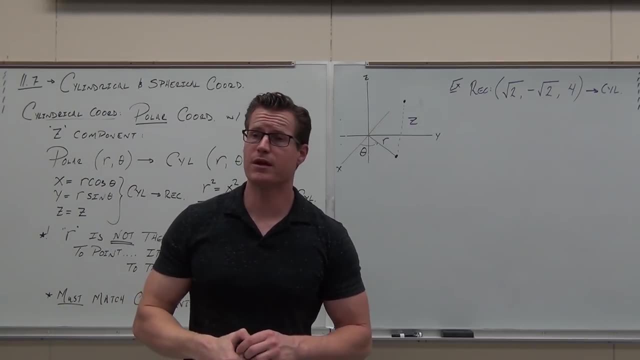 And I want to change this to cylindrical. I want to save the 1950 helps, because that helps. Hey, number 1 thing, man, when you're converting this, you got to make sure what quadrant and what opt-in you're in right from right off the start. 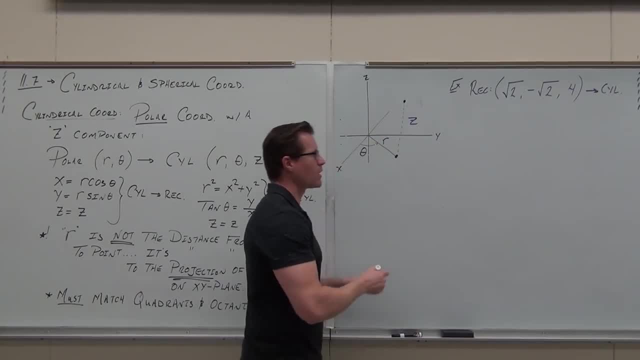 So let's think about where that's at. If we draw a little separate picture here, We're in rectangular coordinate system. Just give yourself an approximation. Is my x, What is? can you identify my x, My z, My w? 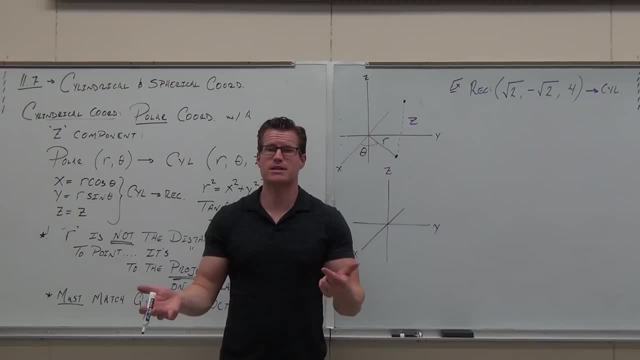 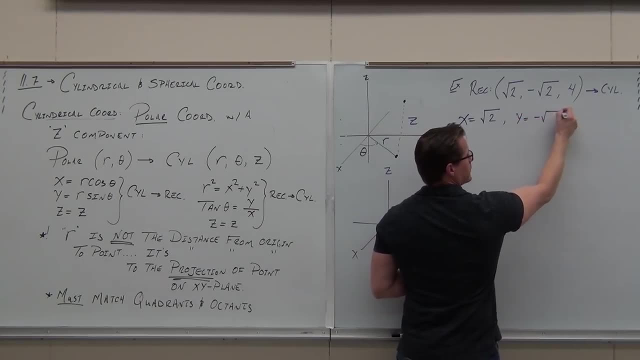 my y and my z, because if I'm in rectangular I should have those things. Can you identify it? What is my x, please, And my y? Negative root of 2.. Negative root of 2. And my z. 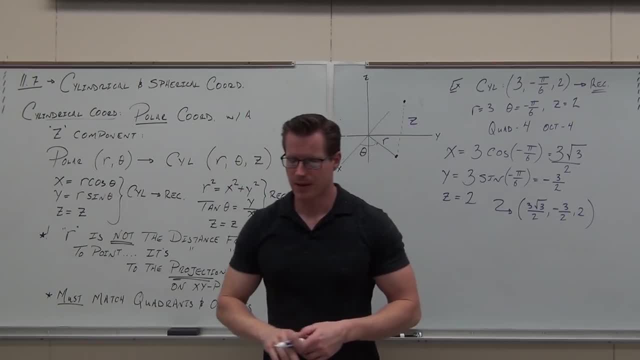 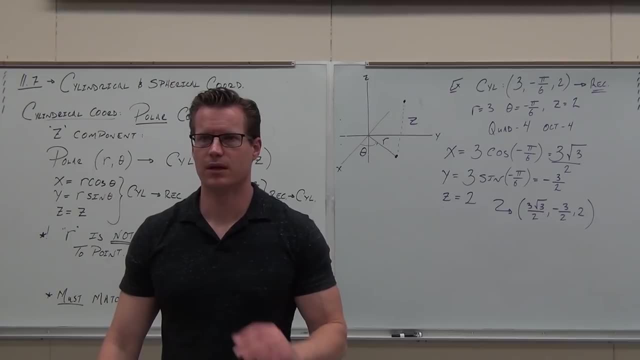 a 3D coordinate system. Do you feel okay with that one? That's the idea. Tell you what. we're going to move a little quickly here, because that idea it's exactly the same every single time, Every time. 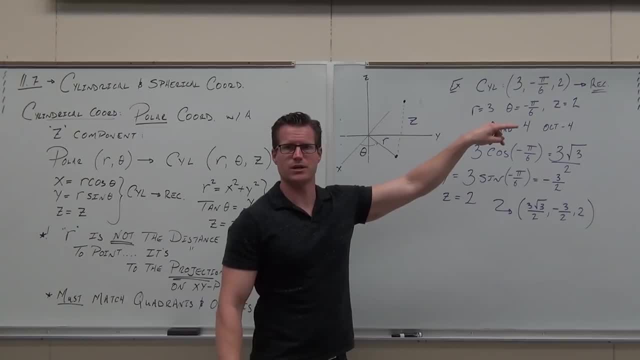 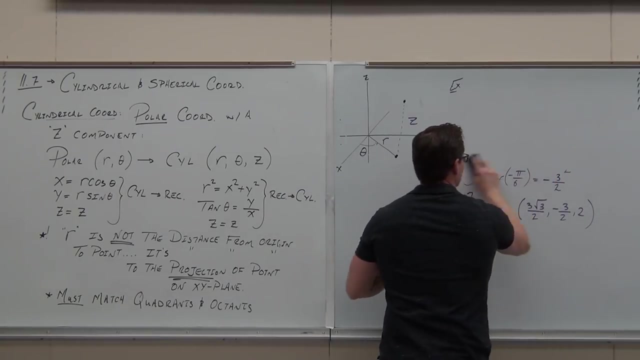 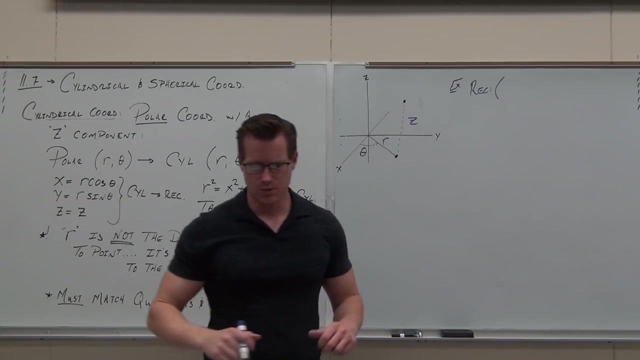 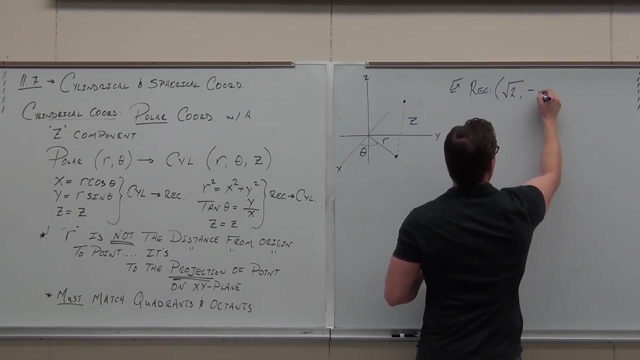 What I do want to do is go from rectangular to cylindrical. Are you guys ready to do that? So let's try that. Any questions at all, because I'm going to work over here. Anything at all, Okay. So, rectangular, I'm going to give you square root of 2,, negative square root of 2, and 4.. 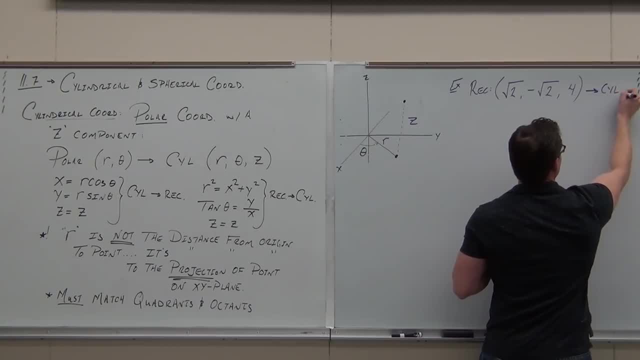 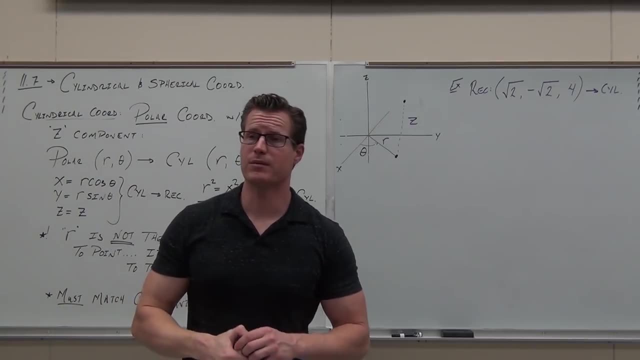 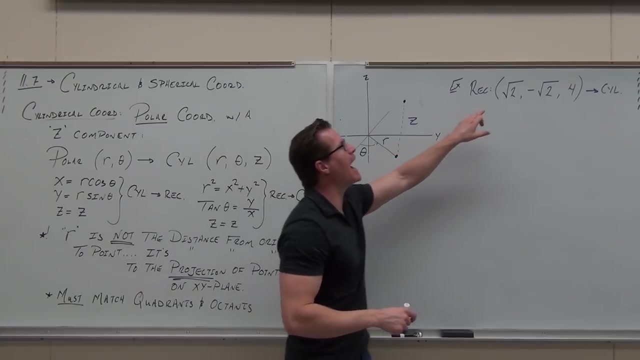 And I want to change this to cylindrical. Okay, Number one thing, man: when you're converting this, you've got to make sure what quadrant and what octant you are in right off the start. So let's think about where that's at. 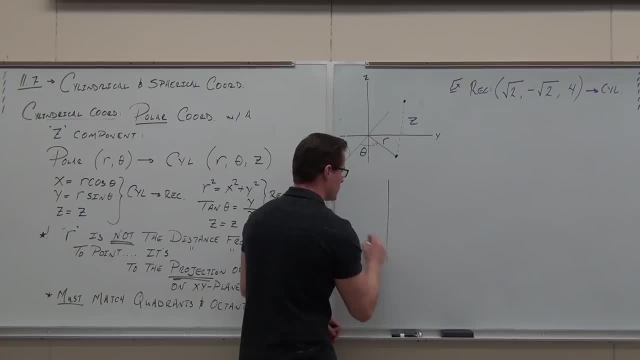 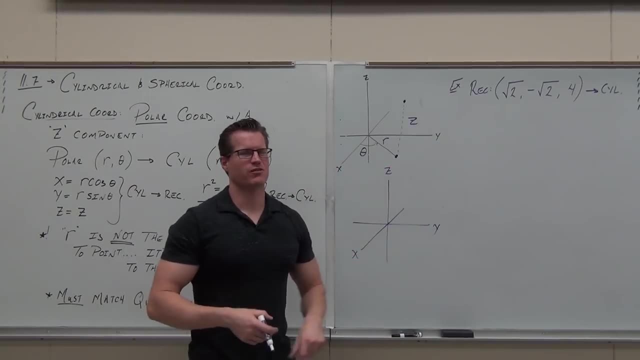 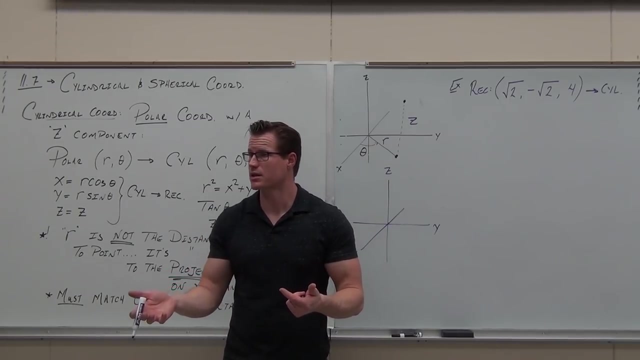 If we draw a little separate picture here, we're in a rectangular coordinate system. Just give yourself an approximation: Is my x, what is it? Identify my x, my y and my z, because if I'm in rectangular I shouldn't have those. 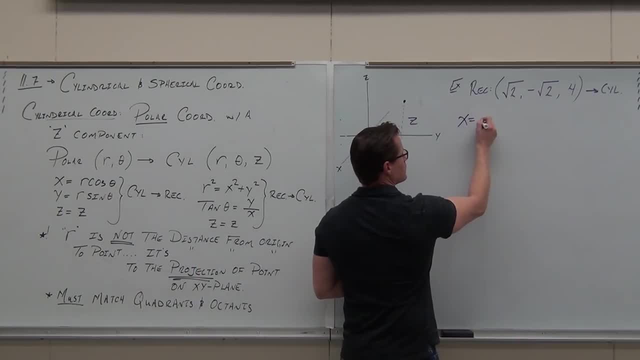 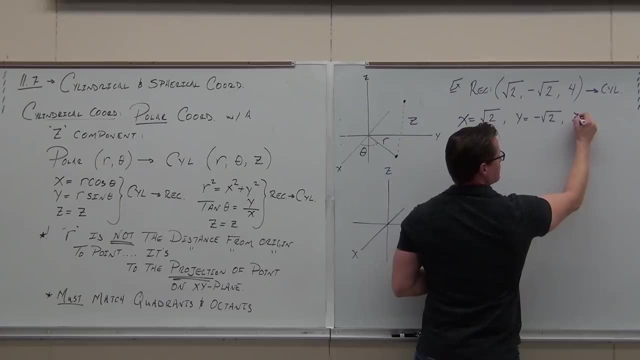 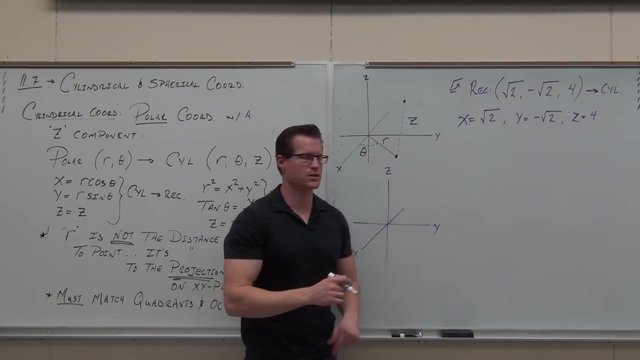 things. Can you identify it? What is my x, please, And my y And my z? So back to like 11.2,. when we first started plotting points, We first go x. would I go positive or negative along the x? 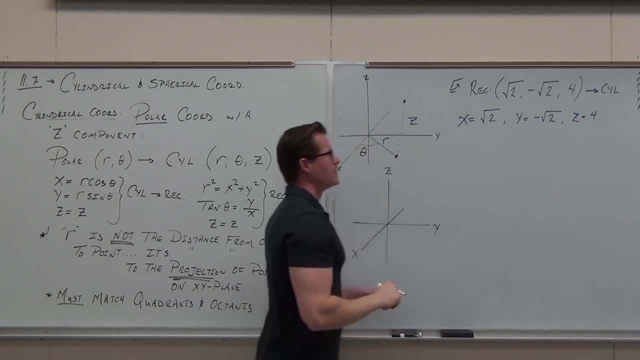 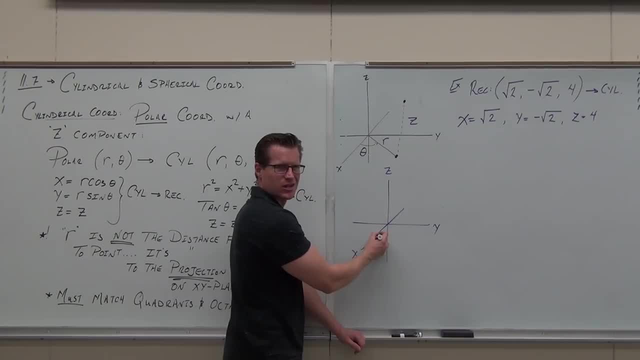 Positive. So I'm out here somewhere- okay, I don't care exactly where, Just somewhere. Would I go positive or negative, along the y Positive. So I'm going to go this way. Does that make sense? I'm still in the x y plane. 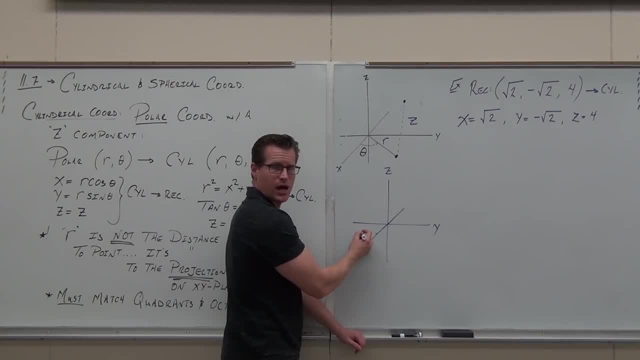 I am in quadrant what Four, Four Beautiful. Do you guys see the quadrant four I'm talking about? Whatever we get, we better make sure we match up the quadrant four And then from there am I going to be going up or down? 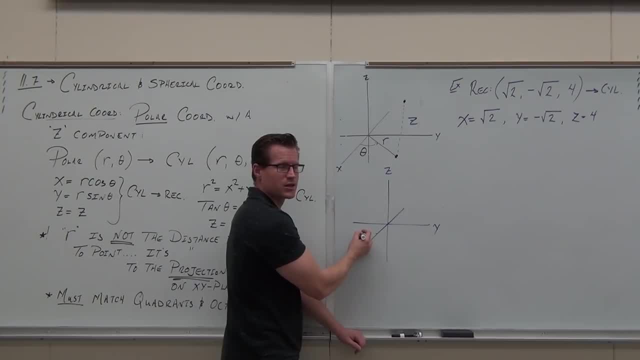 Up. So I'm like here, somewhere over here. I'm right there, I'm in quadrant four, I'm in octant four. Okay, So I'm out here somewhere over here. I'm right there, I'm in quadrant four. 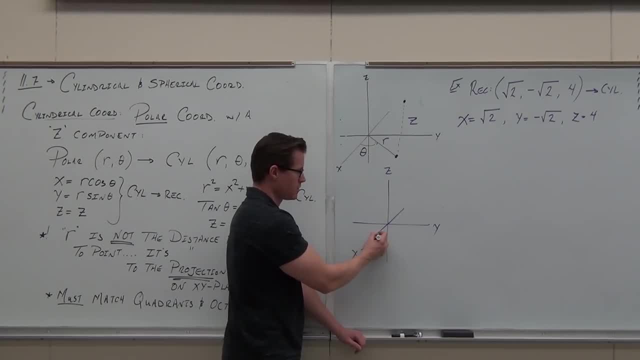 How about this? What'd I do? So as sure as you can see here when I go positive for negative, So I'm going to go this way. Does that make sense? I'm still in the claim. I am in quadrant what? 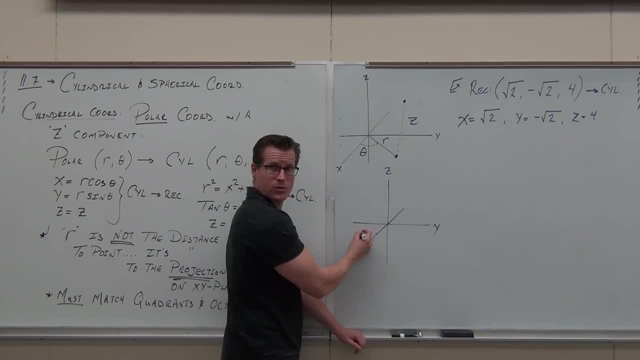 Four, Four Beautiful. Do you guys see the quadrant four I'm talking about? Whatever we get, we'd better make sure we match up with the quadriple 4.. And then, from there, am I going to be going up or down? 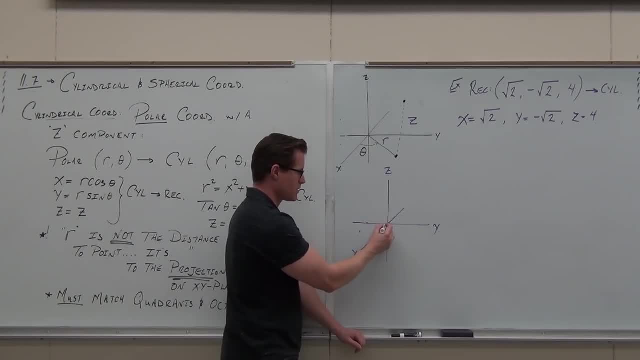 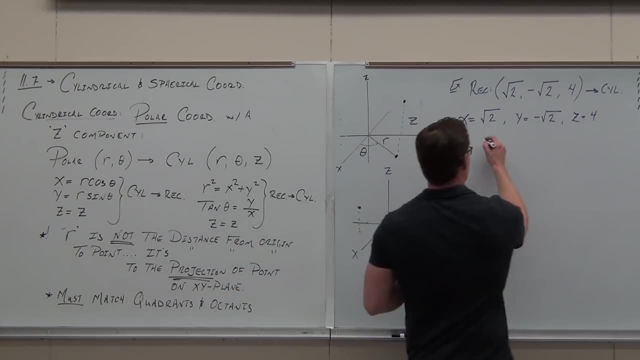 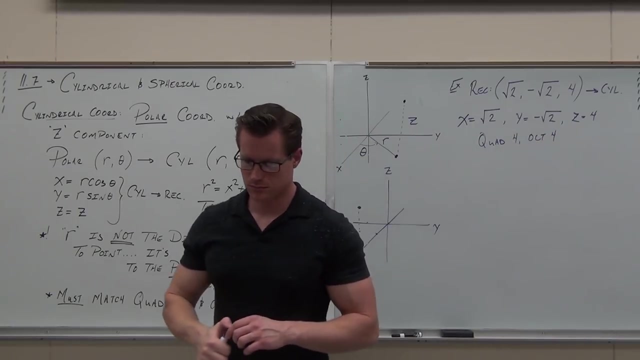 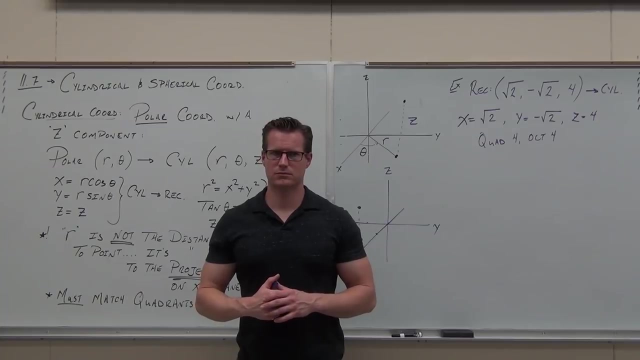 1. 1.. So I'm like here, somewhere over here. I'm right there, I'm in quadrant four, I'm in. Are you sure you're okay? Oh yeah, you're making eye contact, All right. 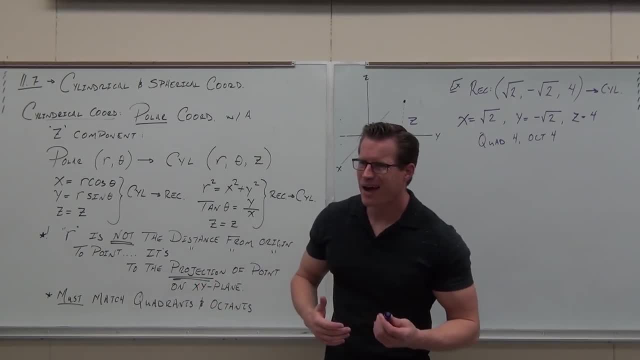 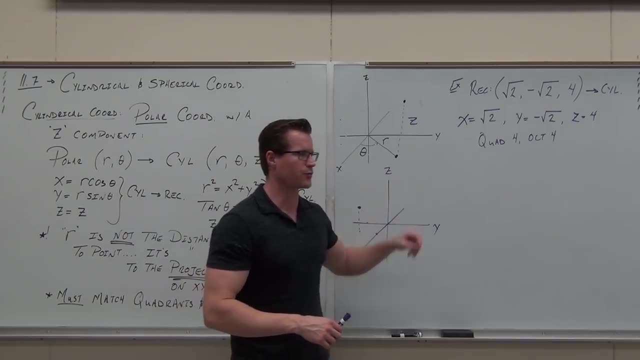 Are you sure you're okay? Sure, Not too bad, but you have to visualize. It's kind of weird. You're in 3D, right. So we're positive X, negative Y, positive Z. We're in octant four for sure. 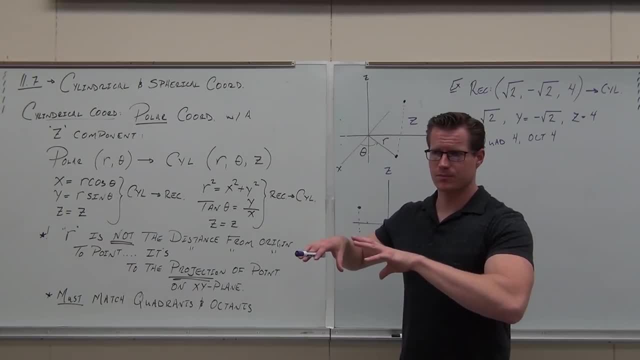 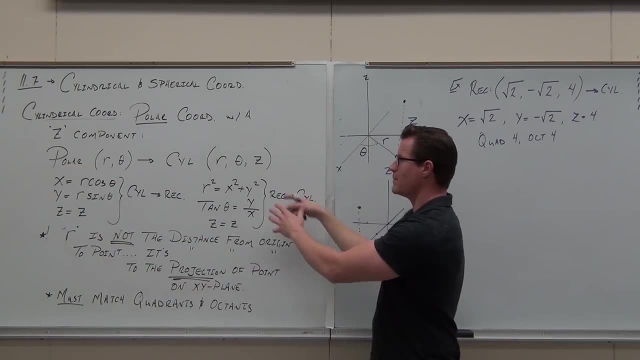 Let's translate this to cylindrical. If we want to go from cylindrical to rectangular, we've got this Plug in the thetas and R's, you get X Y Z. If I want to go from rectangular to cylindrical, I'm going to have X Y Z's and I want thetas and R's. 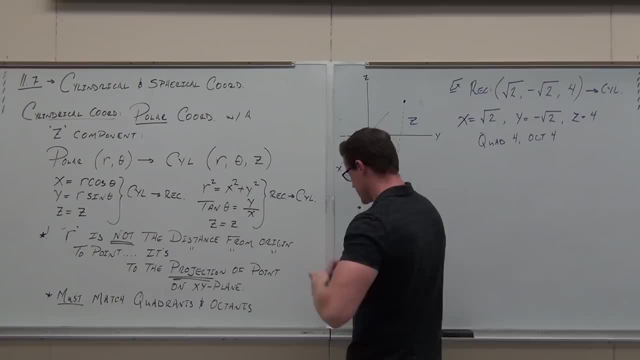 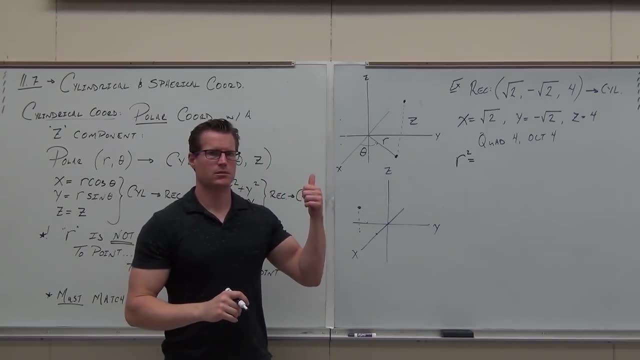 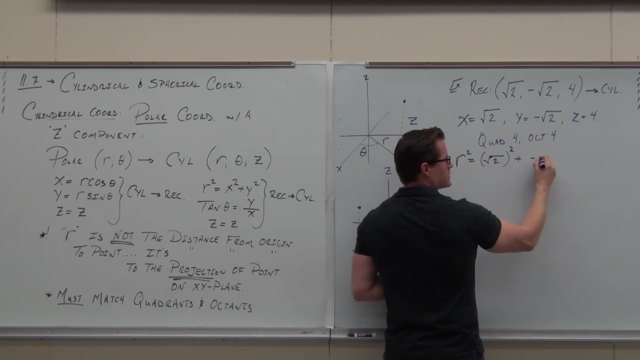 So we're going to have to use this stuff. Let's plug it in. So the first thing I notice is that R squared equals X squared plus Y squared. So R squared equals square root of 2 squared plus negative. I'm going to get a square root of 2 squared. 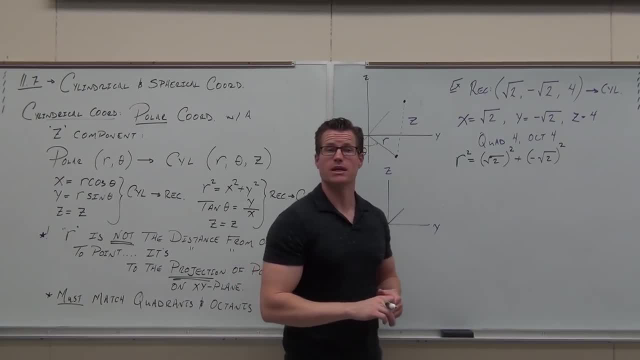 Now you're liking those square roots right. I know How much do we get All of a sudden. how much do we get? R squared equals what? Hopefully you got 4.. Did you get 4?? Okay, What do you do next? 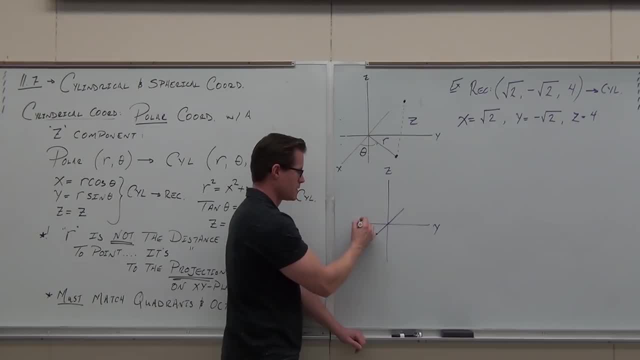 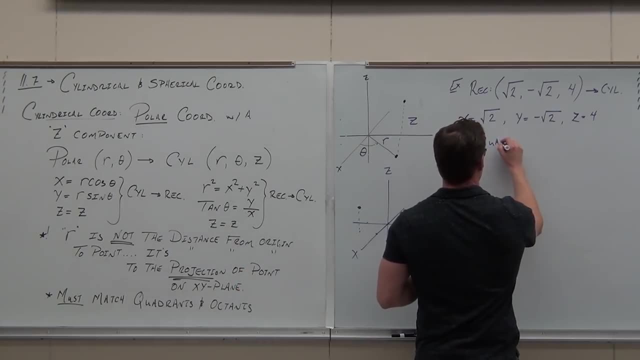 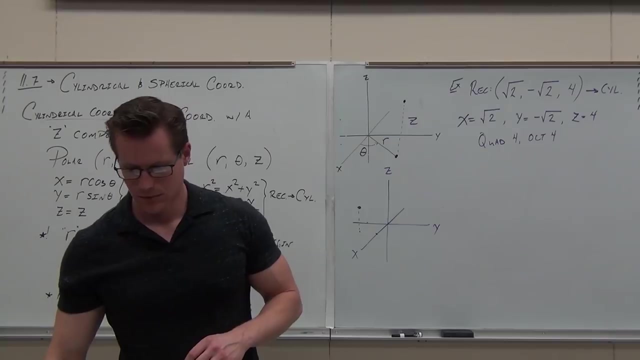 I'm in octant four. Okay, So I'm out here somewhere over here. I'm right there. I'm in quadrant four. I'm in octant four, You sure you're okay? Oh yeah, you're making eye contact. 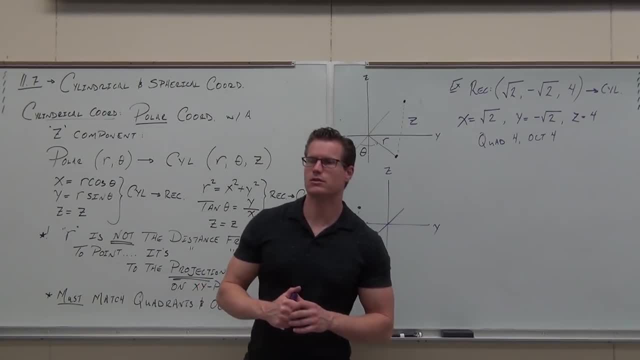 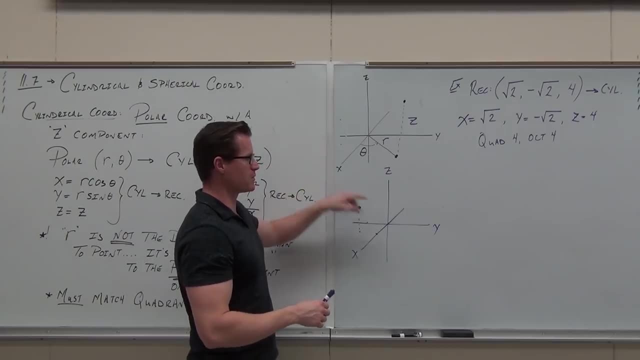 Alright, You sure you're okay. Sure, Not too bad, but you have to visualize. It's kind of weird. You're in 3D, right? So we're positive x, negative y, positive z. We're in octant four. 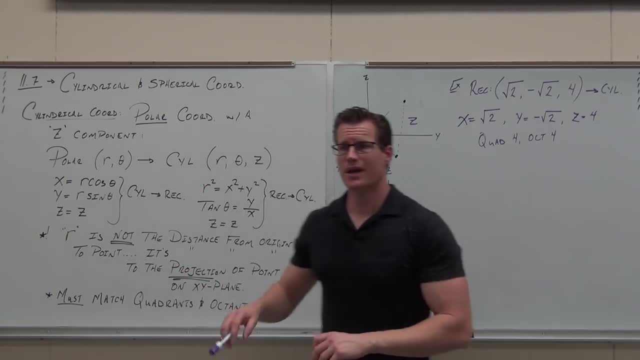 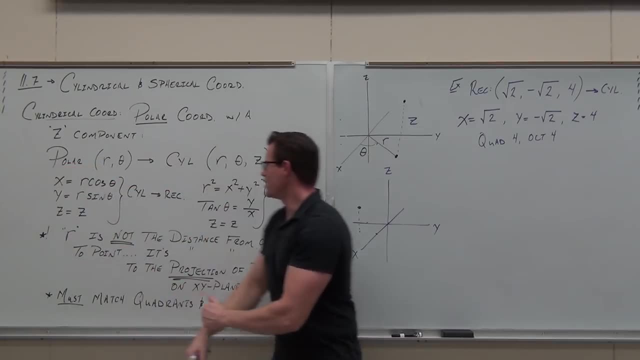 Okay, We'll do that for sure. Let's translate this to cylindrical. If we want to go from cylindrical to rectangular, we got this Plug in the thetas and r's, you get xyz. If I want to go from rectangular to cylindrical, I'm going to have xyz and I want thetas and. 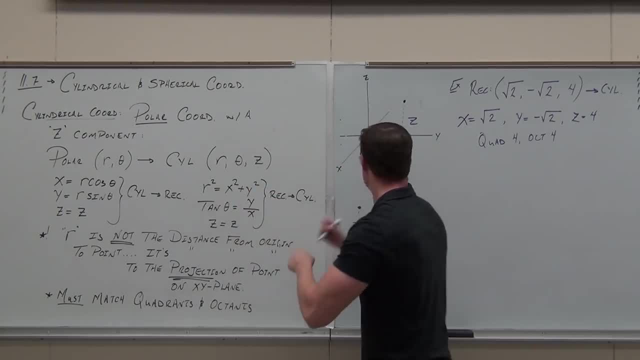 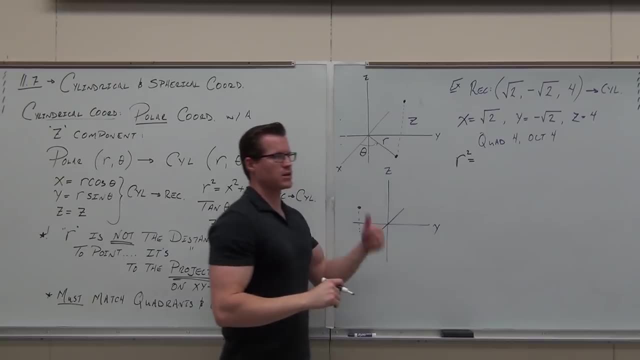 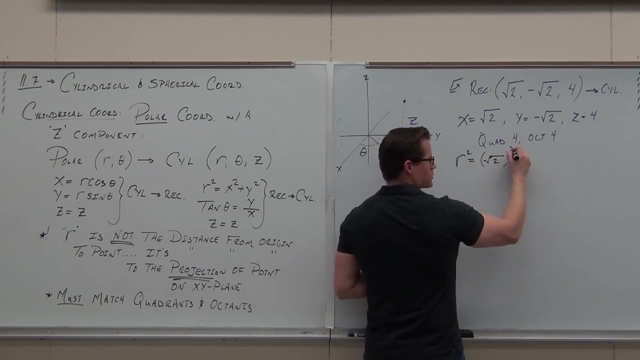 r's, so we're going to have to use this stuff. Let's plug it in. So first thing I notice is that r squared equals x squared plus y squared, So r squared equals square root of 2. Correct squared plus negative square root of 2 squared. 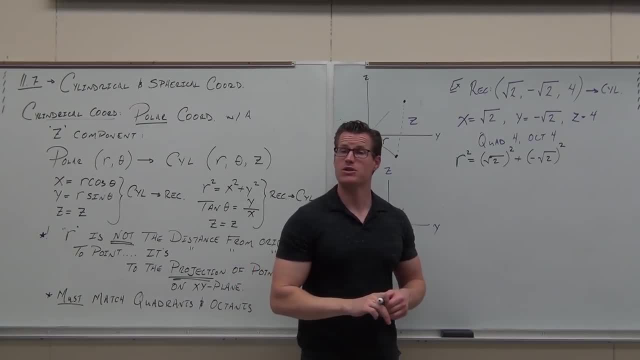 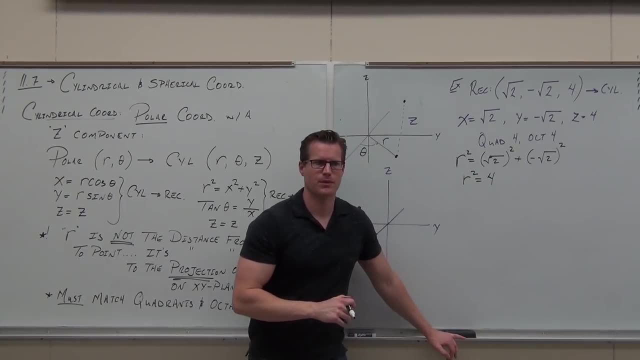 Now you're liking those square roots right. I know How much do we get All said and done. how much do we get? r squared equals what? 2.. Hopefully you got 4.. Did you get 4? Okay? 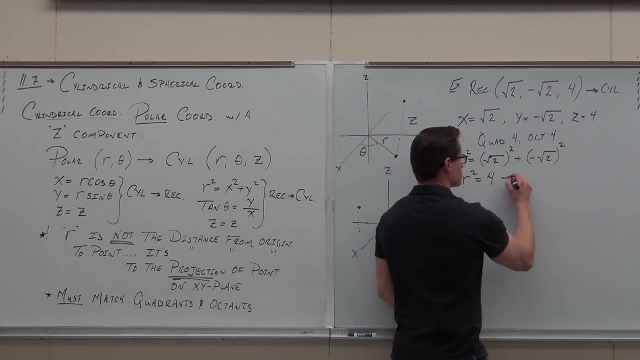 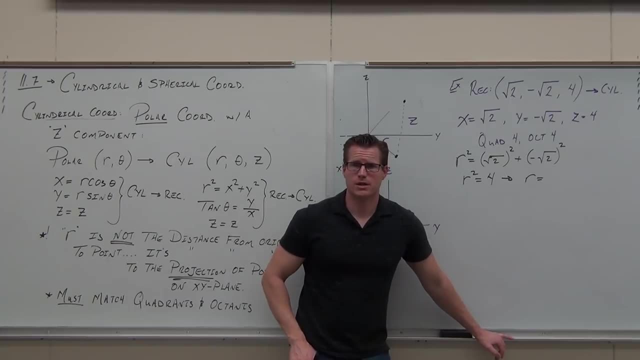 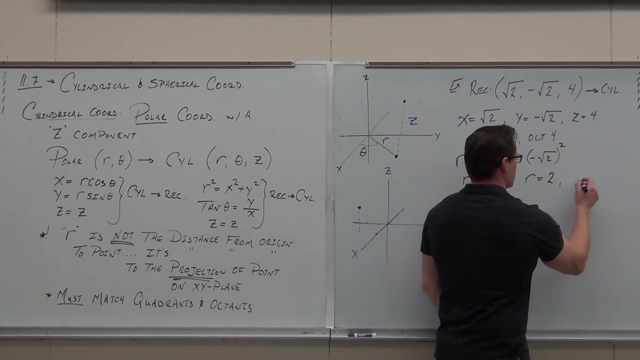 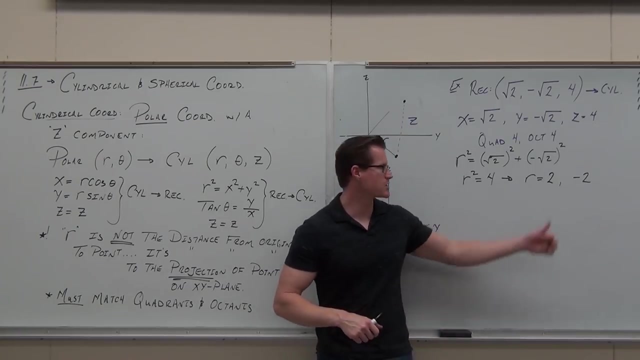 What do you do next? Square root: How much does r equal? How much does r equal 2 plus 2.. No, it's not 2.. Plus or minus 2.. We're going to talk about that Normally. my tip: 99.9% of the time. just take that one and you'll be fine. 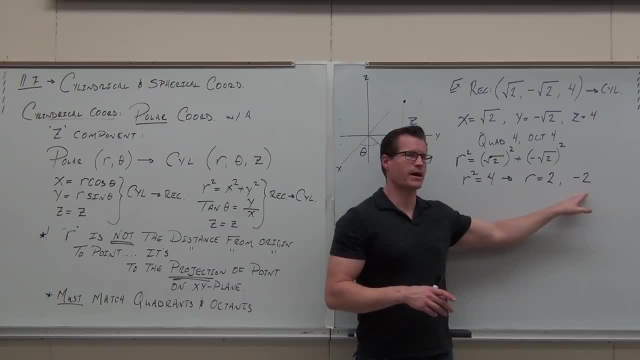 Take the positive 2.. But I want to show you why we have that and why we consider that one. Are you guys okay with that one? Most people just go: yeah, just pick 2.. Fine, whatever, Keep it positive. 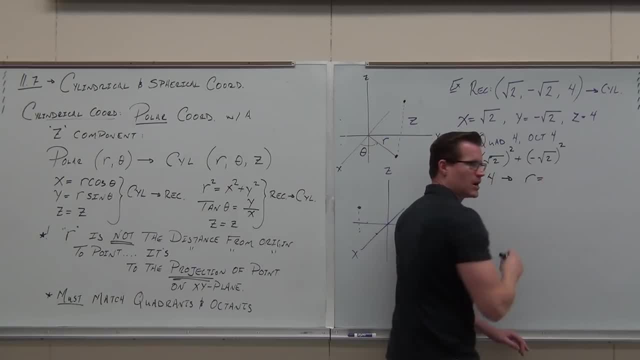 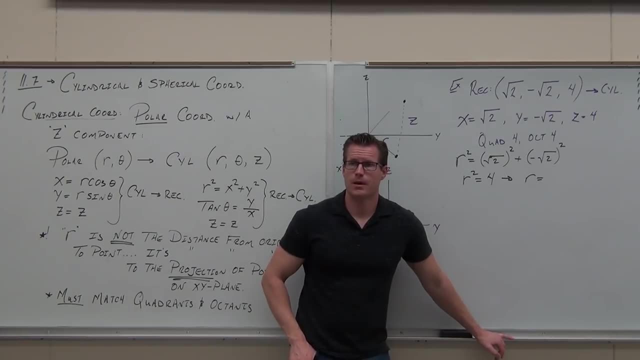 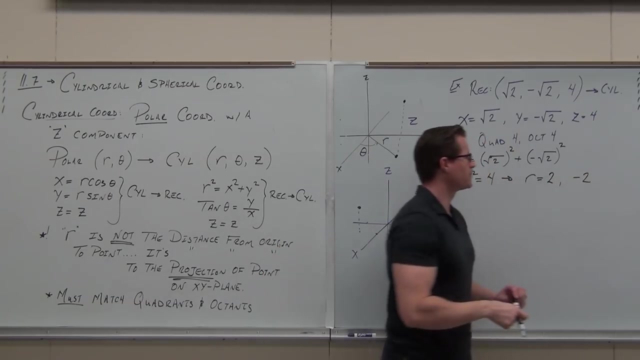 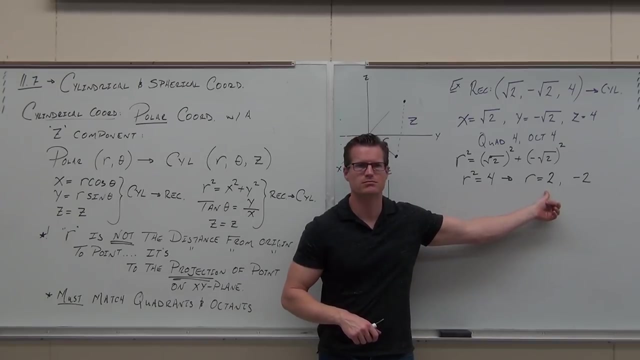 Square root. How much does R equal? How much does R equal Q plus 2.. No, it's not 2.. Plus or minus 2.. Plus or minus 2.. We're going to talk about that Normally like tip 99.9% of the time. just take that one and you'll be fine. 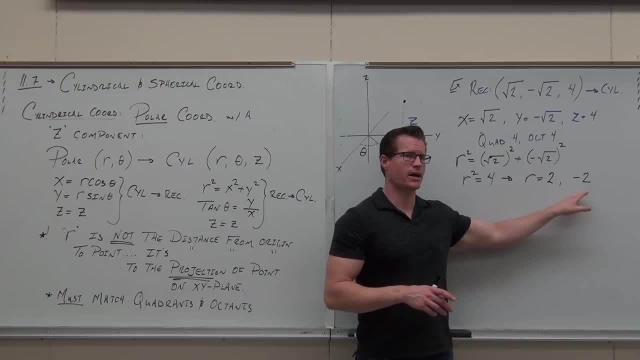 Take the positive 2.. But I want to show you why we have that and why we consider that one. Are you guys okay with that one? Most people just go: yeah, just pick 2.. Fine, whatever, Keep it positive. 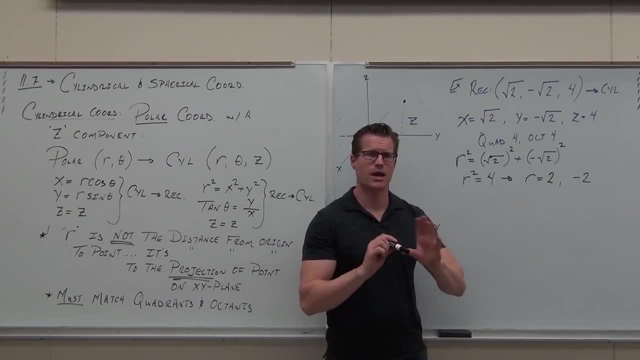 Hey, But we'll talk about why we get two different angles and how that works with this. Okay, So next part: Boom, We got it, We got R. What's the other thing we need? Come on quickly. What is it? 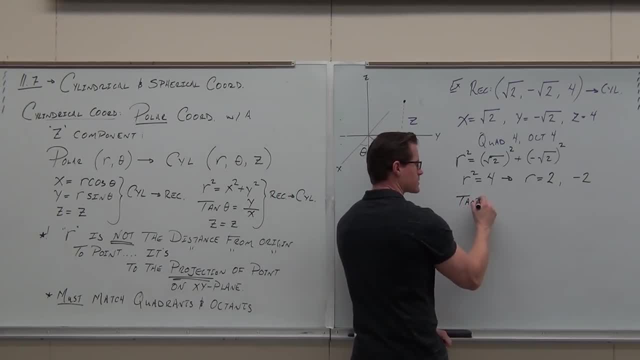 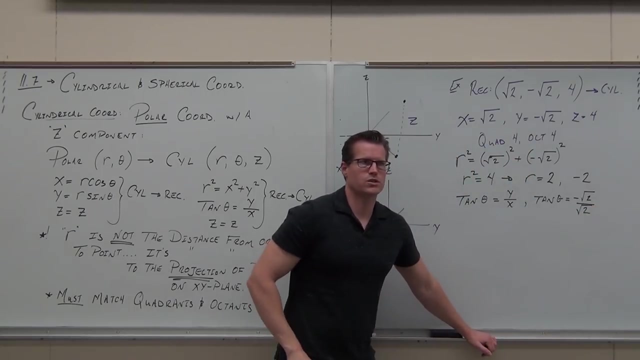 Theta, Theta. Whenever we talk about the thetas, we have this: Tan theta equals y over x, which means tan theta equals man. I gave you nice ones. Negative square root of 2 over square root of 2.. How much is negative square root of 2 over square root of 2?? 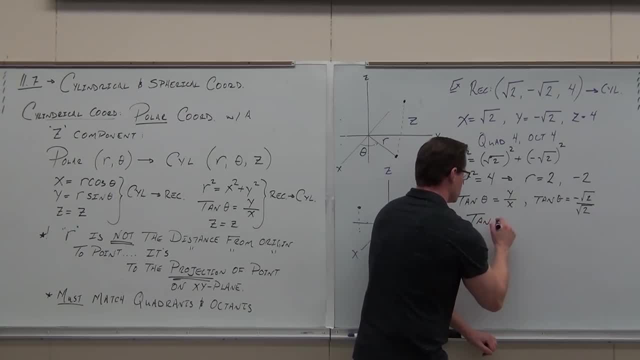 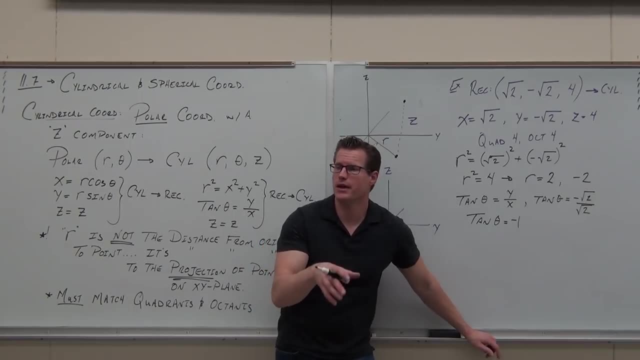 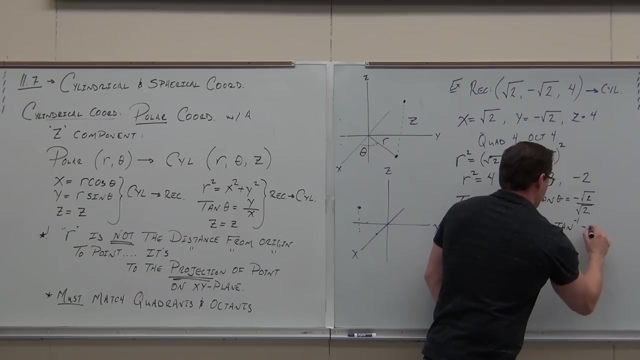 Negative: 1. From there you're fine, You can do it from there. Or if you want to do the theta, how do you find theta from right here? Come on, Can you tell me right now? and then here's the deal. 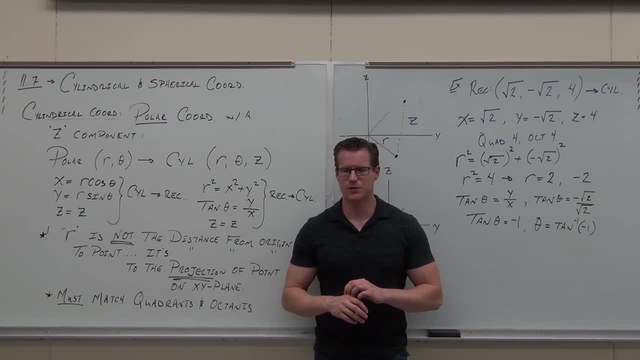 When we talked about polar, when you first did it, theta can go from 0 all the way to pi over 2.. It has the whole range there. So can you give me 2 values? Okay, 2 values of theta for which tangent is negative 1.. 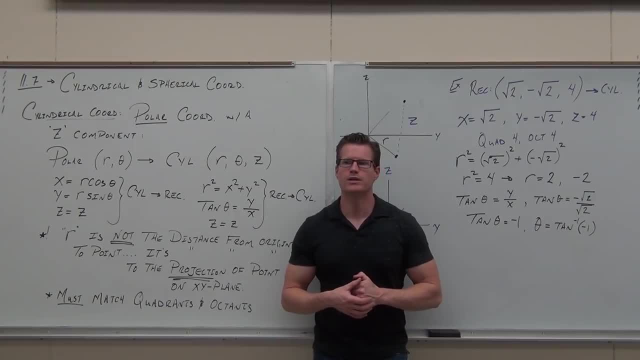 Or in other words tan inverse of negative 1, you're going to have 2 values there. We don't restrict it to that negative pi over 2 to pi over 2. We can go outside of that because we're on that plane. 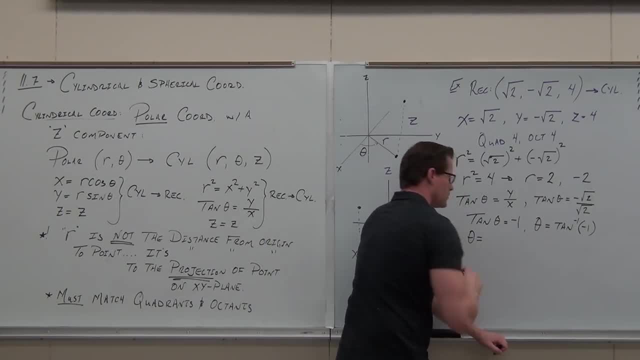 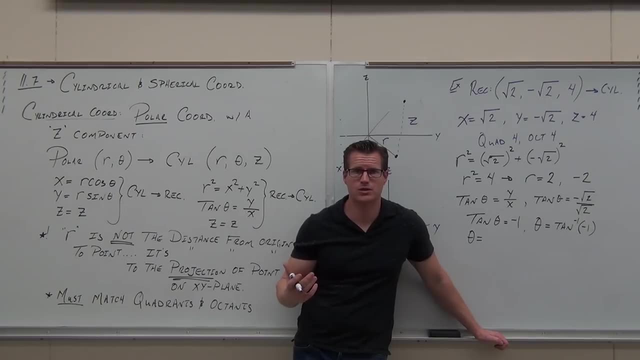 So how much is theta? Cosine and sine have the same values, but 1 is negative. Come on, That's quadrant 2 or quadrant 4.. Are you with me on this? Yes, What is it? 3 pi over 4.. 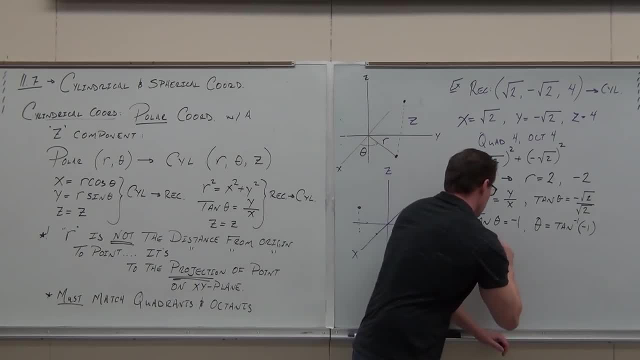 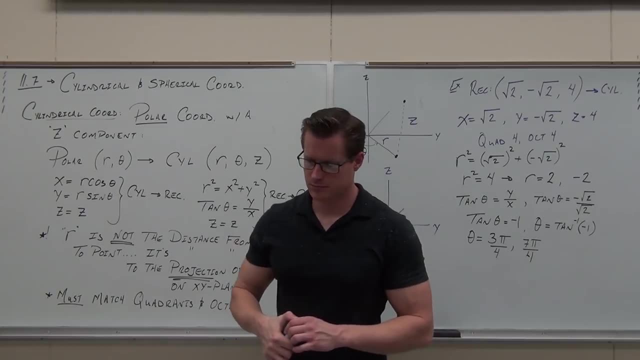 3 pi over 4 or 7 pi over 4.. Head and neck, you're okay with that one. So again, if you want a little side note, keep in mind that theta goes from 0 to 2 pi. 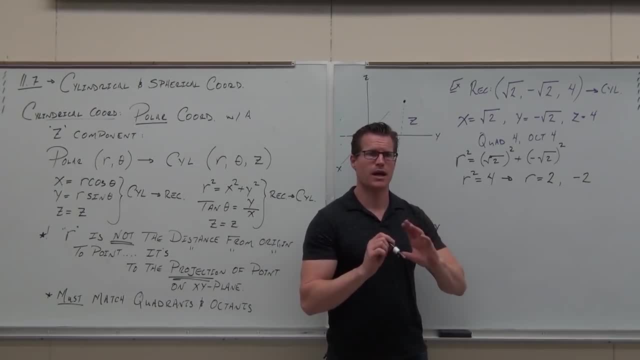 Hey, But we'll talk about why we get two different angles and how that works with this. Okay, So next part: boom, we got an r. what's the other thing we need? Come on quickly, what is it, Theta? 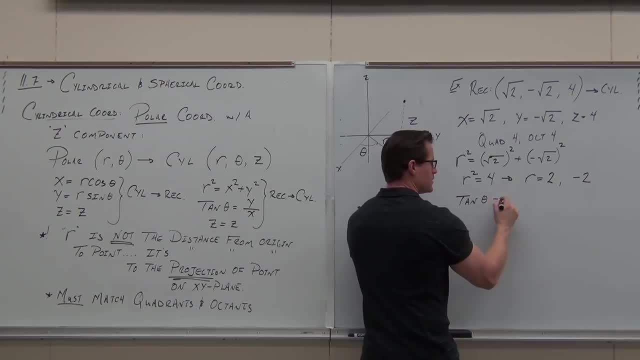 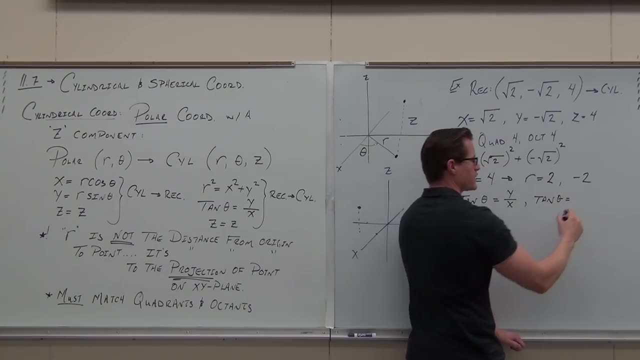 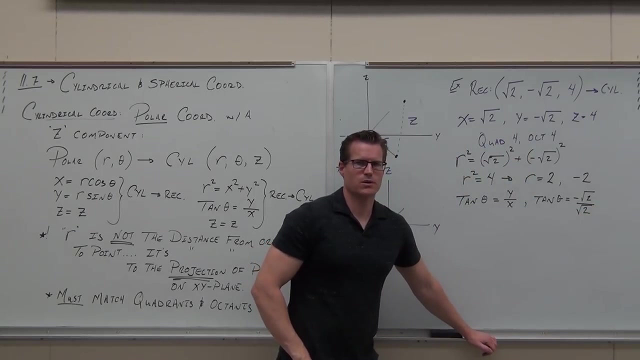 Theta. Whenever we talk about the thetas, we have this: Tan theta equals y over x, which means tan theta equals man. I gave you nice ones. Negative square root of 2 over square root of 2.. How much is negative square root of 2 over square root of 2?? 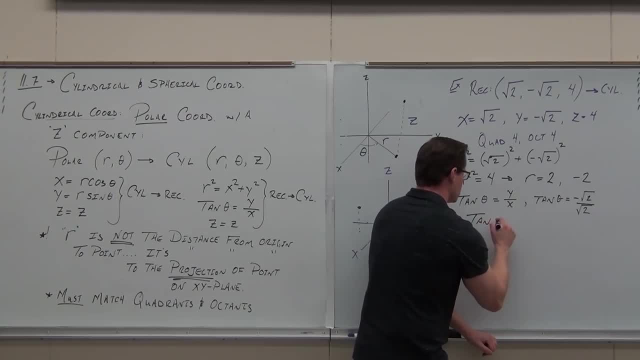 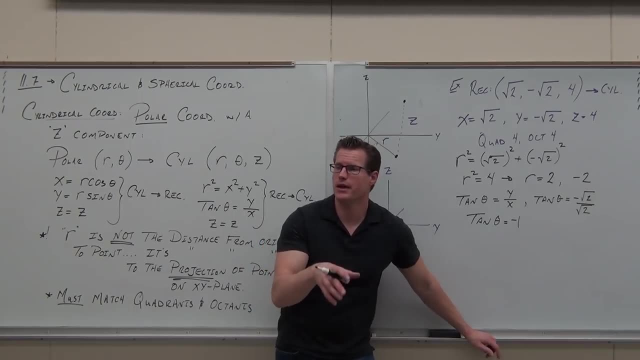 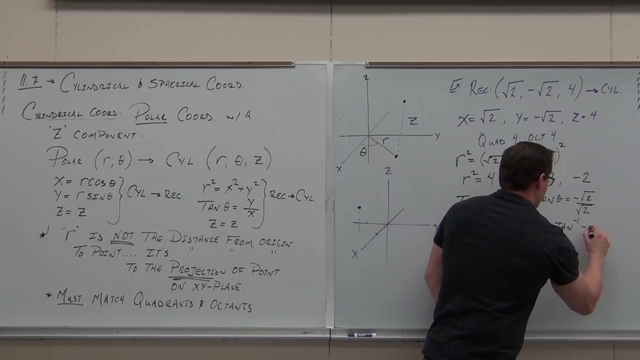 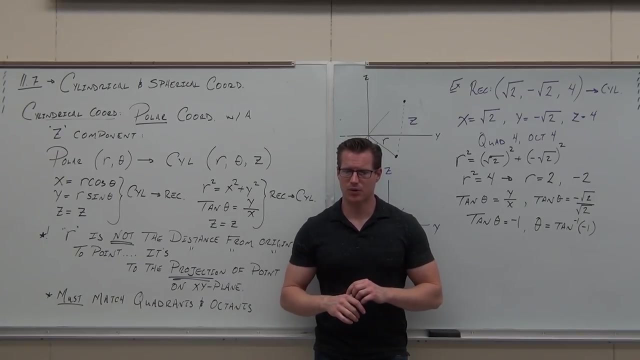 Negative: 1. From there, fine, you can do it from there. Or if you want to do the theta, how do you find theta From right here? come on, Can you tell me right now, and here's the deal, when we talked about polar, when you first did it? 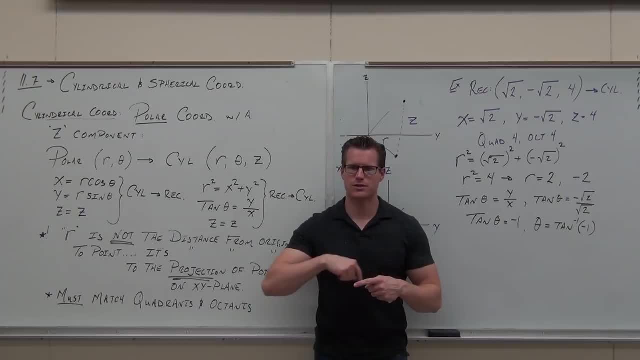 theta can go from 0 all the way to pi over 2.. It has to be negative. It has to be negative, It has the whole range there. So can you give me two values of theta for which tangent is negative 1?? 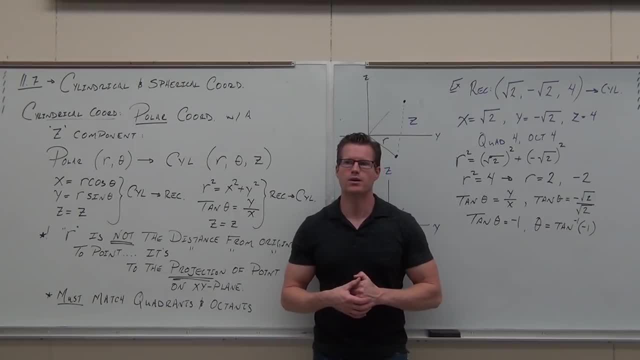 Or in other words tan inverse of negative 1, you're going to have two values there. We don't restrict it to that negative pi over 2 to pi over 2. We can go outside of that because we're on that plane. 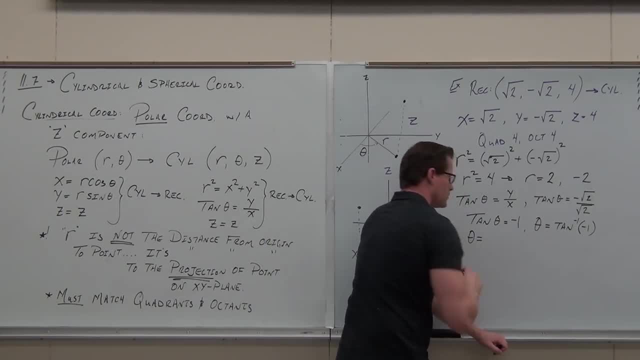 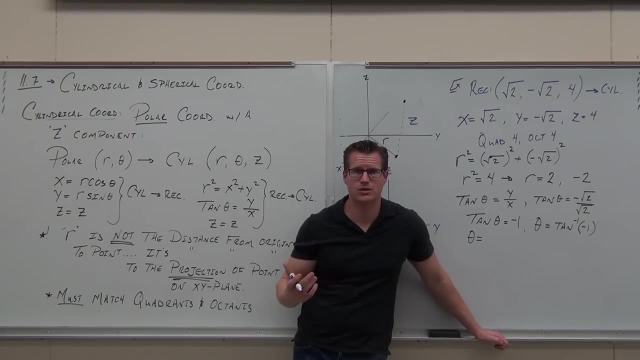 So how much is theta? Cosine and sine have the same values, but one's negative. Come on, that's quadrant 2 or quadrant 4. 4. Are you with me on this? Yes, What is it? 3 pi over 4.. 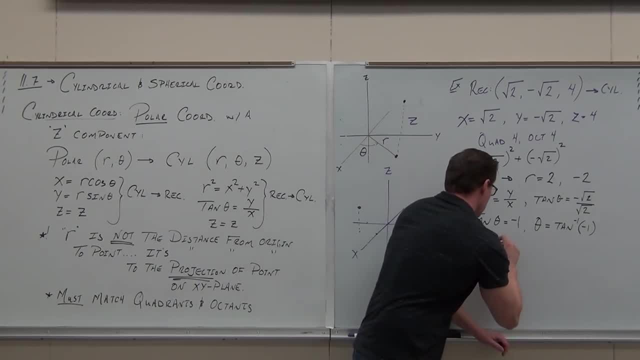 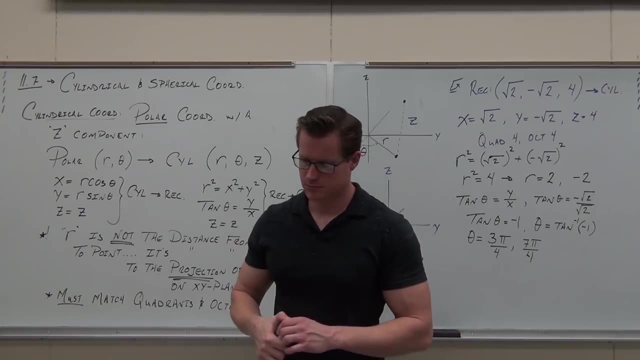 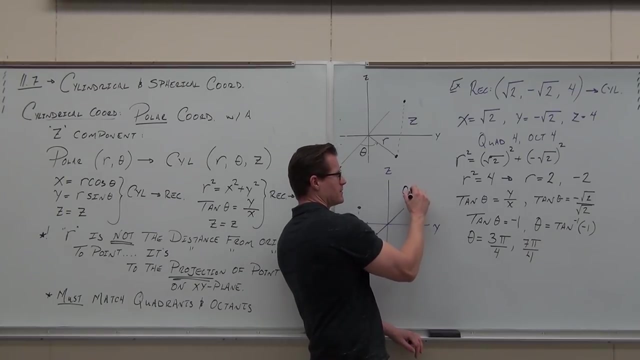 3 pi over 4 or 7 pi over 4.. Head and neck, you're okay with that one. So again, if you want a little side note, keep in mind that theta goes from 0 to 2 pi. 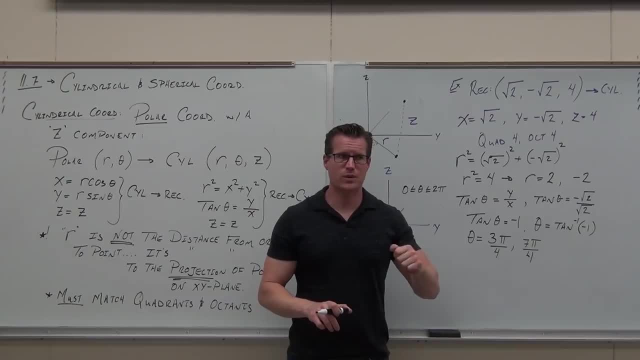 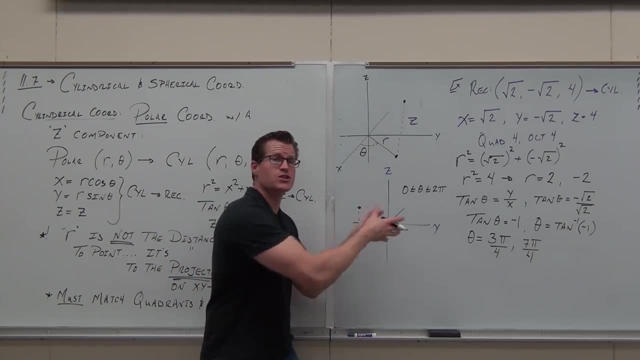 It is the entire. It's the entire, It's the entire plane. So we have these, We have two. No, no wait. This is cool If you didn't understand anything before about why we even did this. this is why we do this. 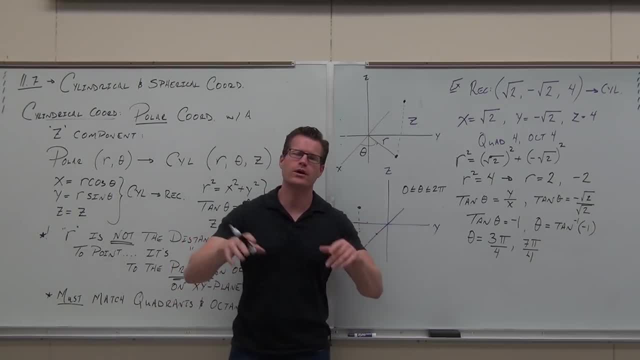 What quadrant? I know we talked about quadrants. It's like why We're in 3D. What quadrant were we in? 4. Quadrant, Which one of these is in quadrant 4?? Pick that one. Pick the one in the correct quadrant, okay. 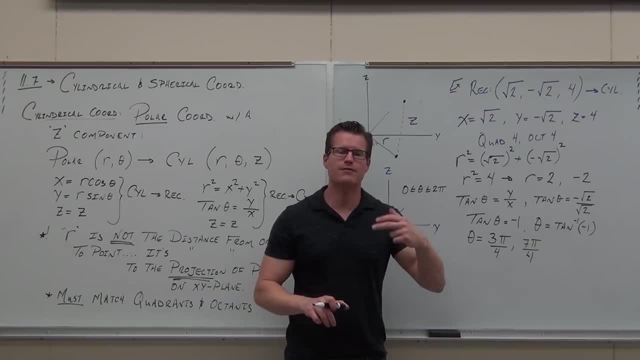 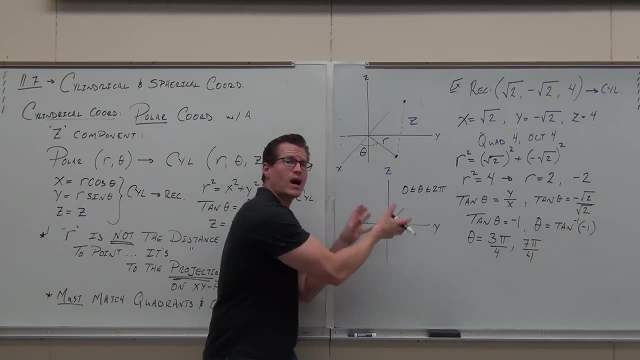 It is the entire plane, So we have 2 pi. No wait, This is cool. If you didn't understand anything before about why we even did this, this is why we do this. What quadrant? I know we talked about quadrants. 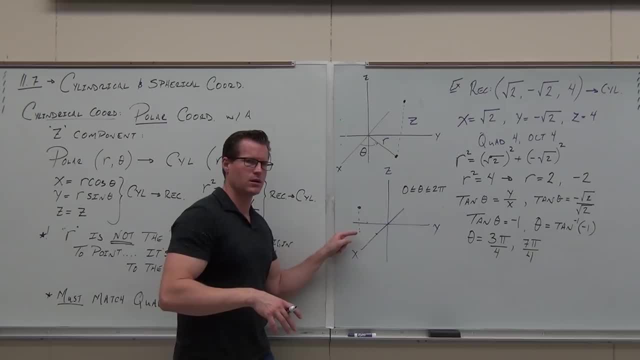 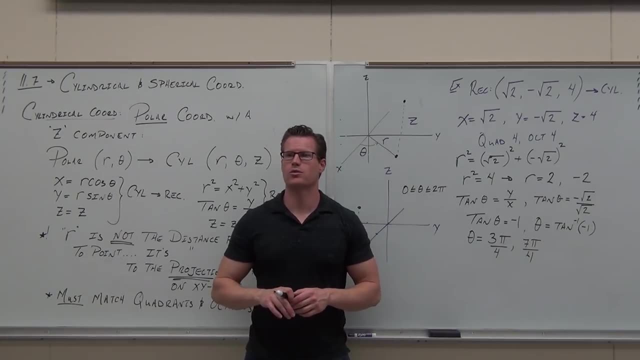 Like why We're in 3D? What quadrant were we in Quadrant? Which one of these is in quadrant 4?? Pick that one. Pick the one in the correct quadrant. okay, My bad, My bad. Pick the one in the correct. 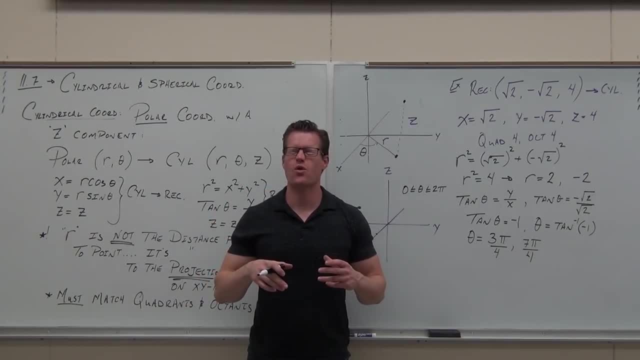 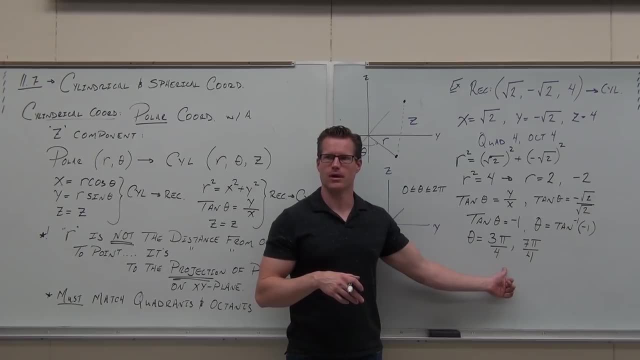 Dang it, It's really hard- In the correct quadrant. This is not in quadrant 4.. This is in quadrant 2.. We're going to talk about that one. We're going to talk about it in a little bit. So yeah, there's two of them, but only one is in the proper quadrant. 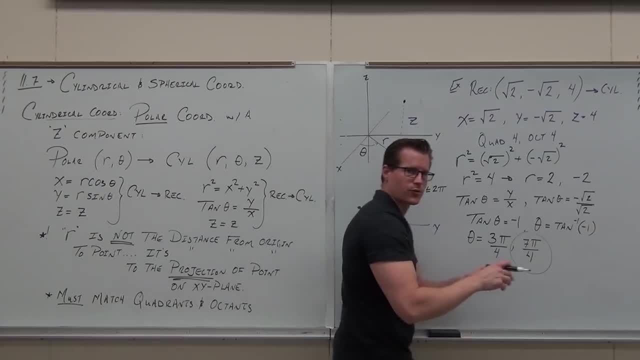 This is in quadrant 4, where our point is is in quadrant 4, on the xy plane. Do you guys see the dilemma that we have here? going from rectangular to cylindrical? We have these two. We've got these two angles Pretty much all the time. 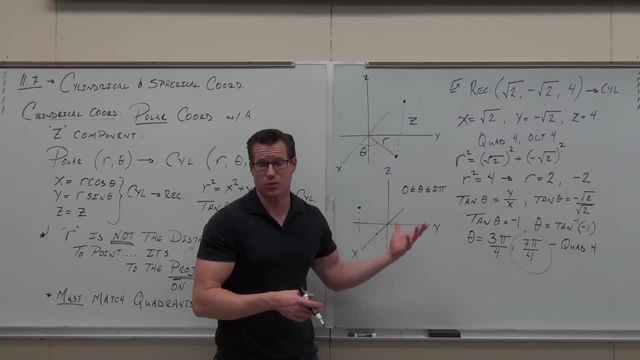 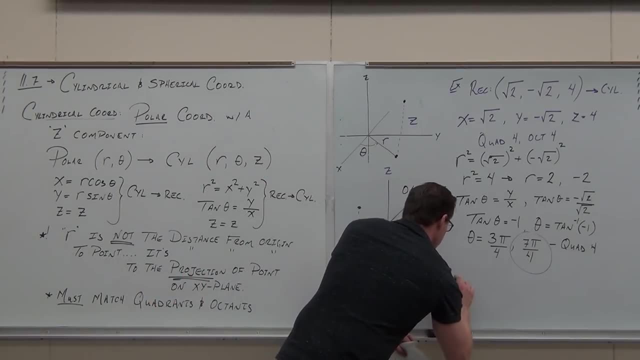 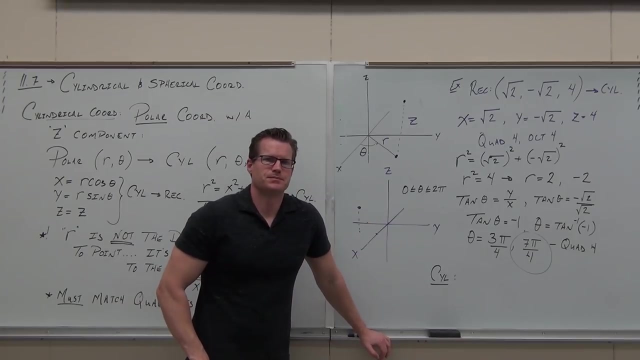 Match the correct quadrant to the correct quadrant. That's what we want to do here. So what's the cylindrical coordinates for that point? What do you think? Well, let's see, I want to be out here, whatever the r is too. 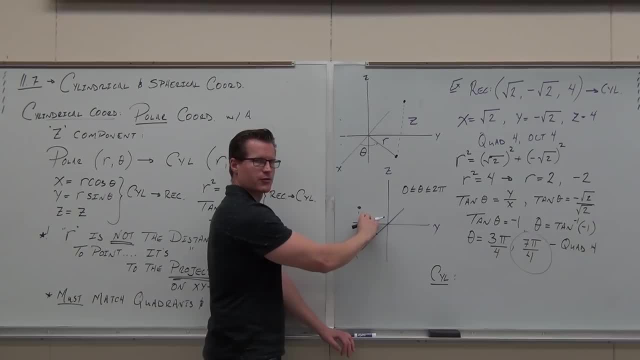 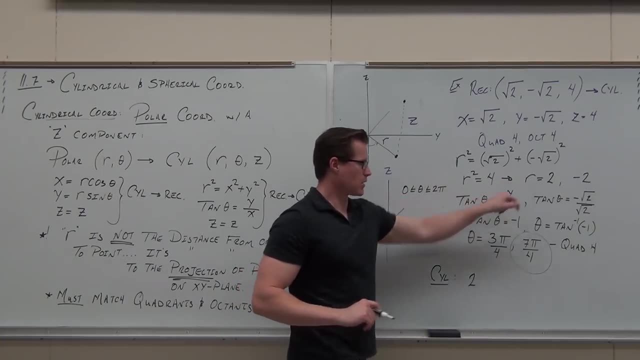 I want to be going All the way around 7 pi over 4, and I want to go up 4.. So we have an r of 2.. We got it. r of 2. What puts us in quadrant 4, everybody. 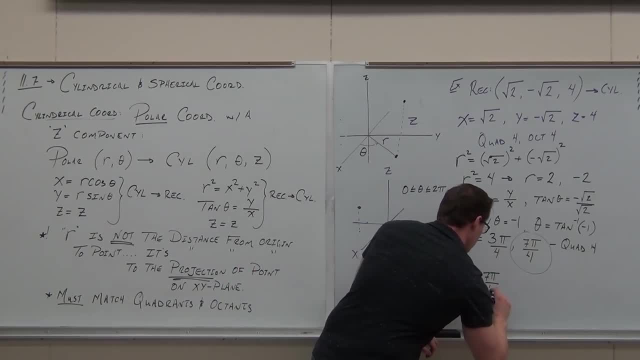 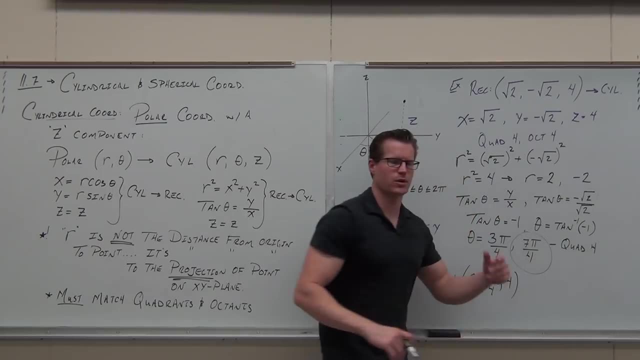 What does that look like And what puts us at the appropriate height? Oh yeah, z is z, So what is it 4. Now I know there's a question hanging out there somewhere. What's? the question 2 is positive. 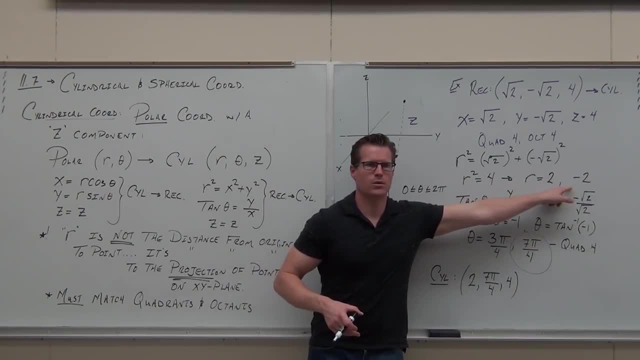 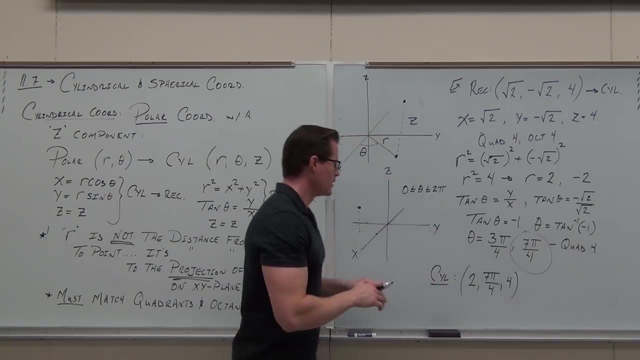 What's the question? What about that one? What's that do? I want you to understand that that's a valid answer, and so is this one, Please, please listen. If we went to 3, please watch. If we went to 3, pi over 4, we would be right there. 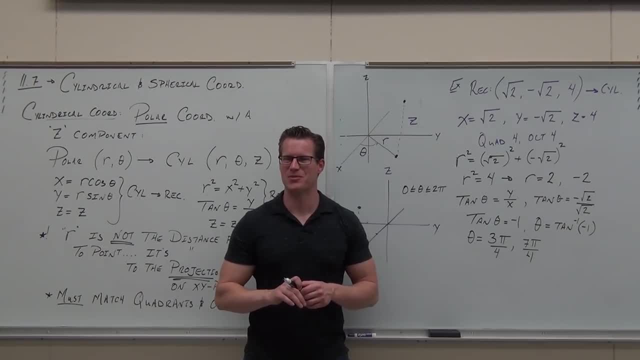 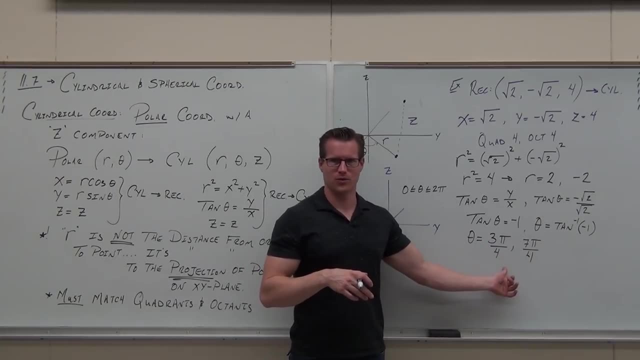 My bad, My bad. Pick the one in the Dang it It's really hard- In the correct quadrant. This is not in quadrant 4.. This is in quadrant. We're going to talk about that one. We're going to talk about it in a little bit. 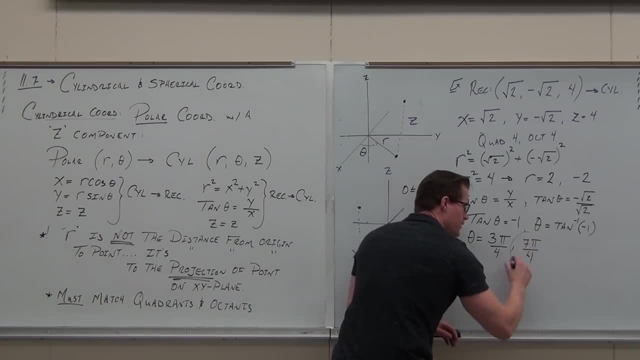 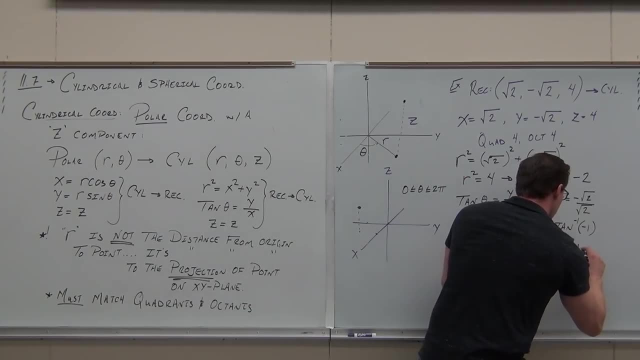 So, yeah, there's two of them, but only one is in the proper quadrant. This is in quadrant 4, where our point is is in quadrant 4, on the XY plane. Do you guys see the dilemma that we have here, going from rectangular to cylindrical? 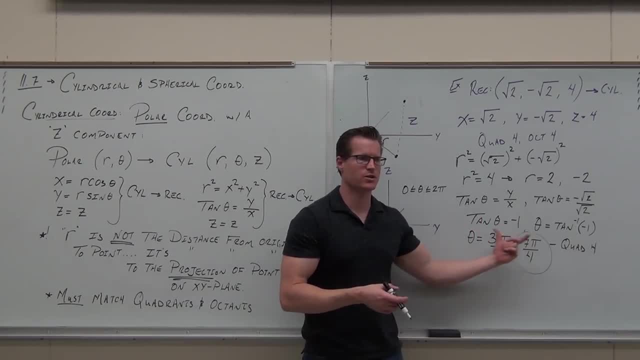 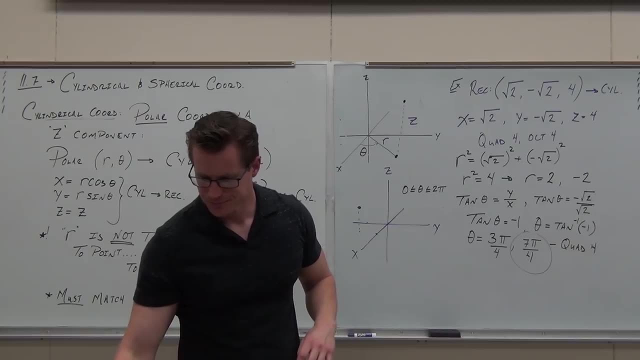 No, We don't have these two. We've got these two angles pretty much all the time. Match the correct quadrant to the correct quadrant. That's what we want to do here. So what's the cylindrical, What's the cylindrical coordinates? for that point. 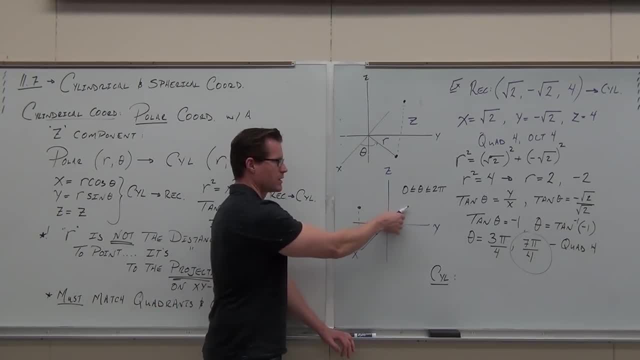 What do you think? Well, let's see, I want to be out here, Whatever the R is 2.. I want to be going all the way around 7 pi over 4, and I want to go up 4.. 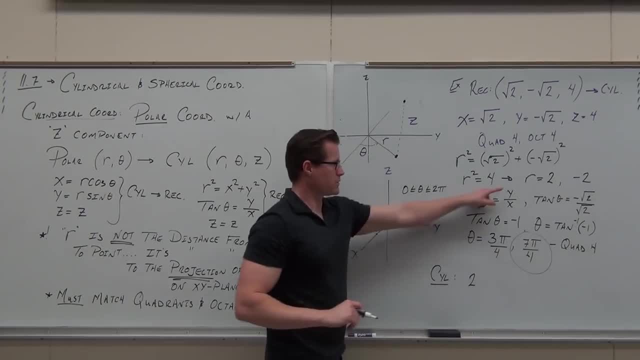 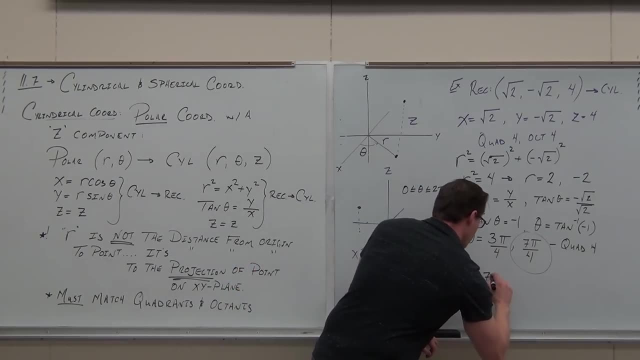 So we have an R of 2.. We got it, R of 2.. What puts us in quadrant 4, everybody? What does that mean? And what puts us at the appropriate height? Oh yeah, Z is Z. 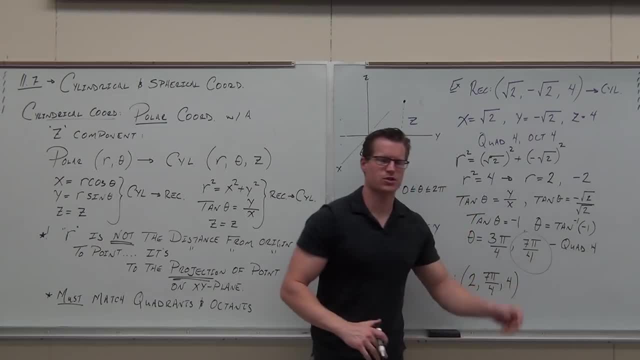 So what is it? Now, I know there's a question hanging out there somewhere. What's the question? 2 is odd. What's the question? What about that one? What's that do? I want you to understand that that's a valid answer, and so is this one. 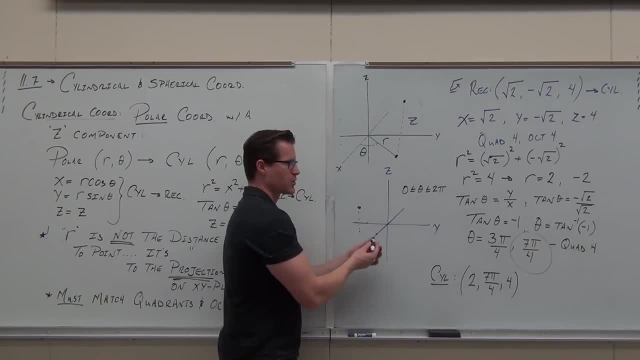 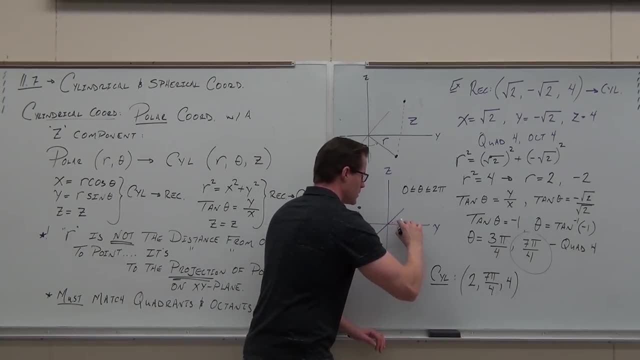 Please, please listen. If we went to 3.. Please watch. If we went to 3 pi over 4, we would be right there. Do you guys see it? 3 pi over 4.. If we went out a radius of negative 2.. 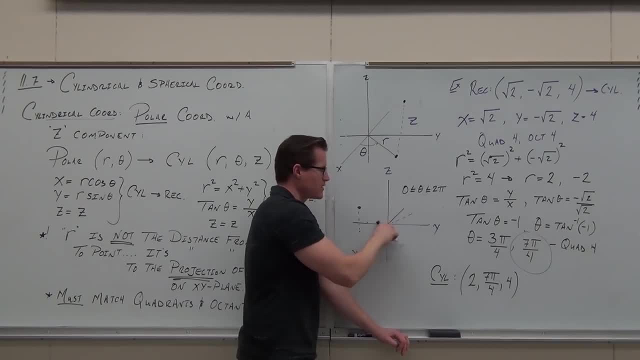 Do you remember what radiuses of negative 2 do with polar? They go: yeah, Here's your angle, but then you reflect it 180 degrees or pi. That puts you back in the correct quadrant. So here's the whole big shebang. 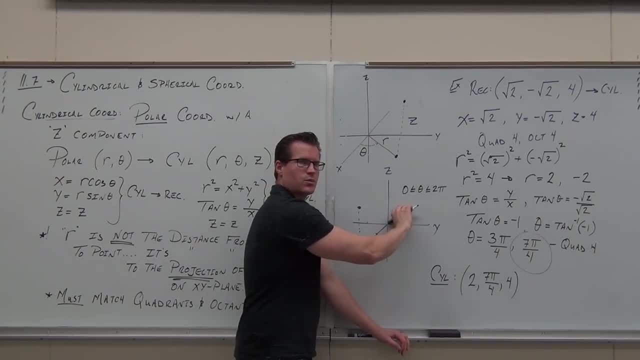 Do you guys see it? 3 pi over 4.. If we went out a radius of negative 2, do you remember what radiuses of negative 2 do with polar? They go. yeah, here's your angle, but then you reflect it. 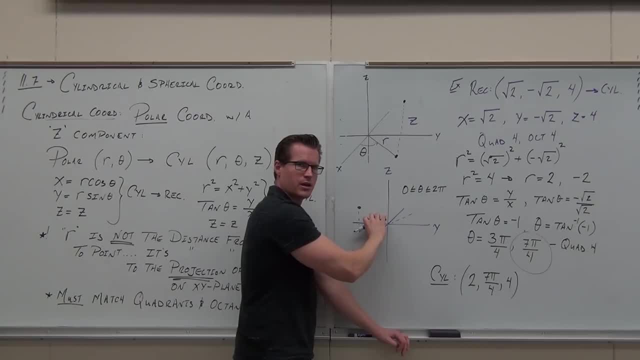 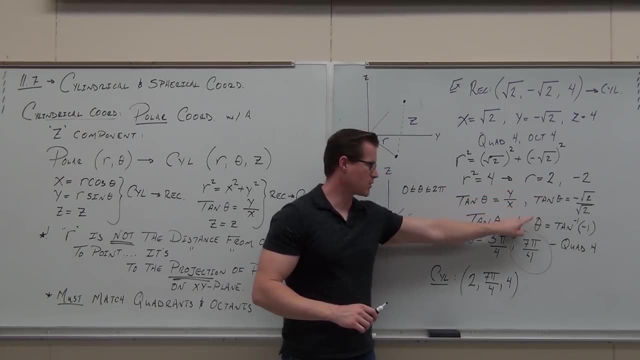 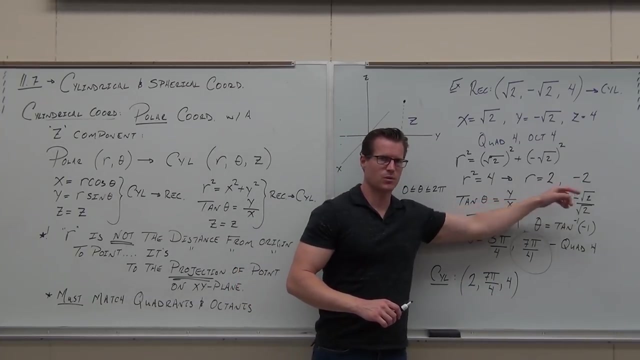 densities of zero certification degrees or pi. That puts you back in the correct quadrant. so here's the whole big shebang. Match up the positive radius with the correct quadrant. Gives you a correct interpretation. Match up the negative radius with the opposite quadrant. 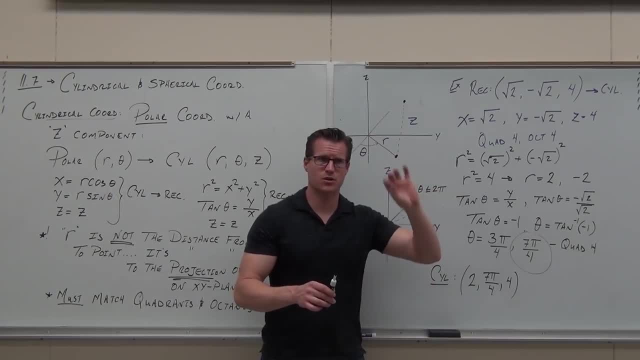 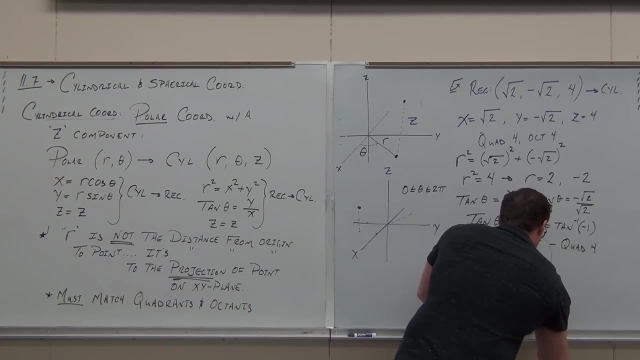 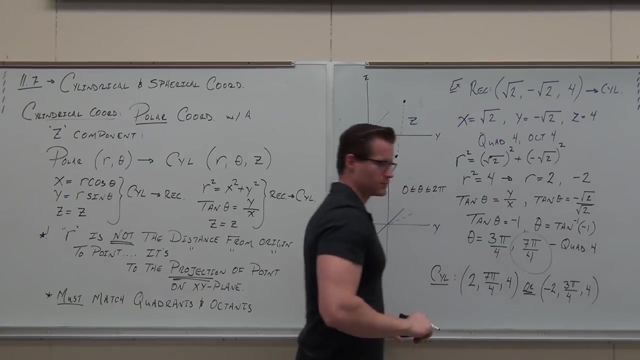 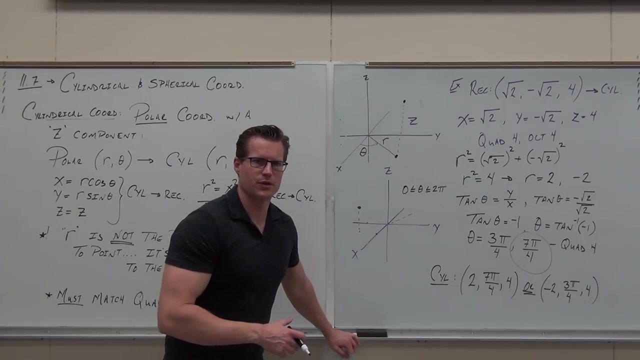 And it also gives you a correct interpretation. You should know which one. to match up. Positive radius: click, click, Boom. I'll put your huge note down there. for this one, Use the positive radius with the theta. that is in the proper one. 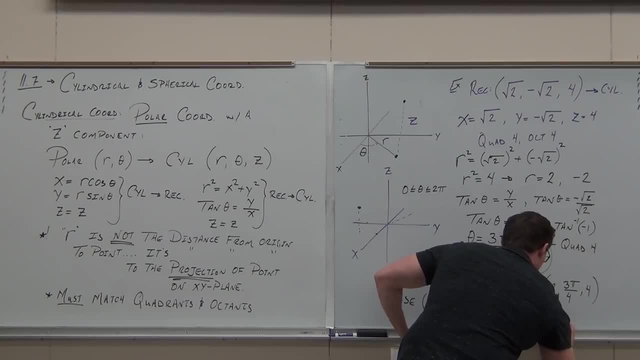 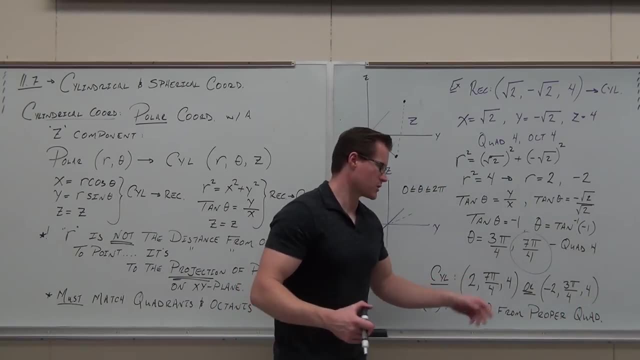 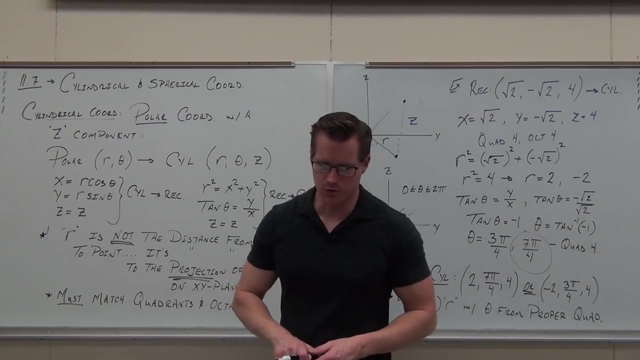 That also. obviously the corollary is: use the negative radius with the theta from the other quadrant, the non-proper quadrant, and it works out for you. I really, really want to know if I've made this make sense to you. 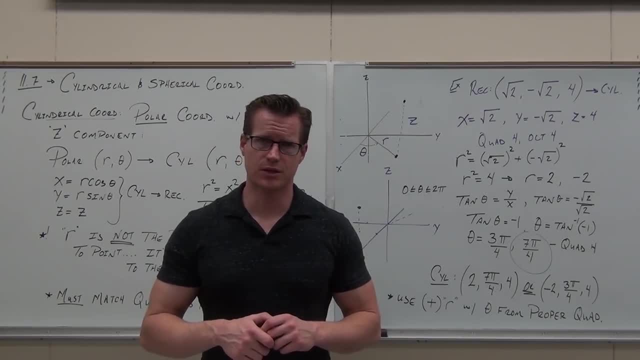 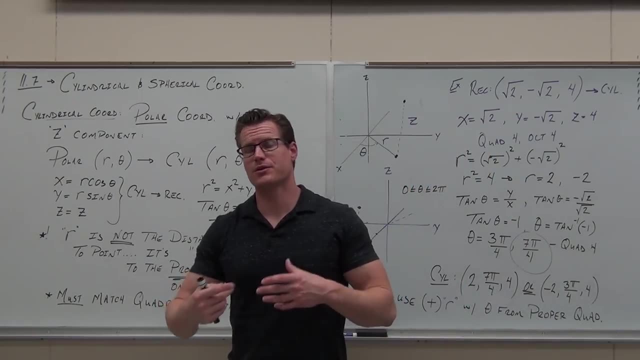 If I give you on a test- hey, let's go from rectangular to cylindrical- can you do it? That one's Not too bad. You've got to watch out for your thetas. If I say go from cylindrical to rectangular, can you do it? 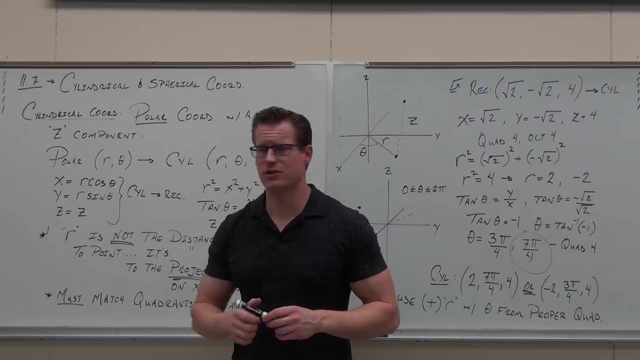 That one's really easy. It almost never fails. You just plug the numbers in. You're pretty good Show of hands, if you feel okay with that one. One more little side note: This is pretty cool because you can do tan inverse of negative 1.. 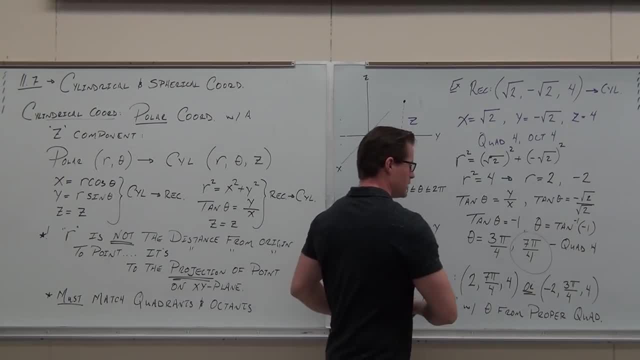 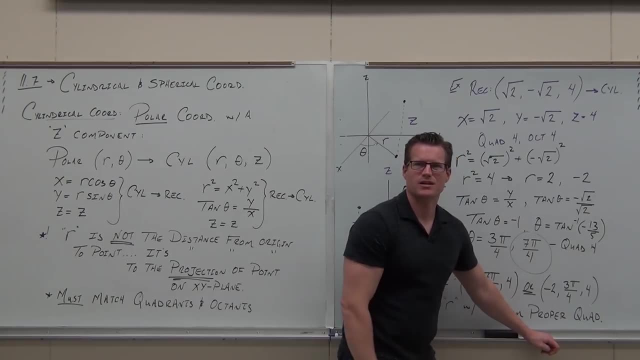 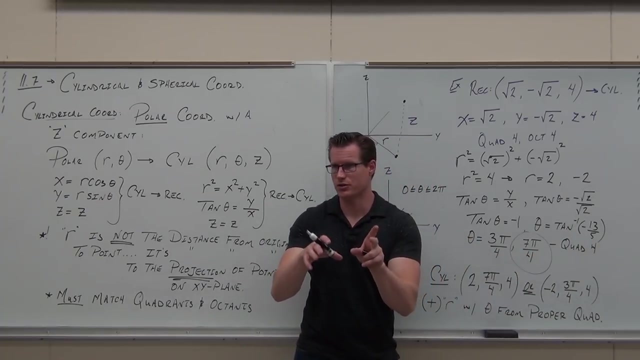 Listen, if you ever get down to here and you go, hey, tan inverse of negative 13 fifths, just leave it please. Then this goes right here. That's still an angle. But you put tan inverse of nasty thing that's not on your unit circle. it goes right there, okay. 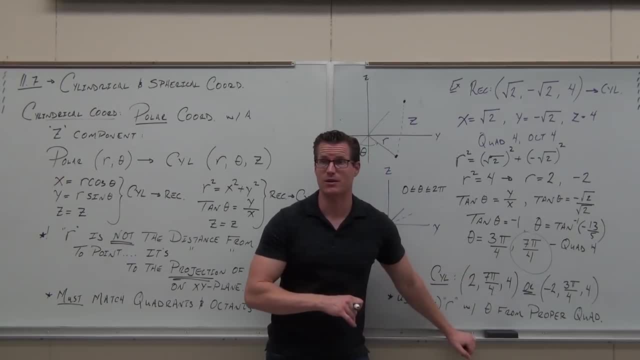 Don't approximate it, Don't decimal it, Just put tan inverse of nasty thing that you can't find Make sense. But if you can find it on your unit circle, for heaven's sakes you need to put it down correctly. 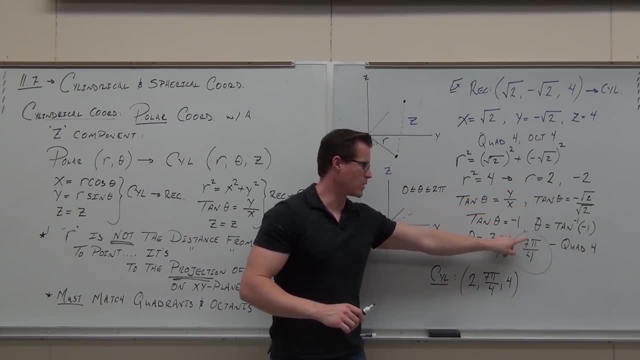 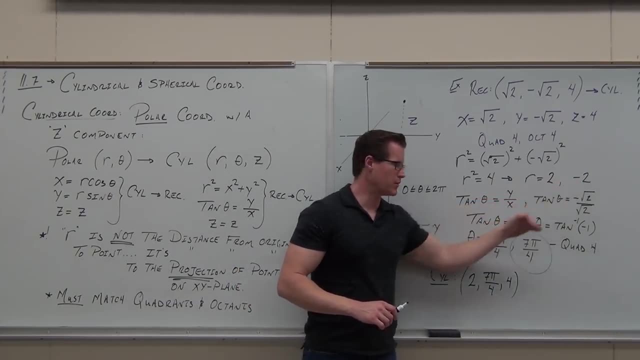 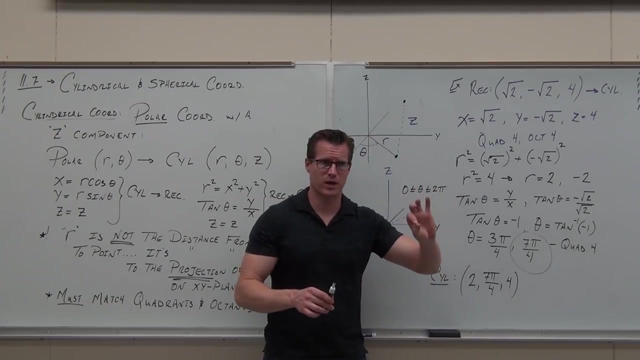 Match up the positive radius with the correct quadrant Gives you a correct interpretation. Match up the negative radius with the opposite quadrant, and it also gives you a correct interpretation. You just need to know which one to match up. Positive radius, correct. 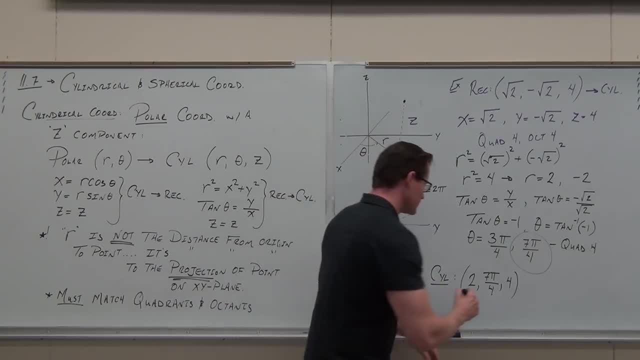 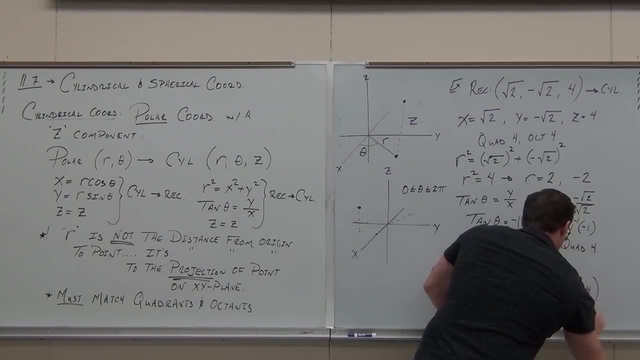 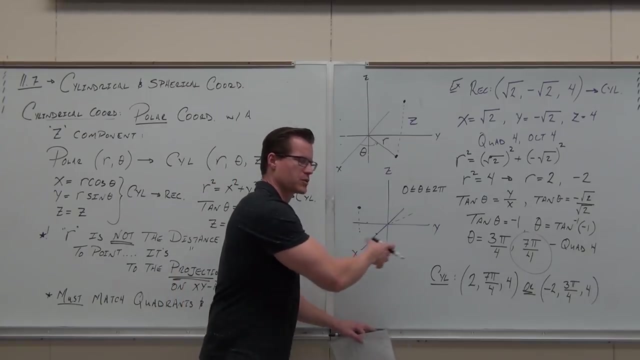 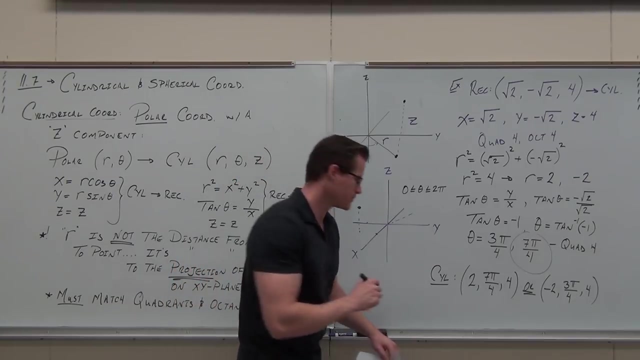 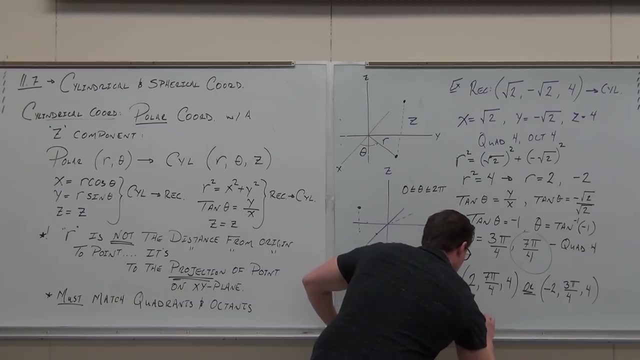 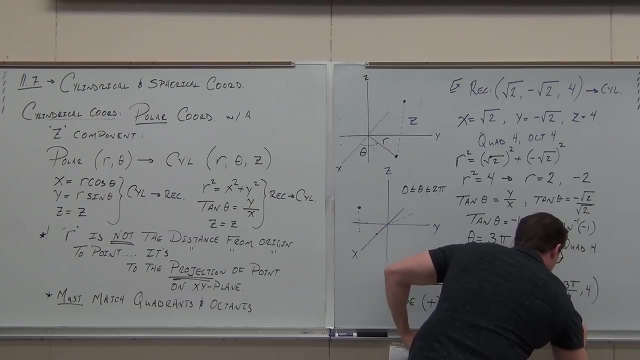 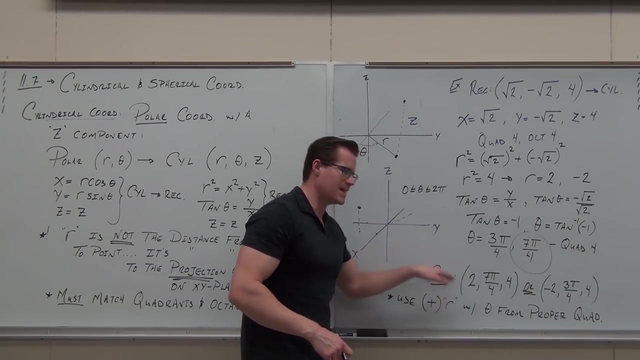 Boom, Boom. I'll put your huge note down there. for this one: Use the positive radius with the theta that is in the proper quadrant. Boom, That also. obviously the corollary is: use the negative radius with the theta from the other quadrant. 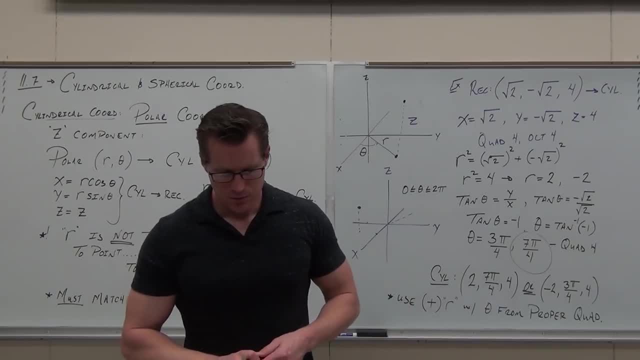 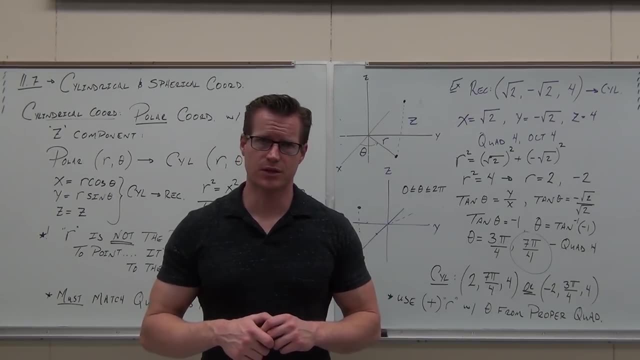 the non-proper quadrant and it works out for you. I really, really want to know if I've made this make sense to you. If I give you on a test, hey, let's go from rectangular to cylindrical, Can you do it? 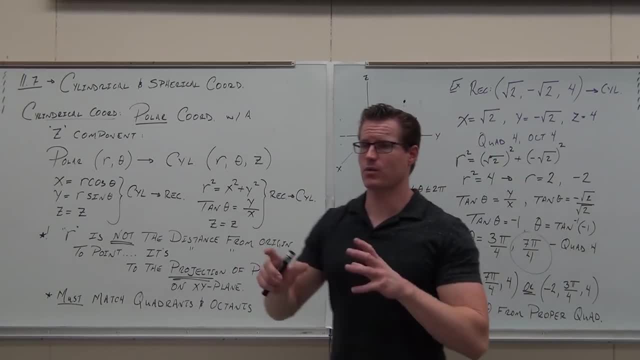 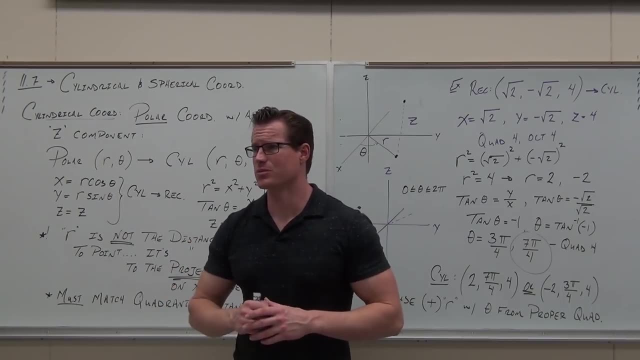 Yes, That one's not too bad. You've got to watch out for your thetas. If I say go from cylindrical to rectangular, can you do it? That one's really easy. It almost never fails. You just plug in the numbers and you're pretty good. 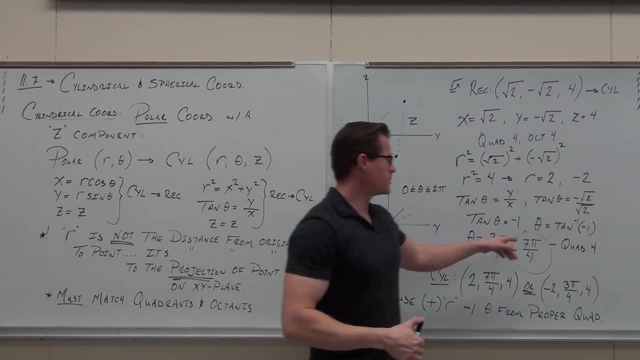 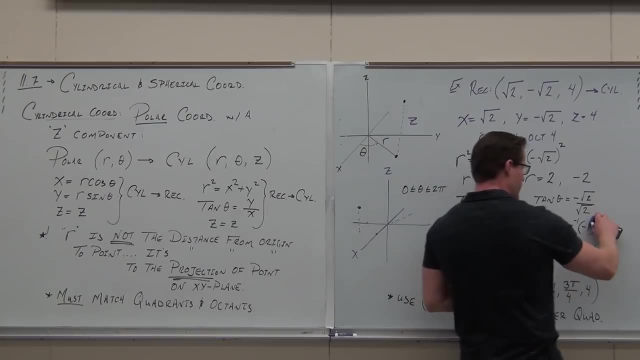 Show of hands if you feel okay with that one. One more little side note. This is pretty cool because you can do tan inverse of negative 1.. Listen, if you ever get down to here and you go, hey, tan inverse of negative 13. fifths, just leave it please. 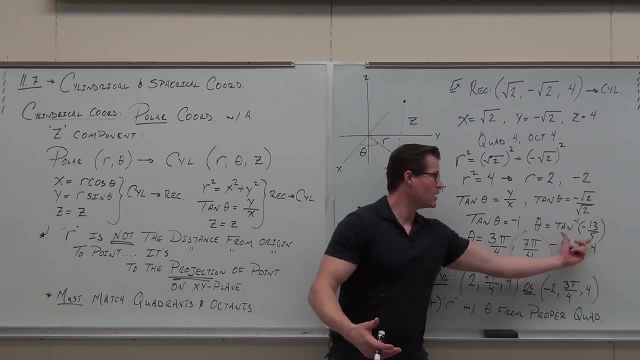 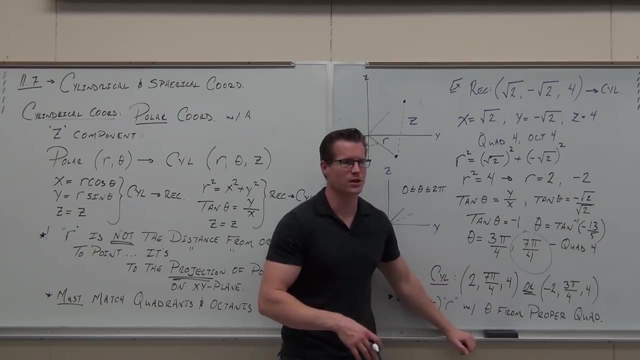 Then this: This goes right here. That's still an angle. but you put tan inverse of nasty thing that's not on your unit circle. it goes right there. okay, Don't approximate it, Don't decimal it, Just put tan inverse of nasty thing that you can't find. 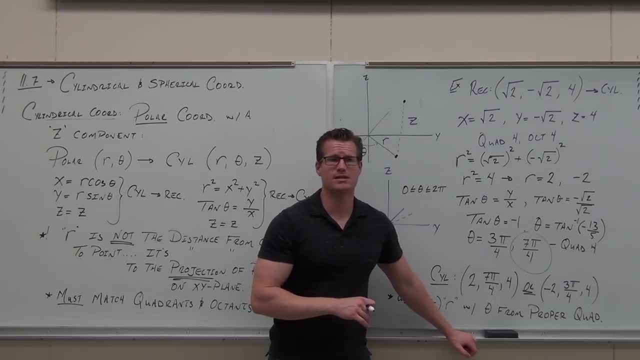 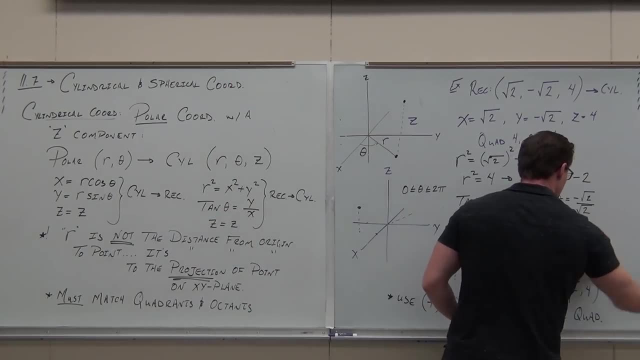 Make sense. But if you can find it on your unit circle, for heaven's sakes you need to put it down directly. Okay, Show of hands if you feel okay with that one, Okay, So kick back and then we're good to go. 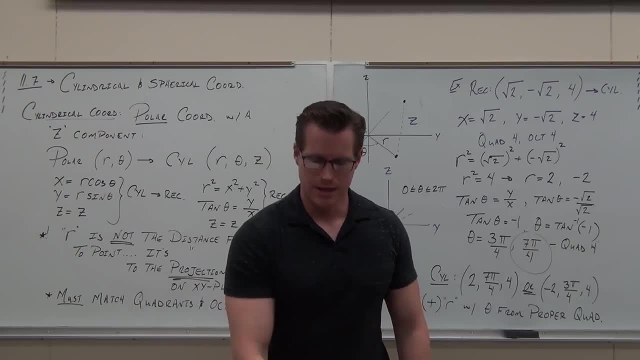 That's literally it. That's literally it for cylindrical. What we're going to do right now is we're going to talk Easy. I told you it's about the easiest thing. You're probably going to get bored. I'll make it harder. 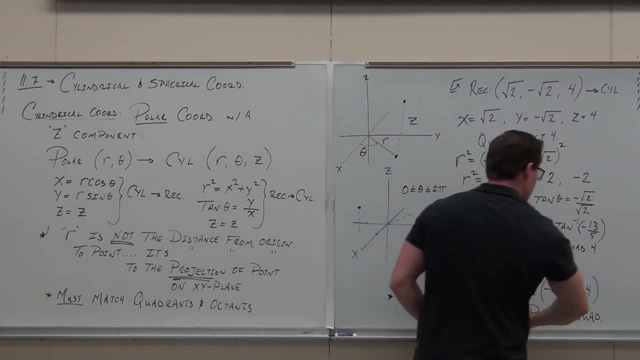 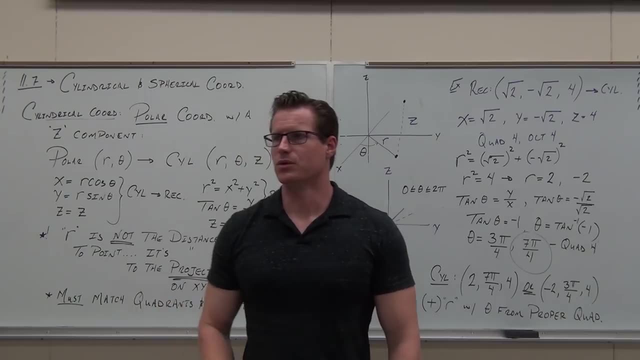 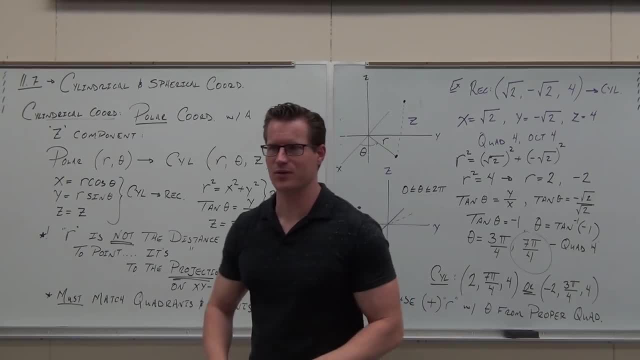 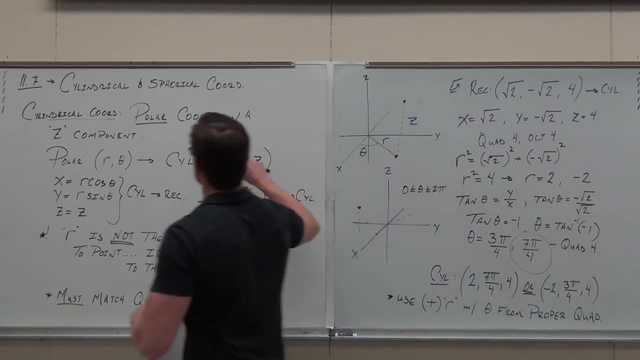 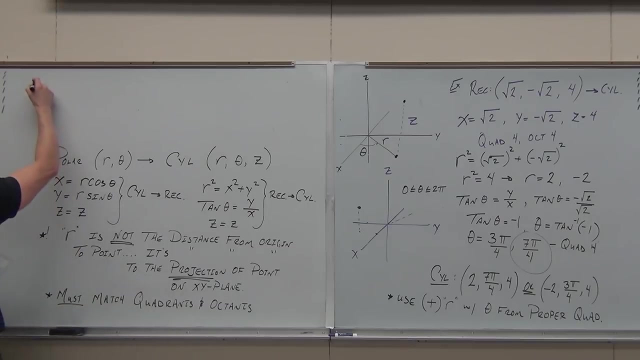 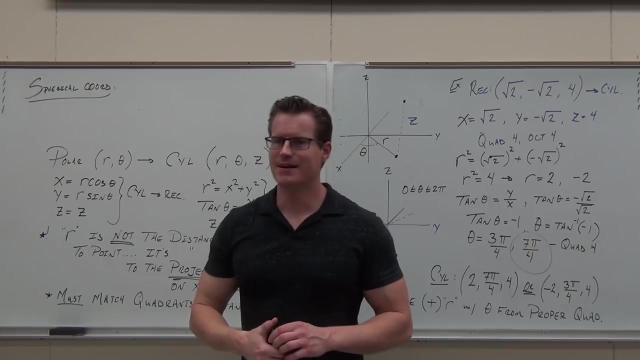 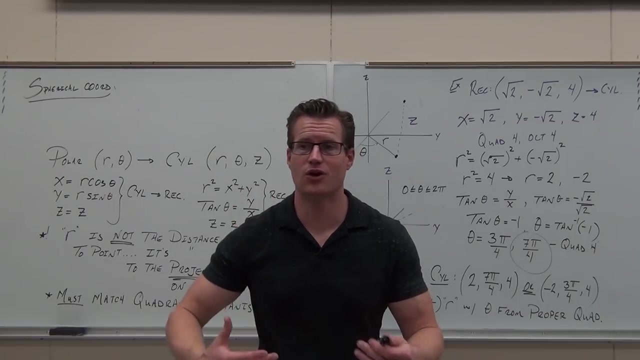 I told you it's not the easiest thing. You're probably getting bored. I'll make it harder. All right, We'll talk about spherical. It's not hard, It's the same stuff. We're going to talk about spherical. Spherical does does use the distance from the origin to the point and it defines it not as r. 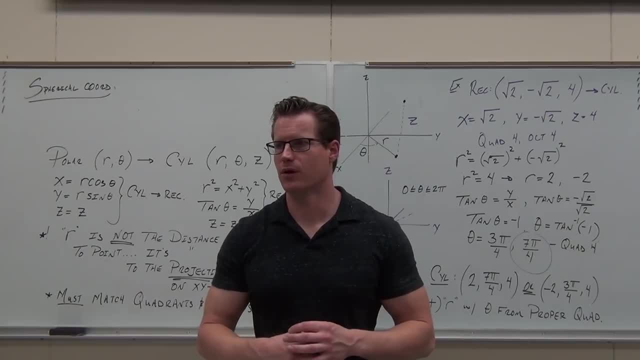 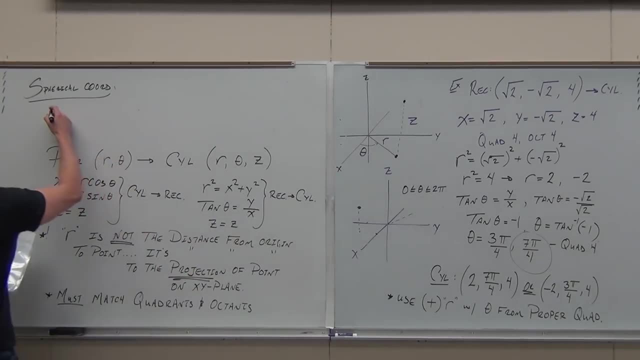 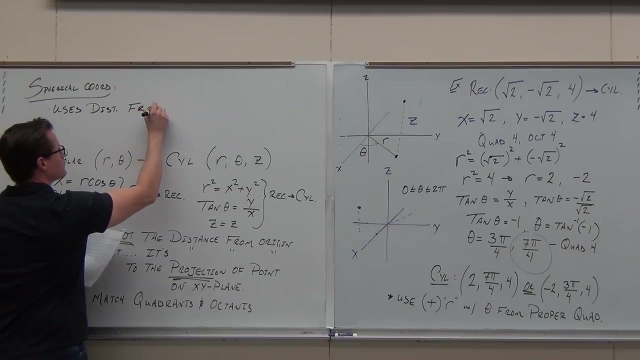 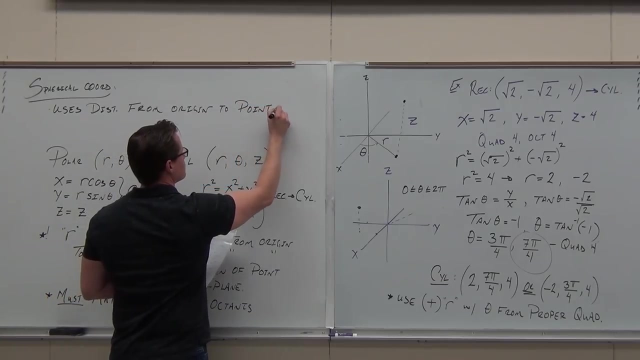 because that's not what that means. It defines it as a thing called rho, That's Greek for r, So it talks about radius, So it uses the distance from the origin to the point. I don't write very good rho's, but that's about what rho looks like, like that. 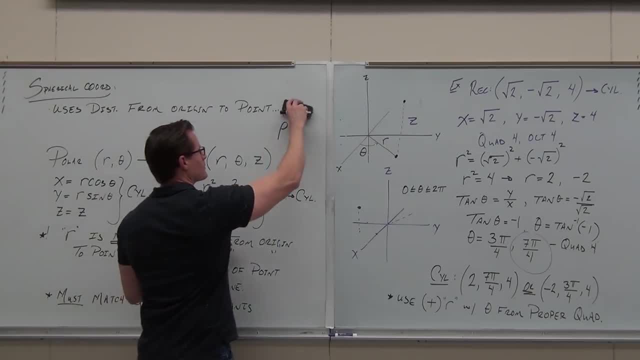 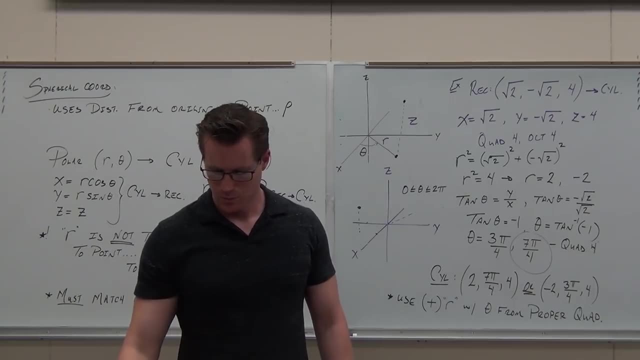 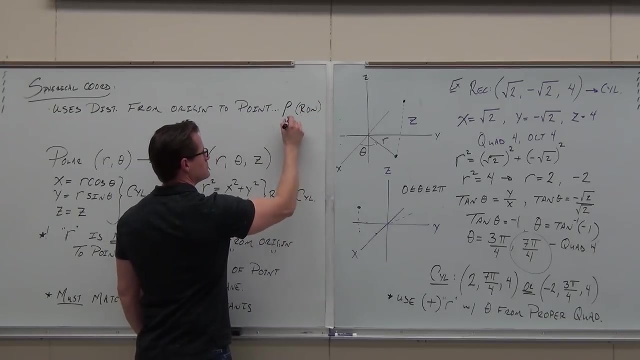 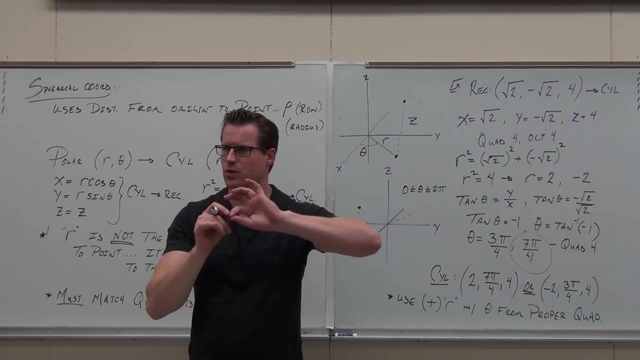 That's a. that's a better one. That's a lowercase Greek letter: rho, Think radius. think radius like it would be on a sphere. Radius goes from the origin to a point on a ball, and that's what. that's what this is doing. 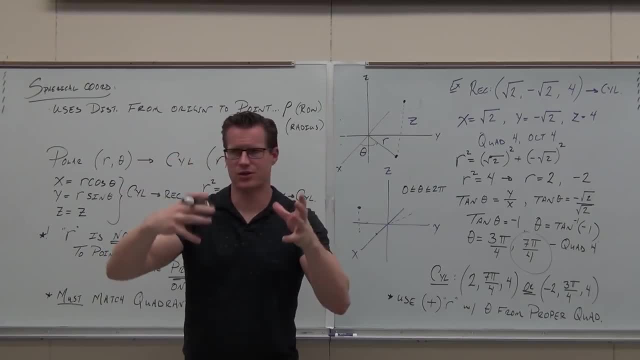 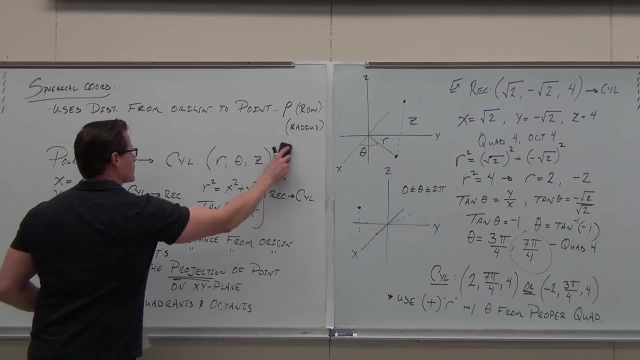 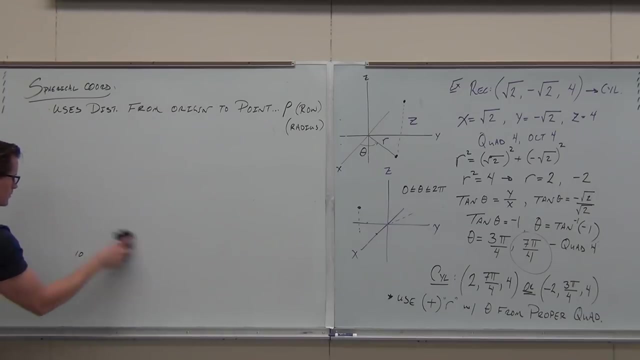 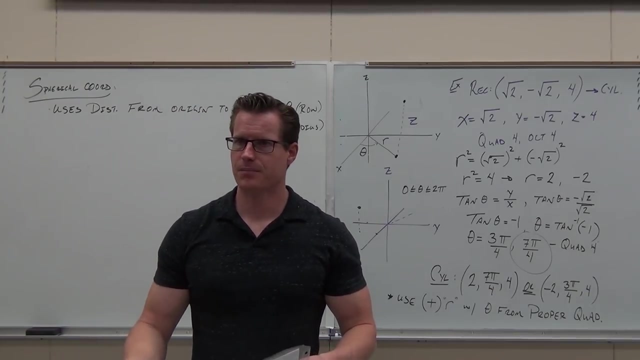 It's going out from the origin to some place on an imaginary ball like a unit ball, but it doesn't have to be a unit. Now, some other cool things. it uses theta. The theta is used in spherical, just like it's used in cylindrical. 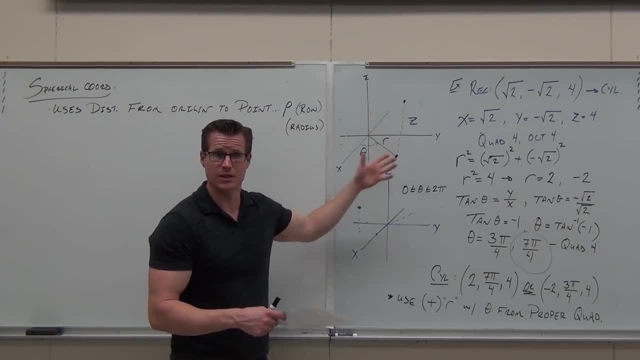 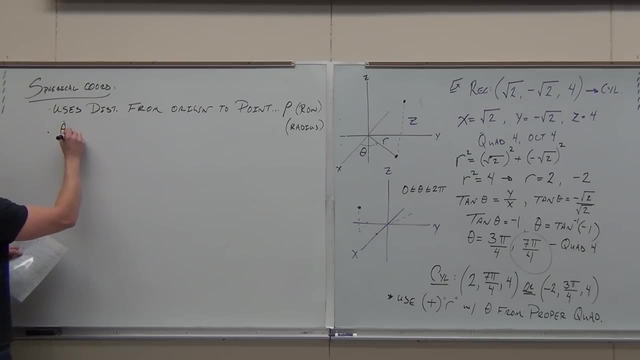 It's still going to be this distance to the projection, that point, That that's what this is is So it uses distance, Uses theta, just like cylindrical, but then it has this other, this other thing that we're going to talk about. 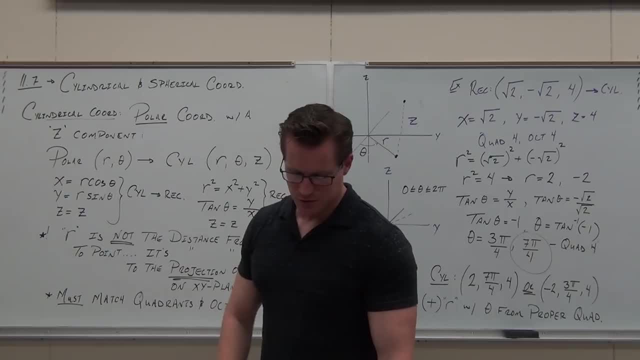 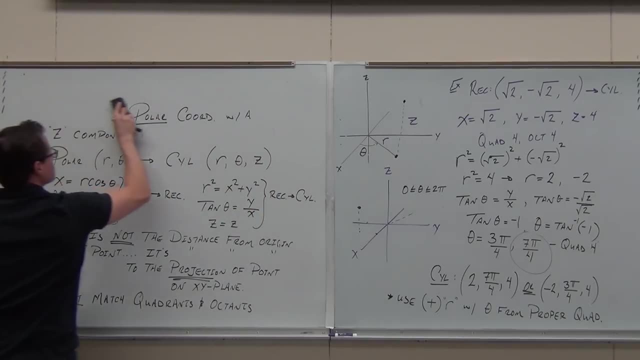 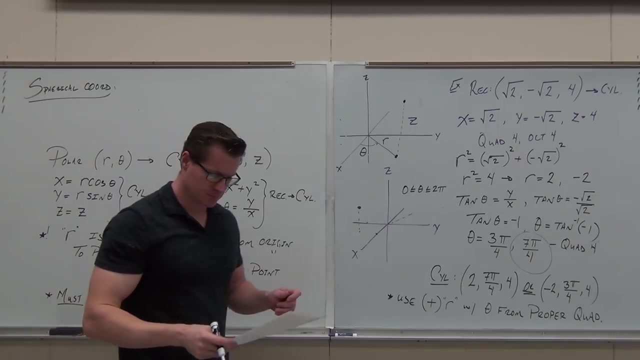 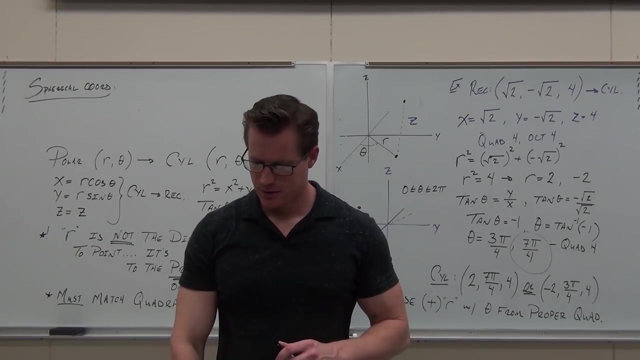 All right, We'll talk about spherical. It's not hard, It's the same stuff. We're going to talk about spherical. Spherical does does use the distance from the origin to the point and it defines it not as R. 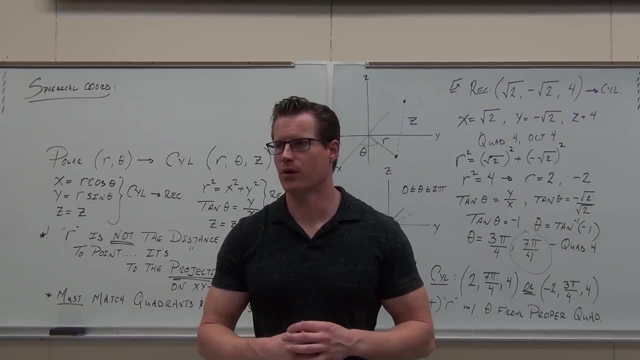 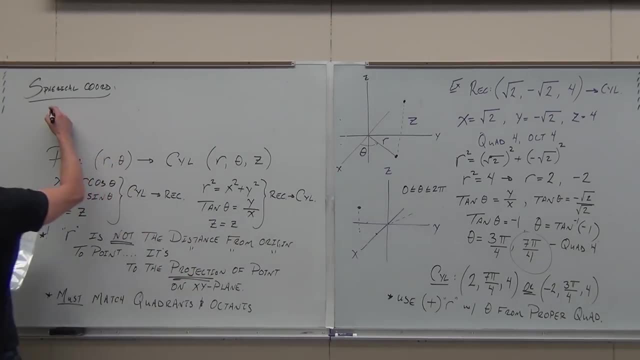 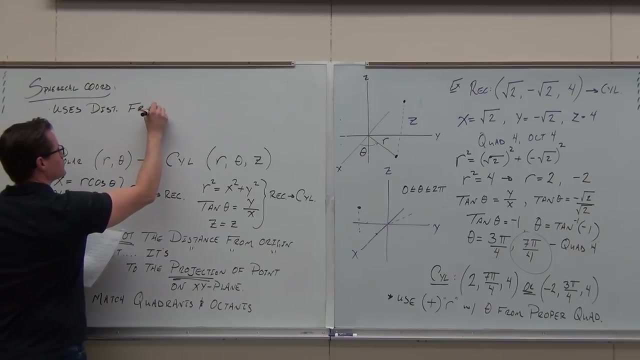 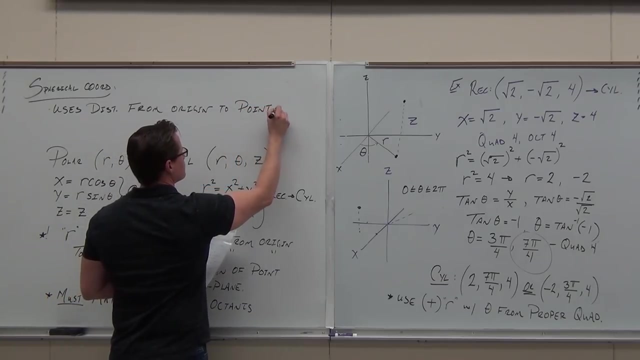 because that's not what that means. It defines it as a thing called rho, That's Greek for R, So it talks about radius, So it uses the distance from the origin to the point. I don't write very good Rho's, but that's about what Rho looks like. 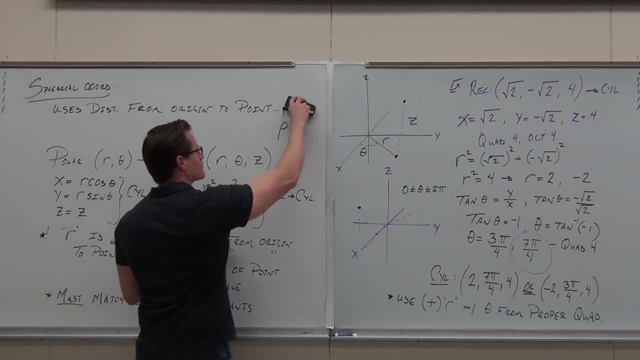 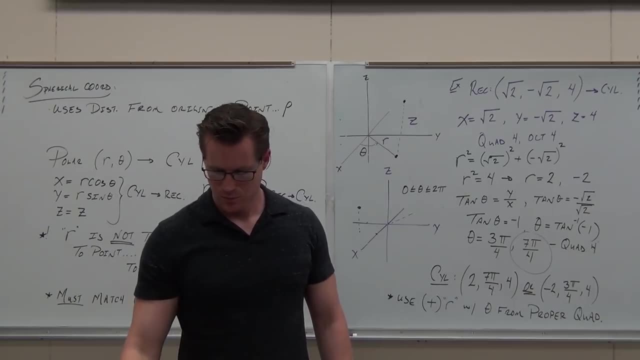 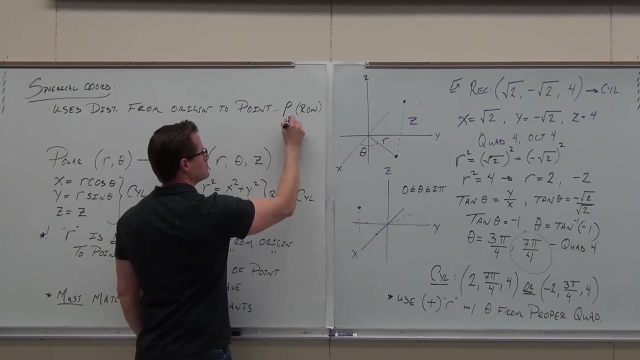 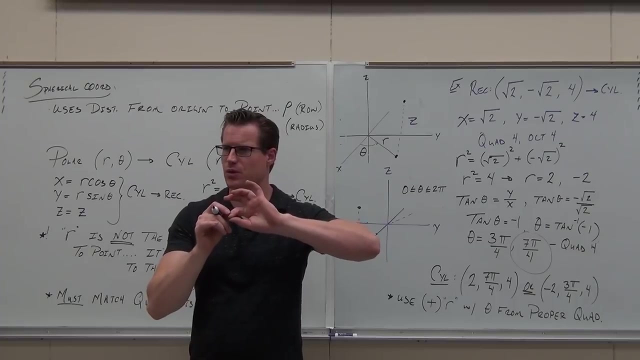 That's a better one. That's a lowercase Greek letter: Rho, Think radius, Think radius, like it would be on a sphere. Radius goes from the origin to a point on a ball, and that's what. that's what this is doing. 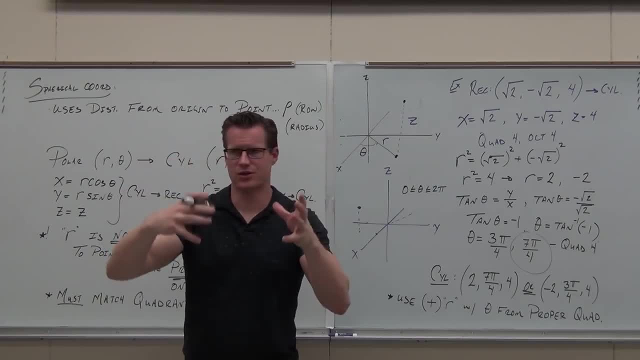 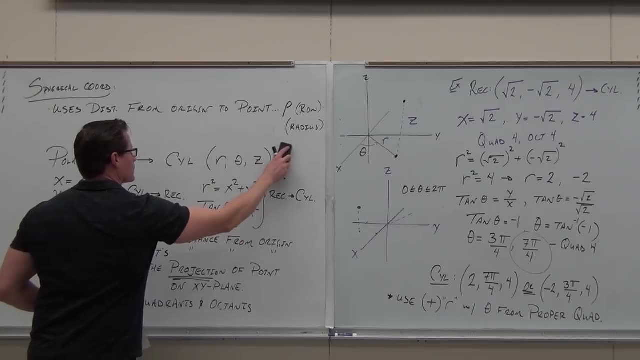 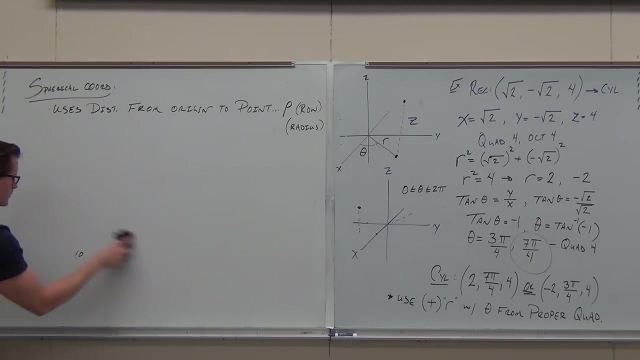 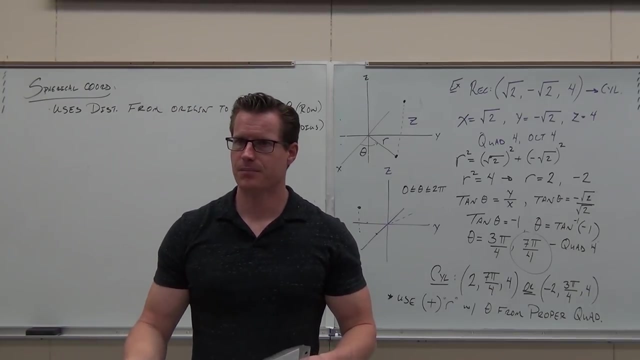 It's going out from the origin to some place on an imaginary ball, like a unit ball, but it doesn't have to be U Now some other cool things. it uses theta. The theta is used in spherical, just like it's used in cylindrical. 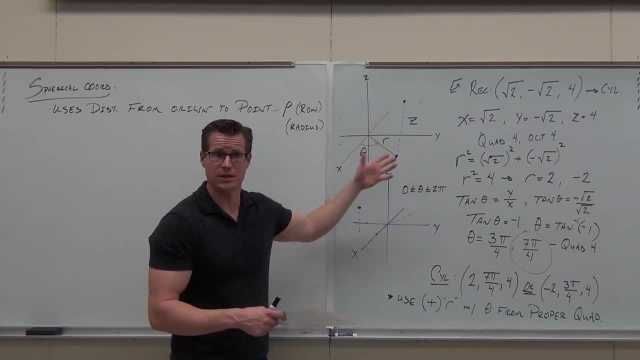 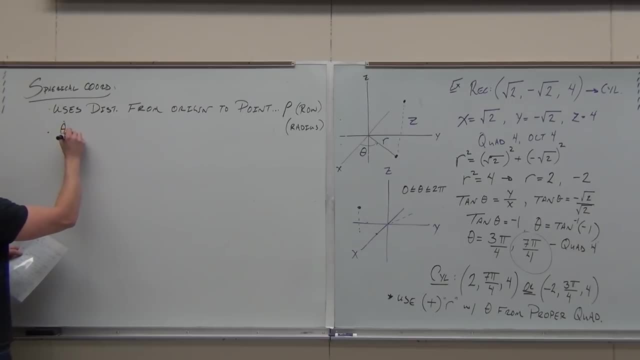 It's still going to be this distance to the projection, that point, That that's what this is is. So it uses distance, Uses theta, just like cylindrical, But then it has this other, this other angle, and we call it phi. 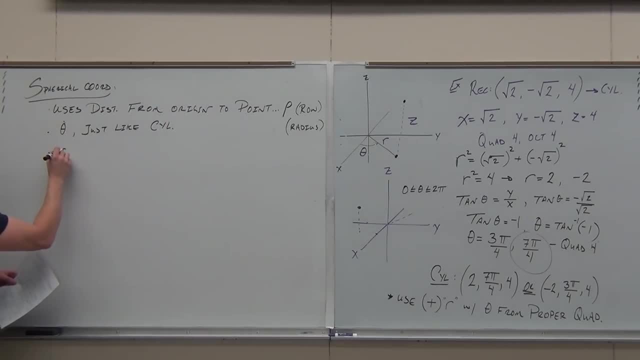 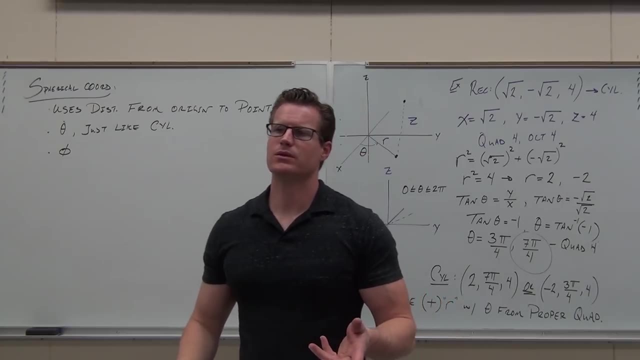 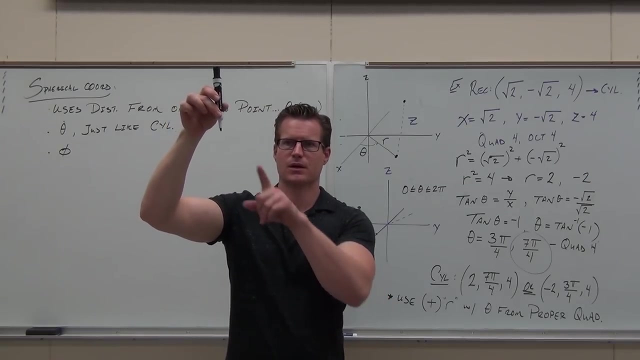 This other angle and we call it phi. So this angle, phi. what this angle does. this angle is from the positive, positive z-axis to where that radius, that rho is. It's the angle from positive z to where the, the, the segment that would connect the origin. 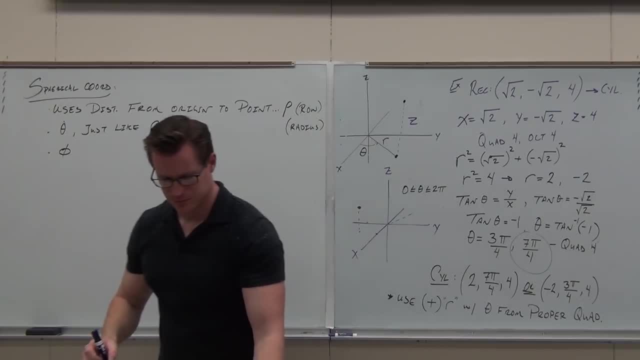 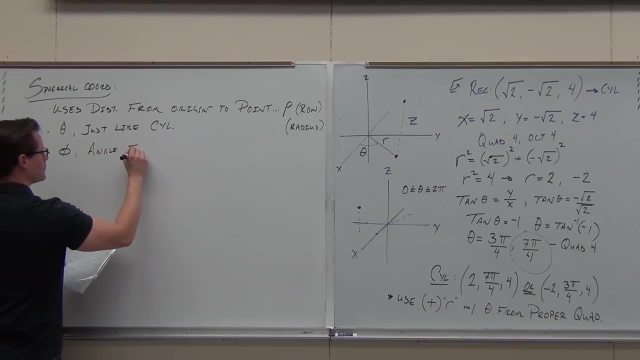 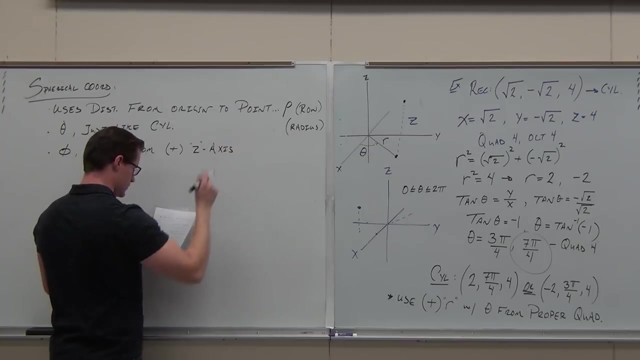 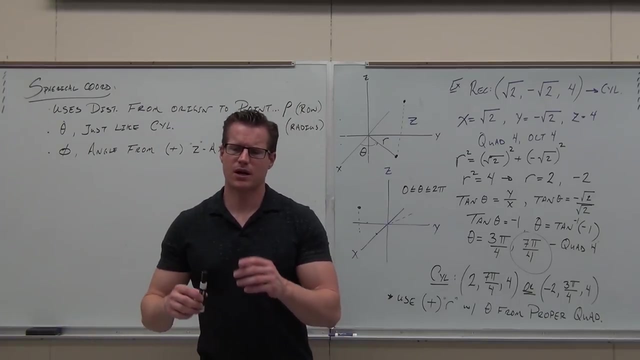 to the, the point rho, where that actually is. Now I do want to talk about you. you you probably can picture it right now, but if I'm talking about an angle from from z to my point z, is this, this line, right here? 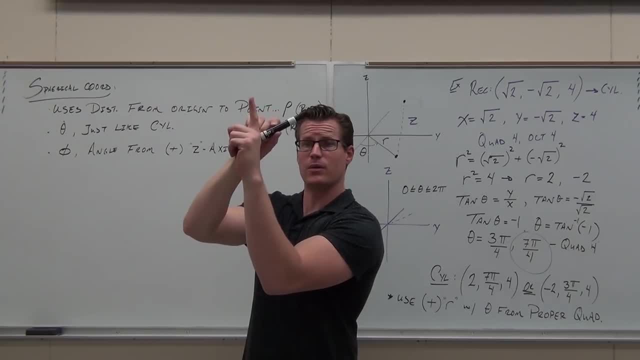 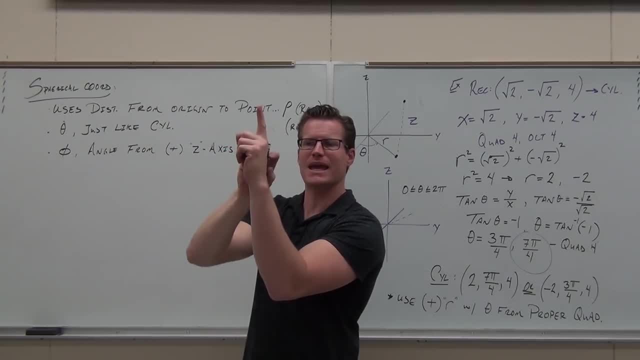 As soon as I get to pi, I can't go any further, because if I go further than pi, I'd be able to measure it from this way. Does that make sense to you? So it's from positive z, no matter where you're at. 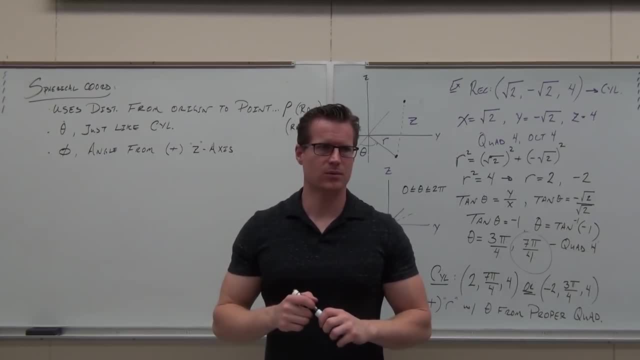 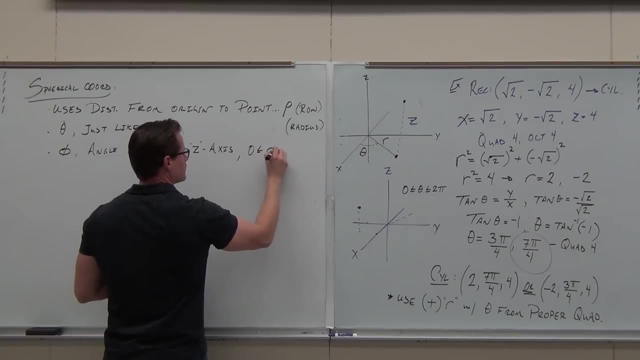 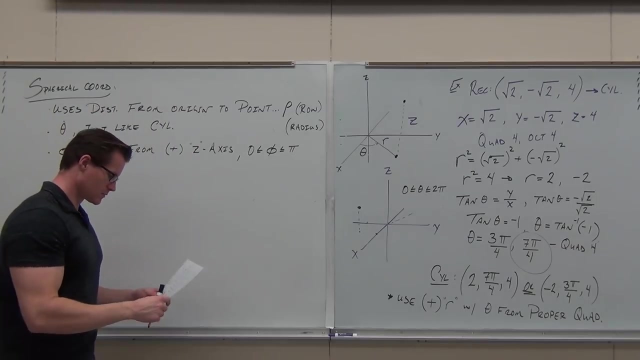 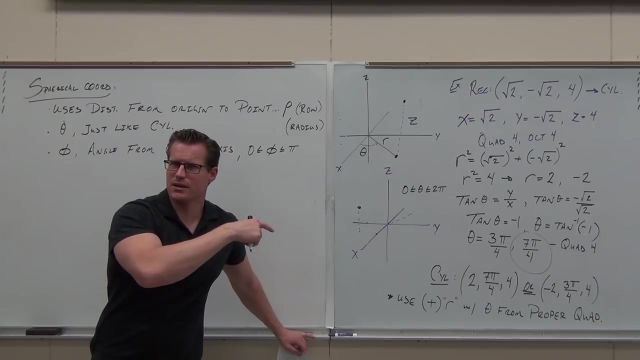 So this: this phi is always between 0 and pi. It does not go past pi. Also, since rho is a distance, it doesn't work exactly like r Rho. we take to be mean that it's never negative. 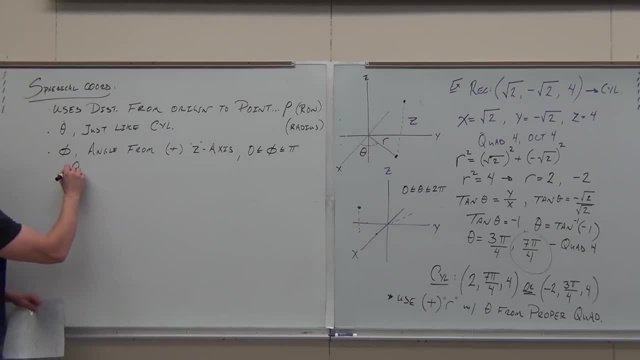 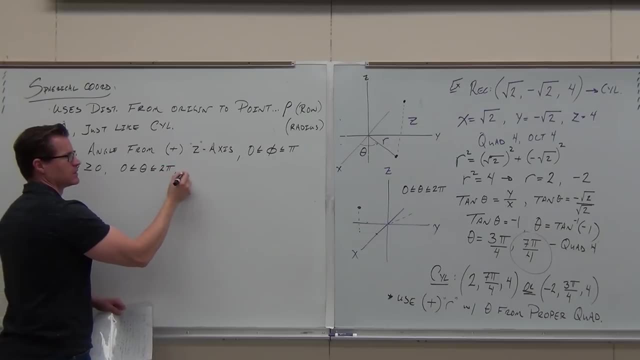 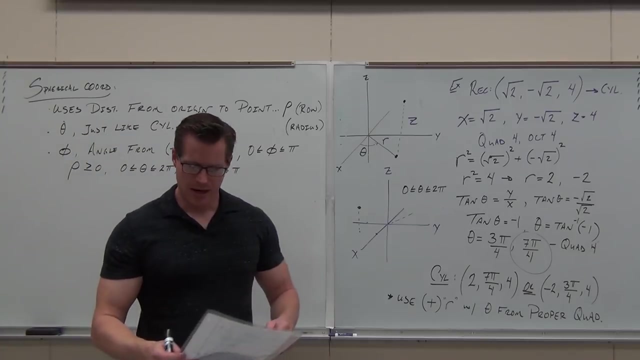 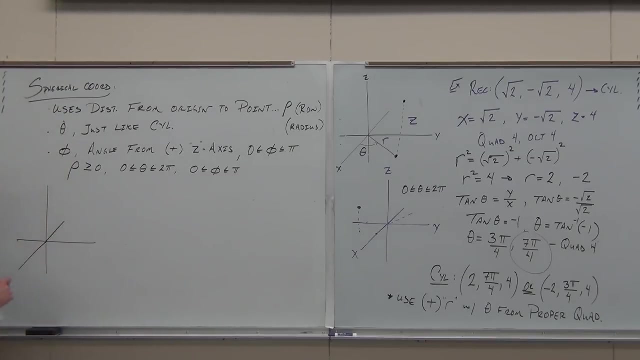 Rho is always defined as being positive, So rho is positive. Theta has exactly the same interval. And now phi. It has to be between 0 and pi, And what we get is this sort of a picture. We still have this, this a, we still have this distance here. 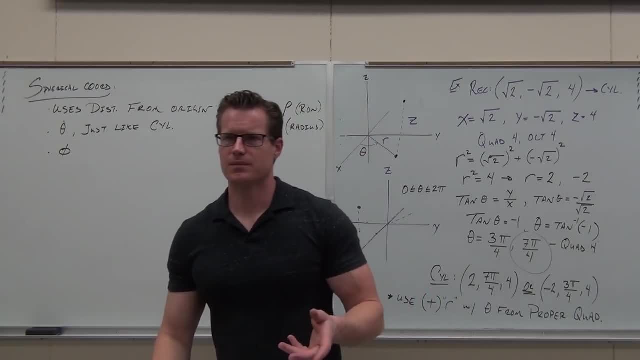 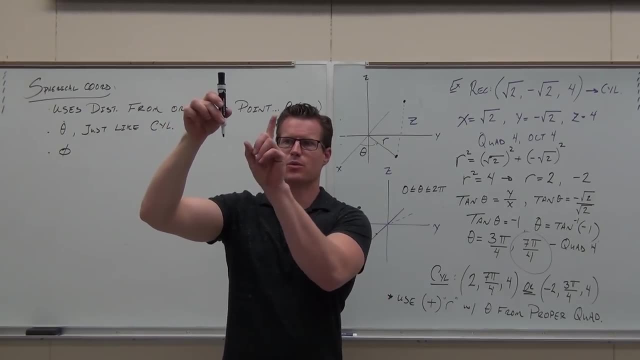 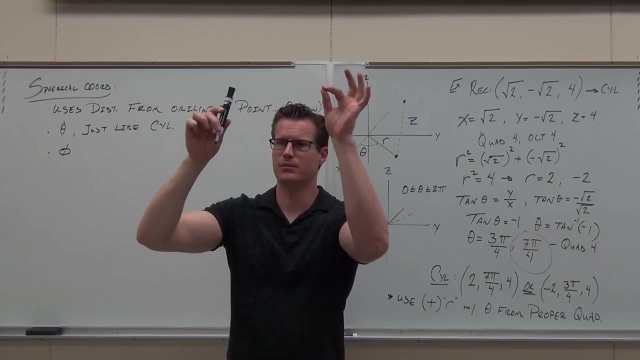 So this angle, phi, what this angle does. this angle is from the positive, positive Z axis to where that radius, that Rho is. It's the angle from positive Z to where the, the, the segment that would connect the origin to the. 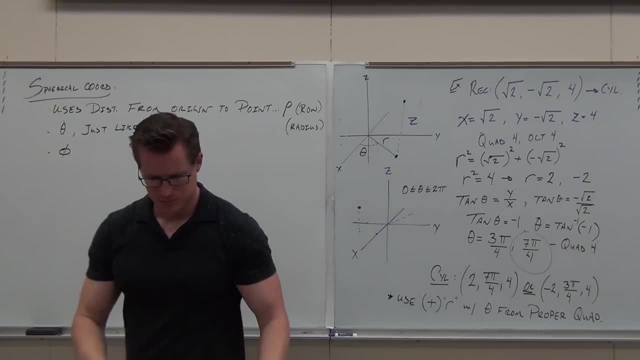 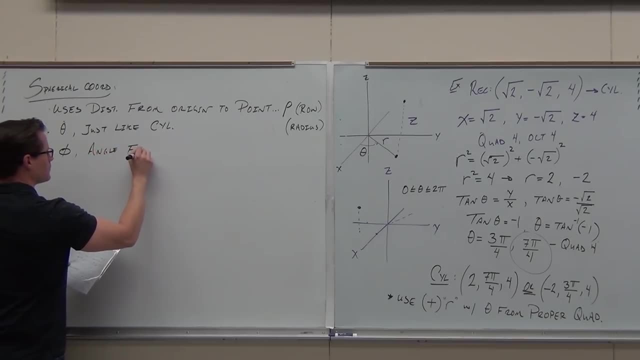 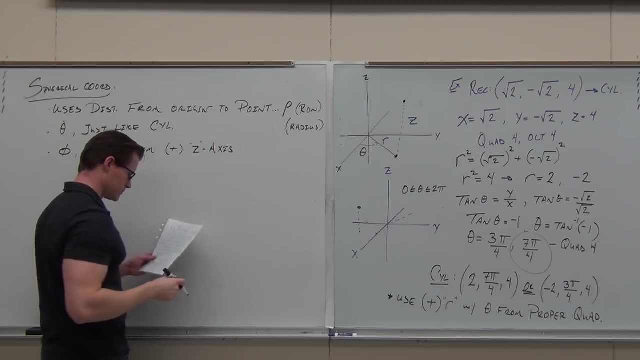 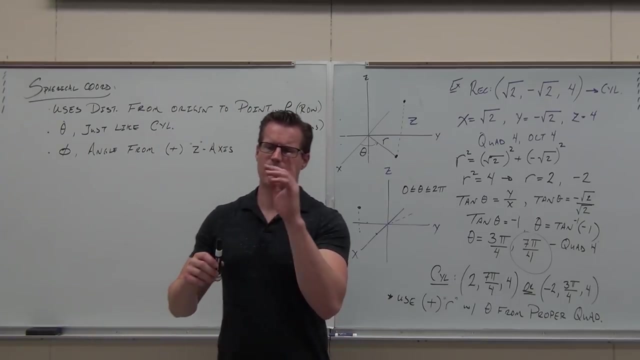 the point Rho, where that actually is. Now I do want to talk about you. you you probably can picture it right now, but if I'm talking about an angle from from Z to my point Z, is this, this line, right here? 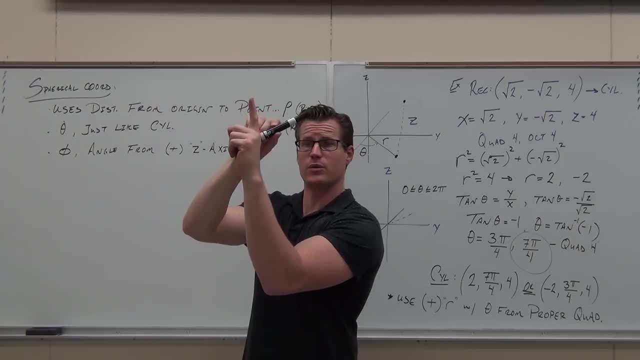 So as soon as I get to here, that would be pi over 2.. Does that make sense to you? This would be like pi over 6,, pi over 4, pi over 3,, pi over 2.. As soon as I get to pi, I can't go any further, because if I go further than pi, 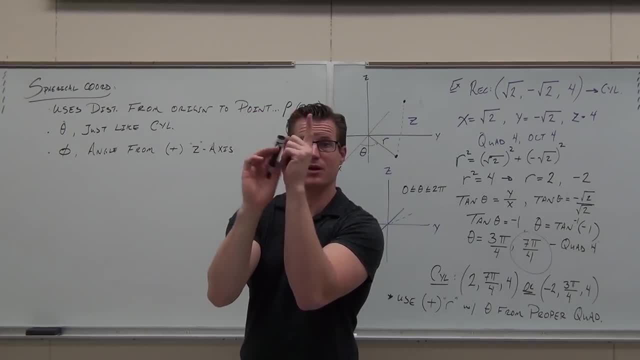 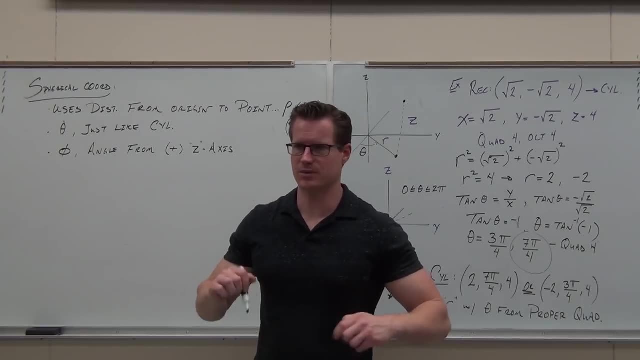 I'd be able to measure it from this way. Does that make sense to you? So it's from positive Z, no matter where you're at. So this, this phi, is always between 0 and pi. It does not go past pi. 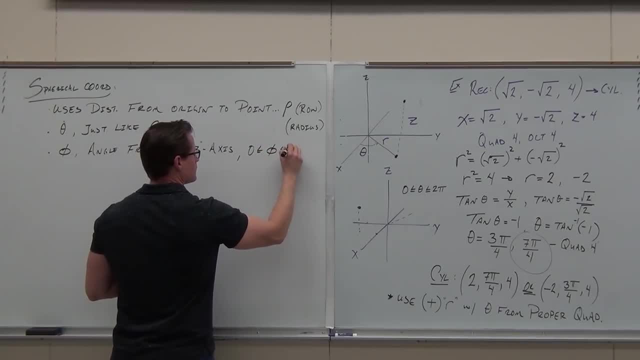 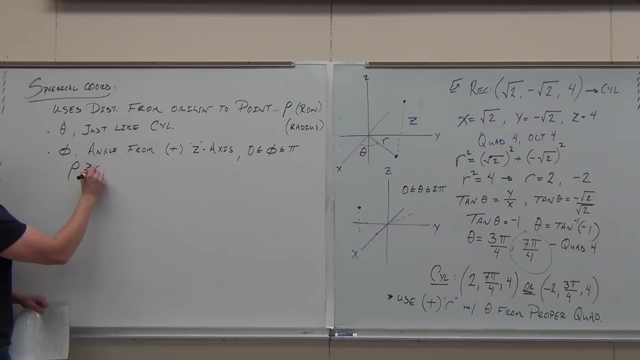 Also, since rho is a distance, it doesn't work exactly like r. Rho we take to be mean that it's never negative. Rho is always defined as being positive, So rho is positive. Theta has exactly the same interval. 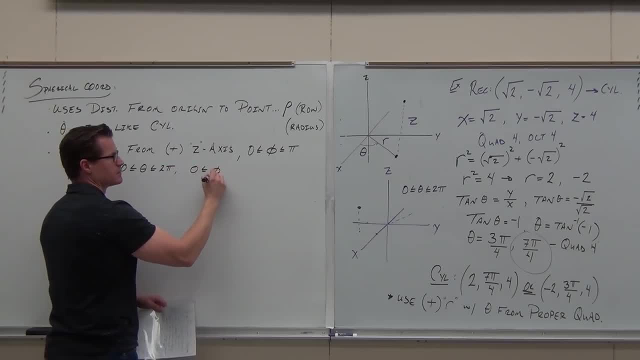 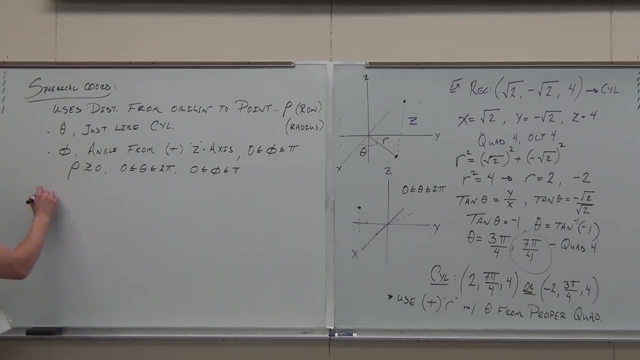 And now phi has to be between 0 and pi, And what we get is this sort of a picture. We still have this, this, hey, we still have this distance. We still have this distance here, but we don't define it in in spherical. 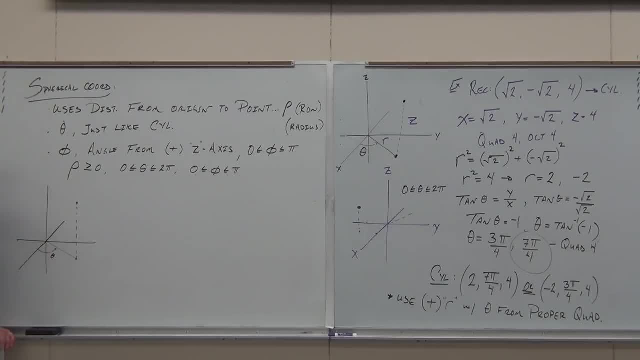 What we do have is the same exact theta. So the theta is still the angle from the positive x-axis to where the projection of that point is in x-y plane. It's still that same angle. We don't have a Z anymore. 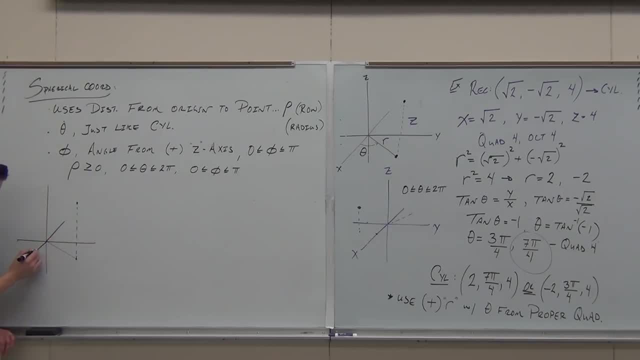 but we don't define it. We don't define it in in spherical. What we do have is the same exact theta. So the theta is still the angle from the positive x-axis to where the projection of that point is in xy-plane. 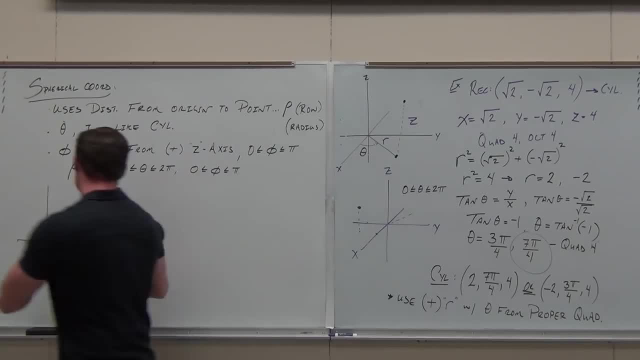 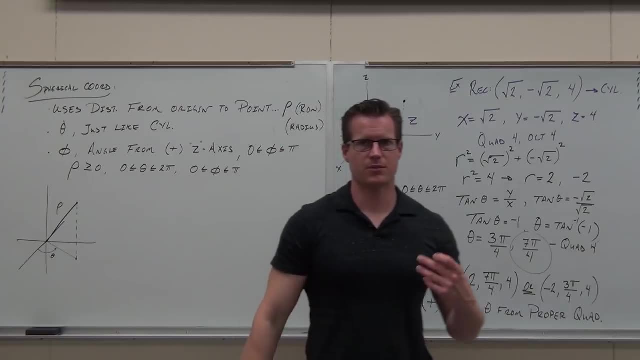 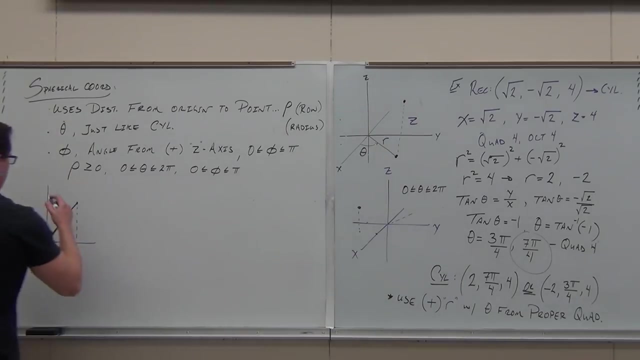 It's still that same angle. We don't have a z anymore. What we do have instead is a rho. The rho is the distance from the origin to the point, like direct straight shot radius. and then we have this guy From the z positive z, not negative z positive z to where that rho is. 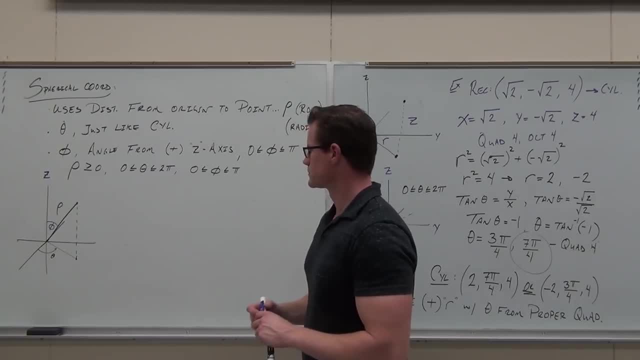 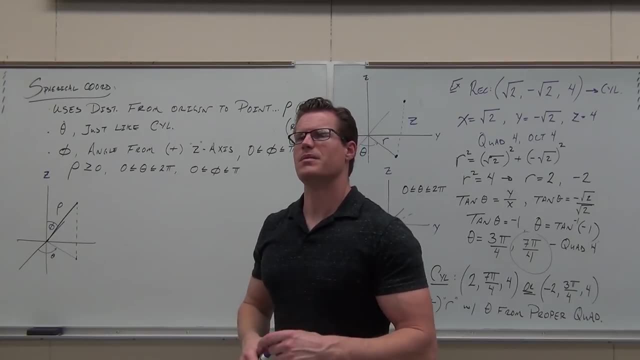 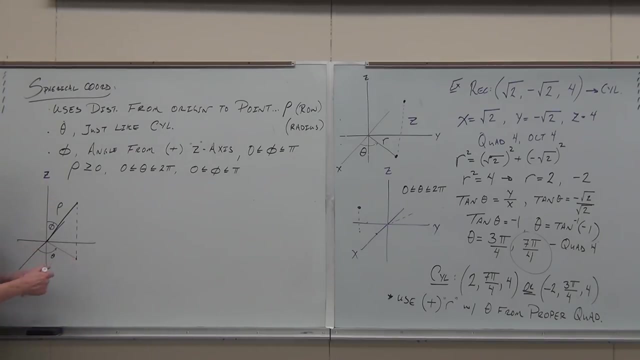 That is what phi is Head down, if you're okay with that one. By the way, if I did want to define it, what would that guy be? That would be r. Do you see that? this distance, if this is parallel to this? 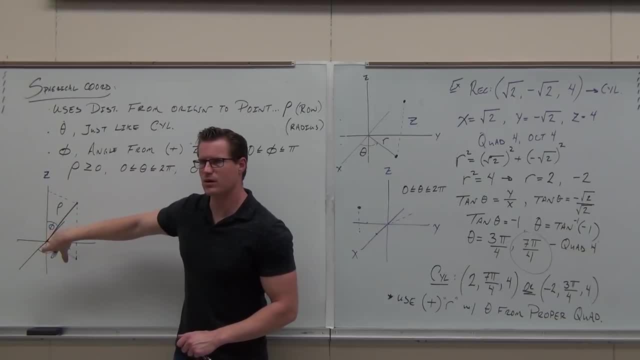 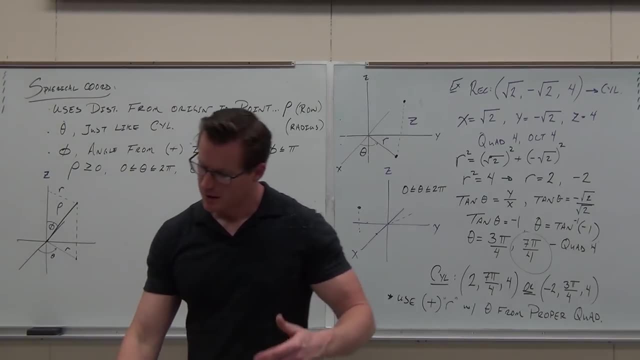 if this is right, do you see that that distance is the same as r? I'm going to use that to define a couple of things. you see, we now we got to have some ways to translate between z and pi, So this is r. 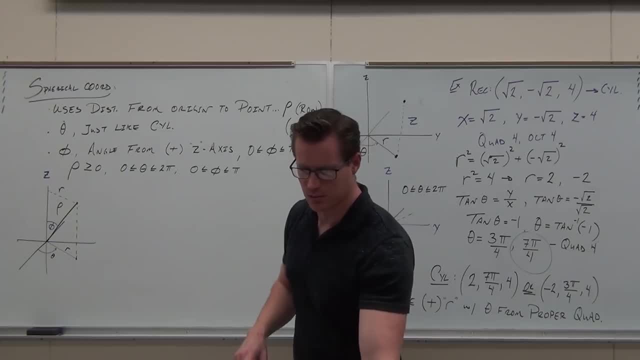 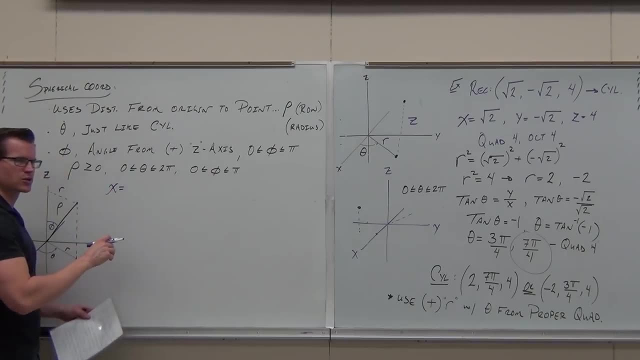 So we're going to do a little proof. It's not hard, It's a little proof here. So here's what we know. Actually, you know it. Come on quickly. What's x equal in terms of r's and theta's? 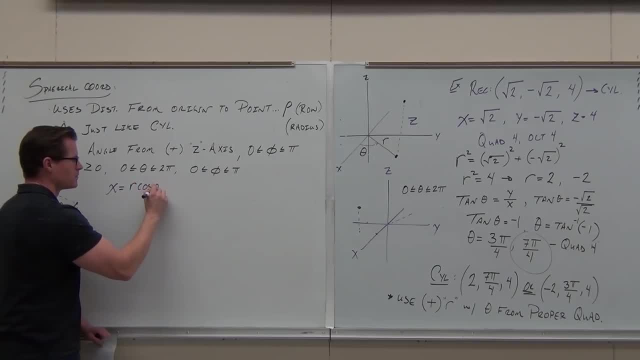 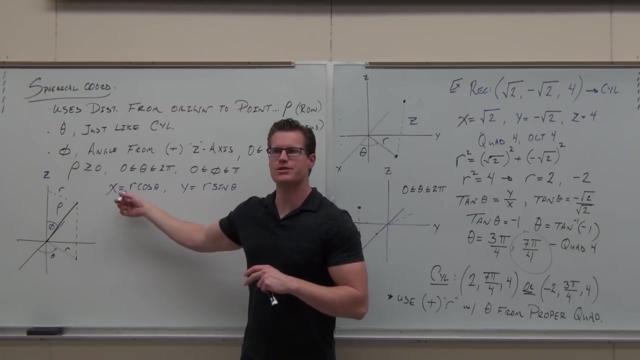 What's equal And what does y equal, please? But there's more. See, there's problems. If I'm going to spherical, I can't have any r's anymore. Do you see what I'm talking about? I need r's, I need theta's and I need phi's. 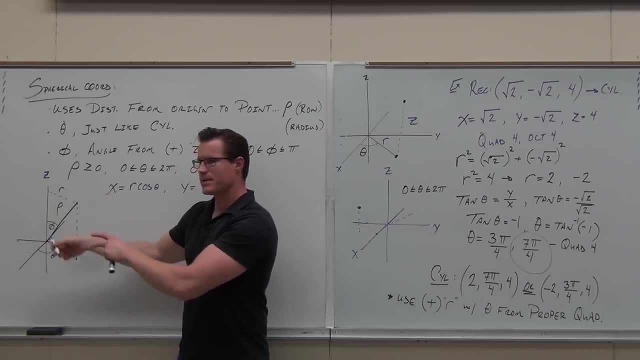 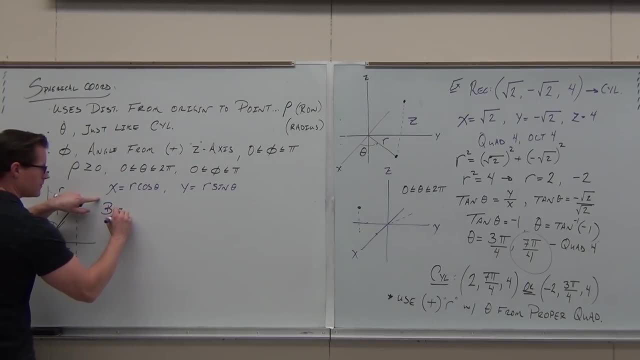 So we're going to translate from r to r's and phi's And here's how we're going to do it. Watch carefully: If you blink, you're going to miss it. okay, Check it out. Let's talk about r If I'm talking about r. 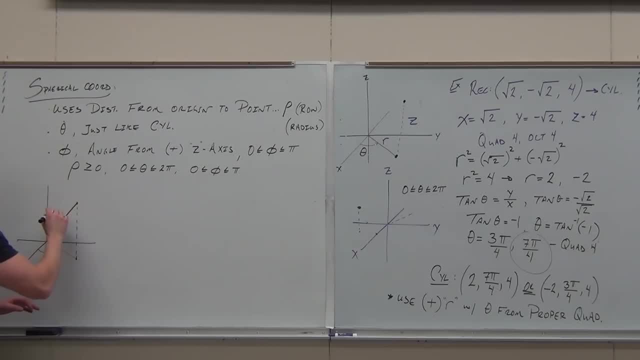 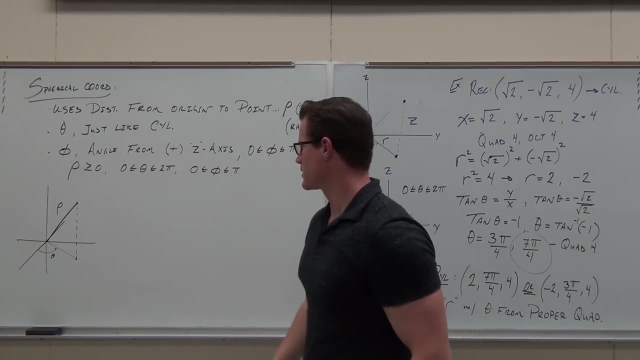 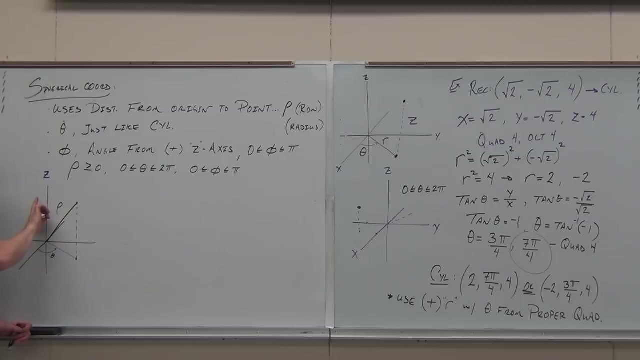 What we do have instead is a rho. The rho is the distance from the origin to the point, like direct straight shot radius. And then we have this guy From the z positive z, Not negative z positive z to where that rho is. 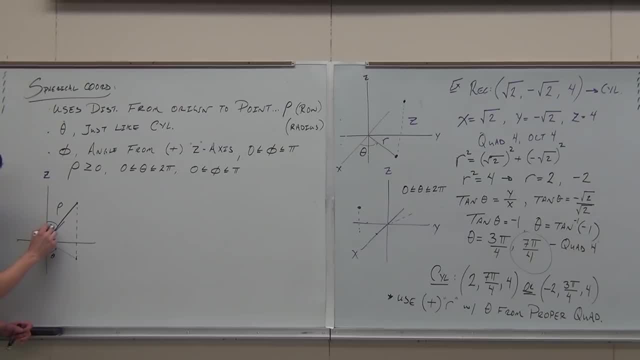 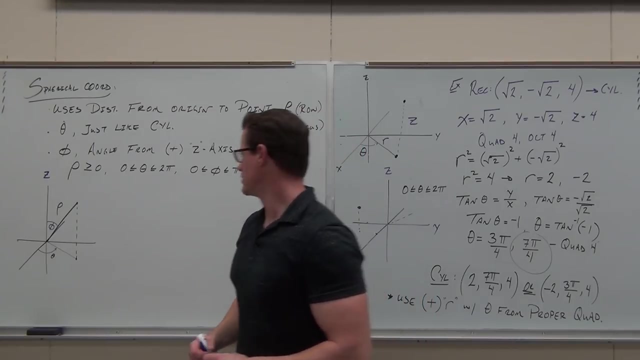 That is what phi is Head down, if you're okay with that one. By the way, if I did want to define it, what would that be? I would go to p times theta. that's the equation for this. I would go to p times theta. that's the equation for this. 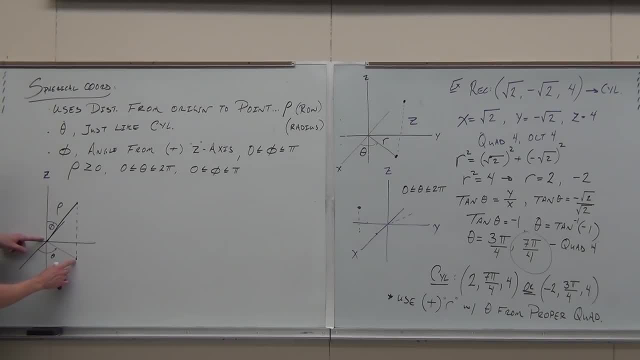 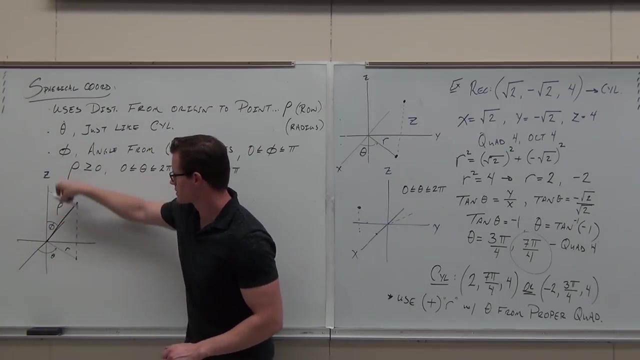 I would go to p times theta. that's the equation for this. What would that guy be? That would be R. Do you see that, this distance, if this is parallel to this, if this is right, Do you see that that distance is the same as R? 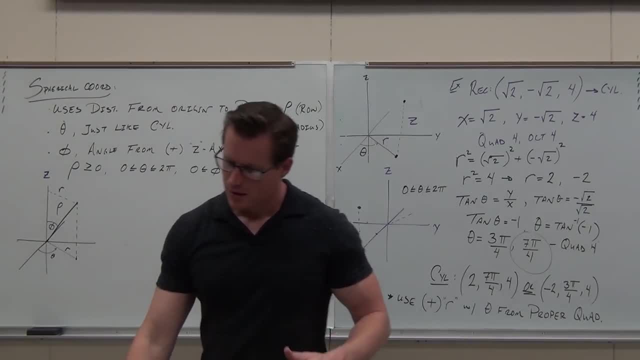 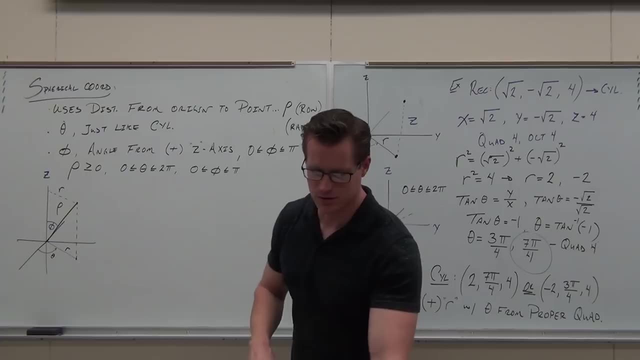 I'm going to use that to define a couple things. You see, we now we've got to have some ways to translate between spherical and rectangular. So we're going to do a little proof. It's not hard, It's just a little proof here. 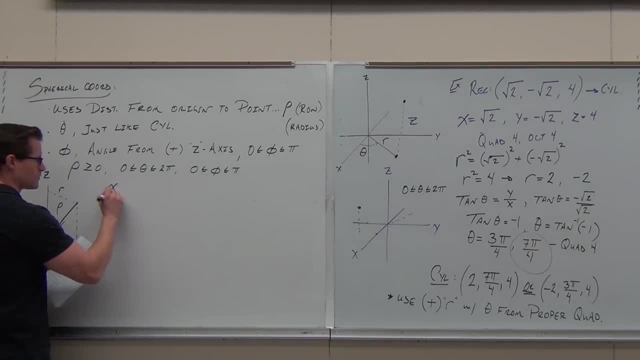 So here's what we know. Actually, you know it. Come on quickly. What's X equal in terms of R's and theta's? What's equal And what does Y equal, please? R equals R, But there's more. 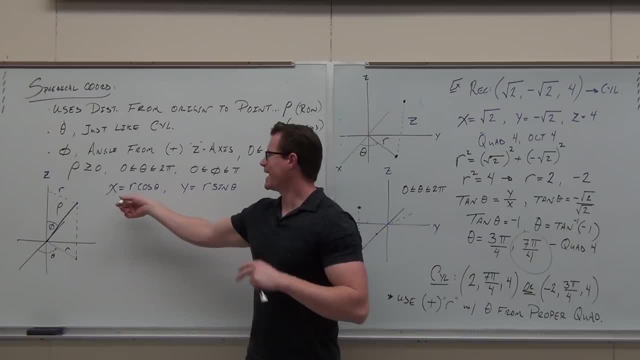 See, there's problems. If I'm going to spherical, I can't have any R's anymore. Do you see what I'm talking about? I need Rho's, I need theta's, I need phi's. So we've got to translate from R to Rho's and phi's. 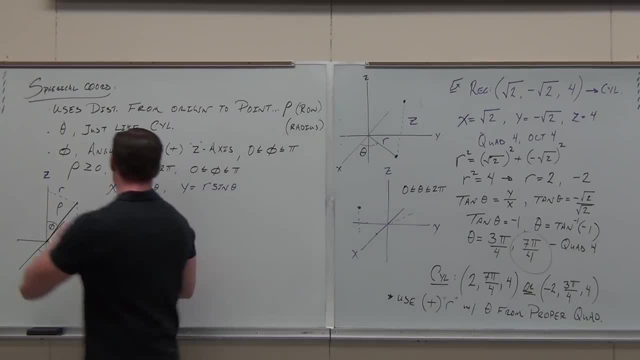 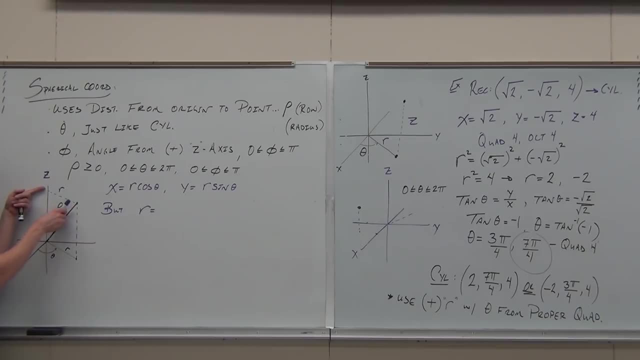 And here's how we're going to do it. Watch carefully. If you blink, you're going to miss it. okay, Check it out. Let's talk about R. If I'm talking about R, my distance from here to here is Rho. 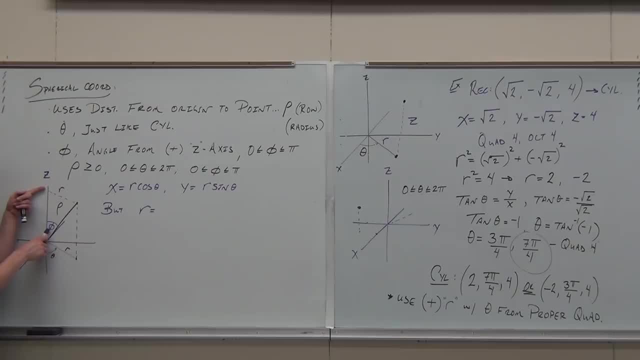 My angle from here to here is phi. So if I'm talking about Rho, sorry R, that's opposite. Just think of the triangle here. That's opposite over hypotenuse. What gives us the relationship of opposite and hypotenuse? 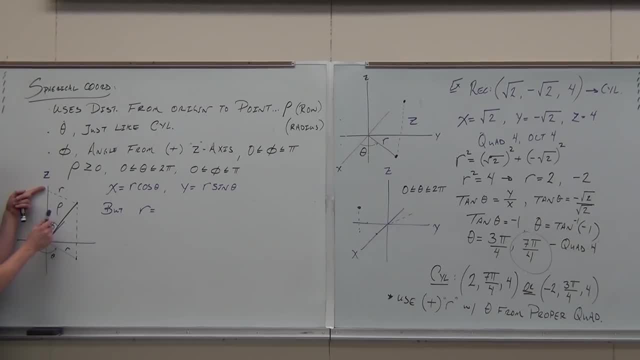 my distance from here to here is rho. My angle from here to here is phi. So if I'm talking about r, I'm going to have to do a little proof. If I'm talking about rho, I'm sorry r, that's opposite. 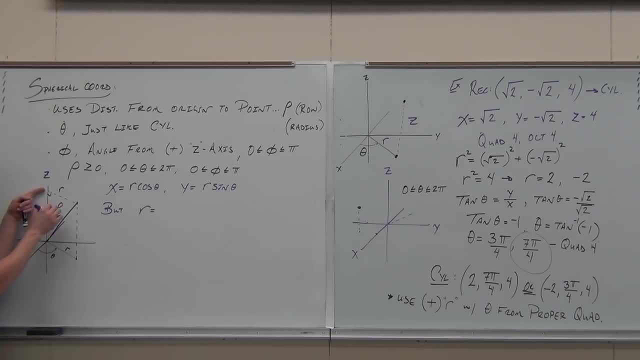 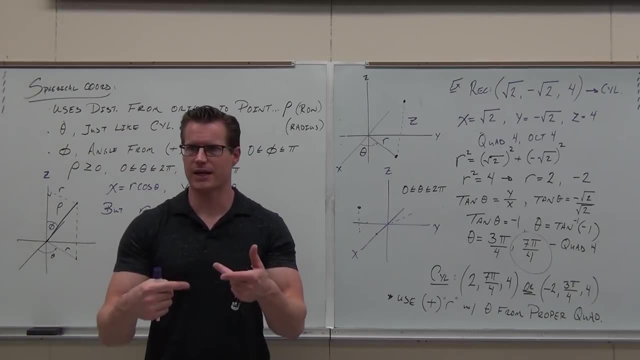 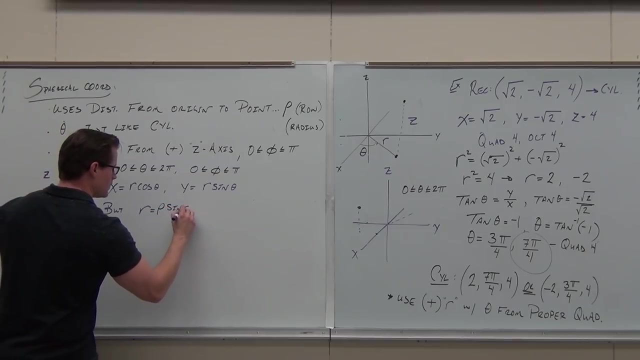 Just think of the triangle here That's opposite over hypotenuse. What gives us the relationship of opposite and hypotenuse? And if I solve for r, we get rho sine phi. Do you see how we get rho sine phi? No, 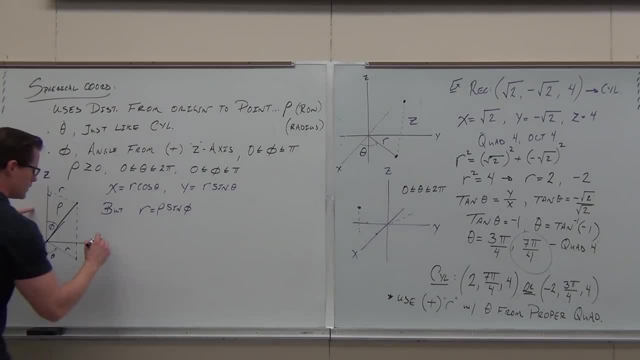 If you don't see it here, it is: Sine phi is opposite over hypotenuse. Did you guys see it? Multiply by rho Boom R equals rho sine phi. So now if we substitute that, well, hey, r is sorry. 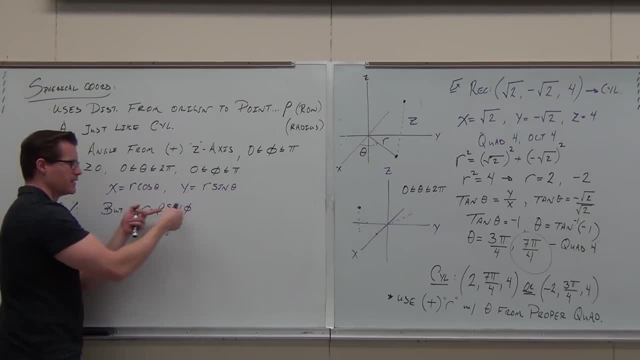 x is r cosine theta, r is rho sine phi, Y is r sine theta, r is rho sine phi. So now we have x equals- looks nasty, R equals rho sine phi, times cosine theta. And y becomes rho sine phi, times sine theta. 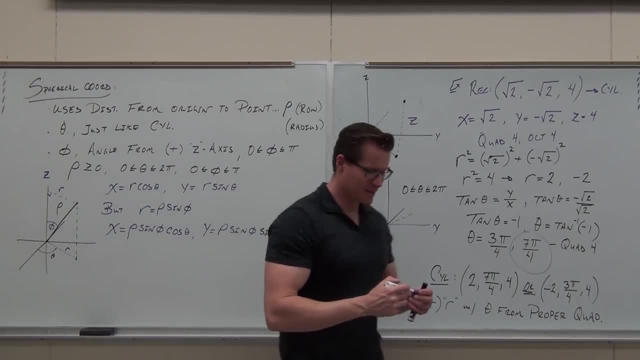 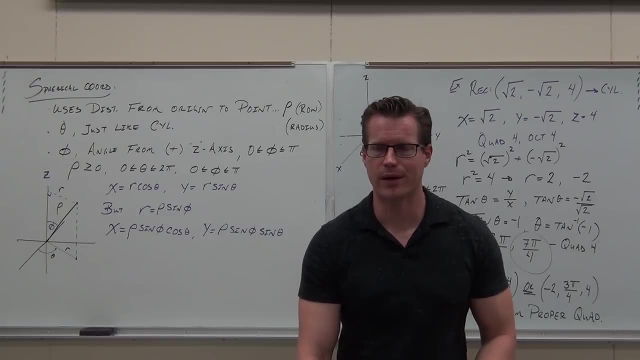 These can get awfully hard to remember- They really can, especially the different phis and thetas. You write the wrong one and they screw it way up. That happens to me all the time, But here's how I always think about it. 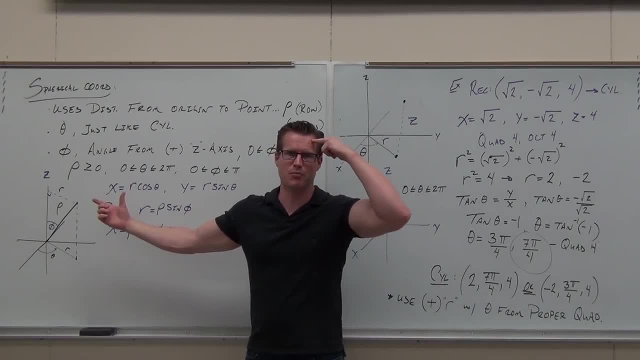 I think about it. I think about x as r, cosine, theta, because that's like burned into my head and I can't get rid of it. all right, It's like you click on the wrong thing. oh, whatever, But it's there. 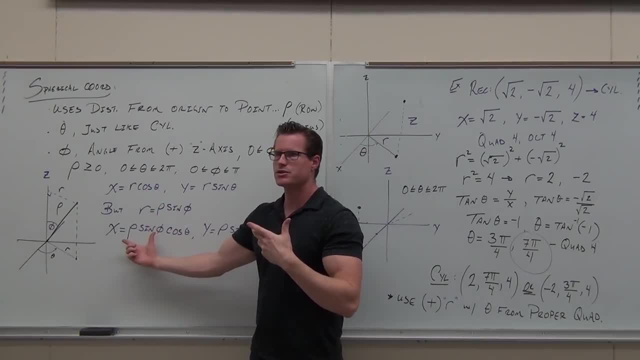 You can't unsee things Or I can't unsee. that's in my head. This one's not. So when I think about x, I think about, I think about r, cosine, theta, And I go: well, what's r? 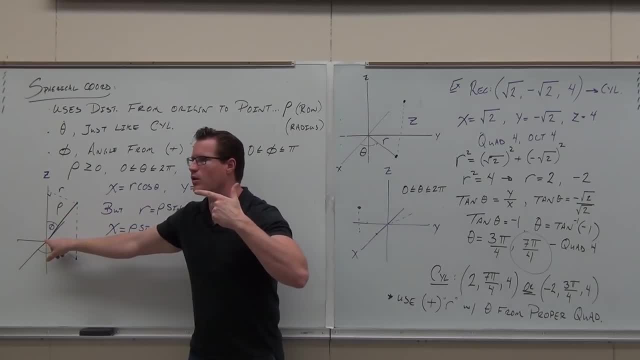 R is the rho sine theta. Why? Because I have a picture of this in my head And I go: okay, this is r is the opposite over hypotenuse. That gives me the r and the sine And the sine aspect of that. 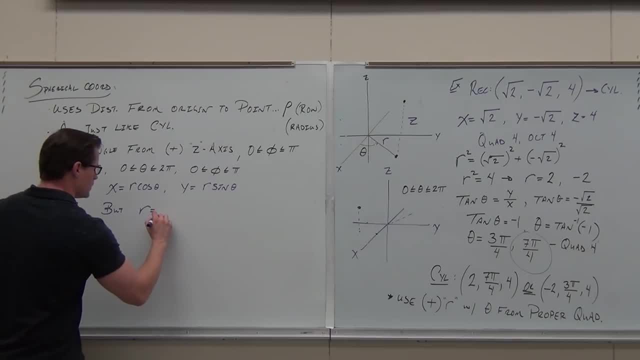 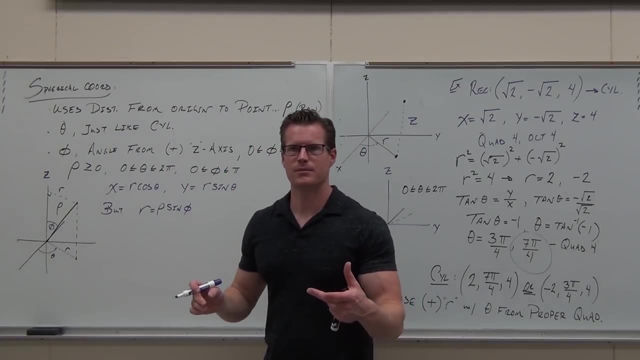 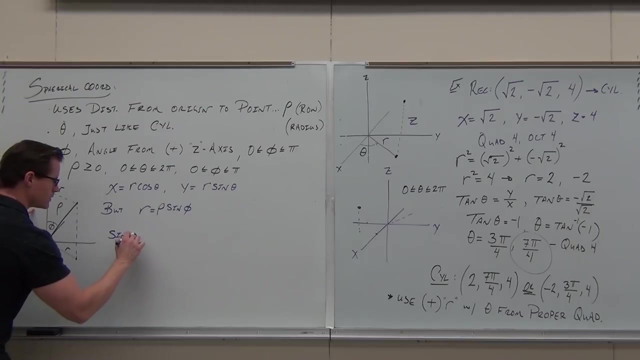 And if I solve for R, we get Rho sine phi. Do you see how we get Rho sine phi? No, If you don't see it, here it is. Sine phi is opposite over hypotenuse. Did you guys see it? 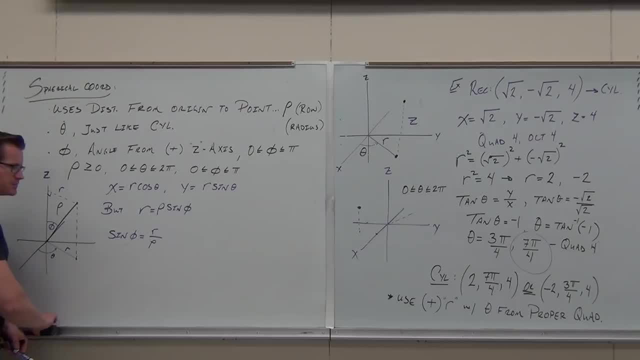 Multiply by Rho Boom R equals Rho sine phi. So now, if we substitute that, well, hey, R is sorry. X is R cosine, theta R is Rho sine phi. Y is R sine theta, R is Rho sine phi. 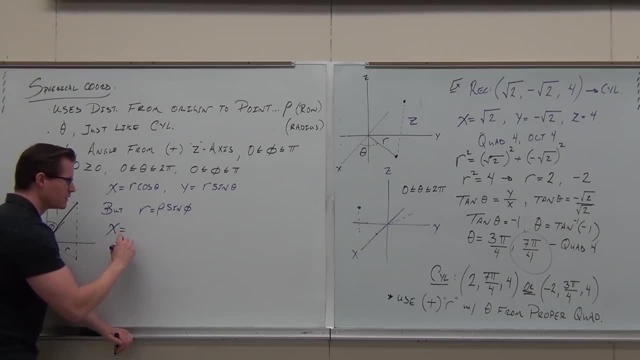 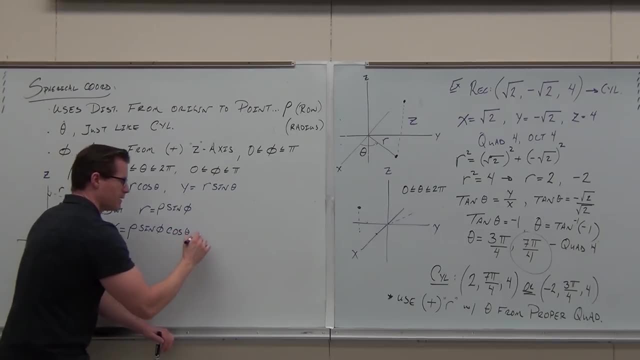 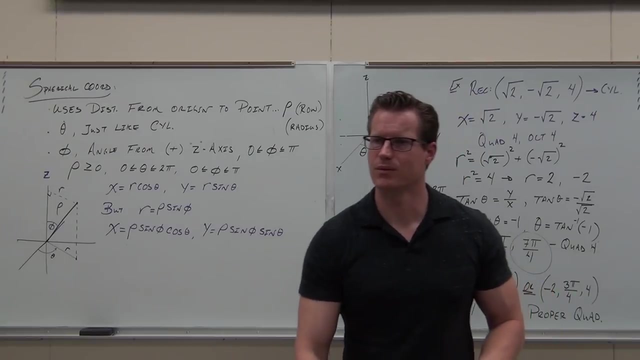 So now we have X equals- It looks nasty- Rho sine phi times cosine theta. And Y becomes Rho sine phi times sine theta. These can get awfully hard to remember- They really can, especially the different phis and thetas. 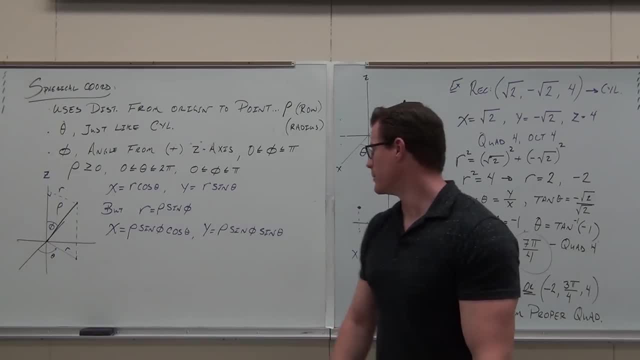 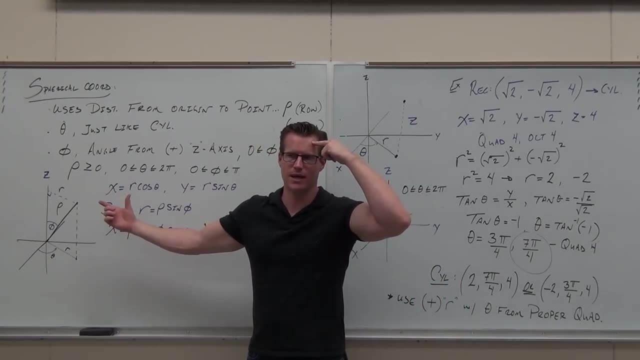 You write the wrong one and they screw it way up. That happens to me all the time, But here's how I always think about it. I think about X as R cosine theta, because that's like burned into my head and I can't get rid of it. all right. 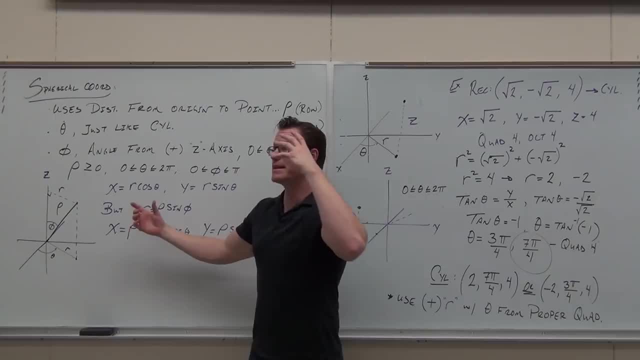 It's like you click on the wrong thing, Oh whatever, But it's there. You can't unsee things, Or I can't unsee. That's in my head. This one's not. So when I think about X, I think about R cosine theta. 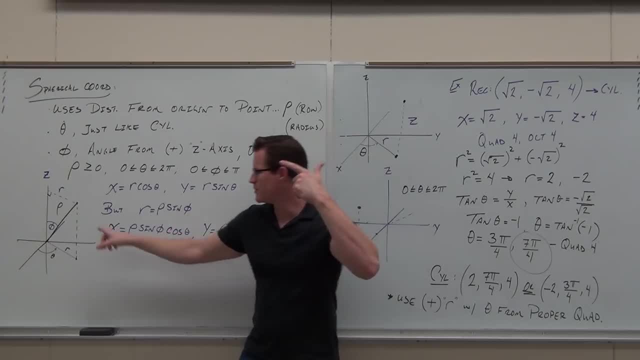 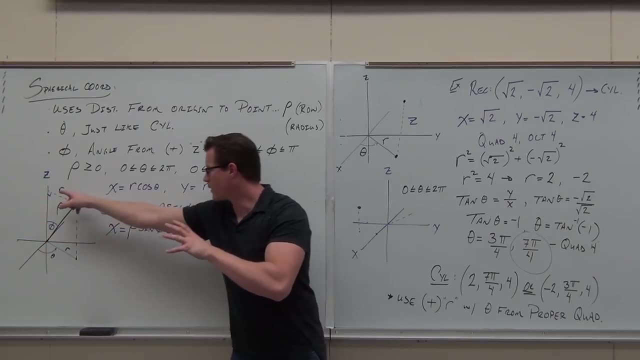 And I go: well, what's R? R is the Rho sine theta. Why? Because I have a picture of this in my head. I go: okay, this is R is the opposite over hypotenuse. That gives me the R and the sine aspect of that. 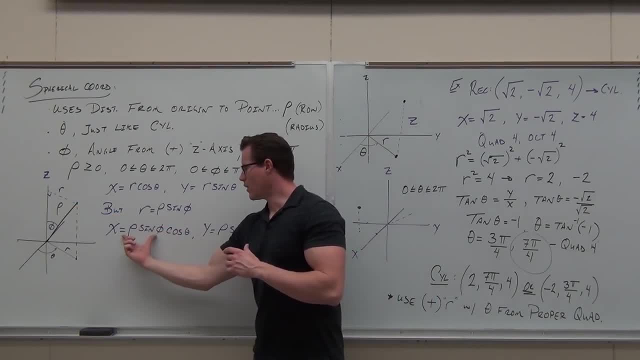 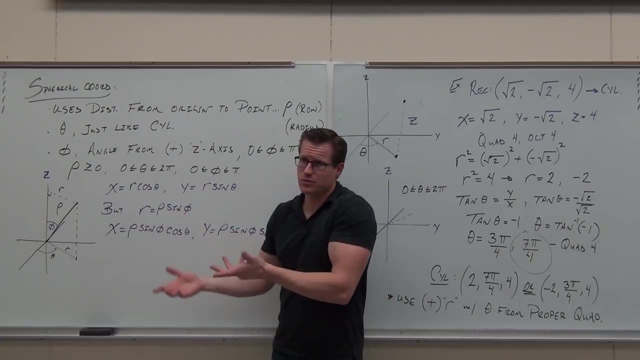 Does that make sense to you? So here we got R cosine theta and R sine theta. It's the same stuff. We now just define what R is. It's Rho sine theta, Sorry, Rho sine phi. So if I just be a little key with, there's only one more that we got to do. 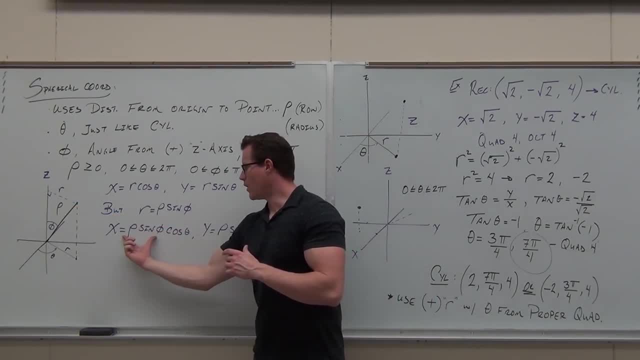 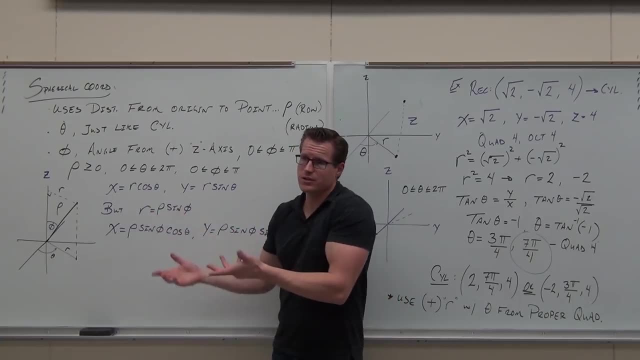 Does that make sense to you? So here we got r cosine theta and r sine theta. It's the same stuff. We now just defined what r is? It's rho sine theta. Sorry, rho sine phi. So if you look here, there's only one more that we got to do. 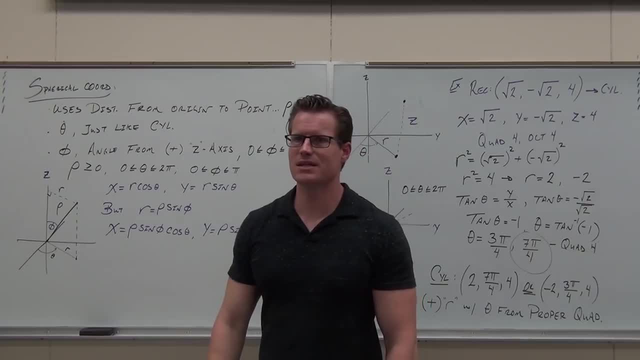 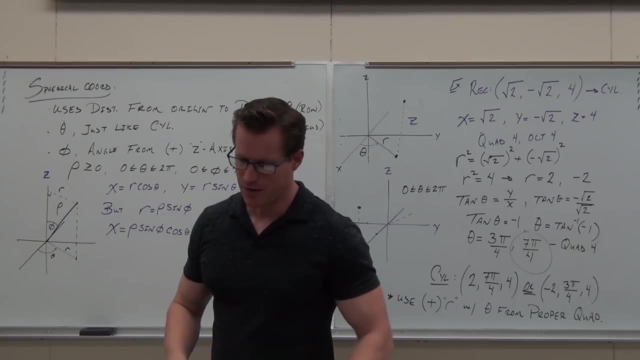 You see, this stuff doesn't have z's in it. It's not going to have z's anymore. What we're going to have to find is well, a way to translate that. So how we translate from Z's in, from z's, let's say: 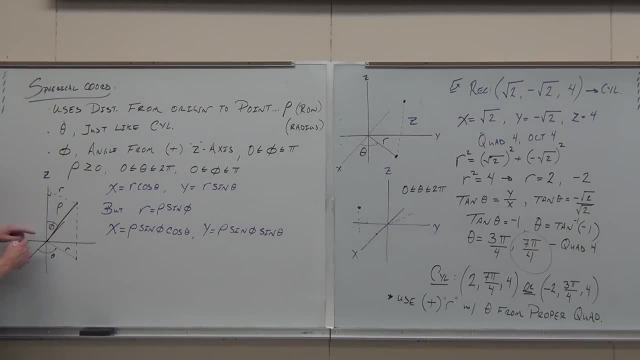 I'm going to be given this, this height, this z here. Well, this, this would be z. How does z compare with phi and rho? Think of the right triangle, you think. Come on, What would? what would take z and rho and put them together with phi? 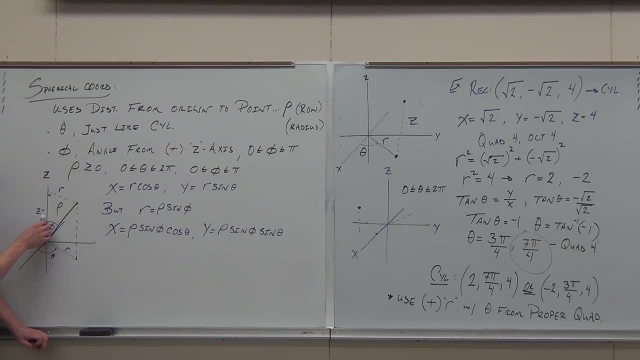 What? what trig relationship? This is the adjacent Cosine, That's the hypotenuse Cosine. Do you guys see the cosine that I'm talking about? So if I'll do it for you, If cosine phi would equal adjacent over hypotenuse, if I solve for the z, 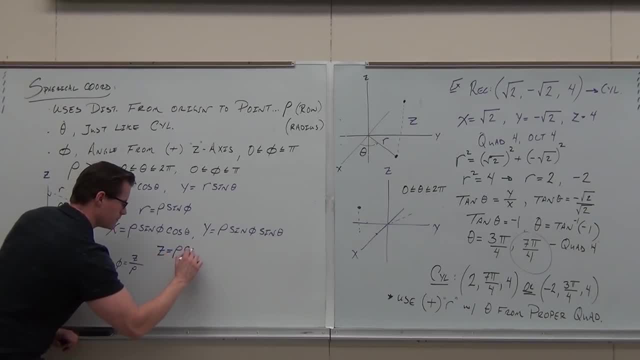 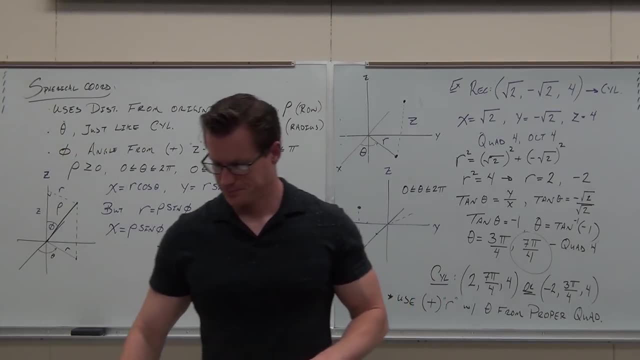 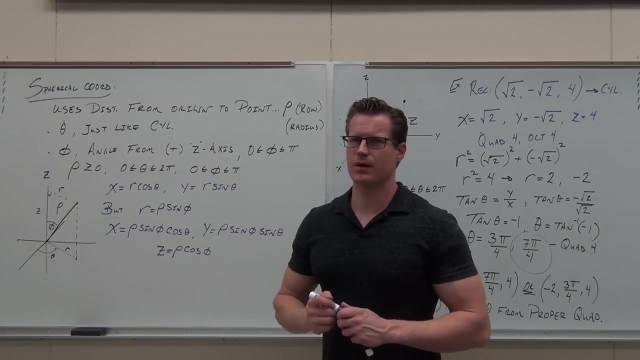 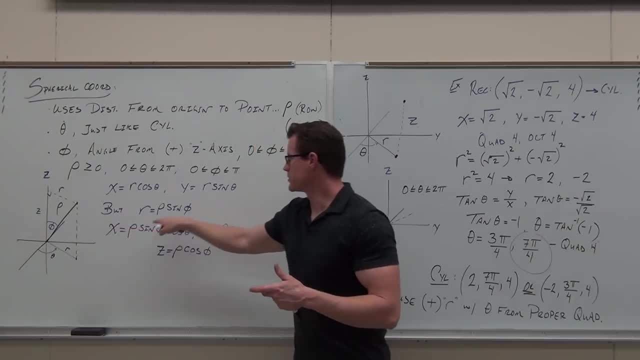 Now how would you use it? Would you go from rectangular to spherical or from spherical to rectangular? here You plug in all the spherical stuff. it's going to give you x's, y's and z's. This is how you go from spherical to rectangular. 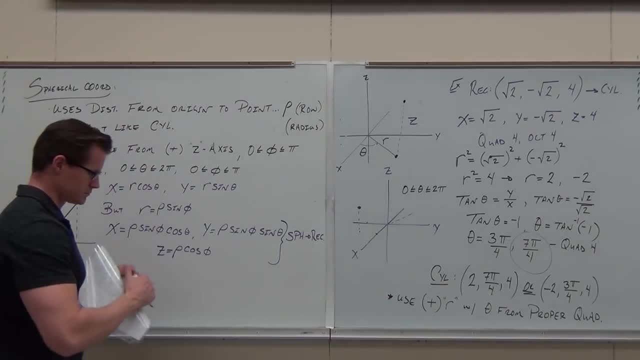 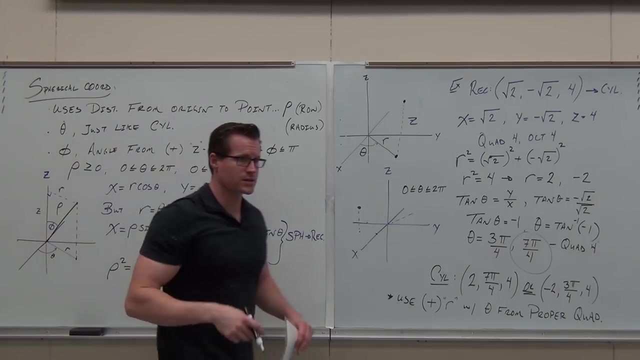 How do you go back? Well, we got something pretty nice here. We know that the equation of a sphere- what a sphere looks like- is: radius squared equals x squared plus y squared plus z squared. Since we have spherical coordinates, that's going to allow us to translate back from rectangular. 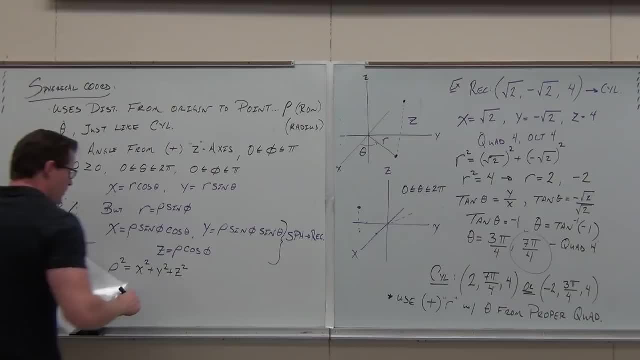 to at least the row aspect. Take a square root- and you're good, By the way, when you take a square root, you only consider positive rows. Unlike the r, you only consider positive rows. We think of this as a true radius. 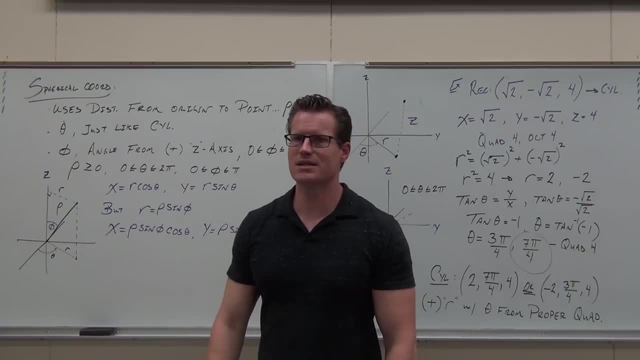 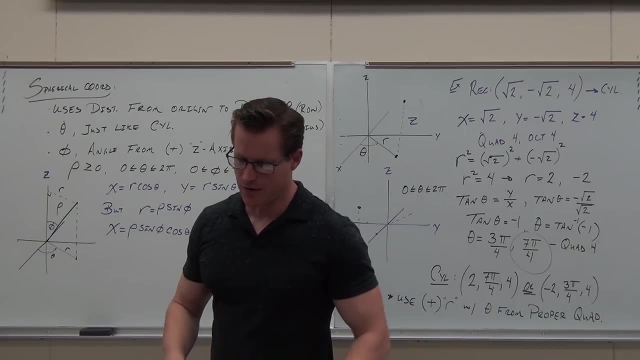 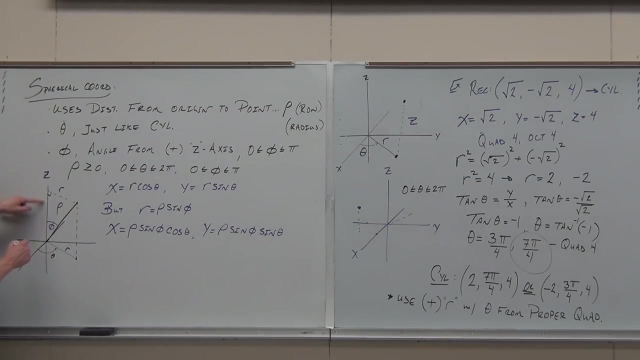 You see, this stuff doesn't have Zs in it. It's not going to have Zs anymore. What we're going to have to find is, well, a way to translate that. So how we translate from Zs. let's say, I'm going to be given this height of Z here. 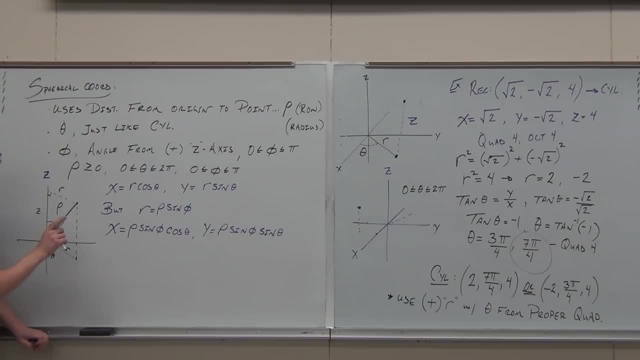 Well, this would be Z. How does Z compare with phi and Rho? Think of the right triangle you're getting. Come on, What would take Z and Rho and put them together with phi? What trig relationship. This is the adjacent. 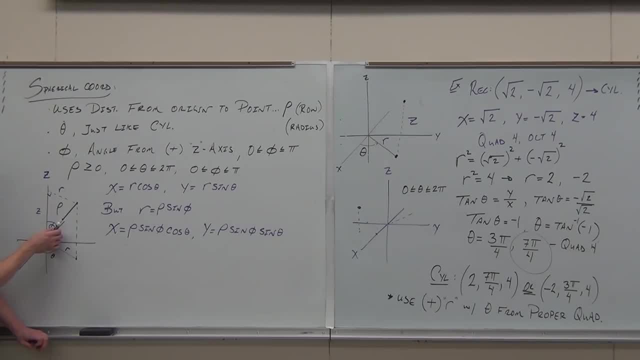 That's the hypotenuse Cosine, Cosine. Do you guys see the cosine that I'm talking about? So if I'll do it for you, If cosine phi would equal, adjacent over hypotenuse, if I solve for the Z. 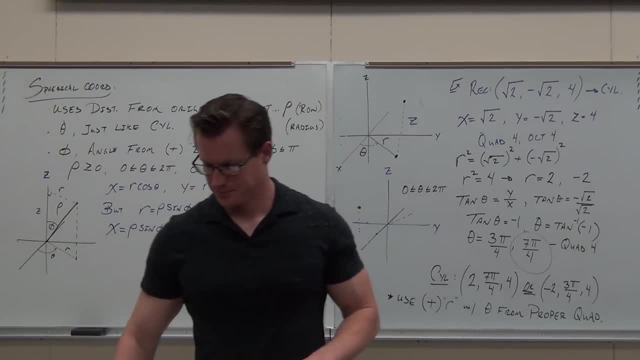 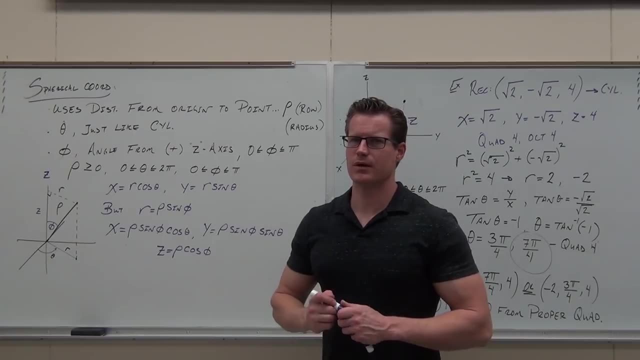 we got Rho, cosine phi. It's Rho, times Rho, So we have a plus and it's minus. I'm going to do a new equation and I'm going to do it for you. We're going to use it for the first time. 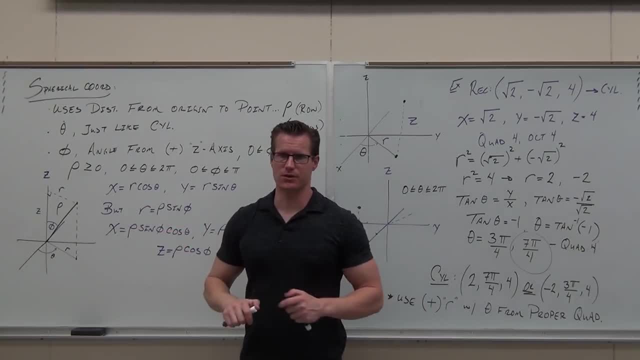 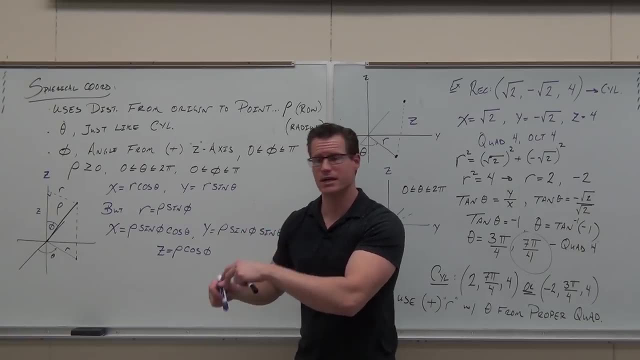 I don't know if you're okay with this. I want to know if you're okay with those ones. Are you? Now, how would you use it? Would you go from rectangular to spherical or from spherical to rectangular? here You plug in all the spherical stuff. 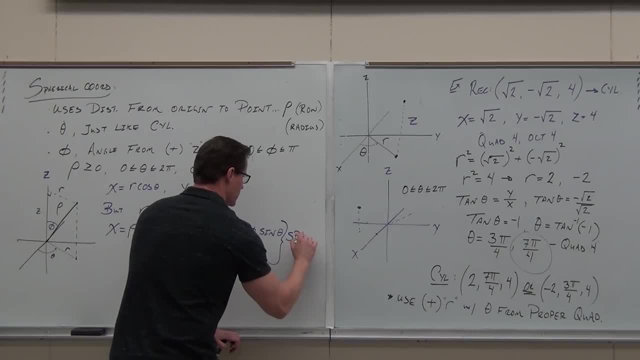 It's going to give Xs, Ys, Zs. This is how you go from spherical to rectangular. Let's do a new equation, Let's try it. Let's do a new question. Let's do a new equation, Let's try it. 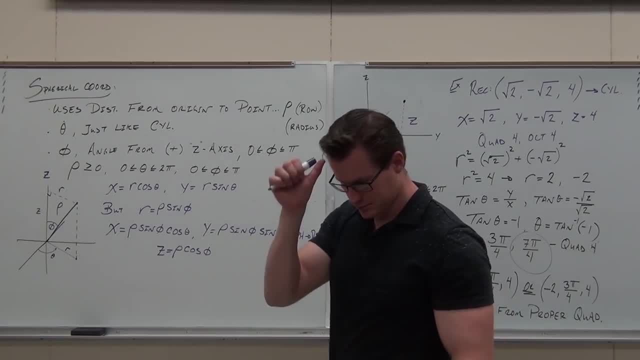 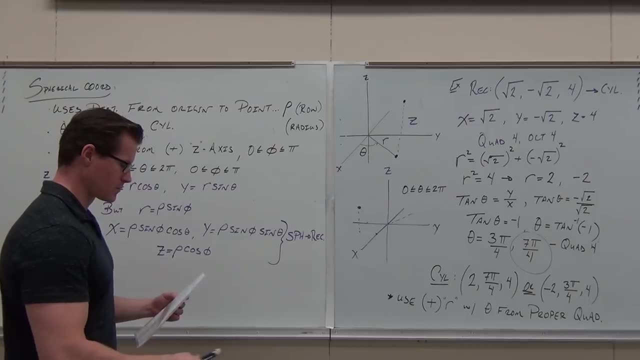 Alright, Let's go with that. How do you go back? Well, we got kind of some pretty nice here. We know that the equation of a sphere- what a sphere looks like, is: radius squared equals x squared plus y squared plus z squared. 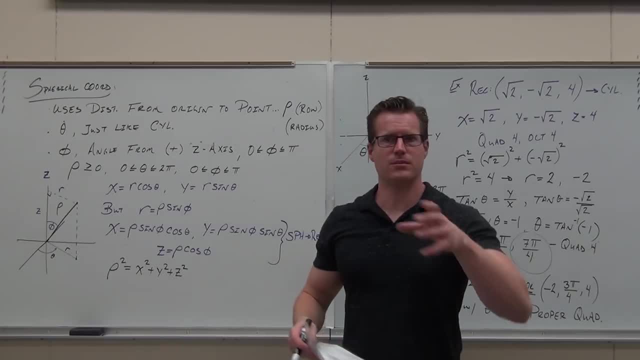 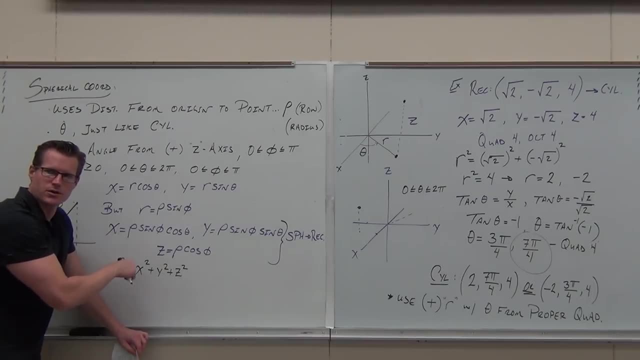 Since we have spherical coordinates, that's going to allow us to translate back from rectangular to at least the row aspect. Take a square root. you're good, By the way, when you take the square root, you only consider positive rows. Unlike the r, you only consider positive rows. 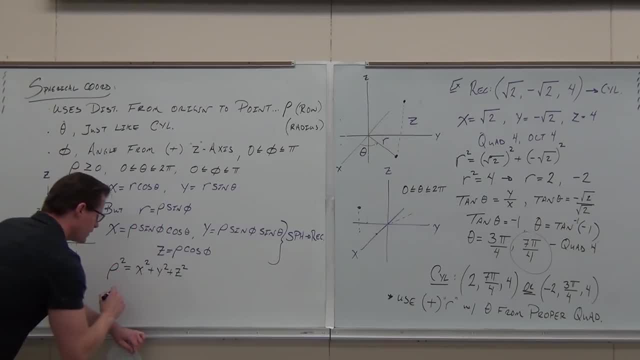 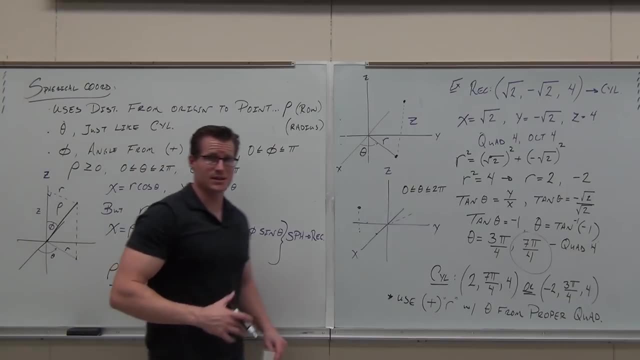 We think of this as a true radius. It is always positive. But then we also have that theta. What's nice about the theta? it's literally the same theta. So you have tan. theta equals y over x. That's the same thing. 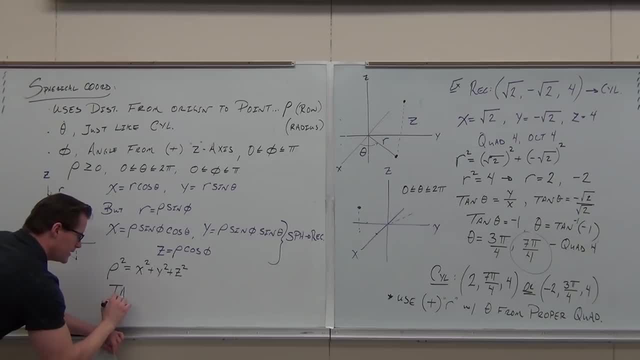 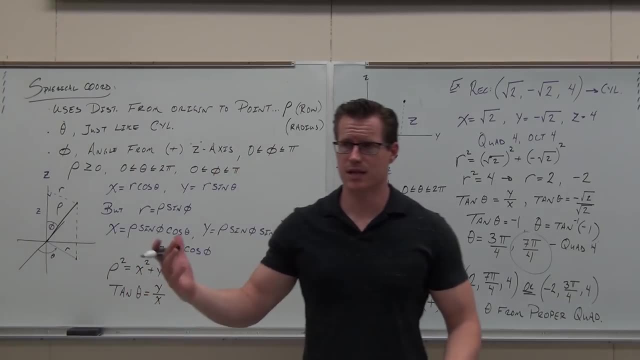 It is always positive. But then we also have that theta. What's nice about the theta? it's literally the same theta. So you have tan. theta equals y over x. That's the same thing. The only other one is this one: 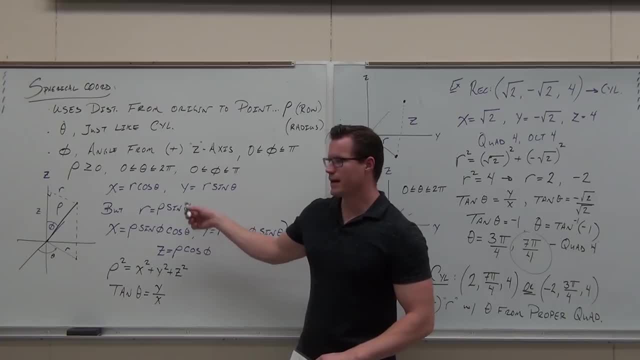 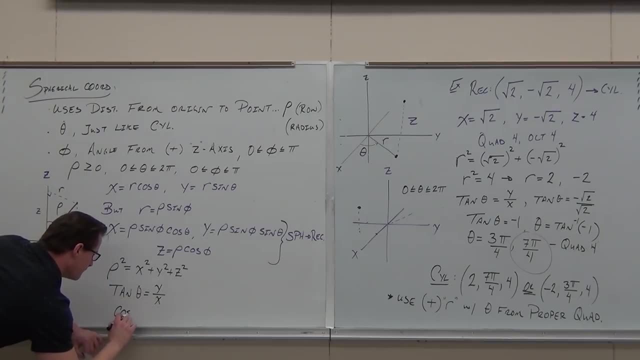 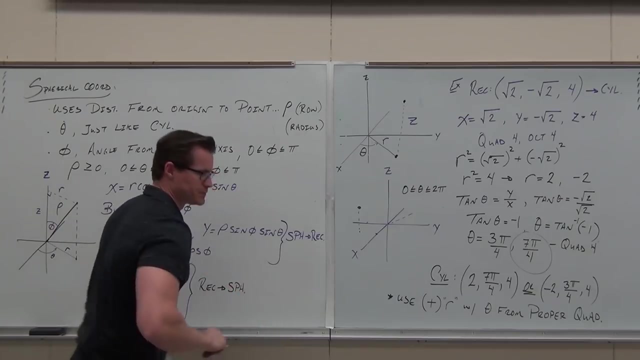 If we use this and solve for cosine phi, we're going to have z over rho and that's the way we get back to our, our phi, And that's how we're going to go back from rectangular to spherical. The examples are actually pretty quick. 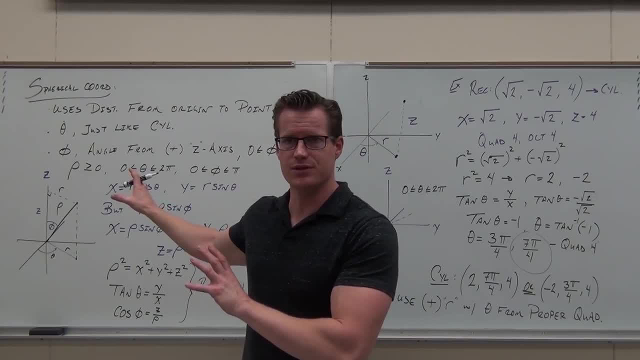 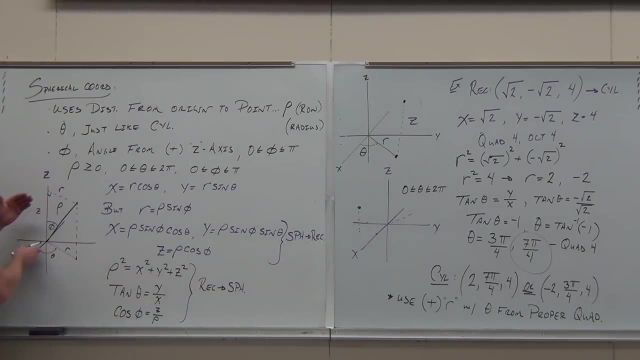 but I want to make sure that you guys understand at least the idea of what these these look like And not if you you do, you feel it, you're okay with that one. So the way spherical works: again, it still has this theta. 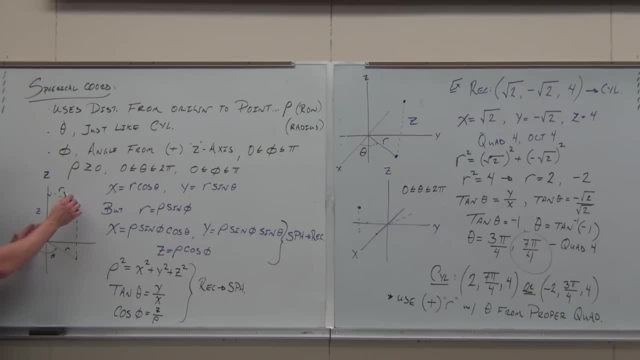 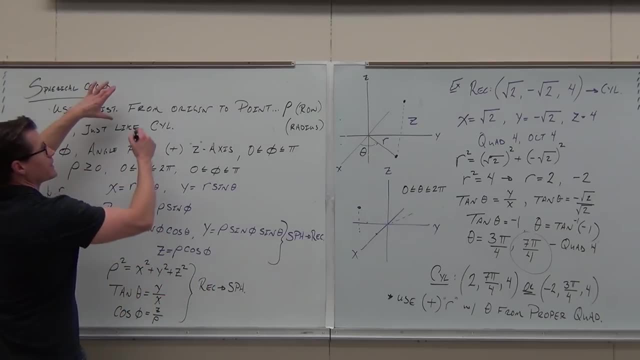 It no longer has a z. It's got a distance straight from origin to point. It has other angle, telling us our our aspect from the positive z axis. All of the spherical coordinates are written in this format. Now that we understand all this stuff. 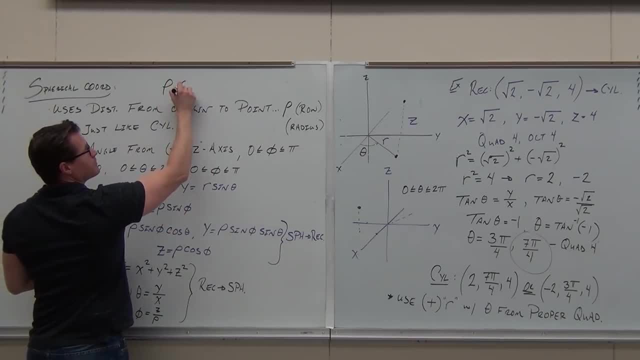 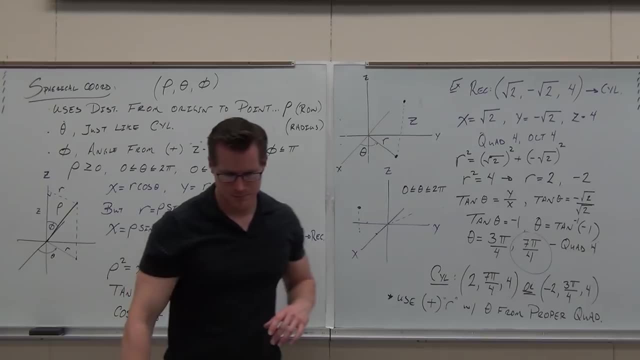 here's how they're written. We've always written rho, then theta, then phi, Rho, theta phi. If I was writing a rectangle, I would have written a vector, an exponential or non-dimensional vector. I do this with a vector. 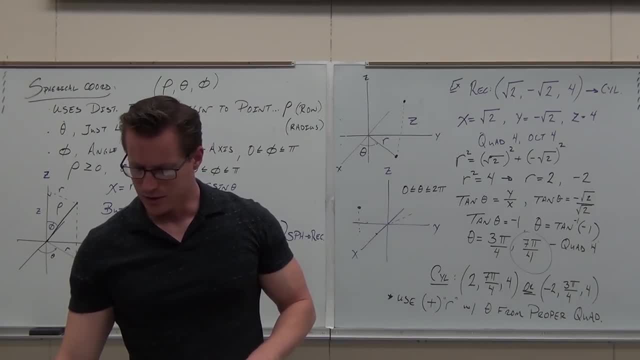 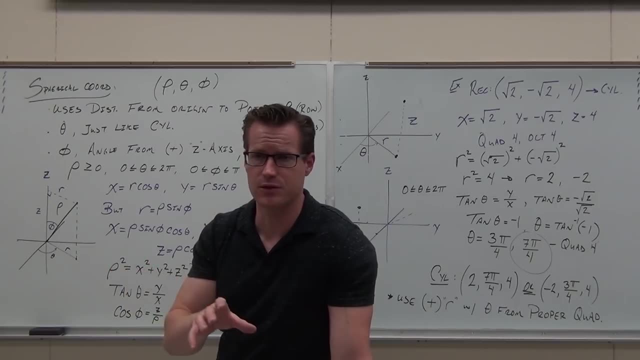 I'll tell you again. I'll tell you what we're going to do. We're going to do two examples: We're going to translate from spherical to rectangular. We're going to translate from rectangular to spherical. We're going to take our break. 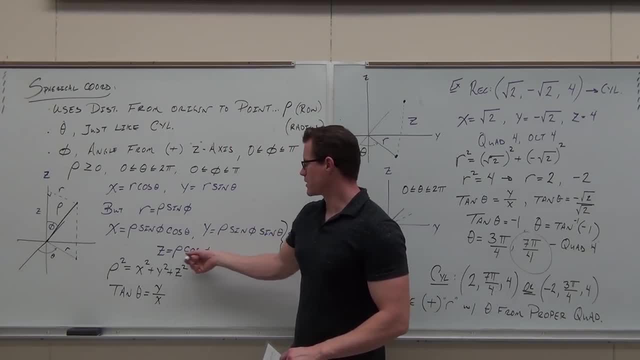 The only other one is this one: If we use this and solve for cosine theta, we're going to get the same thing. If we use cosine phi, we're going to have z over rho, and that's the way we get back to our phi. 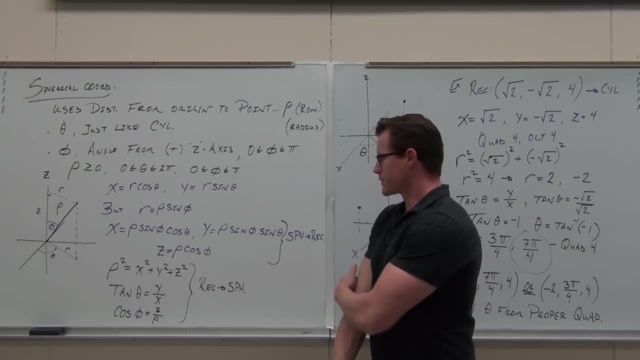 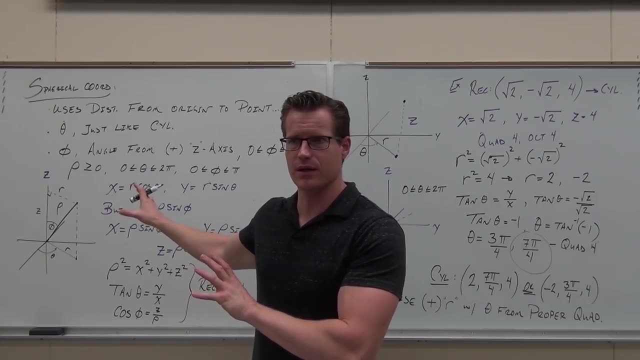 And that's how we're going to go back from rectangular to spherical. The examples are actually pretty quick, but I want to make sure that you guys understand at least the idea of what these look like. If not, if you do, you feel okay with that one. 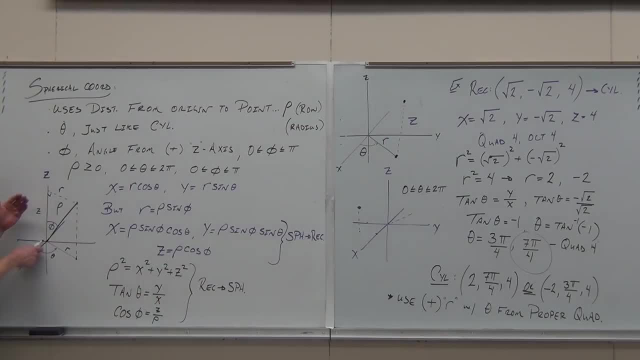 So the way spherical works. again, it still has this theta, It no longer has a z, It's got a distance straight from origin to point, and it has other angles telling us our aspect from the positive z axis. All of the spherical coordinates are written in this format. 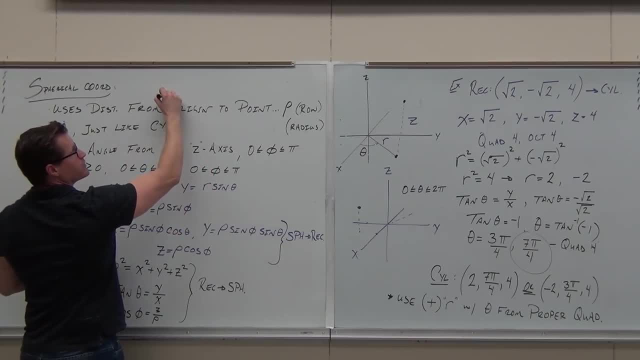 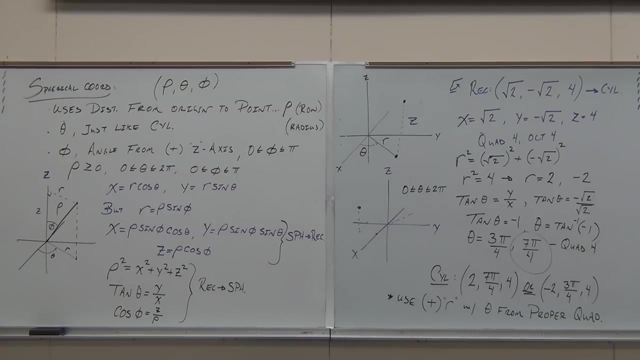 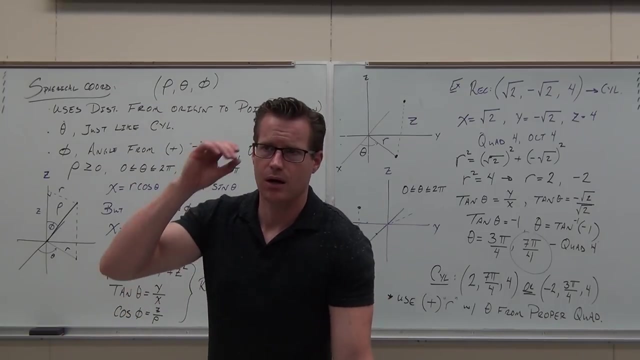 Now that we understand all this stuff, here's how they're written. We've always written rho, Then theta, then phi, rho, theta, phi. Tell you what we're going to do. We're going to do two examples. We're going to translate from spherical to rectangular. 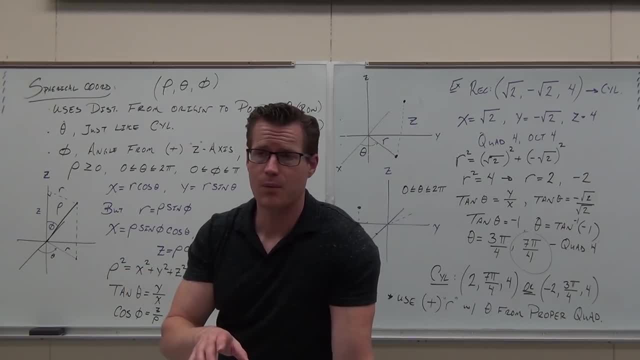 We're going to translate from rectangular to spherical. We're going to take a break and when we come back we're going to do some special ones. We're going to translate from stuff like cylindrical to spherical or spherical to cylindrical. It actually gets easier. 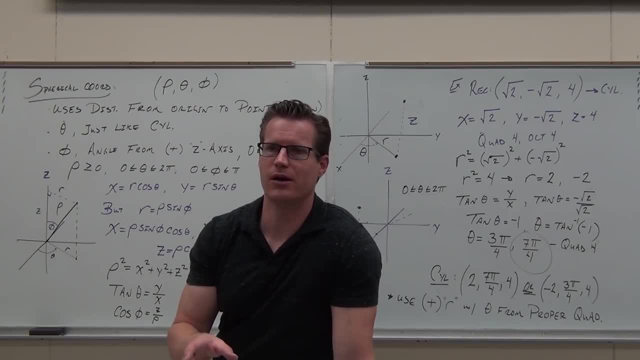 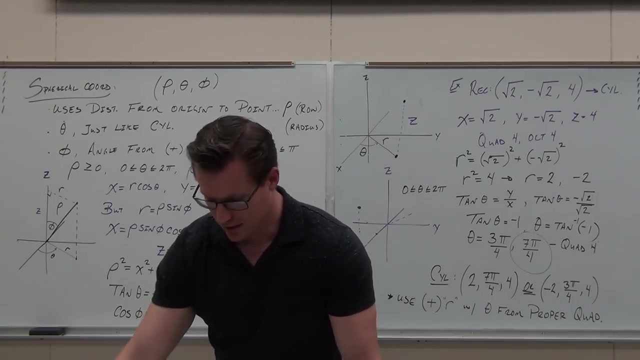 It's not harder, It's easier. And then we're going to start talking about translating some of these equations from like rectangular to you know, spherical stuff- America, booyah, I don't know. We're going to do that. So after we get back we'll do some of that stuff. 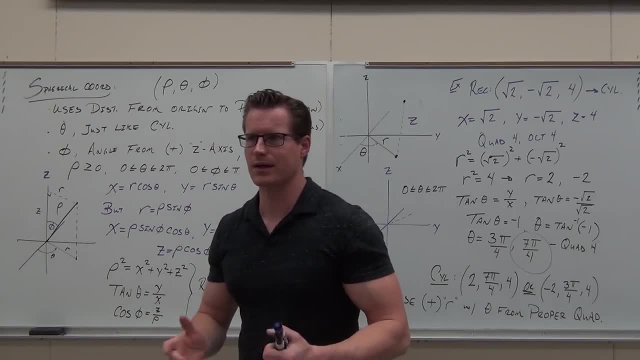 It's not hard. You just got to be a little clever sometimes. So we'll talk about how to be clever with equations. Would you like to do a couple of these, at least twice? You know one from one way, other way. 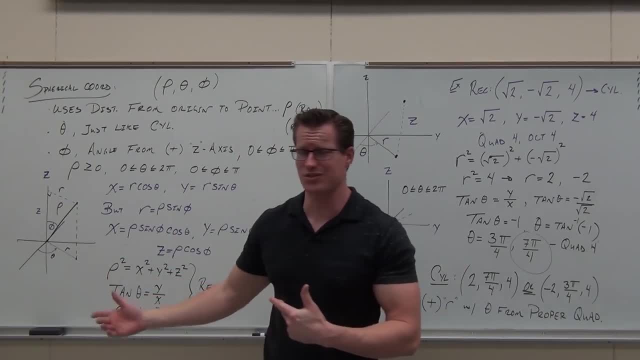 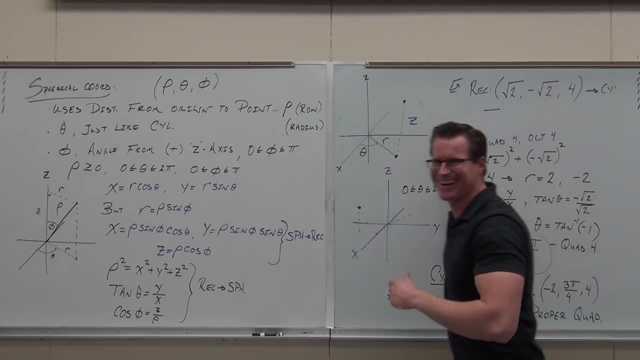 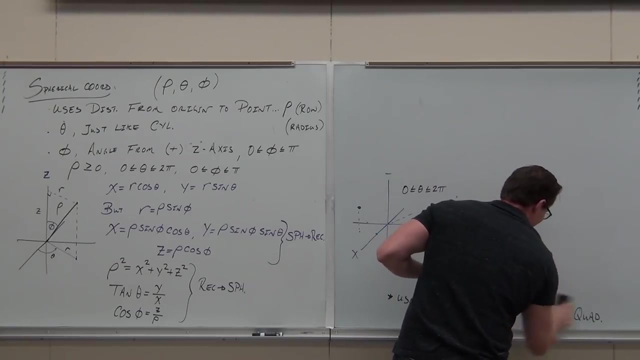 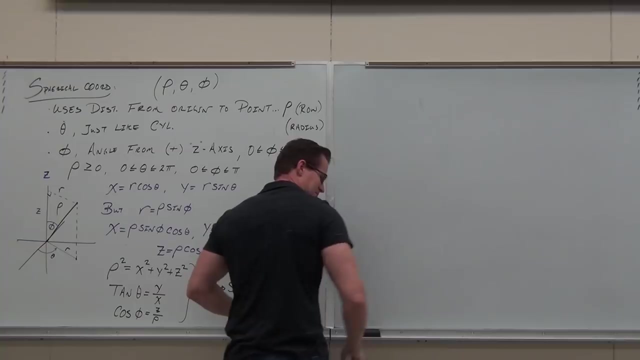 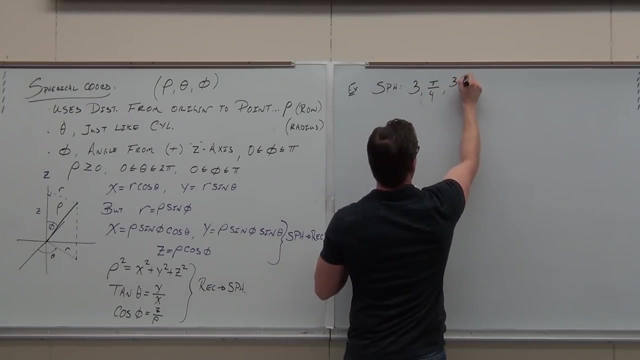 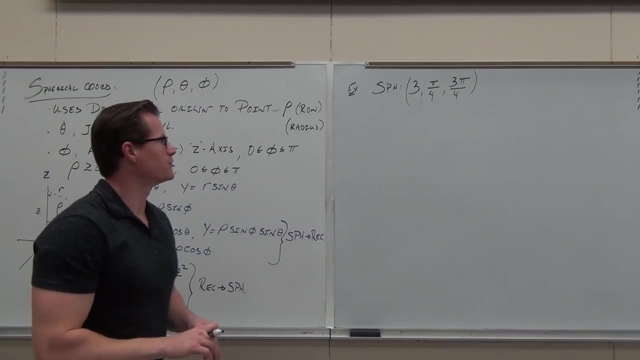 Then we'll make it fun when we get back. It's going to go quicker because I don't have to explain anything. It's just working through it. So that would be nice for me. That's what really matters, right? You know, these can be a little challenging for some people. 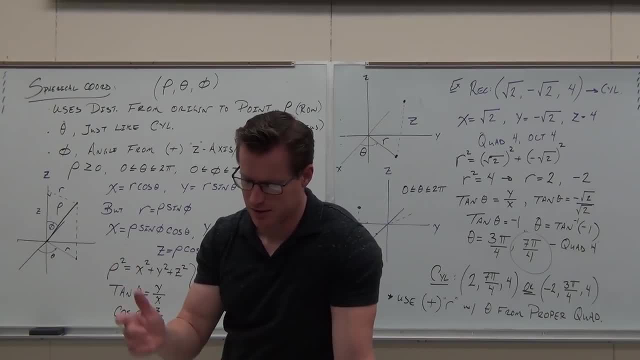 and we come back and we're going to do some special ones. We're going to translate from stuff like cylindrical to spherical or spherical to cylindrical. It actually gets easier. It's not harder, It's easier. And then we're going to start talking. 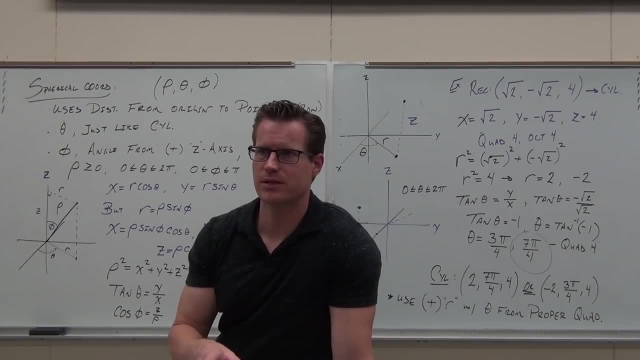 about natural pixels. We're going to do some empirical. We're going to start talking about translating some of these equations from like rectangular to you know, spherical stuff, America, Booyah, I don't know. we're going to do that. 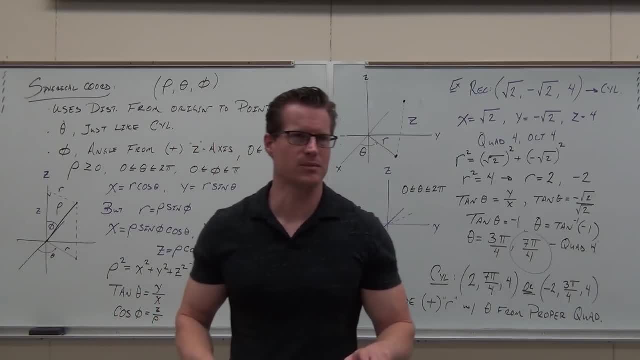 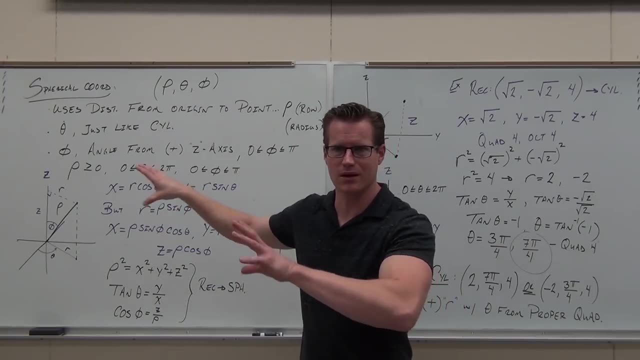 So after we get back we'll do some of that stuff. It's not hard, you just got to be a little clever sometimes. so we'll talk about how to be clever with equations. Would you like to do a couple of these, at least twice? you know one from one way, other. 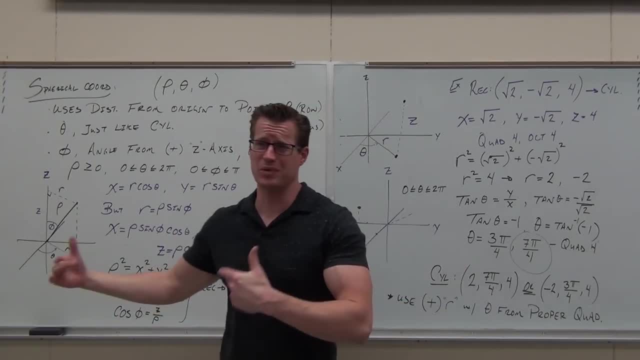 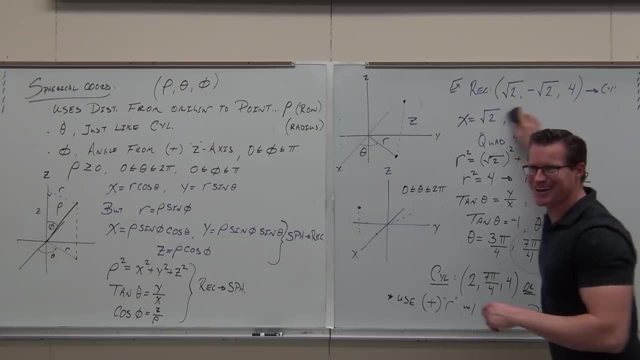 way. then we'll make it fun when we get back. It's going to go quicker because I don't have to explain anything. it's just working through it, So that would be nice for me. that's what really matters, right. 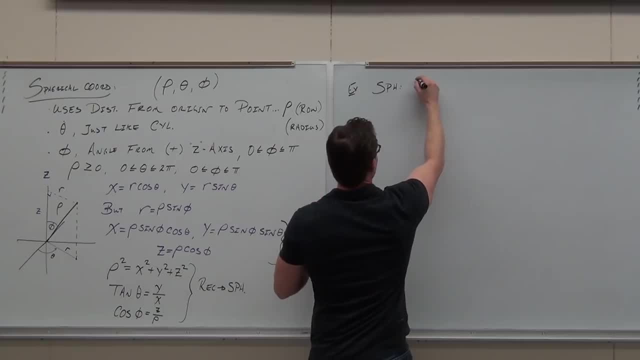 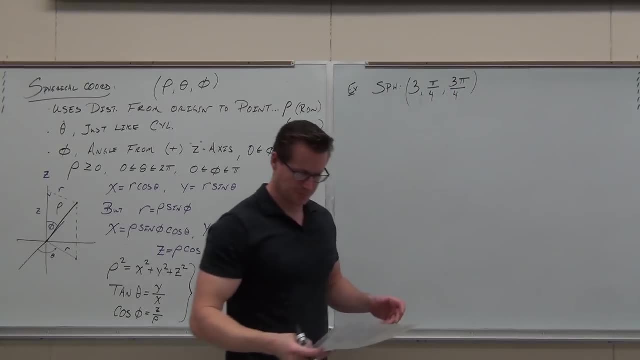 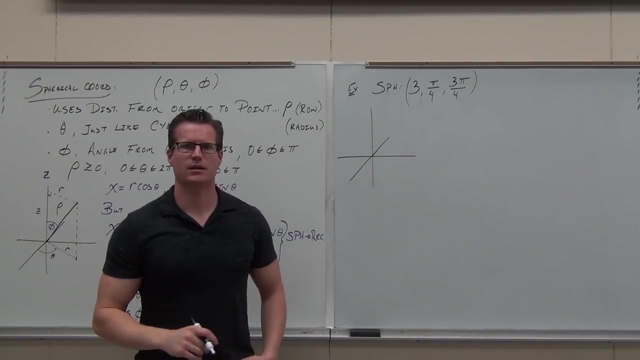 You know, these can be a little challenging for some people to visualize what's going on. So when we take a look at where this is, again, you got to have a picture of where this guy is- quadrant wise, octant wise- before we get going. 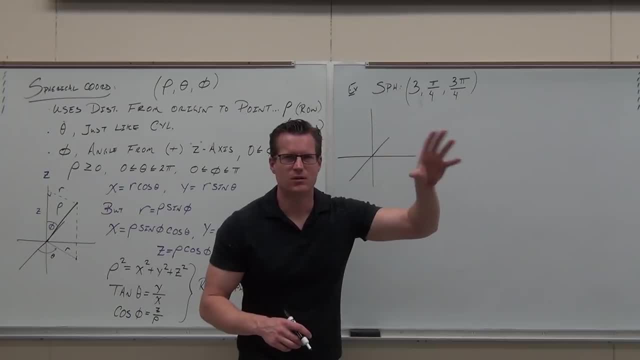 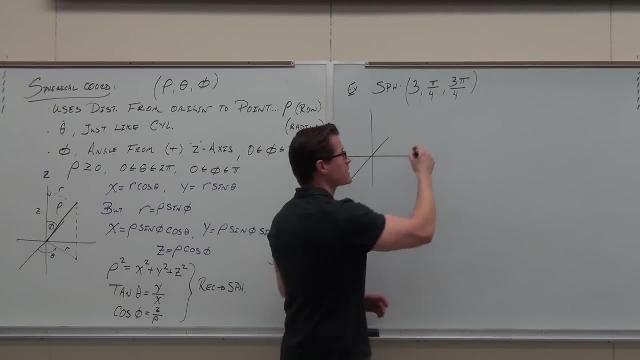 So what do these things mean? what's the three? come on quickly. what's the three mean? what is that? If this is in spherical, which I have to tell you that? what is the three? What's this one? is that phi or is that theta? what is that one that is theta? 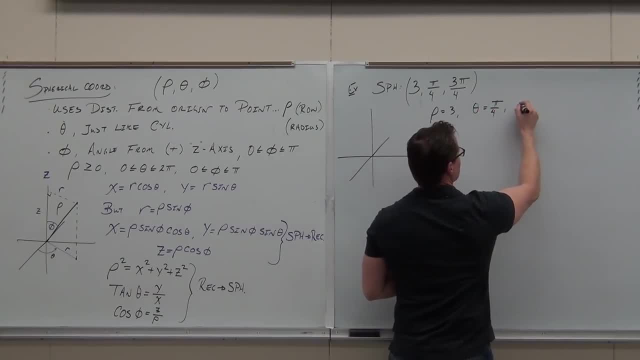 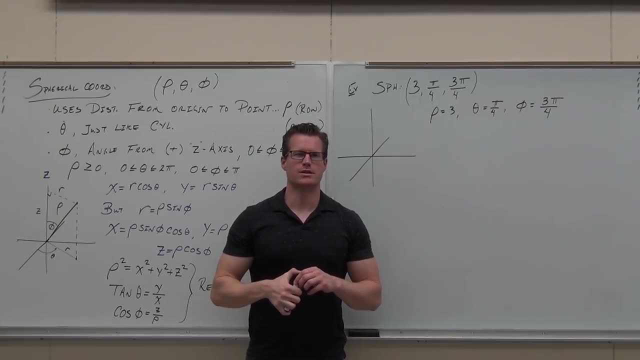 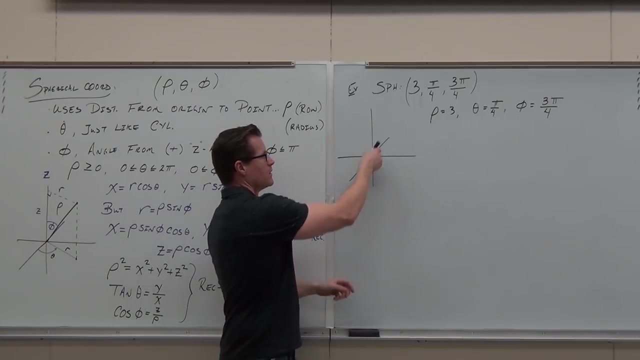 Okay, check it out. I want you to visualize this. If your row is three, that means I'm coming out. I've got a radius of three. so let's imagine it this way. What's the theta going to do? is it going to move it this way- negative, or this way positive? 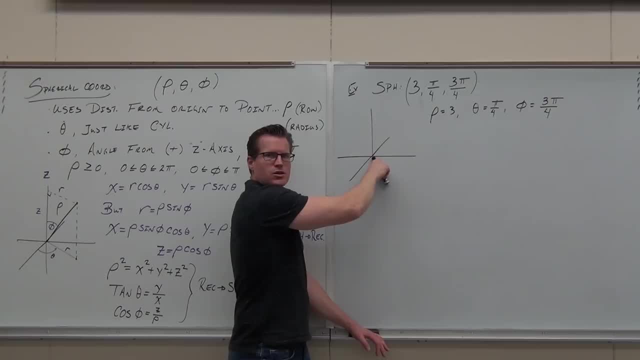 So it's going to put it right here. do you guys see that? So that's in quadrant, what One? Okay, but now I also have that phi saying from the positive z-axis: I'm coming down here: three pi, stop me. stop me when I get three pi over four. so I'm coming down here. 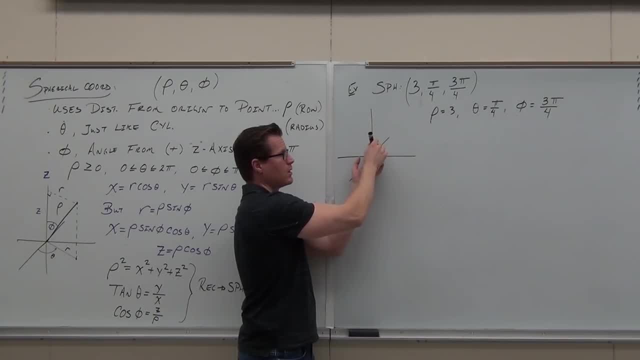 how much about is that? Pi over four? It's like pi over four. What would it be on the xy-plane? It would be pi over two And if I keep on going I'm going to be at three- pi over four, if I get all the way. 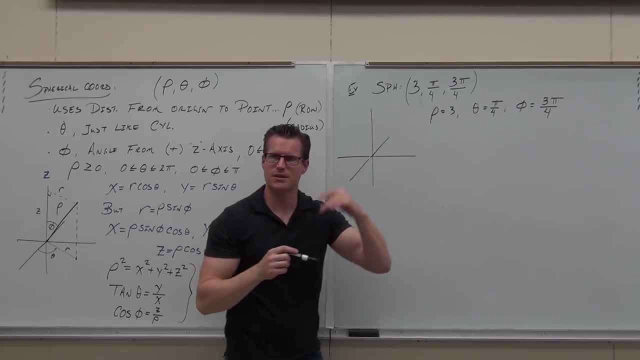 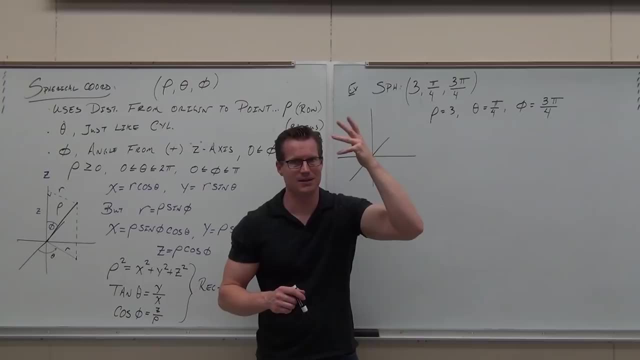 down here. that would be pi. does that make sense? Can you visualize that? this thing is below the xy-plane? I guarantee you any phi value legitimate this and you're in it. you're going to get it in your head here. any phi value past pi over two is going to give you a negative. 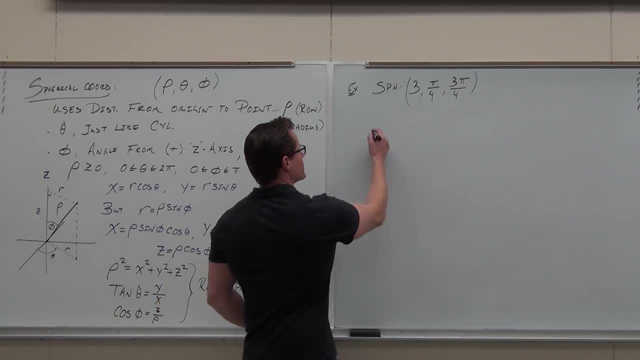 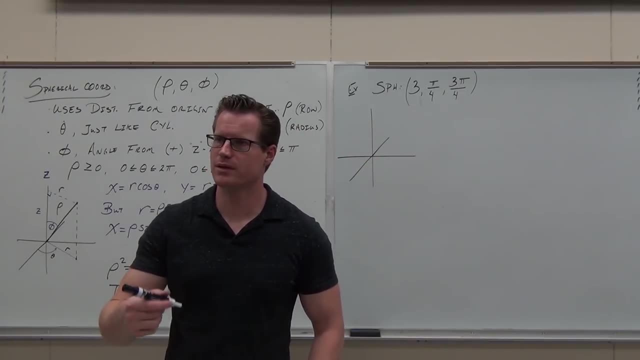 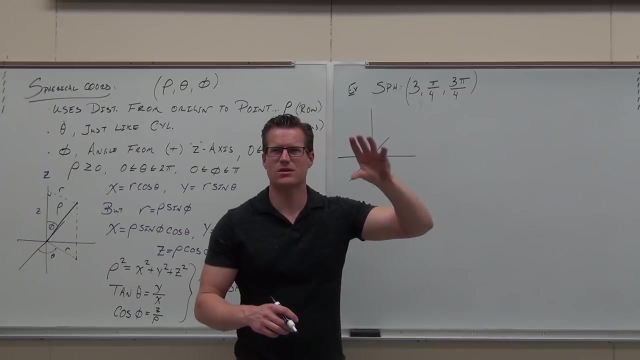 to visualize what's going on. So when we take a look at where this is, again, you got to have a picture of where this guy is- quadrant-wise, octant-wise- before we get going. So what do these things mean? What's the three? 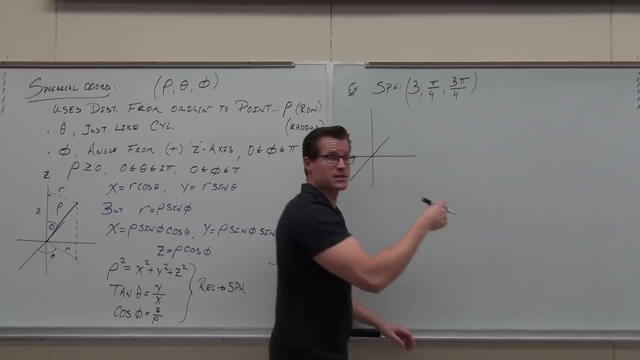 Come on quickly. What's the three mean? What is that? If this is in spherical, which I have to tell you that. what is the three? What's this one? Is that phi or is that theta? What is that one? 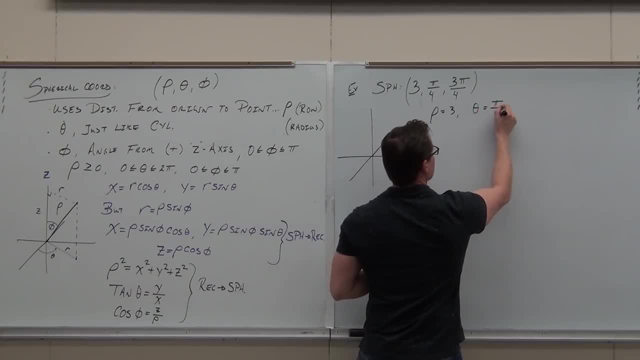 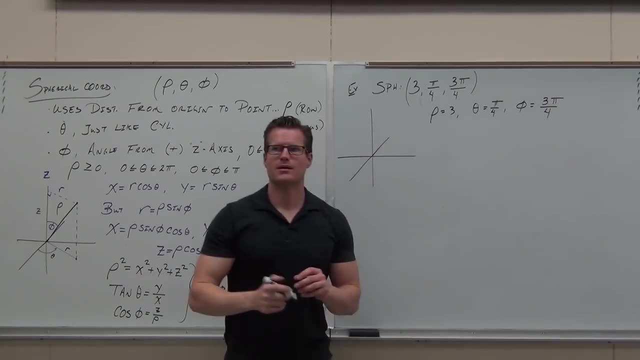 Theta. That is theta. Okay, check it out. I want you to visualize this: If your row is three, that means I'm coming out. I've got a radius of three. I've got a radius of three. So let's imagine it this way. 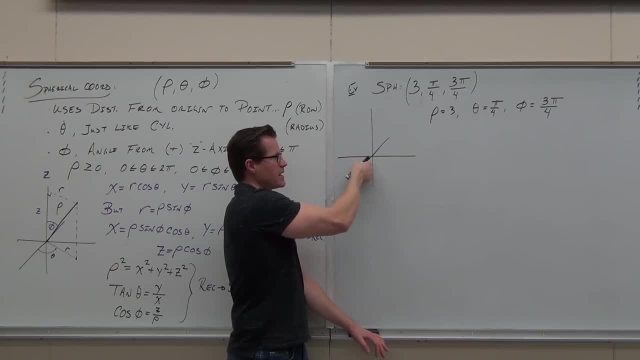 What's the theta going to do? Is he going to move it this way negative or this way positive? So it's going to put it right here. Do you guys see that? So that's in quadrant. what One. Okay, But now I also have that that. 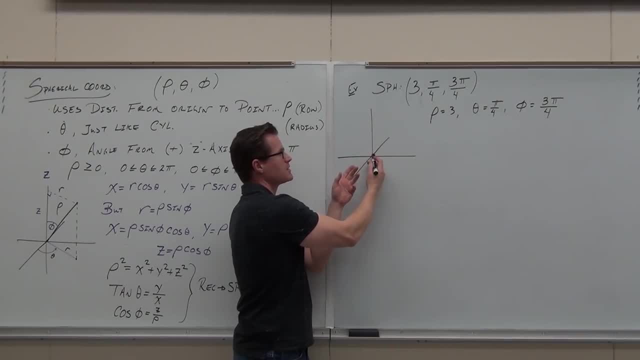 that phi. Okay, So I'm going to put it right here. Okay, So it's going to be saying: from the positive z axis, I'm coming down here: three pi, stop me. Stop me when I get to three pi over four. 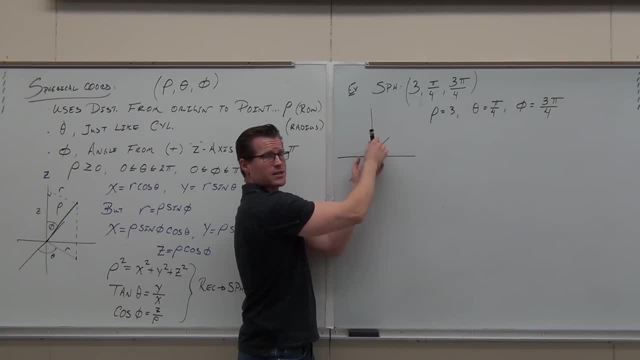 So I'm coming down here: How much about is that? Pi over four. It's like pi over four. What would it be on the xy plane? Maybe Pi over two, Maybe pi over two, Pi over two, And if I keep on going I'm going to be at three: pi over four. 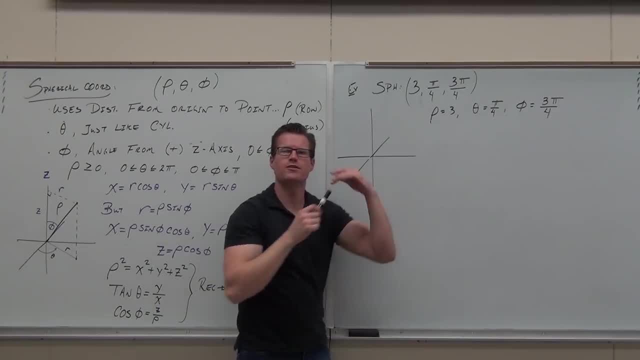 If I get all the way down here, that would be pi. Does that make sense? Can you visualize that this thing is below the xy plane? I guarantee you any phi value. legitimate this in your head here. any phi value past pi over 2 is going to give you a negative z. 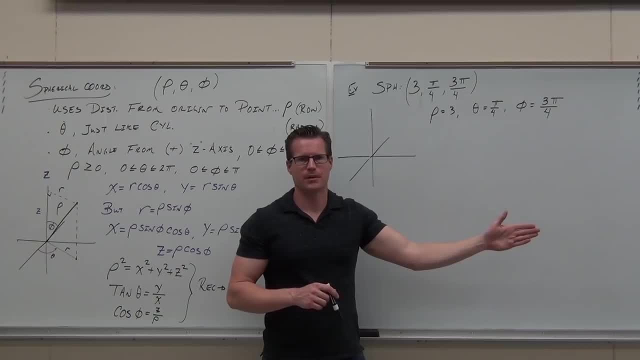 Do you guys see that At pi over 2, you're on the xy plane. Past that negative z Before that positive z. Past pi you can't, You can't. Does that make sense to you? Visualizing it helps a lot. 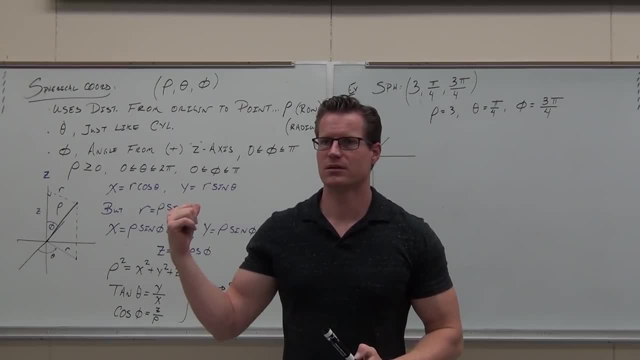 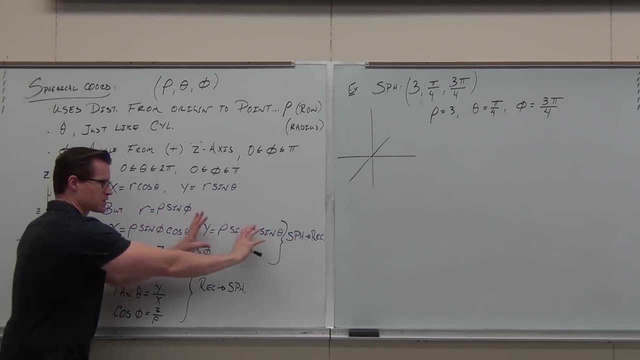 Let's go ahead. Do you guys want to try it? Do you want to try changing that to rectangular? We have some stuff that shows us what to do If I want to go from spherical to rectangular. we're going to plug this stuff in. 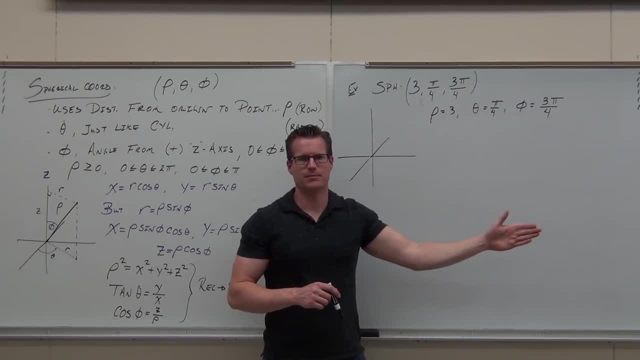 z. Do you guys see that At pi over two you're on the xy-plane. Past that negative z before that positive z past pi you can't, you can't. does that make sense to you? Visualizing it helps a lot. 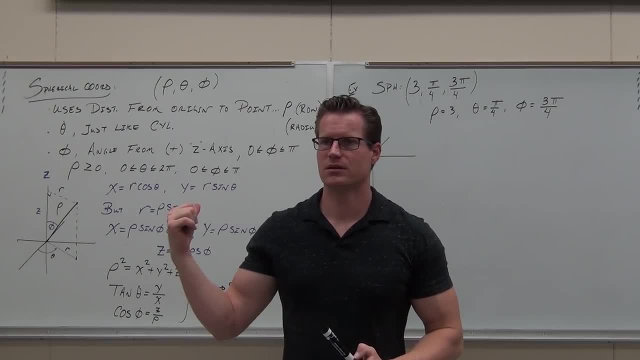 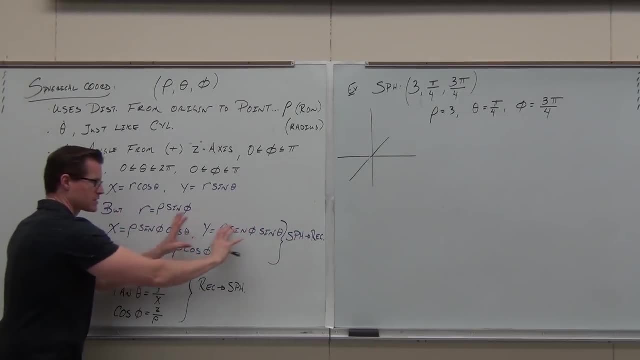 Let's go ahead. do you guys want to try it? do you want to try changing that to rectangular? We have some stuff that shows us what to do if I want to go from spherical to rectangular. we're going to plug this stuff in. 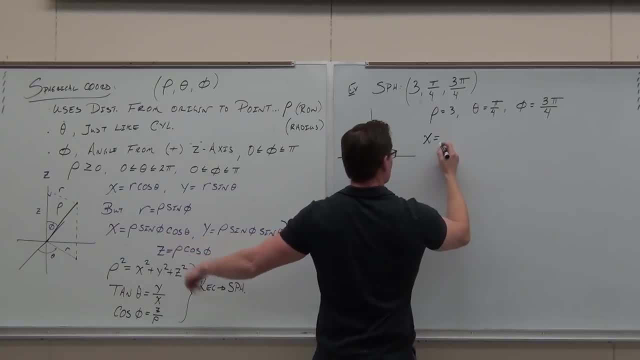 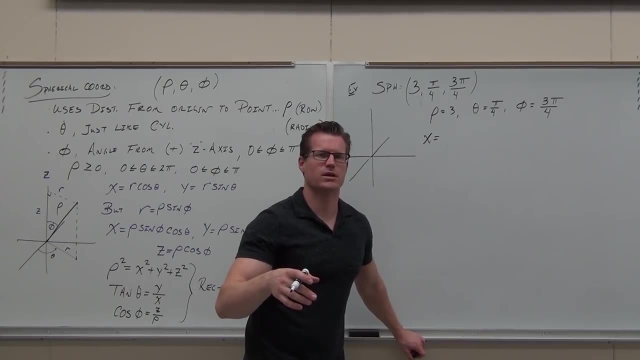 So x equals. well, you know what we'll do one, we'll do the x together. I'll give you the y and the z on your own. What's the first number I should plug in if I'm doing x? 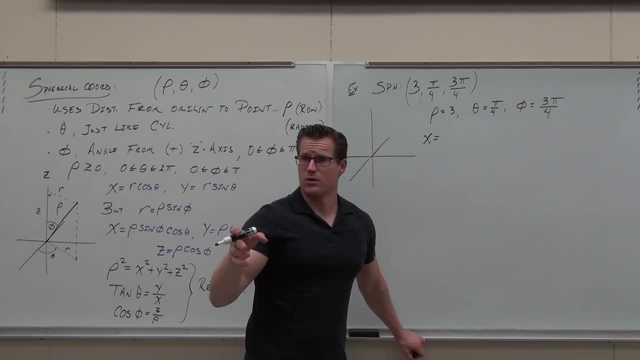 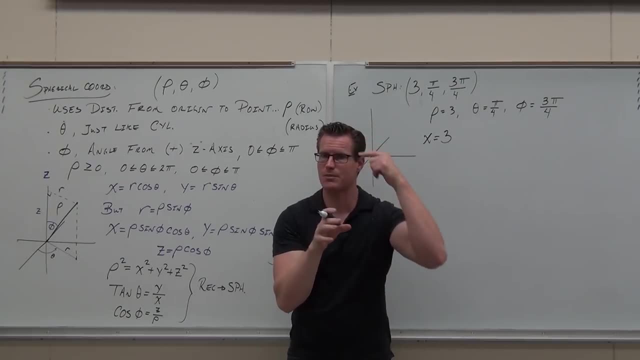 What is it? Three? Three, because the row is three. And then x says: well, x is r cosine theta. I know that's what x is. so in my head I'm thinking: okay, r is row. well, r is row sine. 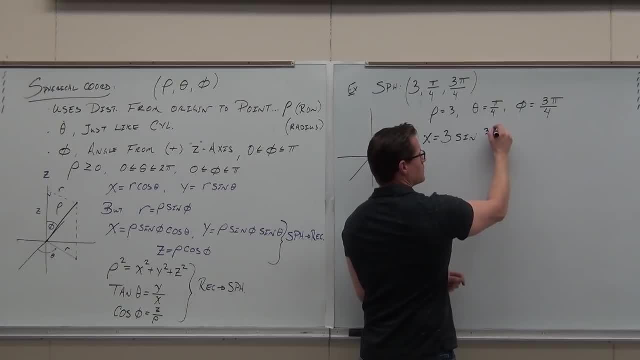 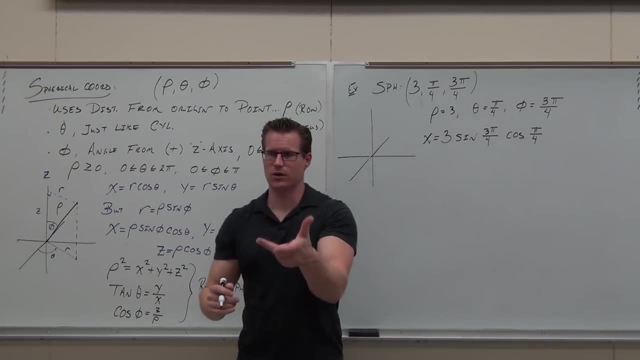 phi, Okay, Okay. But then I have to have that cosine theta because x is r cosine theta. I've got to have a cosine theta up there somewhere because I'm talking about x. You guys see what I'm talking about now. that's how I memorize it, so I can. I can always. 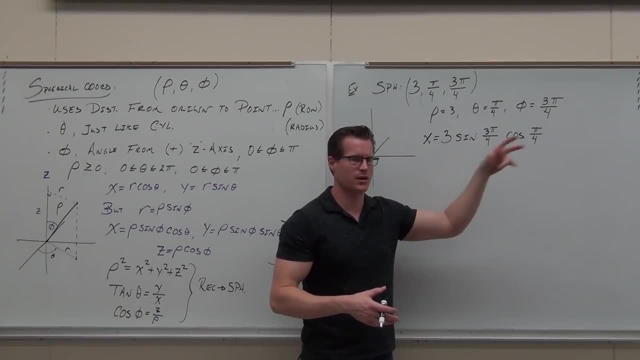 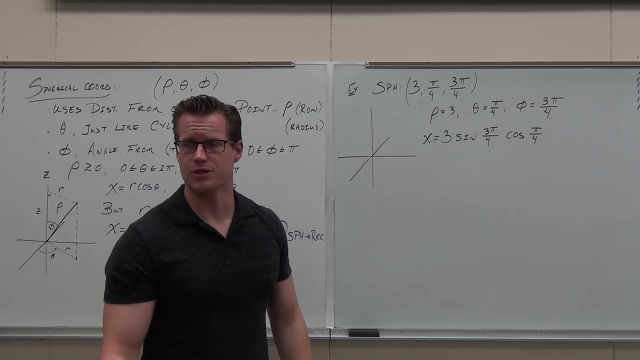 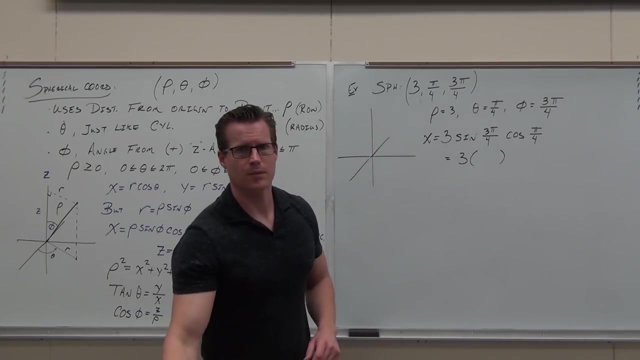 get that cosine for x. I want that in my head. cosine theta for x. You sure you're okay with that one? Are you at all good at your unit circle stuff? Yes, Perfect. Sine of 3pi over 4, all students sine has to be positive 3pi over 4, it's root 2 over. 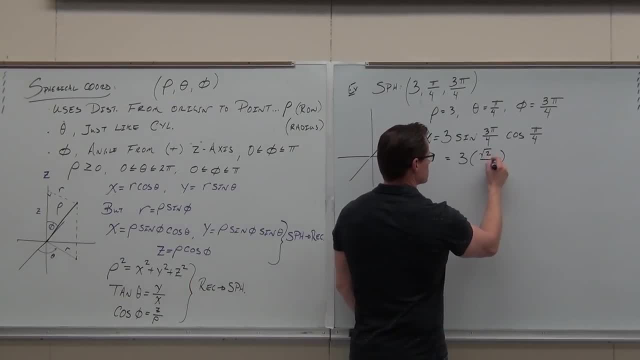 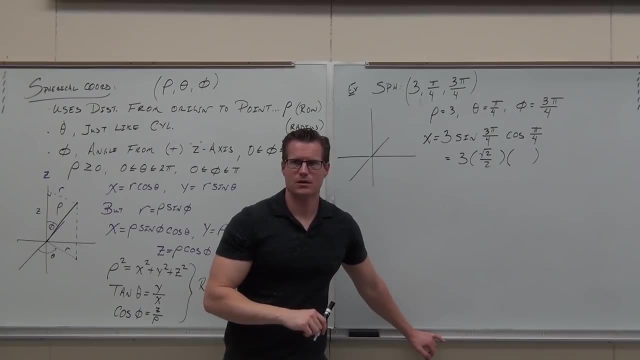 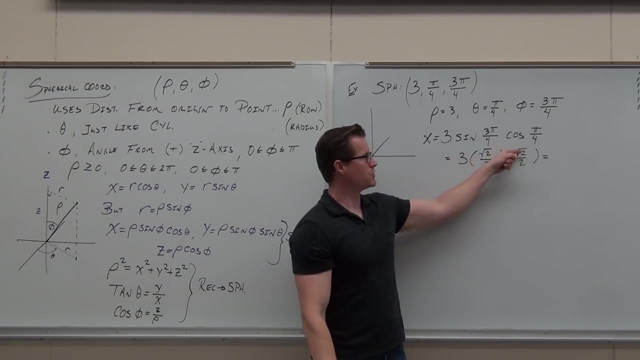 2. Cosine pi over 4, cosine pi over 4, that's in the first quadrant root 2 over 2. Which means that we get 2 over 4, that's 1 half times 3, looks like we get 3 halves. 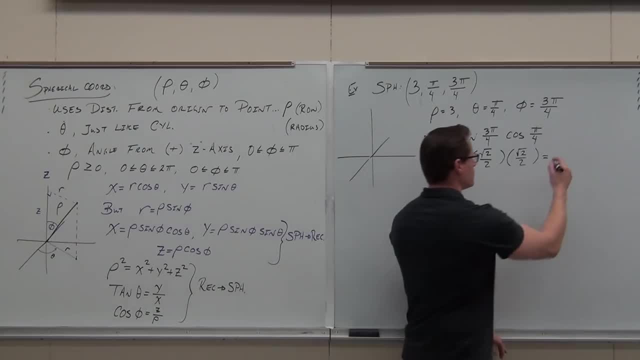 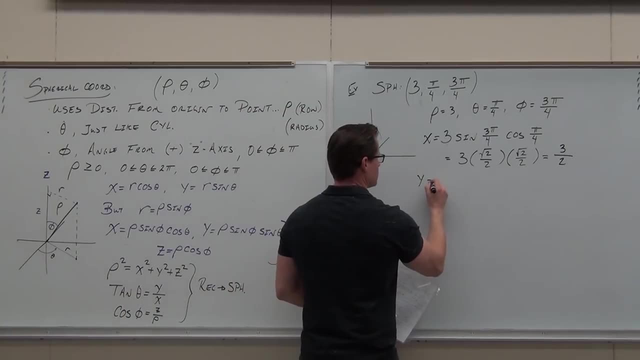 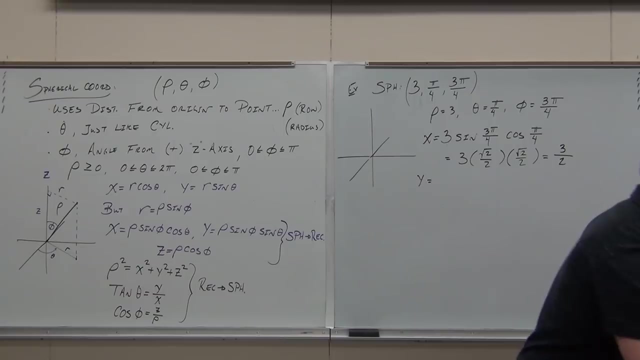 can I get a double check on that work? 4. 2. OK, All right, let's go. Try the y, try the z, go for it, All right. 3. 3., 3., 3.. 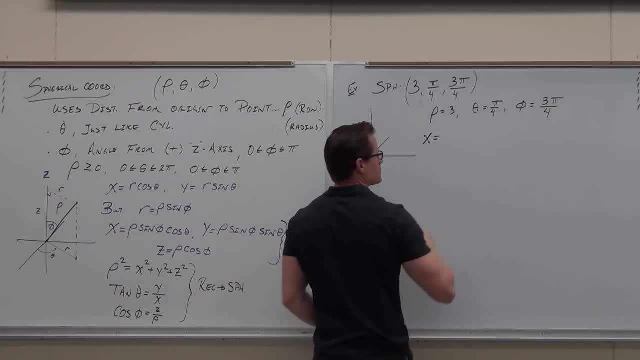 So x equals. well, you know what We'll do: 1. We'll do the x together. I'll give you the y and the z on your own. What's the first number I should plug in if I'm doing x? 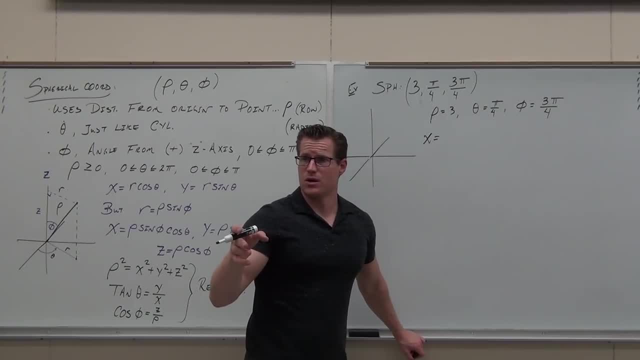 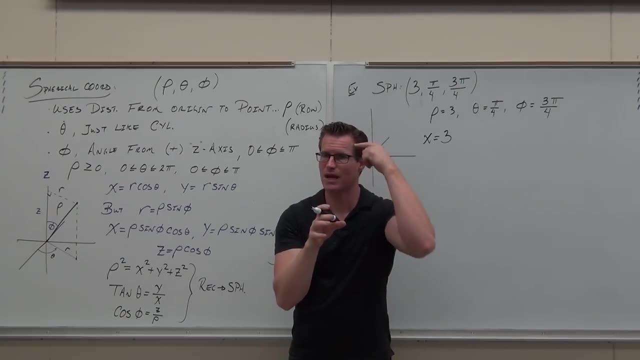 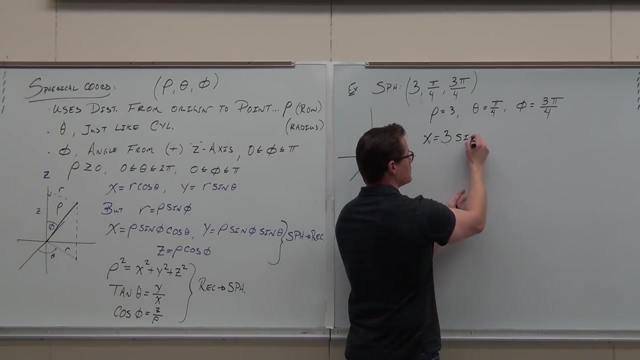 What is it? 3, because the row is 3.. And then x says: well, x is r cosine theta. I know that's what x is. So in my head I'm thinking: Okay, r is row. well, r is row sine phi. 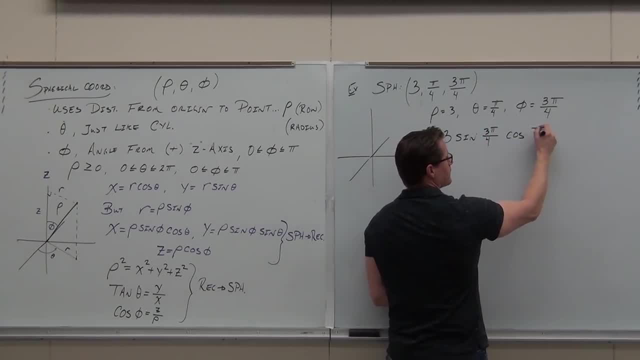 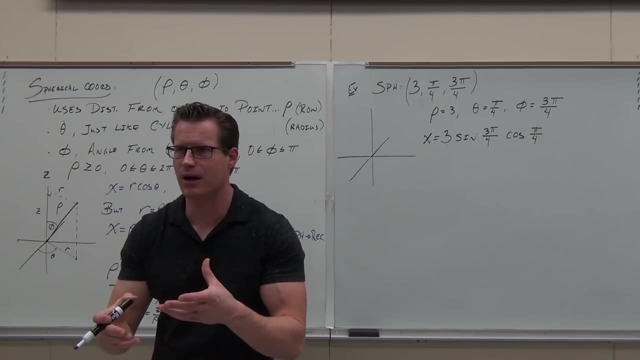 But then I have to have that cosine theta because x is r cosine theta. I've got to have a cosine theta up there somewhere because I'm talking about x. Do you guys see what I'm talking about now? That's how I memorize it, so I can always get that cosine for x. 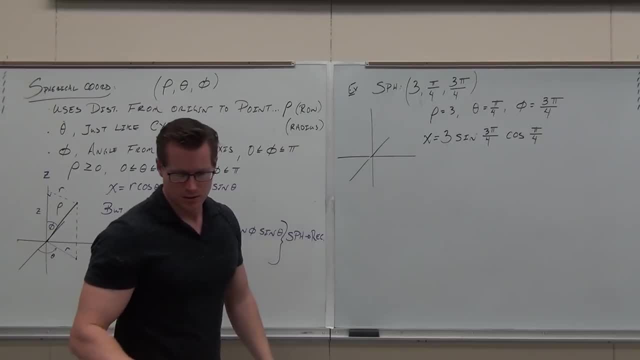 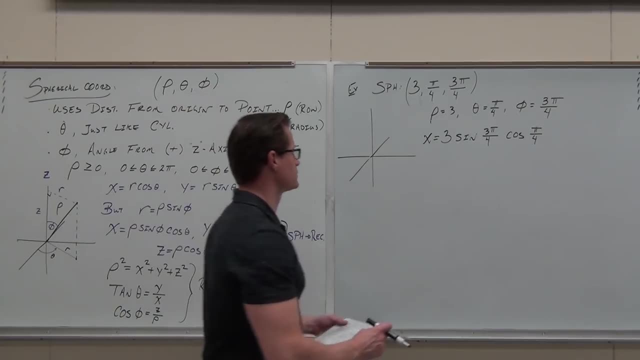 I want that in my head. cosine theta for x. You sure you're okay with that, Are you? Are you at all good at your unit circle stuff? Yes, Sine of 3, pi over 4, all students. sine has to be positive. 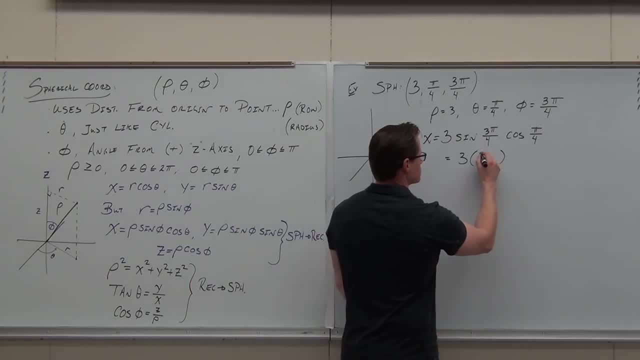 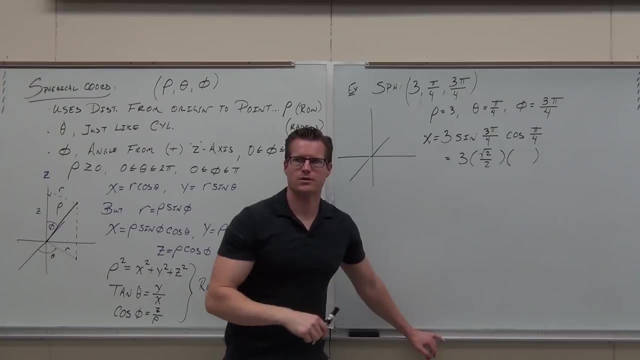 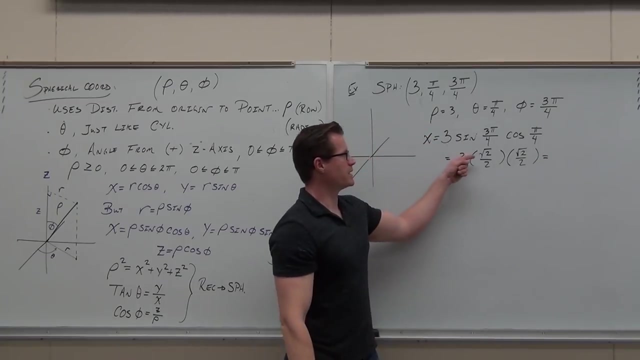 3 pi over 4, it's root 2 over 2.. Cosine pi over 4.. Cosine pi over 4, that's in the first quadrant, Root 2 over 2.. Which means So we get 2 over 4, that's 1 half times 3, looks like we get 3 halves. can I get a double? 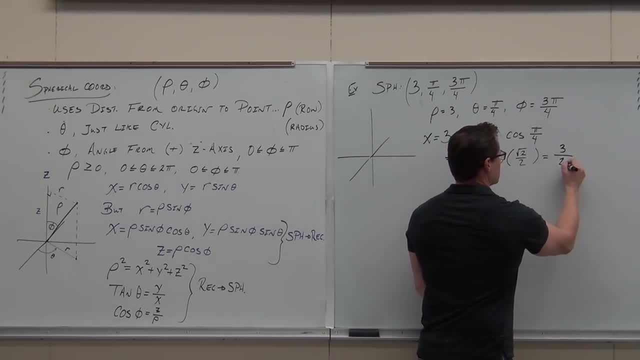 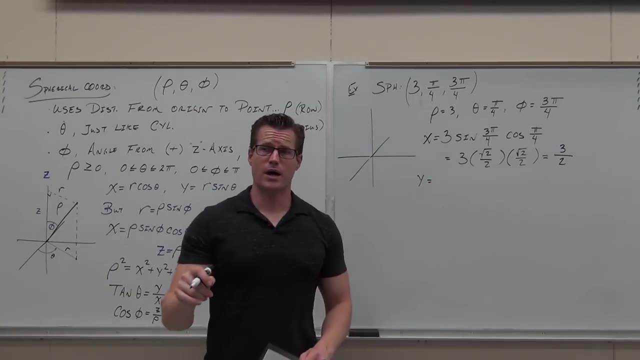 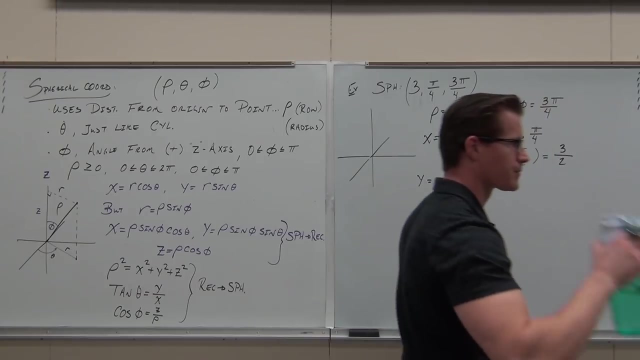 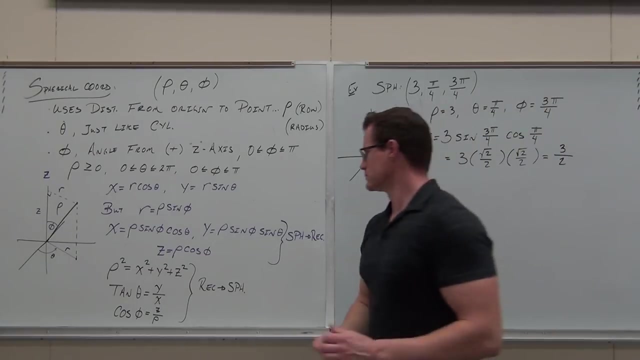 check on that work. Try the Y, try the Z, Go for it. So we get 2 over 4, that's 1 half times 3, looks like we get 3 halves. can I get a double check on that work? 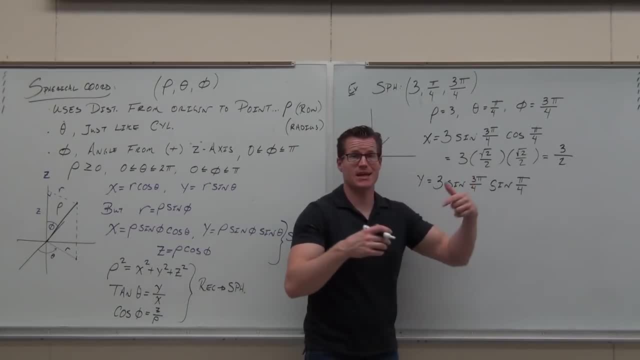 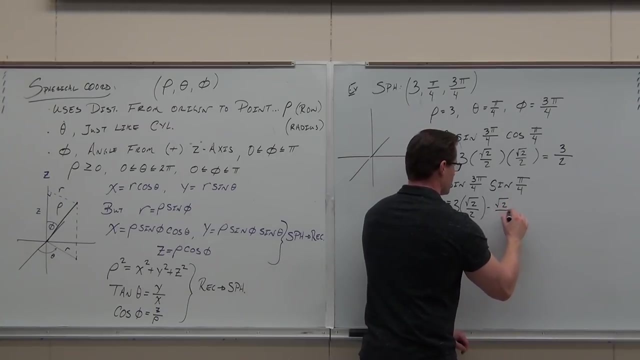 Also. you're going to see this. I mean, hey, it's the same: R right, X is R cosine theta, Y is R sine theta. So you're going to have the same exact thing here and here. take advantage of that. 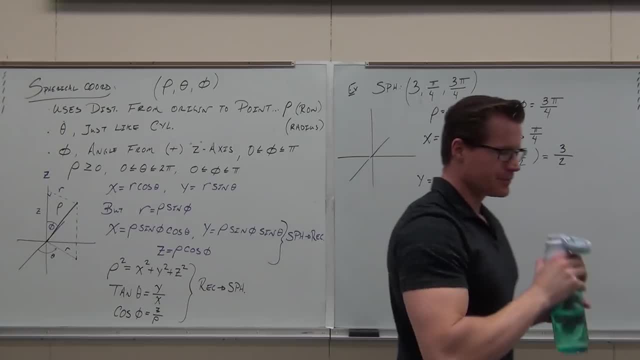 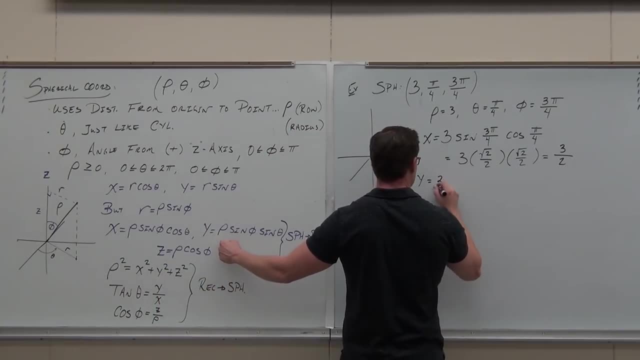 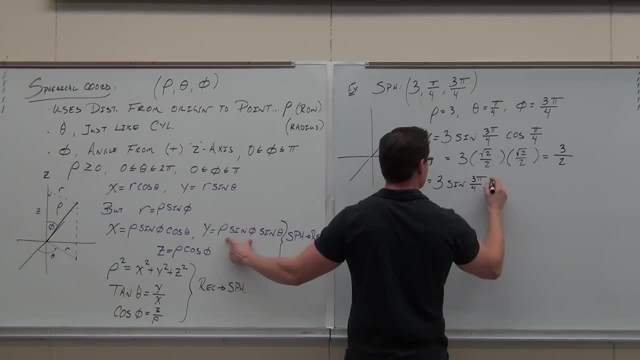 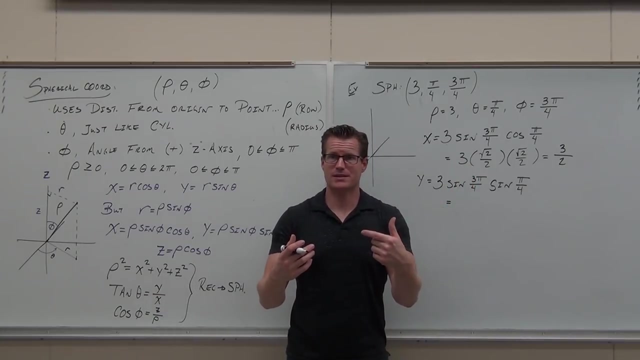 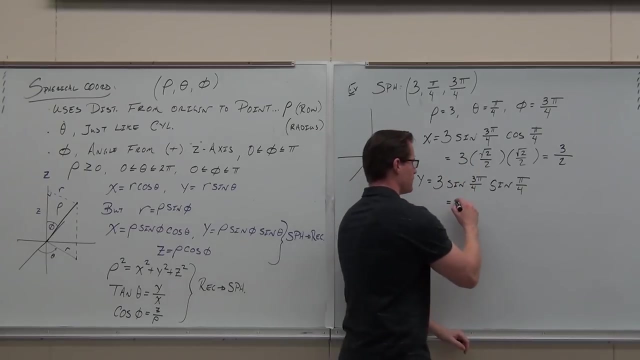 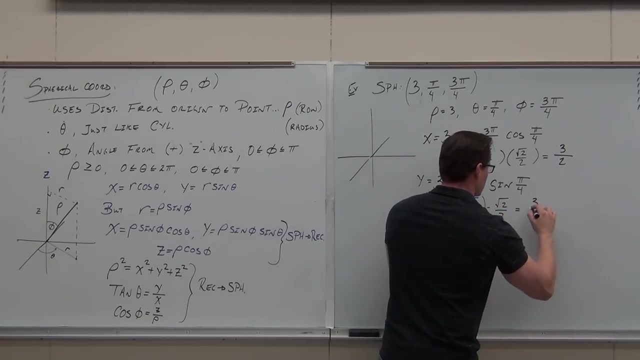 Also. you're going to see this. I mean, hey, it's the same r right, X is r cosine theta, y is r sine theta. so you're going to have the same exact thing here and here. take advantage of that. 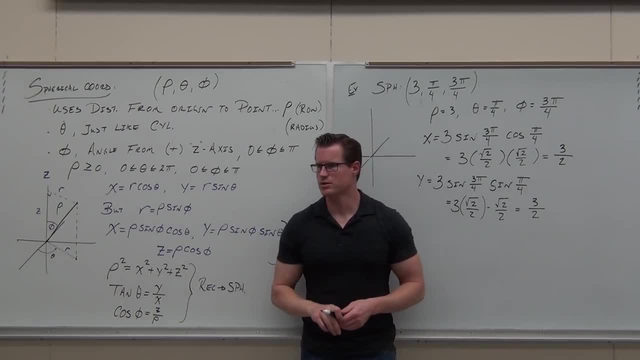 Is it okay to get the same coordinates twice, like x, y? Did you get the same coordinates twice? Did you get three-halves? Still okay with it? Can you find the z? Did you understand that the z has to be negative for sure, like for real? 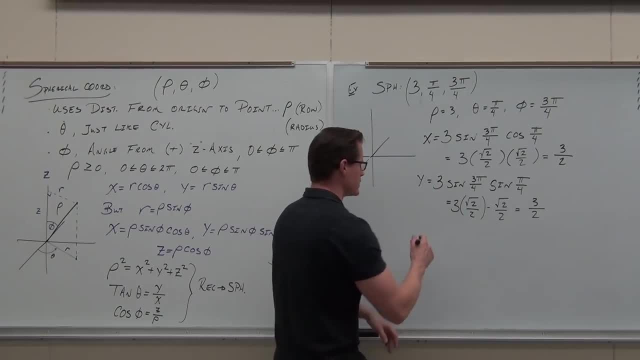 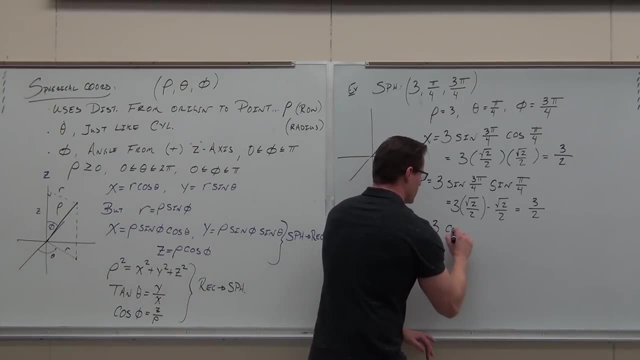 If you're going past pi- over 2, you're going to be below the x y plane. you're going to have a negative z. So z, Z is r and cosine, because that's the adjacent man. I really want this picture in your head. 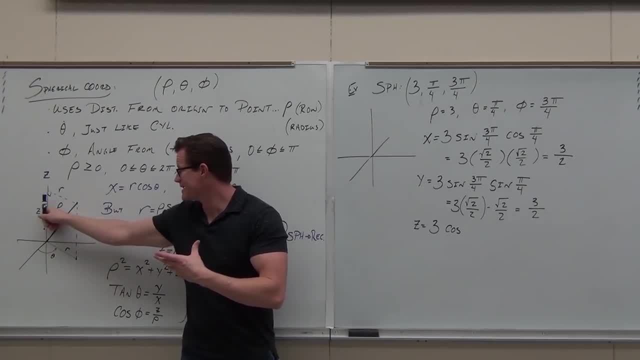 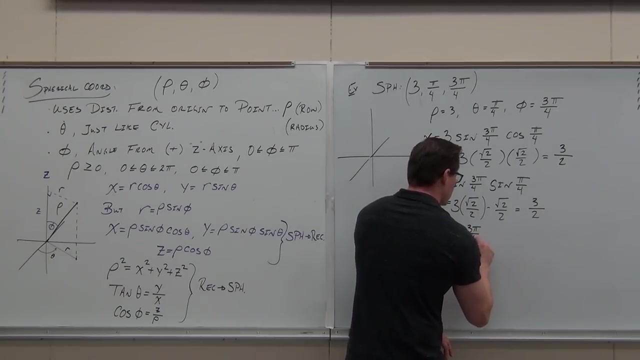 because if it's in your head, you see that the z is part of cosine and it's part of v. You see it? Do you guys see what I'm talking about? Z, the height, it's the cosine part of the v. that's where it's coming from. 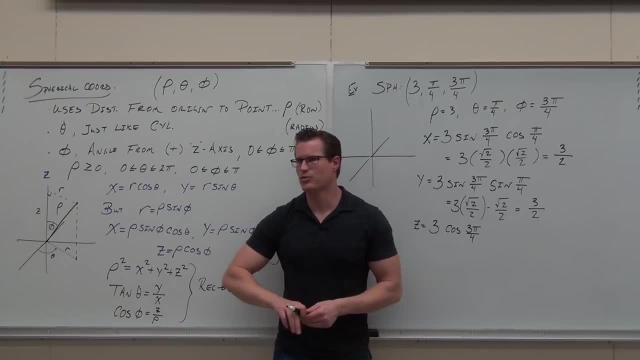 One of the worst things is to have to do a test and do all this stuff And really not get it, And you're just, oh man, my formulas. where's my formulas? What's going on? I lost my formulas, oh crap. 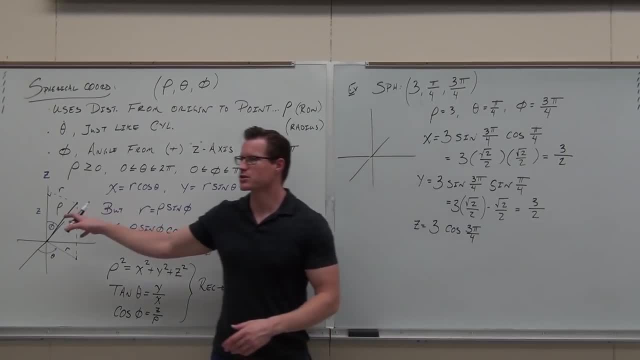 If you get the picture like, you understand how cosine and sine works, you can recreate this stuff And it becomes easier. It becomes easier going. hey, yeah, I actually get it. Cosine relates, cosine phi relates z with rho. 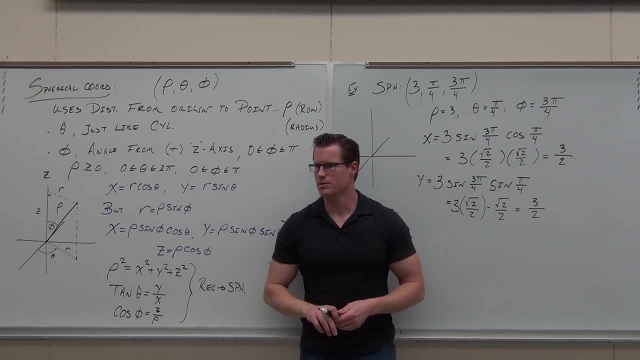 Is it okay to get the same coordinates twice, like X, Y? Did you get the same coordinates twice? Did you get 3 halves? Still okay with it? Can you find the Z, Z? Did you understand that the Z has to be negative for sure, like for real? 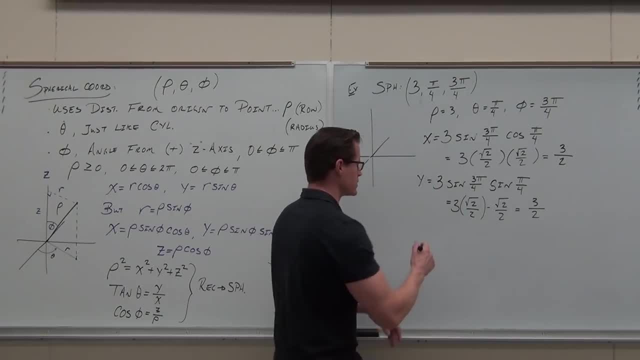 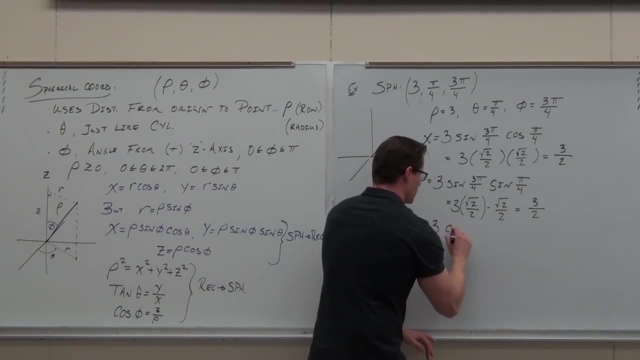 If you're going past pi- over 2, you're going to be below the X Y plane. you're going to have negative Z. So Z is R and cosine, because that's the adjacent man. I really want this picture in your head. 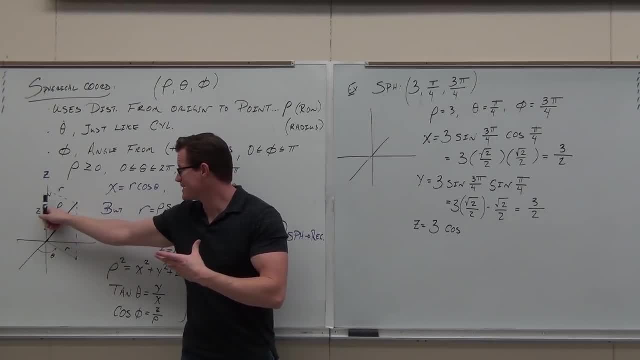 because if it's in your head, you see that the Z is part of cosine and it's part of V. You see it? Do you guys see what I'm talking about? Z, the height, it's the cosine part of the V. That's where it's coming from. 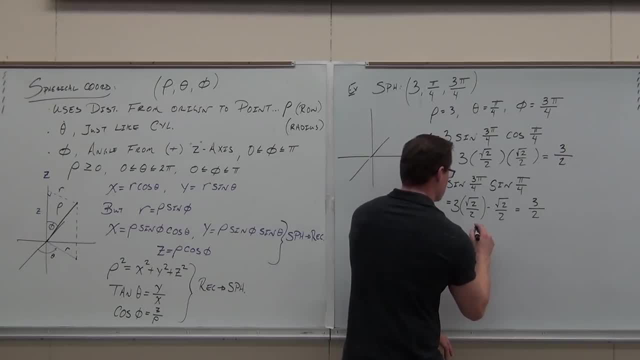 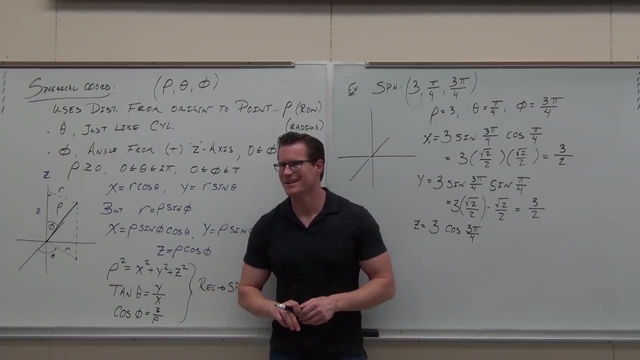 One of the worst things is to have to do a test and do all this stuff and really not get it, and you just, oh man, my formulas. where's my formulas? what's going on? I lost my formulas, oh crap. 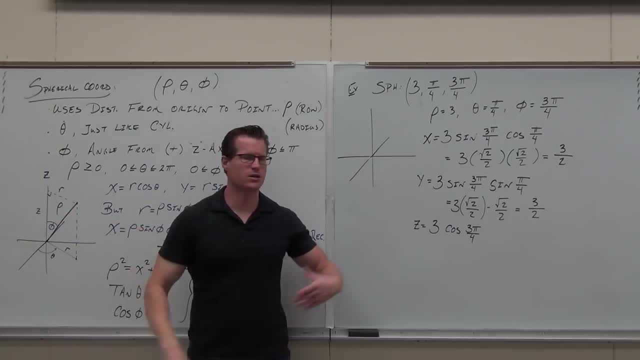 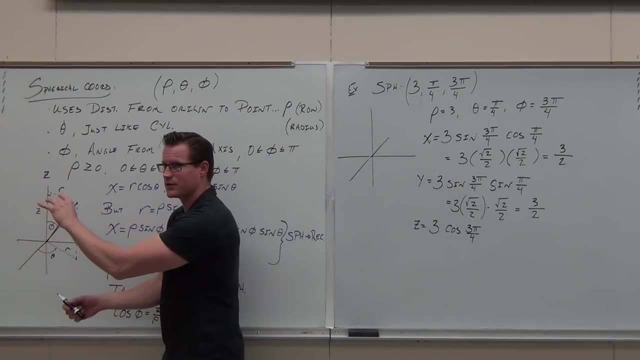 If you get the picture like, you understand how cosine and sine works, you can recreate this stuff and it becomes easier. It becomes easier going. oh yeah, I actually get it. Cosine relates cosine, V relates Z to cosine. That's where it's coming from. 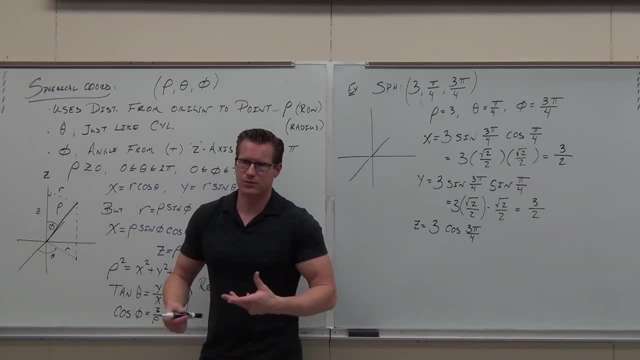 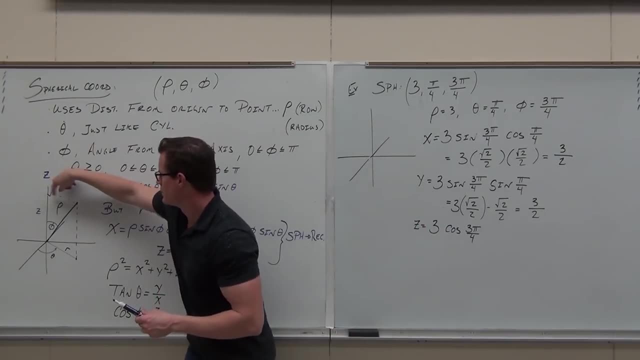 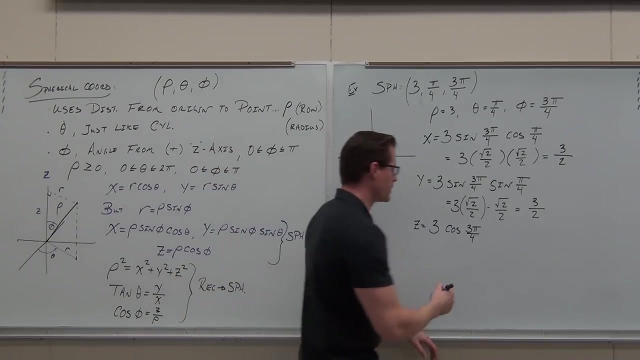 That's where it's coming from. Z with rho, oh then Z. I can get rho, cosine of V. That makes sense. Sine sine relates R with rho and V. That's how these formulas are created. They're in your head. you understand it better. 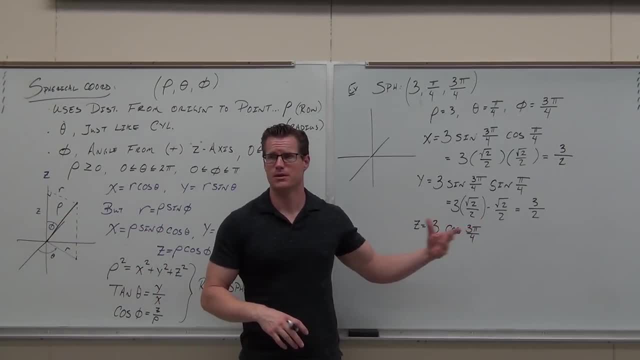 Oh Then z I can get rho cosine of phi. That makes sense. Sine sine relates z with rho. Oh Then z I can get rho cosine of phi. That makes sense. Sine, Sine, Sine. 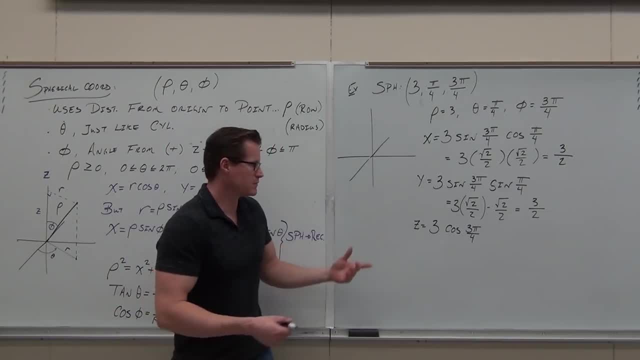 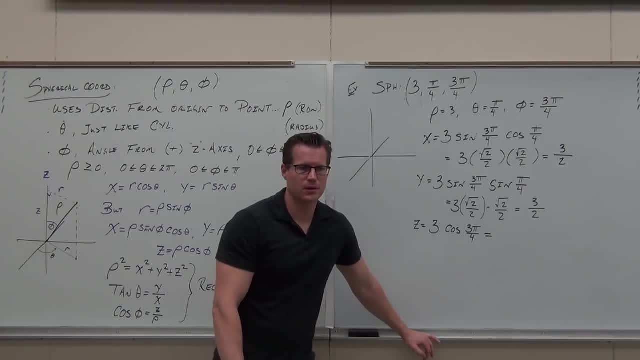 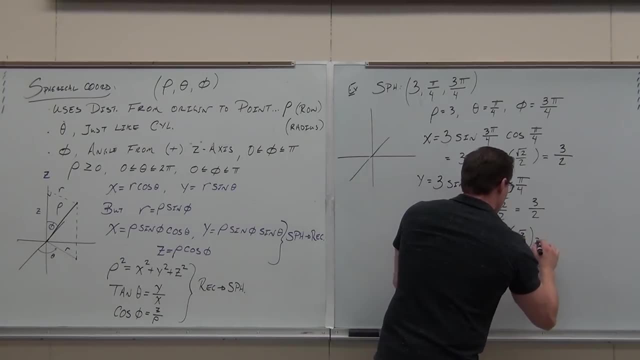 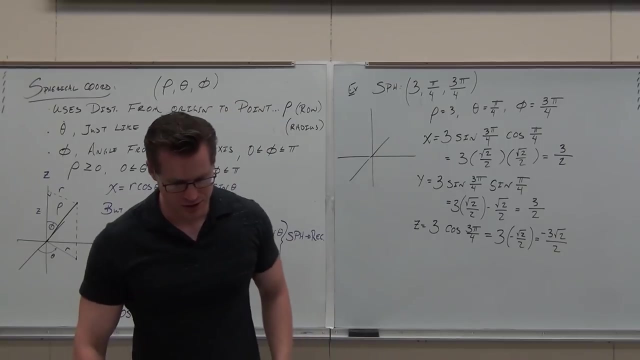 Sorry, I digress Three times. what is cosine three power four Negative- Oh my gosh negative, just like we wanted. So three: Do I have an x coordinate? Yes. Do I have a y coordinate? Yes. 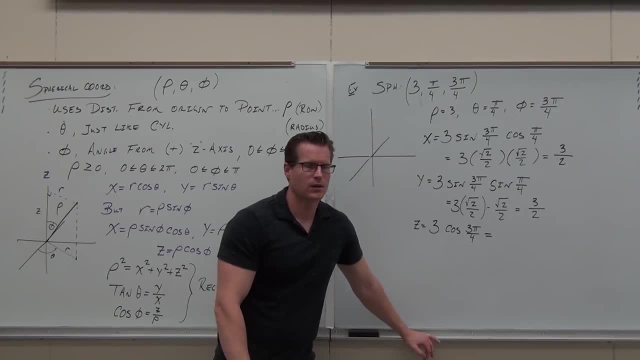 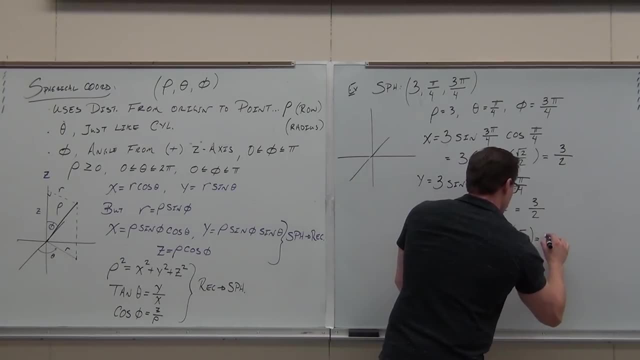 Sorry, I digress Three times. what is cosine of three power four Negative? Oh my gosh negative. just like we wanted. So three. Do I have an X coordinate? Yes, sir, Do I have a Y coordinate? 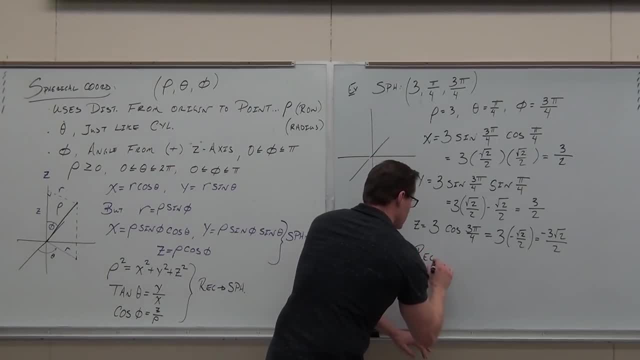 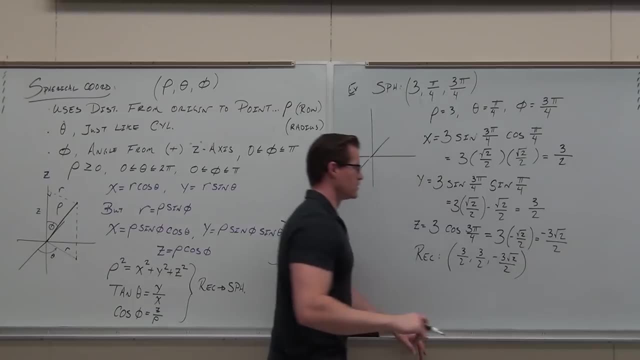 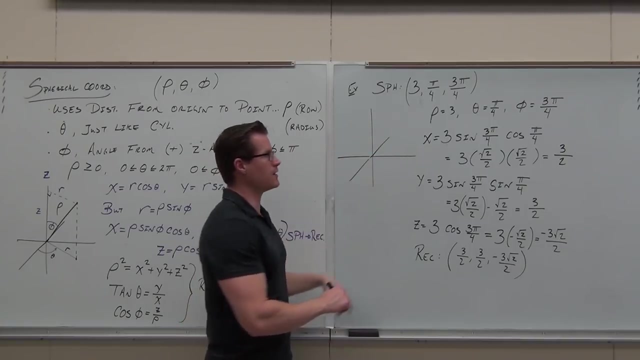 Yes, sir, Do I have a Z coordinate? Yes, sir, So we write the rectangular. We're going to verify that this is in the proper place. This was in quadrant one but octant five, so this guy went out three, however four. 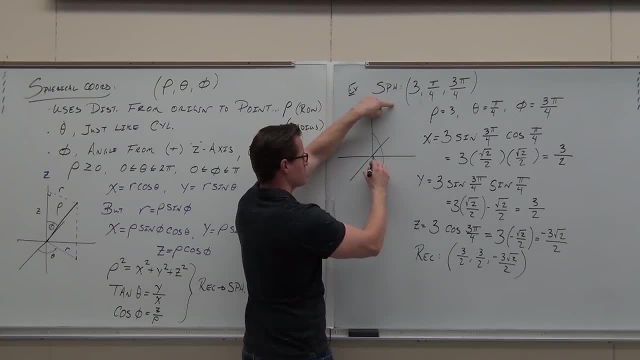 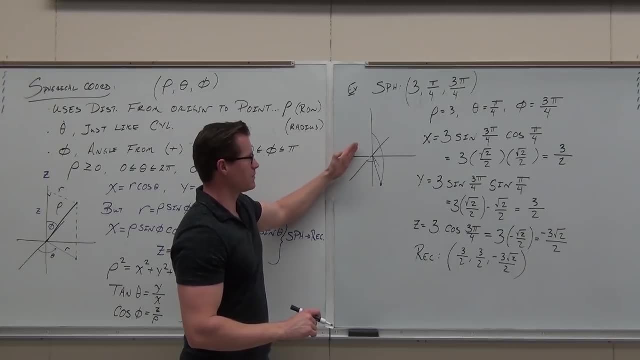 but down like this: Okay Okay. Okay, There we go. All right, That's where that went, That's where that went. This is also in positive X, positive Y, negative Z. It's also in quadrant one, but that octant five. 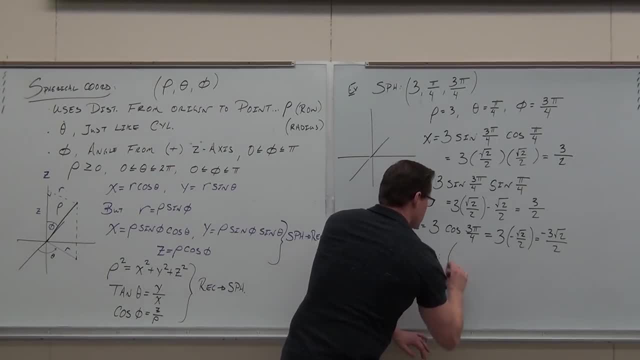 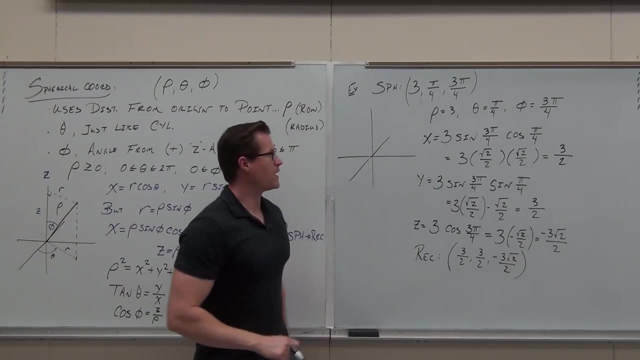 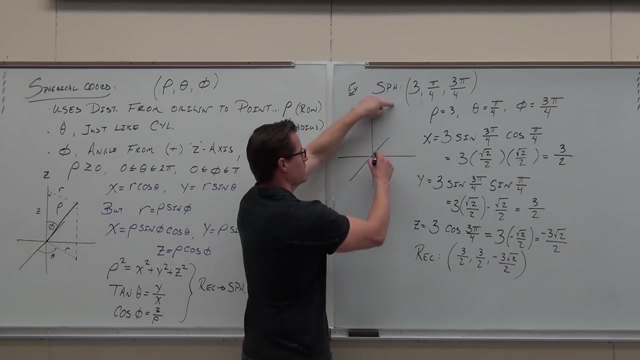 Do I have a z coordinate? Yes, So we write the rectangular. Yes, We're going to verify that this is in the proper place. This was in quadrant one but octant five, So this guy went out three, however four, but down like this: 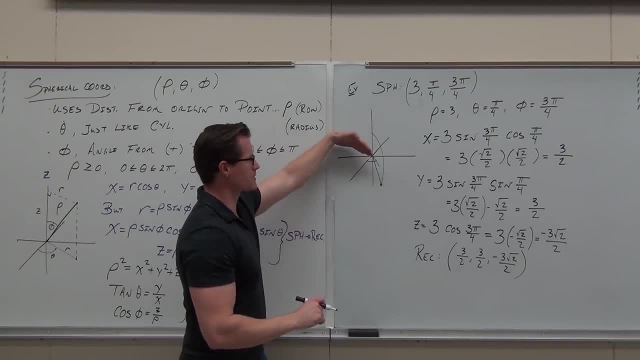 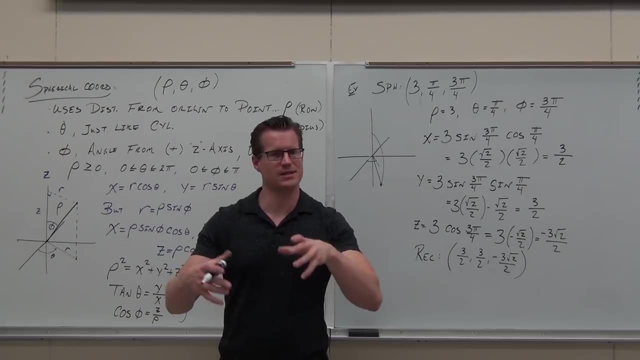 That's where that went. This is also in positive x, positive y, native z. It's also in quadrant one, but that octant five, That's where that thing is. It's the same octant, same quadrant, so I know that we got it right. 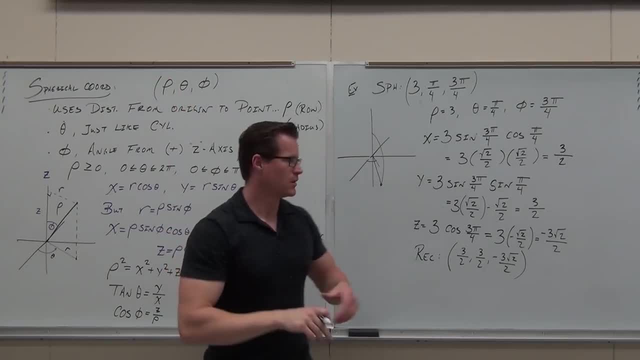 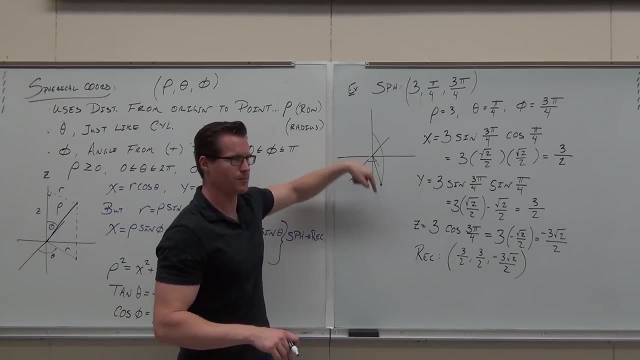 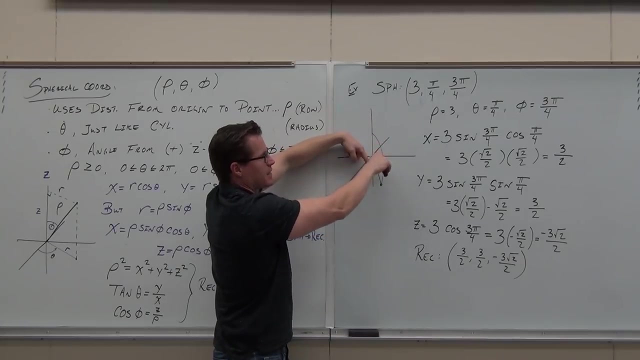 Should fans be okay with that one for real, Are you sure? X positive, y positive, z negative. So out, out and down, This one went. you get this thing floating around, right, But it's, however, four. and then this pushed it down past the x- y plane into octant five. 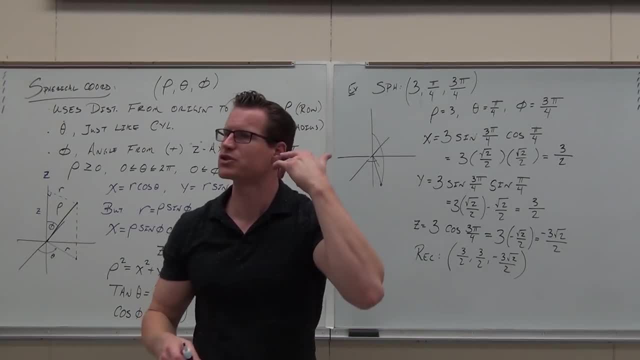 That's where that is. It's hard to draw these things. I don't want to draw these things really accurately, but I want a picture in your head. at least That's what I want. We're going to go backwards and then I'm going to let you. we've got to take a break after that one. 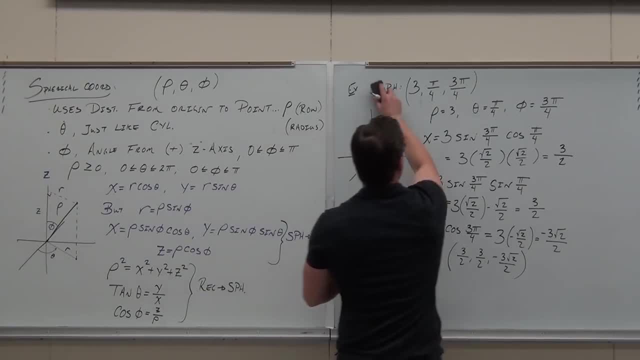 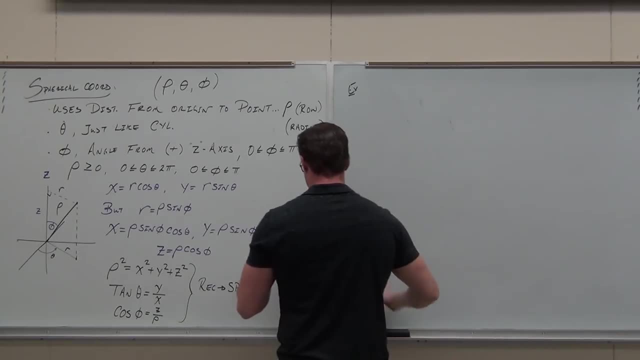 So let's go from rectangular to spherical. Here we go. Okay, We're going to move. We're going to move on this one. all right, The first thing I want you to do is, whatever coordinates this might give you, write down the pertinent information. 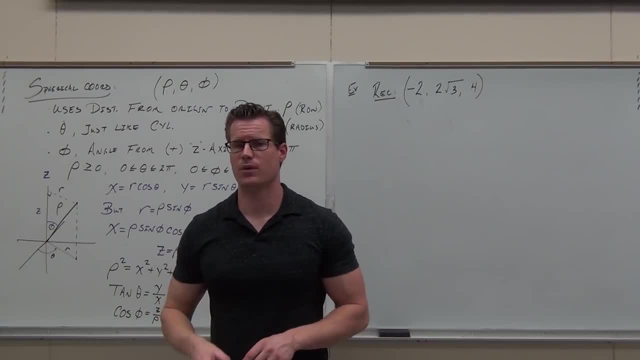 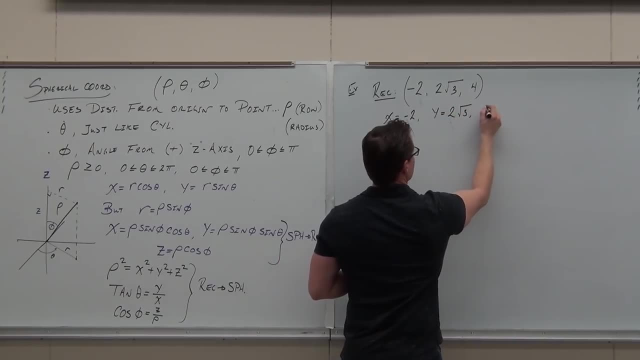 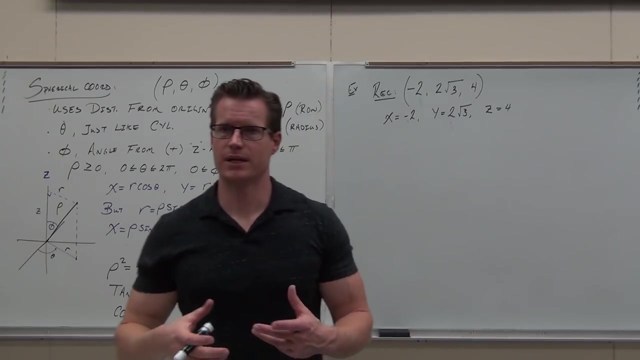 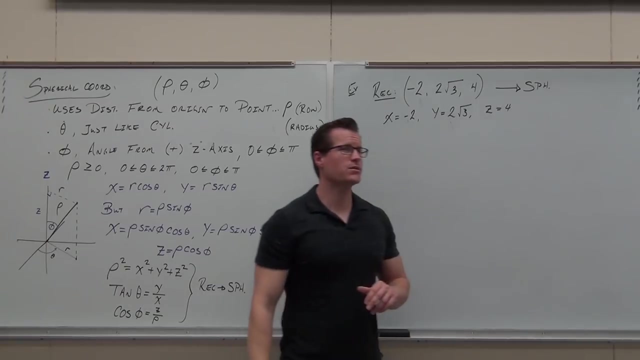 If I give you rectangular, you've got x's, y's and z's. Please, right now, write down the x's, y's and z's Next up. understand where I'm trying to get to. If I want to go to spherical, I've got a way to do that. 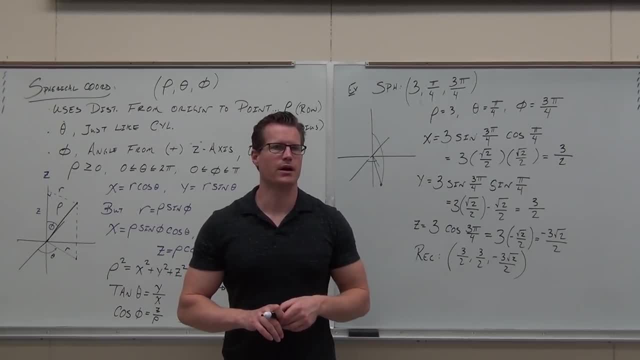 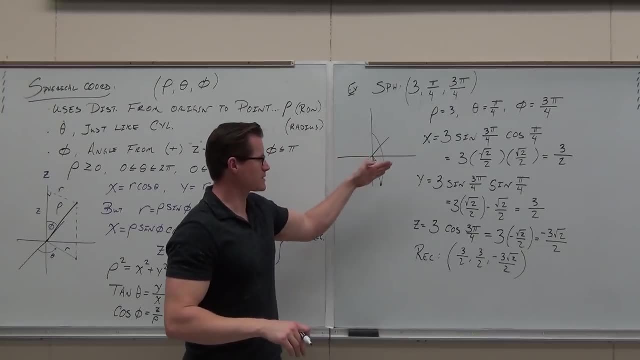 That's where that thing is. It's the same octant, same quadrant, so I know that we got it right. So you're okay with that one for real, Are you sure? X positive, Y positive, Z negative. 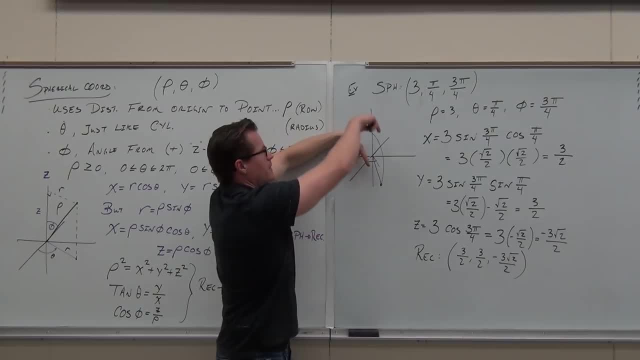 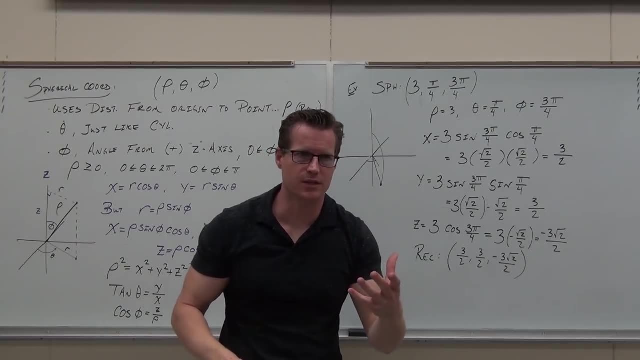 So out, out and down This one went, I have a 4, and then this pushed it down past the xy plane into octant 5.. That's where that is. It's hard to draw these things really accurately, but I want a picture in your head at least. 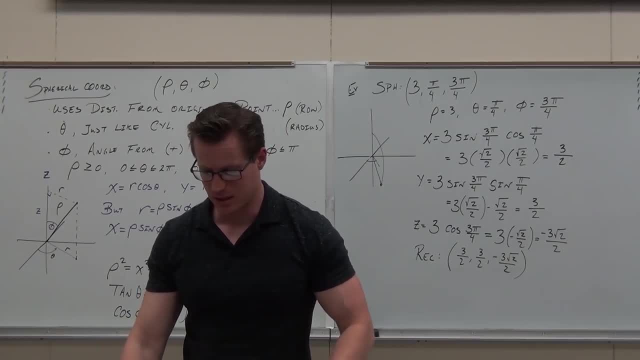 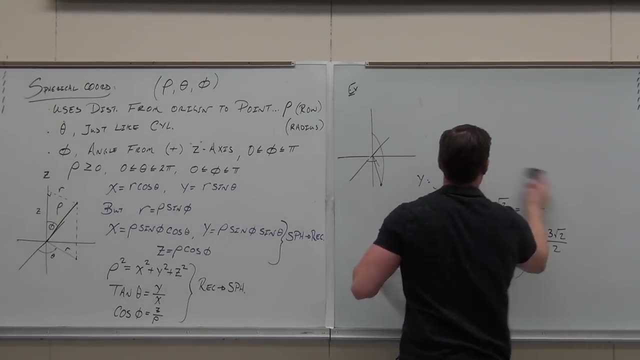 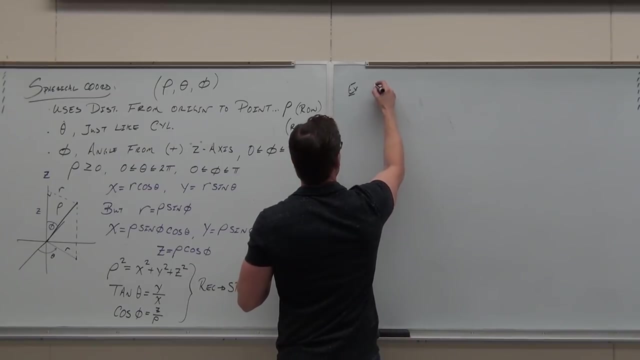 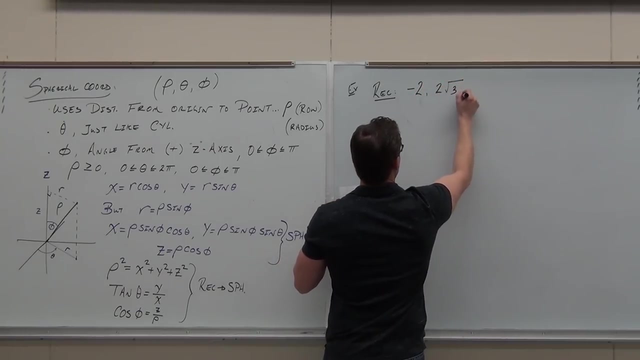 That's what I want. We're going to go backwards, and then we've got to take a break after that one. So let's go from rectangular to spherical. Okay, we're going to move on this one. all right, The first thing I want you to do is whatever coordinates this might give you. 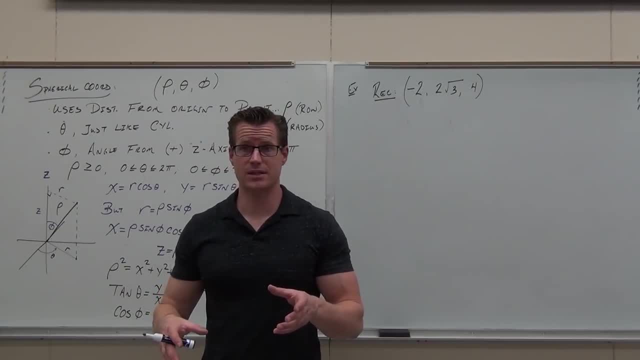 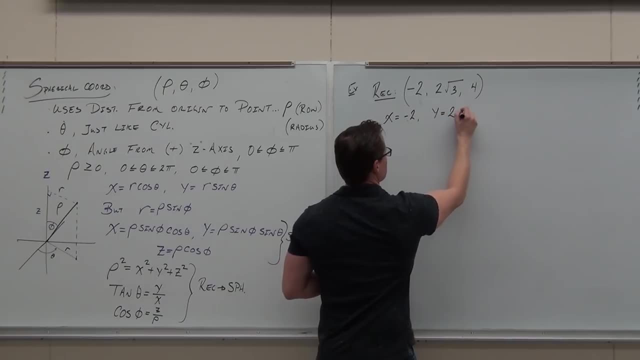 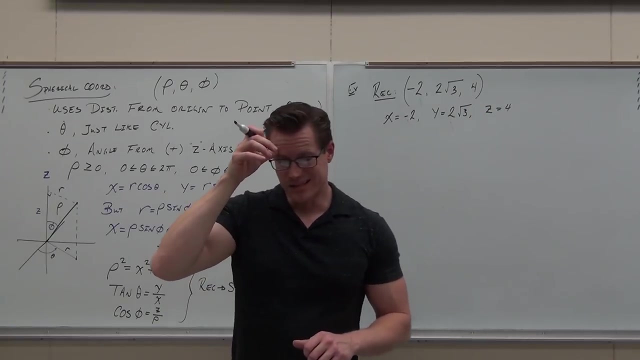 write down the pertinent information. If I give you rectangular, you've got x's, y's and z's. Please, right now, write down the x's, y's and z's. Next step: Understand. Understand where I'm trying to get to. 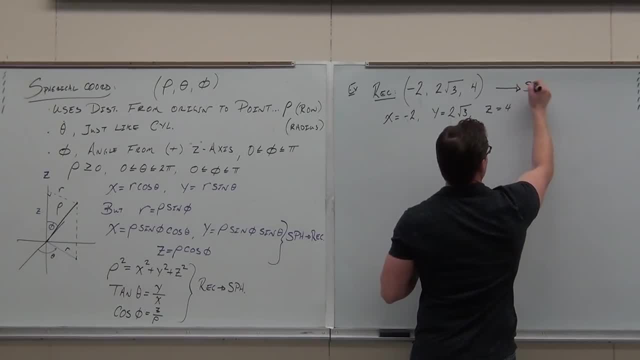 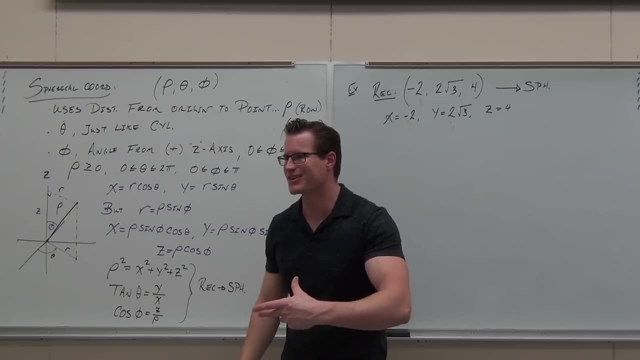 If I want to go to spherical, I've got a way to do that. Now, obviously, going from rectangular to cylindrical is a piece of cake. It's a lot easier, But spherical- we also have some stuff there. So if I'm going from rectangular to spherical, I've got to take my x's, y's and z's. 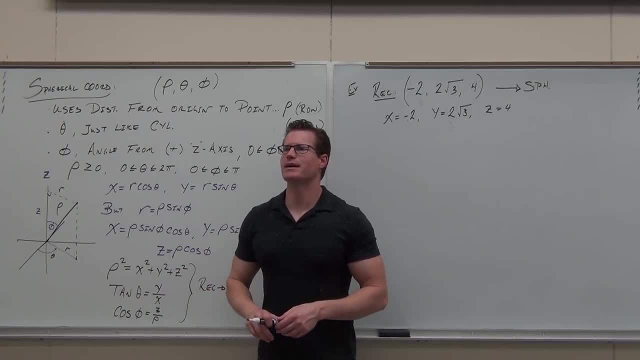 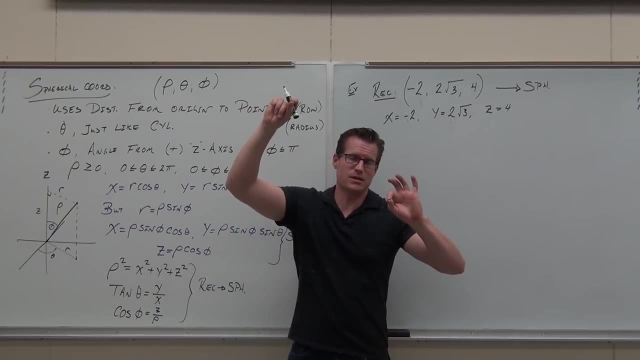 You know what that is. It's a Galdar magnitude of pretty much a vector, because that length from the origin to a point it would be the same exact thing as a magnitude of a. it's a magnitude, That's all we're doing. 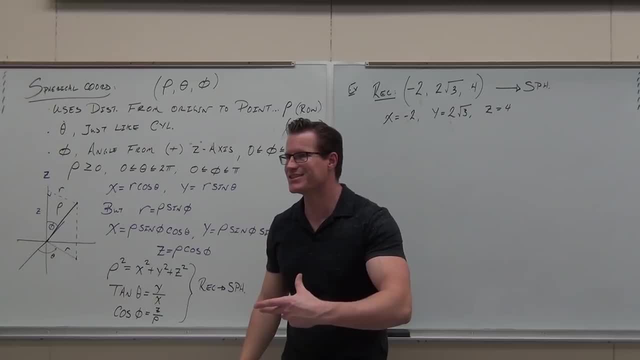 Now, obviously, Going from rectangular to cylindrical is a piece of cake. It's a lot easier, But spherical- we also have some stuff there. So if I'm going from rectangular to spherical, I've got to take my x's, y's and z's. 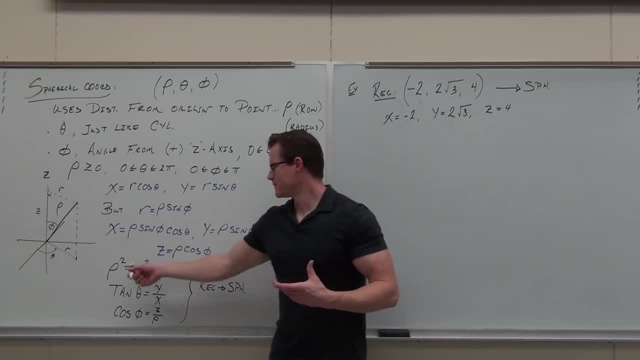 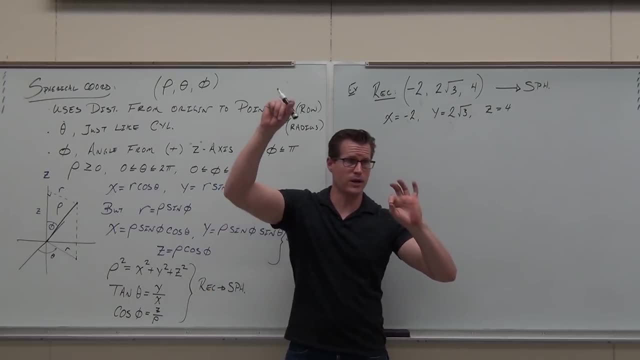 You know what that is. It's a Galdar magnitude of a, pretty much a vector, because that length from the origin to a point would be the same exact thing as a magnitude of a. it's a magnitude, That's all we're doing. 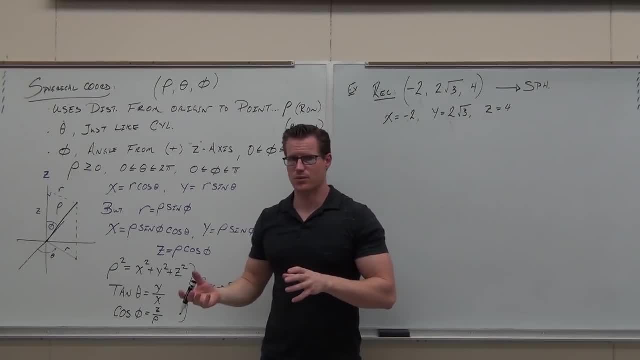 Square the stuff, add them together, take a square root. That's how we find our row. Does that make sense to you? So let's do that first, So to find our row. oh, you know what I forgot something. 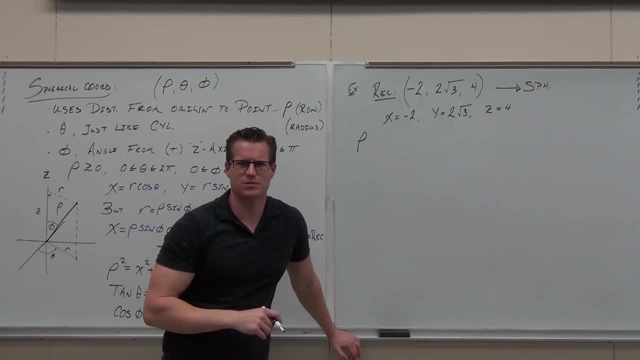 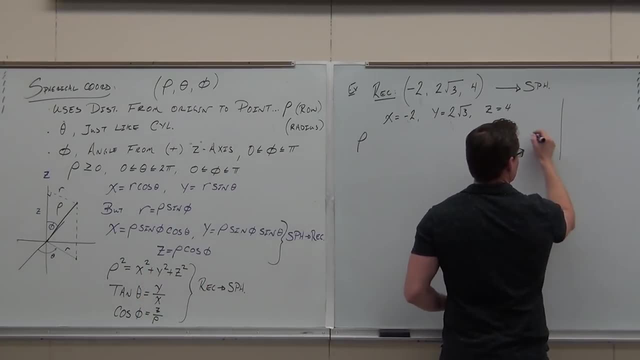 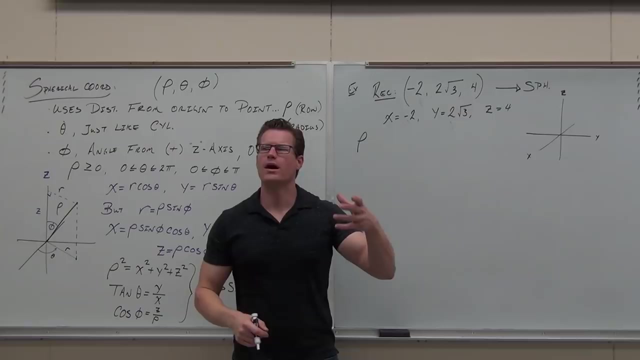 I forgot the major part. Before we even do any of this work, what's important about it? What should we be thinking about, at least? Where is it at? Where is it at? What quadrant is this in? Negative x pushes us back. 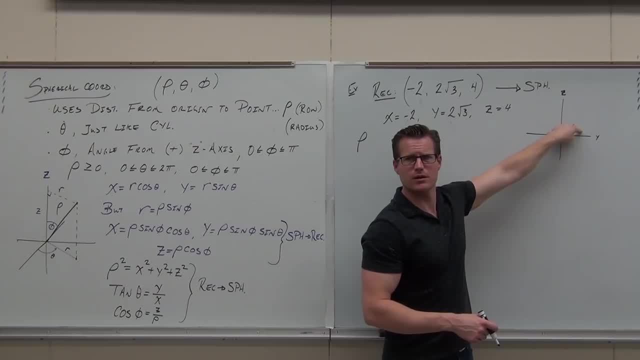 Positive x pushes us back. Positive y comes up this way. What quadrant? Quadrant 2. Quadrant 2.. And then positive z pushes us up this way: What octant 2. 2. So we're in 2, 2.. 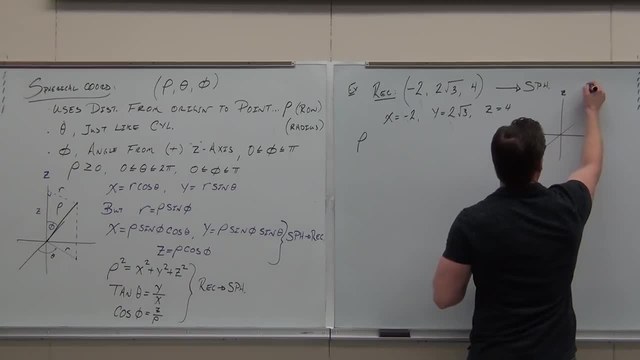 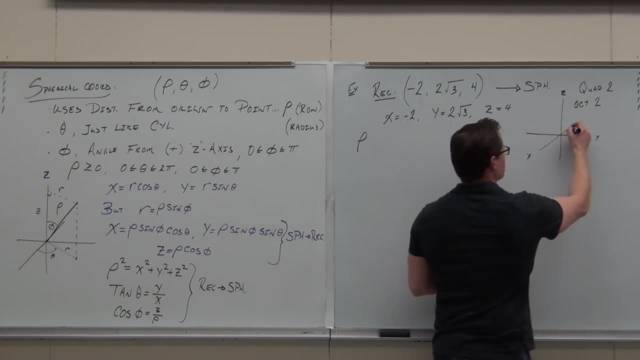 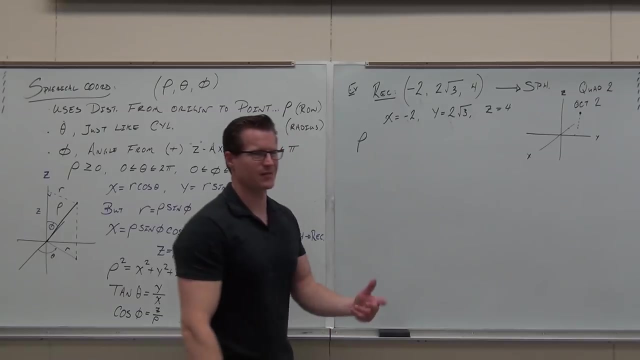 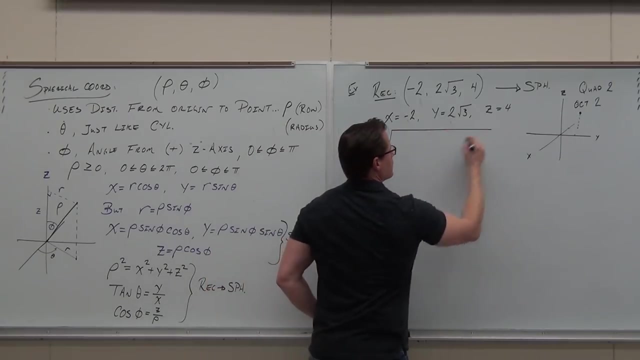 So quadrant 2 on the x- y plane, octant 2.. Floating right about there, It doesn't have to be exact, So let's go ahead. let's find our row. So to find the row, we're going to take the square root of x squared plus y squared plus. 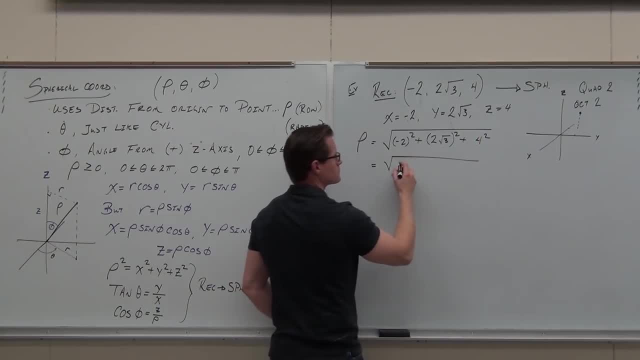 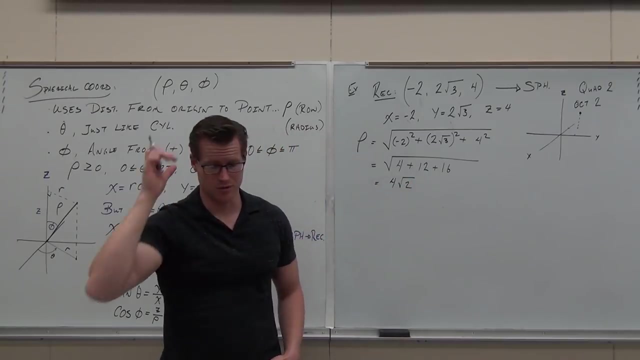 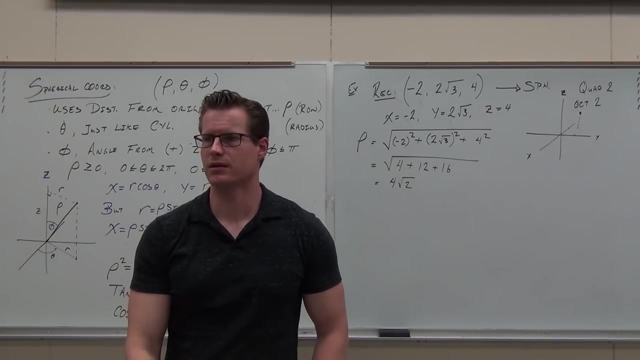 the z coordinate squared. I think it's 4 root 2.. I'm pretty sure. I'm pretty sure: Square root of 32,, 4 root 2.. No, Yeah, Double check, Yes, Triple check. You got the same thing I got. 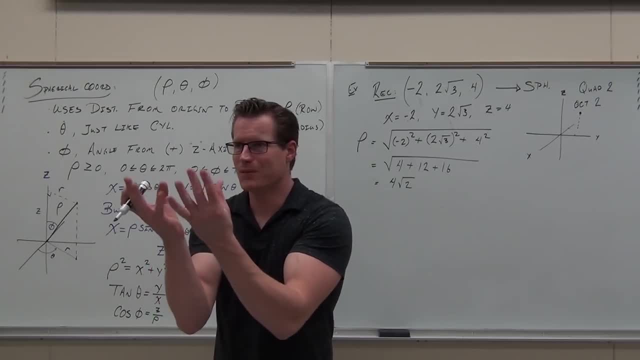 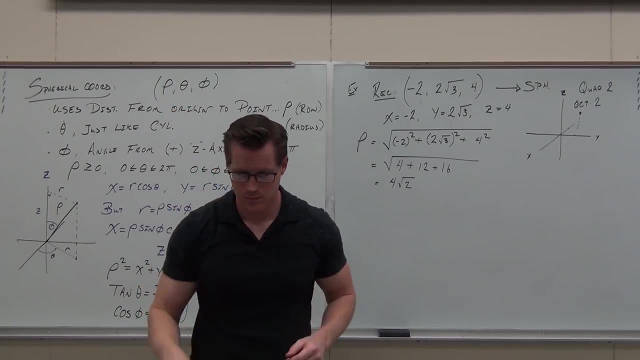 Use calculator, whatever. What else do we need? Come on quickly. What else do we need? We got our row, All these things are row, and then we got. can we find our theta? Yes, How? 10th of u. 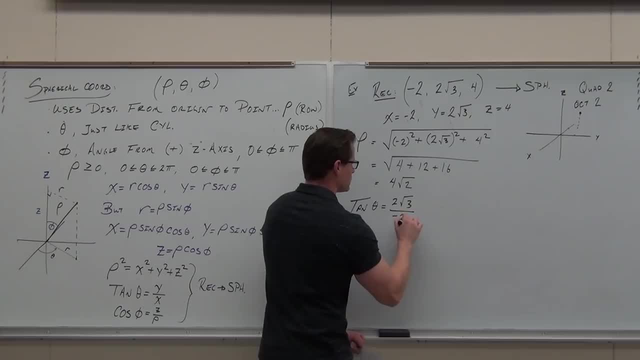 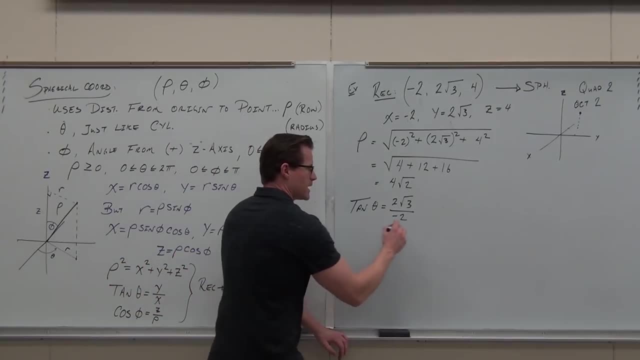 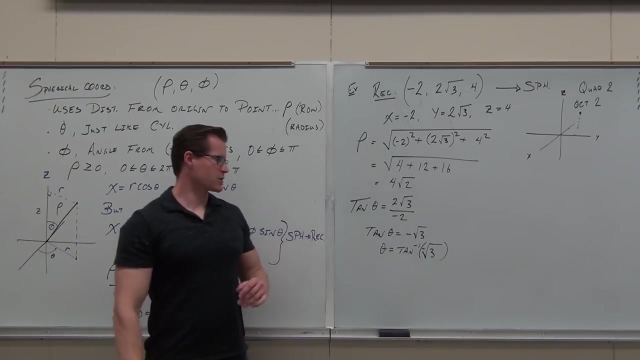 10th of u. Yeah, yeah, yeah. Why is it y over x? Why is it y? Why is it y over x? Why Y over? don't do x over y, Do y over x. Rise over, run y over x. 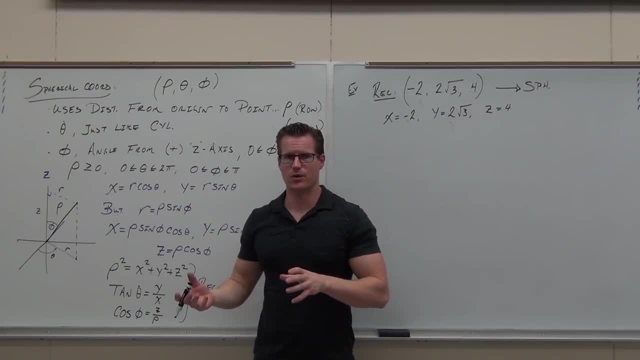 Square the stuff, add them together, take a square root. That's how we find our row. Does that make sense to you? So let's do that first, So to find our row. oh, you know what I forgot something. 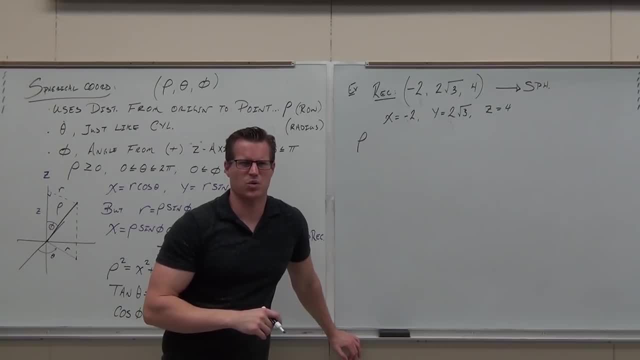 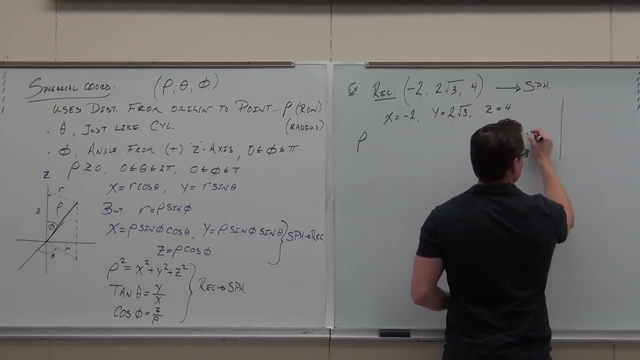 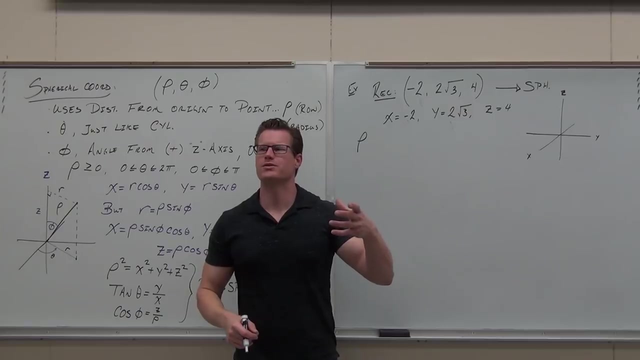 I forgot the major part. Before we even do any of this work, what's important about it? What should we be thinking about, at least? Where is it at? Where is it at? What quadrant is this in? Negative x pushes us back. 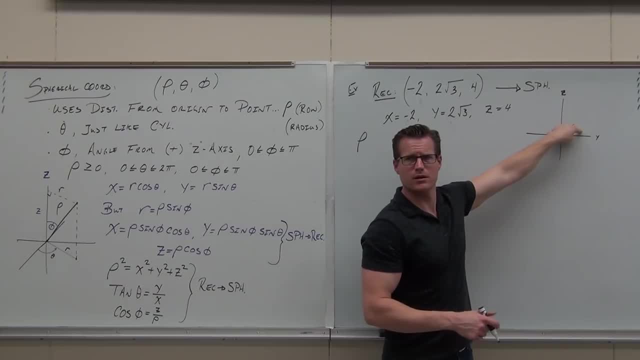 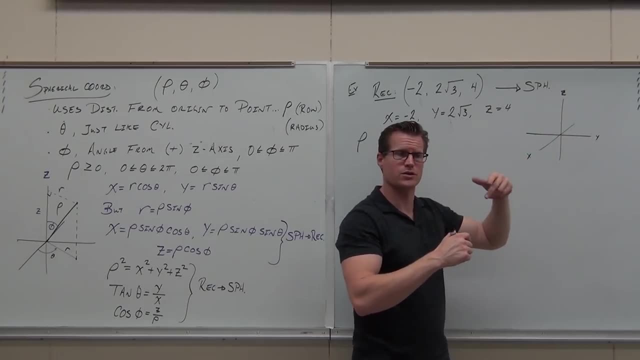 Positive y comes up this way. What quadrant? Quadrant two. And then positive z pushes us up this way: What? octant Two. So we're in two. two, So quadrant two on the xy plane: octant two, Positive z. 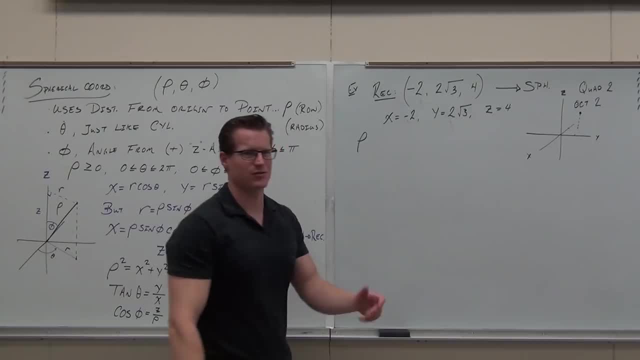 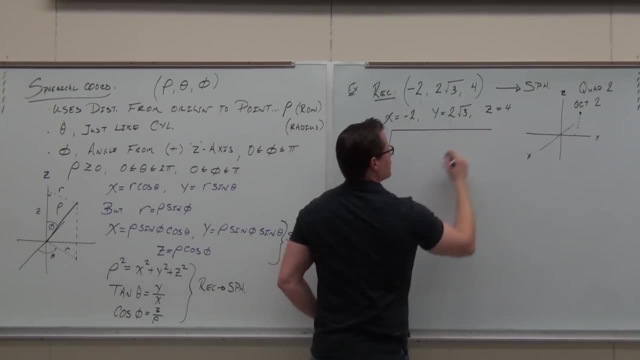 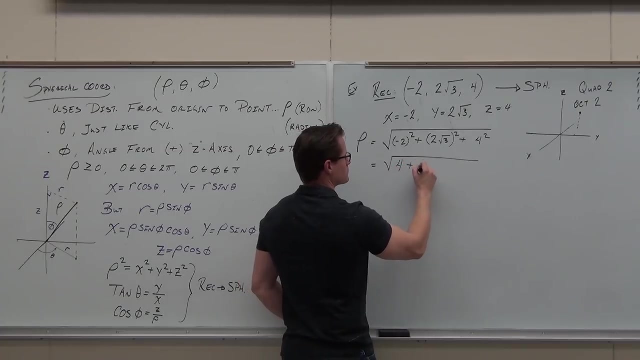 So we're going to do this: We're going to take the square root of x squared plus y squared, plus the z coordinate squared, And then we're going to take the square root of x squared plus y squared plus the z coordinate squared. I think it's 4 root 2.. 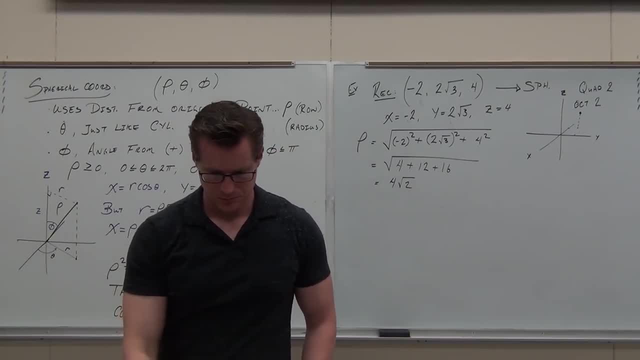 I'm pretty sure. Square root of 32, 4 root 2?? No, Double check, Triple check. You got the same thing. I got, Just calculator, whatever. What else do we need? Come on quickly. What else do we need? 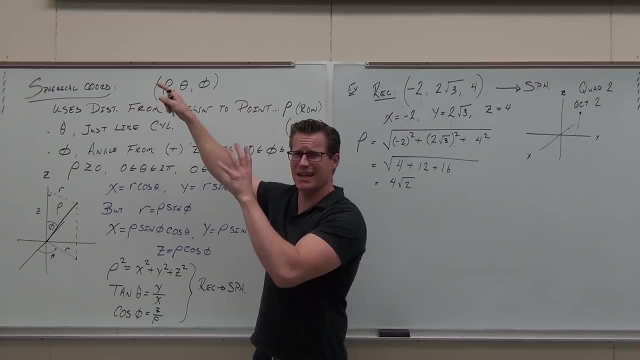 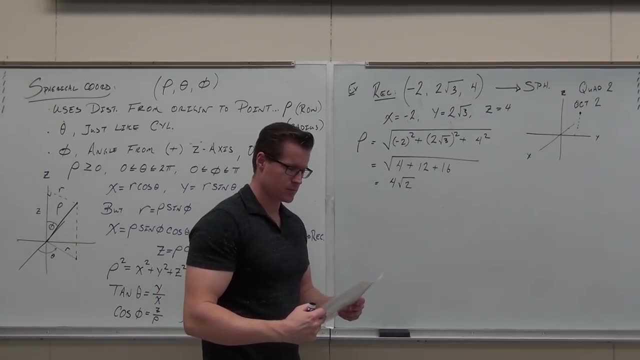 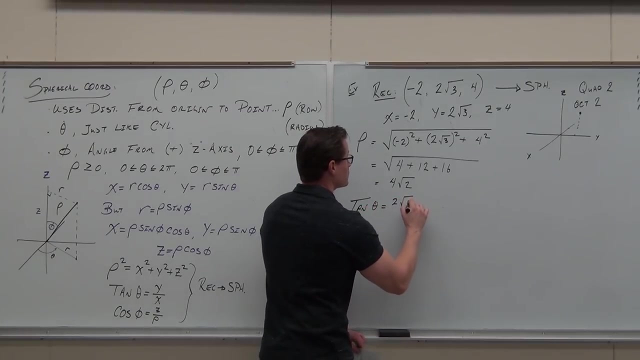 We got a row. All these things are a row. and then we got. can we find our theta? Yes, How? 10 theta Equals x over y over x. 10 theta- You're right there- Y over x. 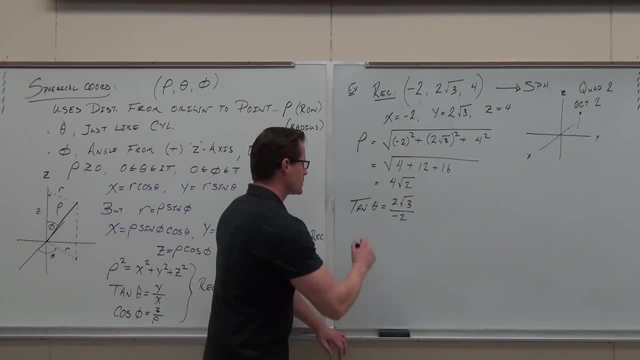 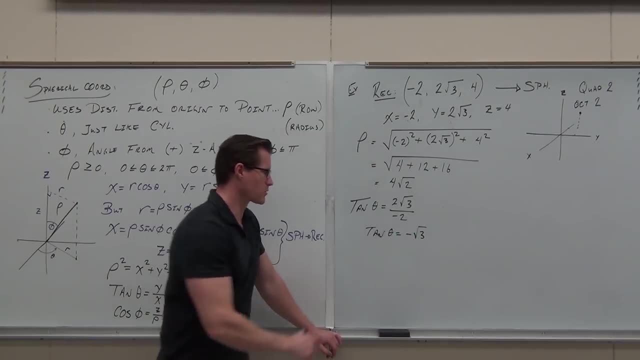 Don't do x over y, Do y over x. Rise over, run y over x. So then, 10 theta Negative square root of 3?. 10 inverse of man. do you know 10 inverse of negative square root of 3?? 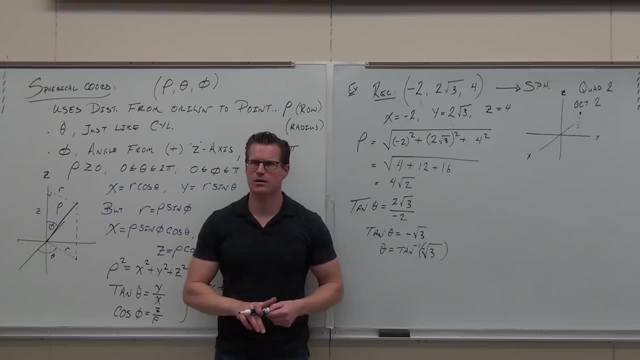 So then, 10 theta Negative square root of 3? 10 inverse of man. do you know 10 inverse of negative square root of 3? Do you know that one? No, That's the problem. No, Give it to me in terms of pi, pi over 6,. so let's see, we want the square, we want sine. 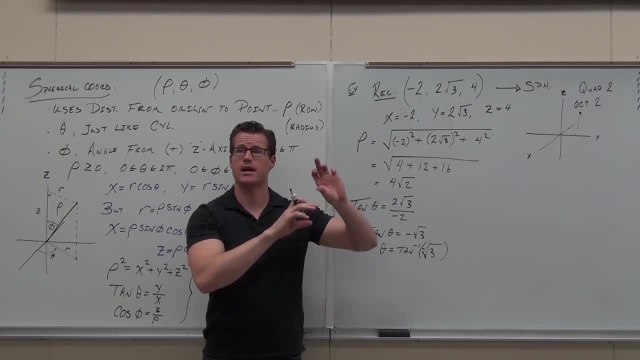 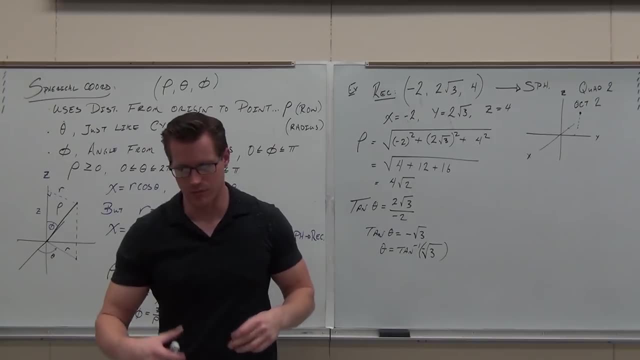 over cosine right, and we want the square root of 3 to be on the sine part and the one half to be on the cosine part, and we want it to be negative. so we want the sines to be wrong with each other. so what would it be? 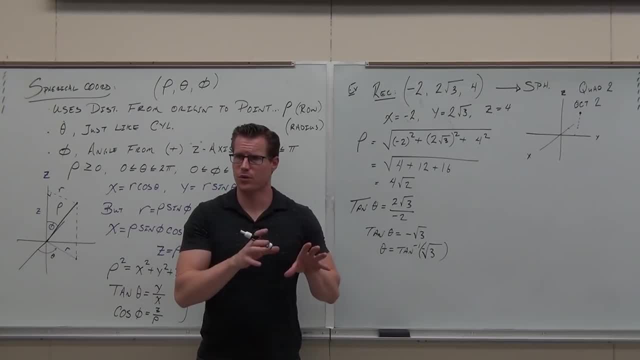 It's got to be in either quadrant 2 or quadrant 4, do you guys see what I'm talking about? Quadrant 2 or 4.. I know that cosine of pi over 3 and 2 pi over 3 is that root is that one half. so I want. 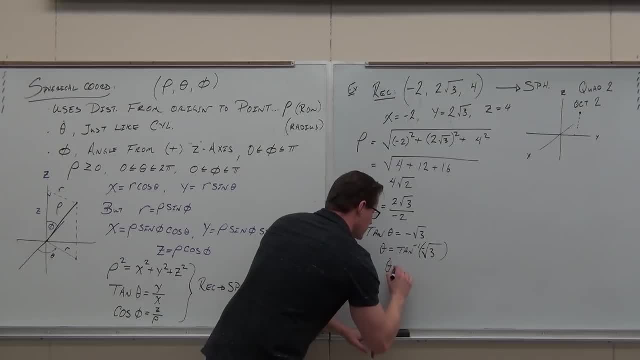 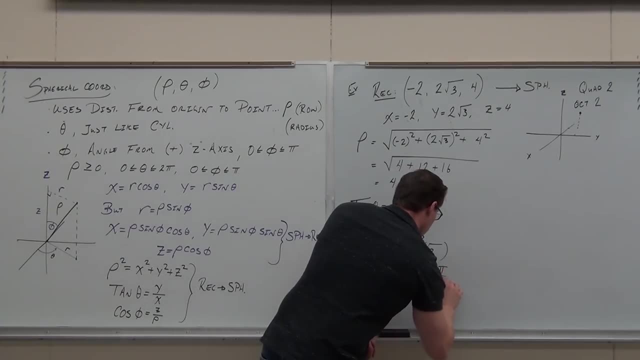 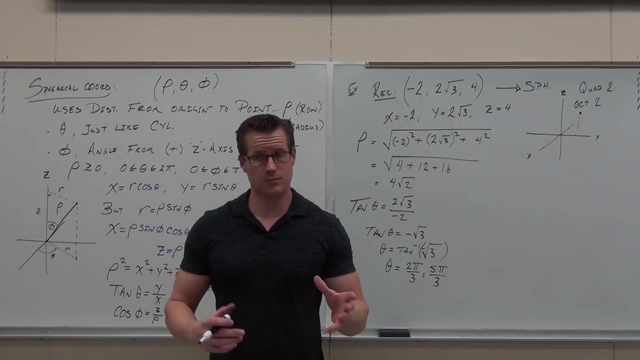 the denominator to be one half, so this has to be 2 pi over 3 or 5 pi over 3.. It's unit circle time, folks. We don't have time to function around with this. Okay, We don't have time to f around with it. sorry, but you have to know how to do that. 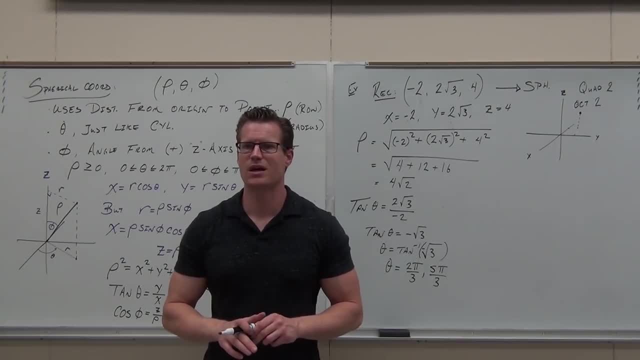 Honestly, I don't want decimals, I don't want 30 degrees. calculus is done in radians. we need radians and I want them in radians and I want them accurate every freaking time. Sorry to be a jerk right, but I want it done because I want you to be successful at it. 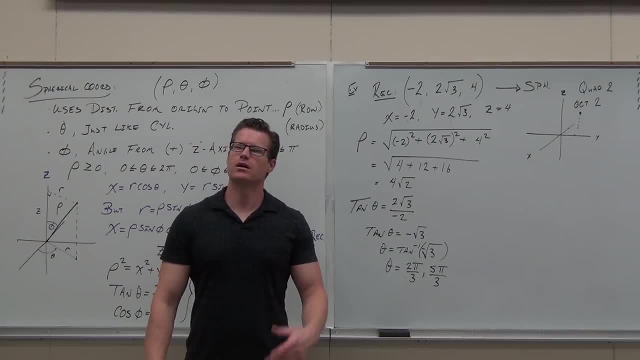 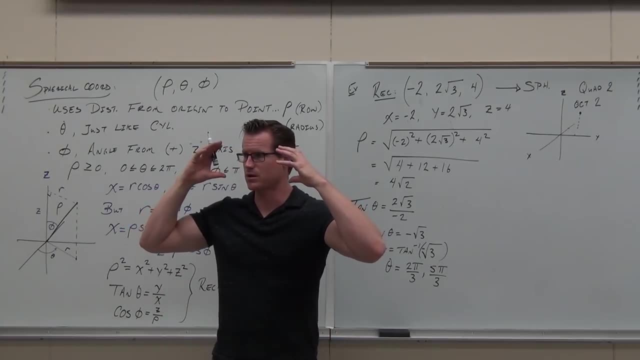 I want you to get down to here and be like: I don't know, Why don't you know, Print out a unit circle, tattoo it right, draw it. I don't care, but I need this like up here. Are you following what I'm talking about? 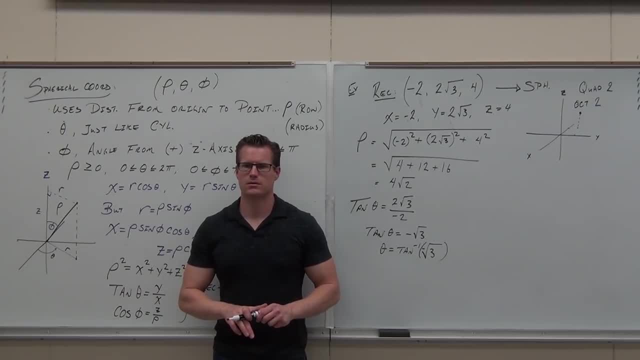 Do you know that one So 30? Give it to me in terms of pi: Pi over 6?, Pi over 6?. So let's see, We want the square, We want sine over cosine And we want the square root of 3 to be on the sine part and the 1 half to be on the cosine part. 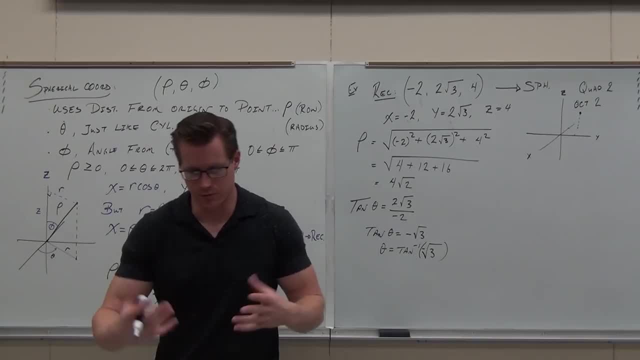 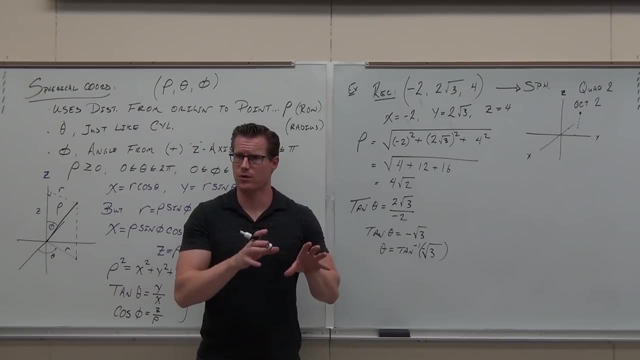 And we want it to be negative, So we want the sines to be wrong with each other. So what would it be? Well, it's got to be in either quadrant 2 or quadrant 4.. Do you guys see what I'm talking about? 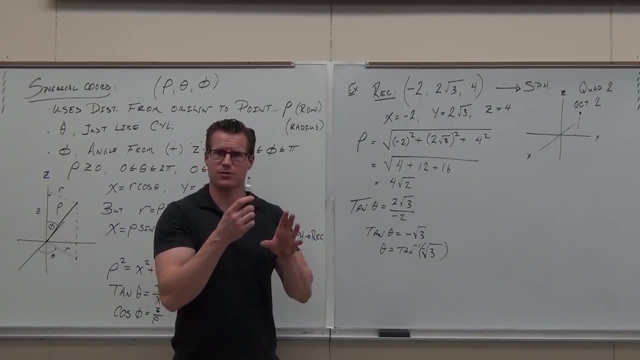 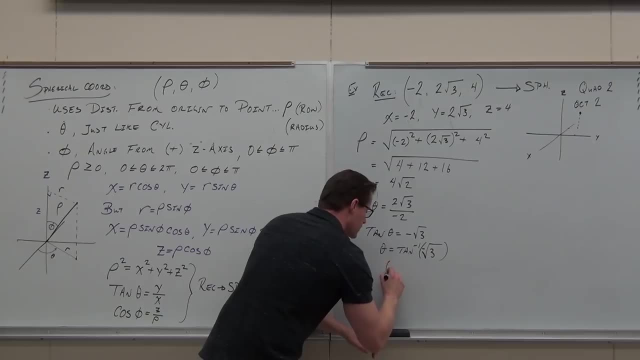 Quadrant 2 or 4.. I know that cosine of pi over 3 and 2 pi over 3 is that root is that 1 half. So I want the denominator to be 1 half. So this has to be. 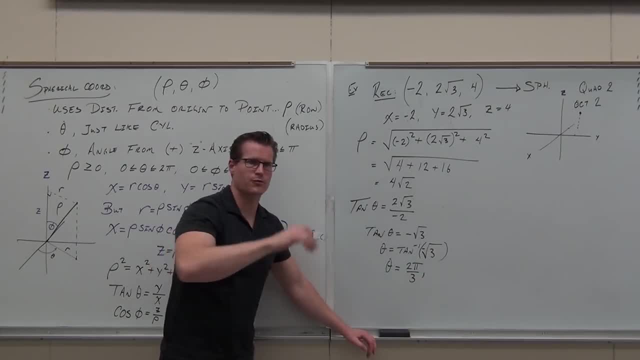 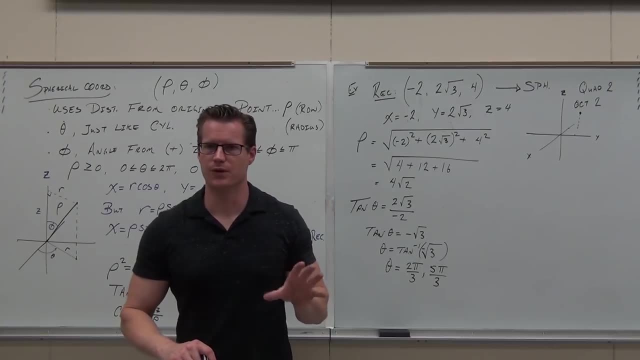 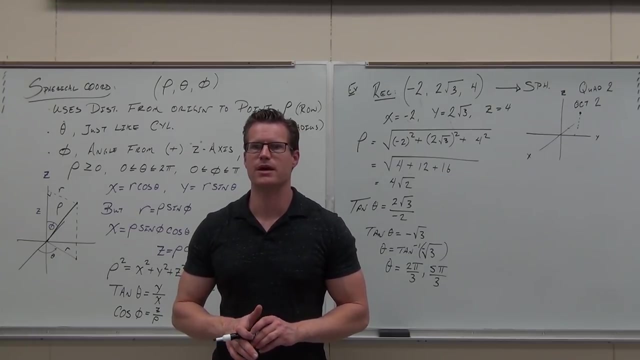 2 pi over 3 or 5 pi over 3? It's unit circle time. folks. We don't have time to function around with this. We don't have time to f around with it. Sorry, But you have to know how to do that. 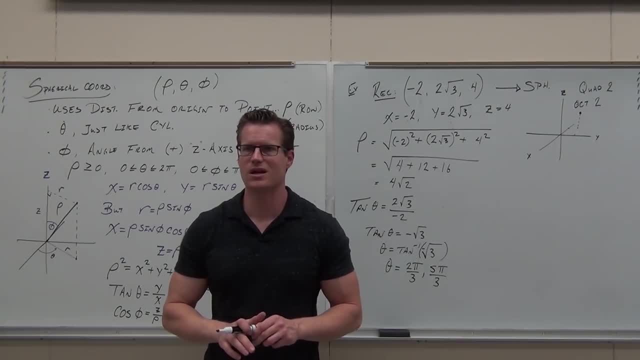 Honestly, I don't want decimals, I don't want 30 degrees. Calculus is done in radians. We need radians And I want them in radians And I want them accurate every freaking time. Sorry to be a jerk right. 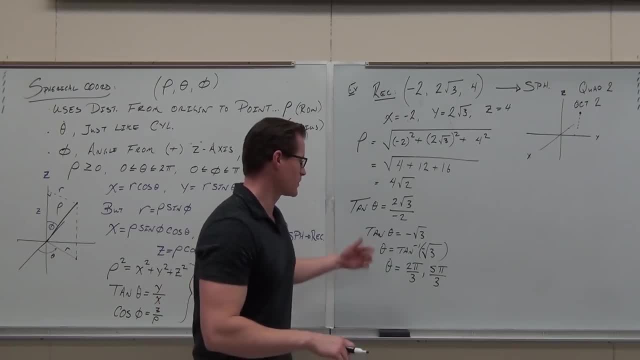 But I want it done Because I want it done. I want it done, I want it done, I want you to be successful at it. I want you to get down to here and be like I don't know, Why don't you know? 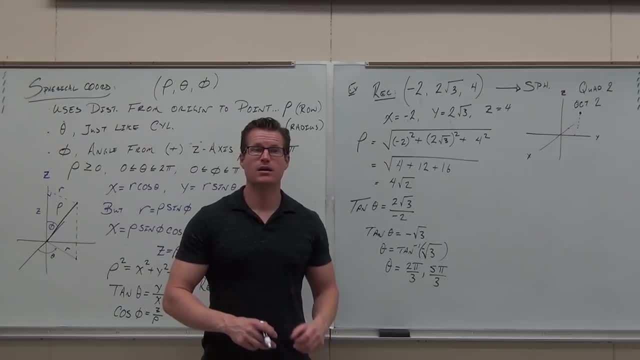 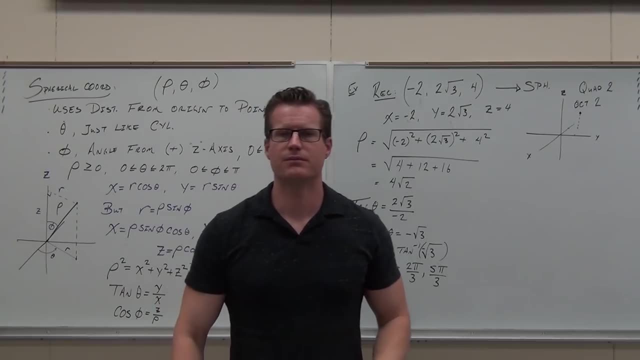 Print out a unit circle, Tattoo it Right there, Draw it. I don't care, But I need this like up here. Are you following what I'm talking about? I need that Now. man, there's something huge we talked about. 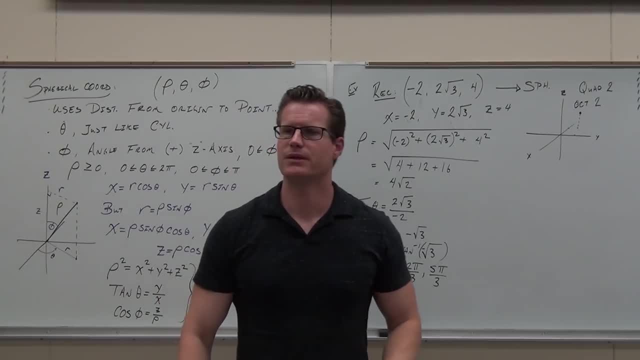 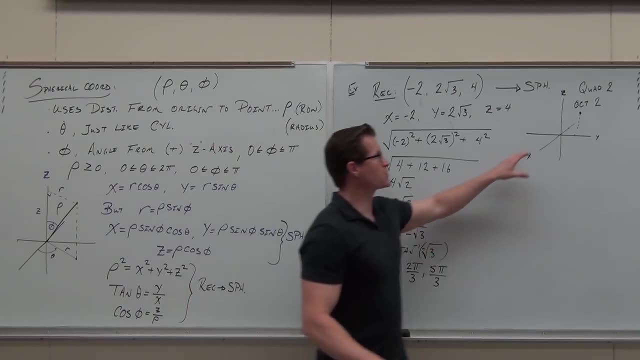 I need that Now. man, there's something huge. we talked about It. was you better make sure that this stuff matches where this is? and we did it, We did it. What quadrant on the xy plane is the projection of our point? 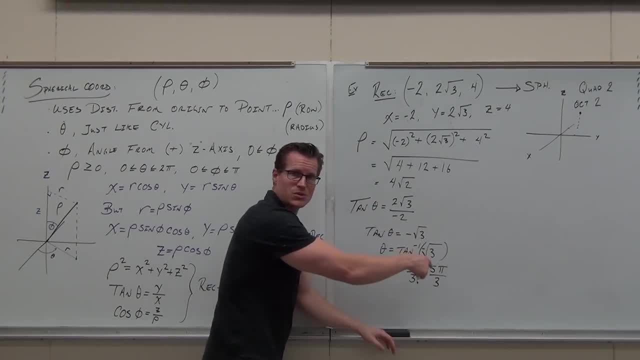 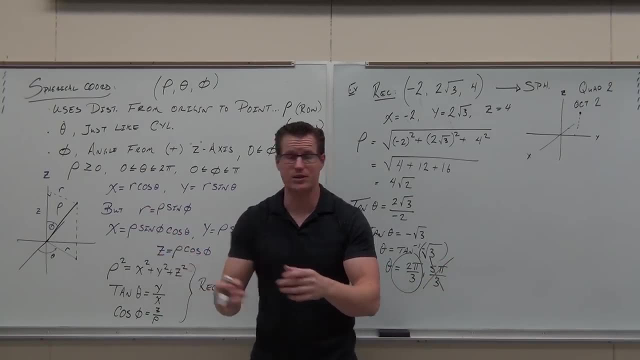 What quadrant's that? in Two, Two? Which one of these is in quadrant two? Quadrant three? That one, Not that one. Only pick one. There's no two options here. You pick the one in the correct quadrant. so, since our projection of our point is in: 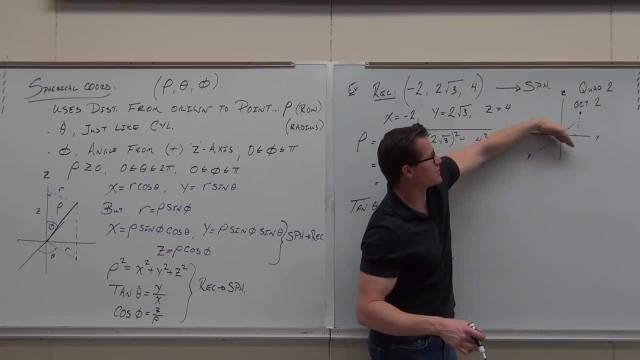 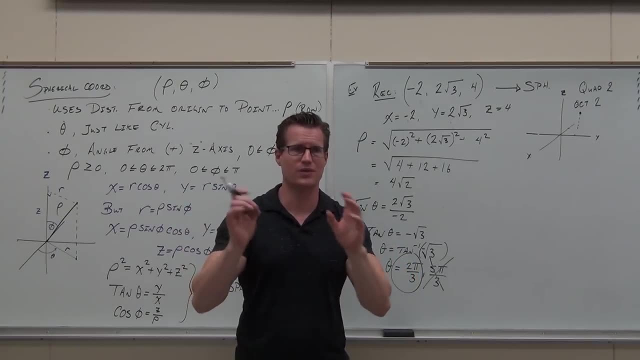 quadrant two. That angle for theta from the positive x is also in quadrant two. It's right there. That's the appropriate theta. That's how you do it. There's no doubles here like there was in cylindrical. That's the only one. 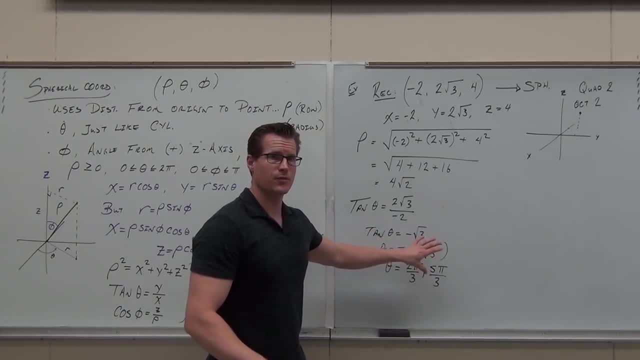 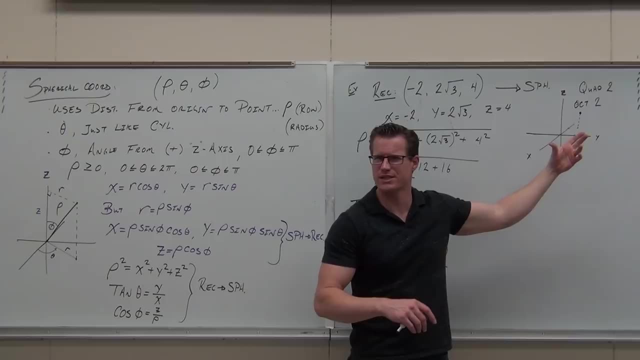 It was. you better make sure that this stuff matches where this is, And we did it, We did it. What quadrant on the xy plane is the projection of our point? What quadrant is that in Which one of these is in quadrant two? 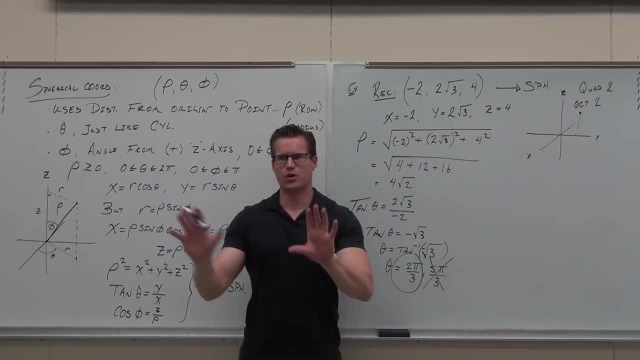 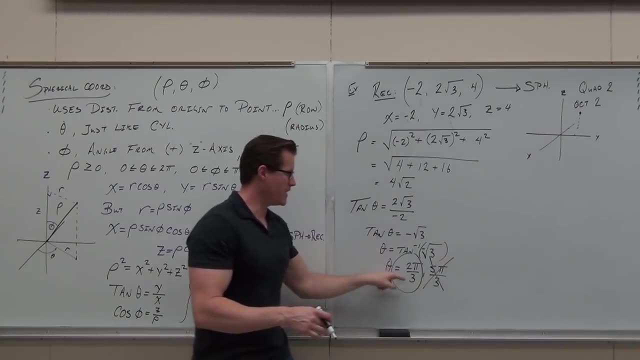 That one, That one, Not that one. You only pick one. There's no two options here. You pick the one in the correct quadrant. So since our projection of our point is in quadrant two, that angle for theta from the positive x is also in quadrant two. 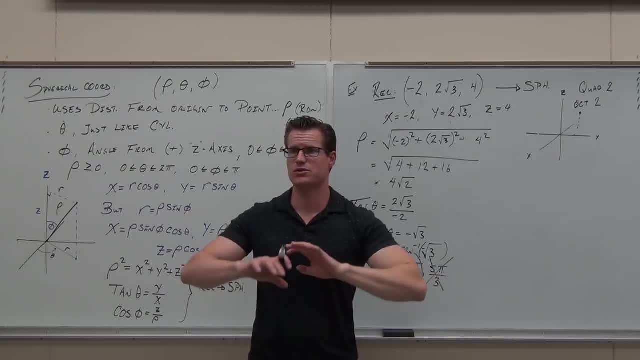 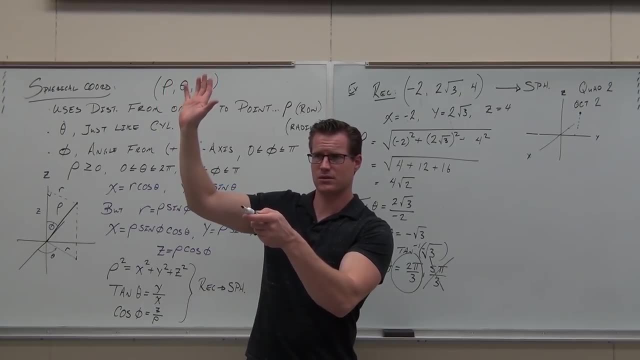 It's right there. That's the appropriate theta. That's how you do it. There's no doubles here like there was in cylindrical. That's the only one. Should fans feel okay with that one? Yes, no, Yeah, Yeah. 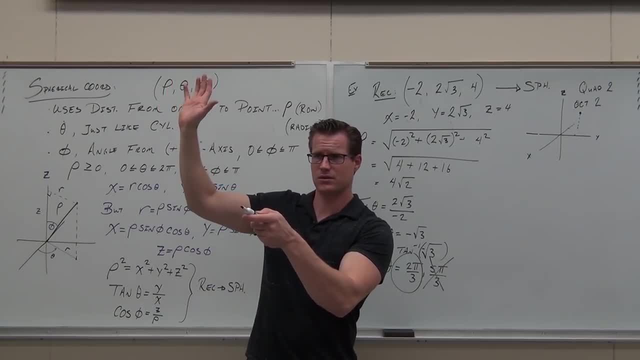 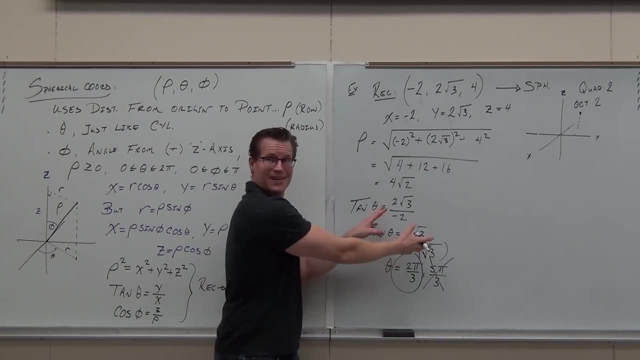 Show of hands if you feel okay with that one. Yes, No, Yeah, Yeah, Yeah, Or this between that, because that's the this one. from here to here we go. that's the one. it is Okay, That's that's the only one over there. 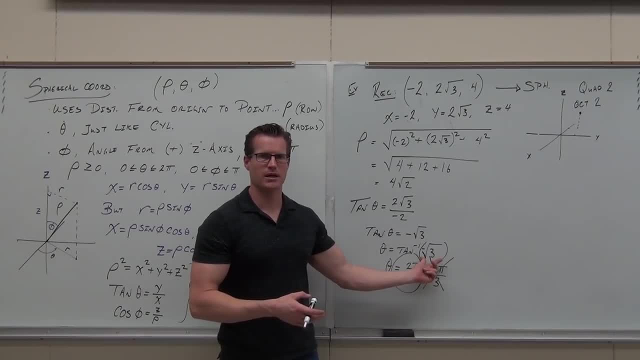 Okay, Okay, Yeah. One over three, 기자. do you know where this goes? Good, It's seven under three. Do you know where this goes? No, because I silvered yours. Well, I skipped one in the last segment. 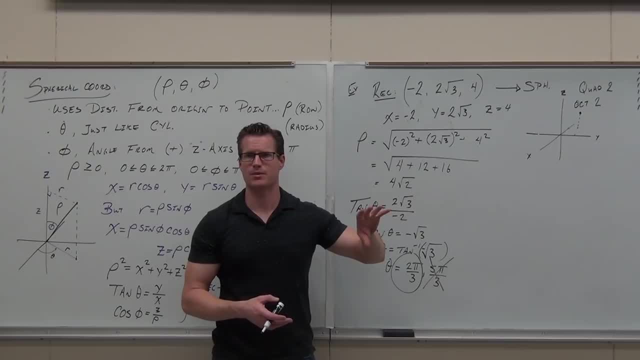 Oh, Oh, good, You may have. This is the one at the end. 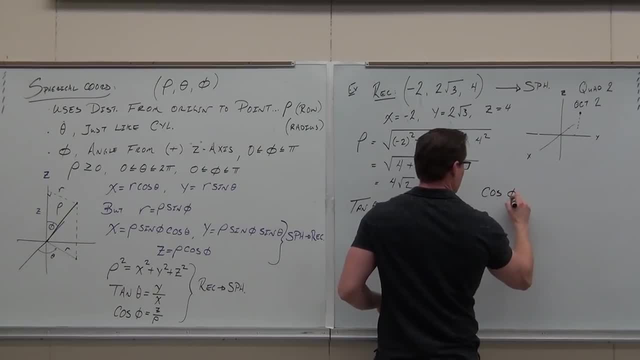 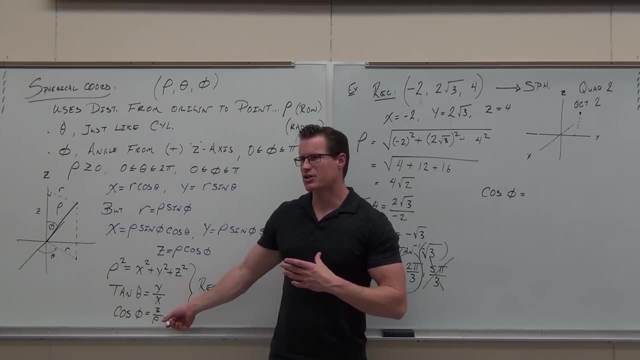 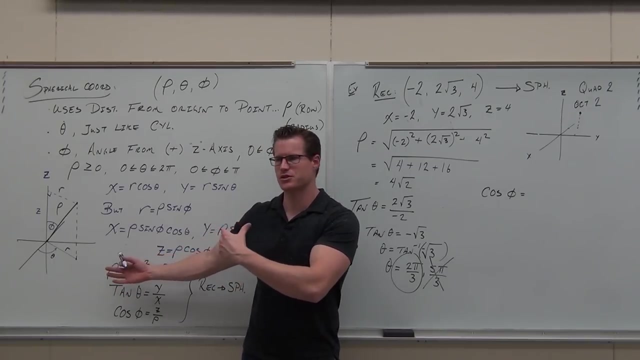 Let's talk about cosine phi. Do you recognize, like in the formula, that in order to actually do this you have to find rho first? You guys see what I'm talking about. You have to be able to find that first. So once you find rho, that's the first thing you do. 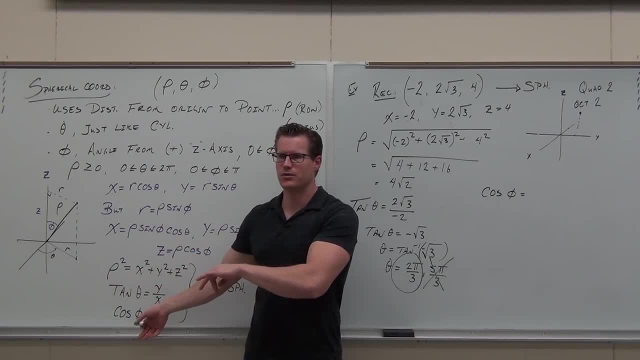 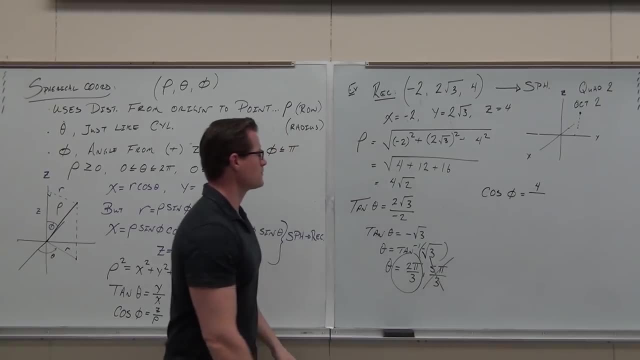 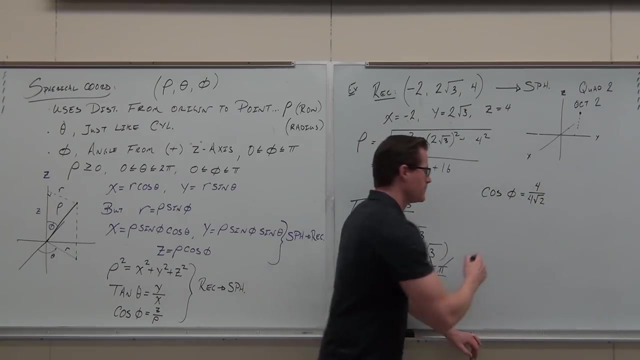 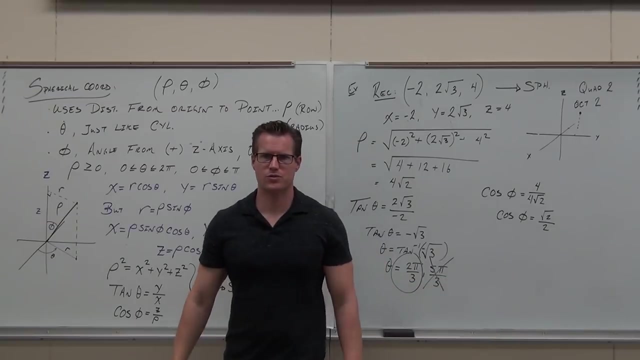 Then you find theta. You just hang on to that a little bit and then we go down and we find phi. So for phi, we're going to put z Over rho. Of course you're going to simplify it. So simplify the fours, rationalize. we've got root 2 over 2,. 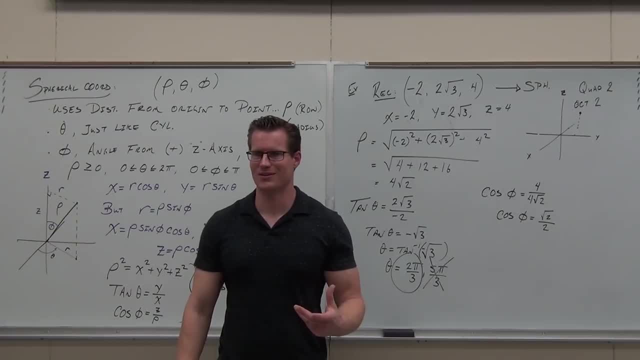 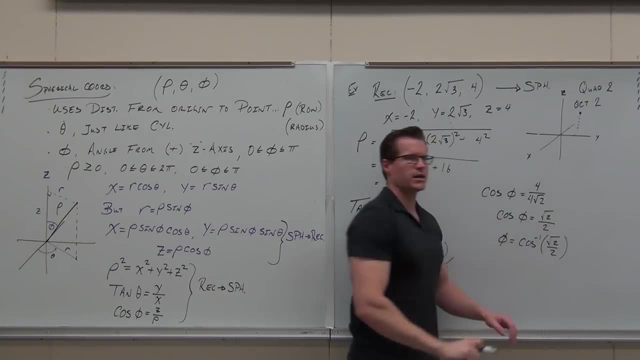 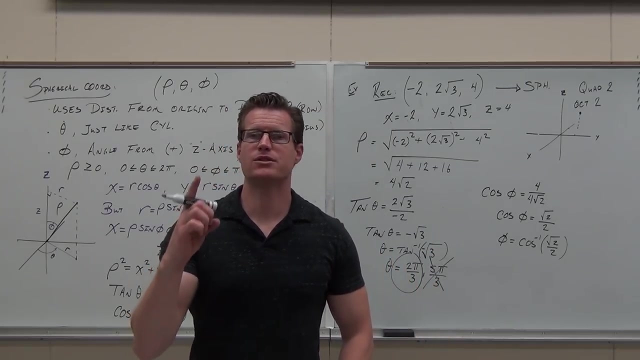 and you get a nice one for once, Thank goodness. What is cosine inverse of root 2 over 2?? And keep in mind, there's only one answer here, because this is only defined from 0 to pi. We don't go past that. 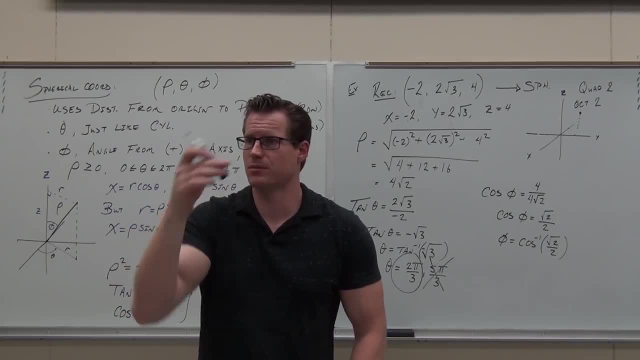 So you don't even have to worry about all the other stuff. It's literally just between 0 and pi, And since cosine is 1 to 1 between 0 and pi, we go. hey, sweet, I love that Cosine just drops like this. 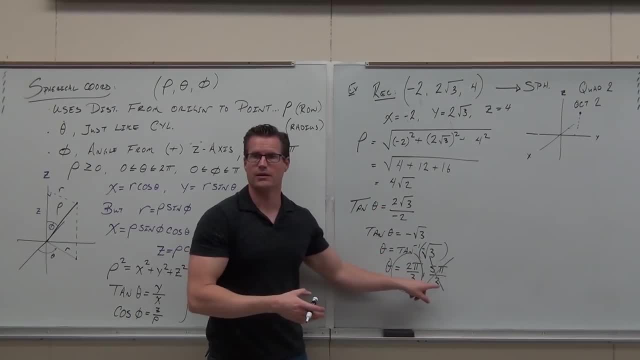 Yeah, Yeah, Or this between that, because that's the this one. from here to here we go, That's the one. it is Okay. So unit circle says tangent of what angle gives us negative square root of three. That's where sine is either positive or negative and cosine is positive or negative. 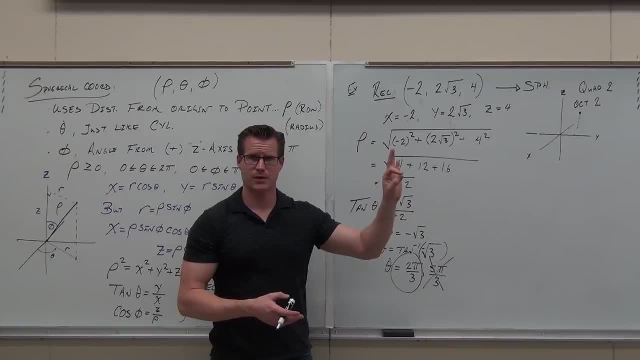 but you have different signs. Sine has to be root three over two, Cosine has to be one half. That only happens at two pi over three and five pi over three. That's only two places it happens. There's only one right answer, though, because only one of those is in the correct quadrant. 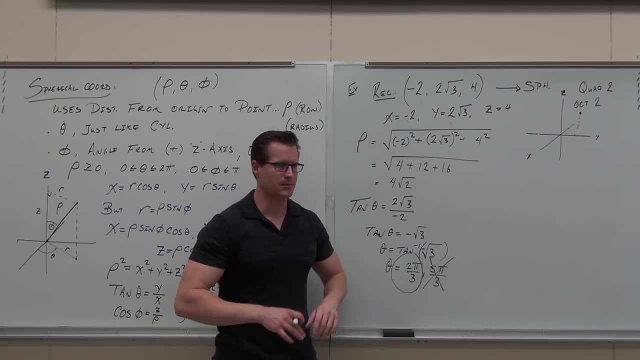 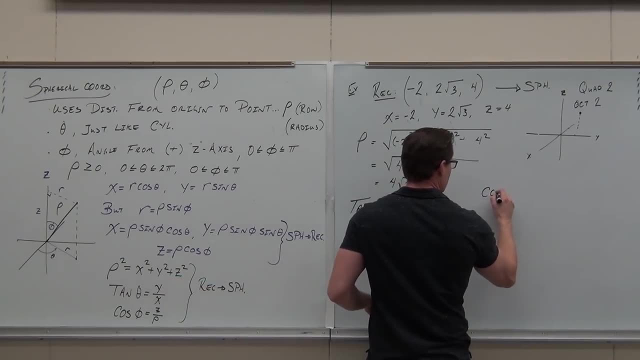 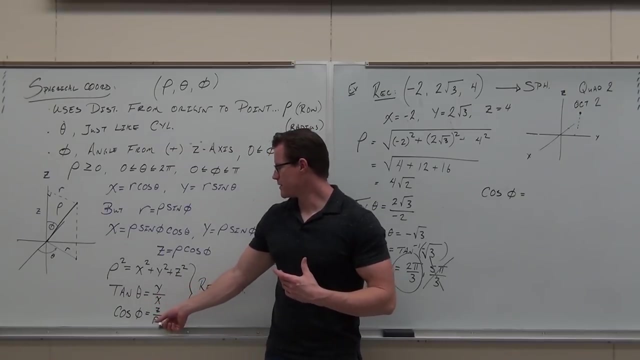 of the xy plane, only one, and it's that one. That's it Now. let's talk about. let's talk about cosine phi. Do you recognize, like in the in the formula, that in order to actually do this you have to find rho first? 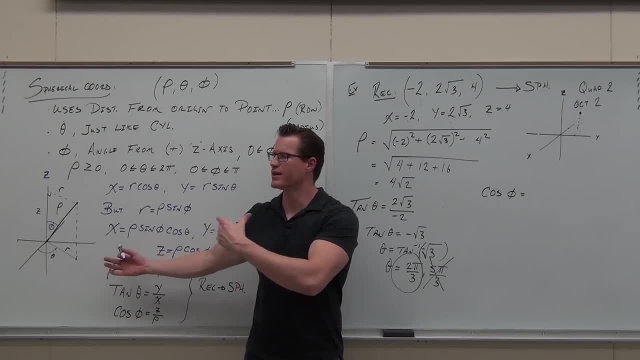 You see what I'm talking about. You have to be able to find that first. So once you find rho, that's four. That's the first thing you do. Then you find theta. You just hang on to that a little bit and then we go down and we find phi. 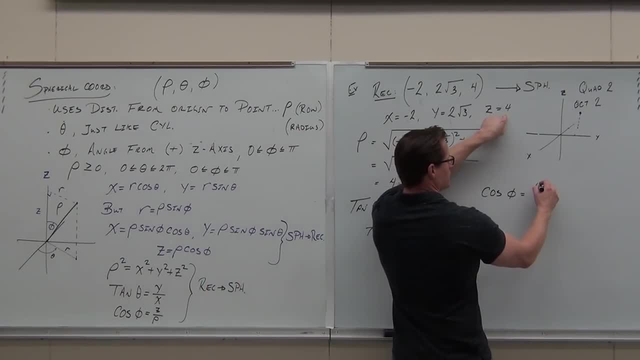 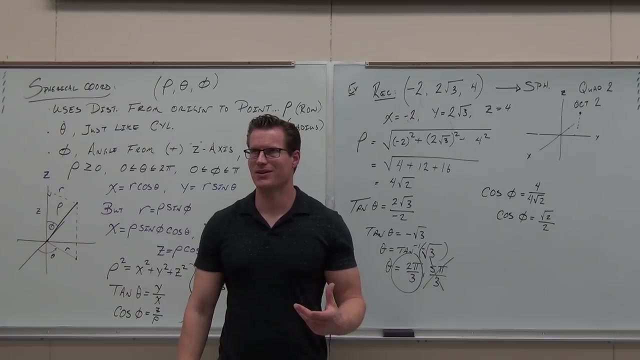 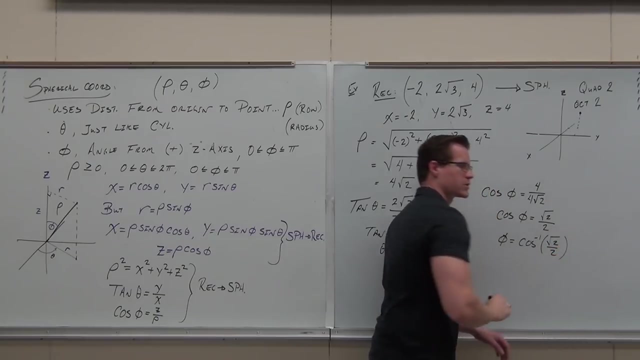 So for phi, we're going to put z over rho. Of course you're going to simplify it. So simplify the fours, rationalize. we've got root two over two and you get a nice one for once, Thank goodness. What is cosine inverse of root two over two? 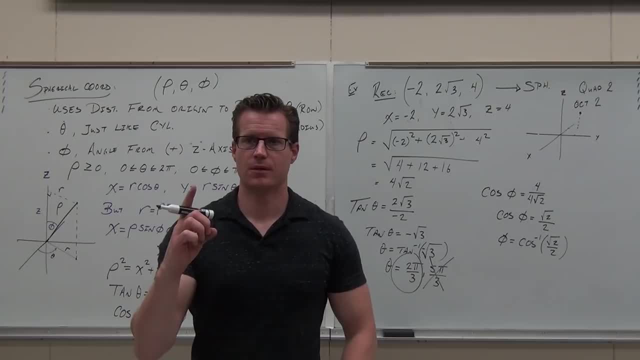 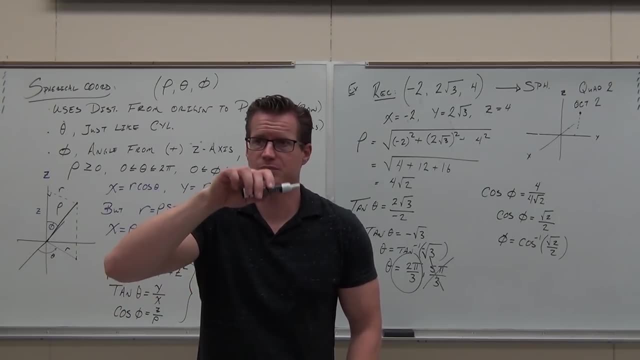 And keep in mind there's only one answer here, because this is only defined from zero to pi. We don't go past that, So you don't even have to worry about all the other stuff. It's literally just between zero and pi. 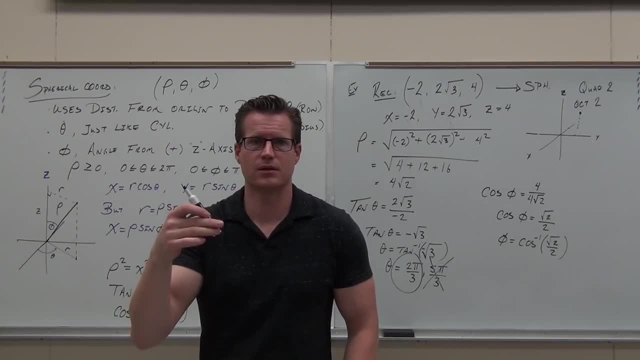 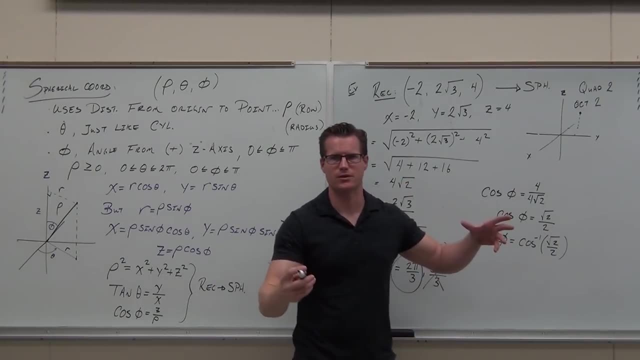 And since cosine is one to one between zero and pi, we go: hey, sweet, I love that Cosine just drops like this: It's a one to one function from zero to pi. There's only one answer. So you have to get pi over four and nothing else. 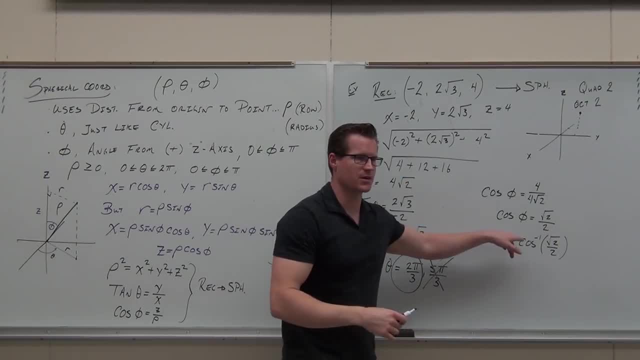 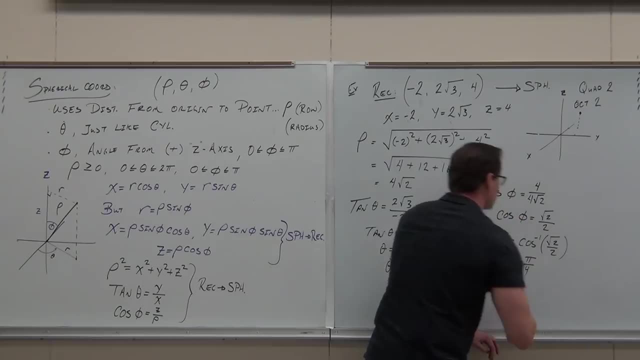 It's a 1 to 1 function, from 0 to pi. There's only one answer, So you have to get pi over 4 and nothing else. Does that make sense to you? Let's also verify that This was in question. 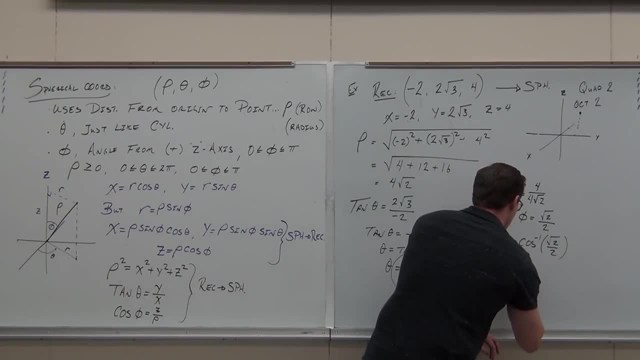 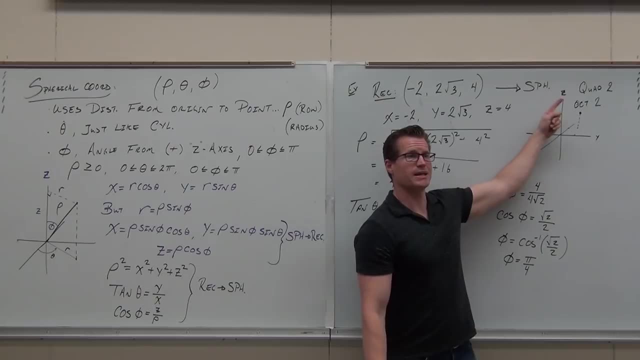 Does that make sense to you? Let's also verify that. This was in quadrant two, but it was also in octant two. It didn't go below the xy plane. This isn't going to go below the xy plane. It looks right. 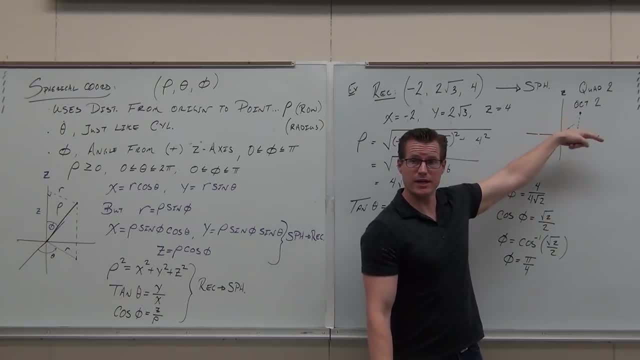 It was in quadrant 2, but it was also in octet 2.. It didn't go below the xy plane. This isn't going to go below the xy plane. It looks right. Double check your work. Have the picture in your head. 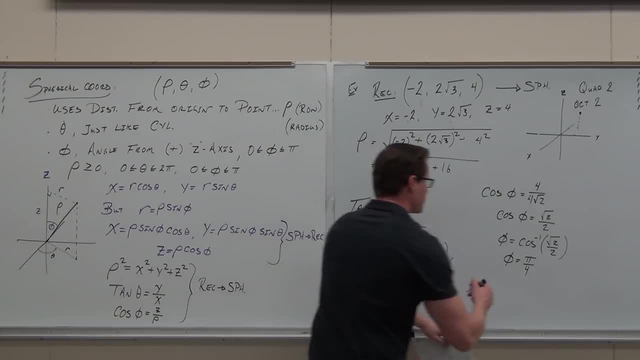 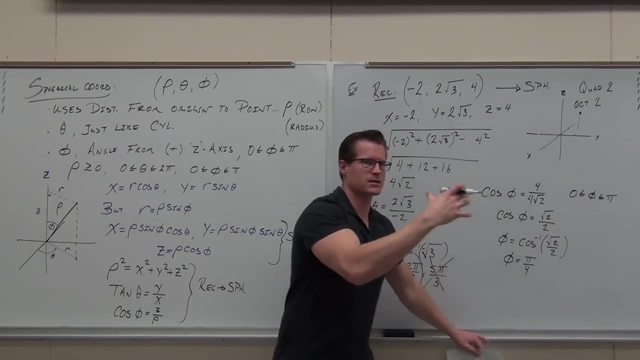 It makes it a lot nicer. And we're going to do one more thing. We go okay. So if you want the little side note here, remember that that's the interval, for phi Doesn't go outside of that- And we put the cylindrical coordinate- sorry, spherical coordinates. 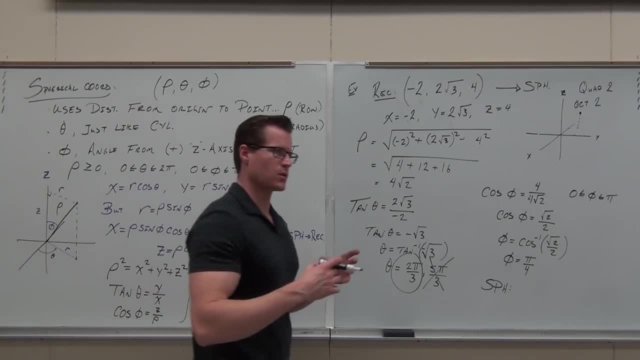 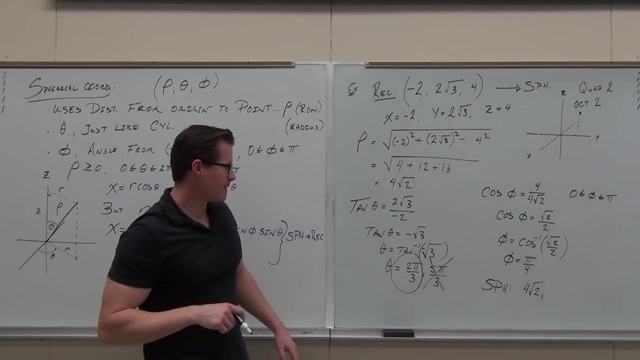 How do we start it off? What do we put first? The rho, the phi or the theta? What's first? Rho rho, rho, rho. What's the next thing that we do? Theta, theta, Theta. which is, what did we get on that one? 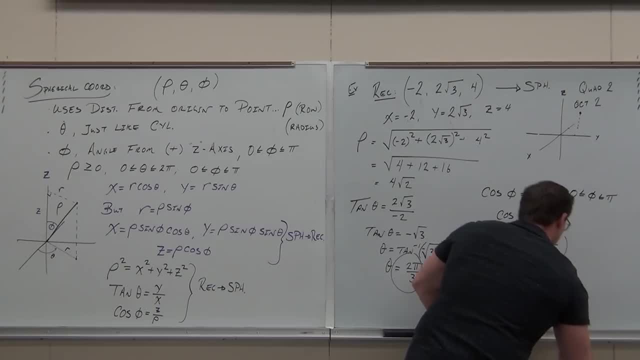 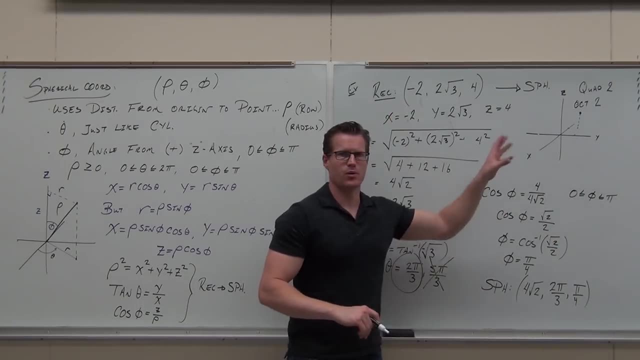 2 parts And then we wrap it up with our feet. It'll give you the same point. It's just two interpretations, and that's what we're talking about. Show your hands if you're okay with this one. We're going to take a little break right now and come back. 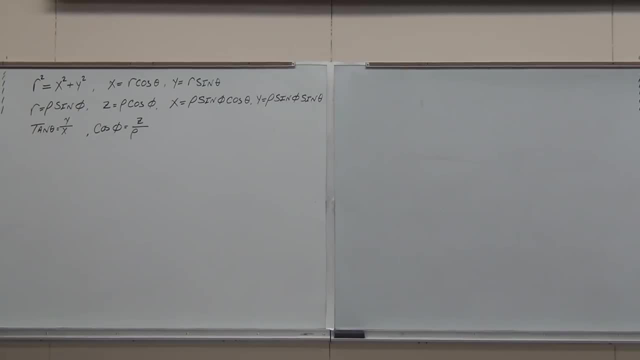 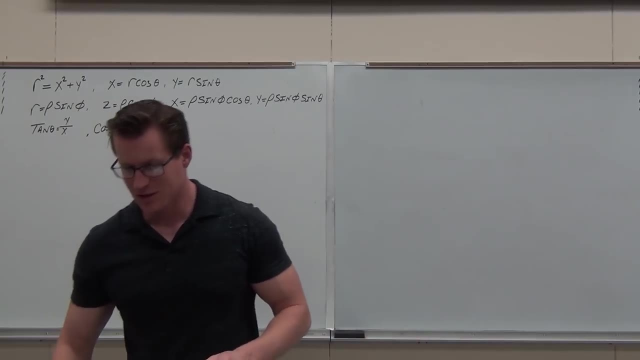 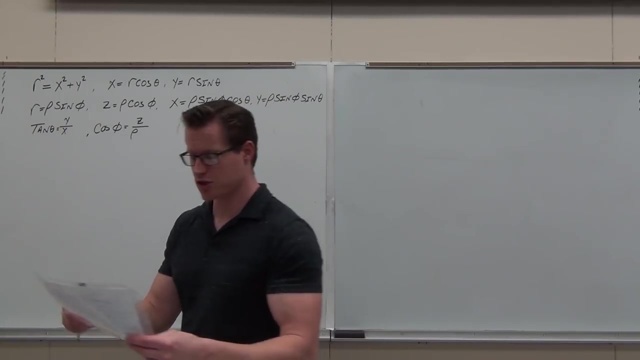 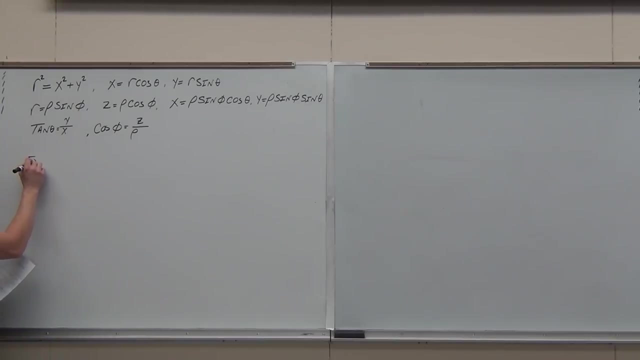 All right back at it. Some quick examples of how to go between like cylindrical and spherical, spherical and cylindrical. Honestly, these become a little easier because they're more related than, say, spherical to rectangular, which there's no relation. So, going from everything we have and use, use this stuff to do any translation. 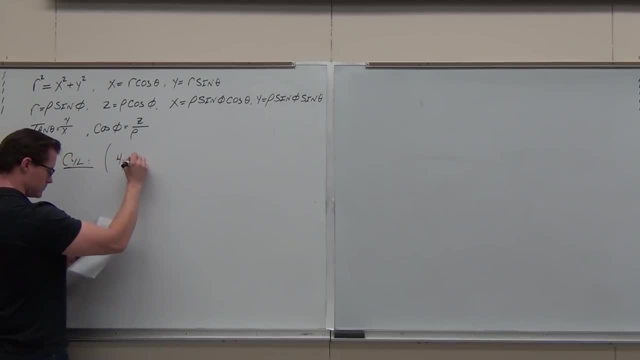 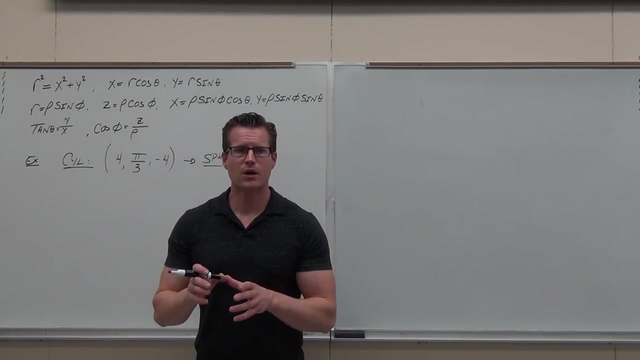 Let's talk about cylindrical And I want to go to spherical, Cylindrical to spherical, The number one thing I want you to do. please write down the stuff you know. So if I'm in cylindrical, your mind has to shift a little bit. 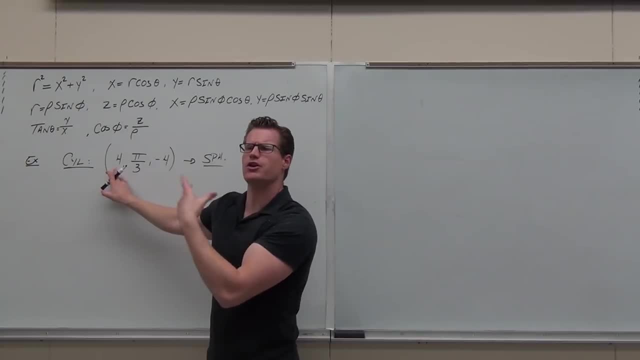 and you've got to tell me what these numbers actually mean. You've got to know what that 4 actually is. What is that 4?? That's not an X, because I'm not in rectangular. What is that 4?? That's an R. 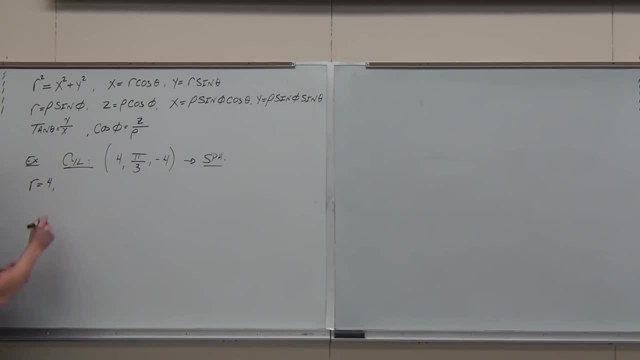 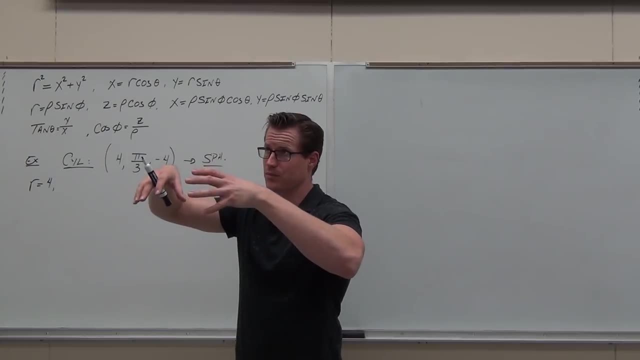 That's an R- R. Are you guys making that shift in your head? That's an R, because I have cylindrical. That's the R: the projection of the distance from the origin to the point, or the distance from the origin to the projection of the point on the XY plane. 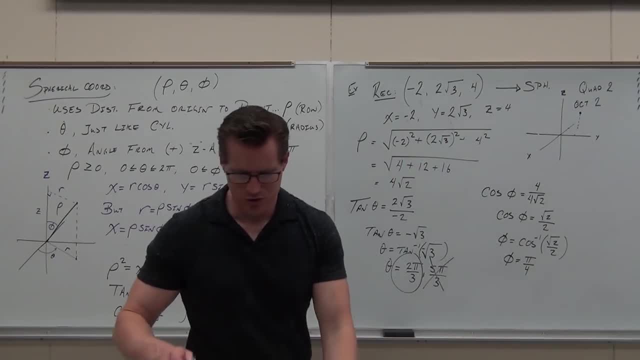 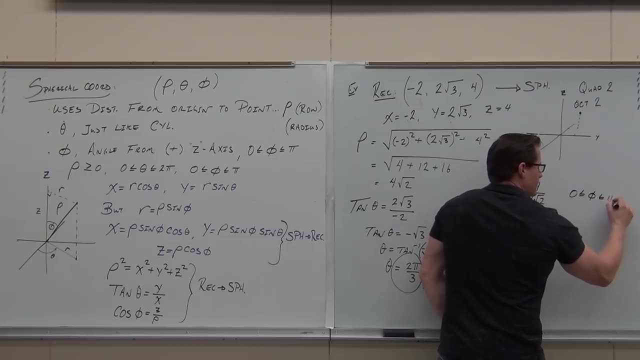 Double check your work. Have the picture in your head. It makes it a lot nicer. Then we're going to do one more thing. We go, okay. So if you want the little side note here, remember that That's the interval for feet. 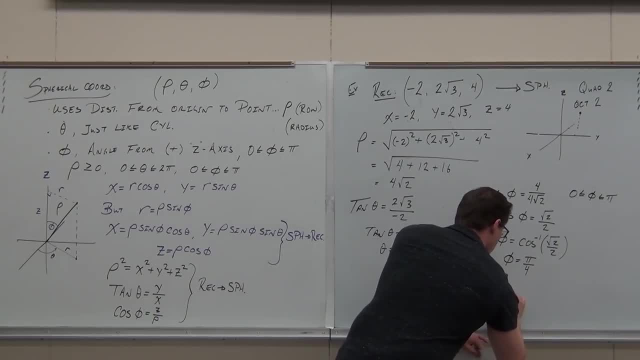 It doesn't go outside of that And we put the spherical coordinates. How do we start it off? What do we put first? The rho, the phi or the theta? What's first? What's the next thing that we do? 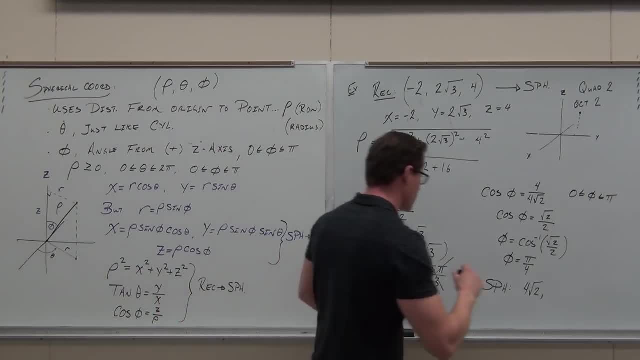 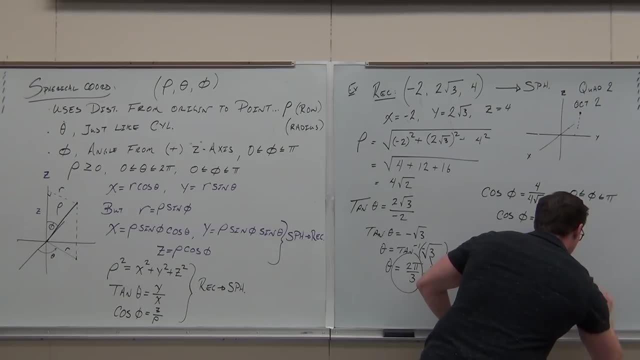 Theta, which is: what did we get on that one, Two parts, And then we wrap it up with our feet. It'll give you the same point. it's just two interpretations, and that's what we're talking about. Show your hands, if you're okay with this one. 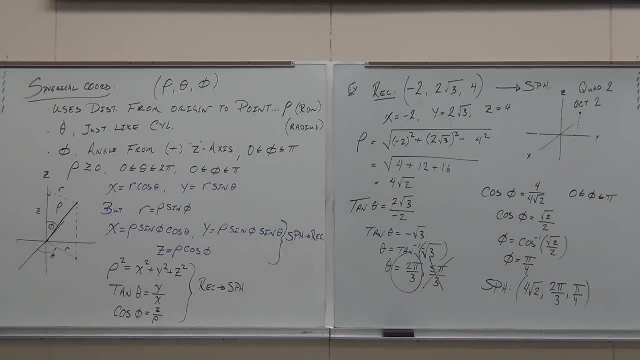 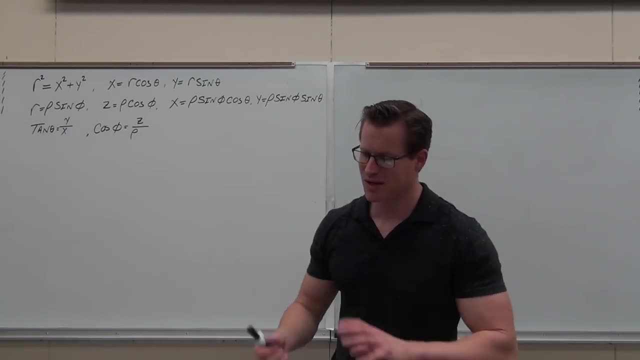 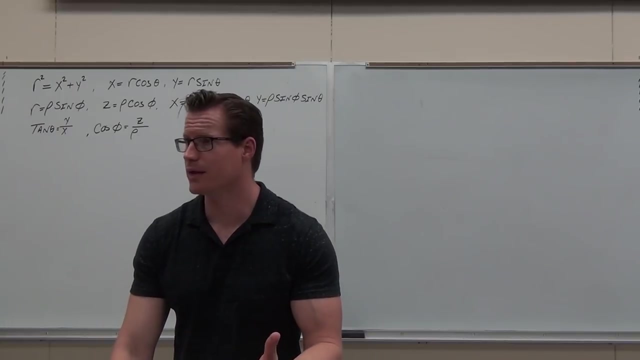 We're going to take a little break right now and come back, Okay, Okay, All right, back at it. Some quick examples of how to go between, like, cylindrical and spherical, spherical and cylindrical. Honestly, these become a little easier because they're more related than, say, spherical to rectangular. 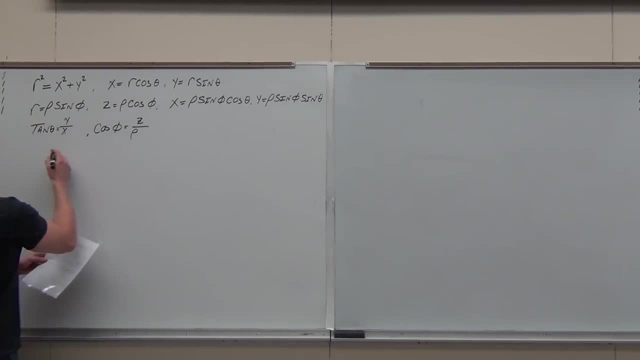 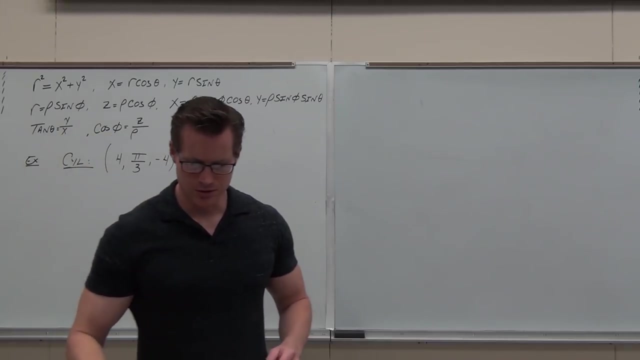 which there's no relation. So, going from everything we have and use, use this stuff to do any translation. let's talk about cylindrical And I want to go to spherical. Cylindrical to spherical, The number one thing I want you to do. 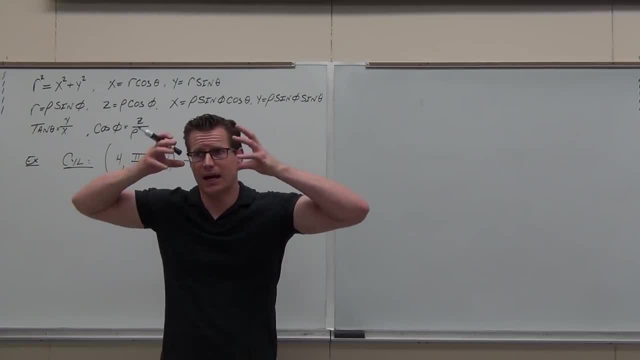 please write down the stuff you know. So if I'm in cylindrical, your mind is going to be going to cylindrical, to spherical. So if I'm in cylindrical, your mind is going to be going to cylindrical. So if I'm in cylindrical, your mind has to shift a little bit. 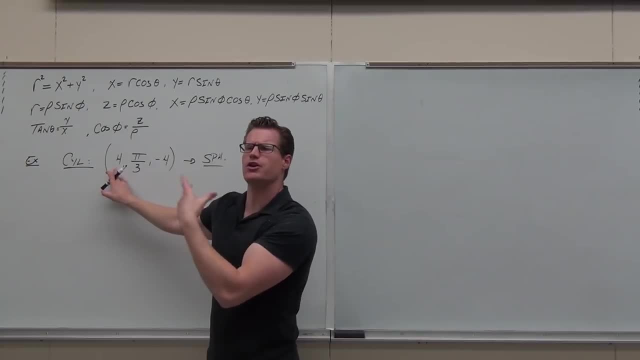 and you've got to tell me what these numbers actually mean. You've got to know what that four actually is. What is that four That's not an X, because I'm not in rectangular. What is that four That's an R? 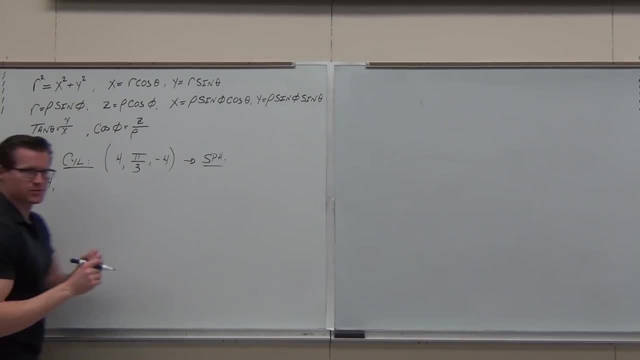 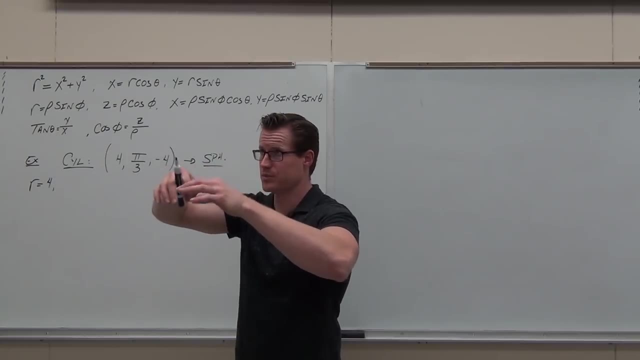 That's an R. Are you guys making that shift in your head? That's an R, because I have cylindrical. That's the R: the projection of the distance from the origin to the point or the distance from the origin to the projection of the point and the XY plane. 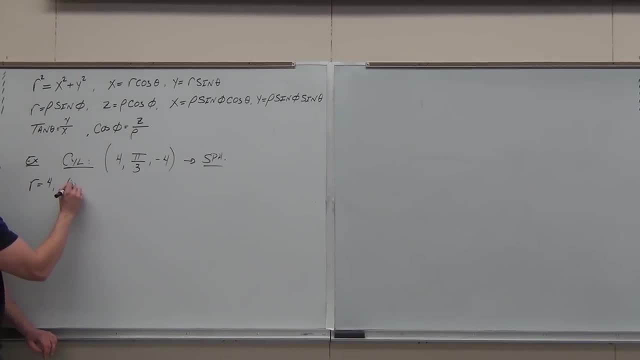 What is what's that? What's that? Yeah, And since we are in cylindrical, what's that? Z? Z, We're in cylindrical, so that is still Z. I'm going to see if you're paying attention right now. 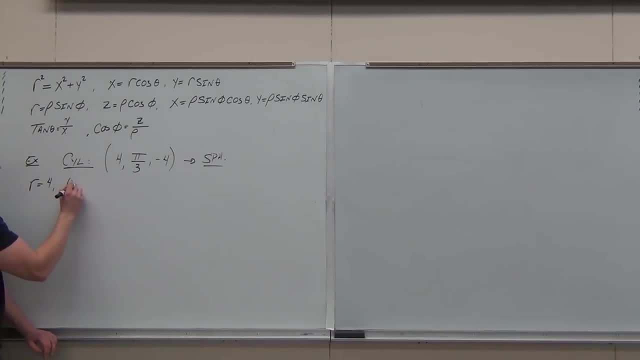 What is what's that? What's that There? And since we're in cylindrical, what's that Z? Z, We're in cylindrical, so that is still Z. I'm going to see if you're paying attention right now. 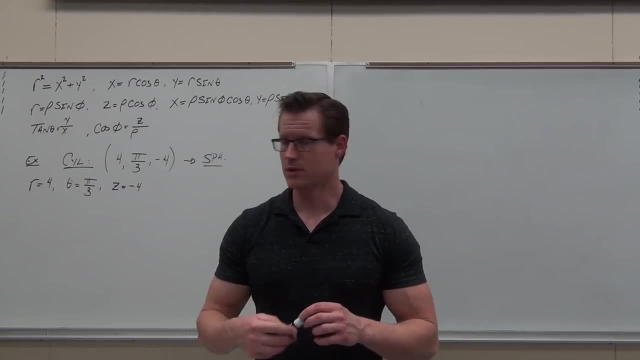 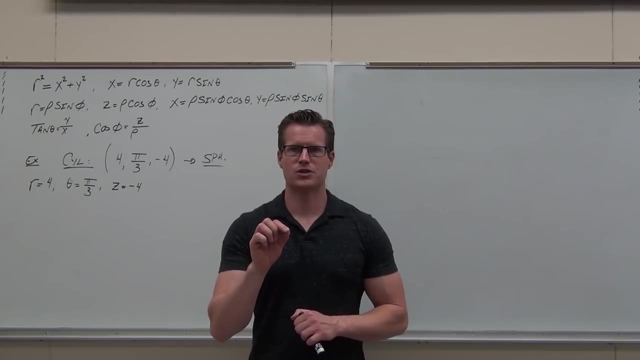 We're about to change to spherical. I want to know. yes, we are. I have had a report for sure. What I want to know is your phi. Is your phi going to be more than or less than pi over 2?? 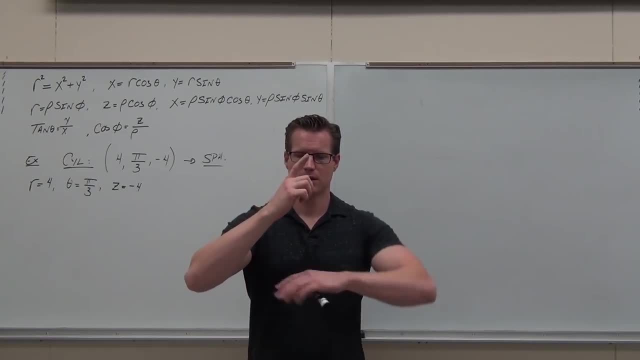 More than Negative Z, More than here's the XY plane, more than, or less than, pi over 2?. More than It's got to be, more than- because I'm going into the negative part- It's got to cross the XY plane. 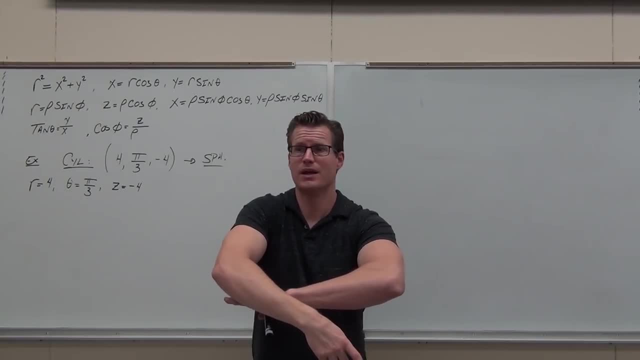 It's got to be more than pi over 2.. It's got to be more than pi over 2.. And I'm not sure if you're okay with that one. Are you sure That's what's happening? So let's translate it. 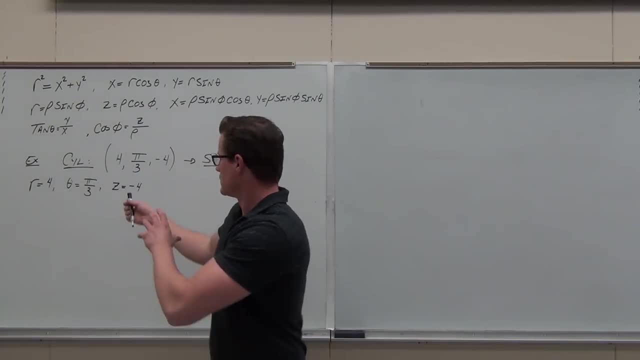 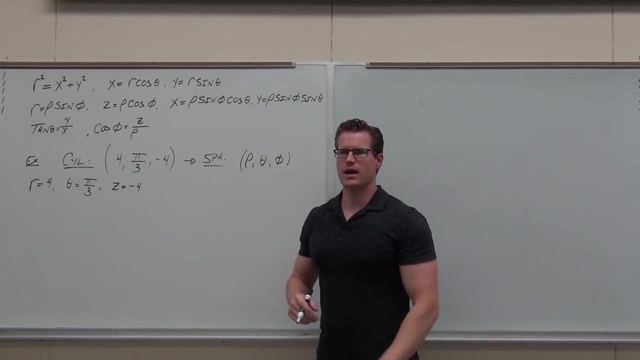 Can we go from R's and Z's and Theta's into stuff like: well, what I want, I want rho, I want Theta and I want theta, I want theta, I want theta And I want B? Which one of these guys do we already have there? 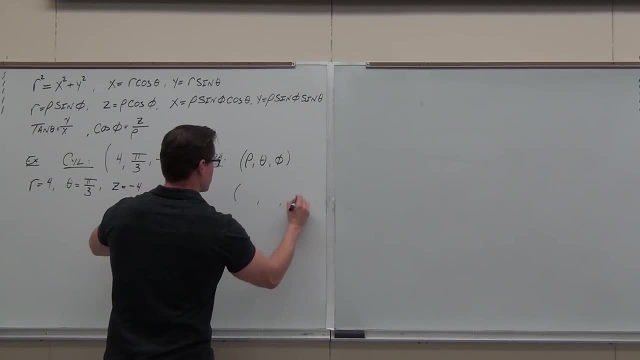 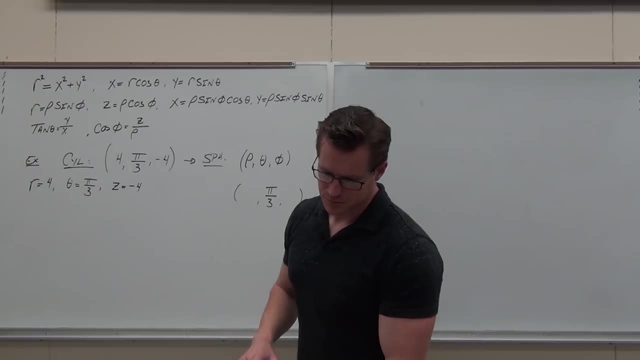 So I already know that spherical, I'm going to get pi over 3, for sure. I know that's going to be there. Now, as far as the rest of it, you're going to be using some of the same stuff. 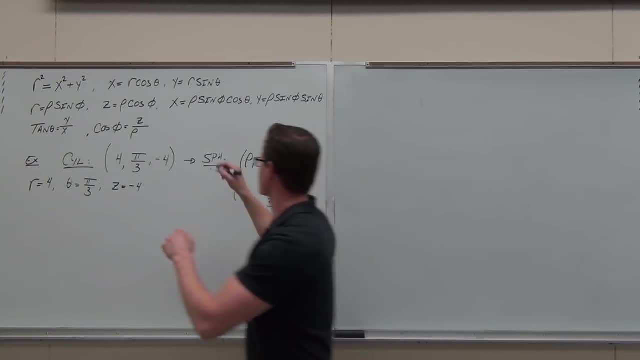 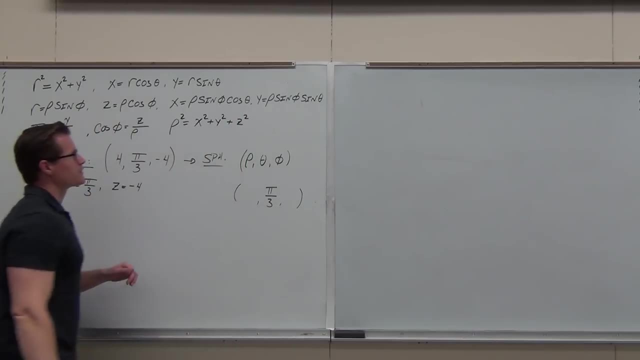 but there's going to be pieces that relate these two. Oh, I forgot one, sorry. There's going to be things that relate this. So, for instance, you go: well, maybe I need rho. That's the only thing that's solved for rho. 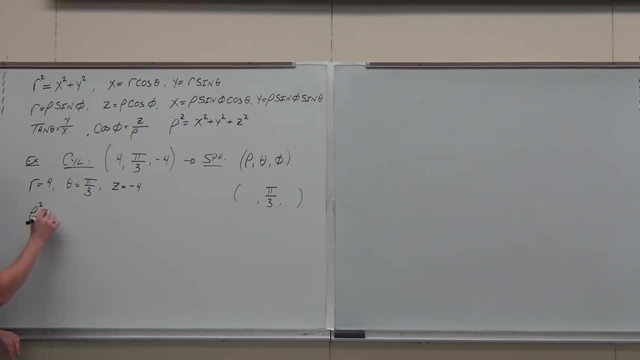 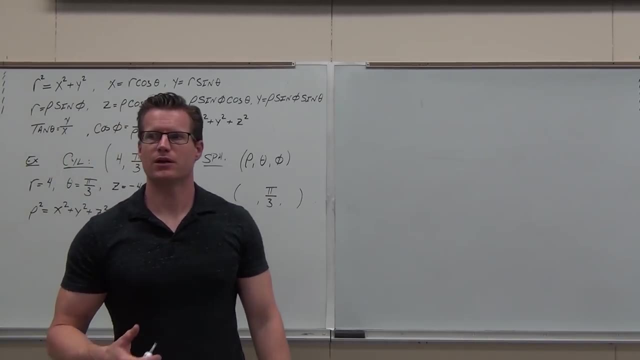 Let's use that. However, I just finished telling you a lot of this stuff. it gets easier when you're doing this. for this reason, Check this out. Yeah, I know that this is X squared plus Y squared plus Z squared, but think carefully on it. 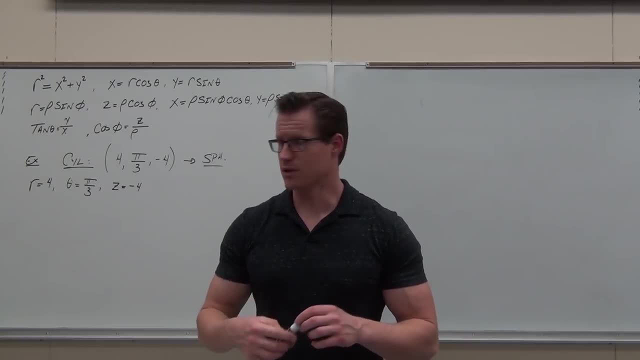 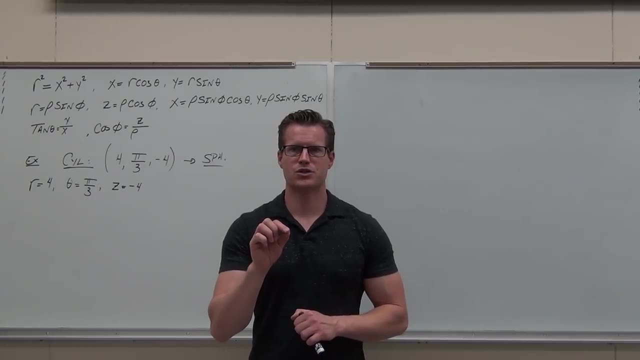 We are about to change to spherical. I want to know. yes, we are. I have had a report, We are for sure. What I want to know is your phi. Is your phi going to be more than or less than pi over 2?? 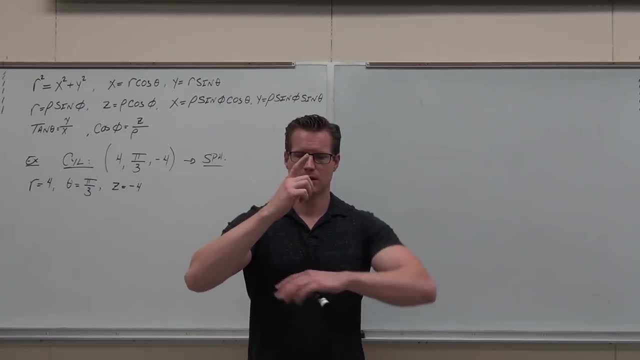 More than Negative Z, More than here's the XY plane, more than, or less than, pi over 2?. More than It's got to be, more than- Because I'm going into the negative part- it's got to cross the XY plane. 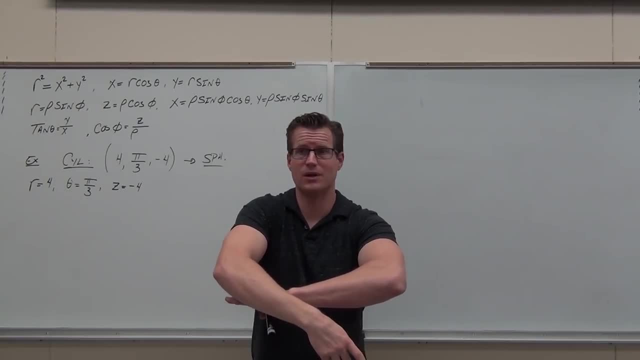 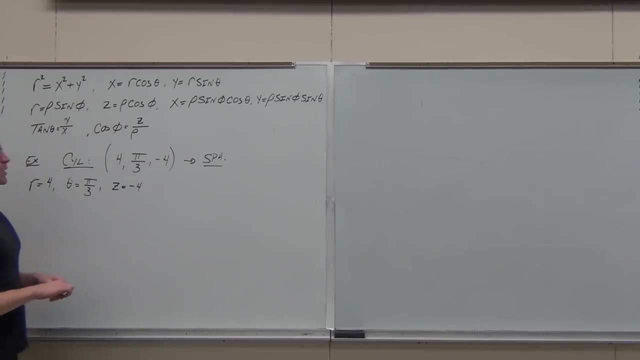 It's got to be more than pi over 2.. It's got to be more than pi over 2.. Head nod, if you're okay with that one. Are you sure That's what's happening? So let's translate it. Can we go from? 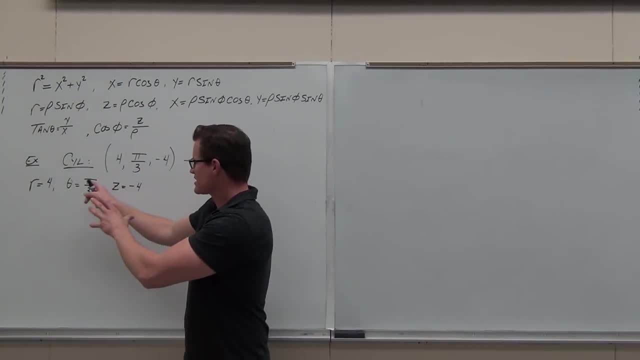 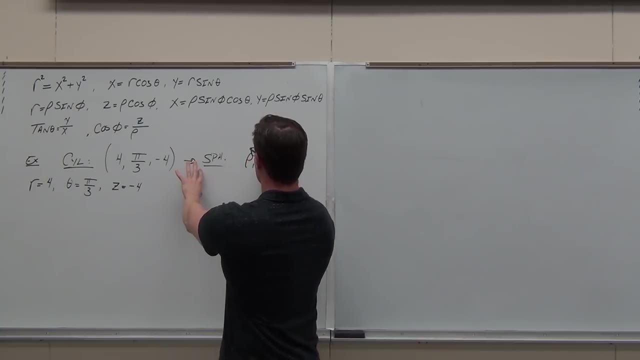 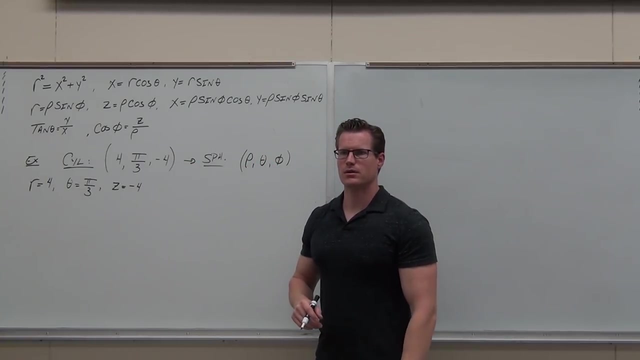 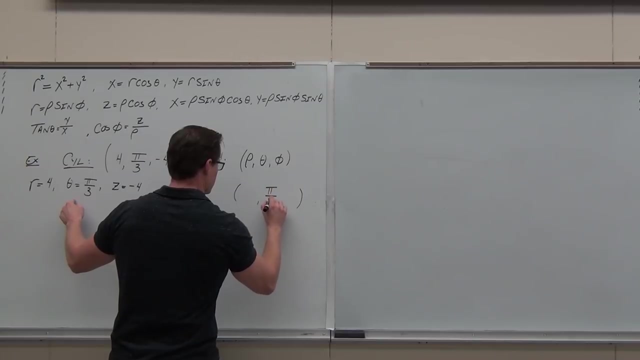 R's and Z's and Theta's into stuff like: well, what I want, I want rho, I want Theta and I want B. Which one of these guys do we already have There? So I already know that, spherical, I'm going to get pi over 3 for sure. 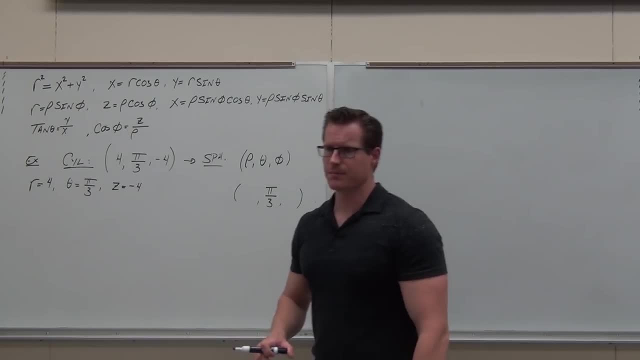 I know that's going to be there Now. as far as The rest of it, you're going to be using some of the same stuff, But there's going to be pieces that relate these two. Oh, I forgot one, Sorry. 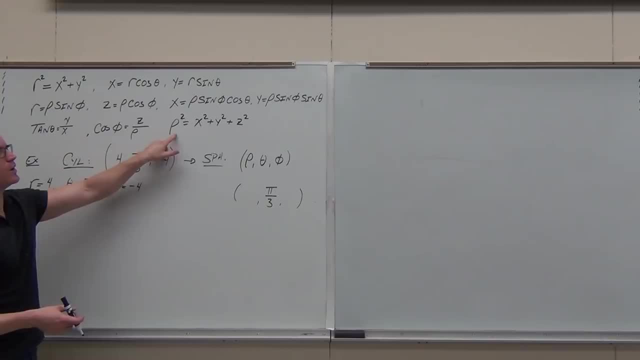 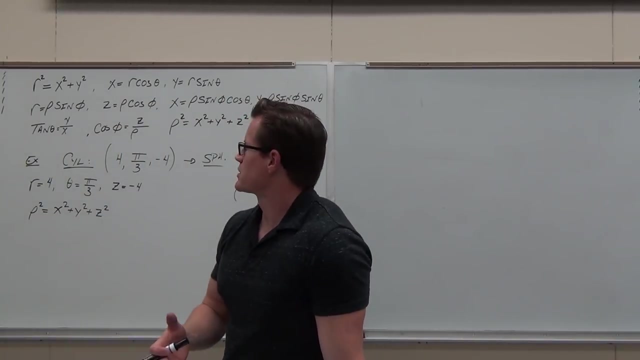 There's going to be things that relate this. So, for instance, you go: well, maybe I need rho. That's the only thing that's solved for rho. Let's use that. However, I just finished telling you A lot of this stuff. it gets easier when you're doing this. 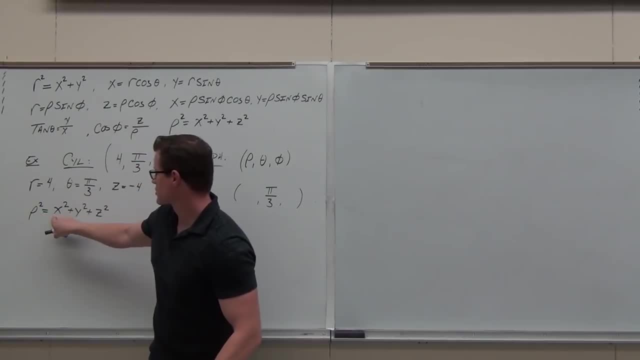 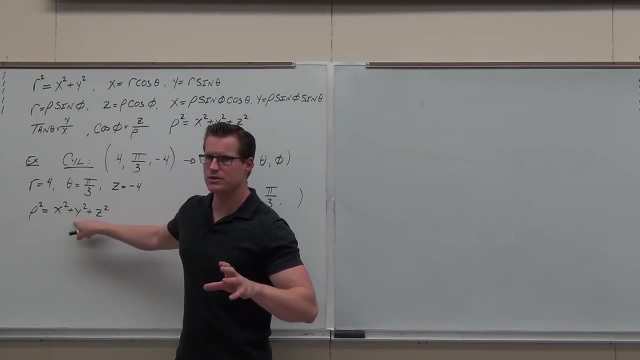 For this reason, Check this out. Yeah, I know that this is X squared plus Y squared plus Z squared, But think carefully on it. What is X squared plus Y squared? R to R? That's R squared. So this formula gets a little easier. 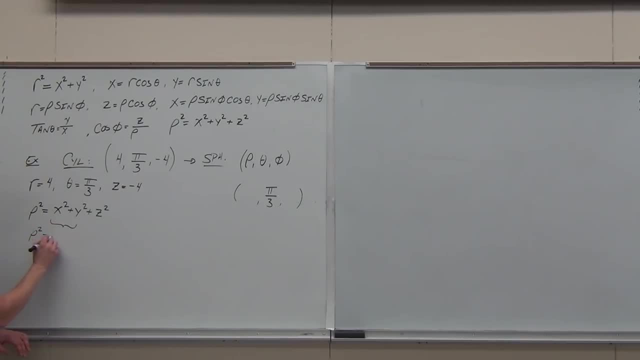 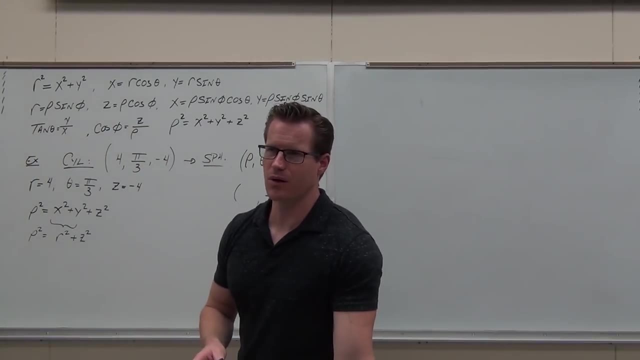 This really becomes R squared plus Z squared. Hey, do you know an R? What's the R? Quickly, what's the R? R to R? Do you know a Z? Can you plug those things in? Let's plug them in. 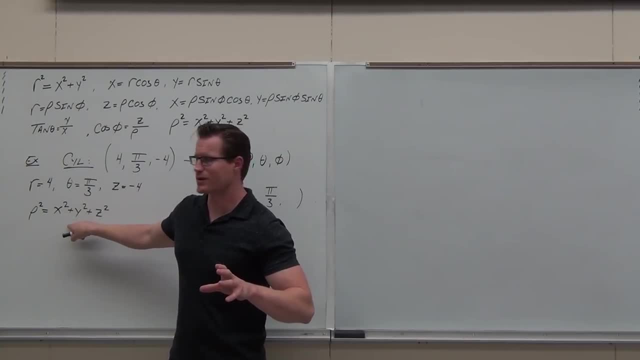 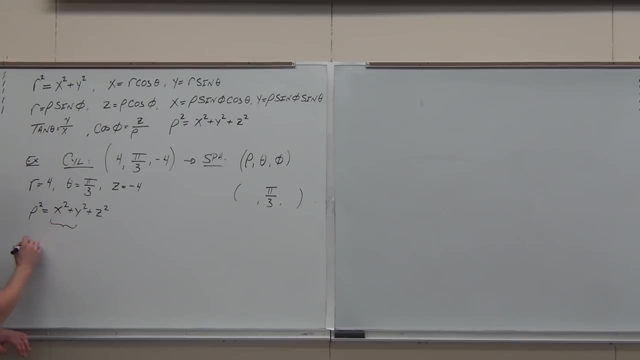 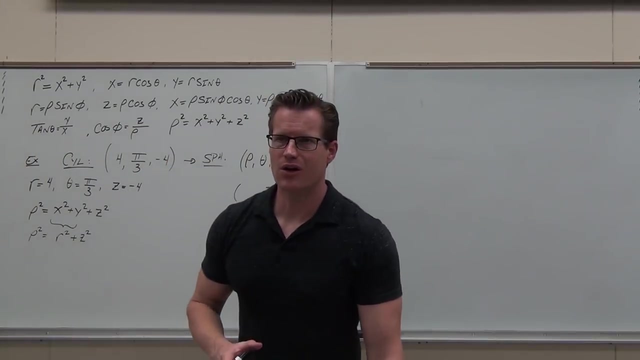 What is X squared plus Y squared? That's R squared, That's R squared. So this formula gets a little easier. This really becomes R squared plus Z squared. Hey, do you know an R? What's the R, Quickly, what's the R? 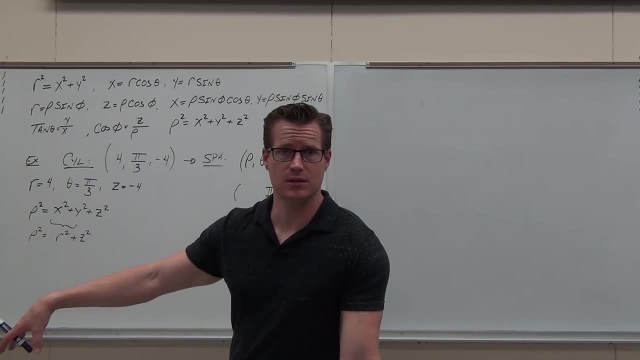 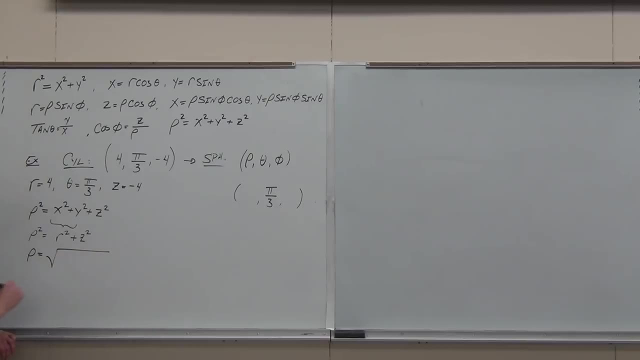 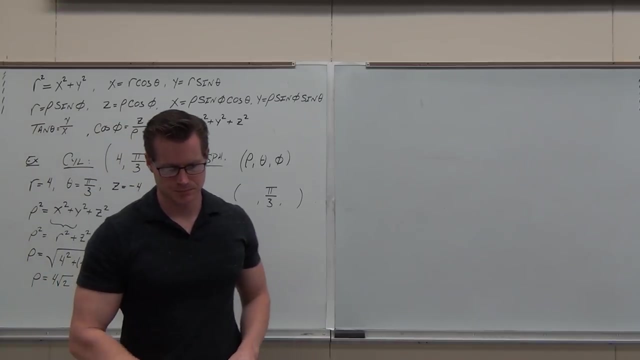 R, R. Do you know a Z? Can you plug those things in? Let's plug them in. Let's solve for phi. OK, I got 4 root 2.. You guys get the 4 root 2?? Yeah, 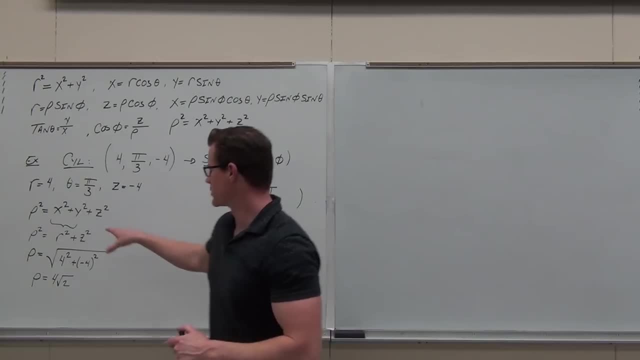 We can have 4 root 2.. I know I'm doing a lot of math fast in my head, but I want to know if you understand where this stuff is coming from. so that man, you don't. Some of you guys aren't even paying attention to math. 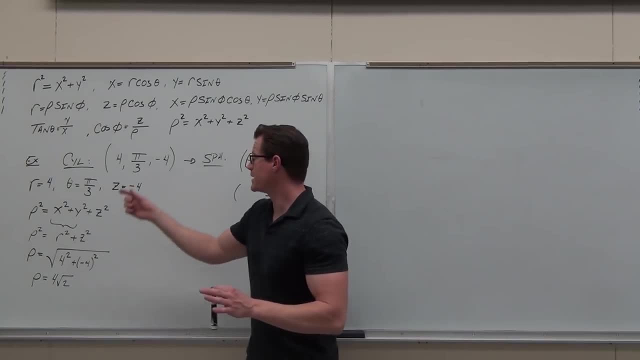 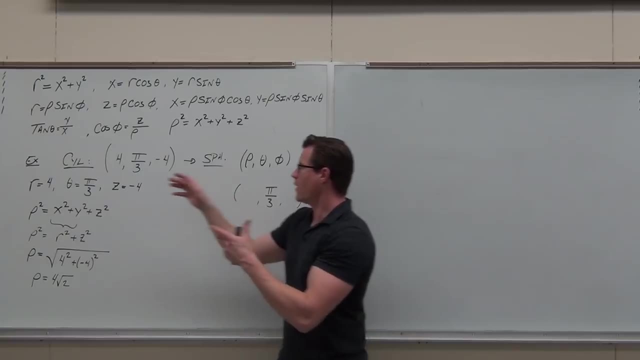 I want to know if I'm getting through to you, to you to understand that the theta that is not going to change between cylindrical and spherical, that that's going to be there. i have the same stuff, the r and the z. yeah, we're going to have. 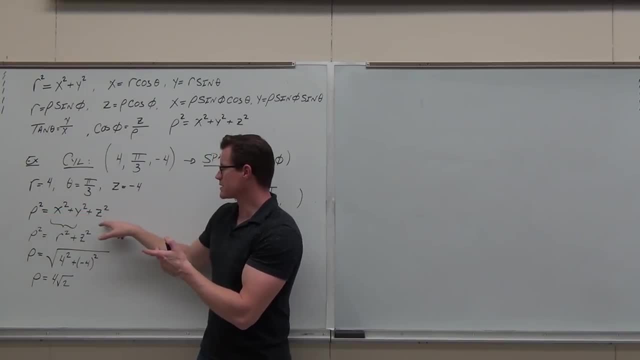 to use that. and one way we use that: if rho squared is defined as this: well, x squared plus y squared is r squared. use that. that makes it even nicer. man, you gotta plug in two numbers. plug in the four, plug in the negative four. square them, add them, take a square root. it's going to be four root. 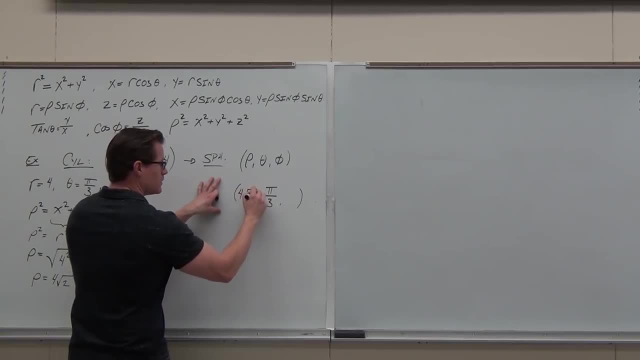 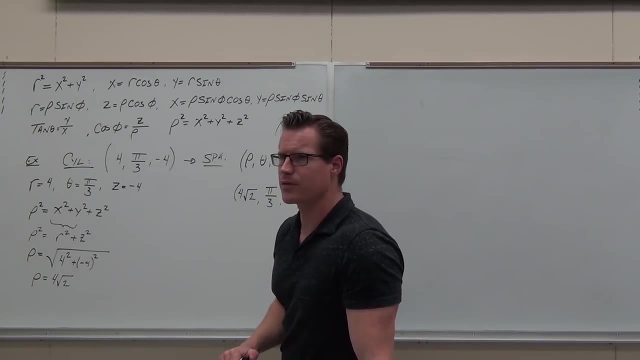 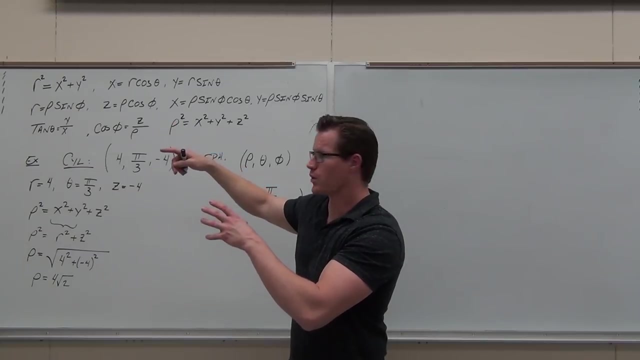 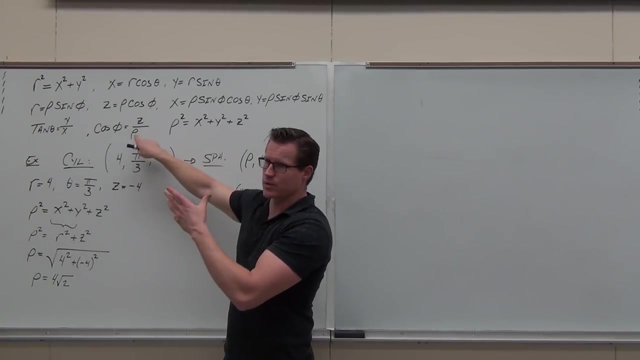 two. so already calculated that one. now, what about the phi? there's really only one thing up here that deals with phi and being able to solve for it. and well, two things. you could use one of two things. you could do cosine phi z over rho, which that's the one i prefer. you could actually do that one. 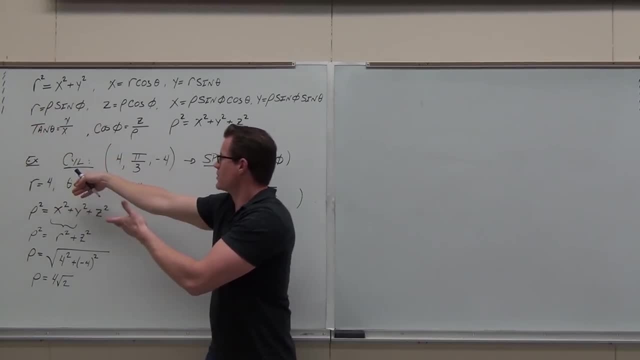 because you could do: sine of phi equals r over rho squared, and since you're given r, either one of these is going to work just fine. it's just the other way of looking at that right triangle that we already talked about. does that make sense to you? pick one. 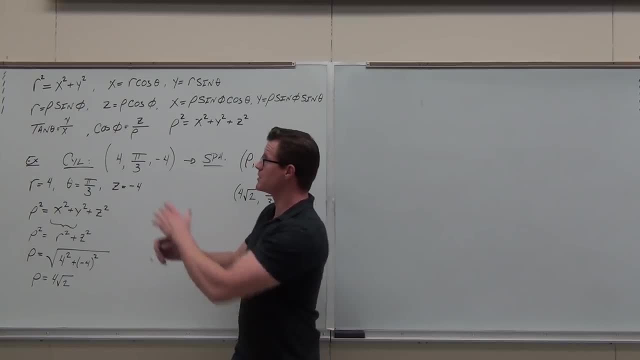 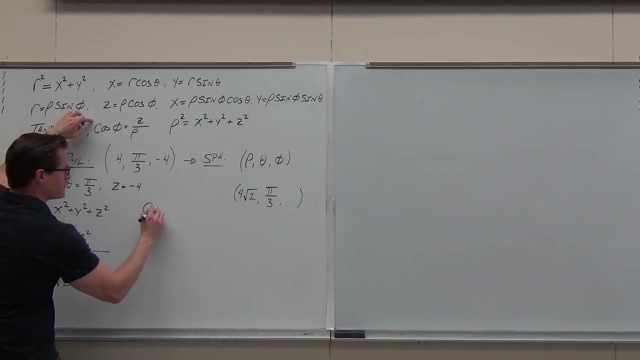 i don't care, as long as you're getting something that's going to solve the, i'm going to use this one, but as long as you're getting something that's going to let you solve for phi based on the information you're given. so this says: 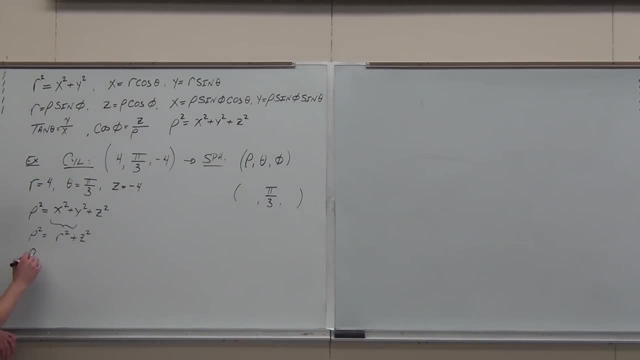 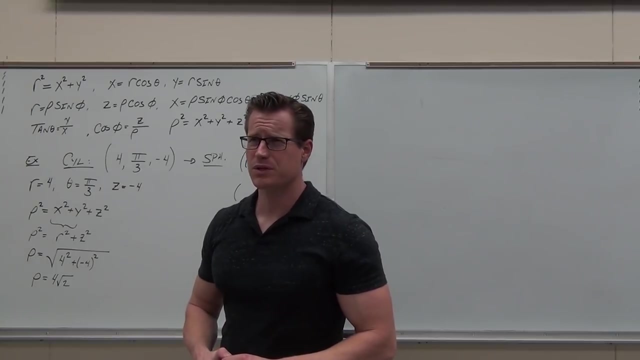 Let's solve for phi. Let's solve for phi. I've got four root two. You guys get the four root two. Yeah, we can't have four root two. I know I'm doing a lot of math fast in my head, but I want to know if you understand where this stuff is coming from. 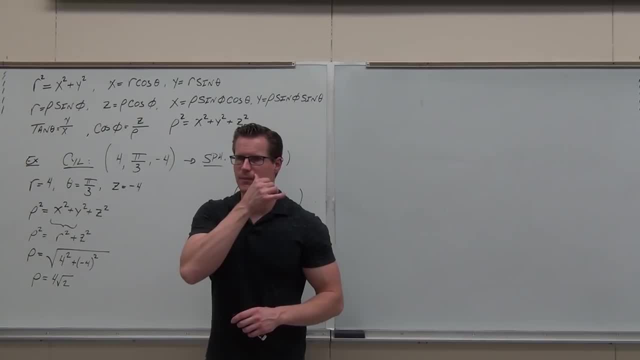 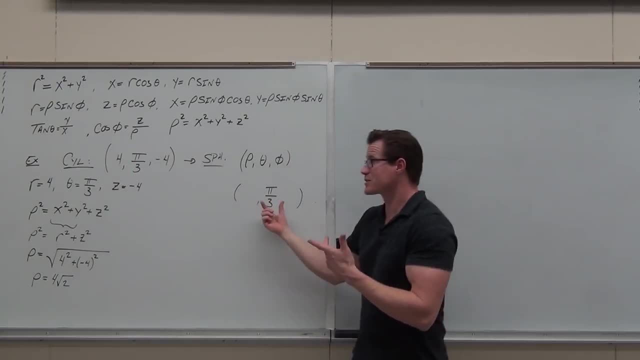 So the man, you don't. so you guys aren't even paying attention to math. I want to know if I'm getting through to you. Do you understand that the theta that is not going to change between cylindrical and spherical, That's going to be there? 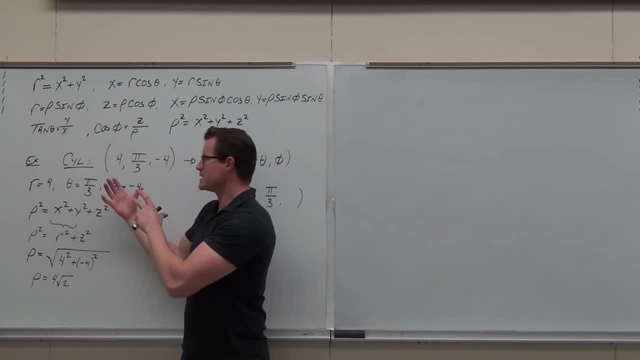 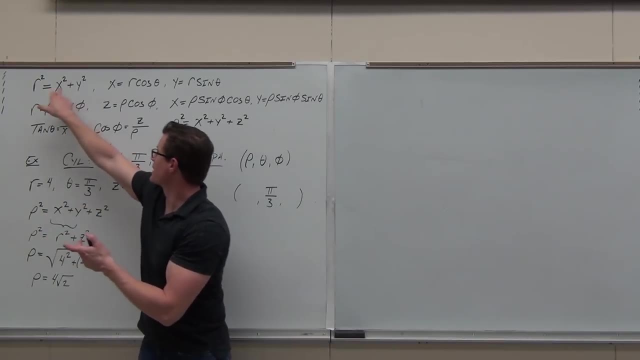 I have the same stuff: The R and the Z. yeah, we're going to have to use that. And one way we use that: if rho squared is defined as this, well, X squared plus Y squared is R squared. Use that, that makes it even nicer. 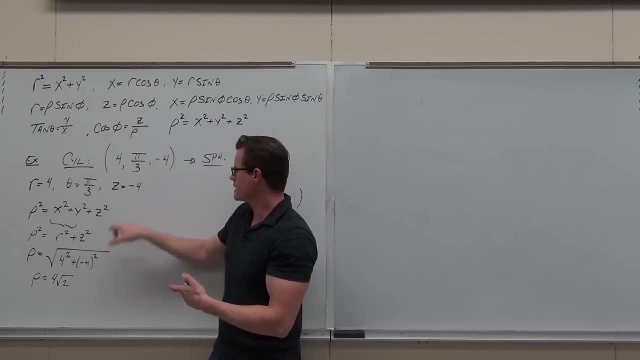 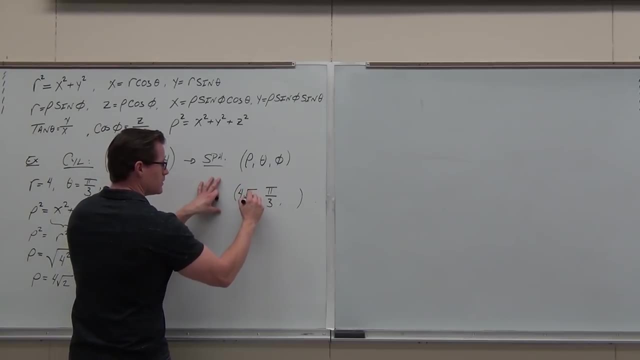 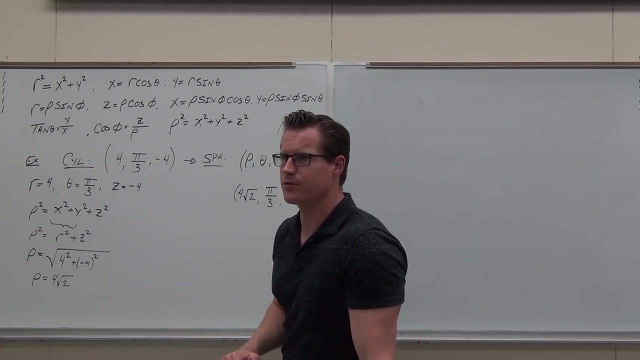 Man, you've got to plug in two numbers. Plug in the four, plug in the negative four, square them, add them, take a square root. It's going to be four root two. so I've already calculated that one. Now what about the phi? 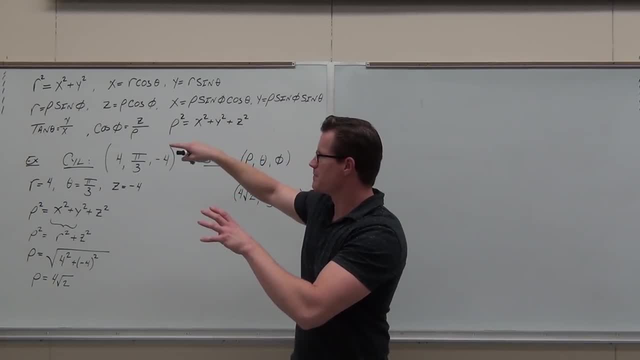 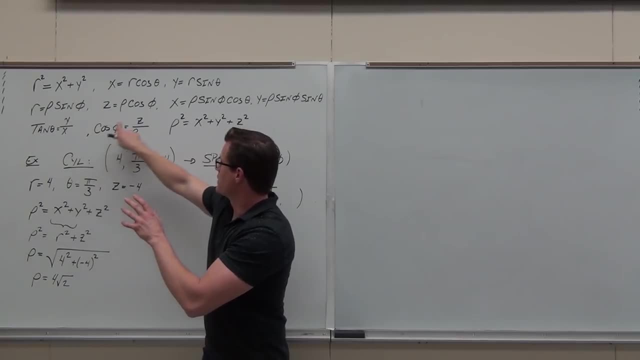 There's really only one thing up here that deals with phi and being able to solve for it. And well, two things You could use. one of two things You could do: cosine phi Z over rho, which that's the one I prefer. 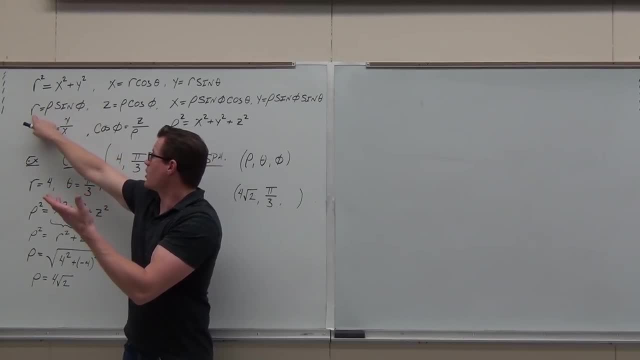 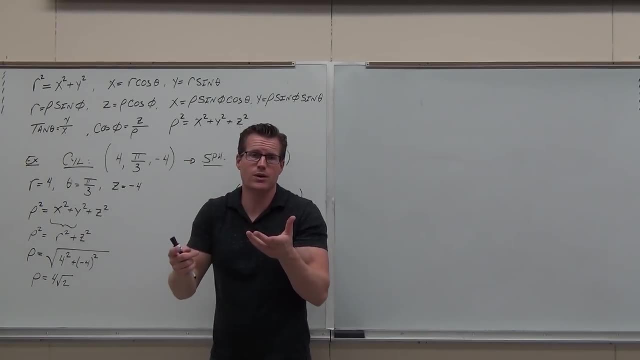 You could actually do that one, because you could do: sine of phi equals R over rho, And since you're given R, either one of these is going to work just fine. It's just the other way of looking at that right triangle that we already talked about. 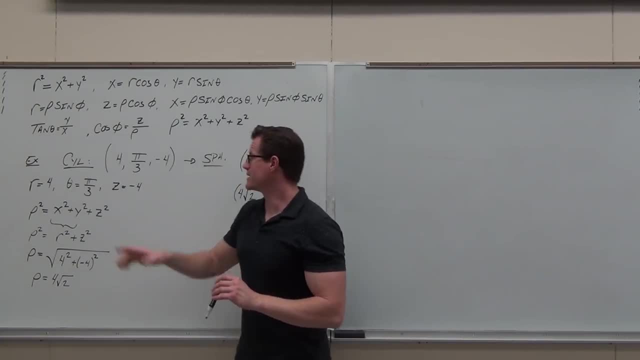 Does that make sense to you? Pick one, I don't care. As long as you're getting something that's going to solve for, I'm going to use this one, But as long as you're getting something that's going to let you solve for phi based. 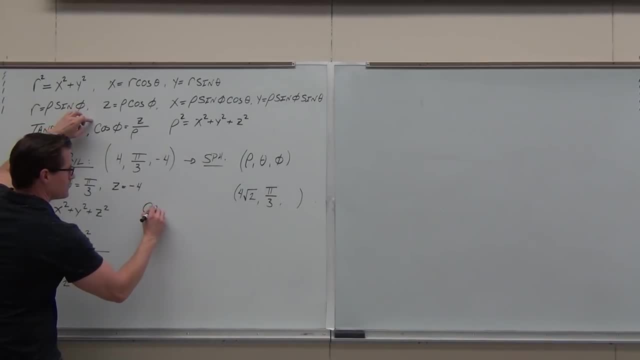 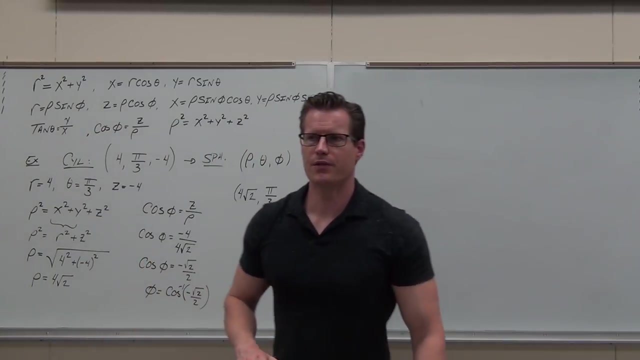 on the information you're given, So I'm going to take this one. So this says negative 4 over. hey, I just found the rho. We talked about how to find phi. You got to find rho first. Can anyone out there tell me on the interval of 0 to pi? 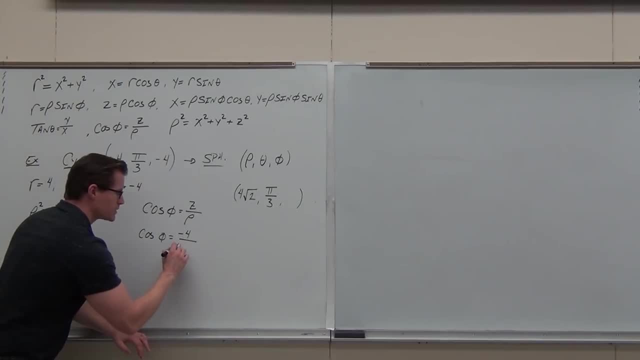 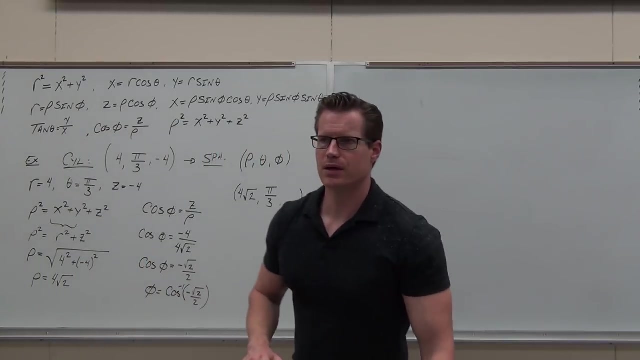 negative four over. hey, i just found the rho. we talked about how to find phi. you got to find rho first. can anyone out there tell me on the interval of zero to pi, because we cannot go outside of that. it's got to be from zero to pi. 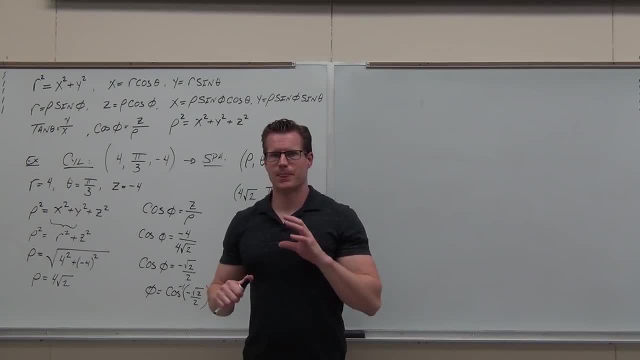 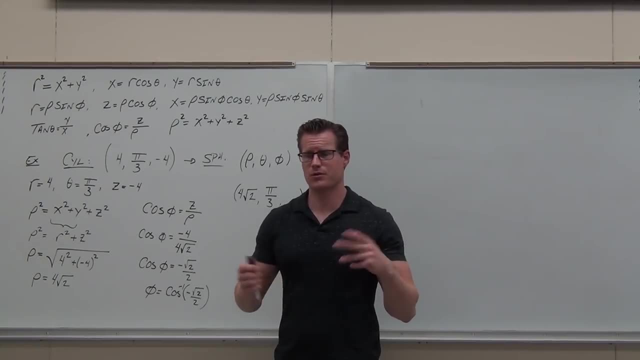 it's got to be from zero to pi. What would give us cosine of? what angle would give us negative root? 2 over 2? I know it's an over 4, because these are all over 4.. Is it pi over 4 or 3? pi over 4?? 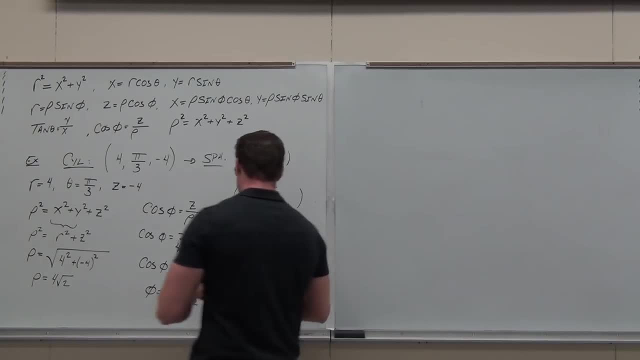 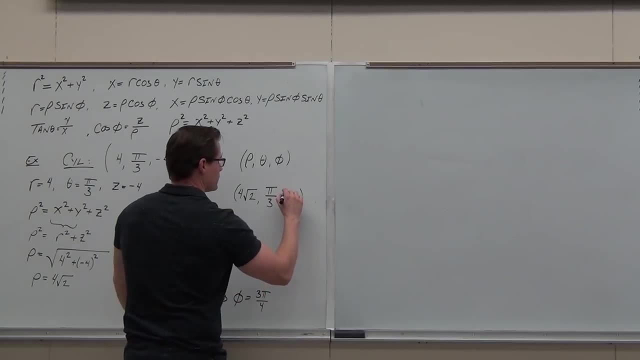 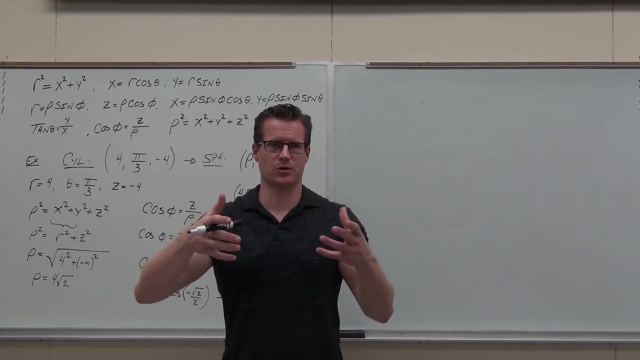 Because there's only those two options: 3 pi over 4.. It's 3 pi over 4.. It's kind of nice because we don't have those two options. There's no way to make a mistake. You can't go outside of 0 to pi for phi. 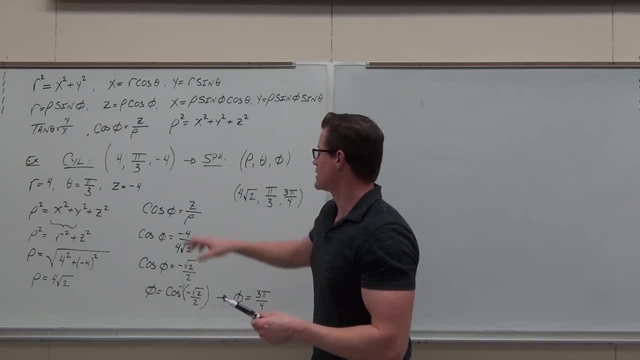 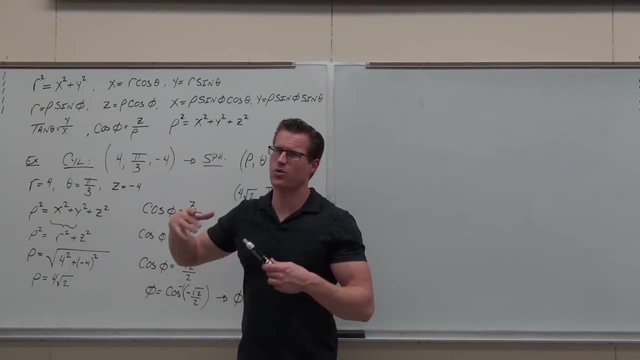 So there's only one choice there and because theta's already given, there's no choice there either, It's literally given to you. That's pretty nice, because that's kind of the hard part. right is knowing quadrant, match up the quadrant, pick the right angle. 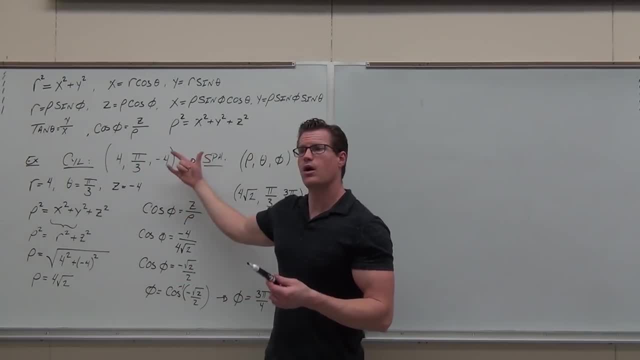 You don't have to do that between cylindrical and spherical or spherical to cylindrical, because theta's always given for both of those things. You guys see what I'm talking about. Show of hands, if this made sense, If you're okay with it. 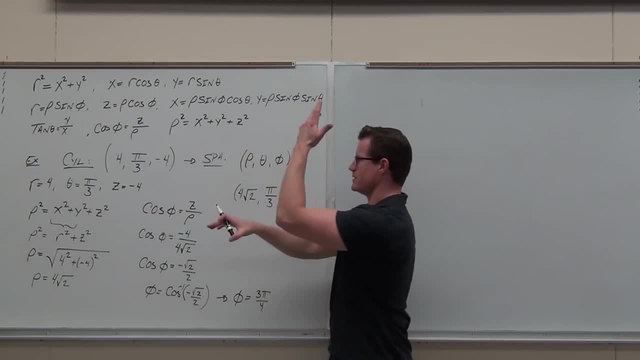 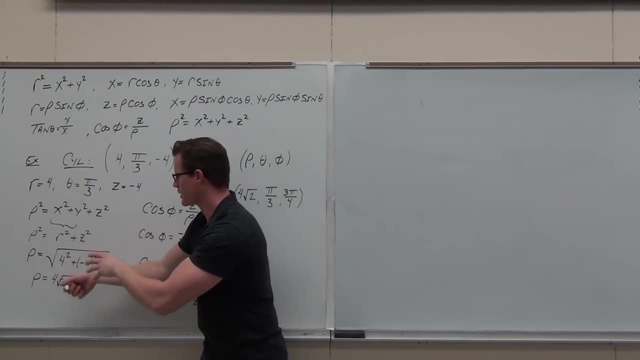 So we had r yeah, we had z yeah, theta given. no problem, We used theta, We used our. any formula that you can, as long as it relates to this information. This changes to r squared plus z squared. plug it in: we get 4 root 2.. 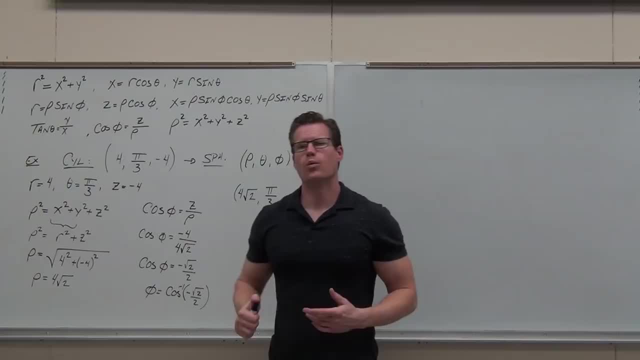 because we cannot go outside of that. it's got to be from 0 to pi. what would give us cosine of what angle would give us negative root? 2 over 2? I know it's an over 4, because these are all over 4.. 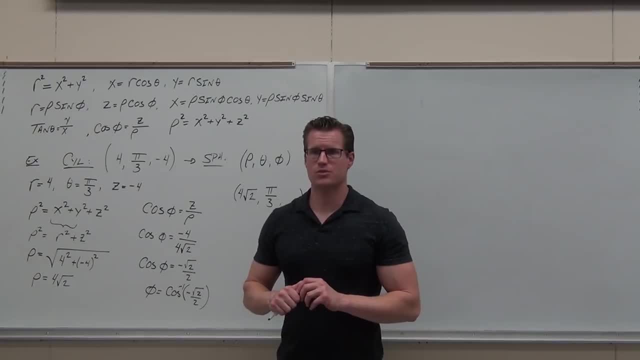 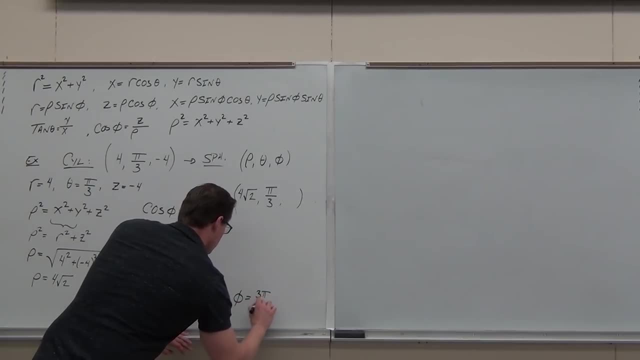 Is it pi over 4 or 3 pi over 4?? Because there's only those two options: 3, pi over 4.. It's 3 pi over 4.. It's kind of nice, because we don't have those two options. 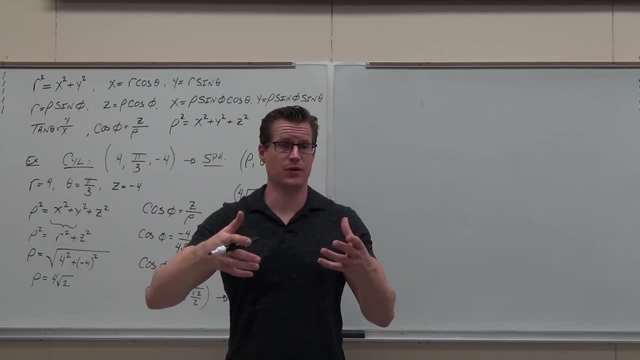 There's no way to make a mistake. You can't go outside of 0 to pi for phi. So there's only one choice there. And because theta's already given, there's no choice there either. It's literally given to you. 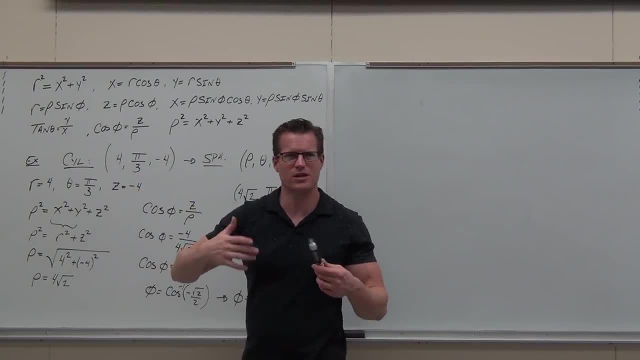 That's pretty nice, because that's kind of the hard part, right is knowing quadrant, match up the quadrant, pick the right angle. You don't have to do that between cylindrical and spherical or spherical to cylindrical, because theta's always given for both of those things. 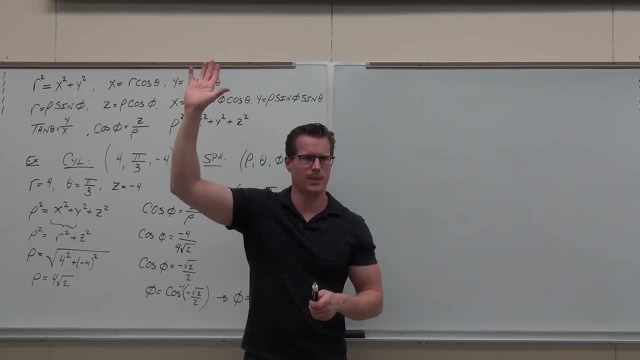 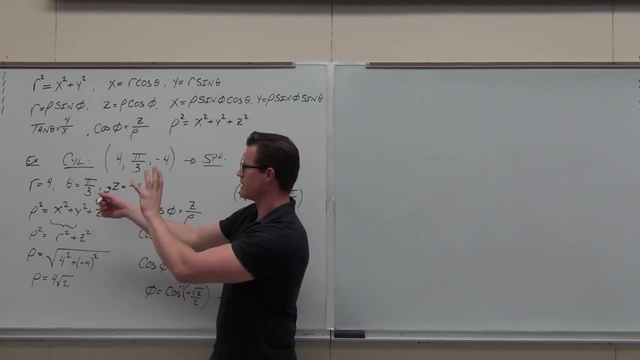 You guys see what I'm talking about. Chauvin's a very good example. This makes sense if you're okay with it. So we had r, yeah. we had z, yeah, theta given. no problem, We use our any formula that you can. 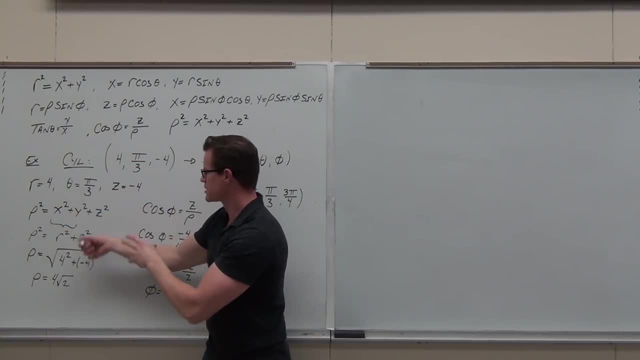 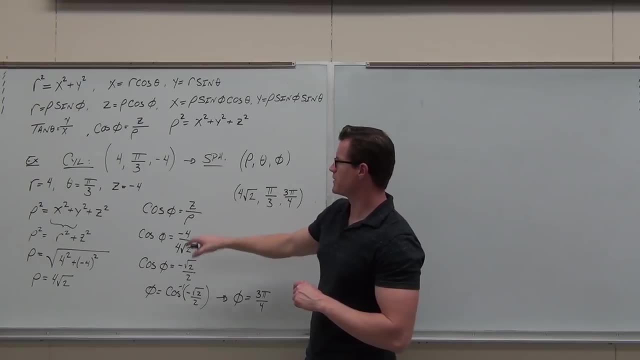 as long as it relates to this information. This changes to r squared plus z squared. Plug it in. we get 4 root 2.. After you find this, use either this or that one. Either one. I chose the cosine phi. 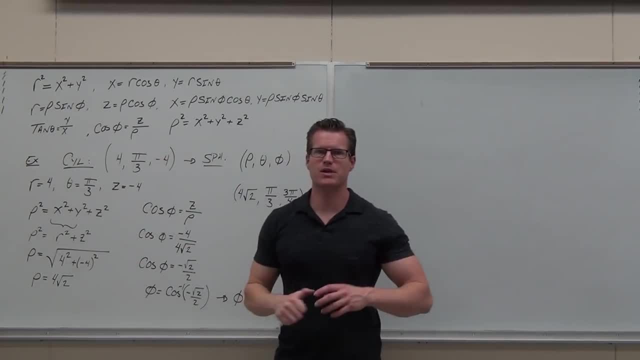 We had our z. You have to find rho first in either case, but then it becomes just a. you look at the inner circle. make sure for phi that you do not go outside of 0 to pi, and then you're going to have that correct. 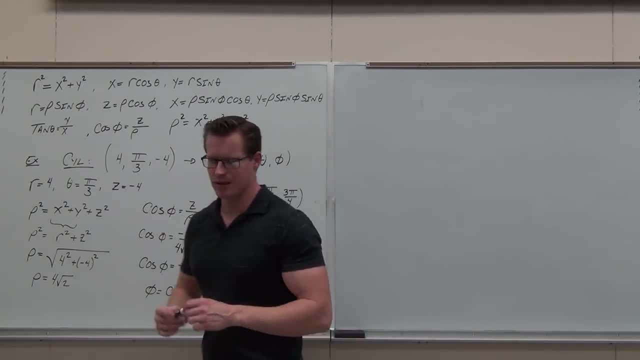 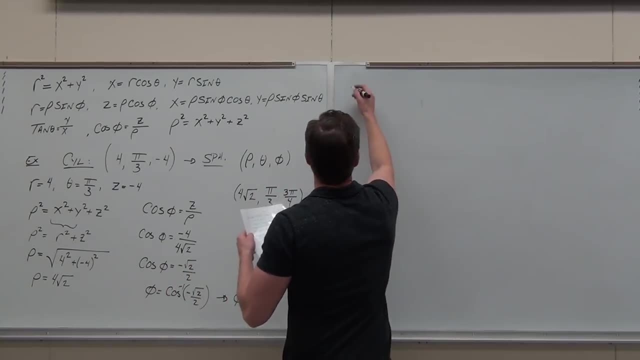 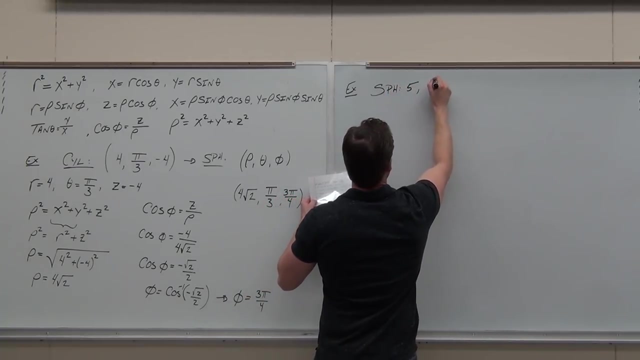 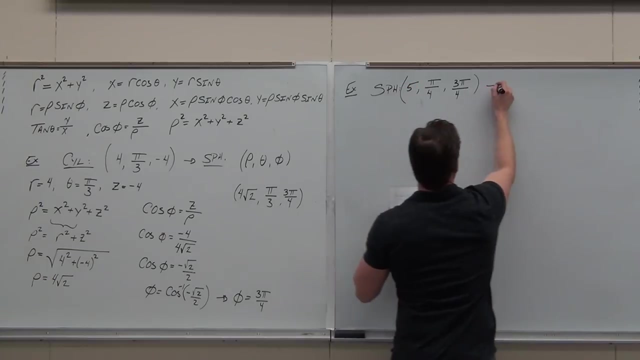 So that's our spherical coordinate. for that point, Let's go backwards. Let's go from spherical to cylindrical. Okay, the two ideas I want you to do is: you're going to have to do the same thing over and over again, Okay. 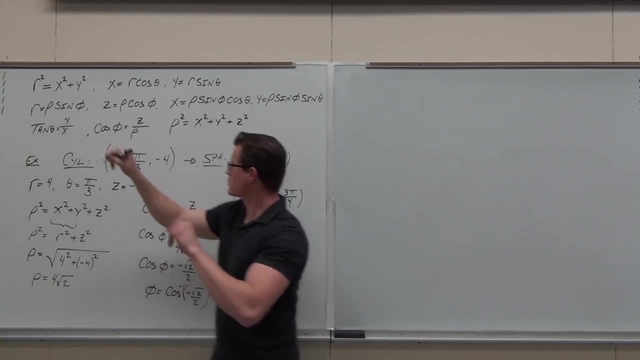 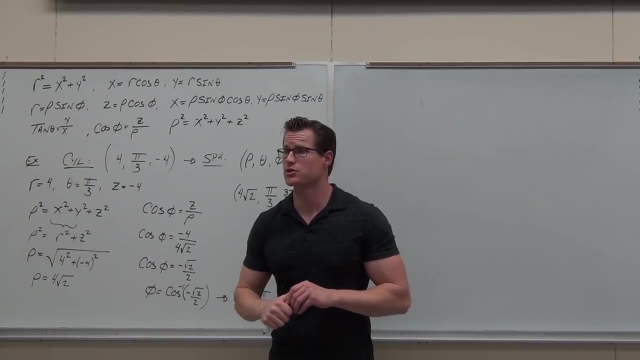 After you find this, use either this or that one, either one. I chose the cosine phi. We had our z. You have to find rho first in either case, but then it becomes just a. you look at the inner circle. make sure for phi that you do not go outside of 0 to pi. 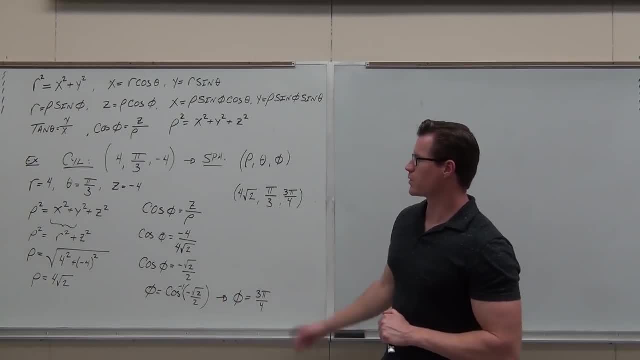 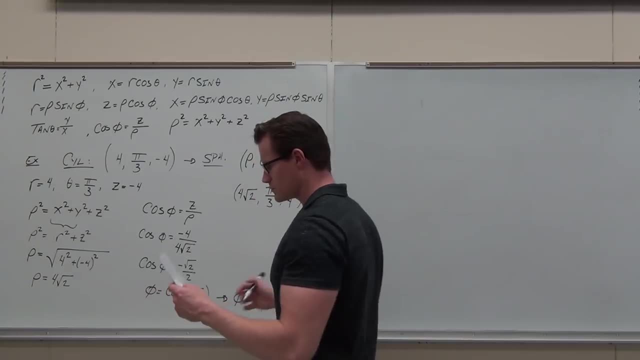 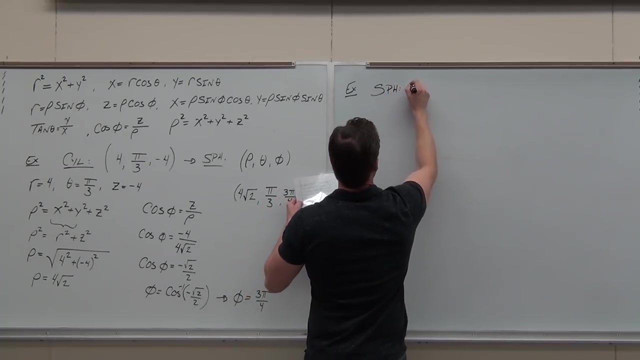 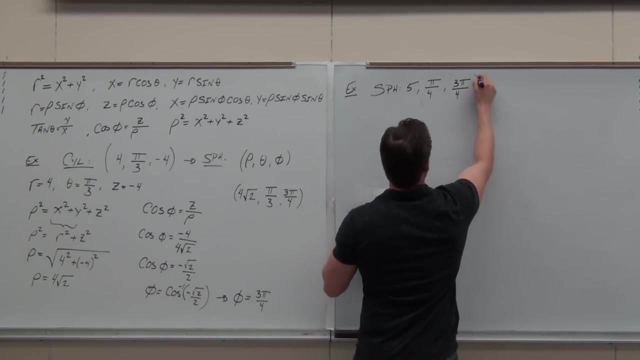 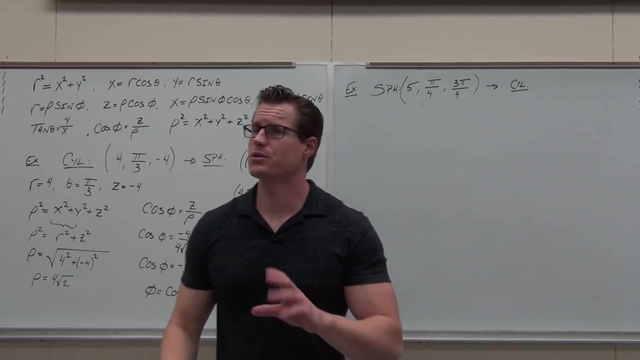 and then you're going to have that correct. So that's our spherical coordinate. for that point, Let's go backwards. Let's go from spherical to cylindrical. Okay, the two ideas I want you to do. The first idea is: if ever I give you a type of coordinate system, 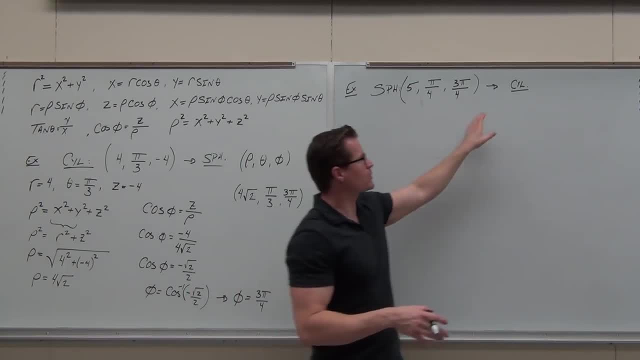 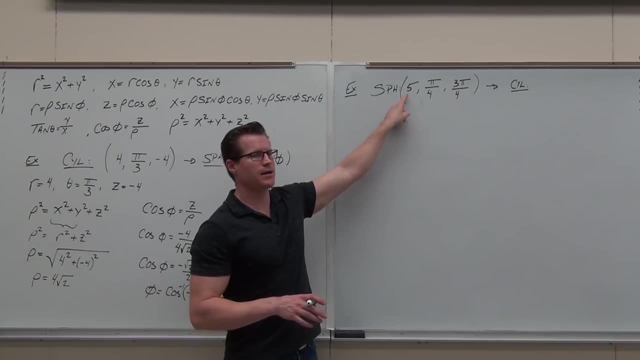 I want you to write down what we have Like, write down what it is and then also now write down what you need. So right now I want to know, if I give you spherical goodness gracious, what does that number mean? 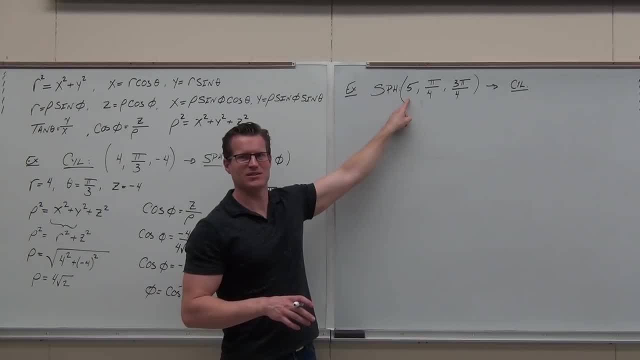 What is the 5?? Rho, Rho, rho, r x. I don't know, it's probably one of those. Which? what's this one? Rho, Rho, that's a rho, because spherical starts with rho. 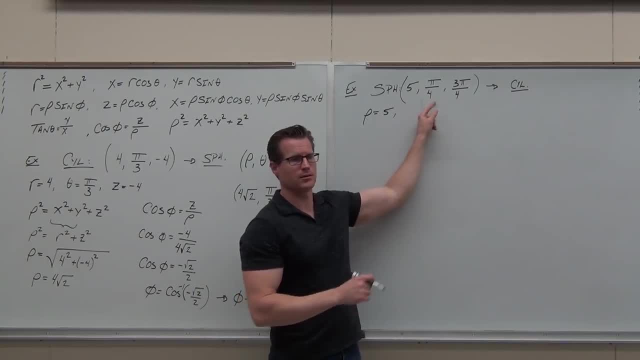 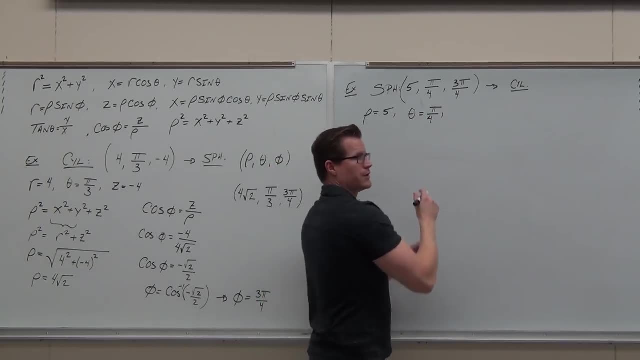 Everyone in class right now. what's that? Rho Rho, Rho, rho r x and that one V V. If you've got an angle last, you're probably in spherical. It's the only one that does that. 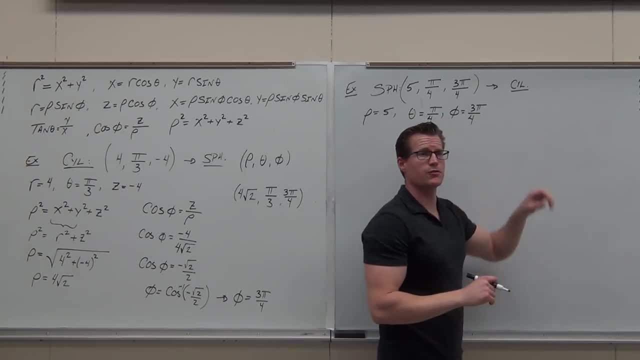 Okay, now right-siders, just you guys. I want to know what you need for cylindrical to work. How is it organized? I know it's three things, but what are those three things? What do we start with? R? 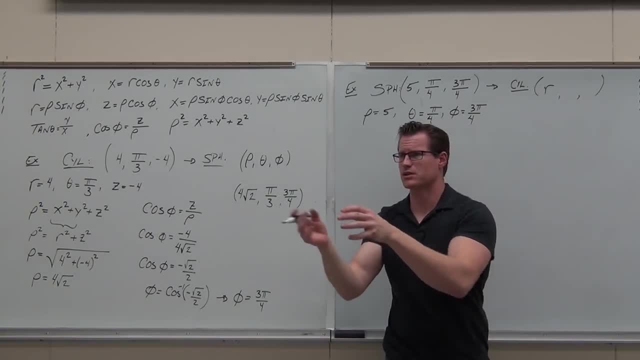 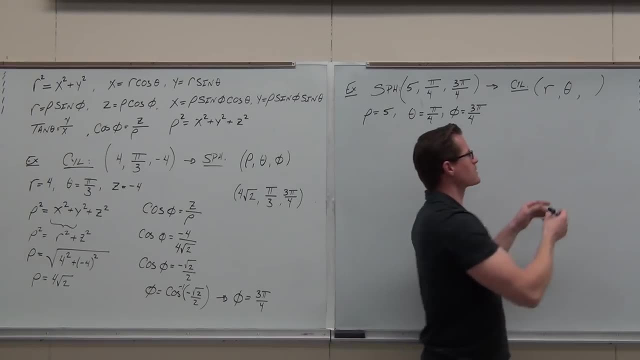 R. So we need R. What's the next thing? that we have Less than R? Is that going to be nice for us? in this It's easier. And then the last thing we have is what? Z? So right now I know that theta pi over 4, done. 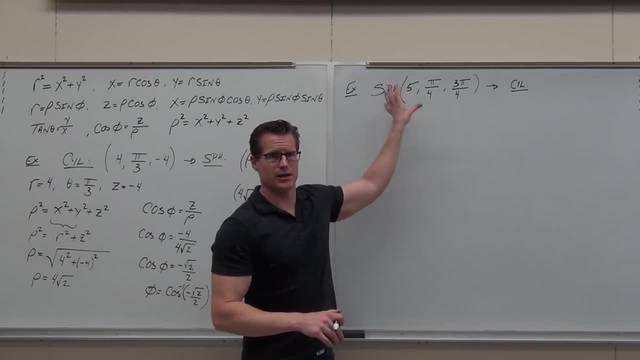 So that's our spherical coordinate for that point. So the two ideas I want you to do: the first idea is, if ever I give you a type of coordinate system, I want you to write down what we have Like, write down what it is, and then also now: 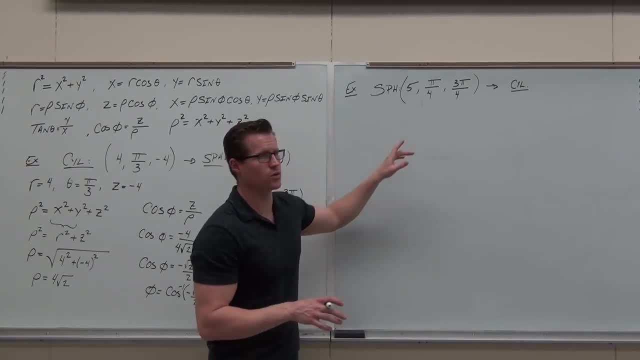 write down what you need. So right now, I want to know, if I give you spherical goodness gracious, what does that number mean? What is the 5?? Rho rho rho, Rho rho R x. I don't know, it's probably one of those. 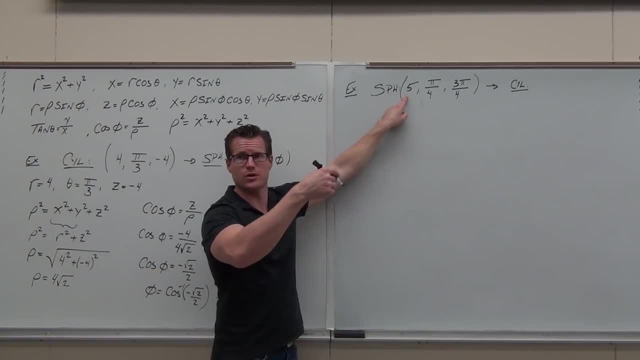 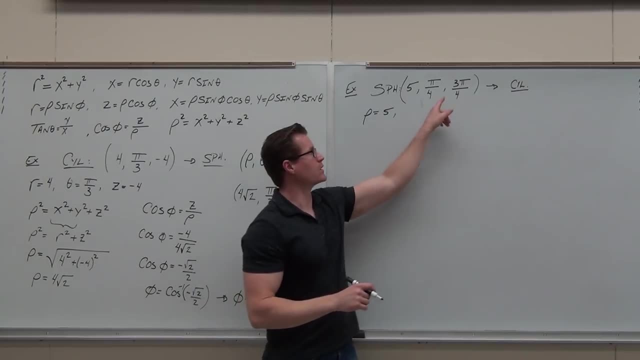 Which? what's this one? Rho, rho. That's a rho, because spherical starts with rho. Everyone in class right now. what's that thing there? And that one? If you've got an angle last, you're probably in spherical. 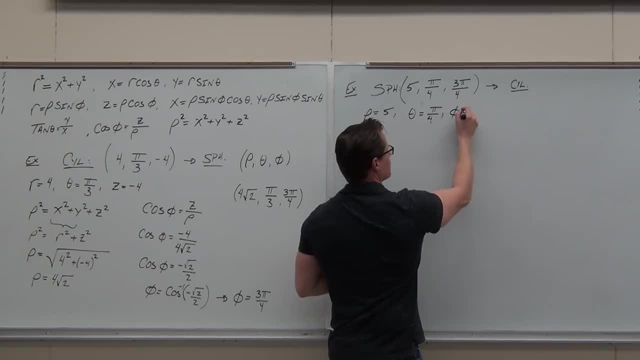 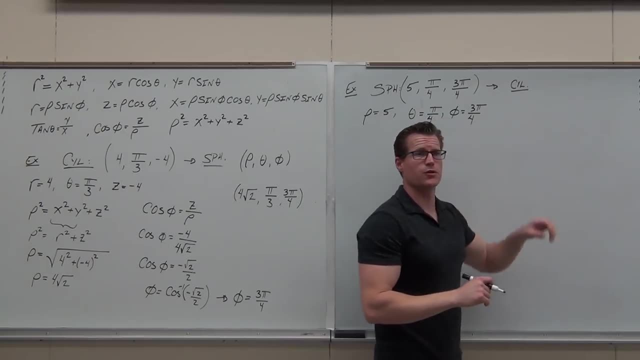 It's the only one that does that. Okay now right-siders, just you guys. I want to know what you need for cylindrical to work. How is it organized? I know it's a lot. It's three things, but what are those? what are those three things? 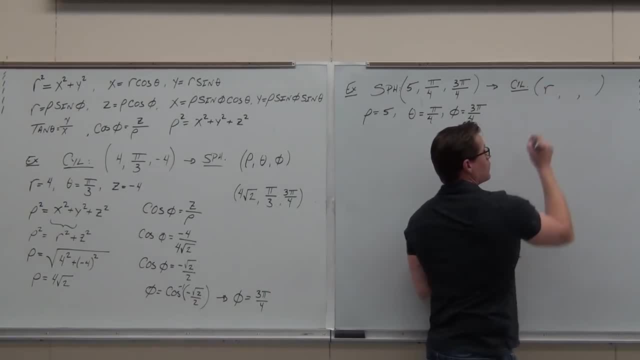 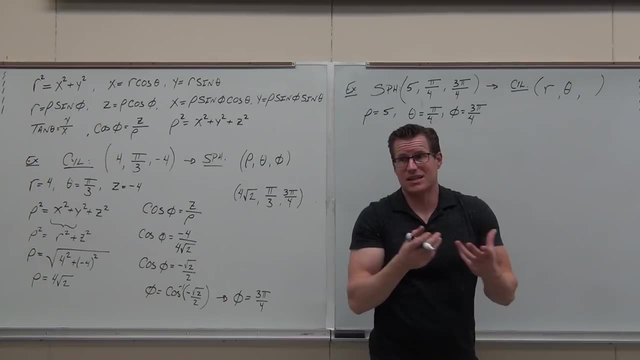 What do we start with R? So we need R. What's the next thing? that we have Left-siders. what do we have Theta? Is that going to be nice for us? in this, It's easier. And then the last thing we have is what? 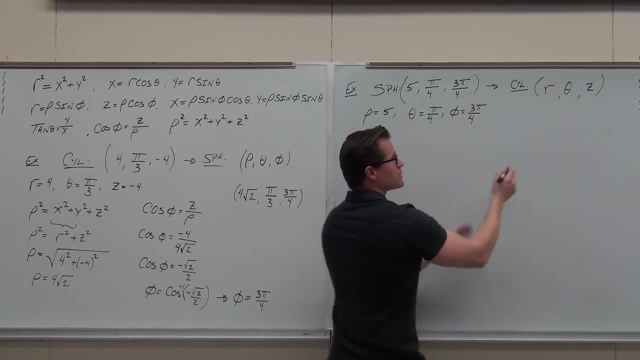 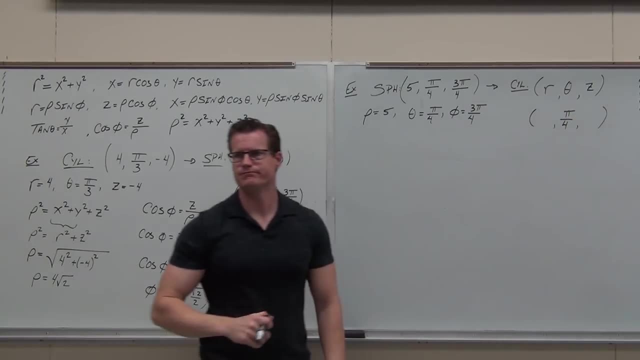 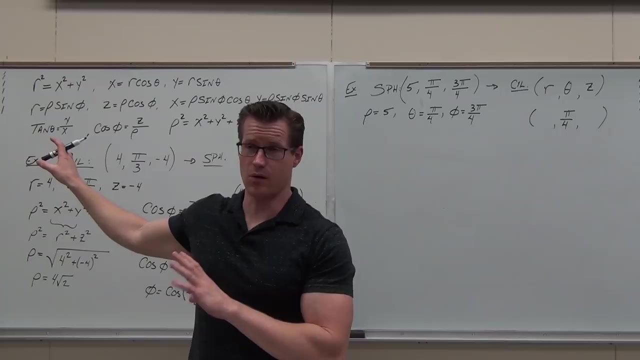 Z. So right now I know that theta pi over 4, done, Done. This is actually going to be the easiest thing that we've done today. I'm pretty sure Do you have the formula up there that's solved for R. 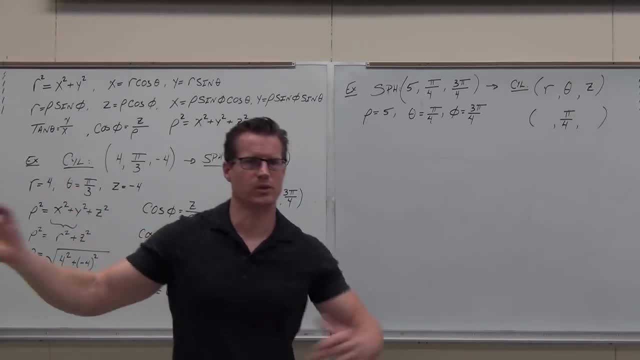 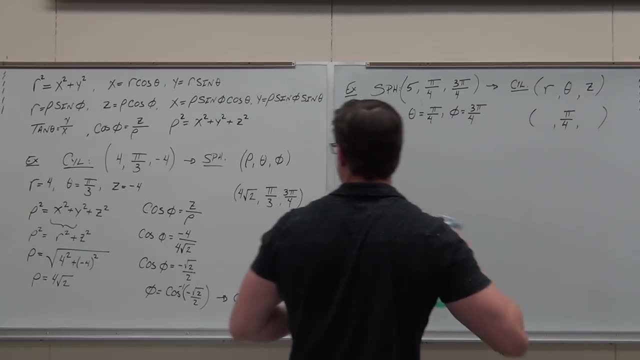 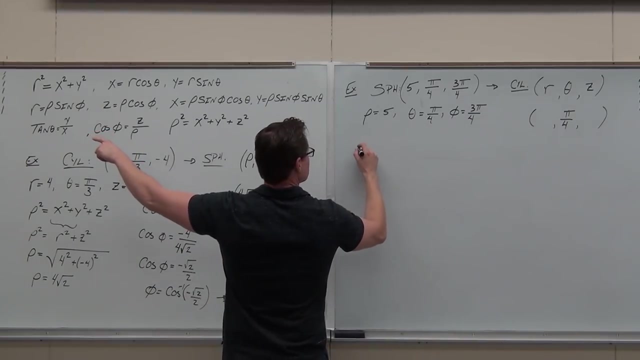 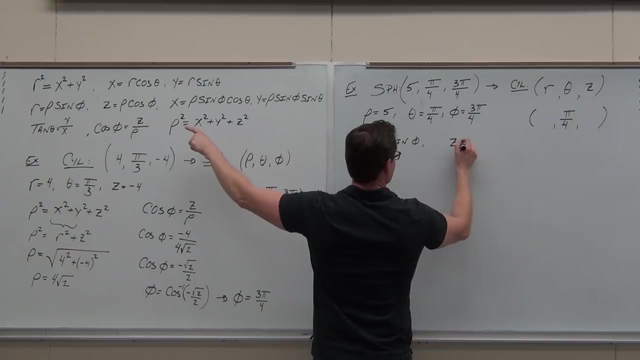 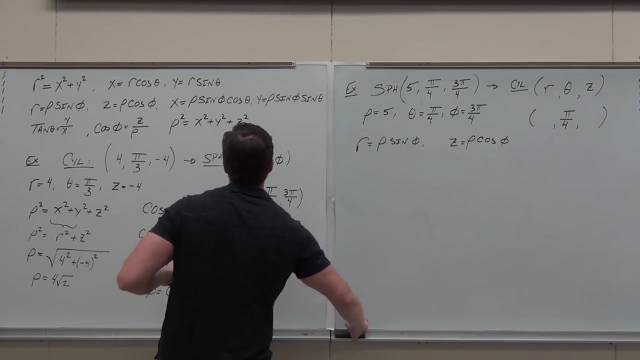 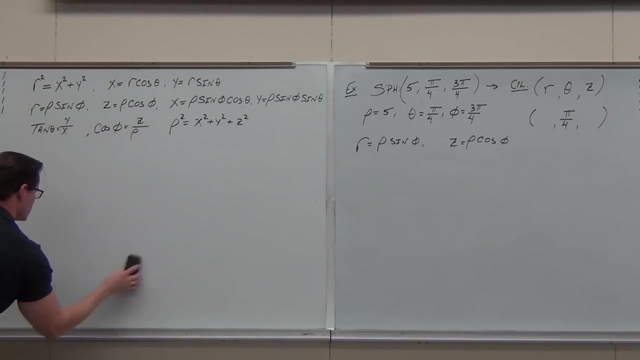 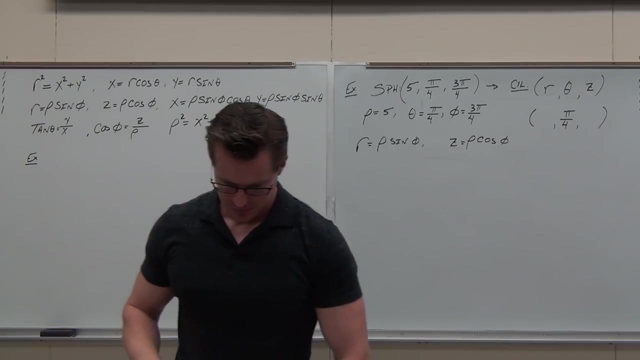 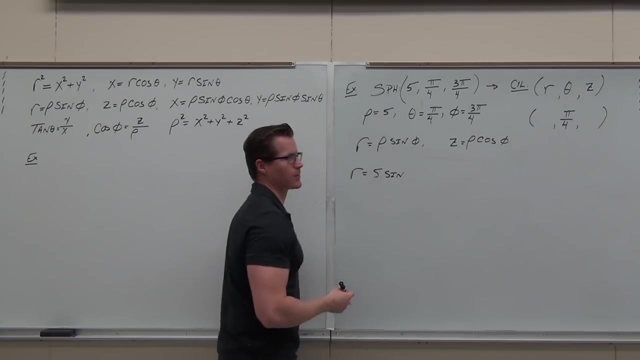 Did you get a formula up there that's solved for Z? Do it. I'll give you about a minute, maybe Go ahead and do it. Hm Man, just make sure you plug in the right angle, right. 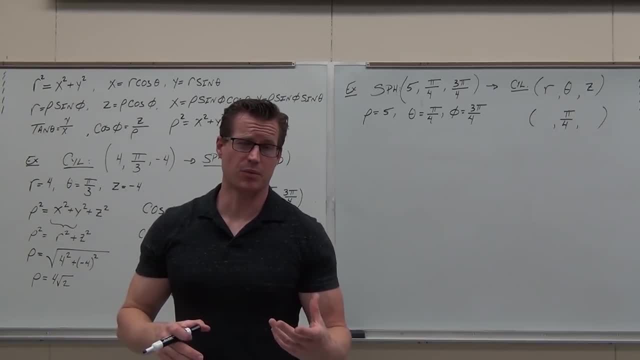 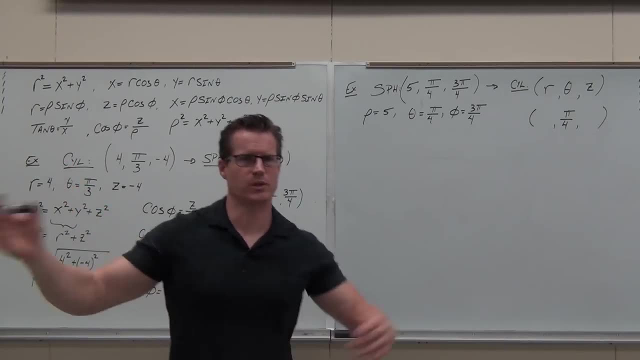 Done. This is actually going to be the easiest thing that we've done today, I'm pretty sure. Do you have a formula up there that's solved for R? Do you have a formula up there that's solved for Z? Do it? 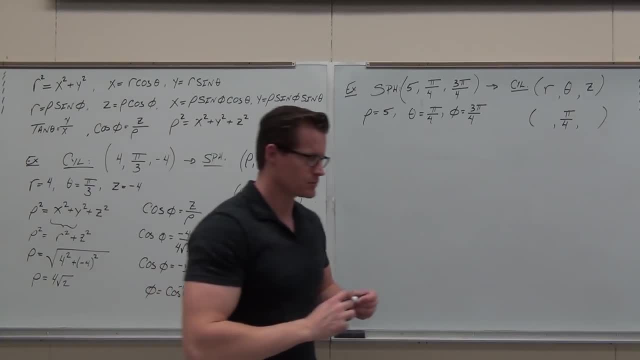 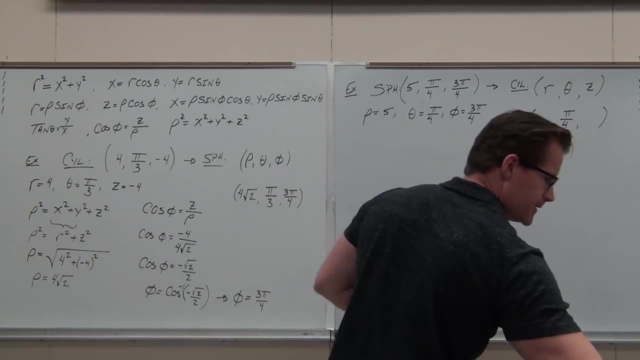 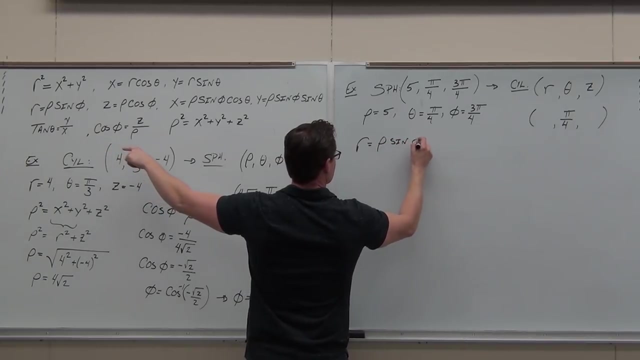 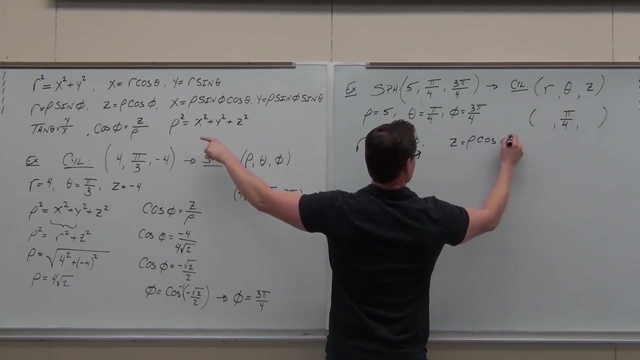 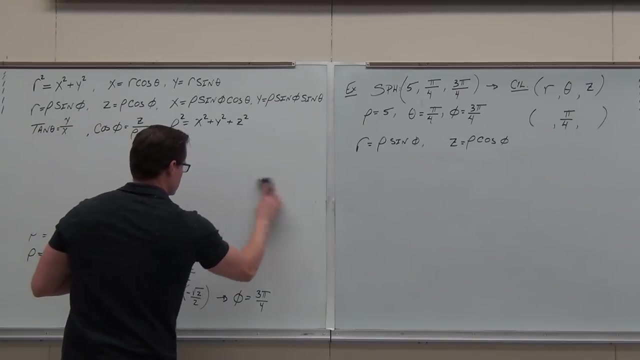 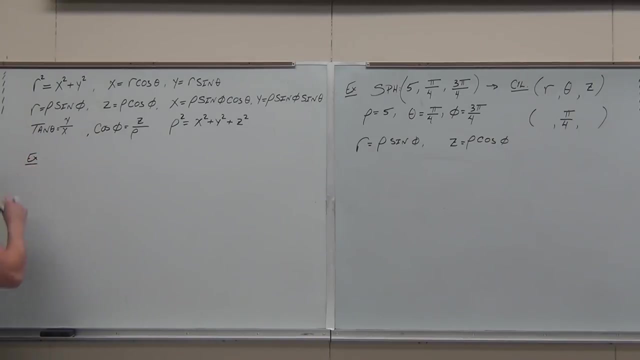 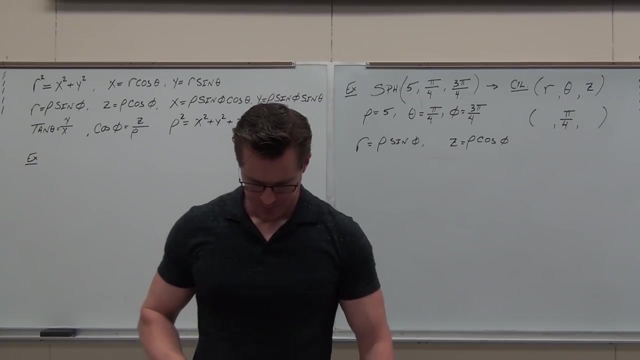 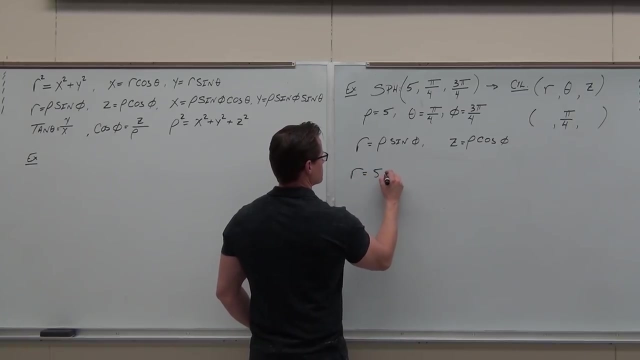 I'll give you about a minute. maybe Go ahead and do it. I'll give you about a minute. maybe I'll give you about a minute, maybe, Man, just make sure you plug in the right angle, right? There's two to choose from. 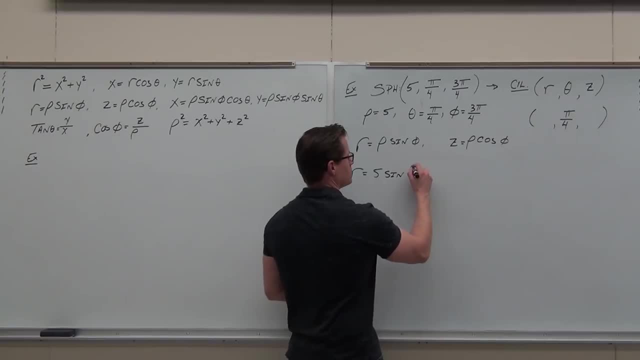 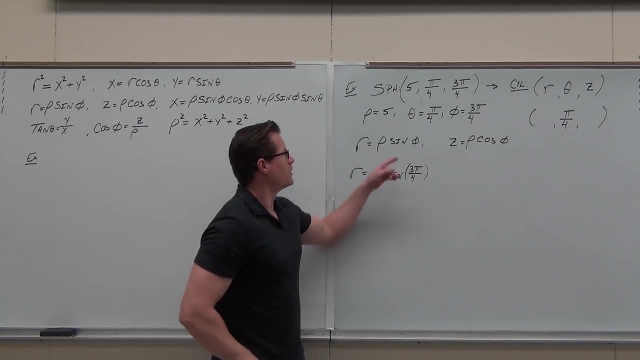 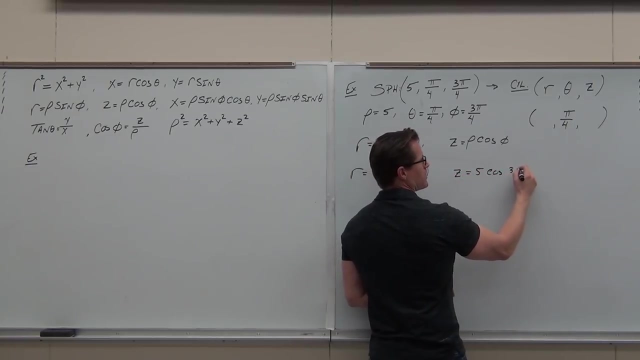 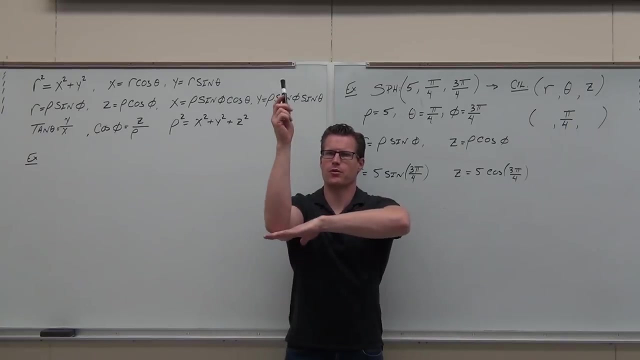 Make sure that we are talking about these right now. Oh hey, how about this? How about this? When we get to the Z, I need to do 5 cosine 3 pi over 4.. If that angle, if that phi is 3 pi over 4,. 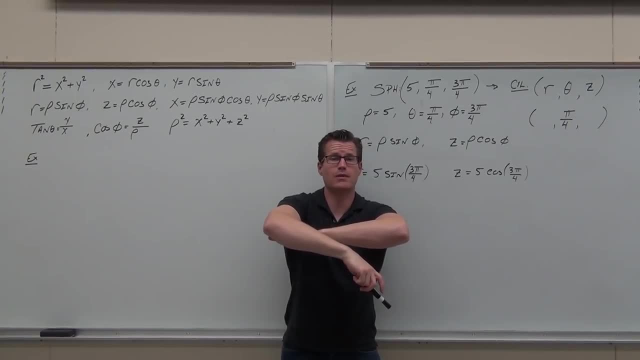 would you expect a positive Z or a negative Z, Negative, Negative. It should be a negative Z. If we don't get that, then we've made a mistake. You guys are starting to see the angle. That's the idea here. 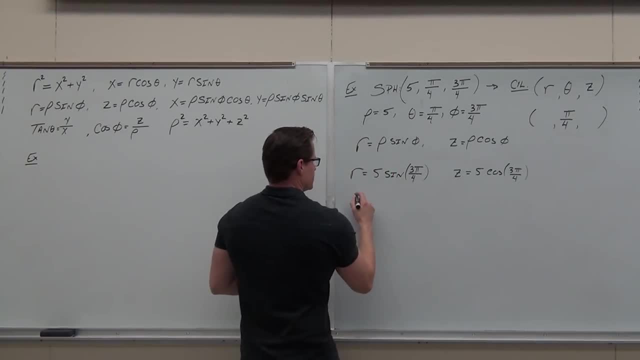 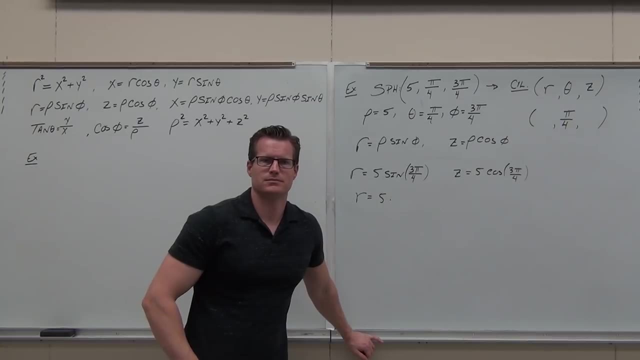 You can check your work if you understand the concepts Five times. oh my gosh, sine of 3 pi. What is that? Root 2 over 2.. Root 2 over 2. You just need to know it's positive because that second. 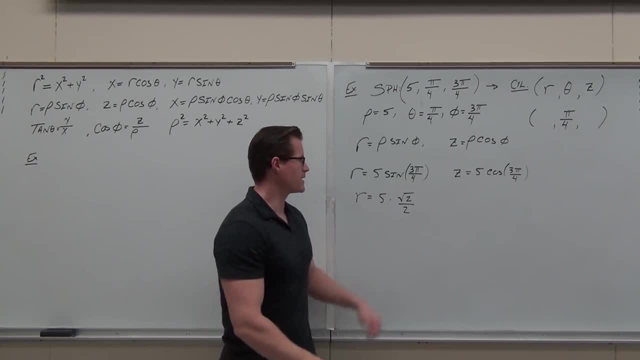 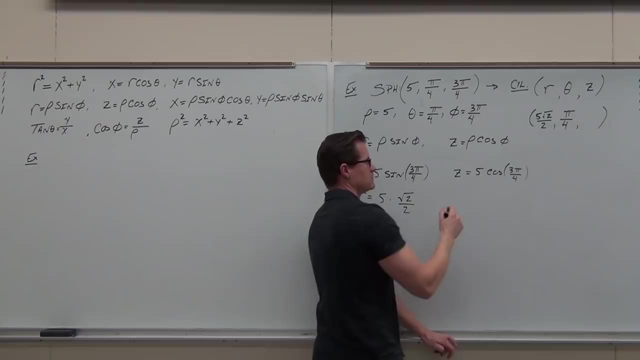 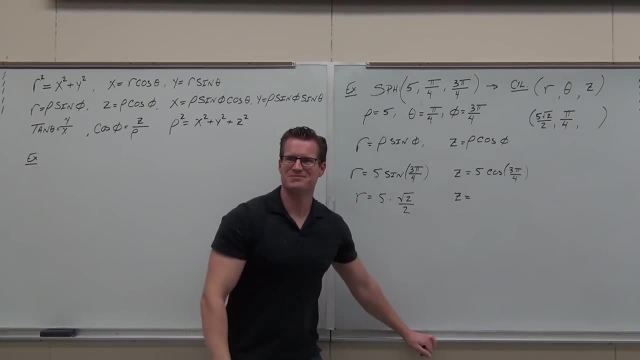 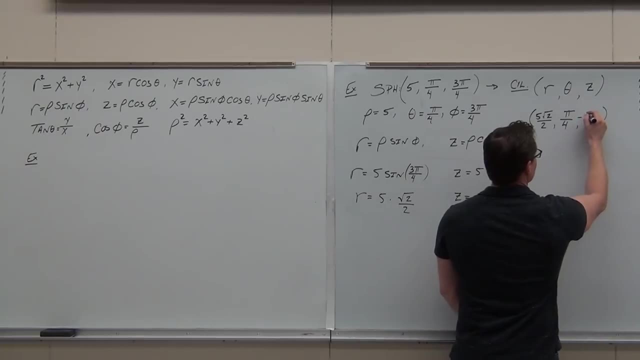 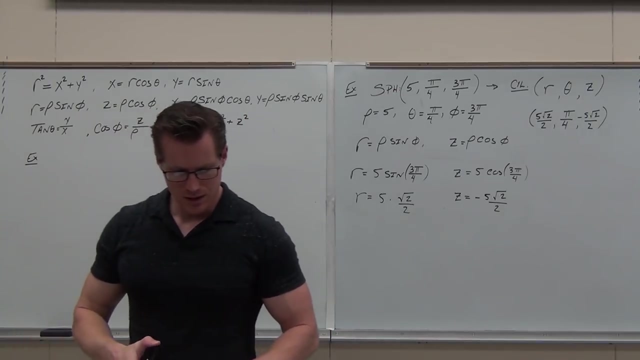 The Z. I'll bet you it's going to be negative. Since this is negative root 2 over 2, we get negative 5 root 2 over 2.. I would really love to know if I have made sense to you today. 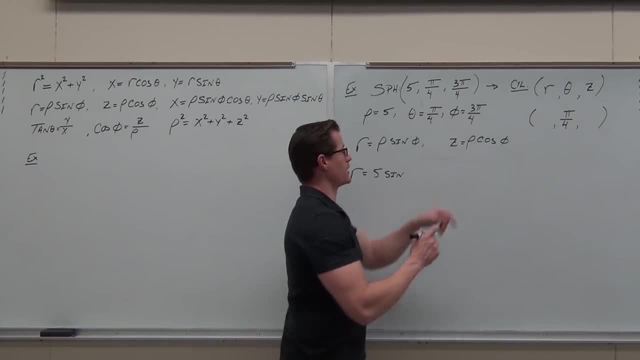 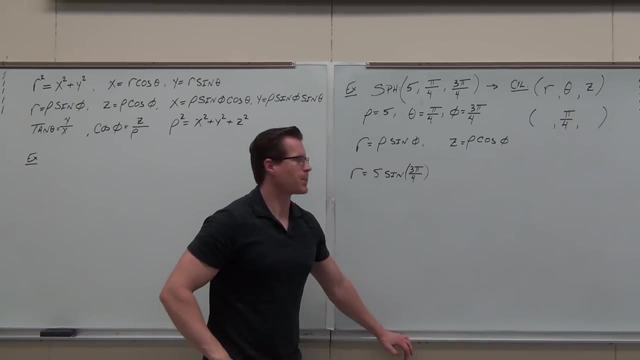 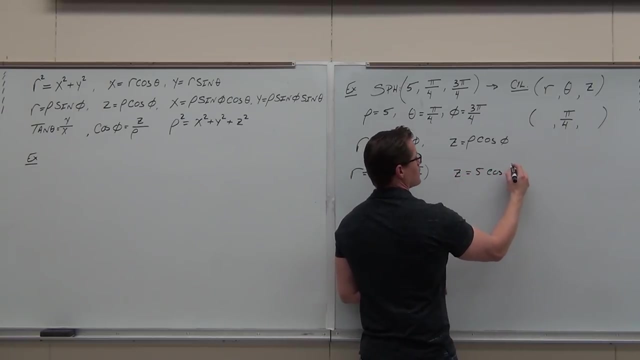 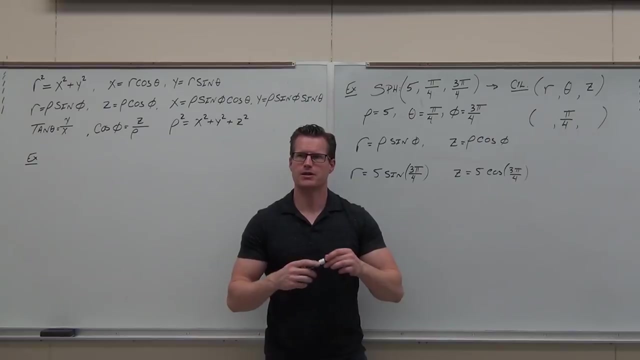 There's two to choose from. Make sure that we are talking about these right now. Oh hey, how about this? How about this? When we get to the z and you do 5 cosine 3 pi over 4, if that angle, if that phi is 3 pi over 4,. 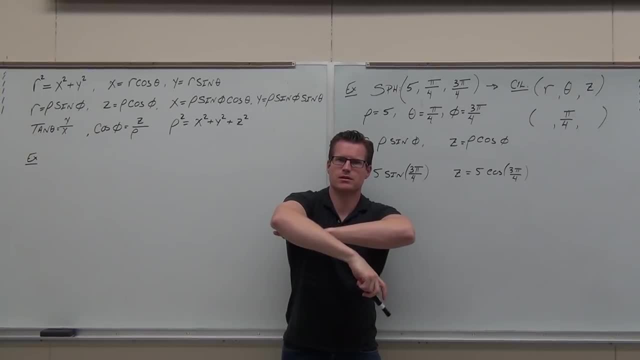 would you expect a positive z or a negative z? Negative, It should be a negative z. If we don't get that, then we've made a mistake. You guys are starting to see the idea here. You can check your work if you understand the concepts. 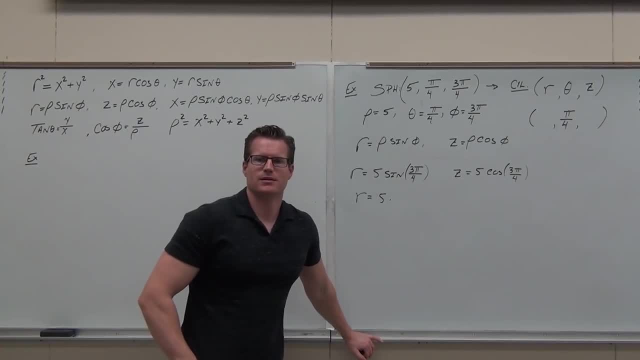 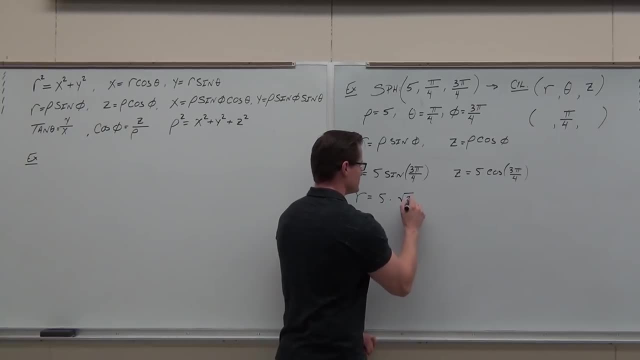 5 times. oh my gosh sine of 3.. What is that? 3 to the 2., 3 to the 2.. You just need to know it's positive because that second quadrant it's all students. It's positive over there. 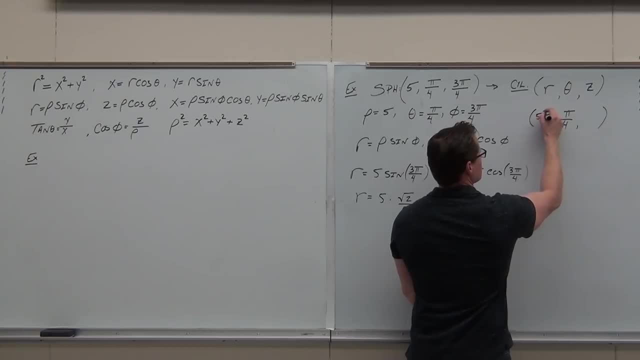 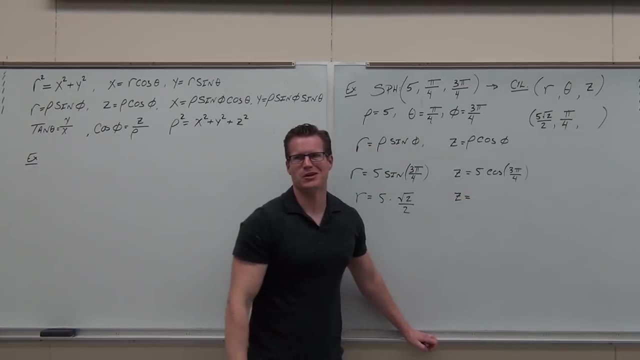 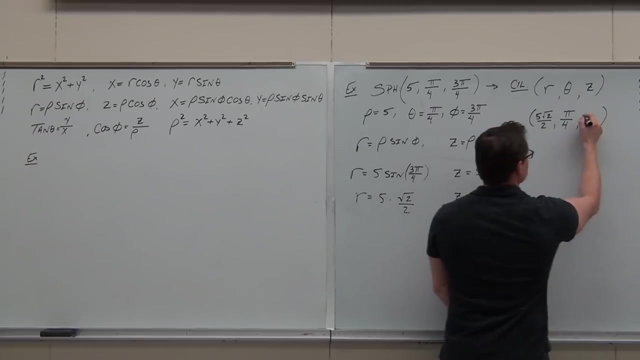 So that's going to be 5 root 2 over 2.. The z: I'll bet you it's going to be negative, Since this is negative: root 2 over 2, we get negative, We get negative, We get negative. 5 root 2 over 2.. 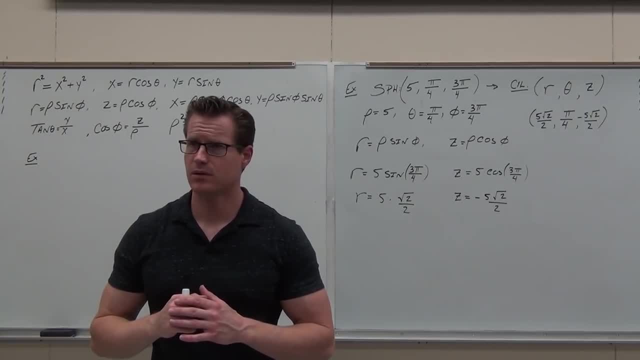 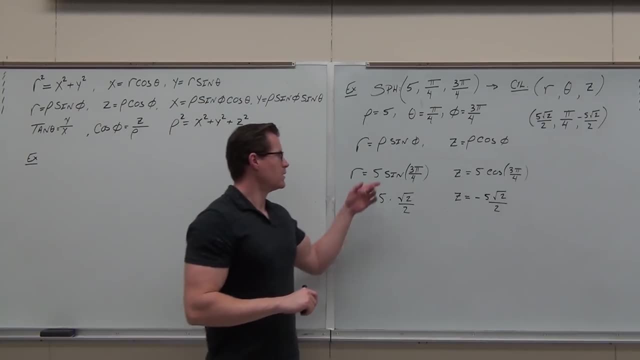 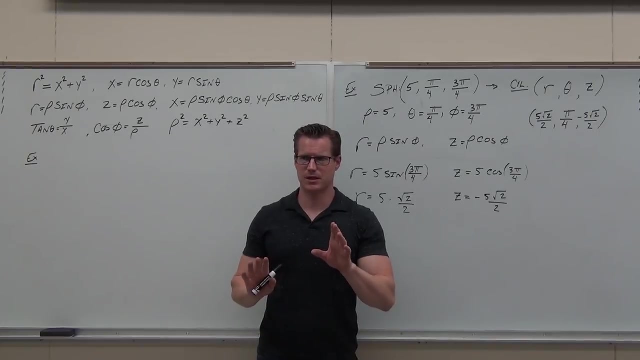 I would really love to know if I have made sense to you today. I do want to talk about this, Just one little blurb Doing this. you cannot possibly get a negative r. You can't possibly get it, And I want to show you why. 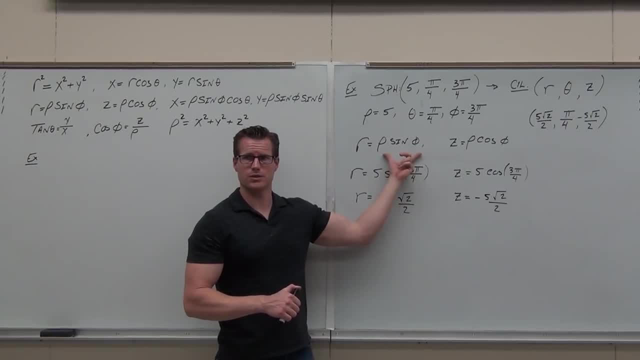 If you talk about this, this is how you get r correct. Please watch carefully. This is how you get r. Rho is always positive. You with me, Always Sine phi. Well, phi can't go past pi. 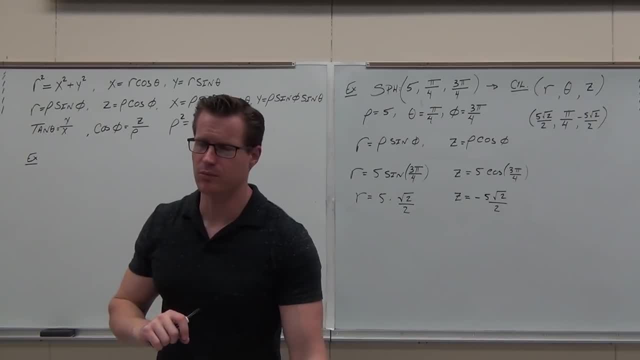 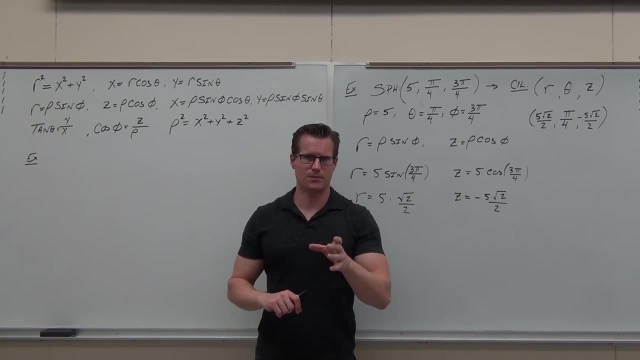 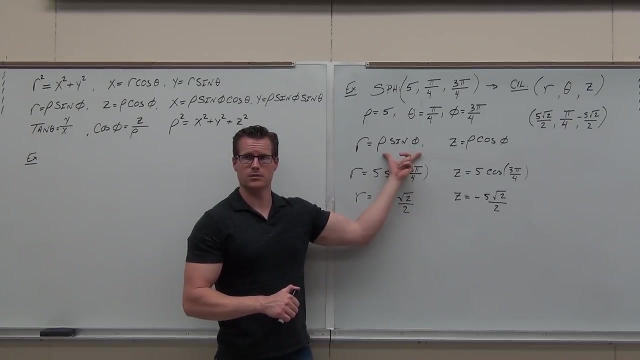 I do want to talk about this. Just one little blurb. Doing this, You cannot possibly get a negative r. You can't possibly get it, And I want to show you why. If you talk about this, this is how you get r correct. 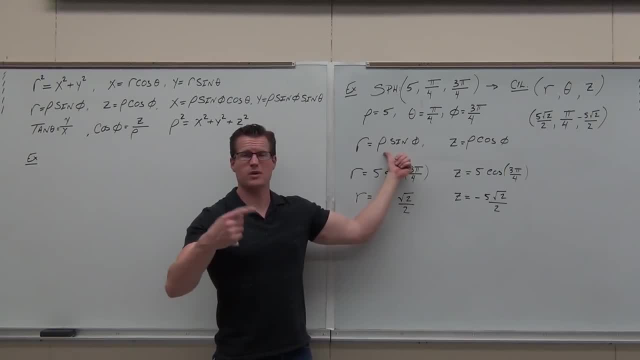 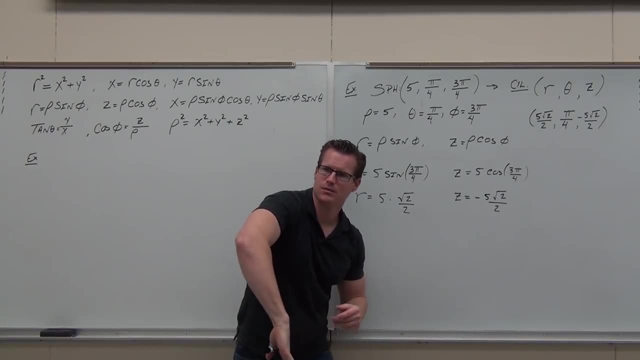 Please watch carefully. This is how you get r. Rho is always positive, You with me, Always Sine. phi. Well, phi can't go past pi. Sine is always positive from 0 to pi. All students remember 0 to pi, all students. sine is always. 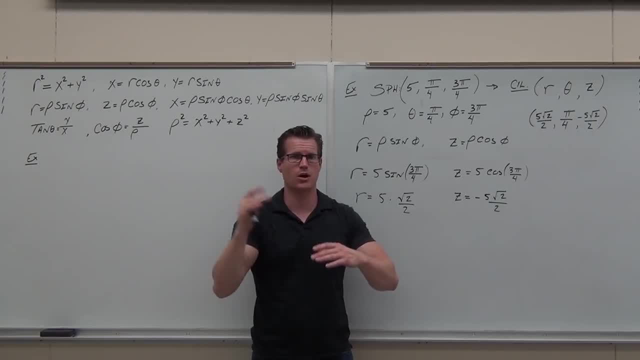 positive there. So if sine is y, y is always positive in the first two quadrants. that is always positive from 0 to pi. Therefore, positive times positive is going to be positive. You don't have to worry about getting negative r's. 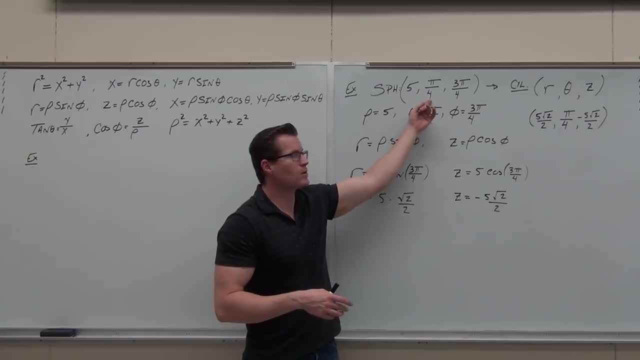 It won't happen. So you always get positive r This guy. yeah, you don't have to worry about it at all. You just take the same exact thing here And then this: it's only from 0 to pi also. 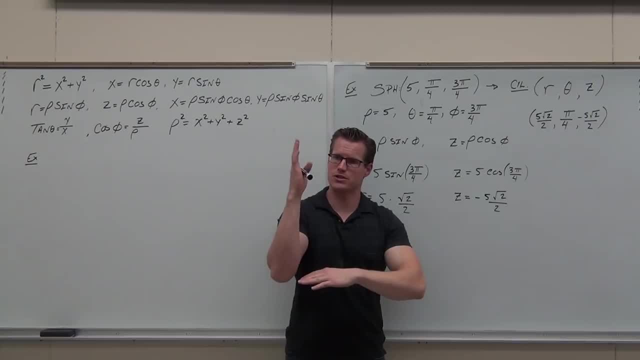 So when you're going on that cosine for the first pi over 2, so we're dropping right: First pi over 2, you're positive, Next pi over 2, you're negative. And that's how these things work. 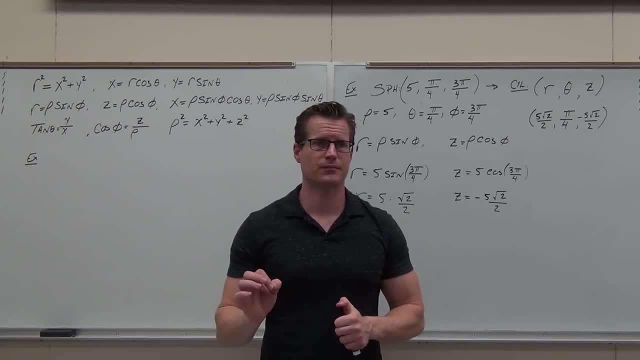 Are you sure you're OK with it for real? Any comments? questions at all. This part I actually like this part. We're going to start talking about how to translate between different types of equations. So I give you an equation like this: 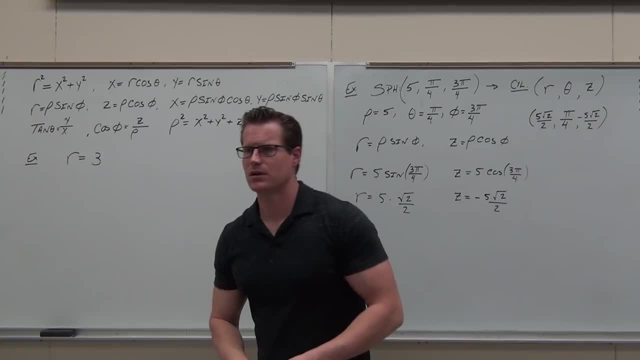 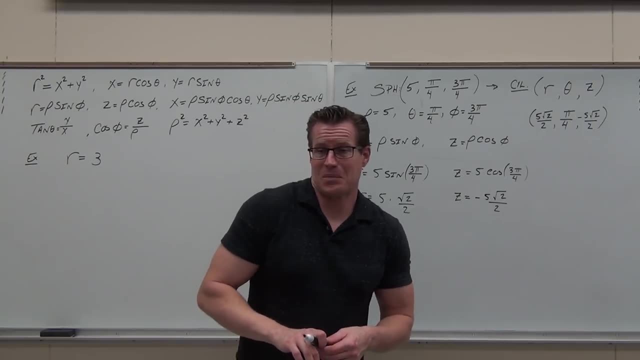 r equals 3. And you go awesome. What does that mean in terms of a 3D picture? What is it? y 0, 0.. What's that mean? 0. 0. 0. 0.. 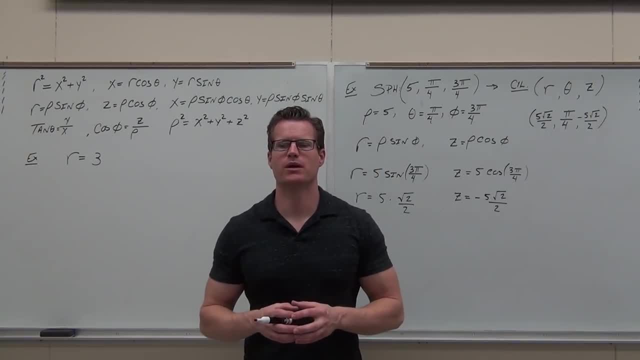 0. 0. 0. It says: well, maybe you can tell me what coordinate system it's even in. Would you say that's rectangular? No, You see a whole lot of x's and y's and stuff. Is that spherical? 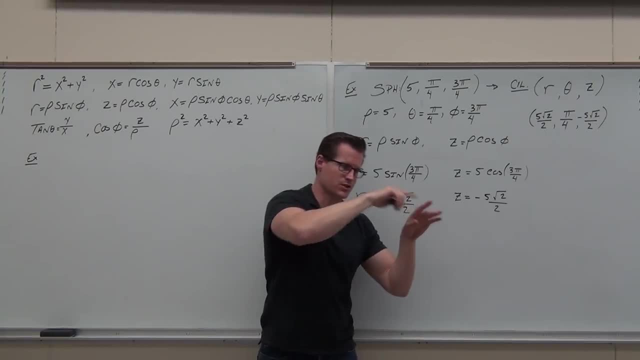 Sine is always positive from 0 to pi. All students Remember 0 to pi. Sine is always positive there. So if sine is y, y is always positive in the first two quadrants. That is always positive from 0 to pi. 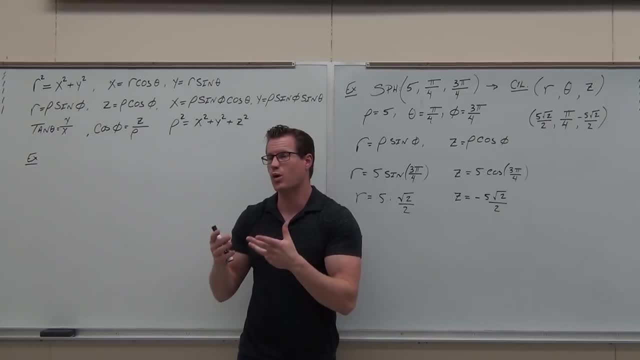 Therefore, positive times, positive is going to give you positive. You don't have to worry about getting negative r. It won't happen. So you always get positive r This guy. yeah, you don't have to worry about it at all. 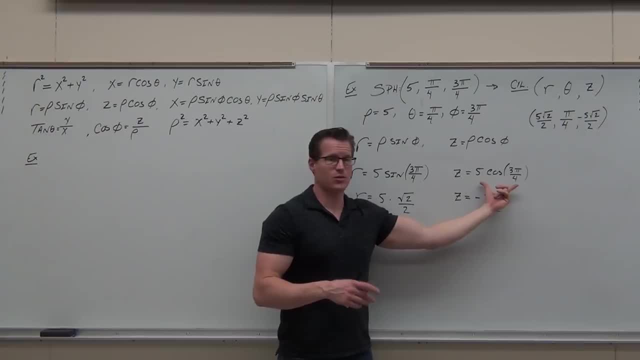 You just take the same exact thing here And then this: it's only from 0 to pi also. So when you're going on that cosine for the first pi over 2, so we're dropping right First pi over 2, you're positive. 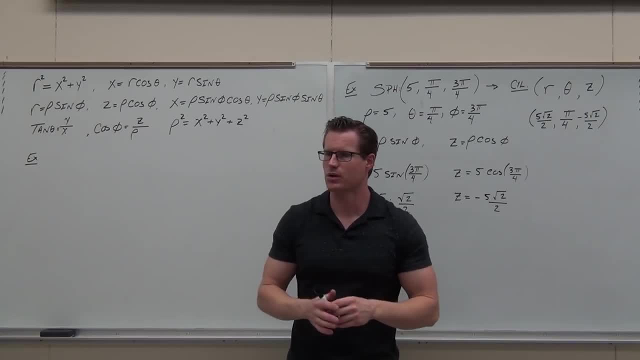 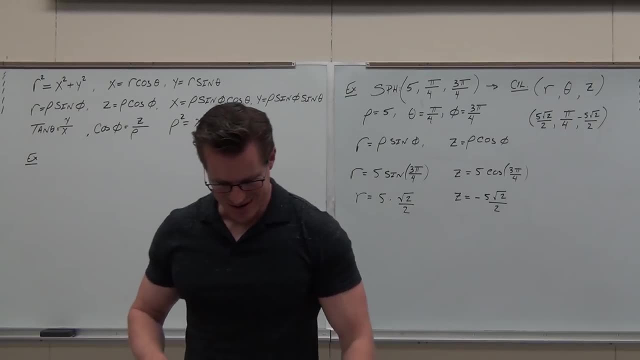 Next, pi over 2, you're negative, And that's how these things actually work. Are you sure you're okay with it for real? Any comments? questions at all? This part I actually like. this part We're going to start talking about how to translate between different types of equations. 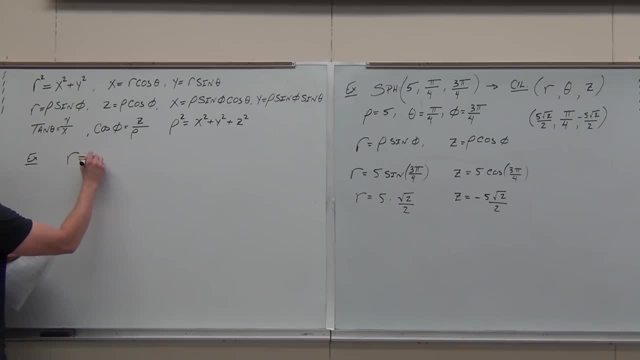 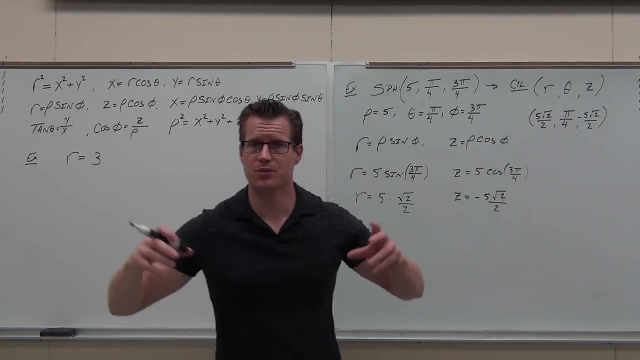 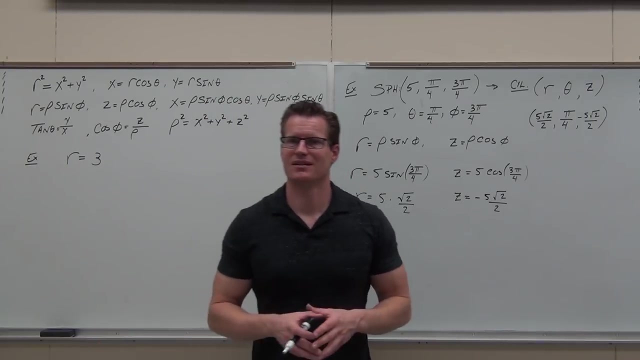 So I give you an equation like this: R equals 3. And you go: awesome. What does that mean in terms of a 3D picture? What is it? What's that mean? It says: well, first of all, maybe you can tell me what coordinate system it's, even in. 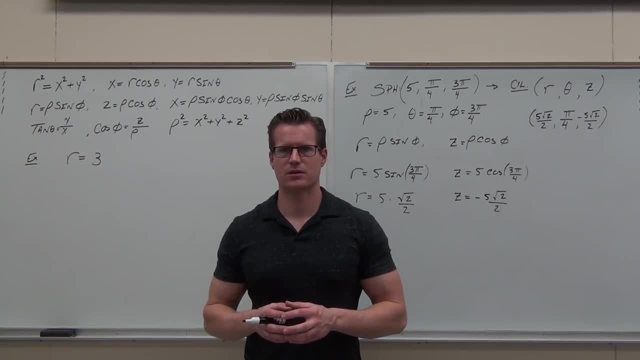 Would you say that's rectangular? No, Do you see a whole lot of x's and y's and stuff? Is that spherical? Do you see a whole lot of rows and phi's? What is that? It's cylindrical. It's what? 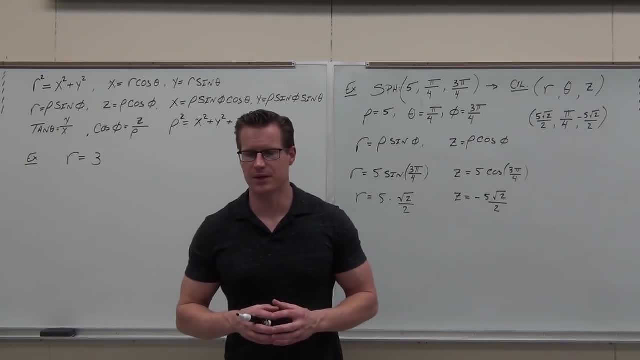 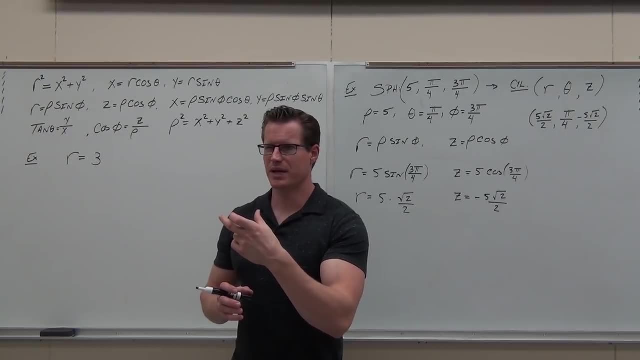 I'll give you probably the biggest hint here: Anytime you have a variable equal a constant, you basically have the type of shape that the coordinates are based on. So if R is cylindrical, that's equal to a constant. you have a cylinder. 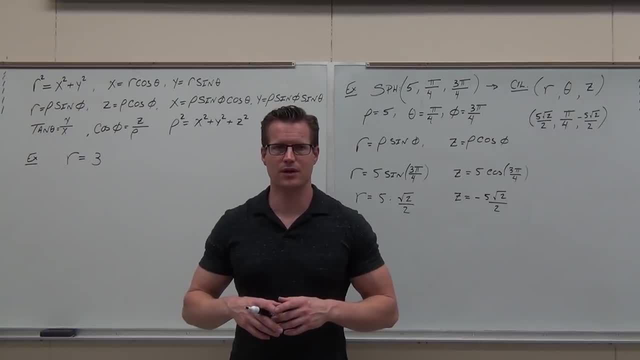 That's what you have. This is a cylinder with a radius of. what do you think? Geniuses, all of you? Yeah, exactly right Now. where is it? It's going along the z Now. how do I know that? 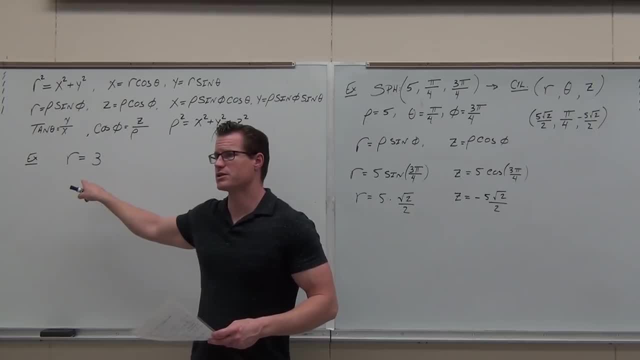 Well, the thing is, that's pretty nice to describe a cylinder, isn't it? But we're not used to it, Because mostly when we think about these pictures, they're all in x's and y's and z's and stuff. 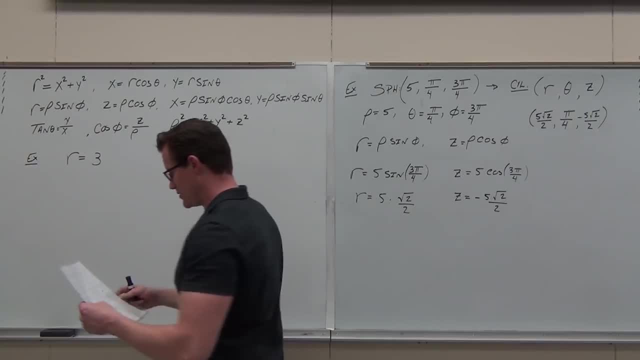 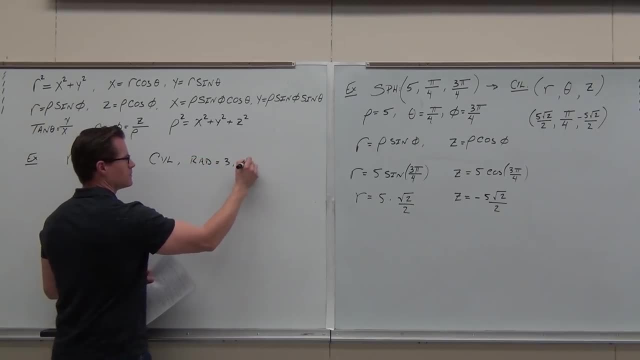 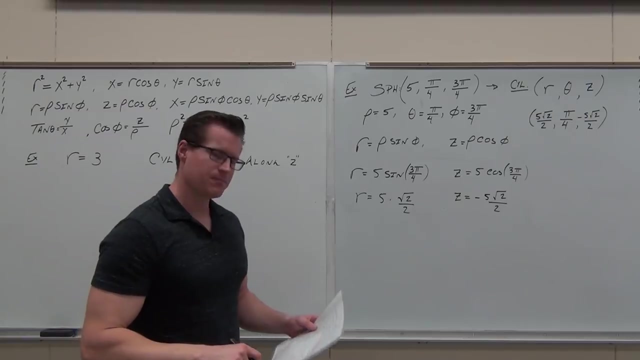 You know what I'm talking about. That's what they're in. So I know it's a cylinder, I know it's a radius 3, and I know it's along z. How can I prove it? How we prove it is by making this stuff out of this thing. 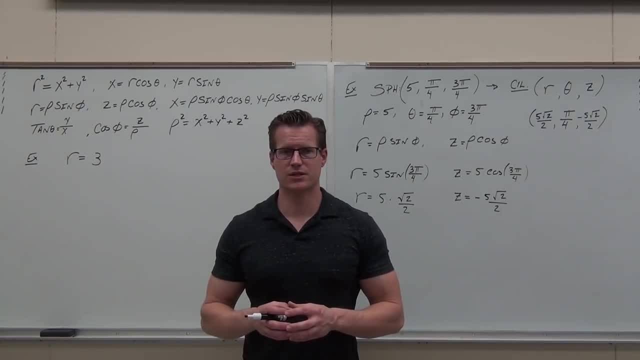 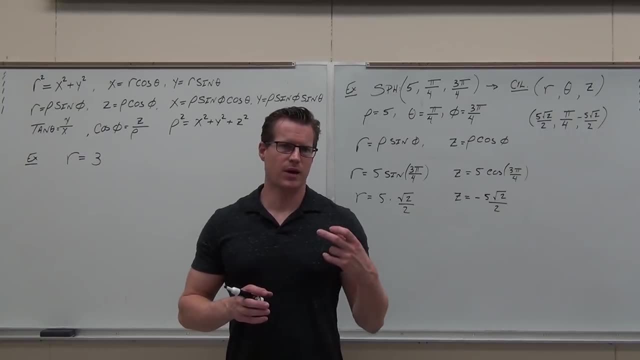 Do you see? a whole lot of rows and phi's. What is that? A cylindrical, A cylindrical, It's what? Cylindrical? I'll give you probably the biggest hint here. Any time you have a variable equal, a constant. 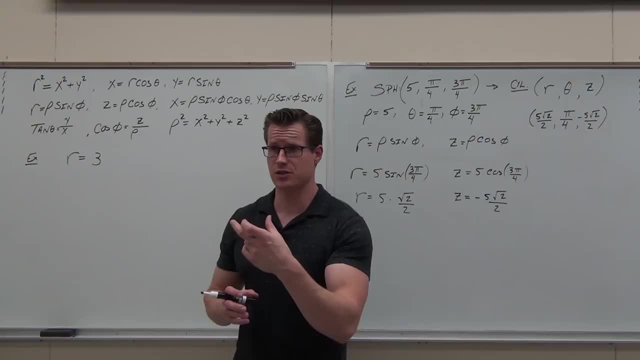 you basically have the type of shape that the coordinates are based on. So if r is cylindrical as equal to a constant, you have a cylinder. That's what you have. This is a cylinder with a radius of what do you think? Geniuses, all of you? 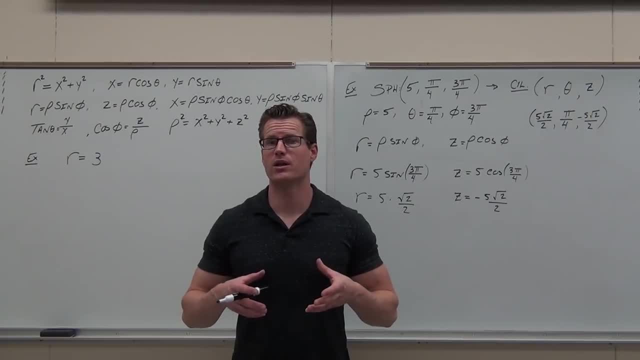 Yeah, exactly right. Now, where is it going along? It's going along the z. Now how do I know that? Well, the thing is that's pretty nice to describe a cylinder, isn't it? But we're not used to it. 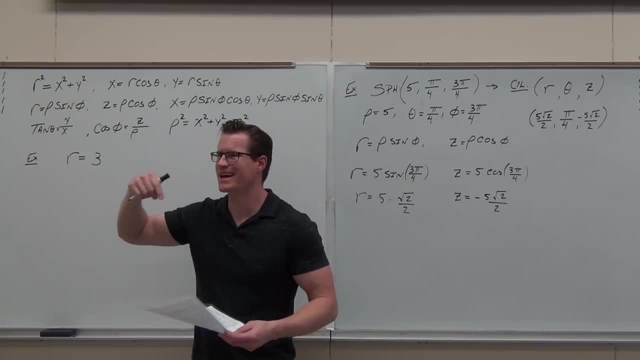 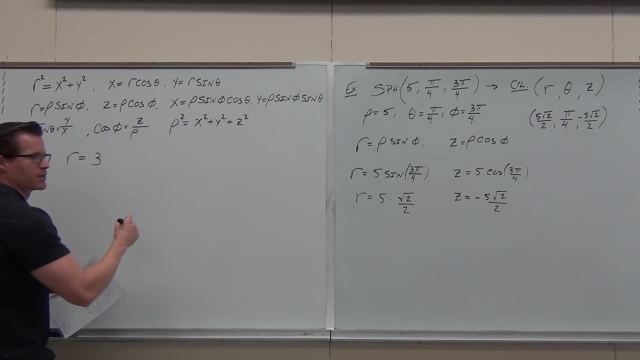 Because mostly when we think about these pictures they're all in x's and y's and z's and stuff. You know what I'm talking about. That's what they're in. So I know it's a cylinder, I know it's a radius 3, and I know it's along z. 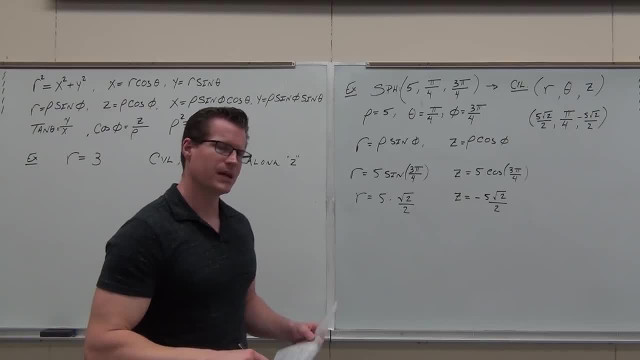 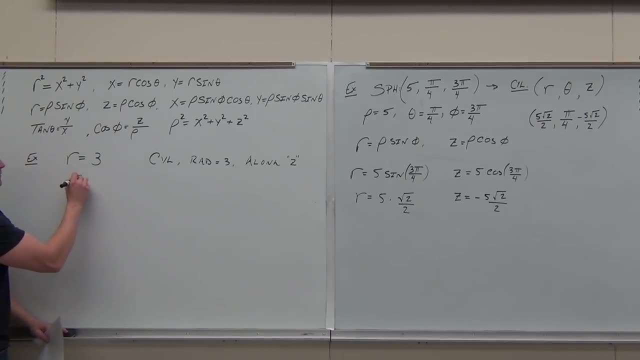 How can I prove it? How we prove it is by making this stuff out of this thing. For instance, if I square both sides, You guys see the r squared equals 9, yeah, Square both sides. Square both sides. Oh, but wait. 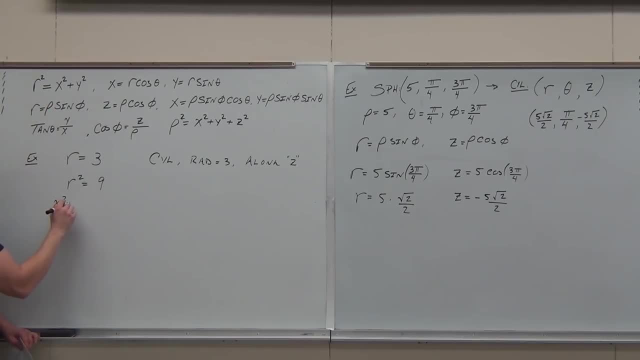 R squared is this: You guys see how to get there. Oh my gosh, this is in 3D. How many variables you got. This will be exciting. How many variables you got. What's that mean? Surface or cylinder? 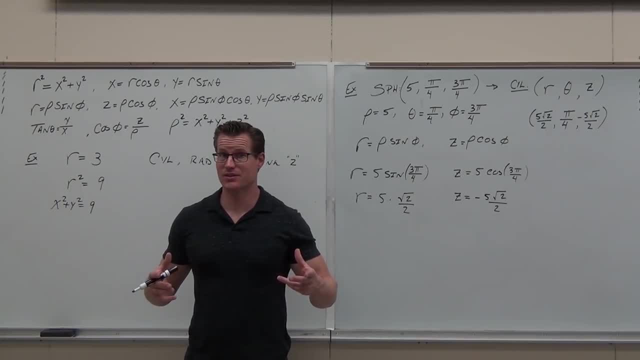 Cylinder Going along what axis With a radius of 3, just like that same stuff. We're used to this, so we typically have to translate it. but look at the ease of the formula here, Man. that's so much nicer to work with. 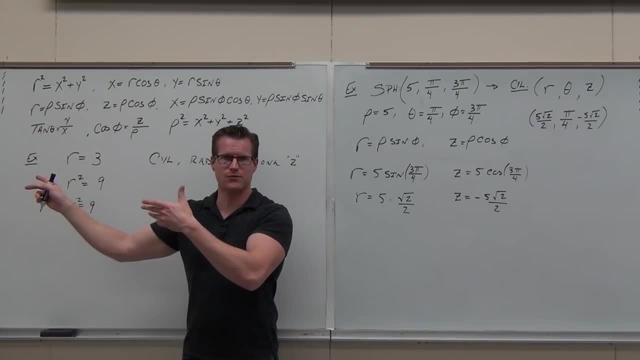 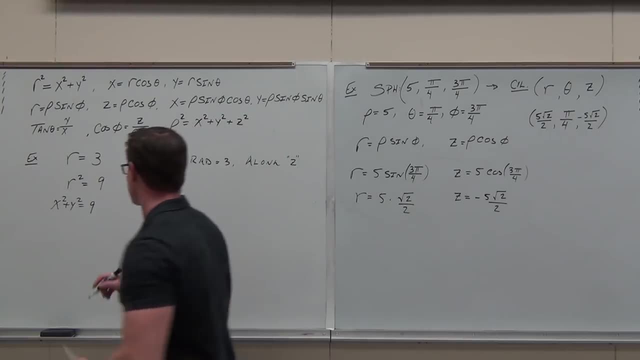 So if you understand that when we get to double integrals and you have to define what the cylinder is, that's an easier way to do it. That's why we have this stuff is to make those connections. How about this one? 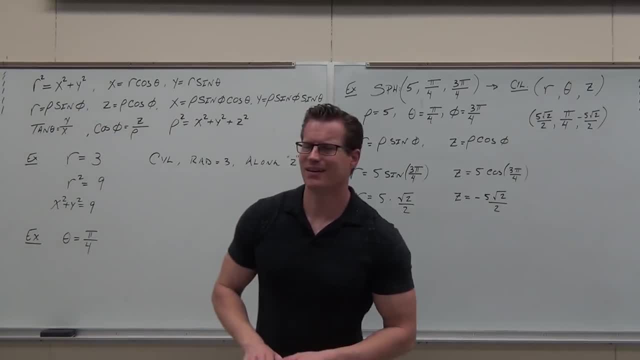 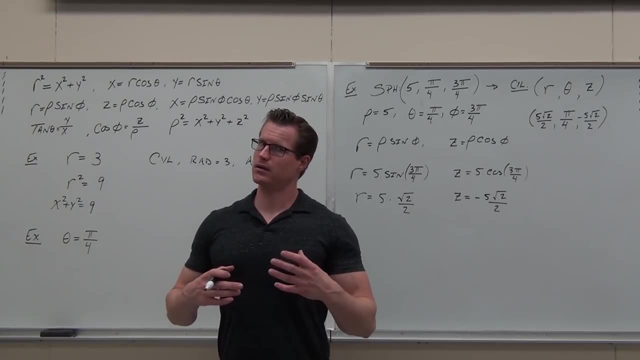 What in the world is that Crazy? What in the world is that? Well, that could be either thought of as cylindrical, because it's got that phi, or spherical, because it's still got that phi, but that phi is constant. 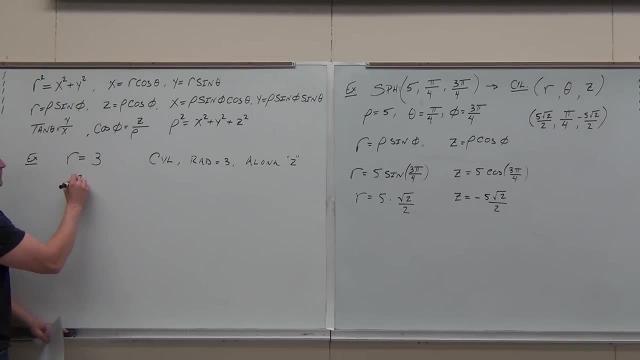 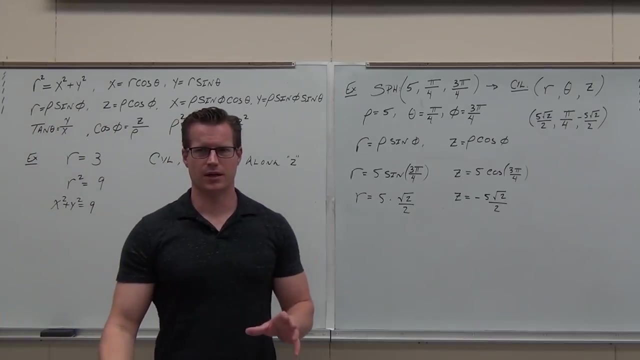 For instance, if I square both sides, you guys see the R squared equals 9? Yeah, Square both sides. Square both sides. Oh, but wait, R squared is this. You guys see how to get there. Oh, my gosh. 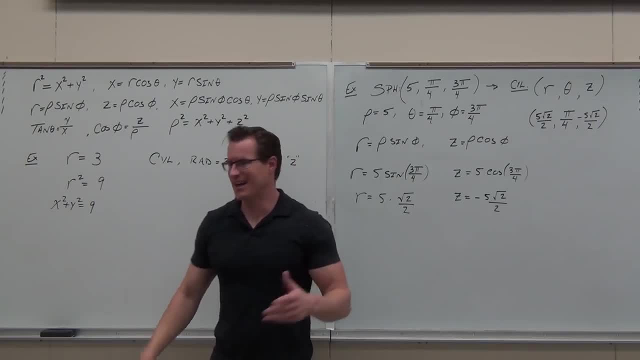 This is in 3D. How many variables? you got Two, Three, Four, Five, Six, Seven, Eight, Nine, Twenty, Twenty, Twenty, Twenty. This should be exciting. How many variables do you got Two. 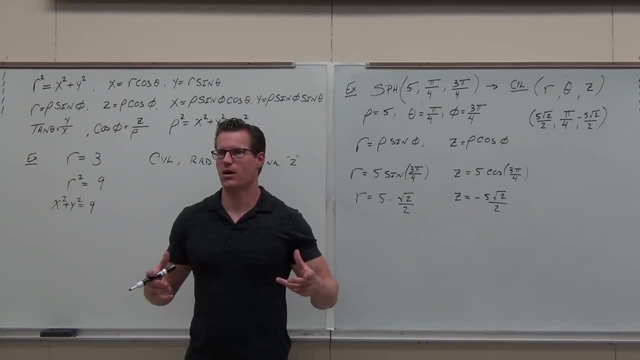 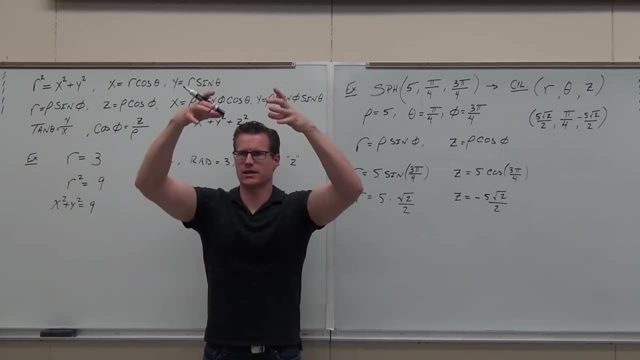 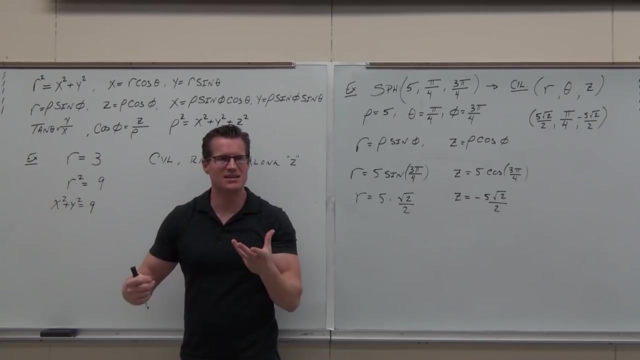 Two, What's that mean? Circus or cylinder, Cylinder Going along what axis? The z With a radius of Three, Just like that Same stuff. We're used to this, so we typically have to translate it. But look at the ease of the formula here. 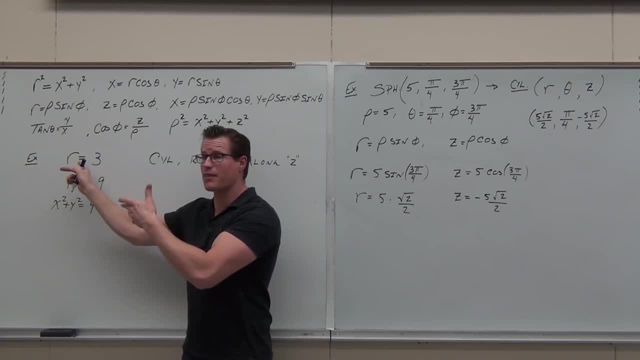 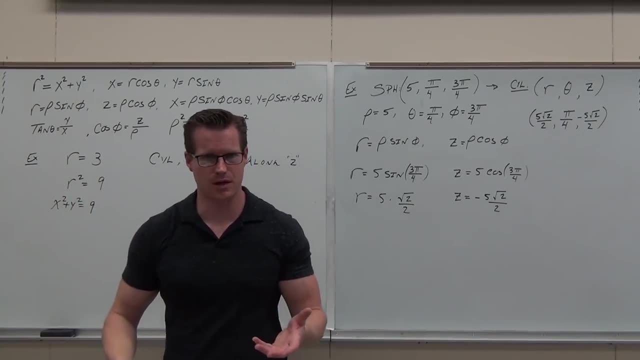 Man that's so much nicer to work with. So if you understand that when we get to double integrals and you have to define what the cylinder is, that's an easy one. That's an easier way to do it. That's why we have this stuff is to make those connections. 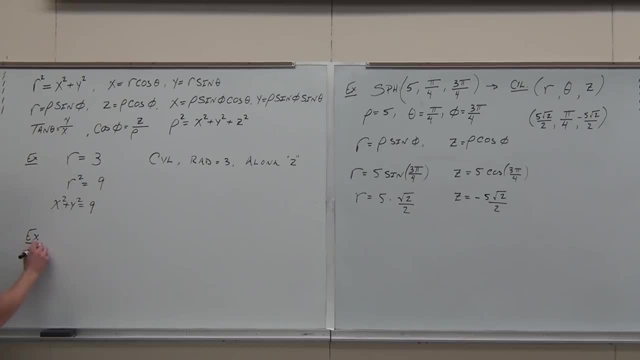 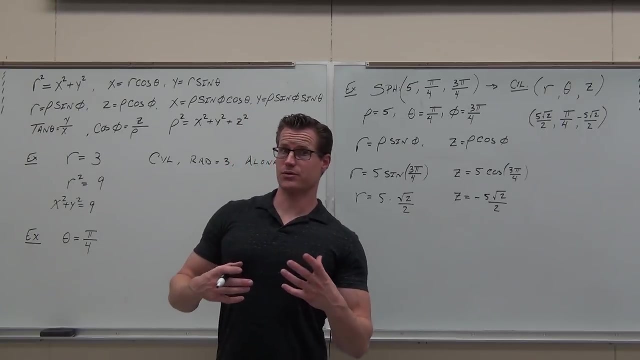 How about this one? What in the world is that Crazy? What in the world is that? Well, that could be either thought of as cylindrical, because it's got that phi, or spherical, because it's still got that phi, But that phi is constant. 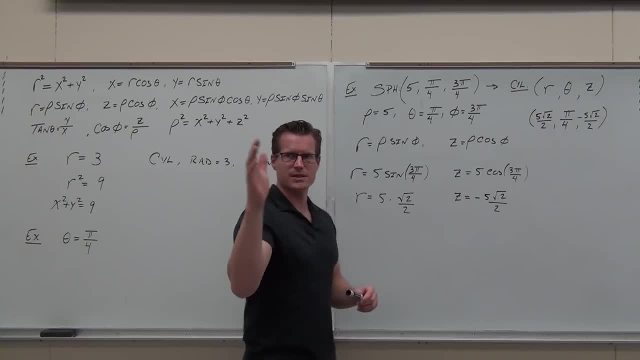 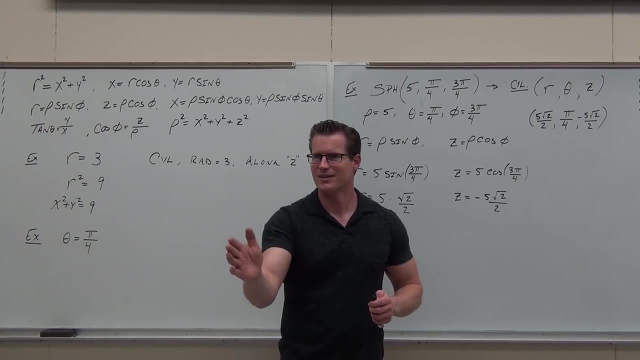 So what it's saying is this: from the positive x-axis. I'm going out. what did I say? Phi fo fun, whatever theta In my head. I was saying theta. It didn't come out that way. 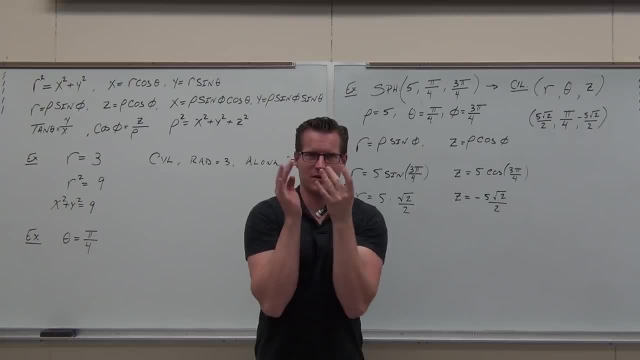 Dang, I'm getting tired. Okay, so theta, edit. so the theta. it comes out from the positive x-axis, pi over 4, and then it's fixed. What's that do If you have a fixed angle and any points along that? that's going to be a plane. 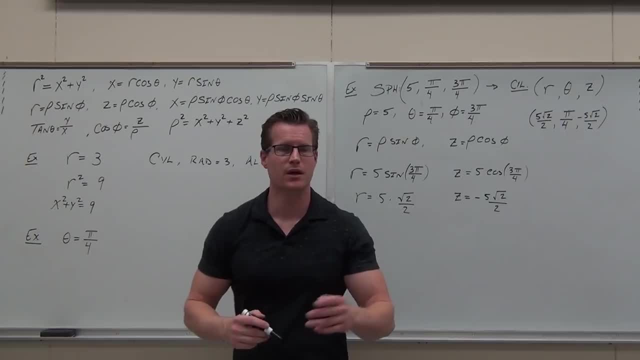 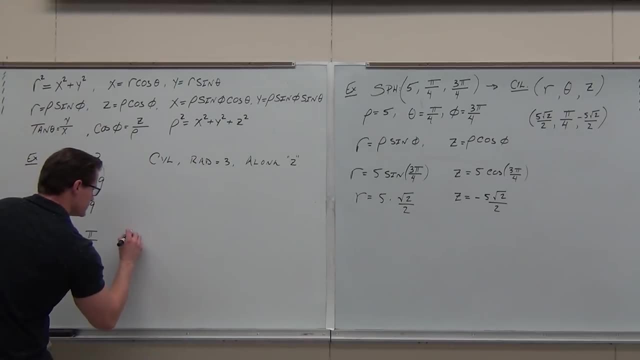 A plane at the angle of pi over 4, I guarantee it's a plane. How can you prove it? Well, I know that tangent theta equals y over x. So tangent of pi over 4, or theta is pi over 4, has to equal y over x. 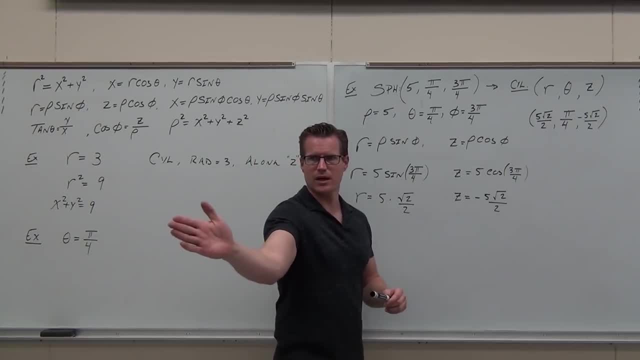 So what it's saying is this: From the positive x-axis I'm going out. what did I say? Phi fo fun, whatever theta. I didn't like that. I didn't like that. In my head I was saying theta. 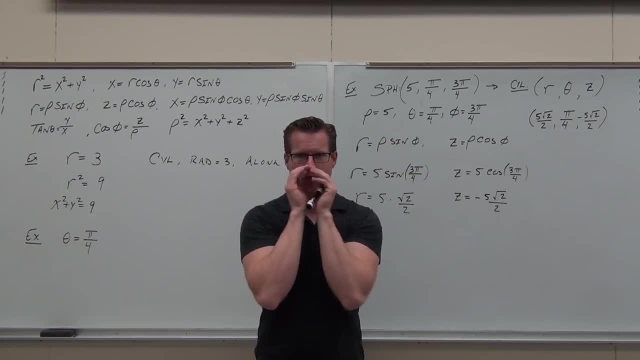 It didn't come out that way. Dang, I'm getting tired. Okay, so theta edit. So the theta: it comes out from the positive x-axis, pi over 4, and then it's fixed. What's that do? 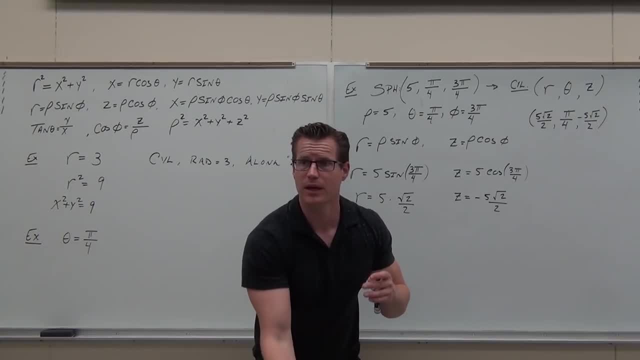 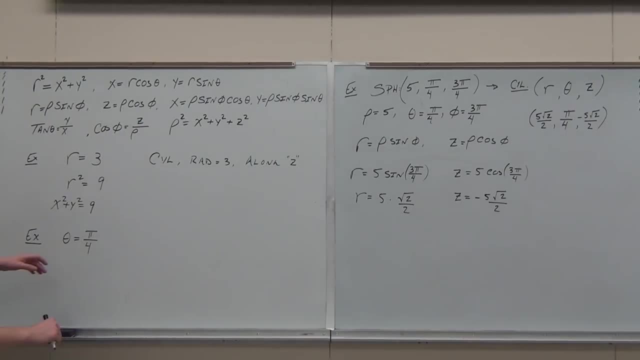 If you have a fixed angle and any points along that, that's going to be a plane. A plane at the angle of pi over 4.. I guarantee it's a plane. How can you prove it? Well, I know that Tangent theta equals y over x. 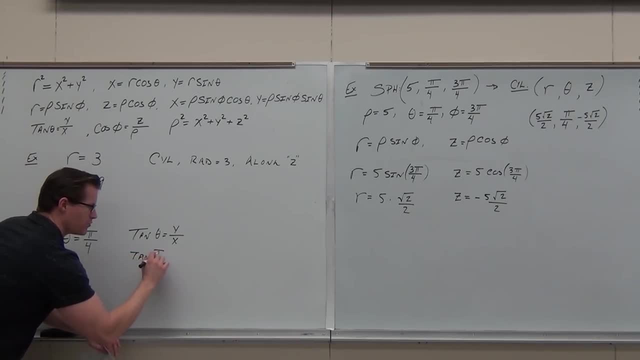 So tangent of pi over 4, or theta is pi over 4, has to equal y over x. But I know what tangent theta is, I know tangent, I'm sorry, tangent of pi over 4 is. I know it's 1, and if I solve for y, y equals x. 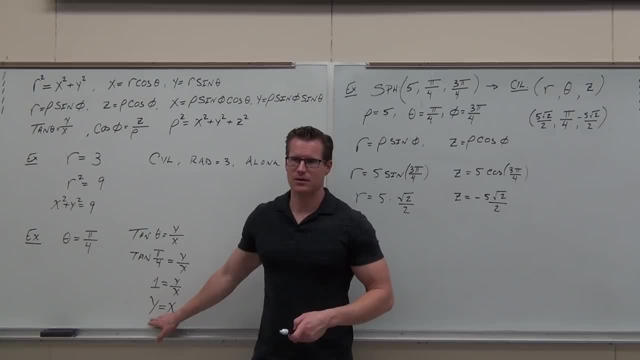 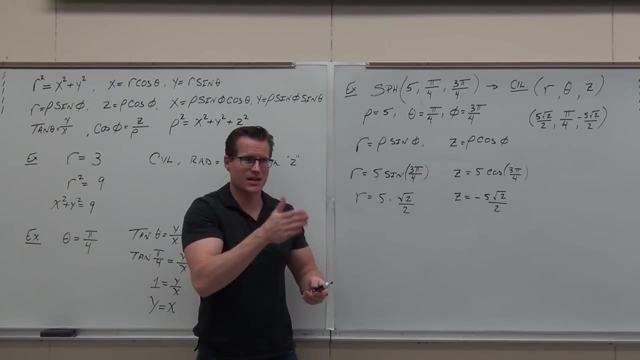 Okay, now stick with it. How many variables do you got? It's a cylinder, a really crappy cylinder called a plane. okay, It's going along the z-axis, but it's just y equals x. It's that line, and then it's going right along the z-axis. 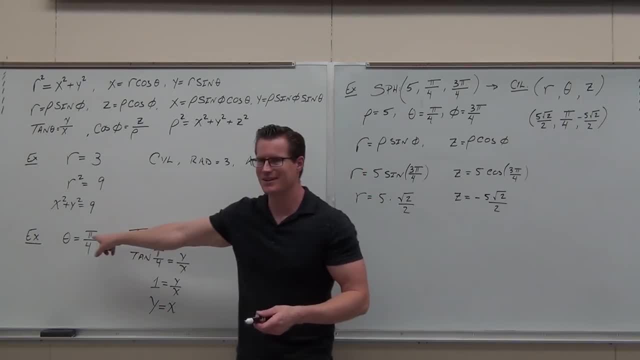 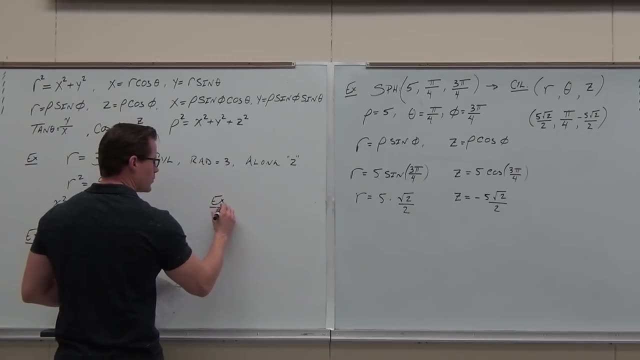 Do you guys see what I'm talking about? That's kind of cool. That's what this is. Which one's easier? That one It's, because it's equal to a constant. Let's talk about one more like this, and then we'll do some tougher ones. 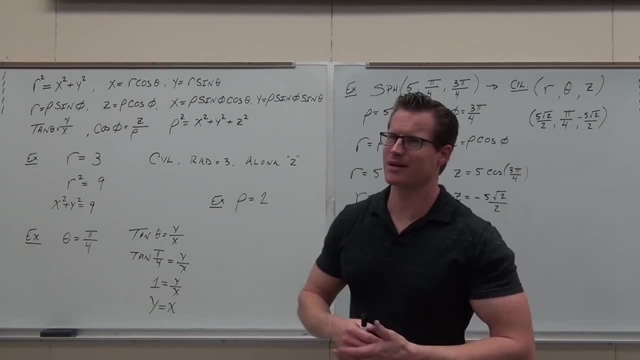 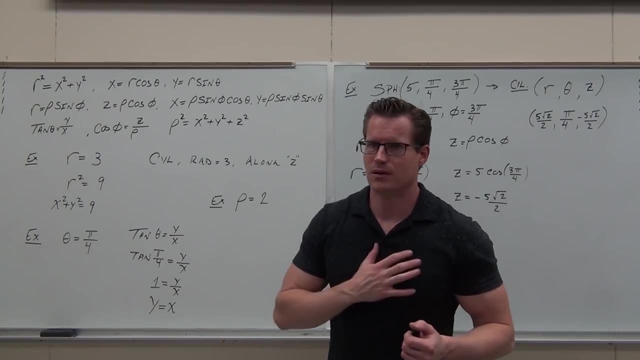 Okay, real quick. what in the world is? what is that? What is that thing? Would that be rectangular or cylindrical or spherical? What is that Spherical? Obviously spherical, because, whoa, I'm palpitating a little bit right there. 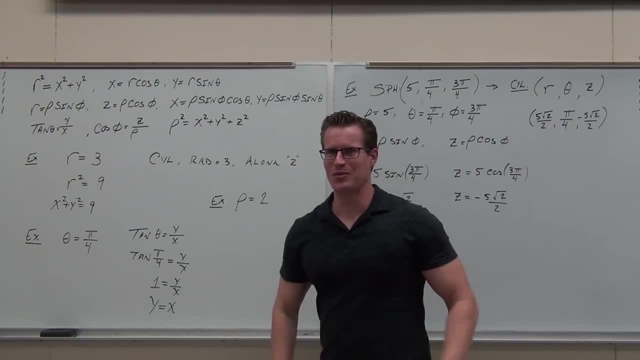 Easy, I'm getting a heart attack. I'm already excitable, man. I have way too much caffeine and candy. Whoa, That's a double whammy. So it's obviously spherical because you've got that row in there. 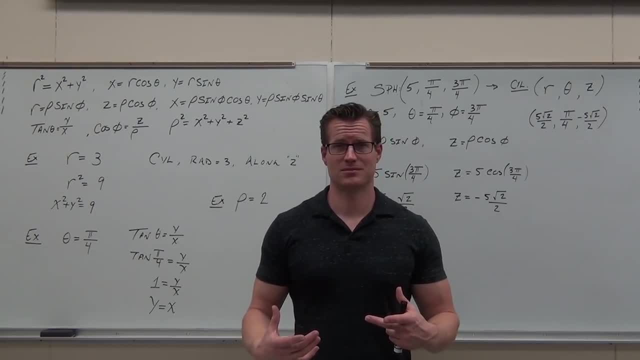 Listen. Okay, that's 2.. You're trying to kill me Anytime. you want to do something, you're going to have to do it. You're going to have to do it. You're going to have to do it. 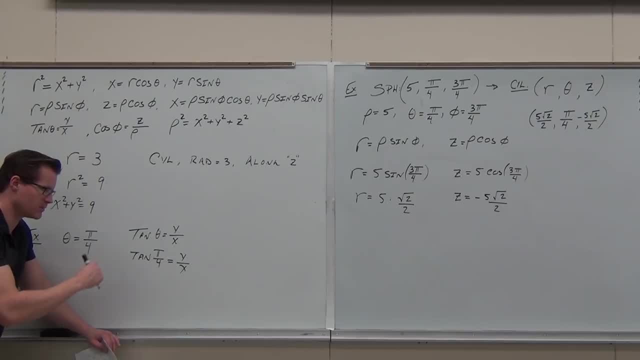 But I know what tangent theta is. I know tangent, I'm sorry, Tangent of pi over 4 is. I know it's 1, and if I solve for y, y equals x. Okay, now stick with it. How many variables you got? 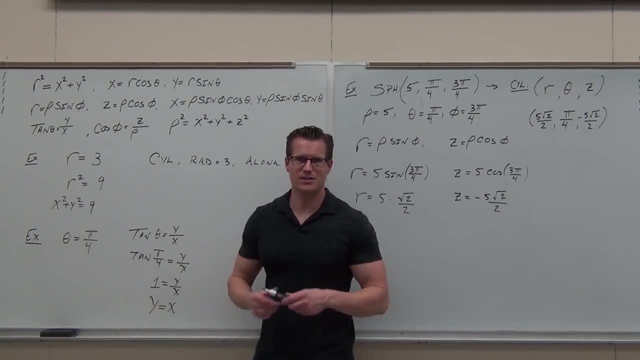 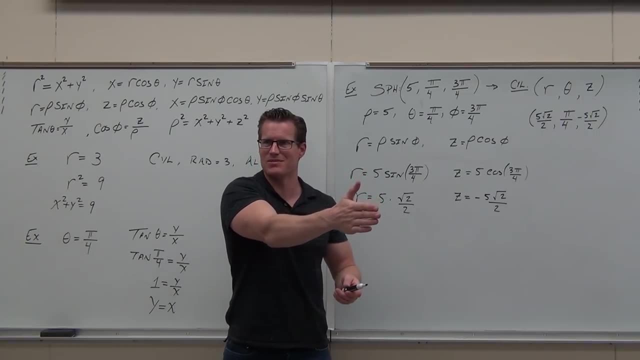 It's a cylinder, a really crappy cylinder, called a plane. okay, It's going along the z-axis, but it's just y equals x. It's that line, and then it's going right along the z-axis. Do you guys see what I'm talking about? 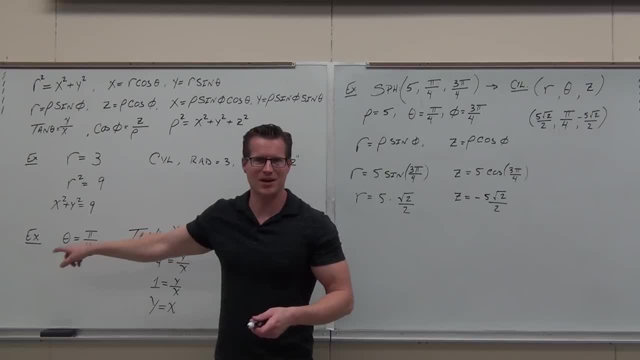 That's kind of cool. That's what this is. Which one's easier? That one It's, because it's equal to constant. Let's talk about one more thing We're going to do like this, and then we'll do some tougher ones. 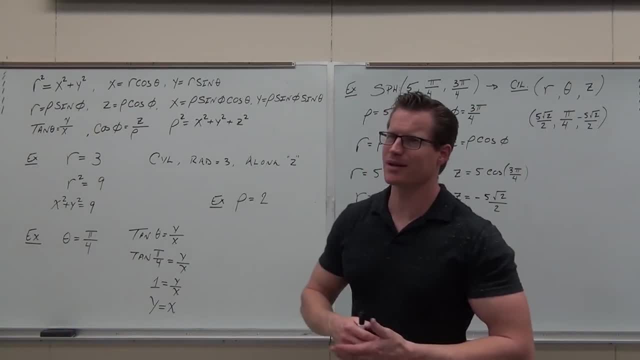 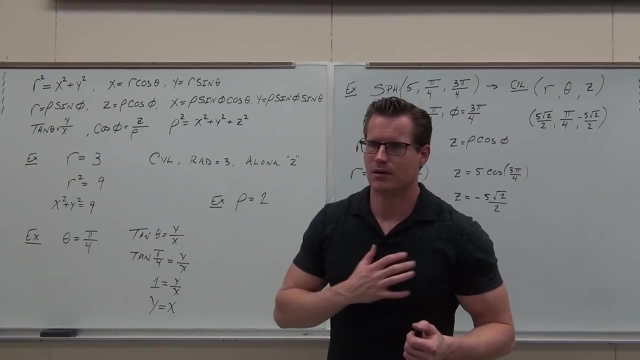 Okay, real quick. what in the world is? what is that thing? What is that thing? Would that be rectangular or cylindrical or spherical? What is that? It's spherical. Obviously it's spherical, because, whoa, I'm palpitating a little bit right there, easy. 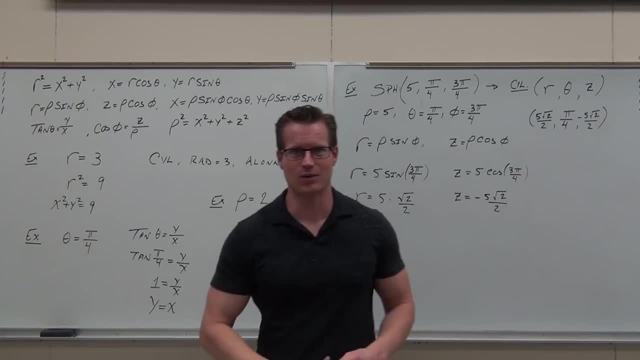 I'm getting a heart attack. I'm already excitable, man. I have way too much caffeine and candy. Whoa, That's a whammy. So it's obviously. It's obviously spherical, because you've got that, that row in there. 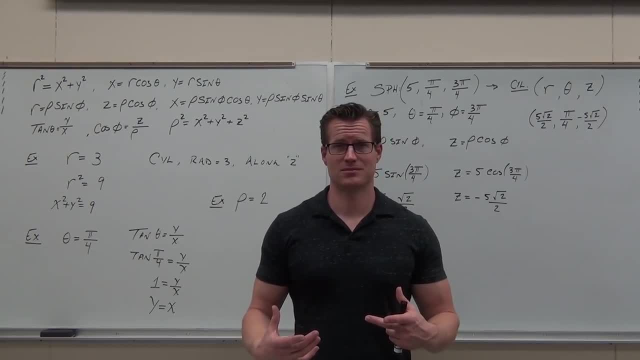 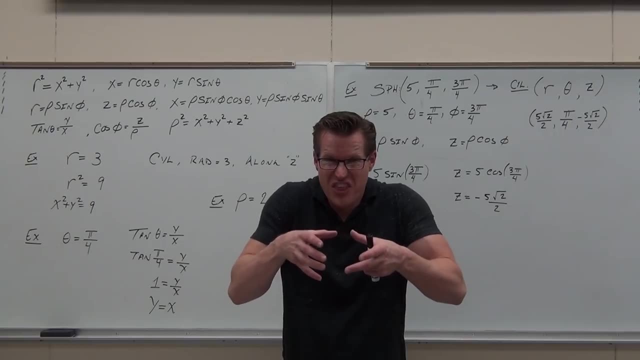 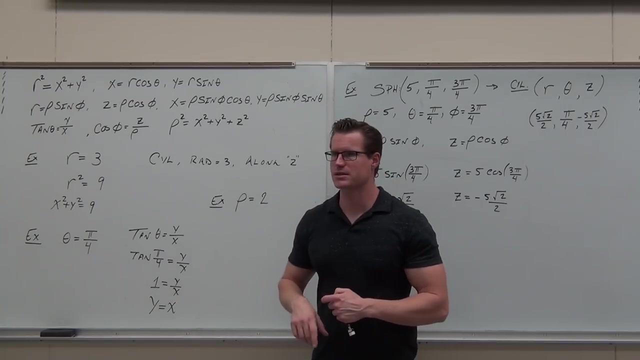 Listen. Okay, that's two. You're trying to kill me. Anytime, you have the base thing of your coordinate system equal to constant. you have the thing. So if I'm in spherical coordinates and that's equal to a constant, that is a sphere. 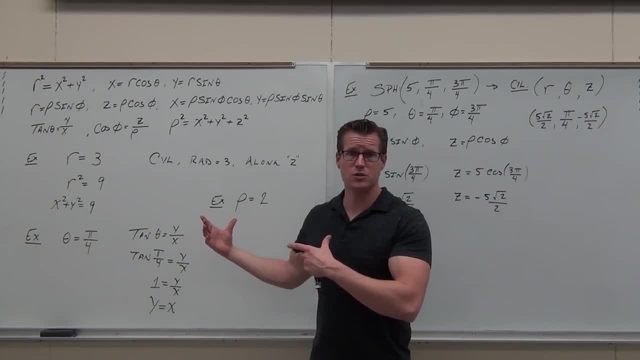 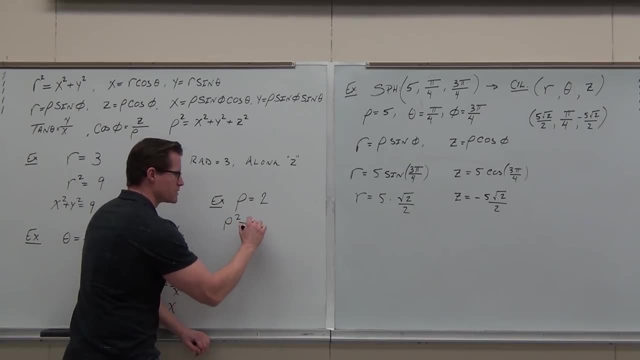 That's a sphere centered at the origin, with a radius of- what do you think? Two, Two. How do I know? Same thing that we would do here. So, sphere radius two, centered at the origin. for sure, Let's square both sides. 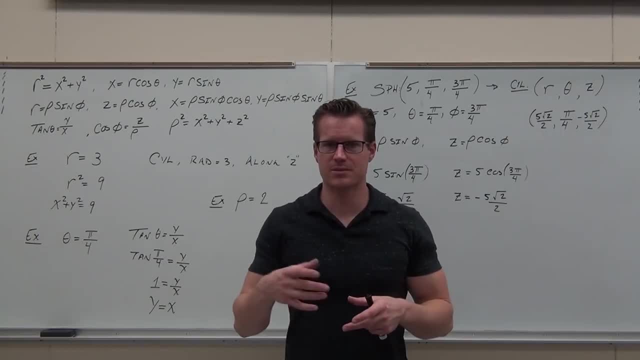 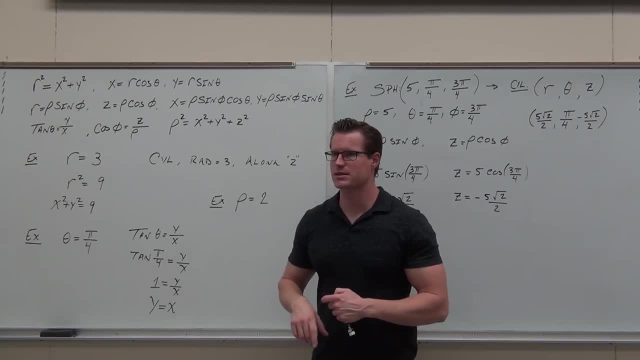 So if I'm in spherical coordinates and that's equal to a constant, that is a sphere, That's a sphere centered at the origin, with a radius of- what do you think? 2., 2. How do I know? Same thing that we would do here. 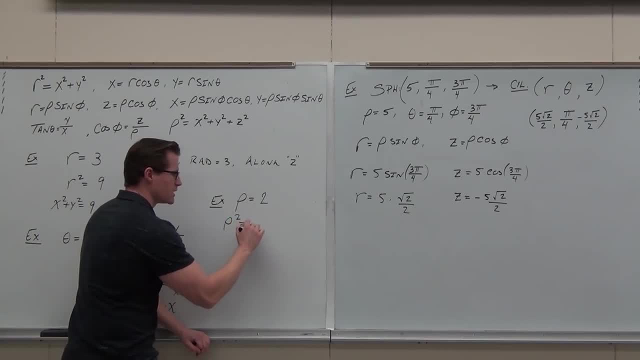 So a sphere radius 2 centered at the origin. for sure, Let's square both sides. Oh but wait. X squared plus y squared plus z squared equals 1.. equals 4.. That's the definition of what a sphere is, In fact, if you want to put it. 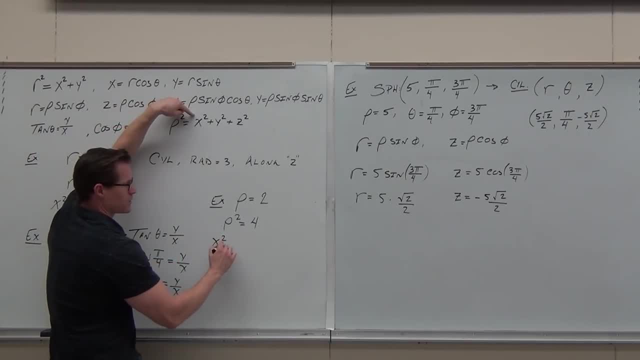 Oh but wait. X squared plus Y squared plus Z squared equals four. That's the definition of what a sphere is In fact. if you want to put it in standard form, just divide by four, you've got square plus square plus square equals constant. 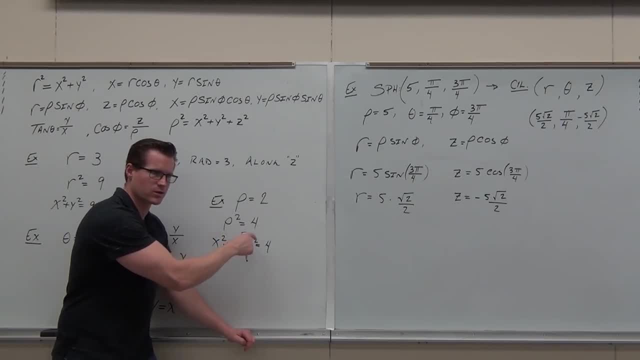 You guys see what I'm talking about. It's square plus square plus square, all squared, All pluses equal to a constant. That's an ellipsoid. However, it's an ellipsoid. It's an ellipsoid where all the denominators are the same. 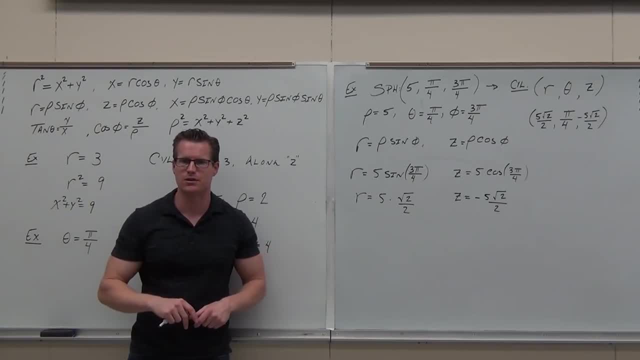 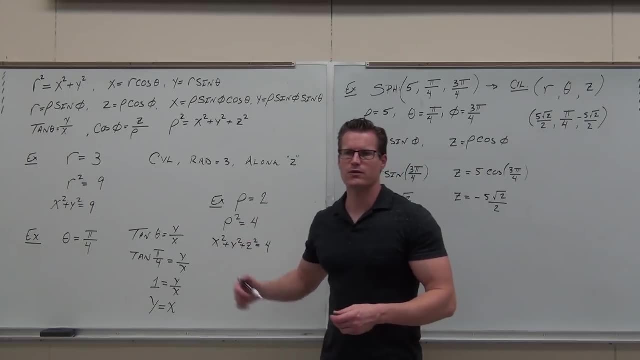 Ellipsoids spread out equal and distant from the origin, creates a sphere, That's a sphere centered at the origin, with a radius of two. Which one's an easier formula to work with? Oh, my goodness, that one. It's got one variable and it's really nice. 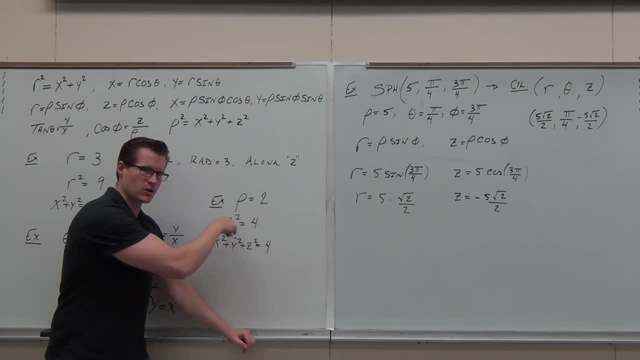 in standard form, just divide by 4, you've got square plus square plus square equals constant. You guys see what I'm talking about. It's square plus square plus square, all squared, All pluses equal to a constant. That's an ellipsoid. However, it's an ellipsoid where 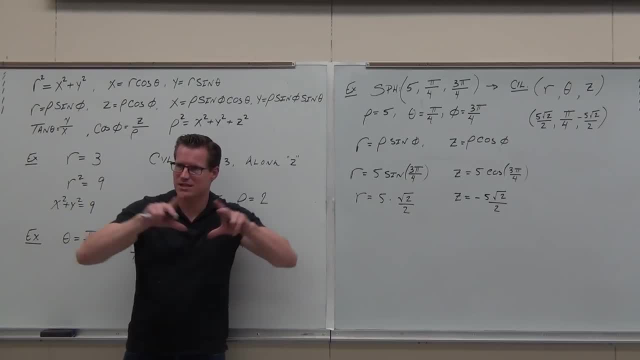 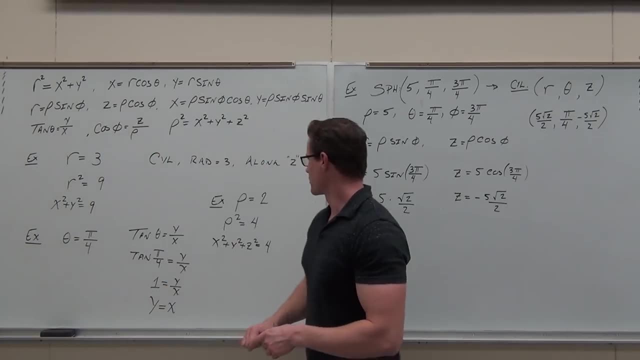 all the denominators are the same. Ellipsoids spread out equal and distant from the origin creates a sphere, That's a sphere centered at the origin, with a radius of 2.. Which one's an easier formula to work with? Oh, my goodness that one. It's got one variable and it's really. 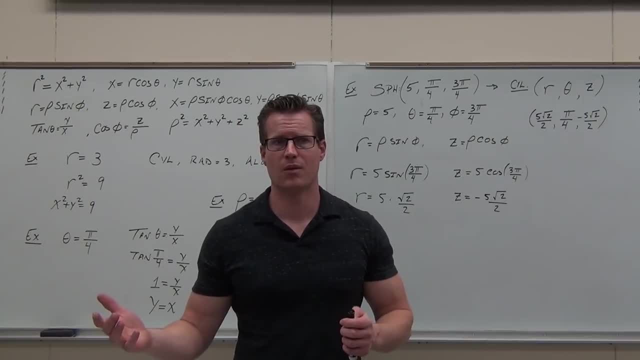 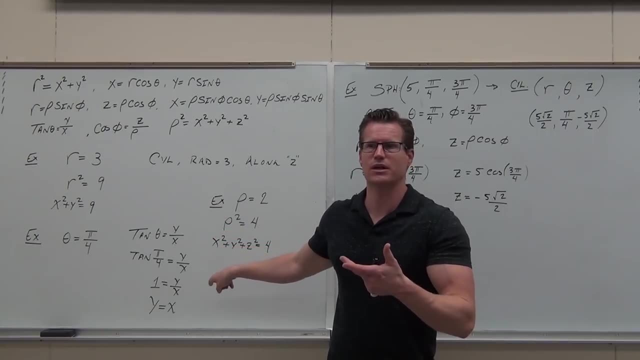 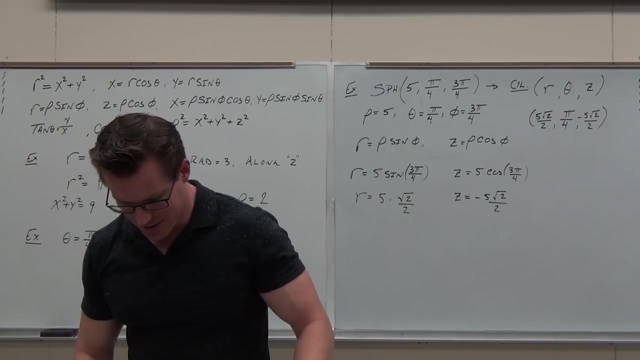 nice. So when we get to stuff like triple integrals and we have to integrate over spheres, try to use that, because that sucks to work with in an integral. You can picture it. It's not fun. So that's what we're using this stuff for Now. some of them, man, they're 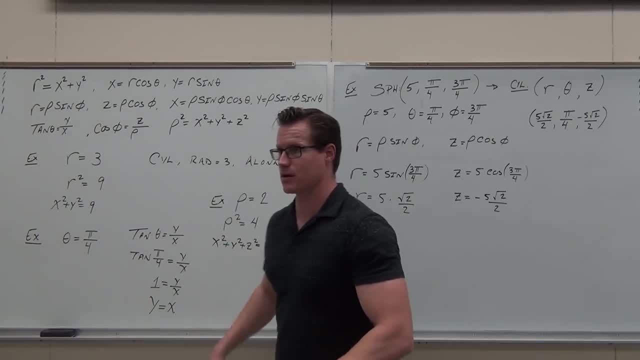 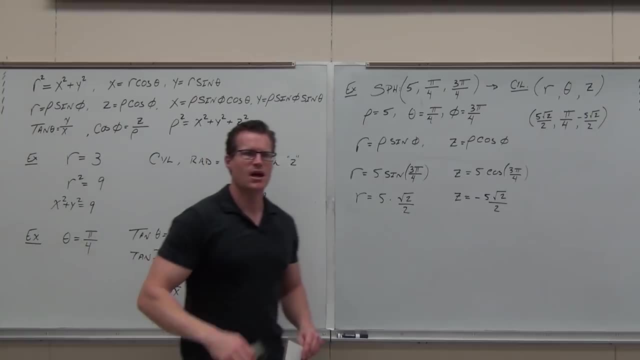 not that obvious, honestly, These. I mean that's not obvious, man. Well, at least there's something there You can get there. Sometimes we get something. These are really not obvious ones. That's what I really want to work on right now. This. 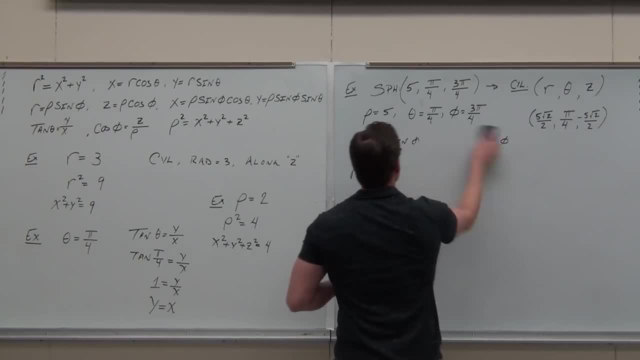 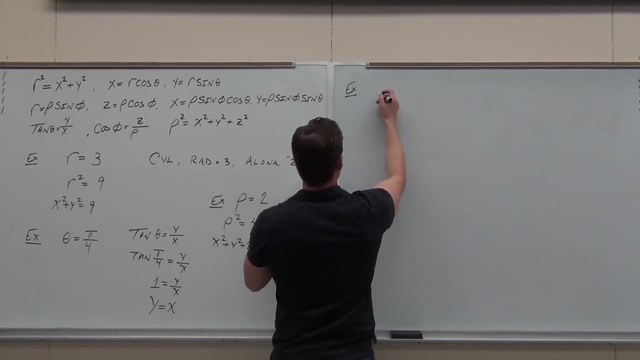 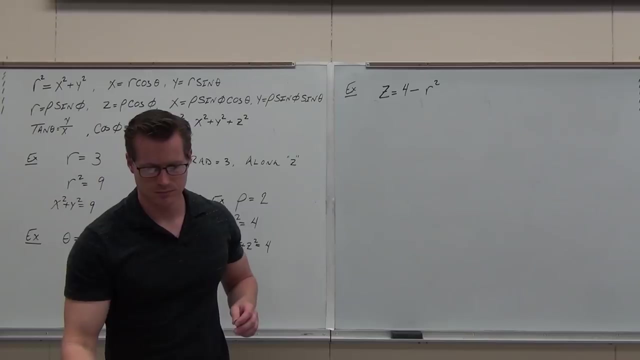 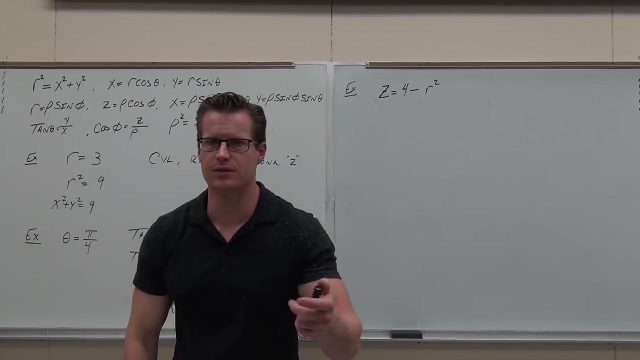 should be okay. I really want to work on these ones, Because these ones really don't look very nice And they're not readily apparent, like what in the world this thing even is. So when that's the case, when it's not obvious what they are, that should be obvious from. 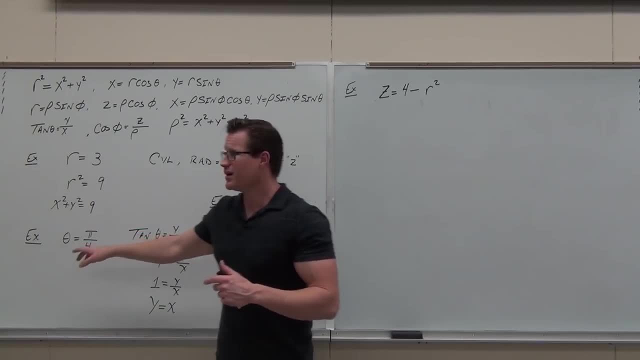 now on, That's a cylinder. That's pretty obvious. from now on, That's a plane. That's pretty obvious. That's a sphere. But from here on out, if it's not obvious, convert it to rectangular. Convert everything to rectangular. If it's not obvious, convert to rectangular. Why? 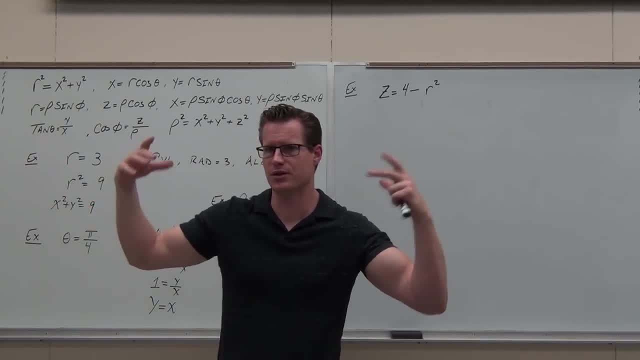 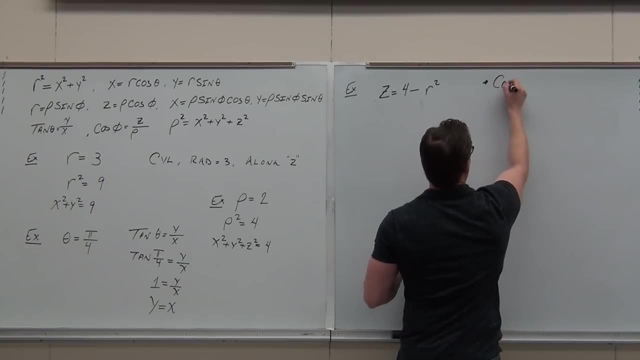 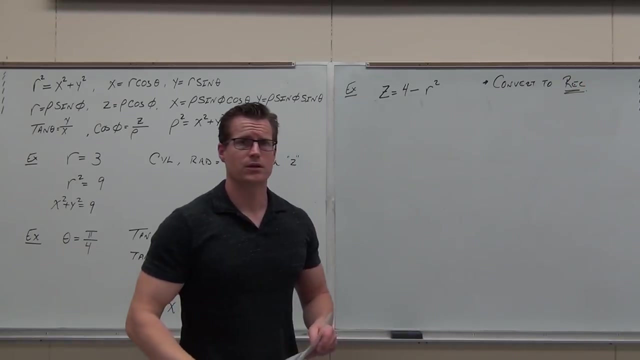 Because we already have rectangular set up in our heads. Does that make sense to you? I don't want to switch everything, Just kind of the easy ones. So when not obvious, convert to rectangular. Convert to rectangular. How, Using anything, you can, Don't change out variables that are: 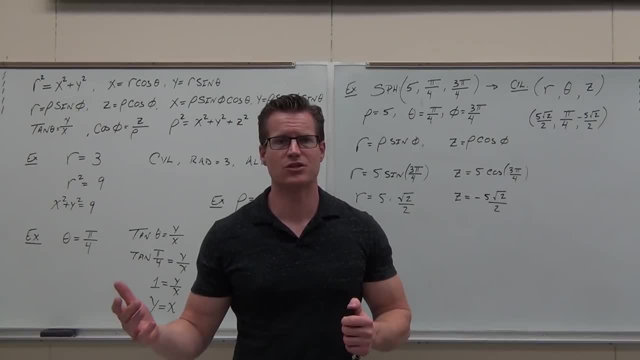 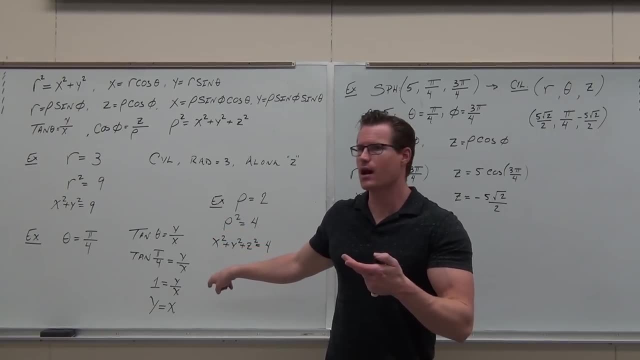 So when we get to stuff like triple integrals and we have to integrate over spheres, you're going to use that because that sucks to work with in an integral. You can picture it. It's not fun. So that's what we're using this stuff for. 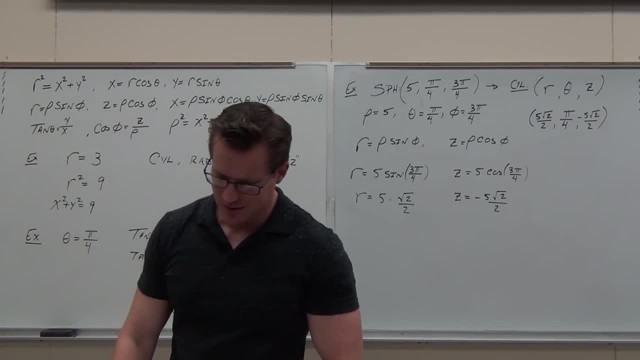 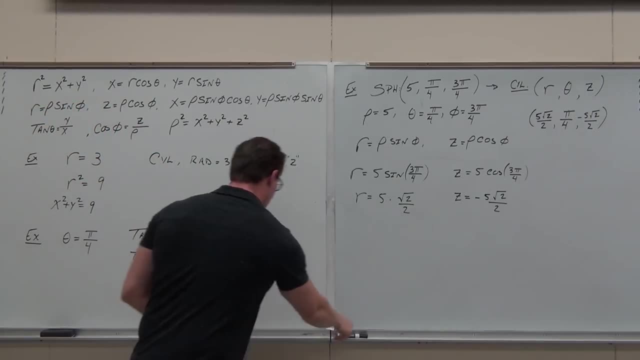 Now some of them, Man. they're not that obvious, honestly, These. I mean that's not obvious man. Well, at least there's something there You can get there. Sometimes we get some really not obvious ones. 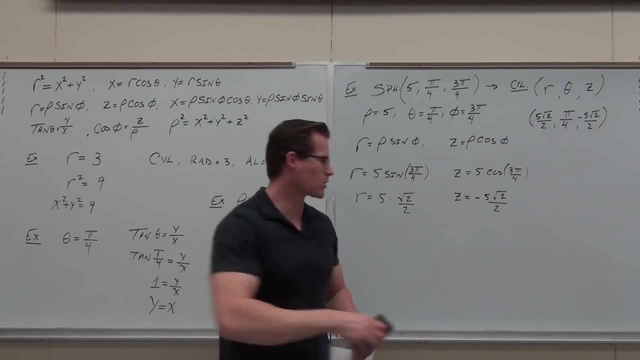 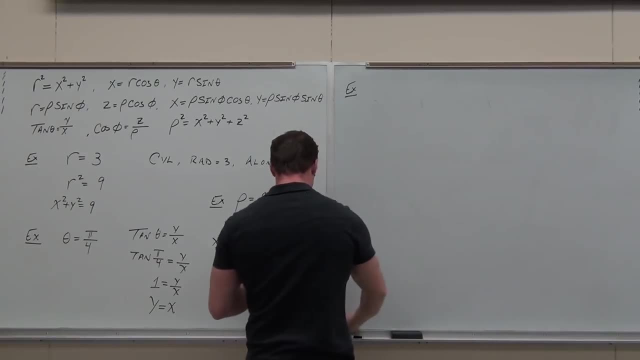 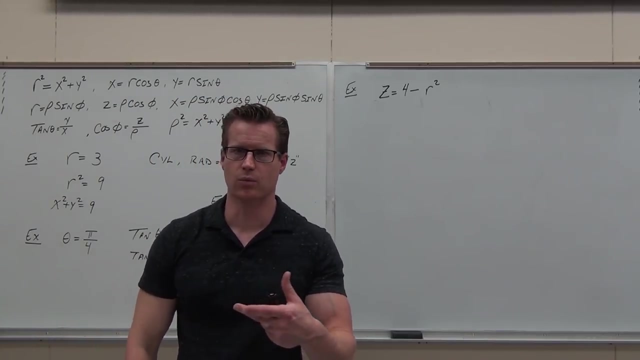 That's what I really want to work on right now. This should be okay. I really want to work on these ones, Because these ones really don't look very nice. They're not regularly apparent, like what in the world this thing even is. 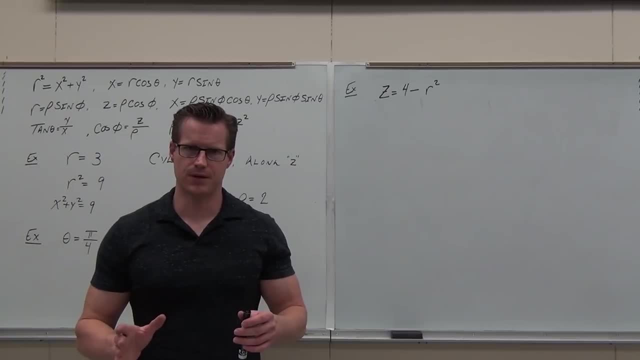 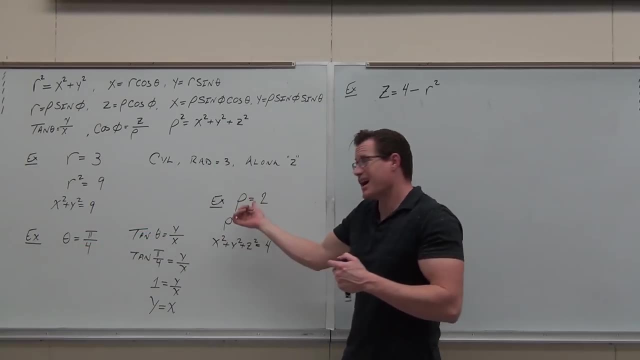 So when that's when that's the case, when it's not obvious what they are, that should be obvious from now on. a cylinder, That's pretty obvious from now on. that's a plane, Pretty obvious. that's a sphere. But from here on out, if it's not obvious, convert it to rectangular. 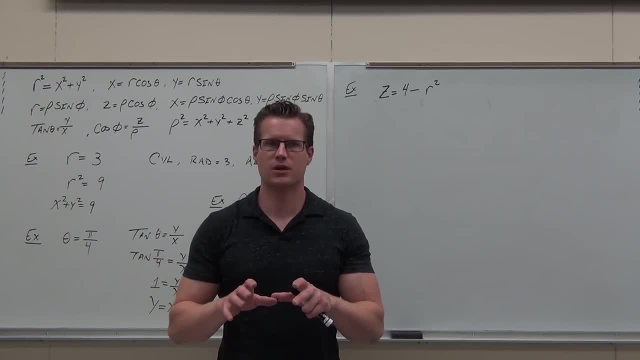 Convert everything to rectangular. If it's not obvious, convert all or something else, Then hey, well, I'm using it all the time. often: convert to rectangular. Why? Because we already have rectangular set up in our heads. Does that make sense to you? 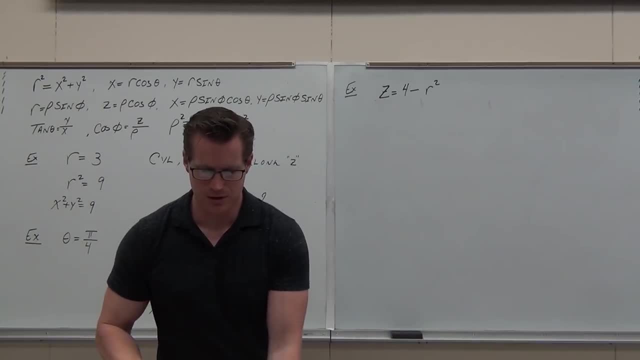 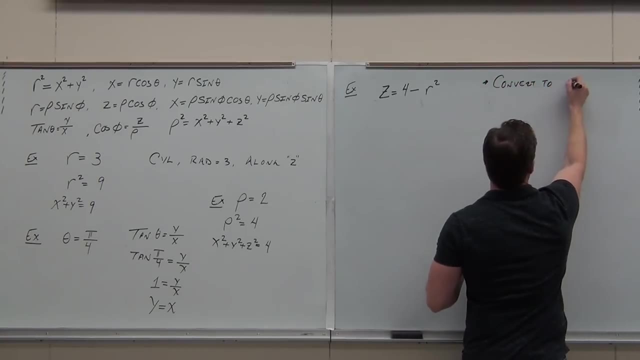 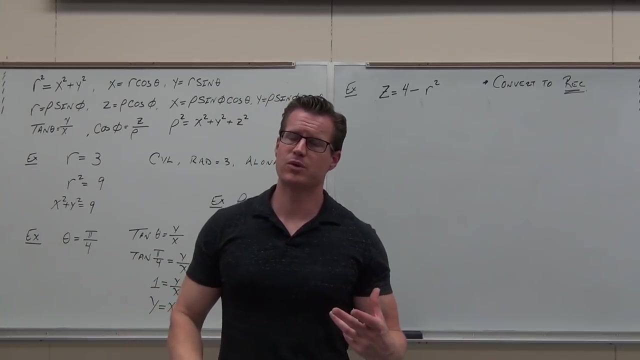 I don't want to switch everything, just kind of the easy ones. So, when not obvious, convert to rectangular. How, Using anything you can, Don't change out variables that are good for you. So, for instance, z's are pretty good for me for rectangular. 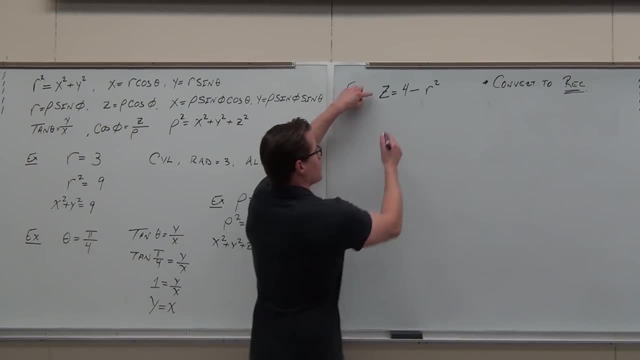 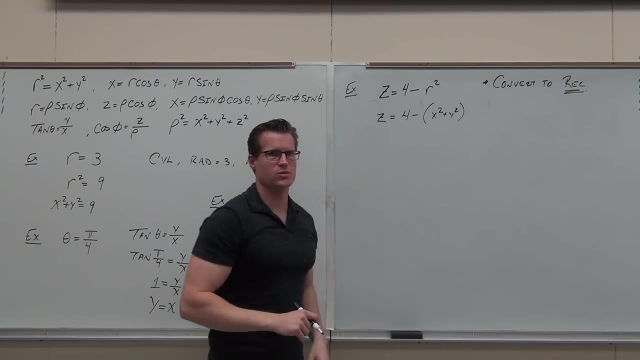 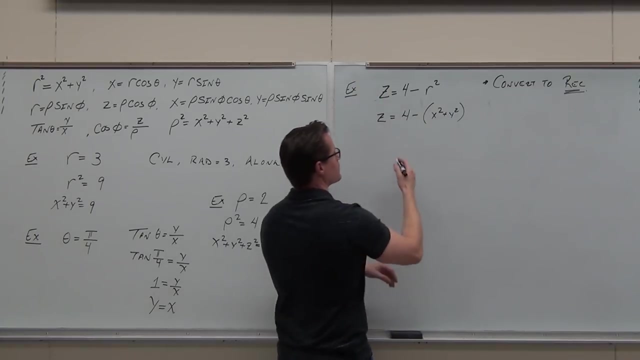 I'm going to change. these R's are pretty easy to change, So I know R squared- use parentheses- is x squared plus y squared. Make it a little bit prettier. In fact, what I would do is I'd add this to both sides: 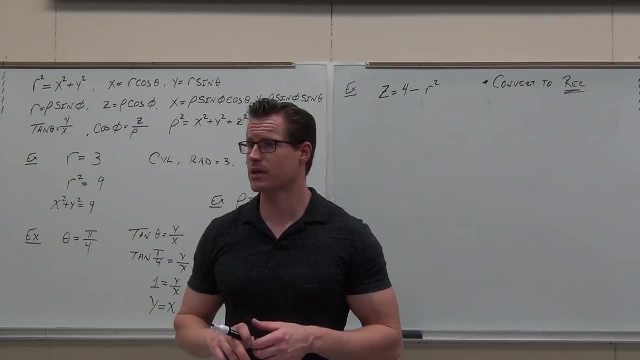 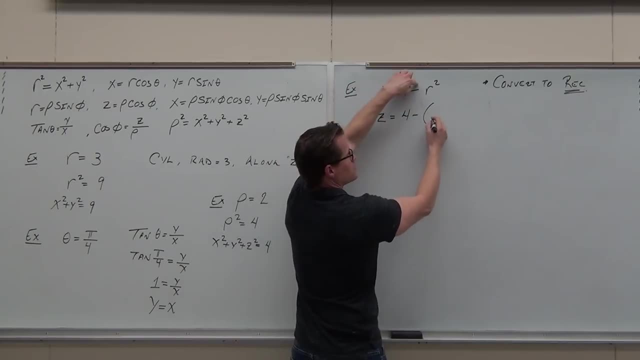 good for you. So, for instance, z's are pretty good for me for rectangular. Don't change z's. R's are pretty easy to change. So I know R squared- use parentheses- is x squared plus y squared. Make it a little bit prettier. In fact, what I would do is I'd add this to both sides. 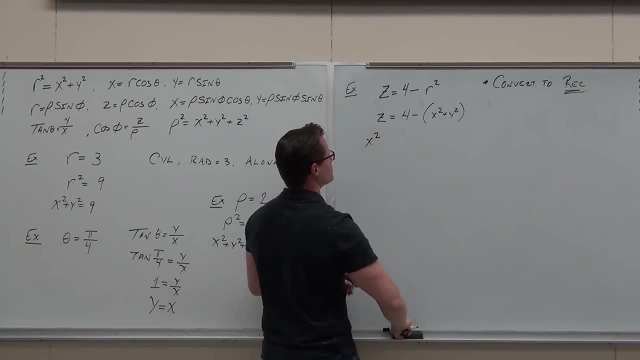 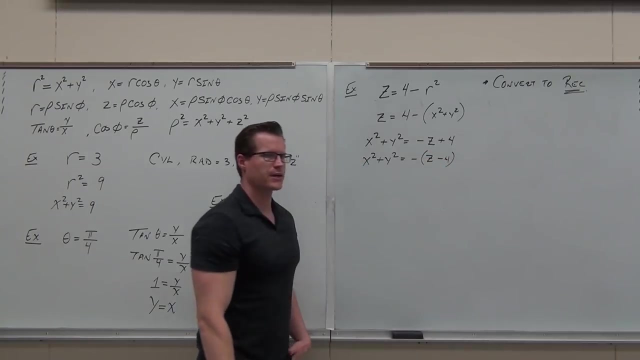 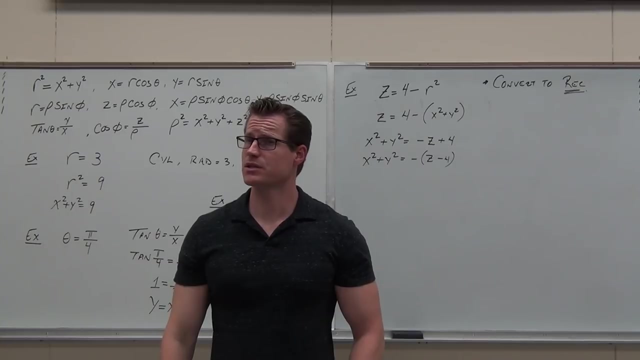 Well, no, Yeah, I would. I'd factor it, so it looks like something we started our day with. Do you remember that shape at all? It's a hyperboloid. It's obviously a surface. This is either a paraboloid or a hyperbolic paraboloid. Why? 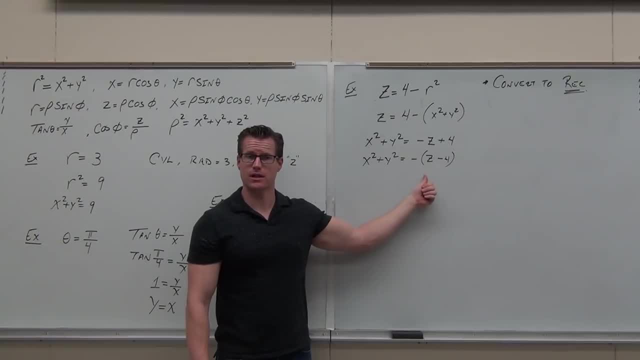 How many squares? you got Two, Two of them, And you have one that's not square, but these are both pluses. Come on, Hyperbolic paraboloid or paraboloid Paraboloid Paraboloid: Where Along what axis? 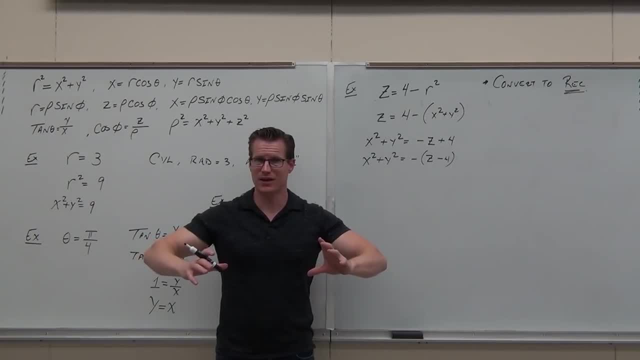 Z Opening towards the positive or negative, Negative, Negative And shifted up four. So this is shifted up four on the z opening this way with pictures of circle. Pictures of circle on the xy plane is what that looks like. That's. 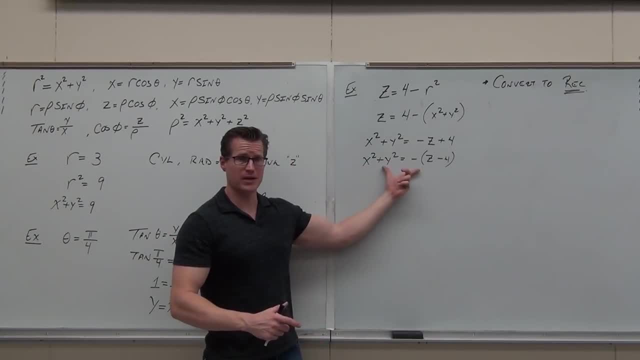 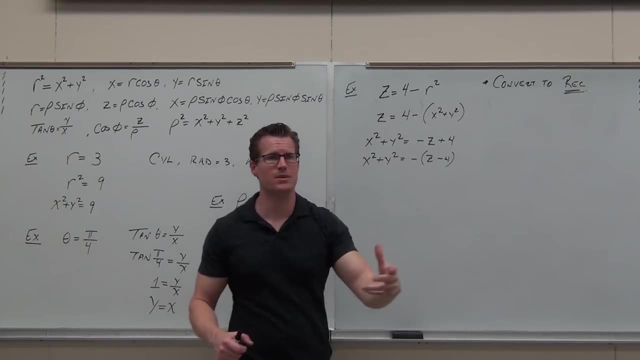 what it is, Just like that. Can you see this better than you can see that? Yes, Yes, You guys understand how to get from here to here. That's not the hard part. but I want you recognizing the shapes. I know you haven't practiced it yet, but I want you recognizing. 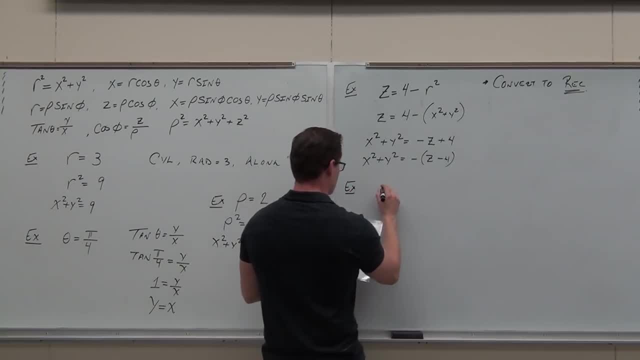 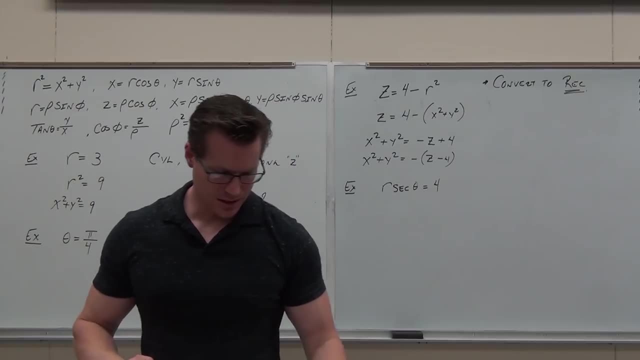 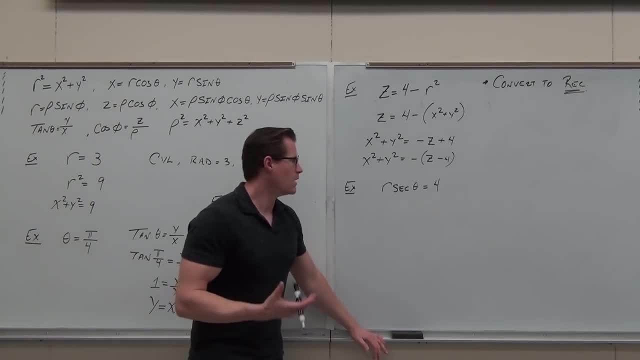 h. No, Some of them look really hard. You got to kind of be a little bit tricky on this stuff. So R secant theta equals four. This doesn't look good. I have nothing that. I don't want to start putting square roots up there. You can do things like this, OK. First thing: 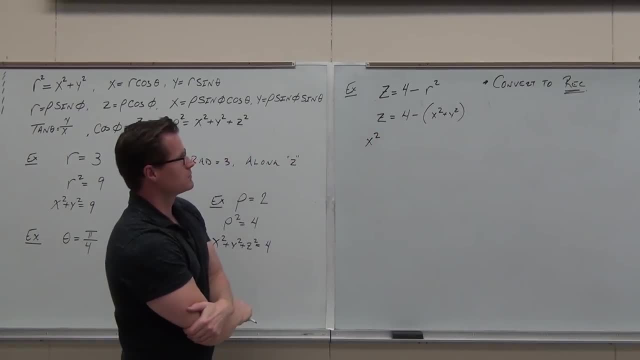 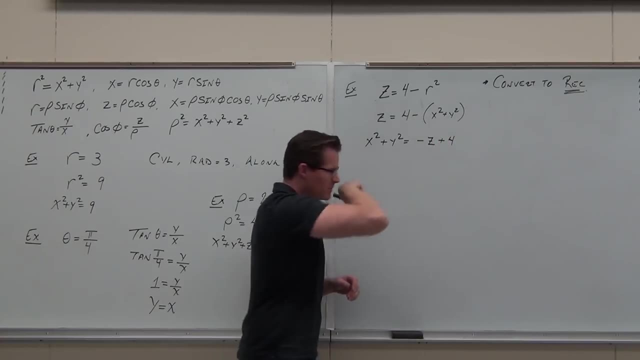 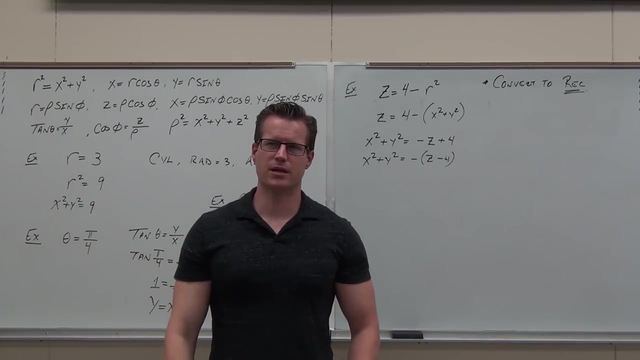 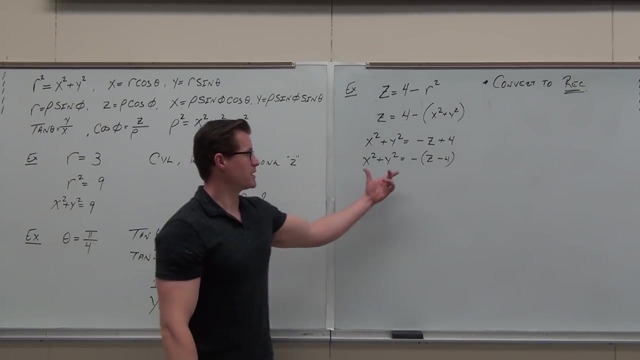 Well, no, Yeah, I would. I'd factor it, so it looks like something we started our day with. Do you remember that shape at all? It's obviously a surface. This is either a paraboloid or a hyperbolic paraboloid. 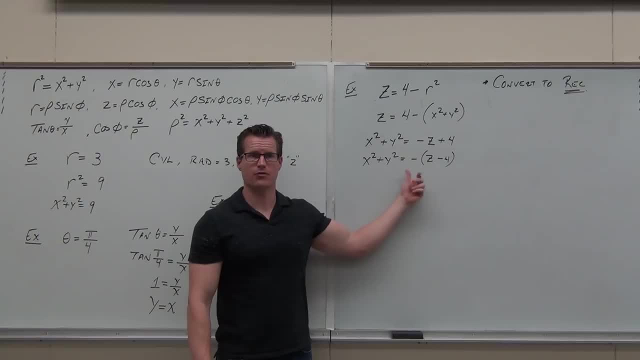 Why? How many squares? you got Two, Two of them, And you have one that's not square, But these are both pluses. Come on, hyperbolic paraboloid or paraboloid Paraboloid Paraboloid. 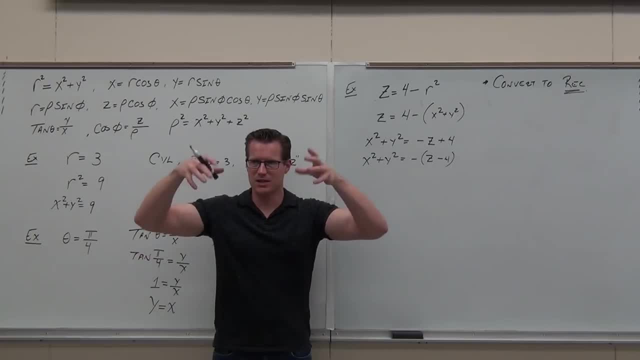 Where Along what axis, Z Opening towards the positive or negative, Negative, Negative, and shifted up four. So this is shifted up four on the z, opening this way with pictures of circle. Pictures of circle on the xy plane is what that looks like. 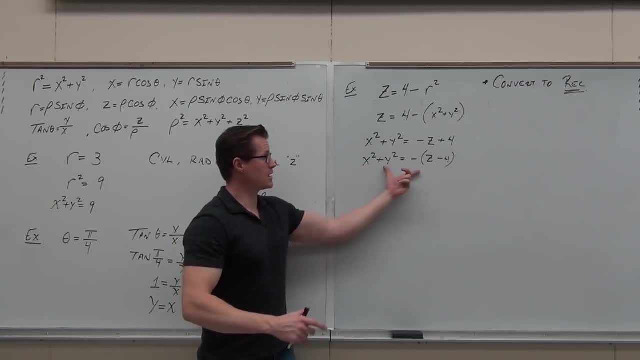 That's what it is. Just like that. Can you see this better than you can see that? Yes, Yes, You guys understand how to get from here to here. That's not the hard part, but I want you recognizing the shapes. 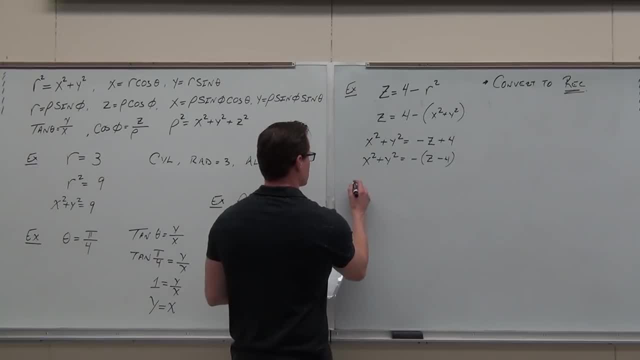 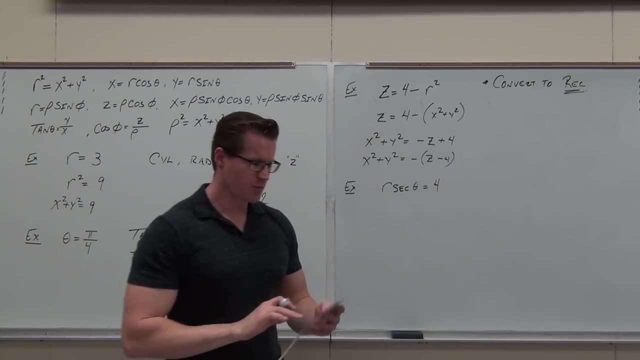 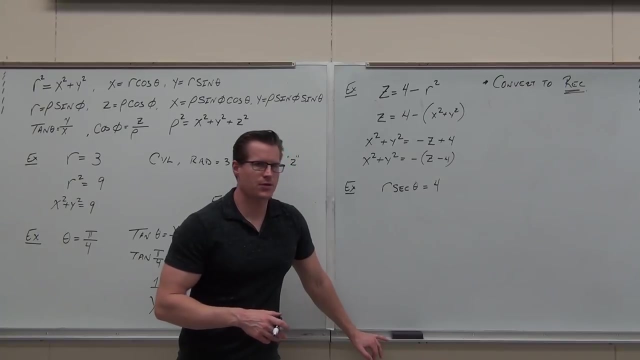 I know you haven't practiced it yet, but I want you recognizing the shapes. Some of them look really hard. You got to kind of be a little bit tricky. a little tricky on this stuff. So r secant theta equals four. This doesn't look good. 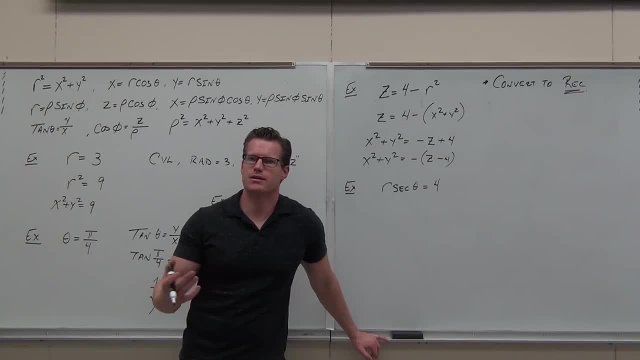 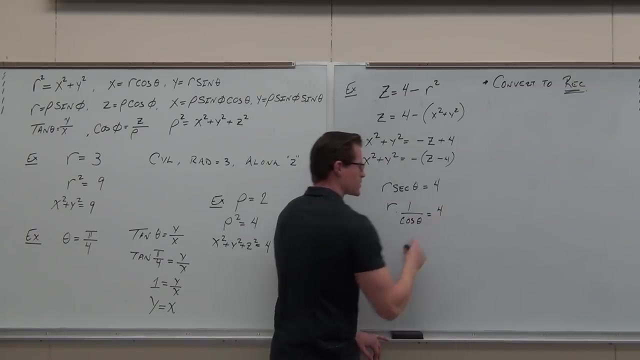 I have nothing that I don't want to start putting square roots up there. You can do things like this: First thing, try to get sines and cosines, because I don't see a secant anywhere up there. So what I know is that this is r times one over cosine. 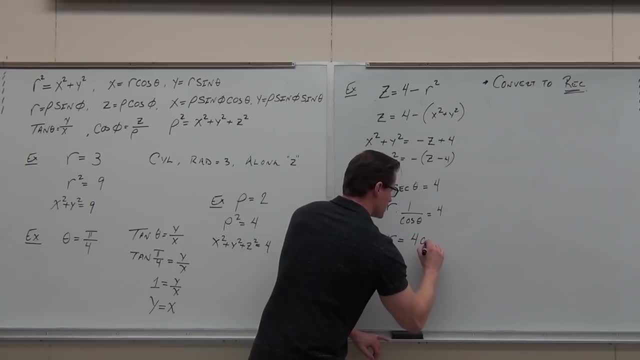 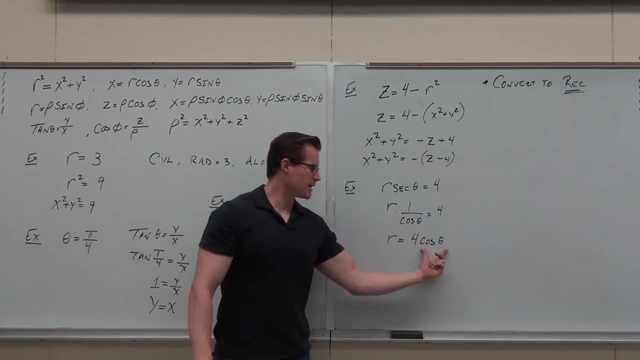 If I multiply by both sides, both sides by cosine, it looks a little better, but not way better. And then you go: how about this one? I know that I like cosine, as long as cosine has an r in front of it. 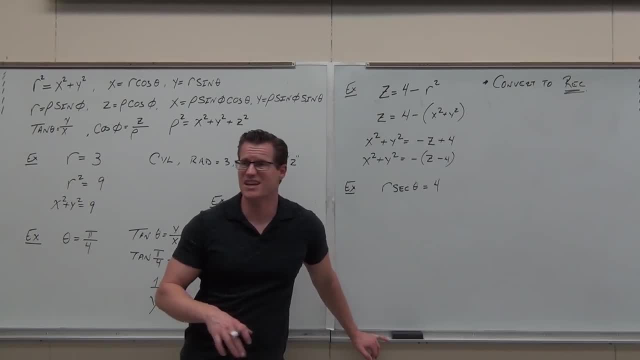 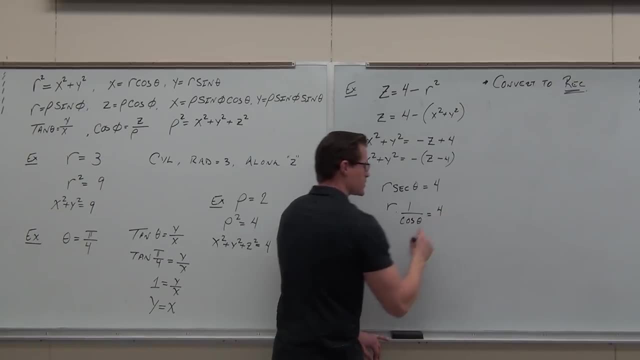 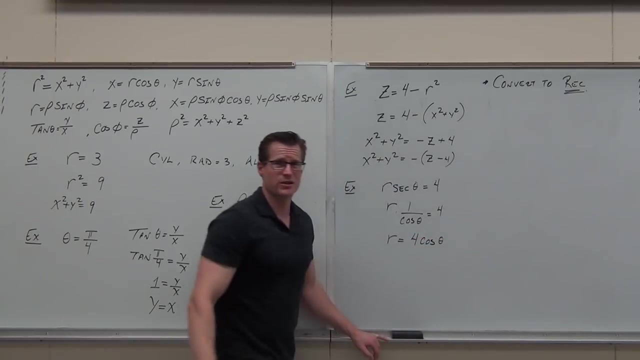 try to get sines and cosines. I don't see a secant anywhere up there. So what I know is that this is R times 1 over cosine. If I multiply both sides by cosine that looks a little better, but not way better. 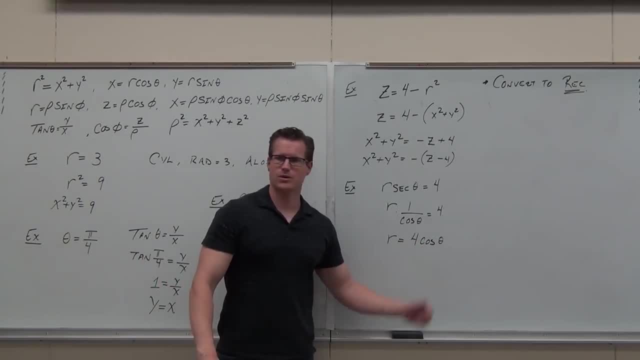 And then you go: how about this one? I know that I like cosine as long as cosine has an r in front of it. I know I like r's as long as they're squared. Let's multiply both sides by r. These are things that you can do. 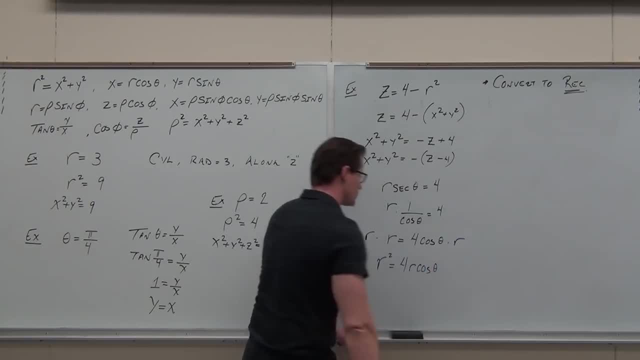 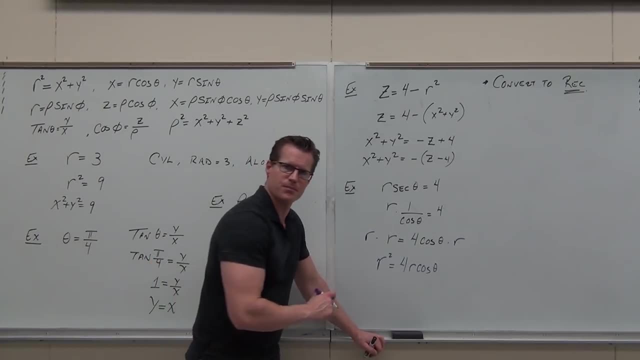 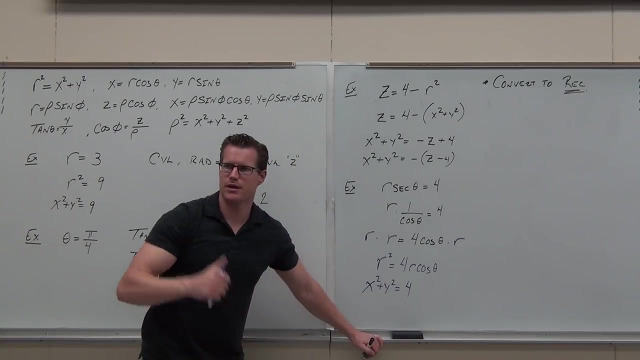 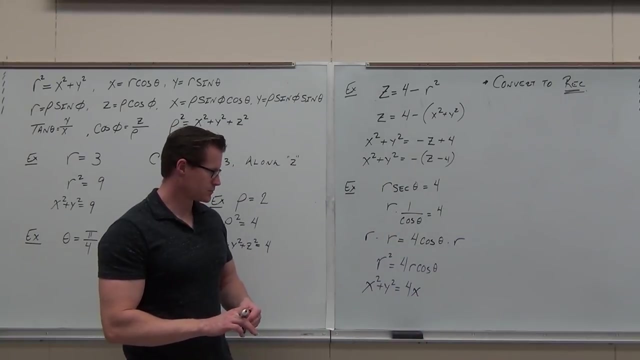 Tell me right now what is r squared in terms of x's and y's. What is that? How much is r cosine theta? Hopefully this will be burning in your head. How much is r cosine theta? That's x. You guys? okay with that one. 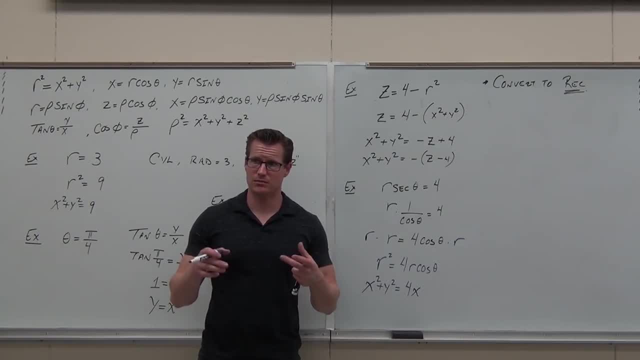 Multiply both sides, if you can Be creative with this, As long as you're not dividing out, well, multiply whatever you want. As long as you're doing the same side, That's okay. Square both sides, it's fine. Now do you know what that is? 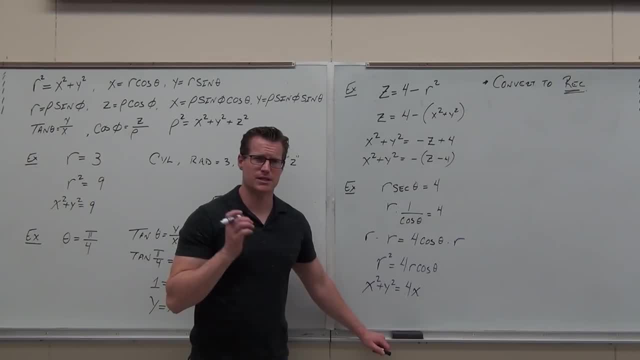 How many variables do you have? So I guarantee it's a. it's got to be a cylinder, For sure it's got to be a cylinder. Now what's it look like? That takes a little bit more math magic here. 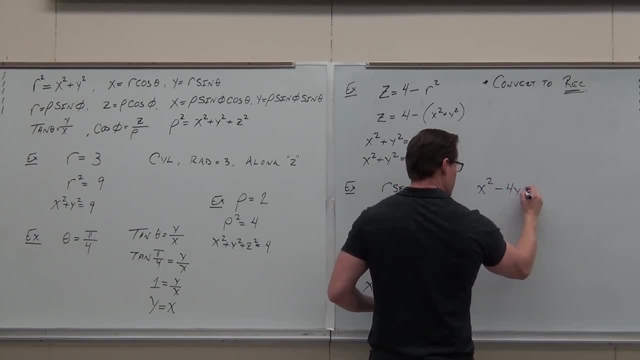 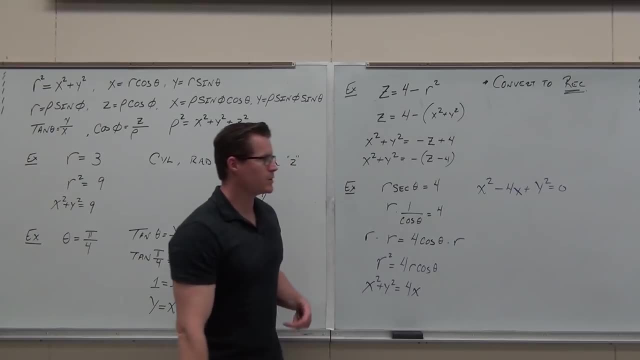 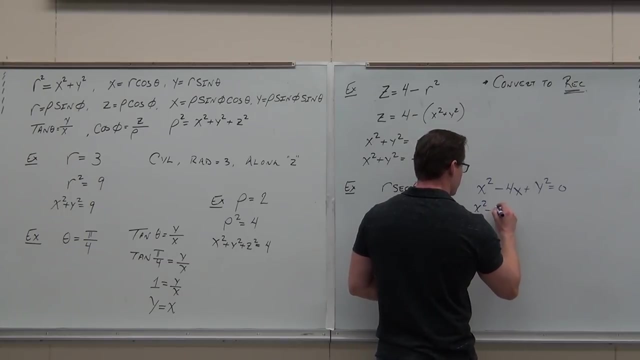 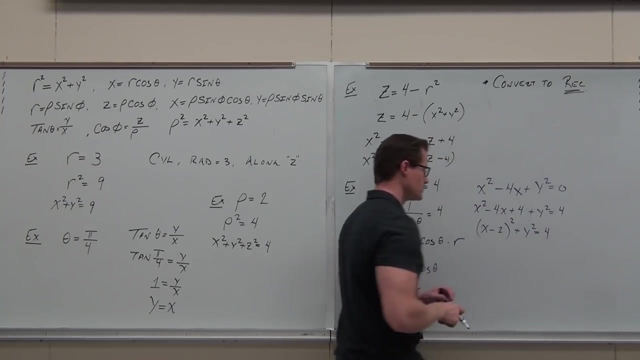 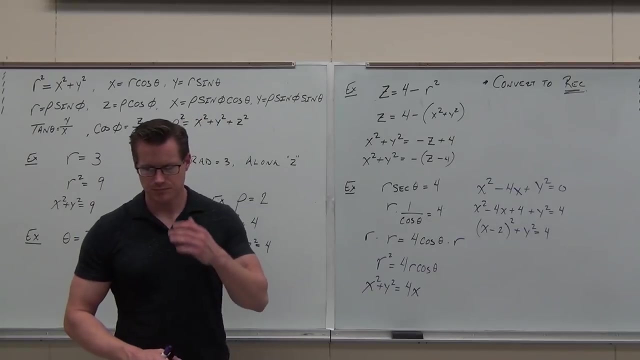 So we do things like x squared minus 4x Plus y squared. We do things like complete the square. We did it. I think one of the first days of class We did it a little bit more. okay, Can we get something? at least a little bit? 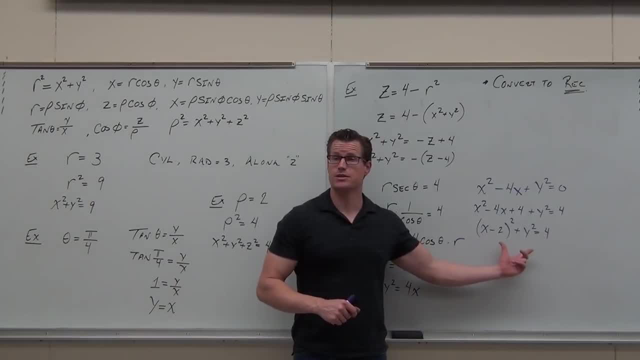 more identifiable. Is it still a cylinder? Yes, It's traveling along what axis please? And this is a circle with a radius of two. but it shifted, oh, come on, shifted along the x axis, positive 2. Positive, All right. 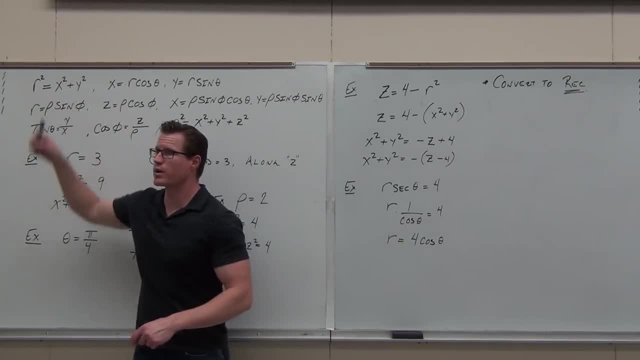 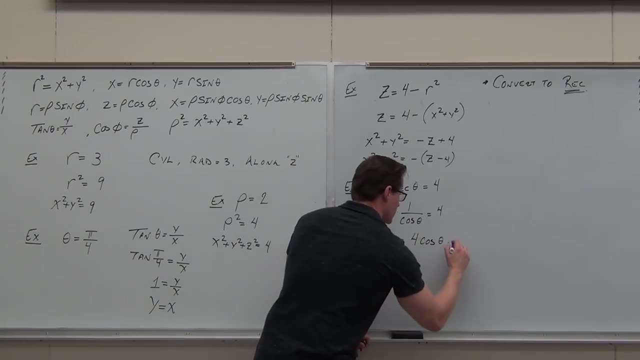 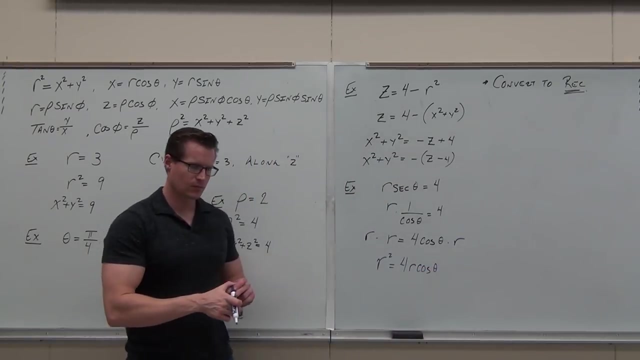 I know I like r's, as long as they're squared. Let's multiply both sides by r. These are things that you can do. Tell me right now what is r squared in terms of x's and y's? What is that? 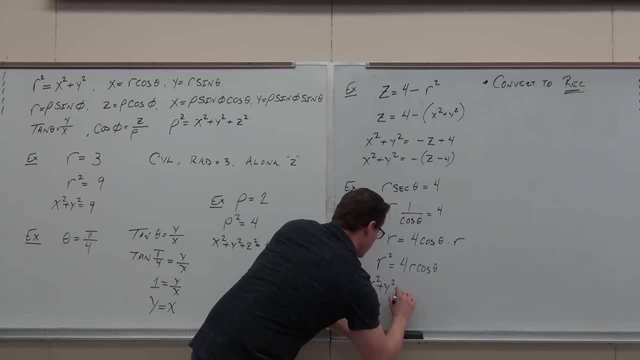 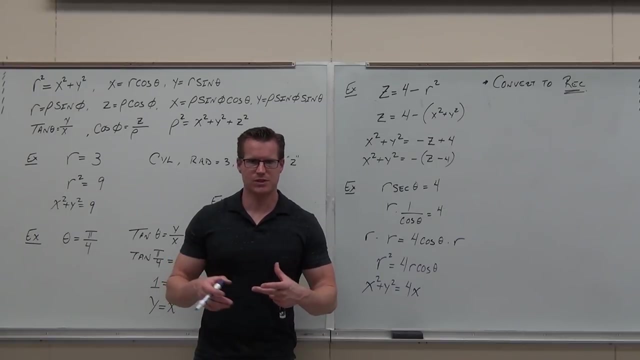 How much is r cosine theta? Hopefully this should be burning in your head. How much is r cosine theta x? You guys, okay with that one. Multiply both sides, if you can Be creative with this stuff, As long as you're not dividing out, well, multiply whatever you want. 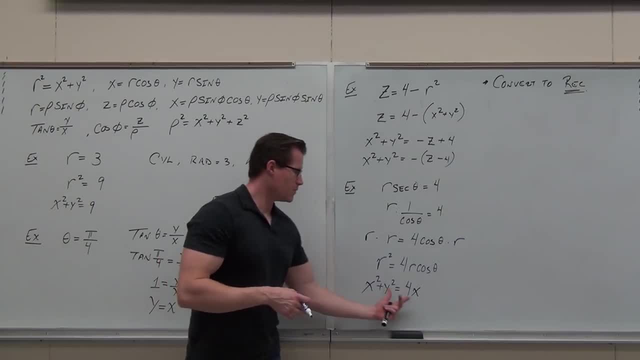 As long as you're doing the same side, That's okay. Square both sides, It's fine. Now do you know what that is? How many variables do you have? Two? So I guarantee it's a Cylinder. It's got to be a cylinder. 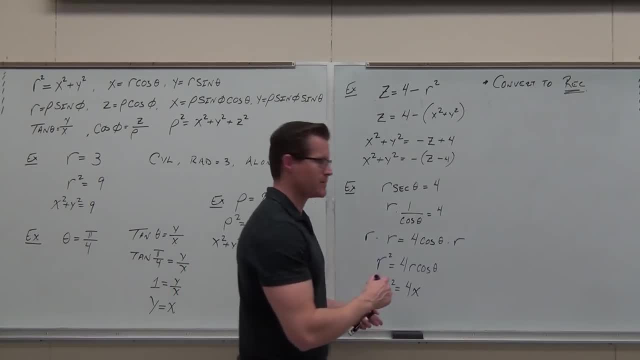 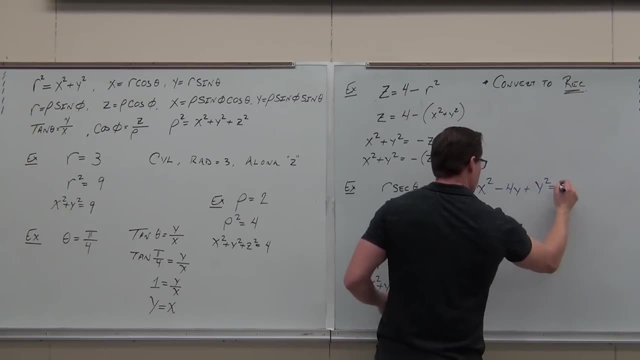 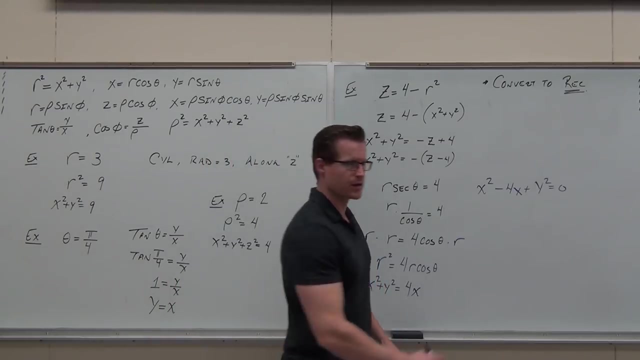 For sure going to be a cylinder. Now what's it look like? That takes a little bit more math magic here. So we do things like x squared minus 4x plus y squared. We do things like complete the square. We did it, I think, one of the first days of class. 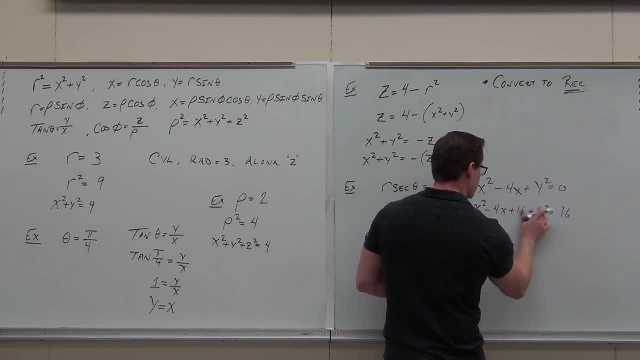 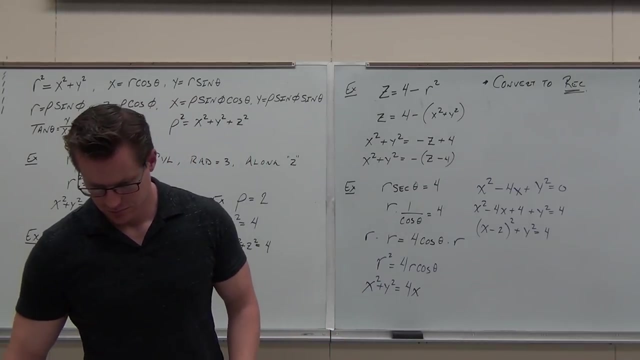 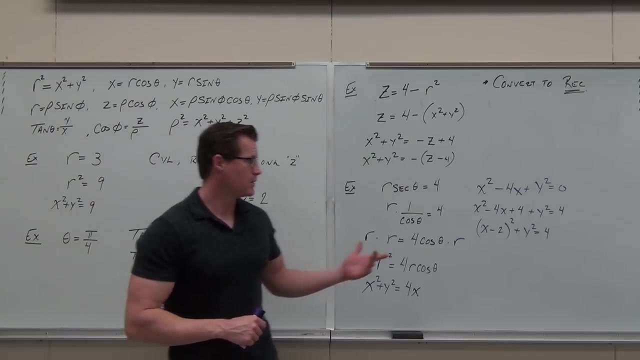 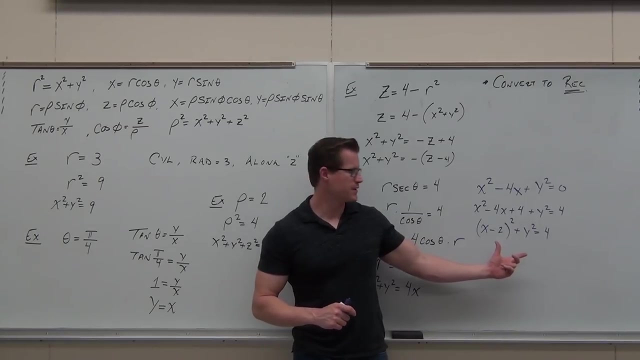 We did it, I think, one of the first days of class. We get something at least a little bit more identifiable. Is it still a cylinder? Yes, It's. traveling. along what axis? Y, Y. Then what is this? Y is a circle with a radius of 2.. 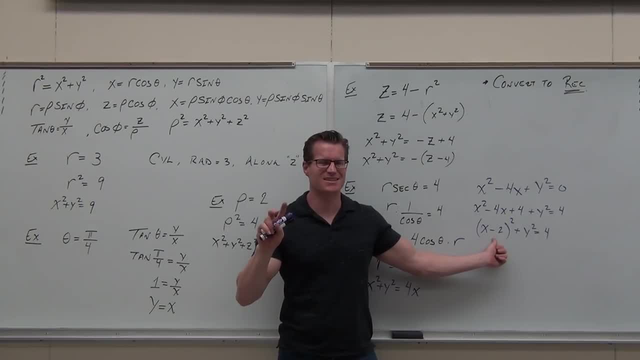 But it shifted, oh, come on, shifted along the x-axis positive 2.. So on the x-axis we're coming out 2, making a circle and then, right like that, It's a soda can. that's been shifted away from the center. 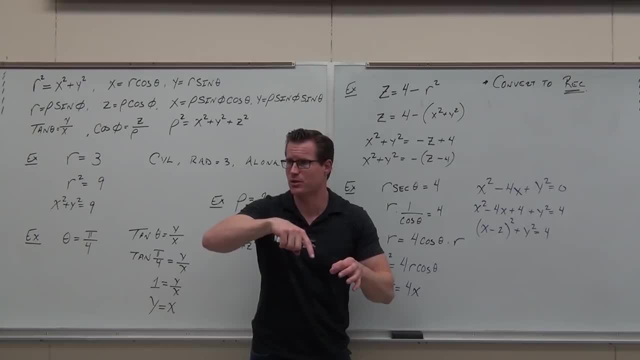 It's actually going to touch the origin because it would radius 2 and it shifted away 2.. It's going to touch the origin. It's going to be right along the z, But that's what that picture. Are you starting to see them in your head? 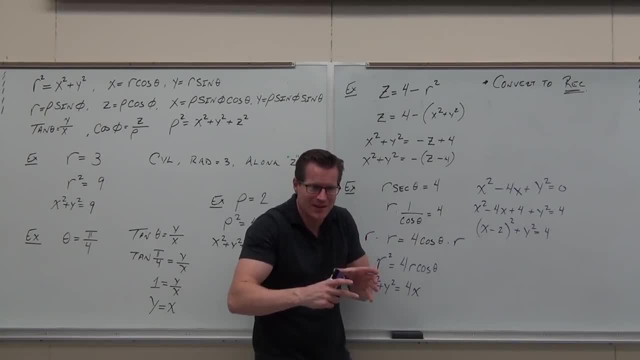 So on the x axis we're doing two and on the y axis we're doing 2.. coming out, two making a circle and then right like that, It's a soda can that's been shifted away from the center. It's actually going to touch the origin because it was radius two. 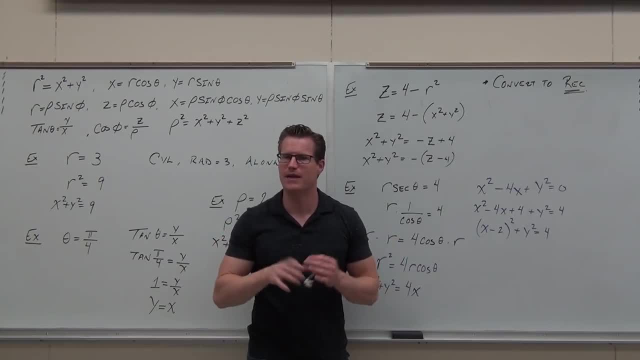 and it shifted away. two: It's going to be right along the Z, but that's what that picture is. Are you starting to see them in your head? I don't have time to draw, man. I don't have time for that. 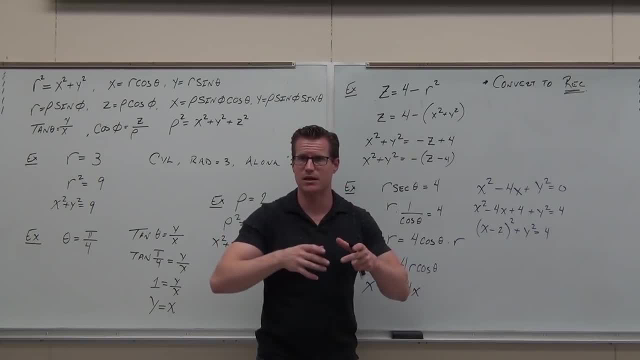 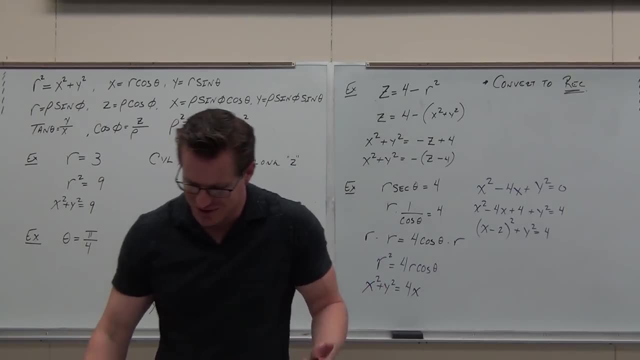 But I want you to at least see them to understand. That's a cylinder along the Z, It's got to be a circle with a radius of two and it's also shifted positive x-axis two spots. It's pretty cool when you can do stuff like that. 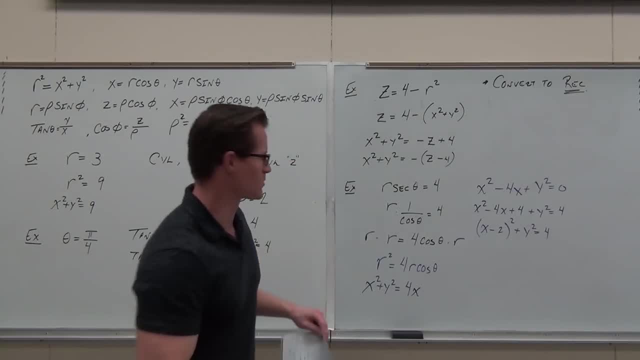 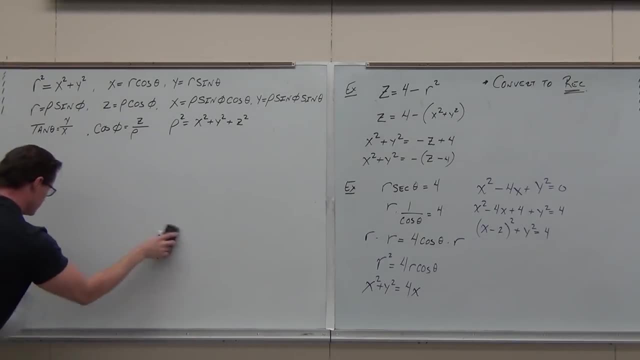 So let's try it as many as we can in the next about ten minutes. I'm going to be good For things like this. try the same exact technique that we used for this. So when you have rows and you want rows squared and you have co-incisions. 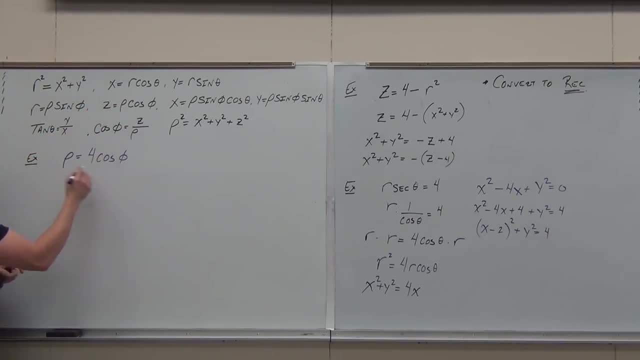 you want cosine phi's and you want row cosine phi's. Try doing things like multiply by row on both sides And then we get some nice stuff. I know row squared is x squared plus y squared plus z squared. I know that this is Z. 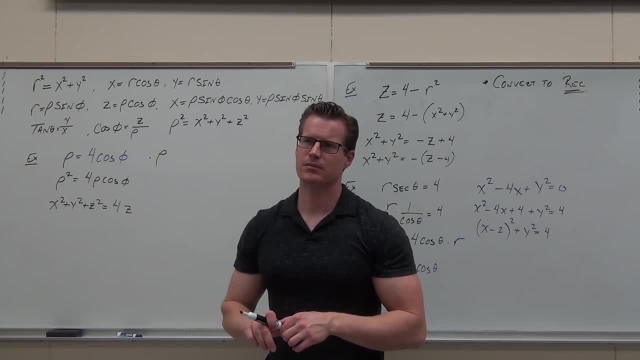 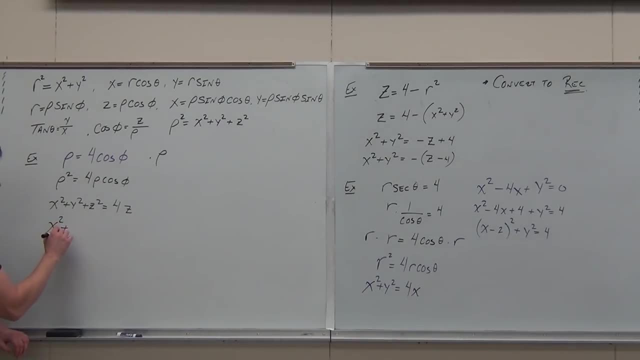 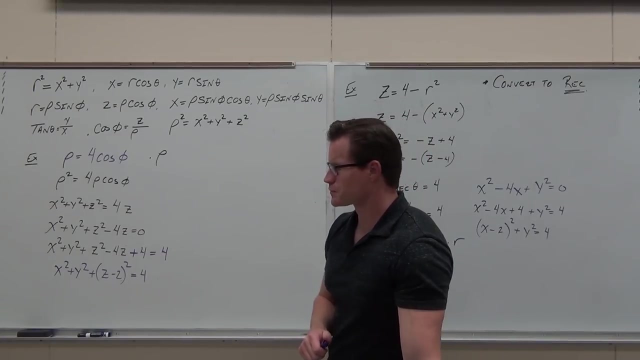 You guys? okay with that one. What, Which shape do you think that is? What shape do you think that is? Yeah, Yeah, How about now? What shape do you think that is now? What do you think it is? If anything, that's an ellipsoid. 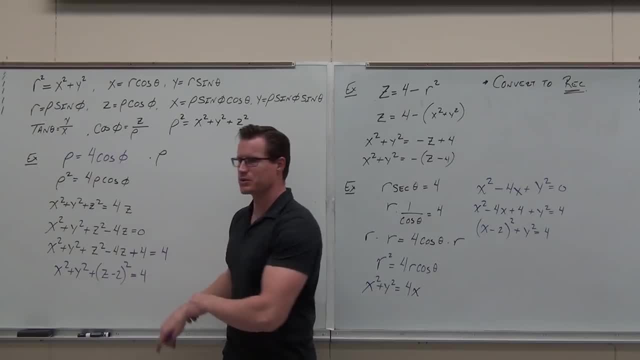 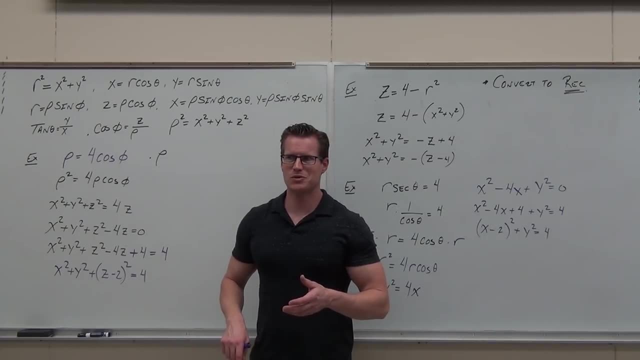 If anything, that's an ellipsoid, because, hey, all squares, all pluses, equal to a constant. Look at it. Look at it. Are all the denominators the same. What's an ellipsoid where all the spreading out stuff is the same? 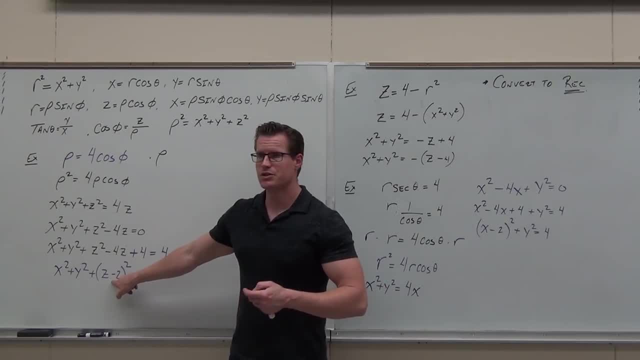 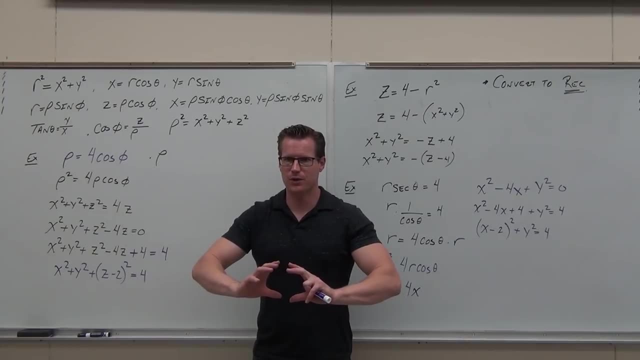 What's that called? That's a sphere. It's shifted up two spots on the z-axis. Are you guys starting to see it? This is a ball that is floating right on the xy plane. It's got a radius of 2.. 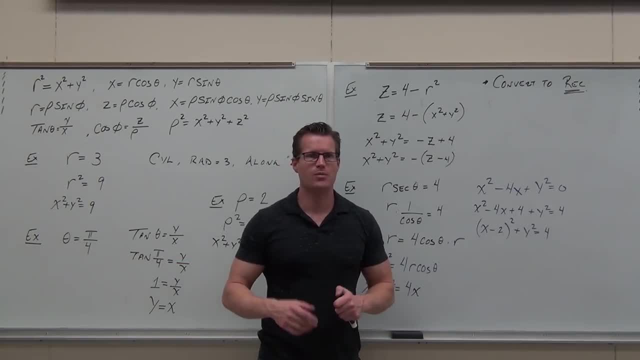 I don't have time to draw man, I don't have time for that. I don't have time for that. but I want you to at least see them to understand. it's a cylinder along the Z, It's got to be a circle with a radius of 2 and it's also shifted positive x-axis two spots. 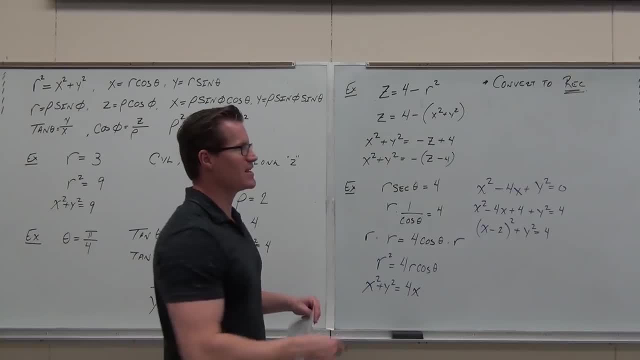 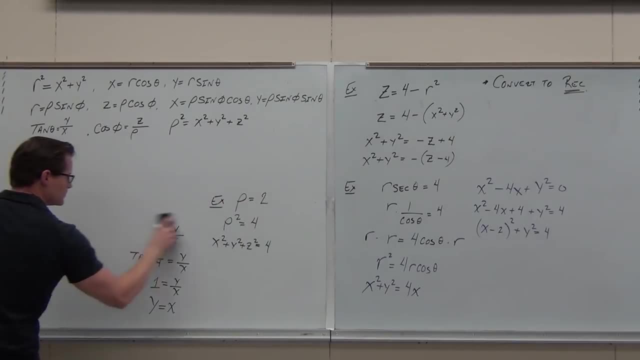 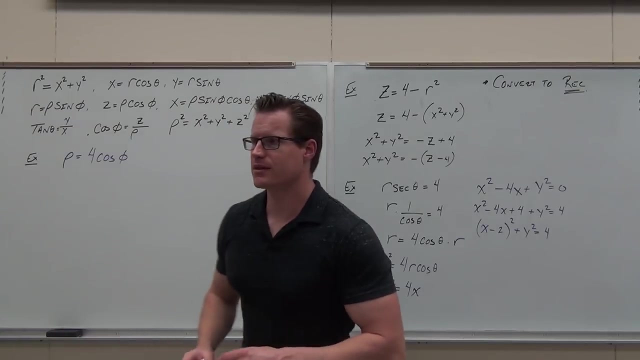 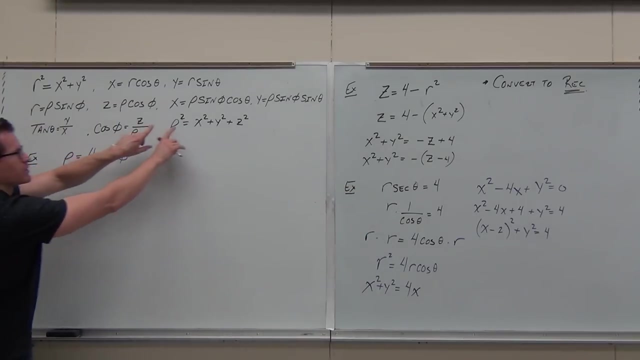 It's pretty cool when you can do stuff like that. Let's try it as many as we can in the next about 10 minutes. For things like this, try the same exact technique that we used for For this. so when you have rows and you want rows squared, you have cosine fees and you want row cosine fees. 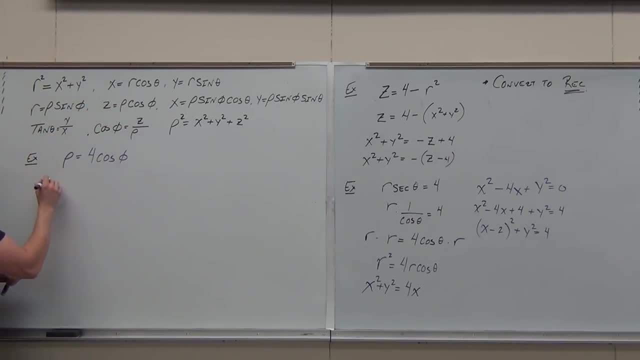 Try doing things like multiplied by row on both sides, And then we get some nice stuff. I know row squared is x squared and then I get x squared Plus y squared plus z squared. I know that this is Z. He is okay with that one. what shape do you think that is? 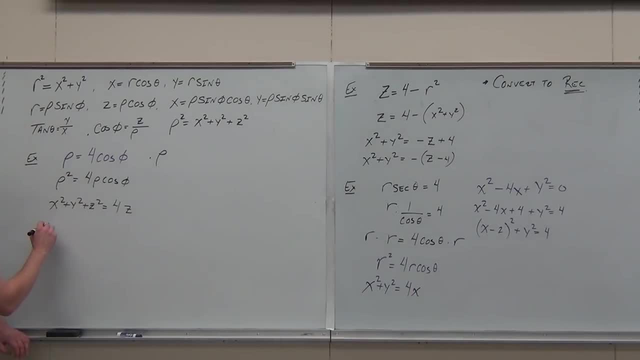 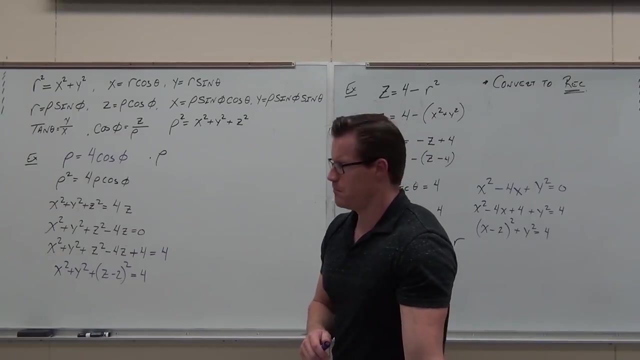 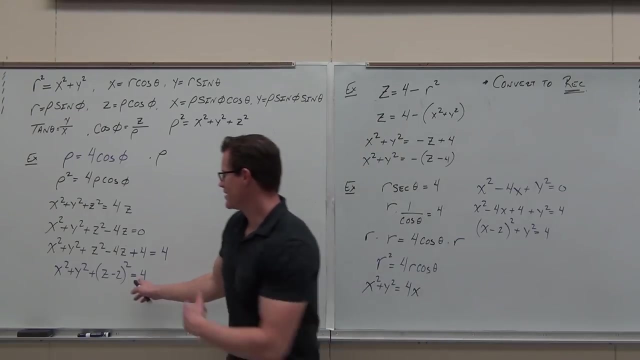 What shape do you think that is? Yeah, I Now. what shape do you think that is now? What do you think it is? If anything that's an ellipsoid, If anything that's an ellipsoid, because, hey, all squares, all plus is equal to a constant. 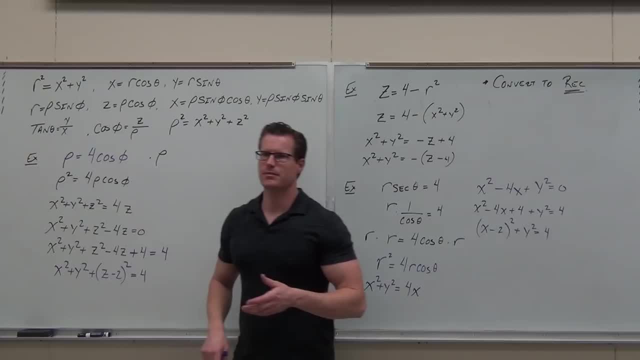 Look at it. Look at it. Are all the denominators the same? What's an ellipsoid where all the spreading out stuff is the same? What's it called? That's a sphere. It's shifted up two spots on the z-axis. 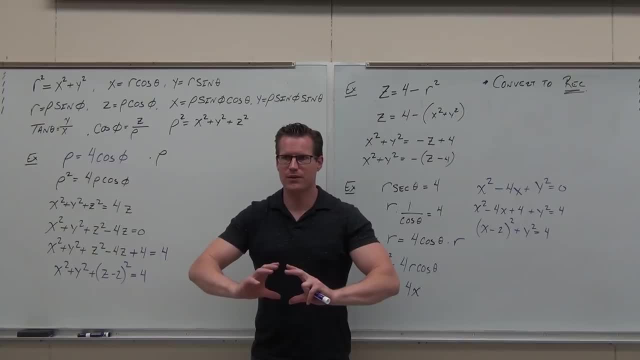 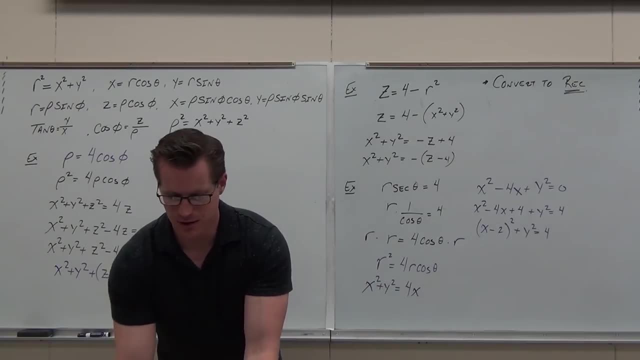 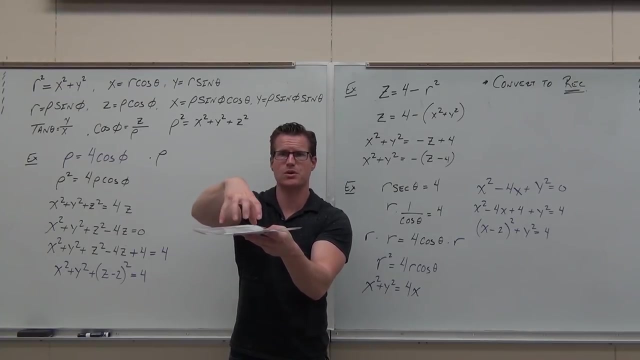 Are you guys starting to see it? This is a ball that is floating Right on the xy plane. It's got a radius of 2.. It's shifted up two spots. so Think plane xy, plane ball. It's sitting right on there because if the center shifted up two spots got a radius of 2.. That's what's happening. 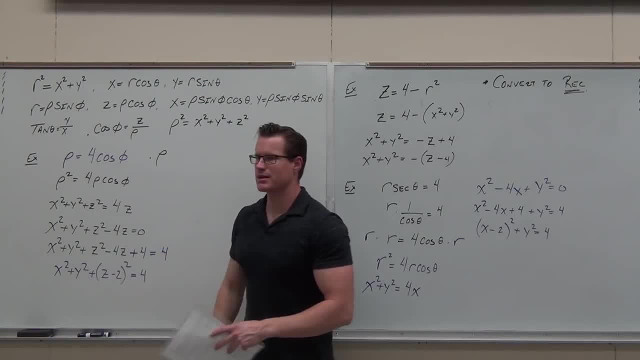 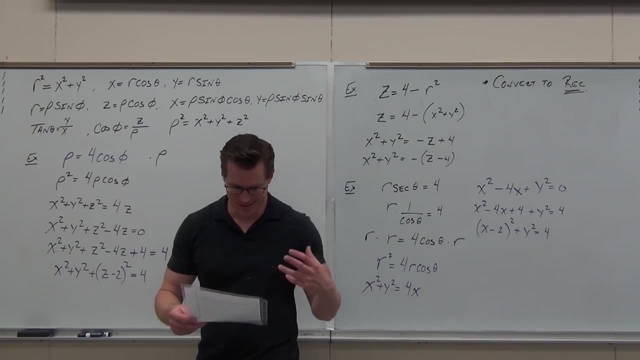 So if you look here with that, Which one's easier to identify, that it's not easier to work with, though That's easier to work with, but you can visualize that better. So that's, it's a, it's a trade-off. Yeah, we get like three more of this. 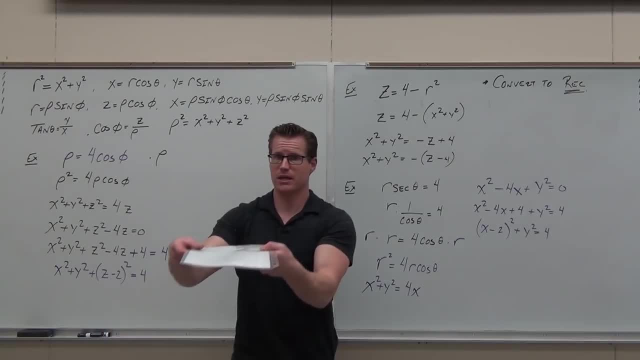 It's shifted up two spots. So think plane xy, plane ball, It's sitting right on there because the center shifted up two spots, It's got a radius of 2.. That's what's happening. So if you guys feel okay with that one, which one's easier to identify, 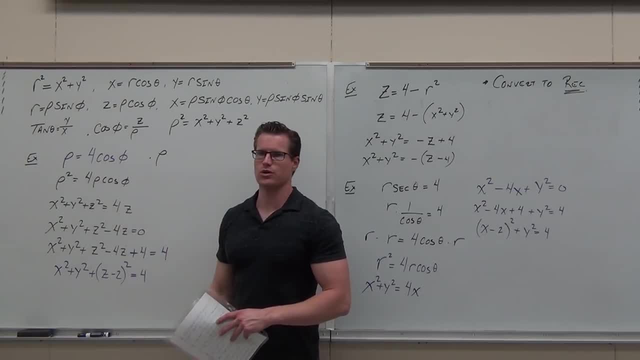 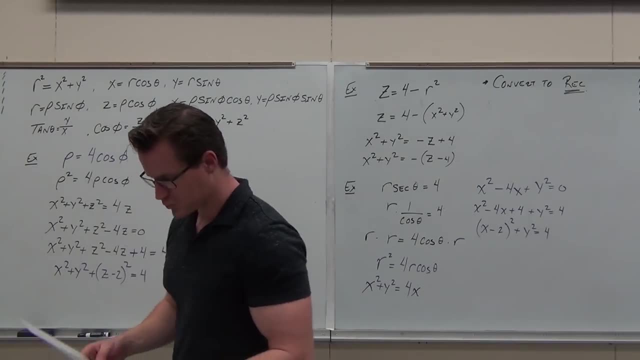 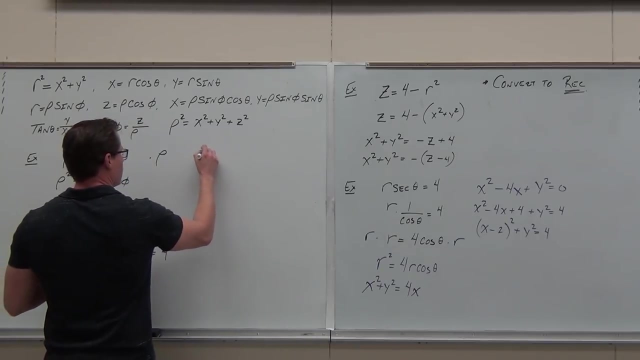 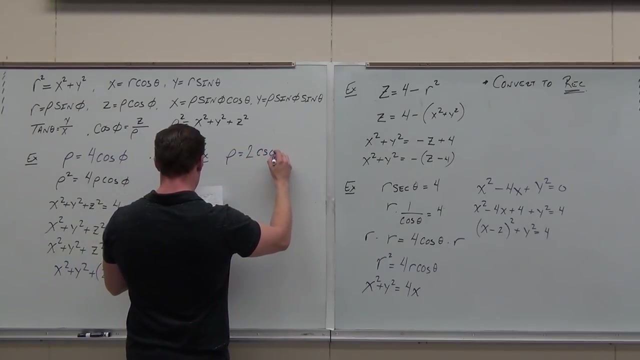 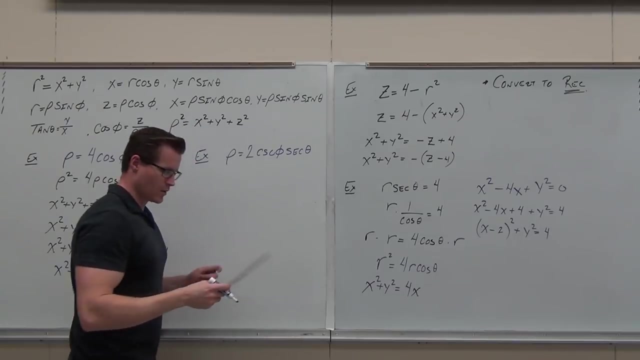 That It's not easier to work with, though That's easier to work with, But you can visualize that better. So it's a tradeoff. Yeah, We have like three more of this. You can do it. What is the first thing that you would do on that problem? 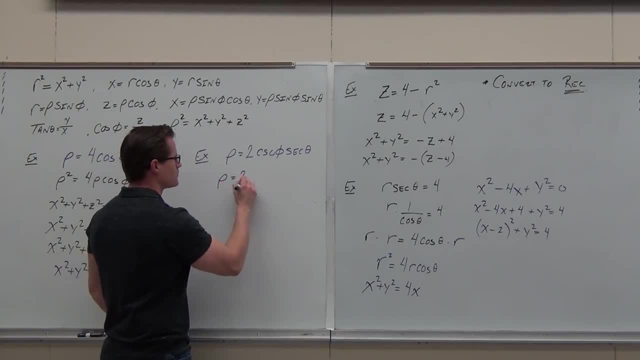 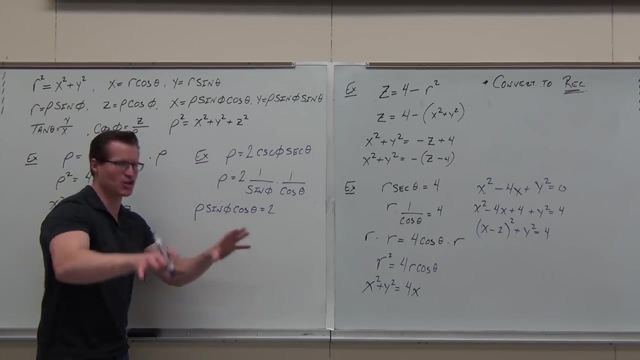 This is nasty man, Nasty. I'd clear those also. You're going to like this one. You're going to like this one. You're going to like this one. Tell me right now what is that? Or what's the whole thing. 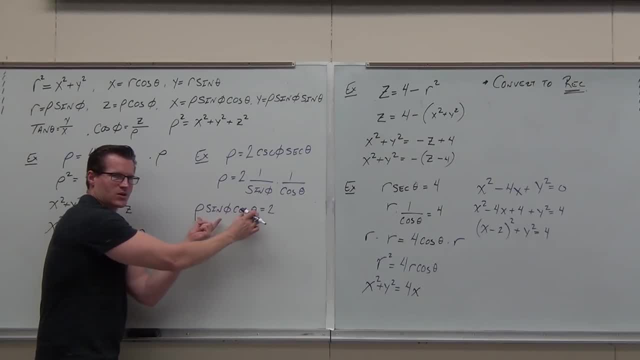 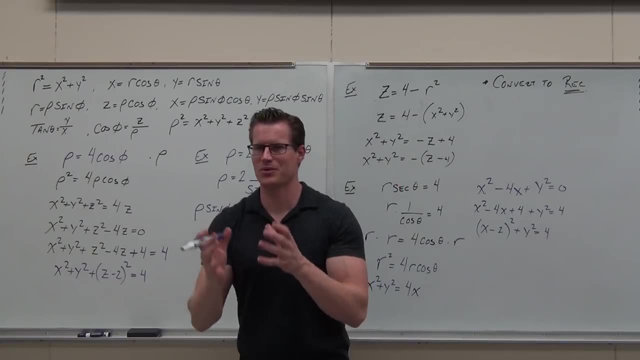 X. Do you see that? that's r? Yeah, And that's cosine r. cosine theta is X. What is x equals 2?? What is x equals 2 on a 3D coordinate system? What is it? It's a plane. 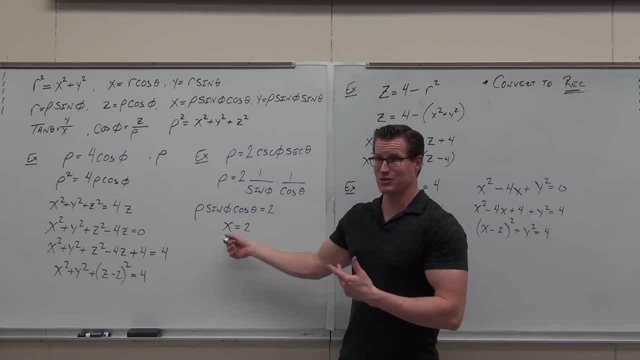 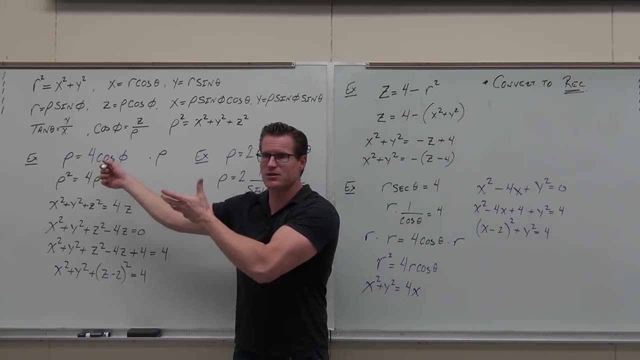 It's a plane. It's just a plane. Which one's easier? That's way easier, Because when we start talking about rectangular figures, rectangular's easier. Spherical figures, spherical's easier. That's why we have these different coordinate systems. 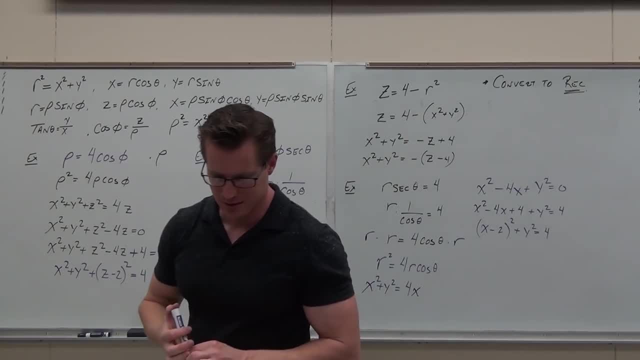 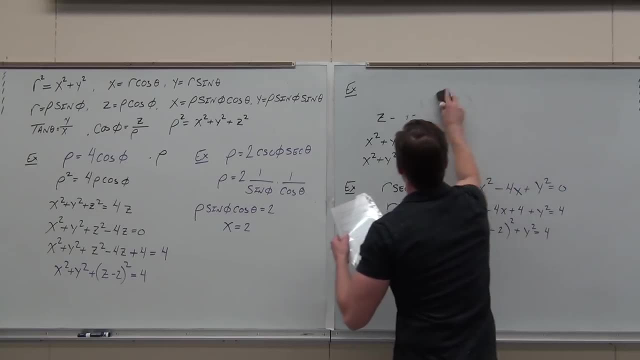 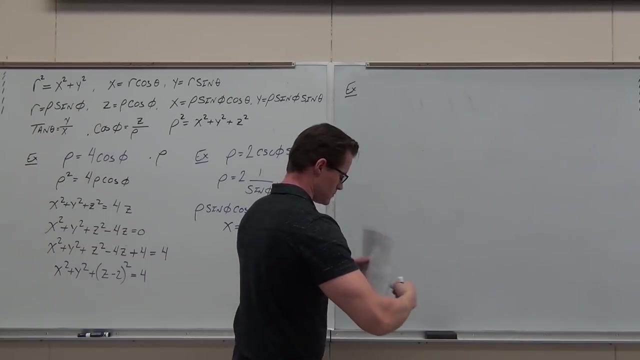 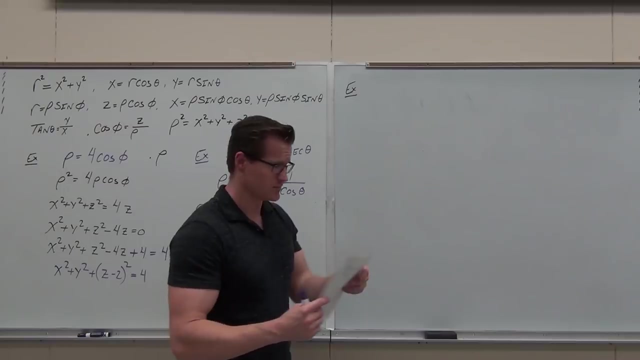 That's describing a plane at x equals 2 is what that is, Just a plane. That's it. You're welcome. Tell you what we're going to do. three more examples: I hope, I hope to. I want to. 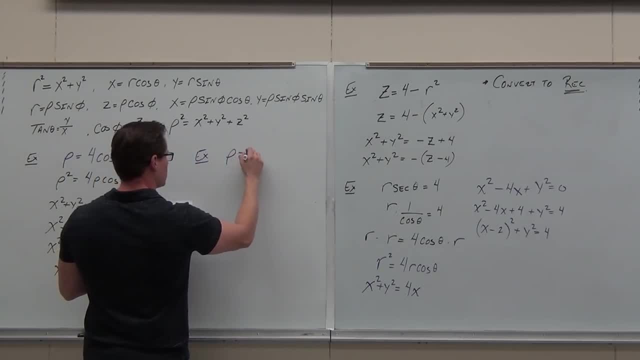 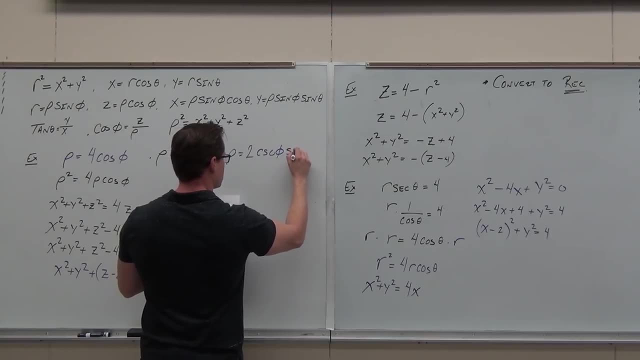 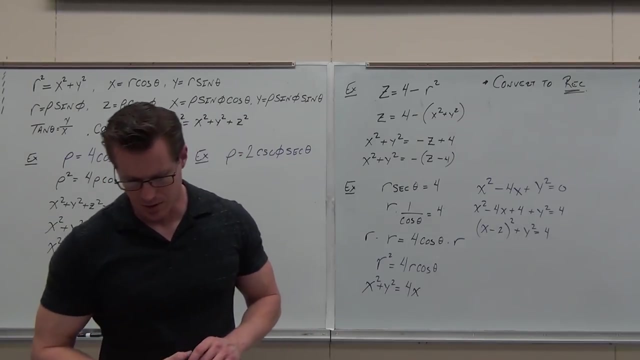 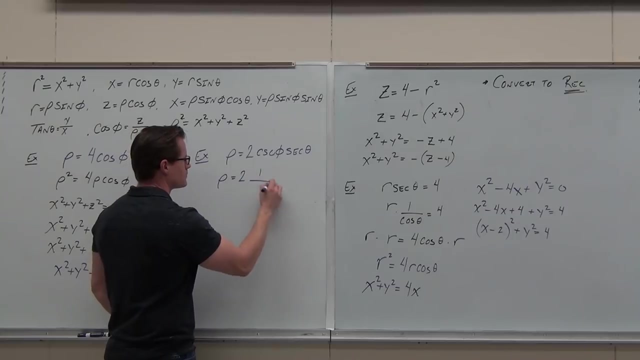 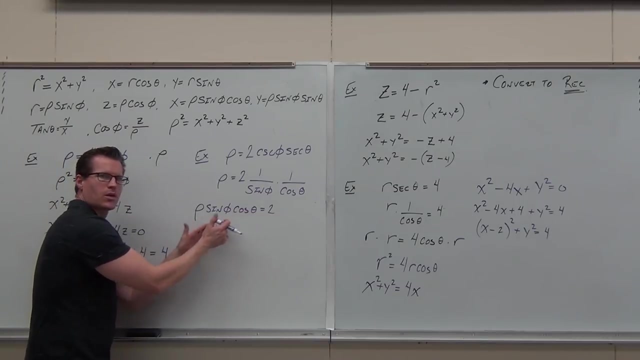 What is the first thing that you would do on that problem? this is nasty, nasty you. I Clear those also. You like this one, you're like this one, hey, you're like this one. tell me right now what is that? Or what's the whole thing? 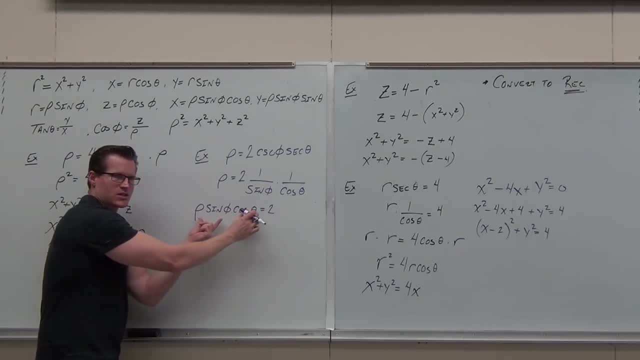 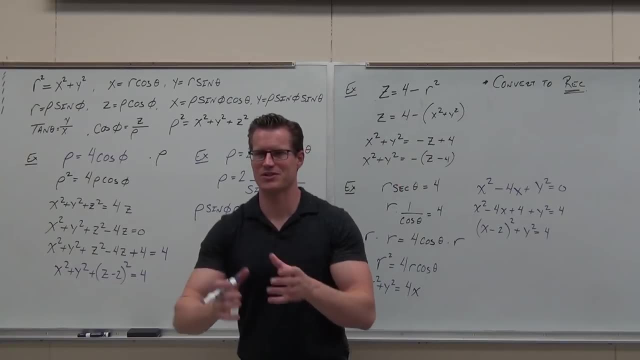 Do you see that? that's R and that's cosine R. cosine theta is: What is x equals 2? what is x equals 2 on a 3d coordinate system? What is it? It's a plane. it's floating higher x equals. It's just a plane which one's easier. 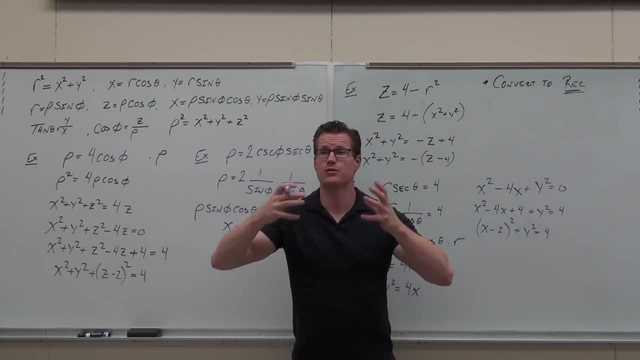 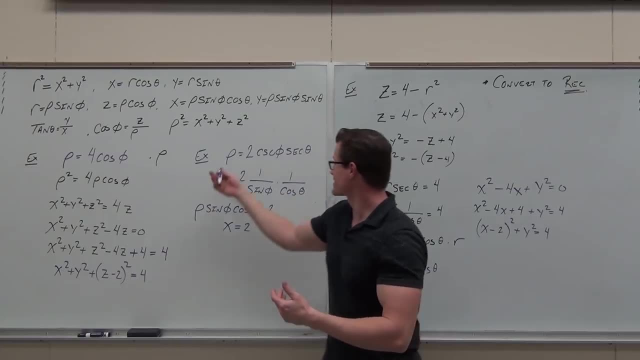 That's way easier because when we start talking about rectangular figures, rectangular is easier. spherical figures: Spherical is easier. That's why we have these different coordinate systems. That's describing a plane, and x equals 2 is what that is, Just a plane, That's it. 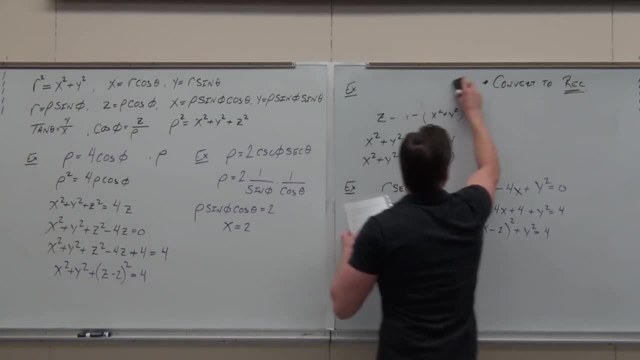 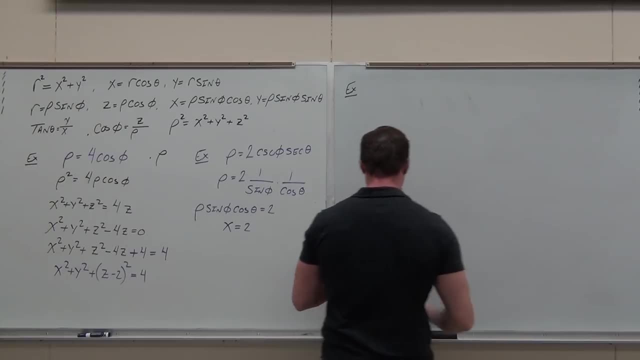 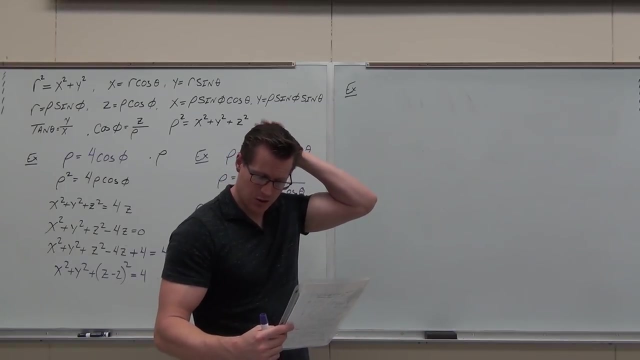 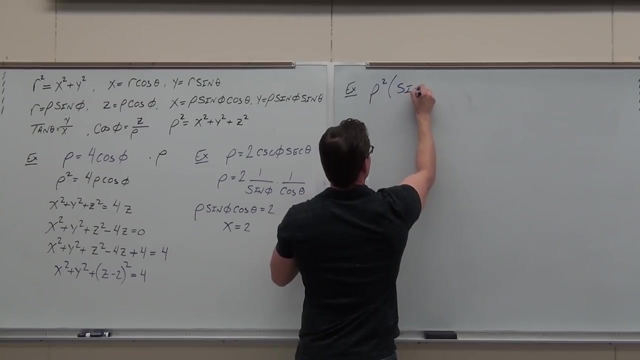 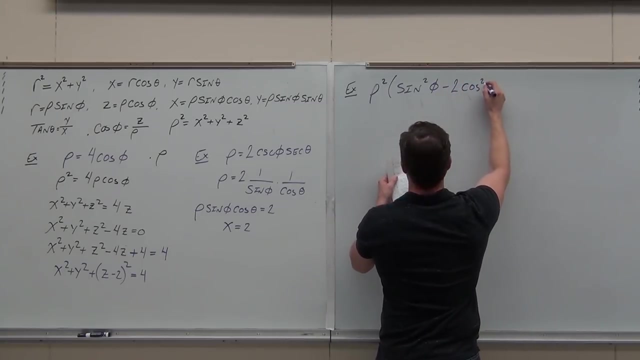 a Ahmed. I'll tell you what we're gonna do. three more examples: I hope, I hope to. I want to right, Are you gonna kill me, buddy? All run fast. Leonard. I used to be to be. I haven't ran in like eight years, so I'm imagining it's still true. That's what. 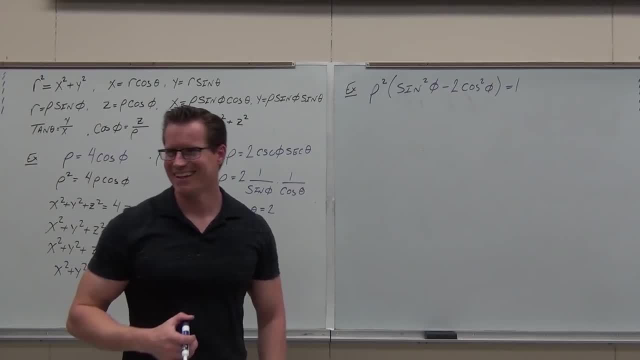 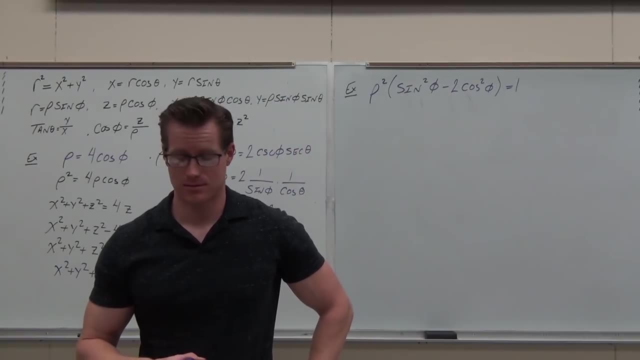 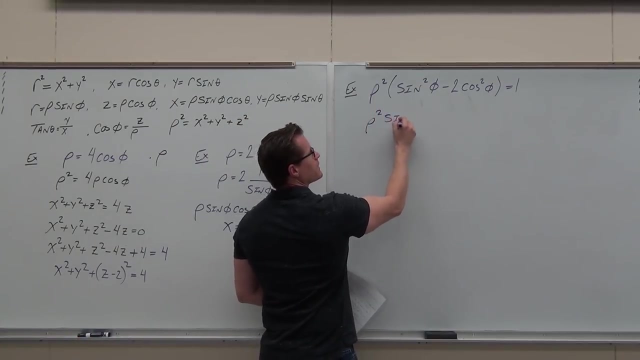 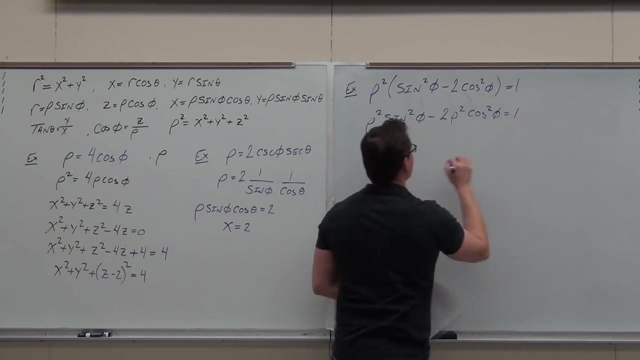 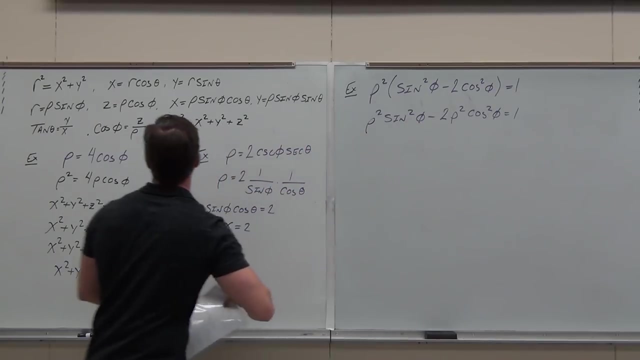 happens right. So what is that? Oh, it's obviously a one-sheet hyperboloid along the z-axis. Duh, How do you know? Because you do things like: hey, let's find some stuff that looks familiar here. This right here, if this: if rho sine phi is r, then this is. 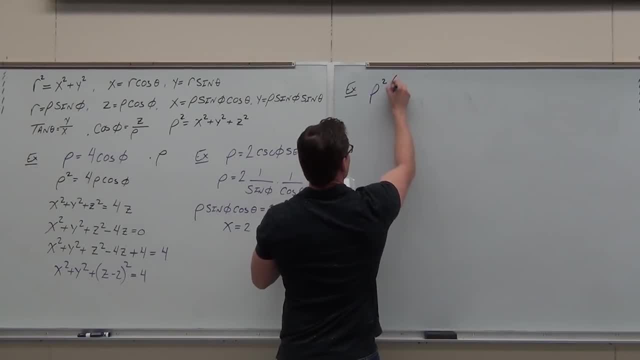 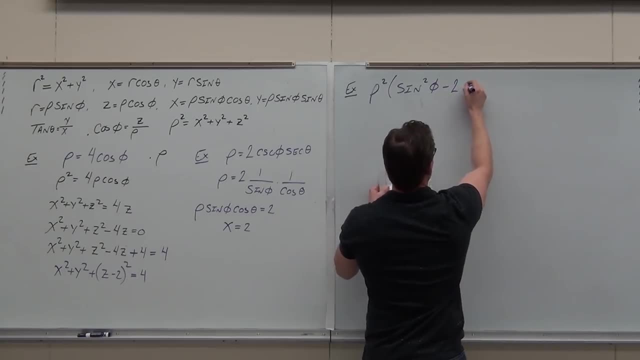 You want to try? Are you going to kill me if I do? No, Oh man, I'll run. I'm a fast runner. Well, I used to be. I haven't ran in like eight years, So I'm imagining it's still true. 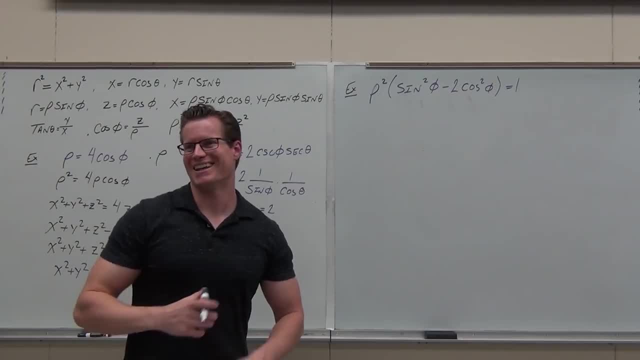 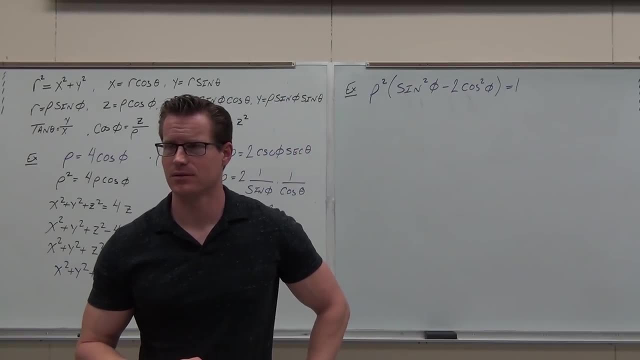 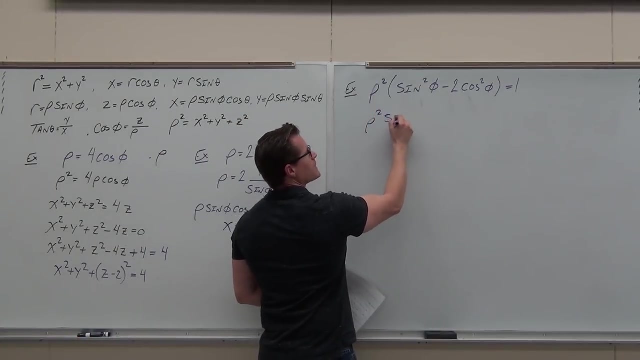 That's what happens, right? So what is that? Oh, It's obviously a one sheet. It's a one sheet hyperboloid along the z-axis. Duh, How do you know? Because you do things like: hey, let's find some stuff that looks familiar here. 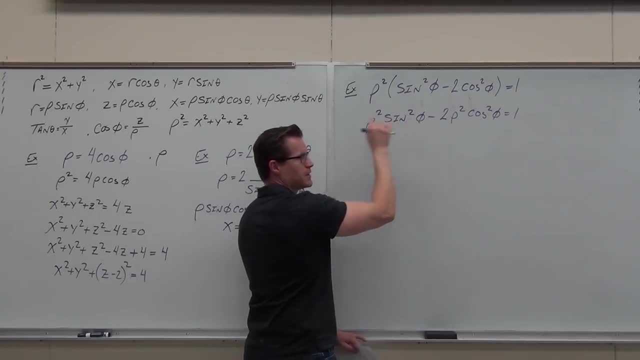 This right here. if this: if rho sine phi is- well, let's see r, then this is r squared. If rho cosine phi is r squared, then this is z, then this is z squared. You guys catching the picture here. 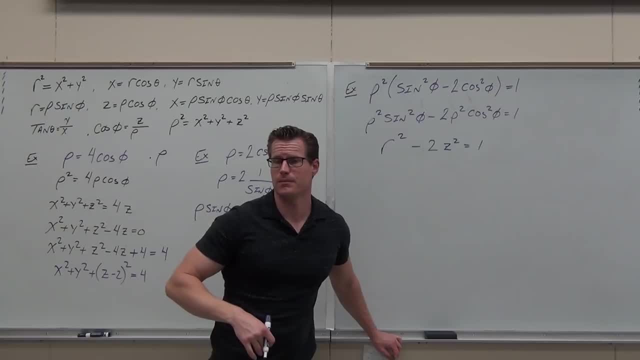 Use that stuff. But wait, I want rectangular. What's r squared, Quickly? how many variables All squared? One negative with a constant. what is it? One sheet hyperboloid along the z. Well, do I know what it looks like? 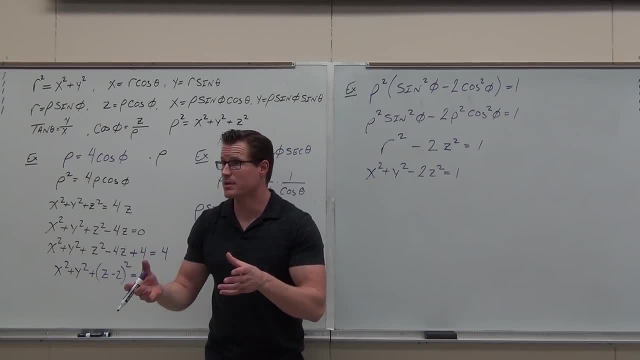 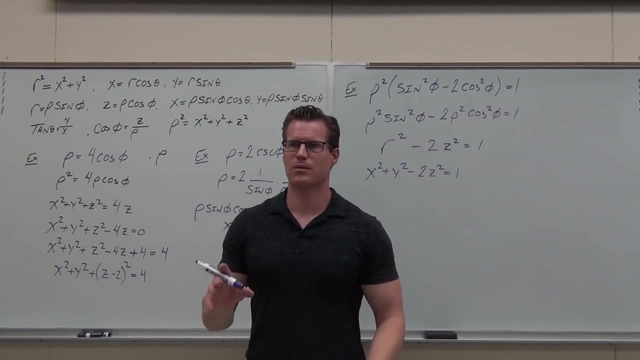 No, I'd have to do a little more work. I don't know more than that, but at least I know what the shape is. It's this hourglass along the z. That's what I meant. Are you picking up when I'm laying down? 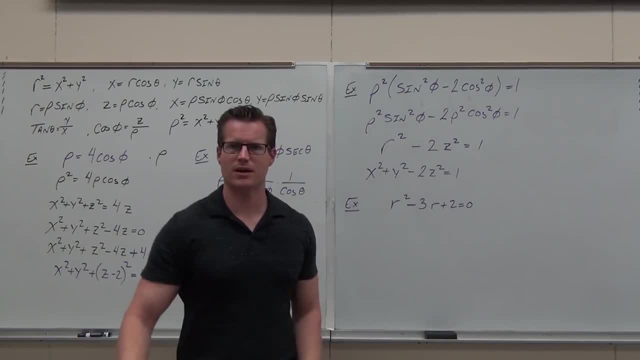 Told you they're quick, Don't worry. Don't worry, Just stay, hang with me, We're going to have some fun. man, I got more candy and everything. all right, These are weird ones. They're kind of cool though. 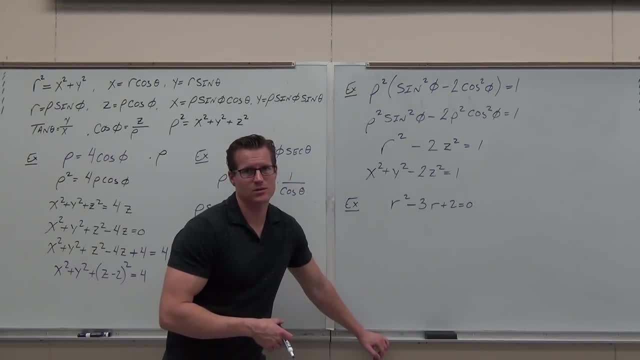 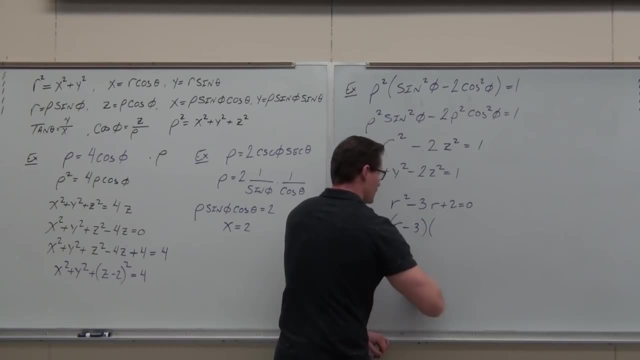 They're kind of cool When you get some weird stuff. they're like: wait all r's, but it's factorable. If you can factor it correctly, Do you follow the factorization, Basic, basic algebra, but in this context it's pretty freaking cool. 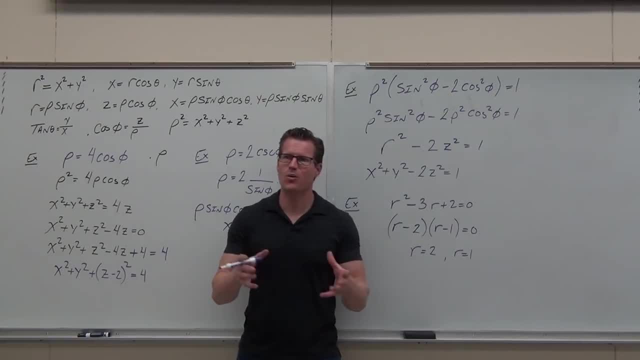 Now we just covered one a little while ago. What is r equal 1? Cylinder, It's a cylinder. What's r equals 2?? So this describes two cylinders. one of them, and along what axis? The z axis cylinder with a radius of 1, centered at the origin, going along the z. 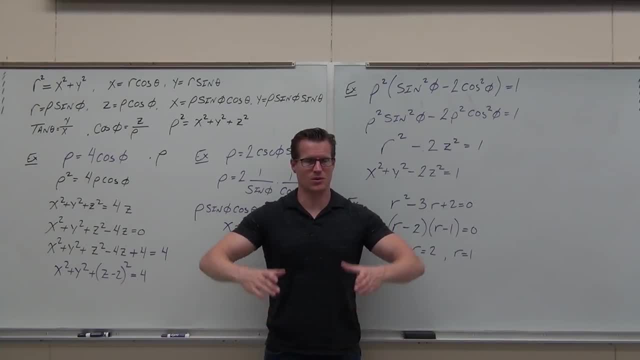 and then another one cylinder, radius 2.. It's like a toilet paper roll, all right, where you get the inside and outside. That's what it looks like. It's not filled in, but it's those two cylinders, that's one inside the other. 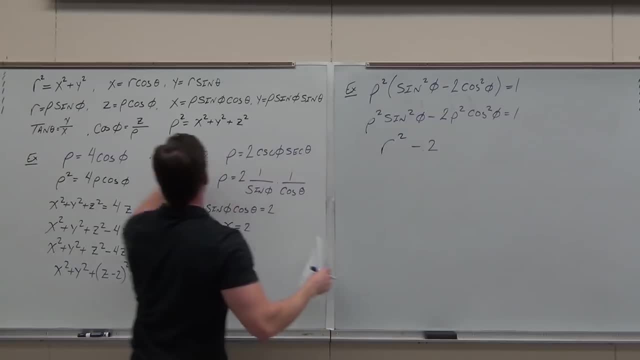 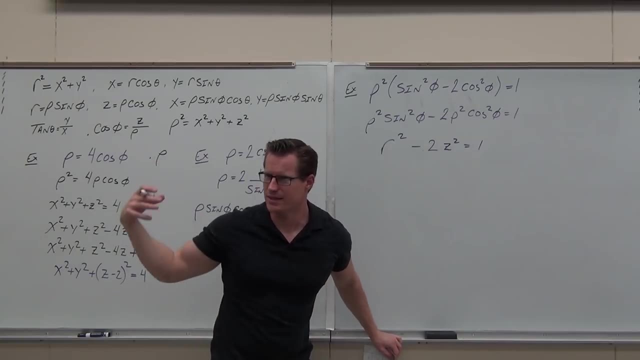 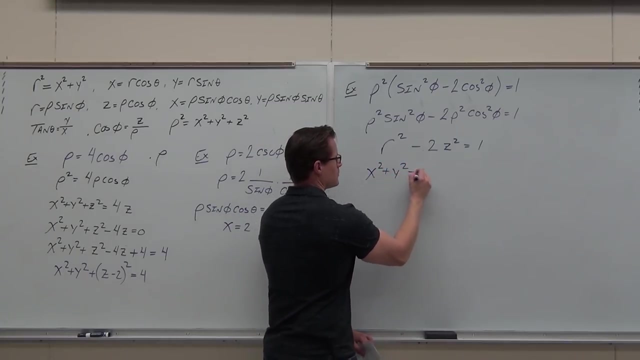 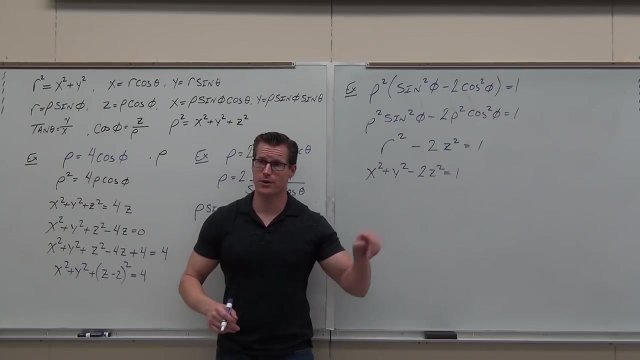 r squared. If rho cosine phi is z, then this is z squared. You guys catching the picture here, Use that stuff. But wait, I want rectangular. What's r squared? Quickly? how many variables All squared, One negative with a constant? what is it? 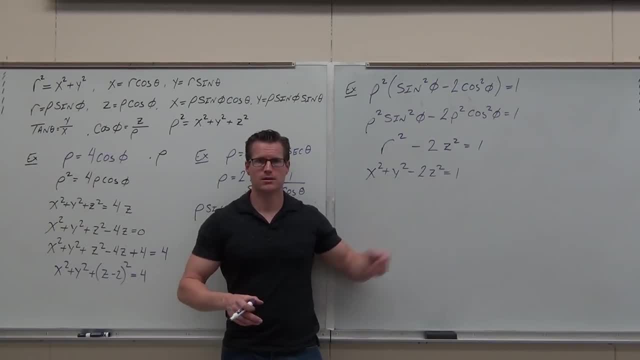 One sheet hyperboloid along the z. Do I know what it looks like? No, I'd have to do a little more work than that, but at least I know what the shape is. It's this hourglass along the z. That's what I know. Are you picking up when I'm laying down? 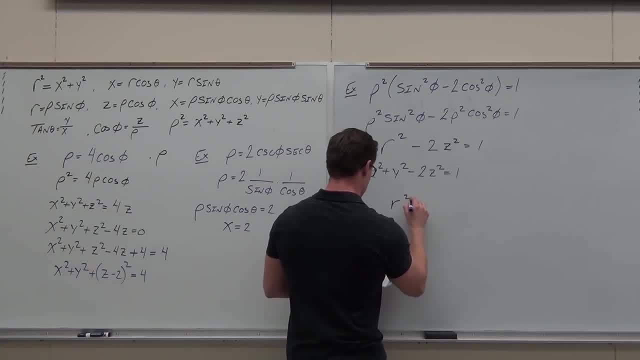 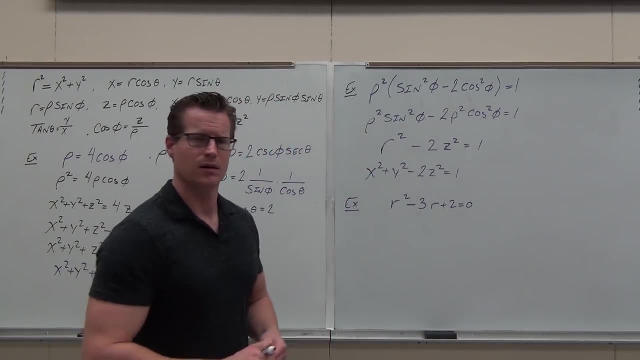 I told you they're quick, Don't worry. don't worry, Just stay and hang with me. We're going to have some fun. I got more candy and everything. all right, These are weird ones. They're kind of cool, though. They're kind of cool When you get. 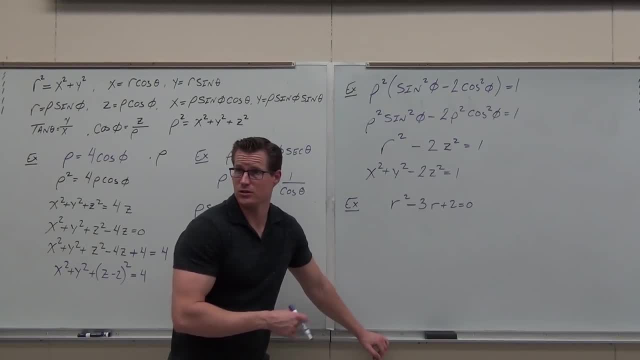 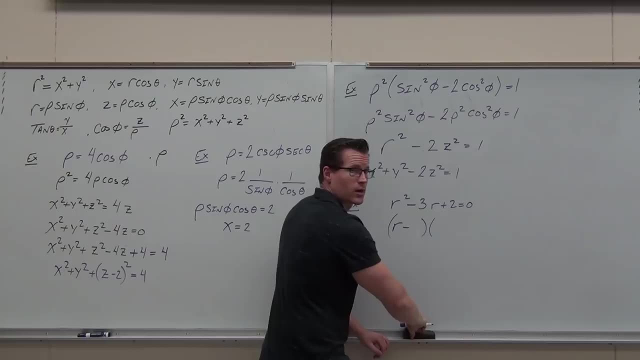 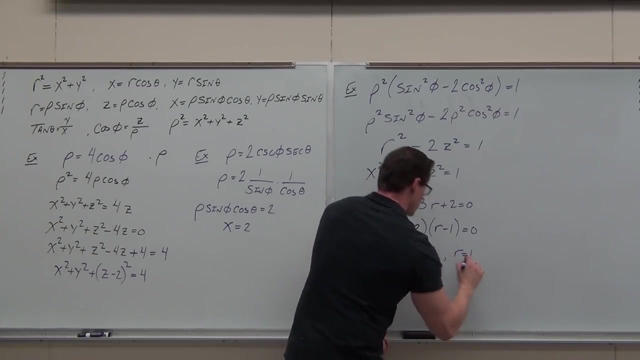 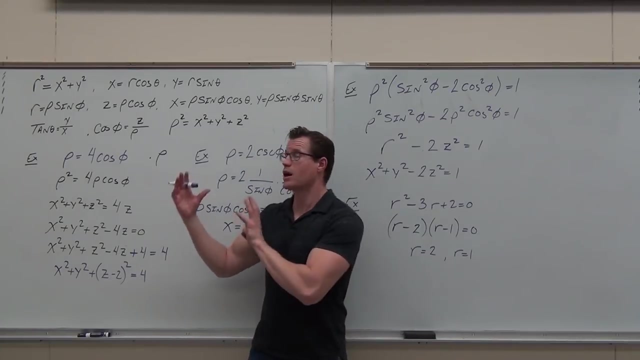 some weird stuff. they're like: wait all r's, but it's factorable, You can factor it in. Do you follow the factorization? Basic, basic algebra, but in this context it's pretty freaking cool. Now we just covered one a little while ago. What is r equal 1?? 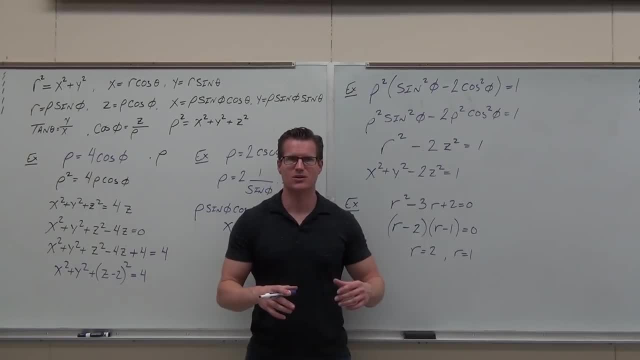 Cylinder. It's a cylinder. What's r equals 2? Cylinder. This describes two cylinders. one of them- along what axis? The z axis Cylinder with a radius of 1, centered at the origin, going along the z, and then another one cylinder radius 2.. It's like a toilet paper roll all. 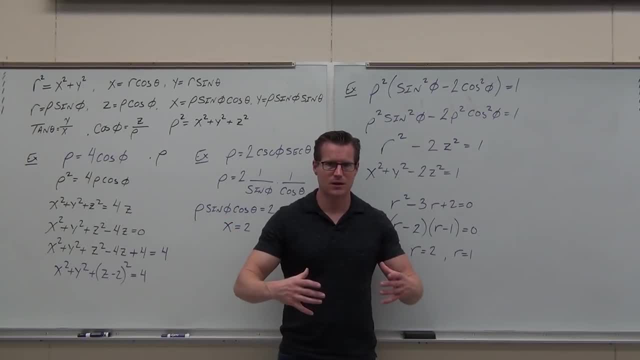 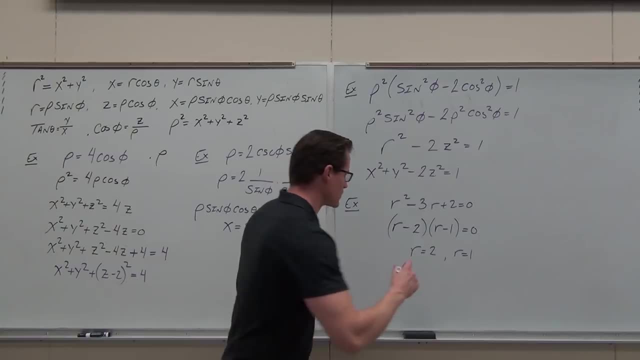 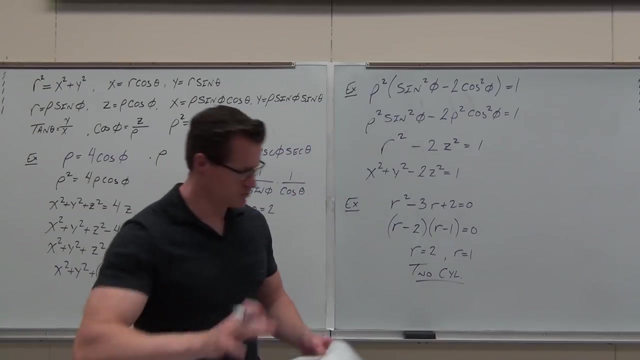 right where you get inside and outside. That's what it looks like. It's not filled in, but it's those two cylinders That's one inside the other. Isn't that kind of cool? That's what that describes: two cylinders, Just for fun. Just for fun. 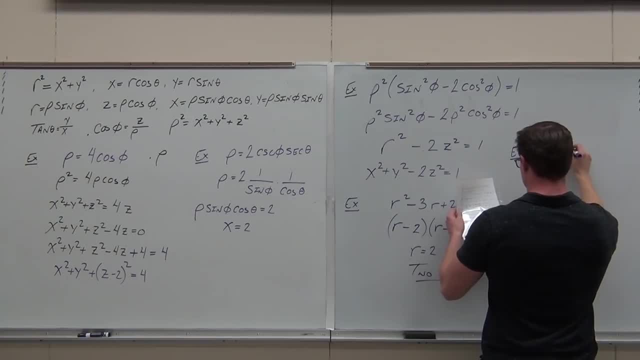 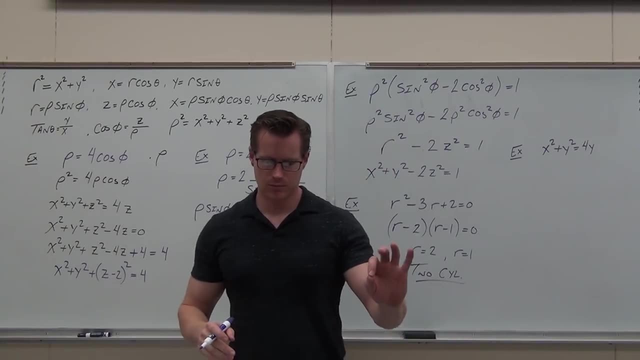 Can you give that to me in cylindrical and then spherical? If you have to do both, do cylindrical first. I'm begging you because it's like a halfway step. Do cylindrical first. As long as you have r's and z's and thetas, you're done. That's what cylindrical is, and 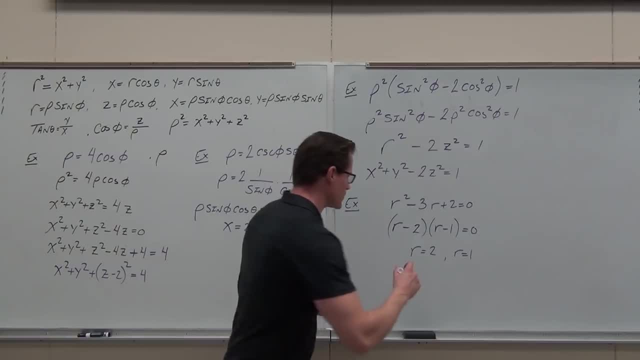 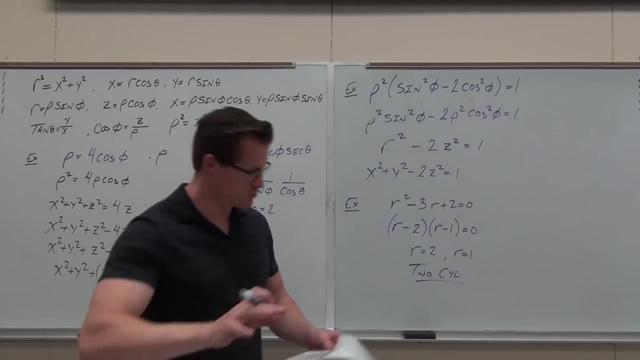 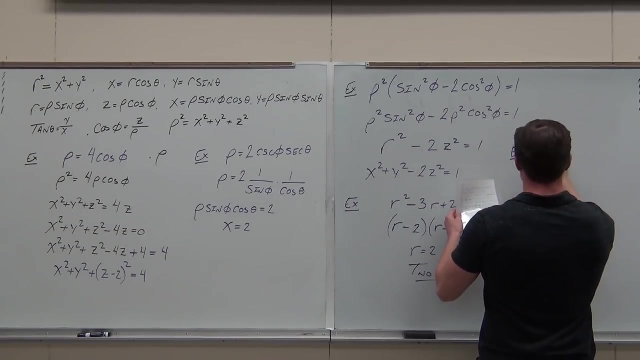 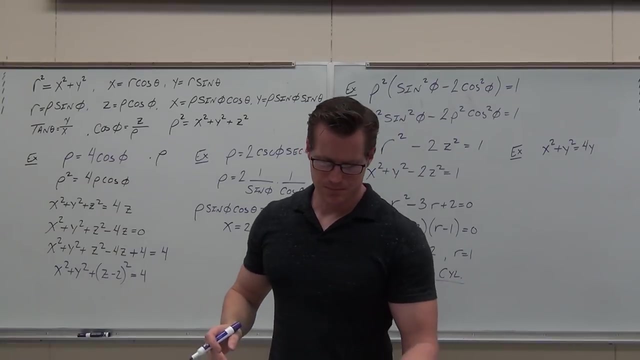 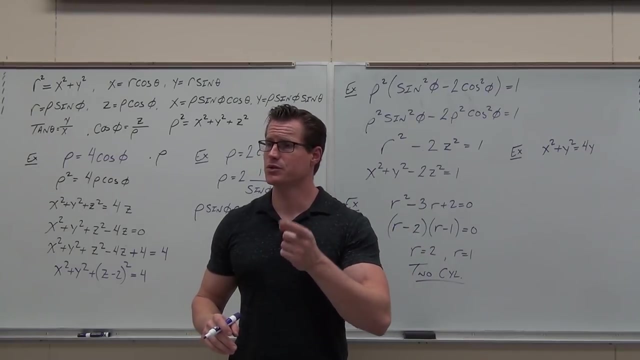 Isn't that kind of cool. That's what that describes: two cylinders Just for fun, just for fun, just for fun. Can you give that to me in cylindrical and then spherical? If you have to do both, do cylindrical first. I'm begging you. 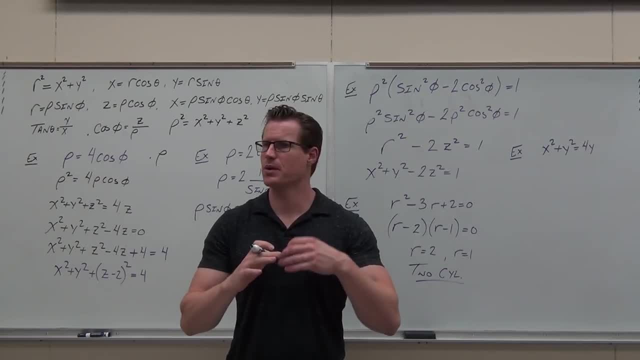 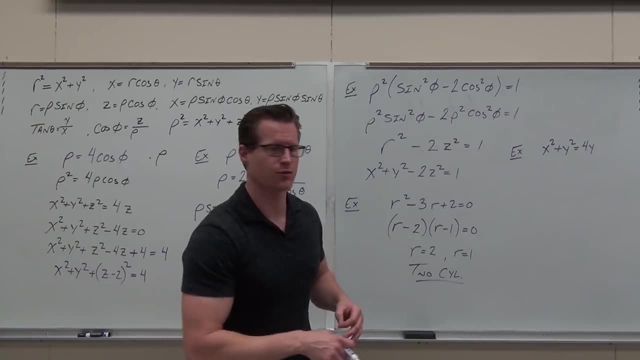 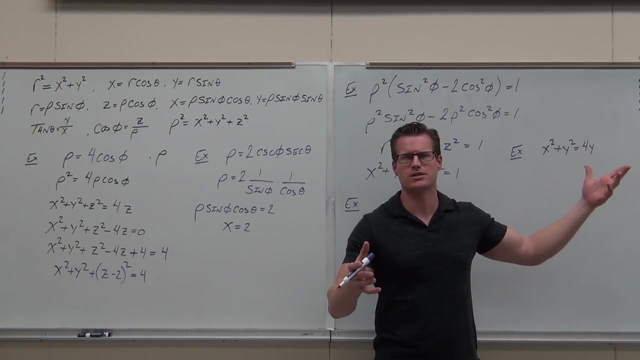 because it's like a halfway step. Do cylindrical first, As long as you have r's and z's and theta's, you're done. That's what cylindrical is- And then go to spherical. So for instance, for, for, so this is oh, by the way. what would you categorize as that? 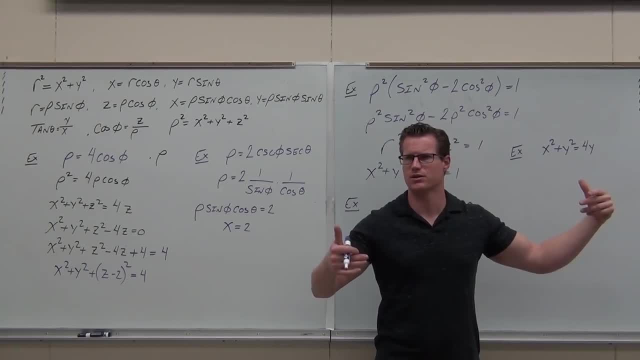 Rectangular, cylindrical or spherical? It's obviously rectangular because it's only x's and y's. Do you know how much x squared plus y squared is R squared? Use that, Goodness gracious, If it's a minus. you got a little bit more work. 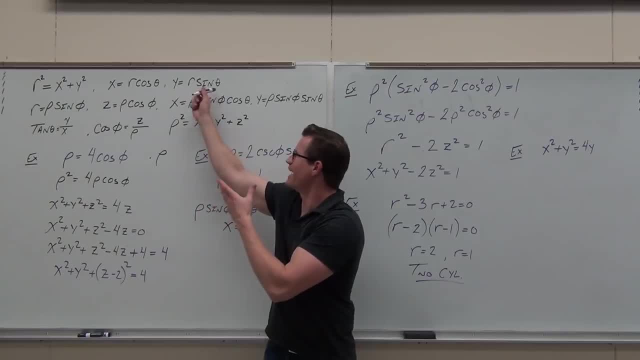 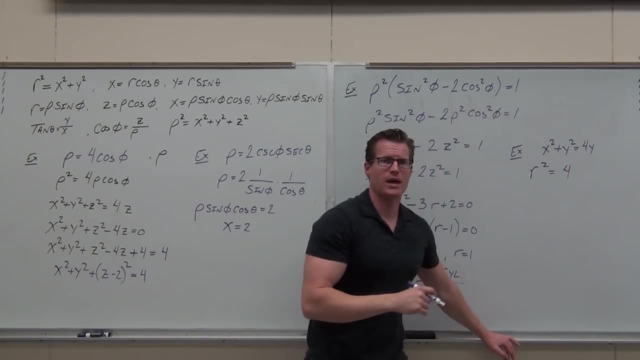 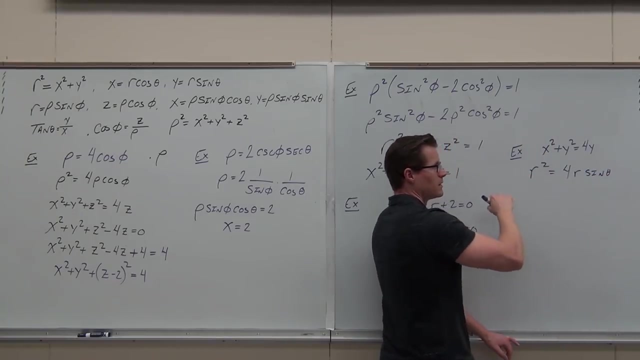 Work to do, because then you got to do the whole this and that Does that make sense. You got to do that stuff. But if you got something nice and then y, y is r's Right there, Use the same stuff you used right here. 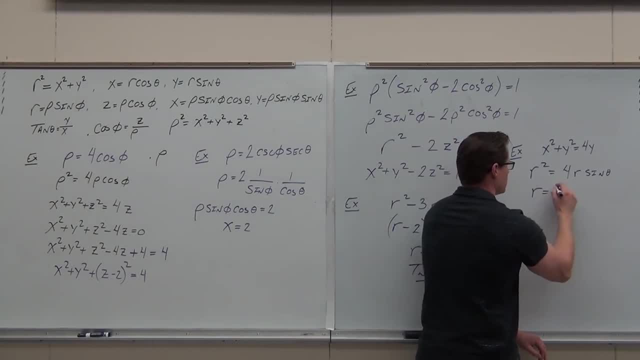 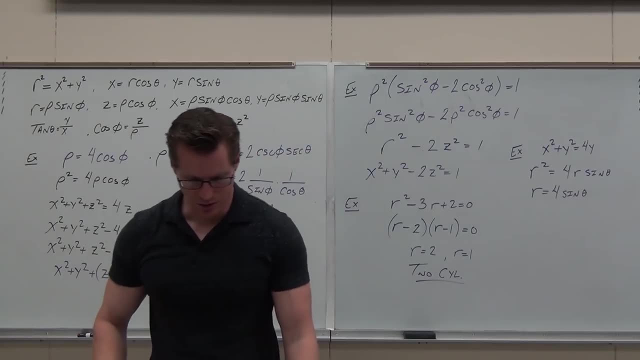 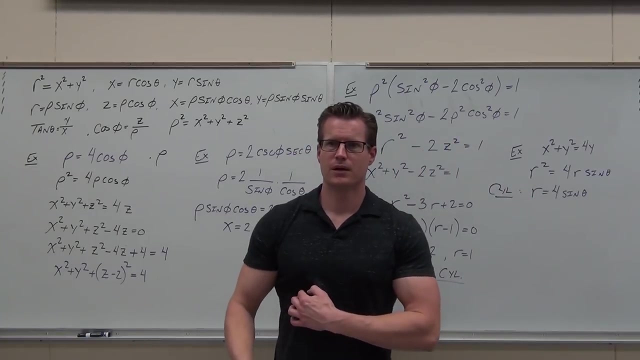 Start dividing by r's. That's okay. Okay, That right. there is a cylindrical equation. It has only r's and theta's in it, So this would be cylindrical. Is that okay with you? Now, spherical doesn't have r's, but it can have theta's. 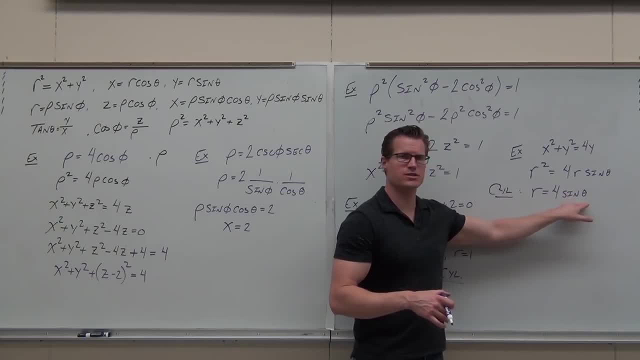 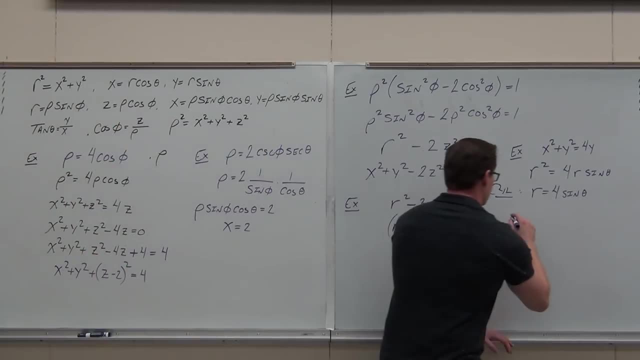 So it's just a little translation more. This is like a halfway step. Do I need to change the sine theta? No, don't worry about it. Do I need to change the r? Yeah, Oh, that one Done. That's spherical. 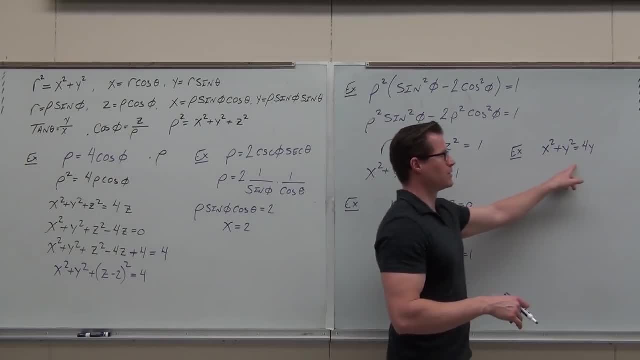 then go to spherical, So for instance, 4.5. 4.5. 4.5. No, this is just. This is for. Oh, by the way, what would you categorize as that? Rectangular, cylindrical or spherical? 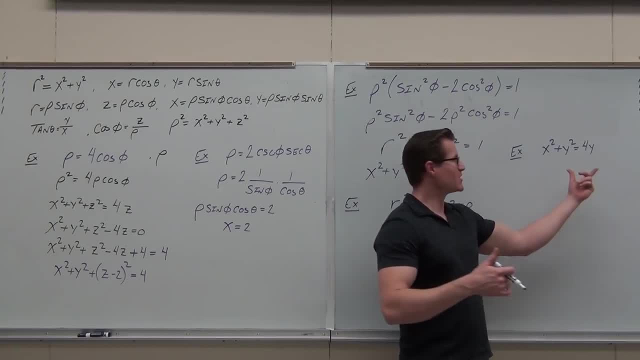 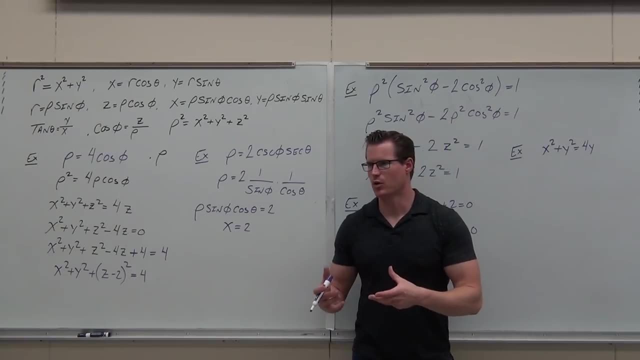 Rectangular. It's obviously rectangular because there's only x's and y's. Do you know how much x squared plus y squared is h square squared? h square squared. Use that, Goodness gracious, If it's a minus, you've got a little bit more work to do, because 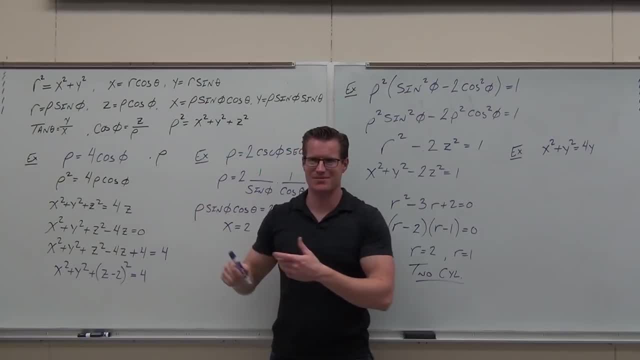 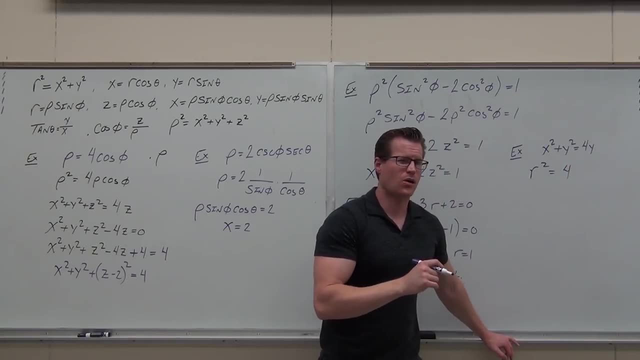 then you've got to do the whole this and that. Does that make sense? You've got to do that stuff. But if you've got something nice, and then y, Y is R Right there, use the same stuff you used right here. 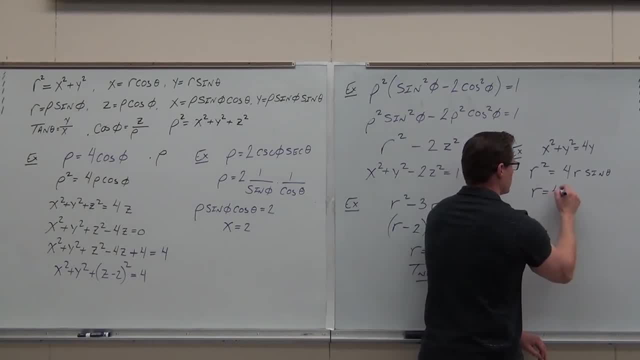 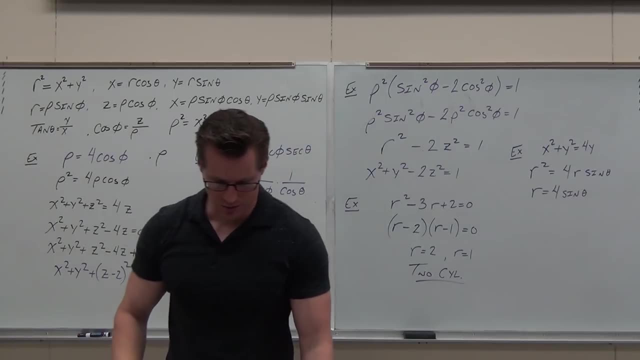 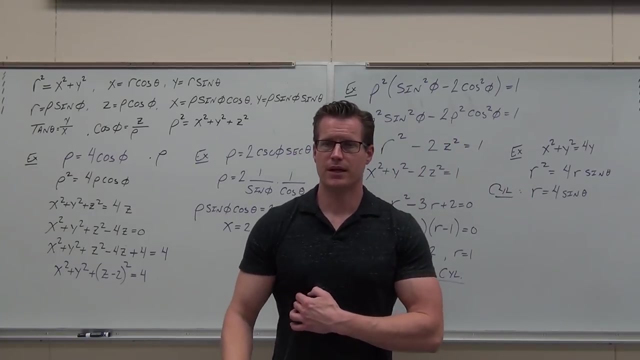 Start dividing by R's. that's okay, That right. there is a cylindrical equation. It has only R's and theta's in it, So this would be cylindrical. Is that okay with you? Now, spherical doesn't have R's, but it can have theta's. 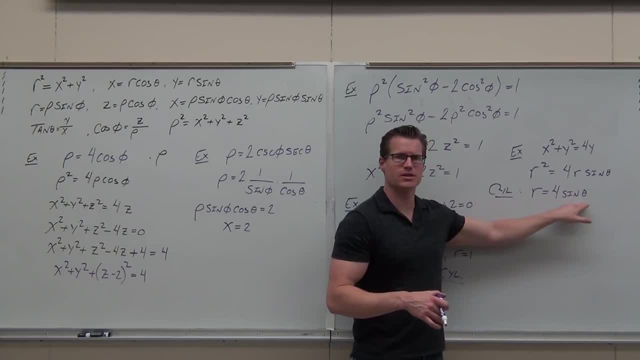 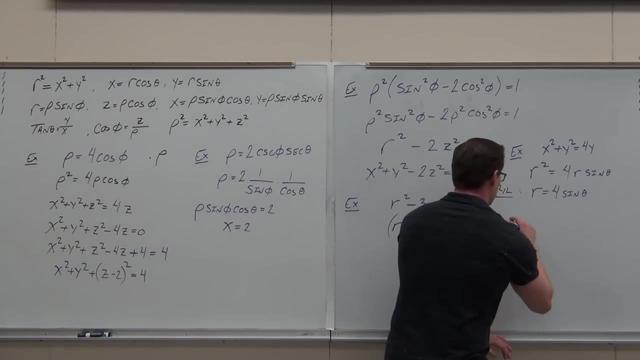 So it's just a little translation more. This is like a halfway step. Do I need to change the sine theta? Nah, don't worry about it. Do I need to change the R? Yeah, Oh, that one Done, That's. that's spherical. 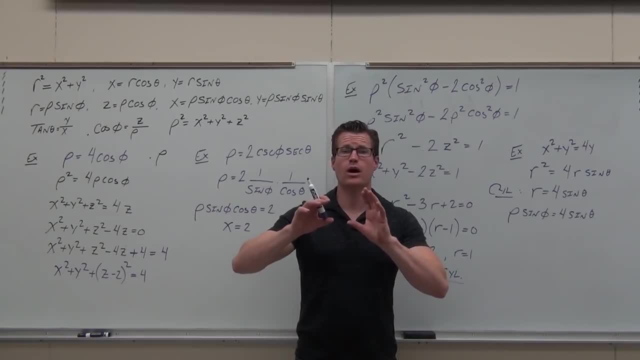 Get rid of what you did. That's what you don't want. If I'm trying to get cylindrical, I don't want X's and Y's, I want R's and theta's and Z's. If I'm getting to spherical, I don't want R's and I don't want Z's. 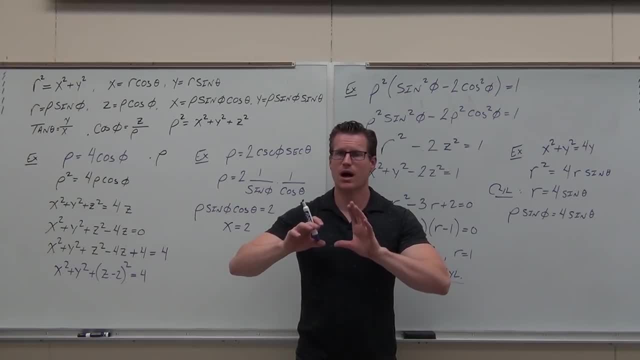 Get rid of what you don't want. If I'm trying to get cylindrical, I don't want x's and y's, I want r's and theta's and z's. If I'm getting to spherical, I don't want r's and I don't want z's. 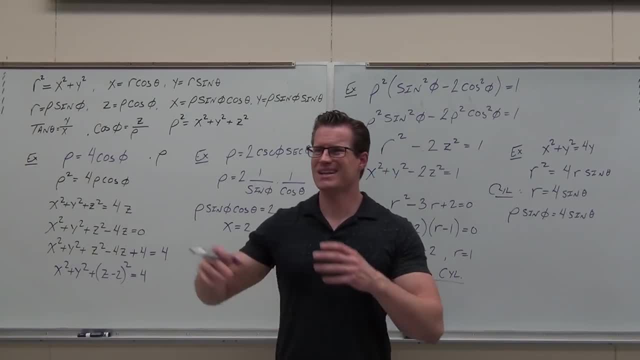 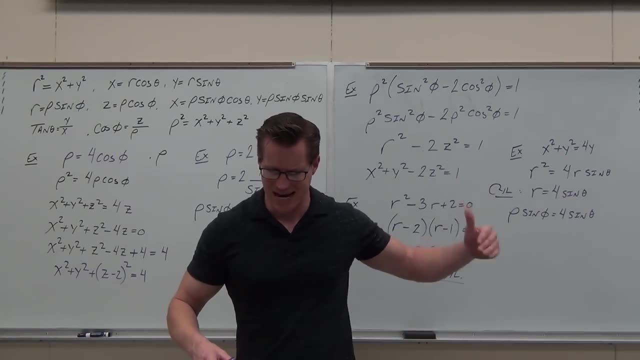 So we've got to translate those pieces that we don't want out of the equation. Is this clear enough? I want to make sure that we do. Is it good enough that you understand it? I have one more. I really don't want to go over it because it's almost exactly the same thing that we 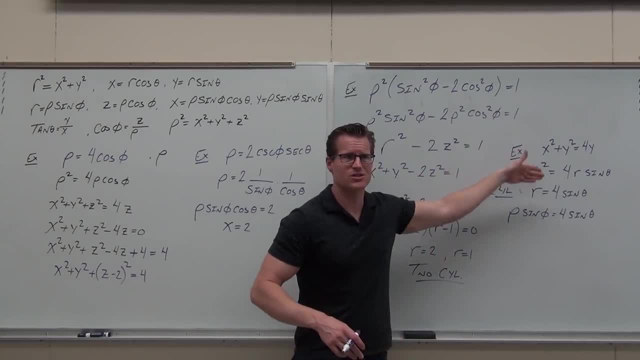 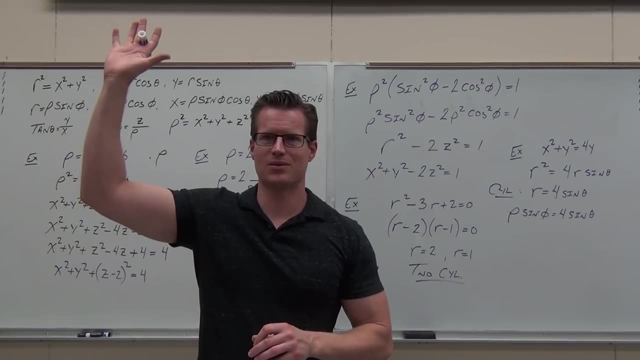 have. It's just translating into R's and Z's, R's and and rows and you know other stuff. Hello, Yes, no Show of hands. feel okay with the topic. Easy, medium, hard, What do you think? 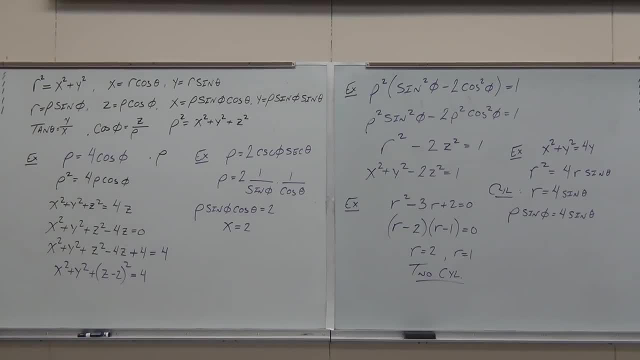